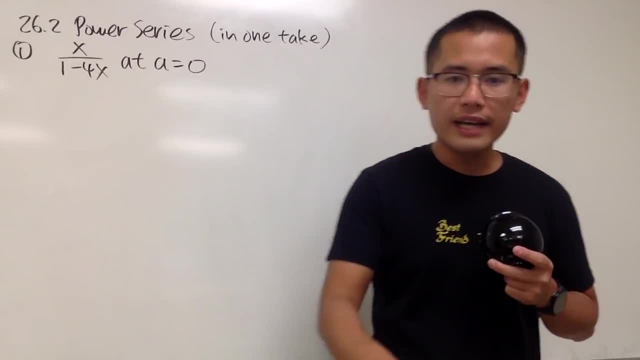 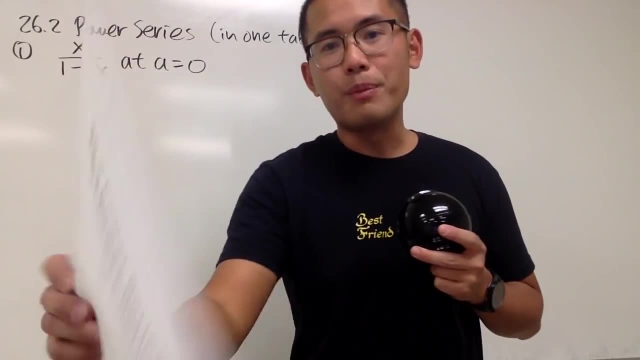 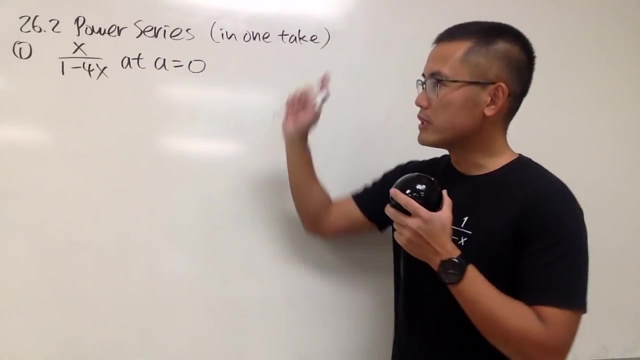 Okay, so all the things right here will be in the description for you guys, and this video is dedicated to all the students who are taking Cal 2, and also for the people who need to know about power series. Okay, so here we go. First of all, you need to know your best friend really really well. For example, the first question we have: x over 1 minus 4x. 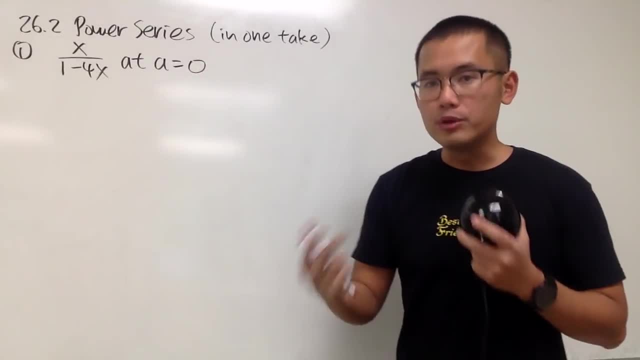 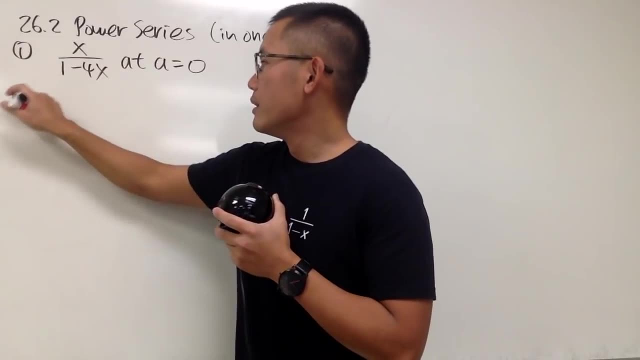 I will tell you, guys the function. right here and in the center, We will be using sigma notations to write down the power series, right? Anyway, for the best friend, for this one right, Let me just write this down: Bf. for the best friend. 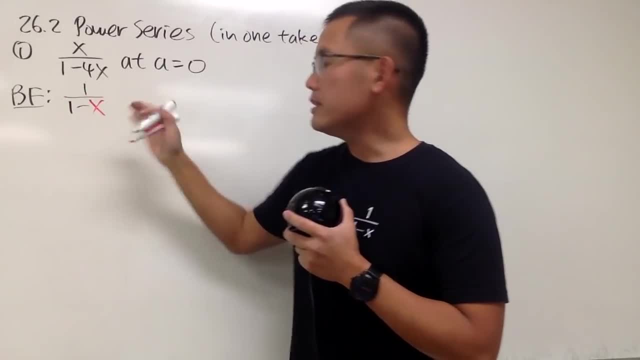 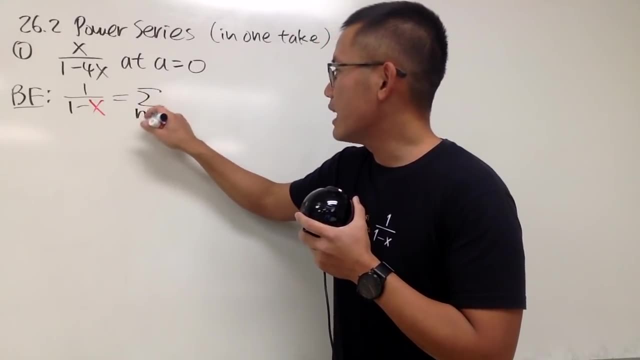 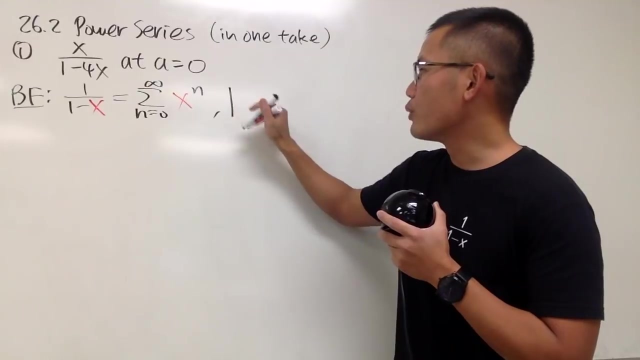 Well, 1 over 1 minus x. This is our best friend, namely the geometric series, but we like the best friend much better. This is equal to the series as n goes from 0 to infinity, x to the nth power, and this only works if the absolute value of x is less than 0.. 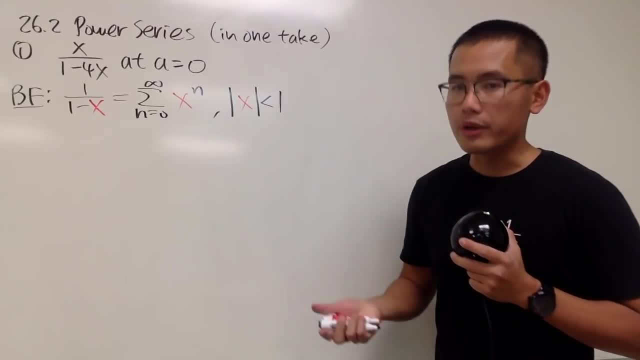 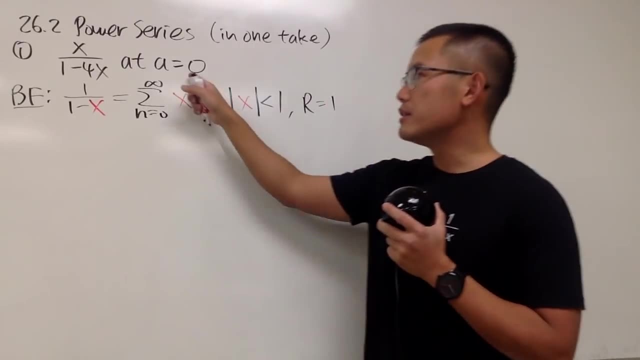 So include this inequality, because it will tell you about the radius of convergence. Based on this, we know r is equal to 1, and because the center is just 0, and r is equal to 1,, that means we can move to the left and also the right, one unit in each direction. 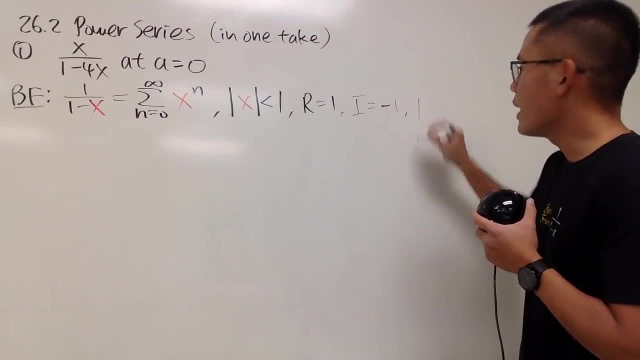 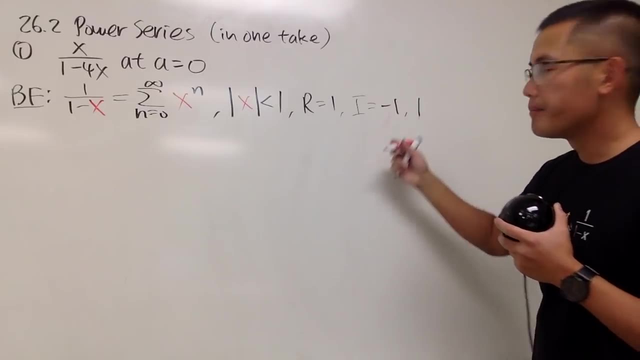 So we know the interval of convergence will be going from negative 1 to 1, and you also have to remember that, for the best friend, at the endpoints of we have 2.. Very interesting. That is why we shouldn't Thorin in here. Okay, now we do call for the best friend to write down the data. Okay, so this is ourProcess мощnplider term and, anyway, this is ourProcess Messiah capacitor real time, and let's sprout it for the rest of the-or. we also have to remember that for the best friend, at the endpoints of the i, we are saying your good friend, 7 over 20.. 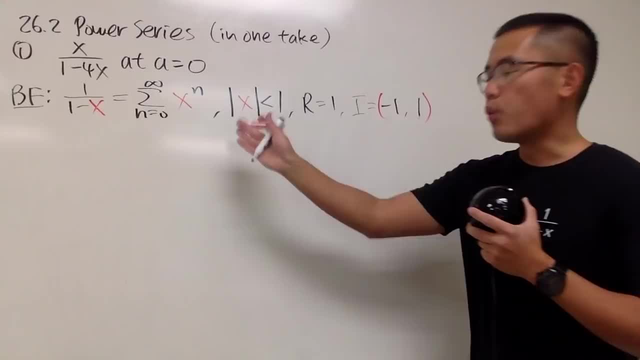 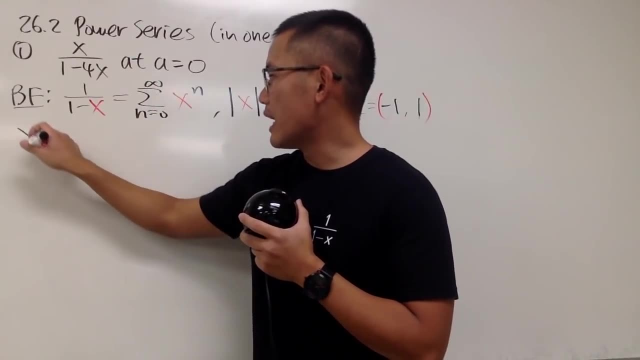 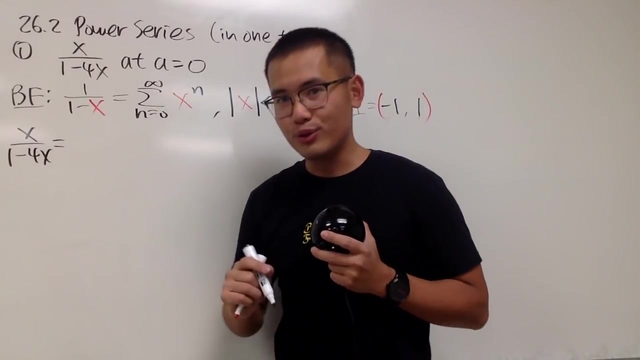 we do not include the endpoints because it won't converge. and Let's take a look of how to do this one. Here we go. I will recommend you guys to write it down right here: x over 1 minus 4x. And now we see that, in order for us to use our best friend, 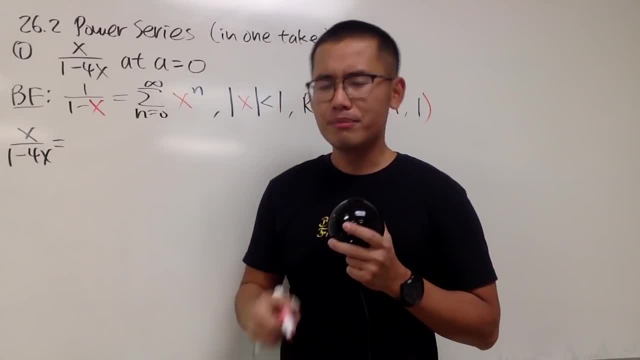 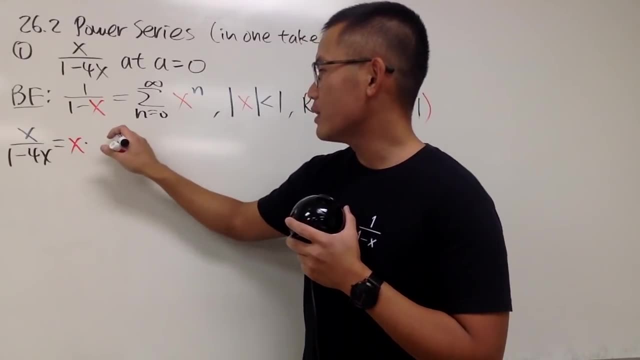 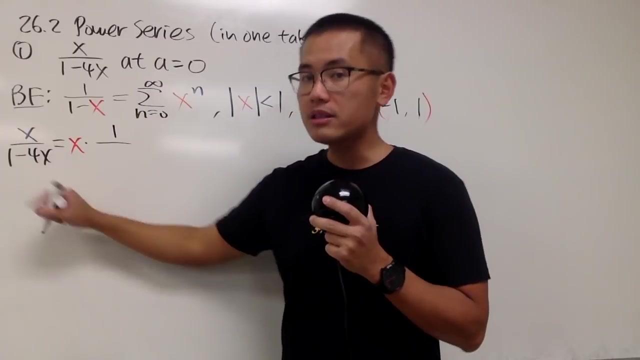 We need to have a 1 on the top, but this is an x. not so good, But it's okay because we can just put the x in the front, like so then we can just look at this as times 1 over and Notice that for the best friend, We must have 1 minus and this is 1 minus, so that's perfect. 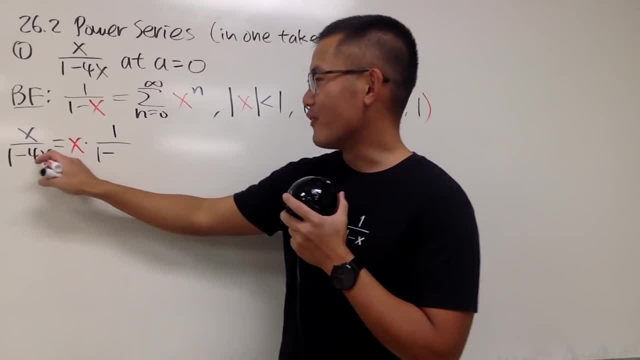 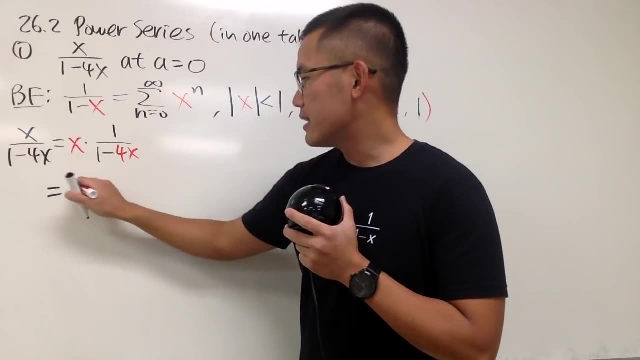 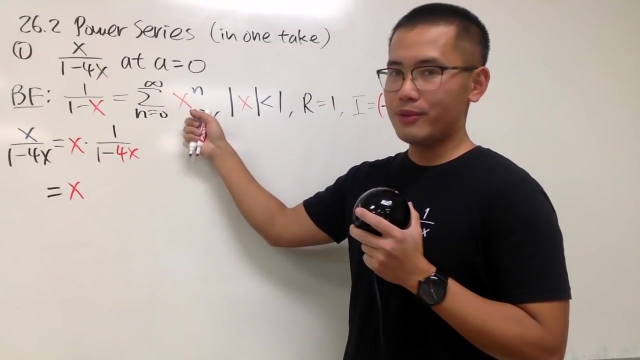 we have the 4 that we want, and This right here is just a 4x, and in fact that will be our new input. Now let me show you This: x stays in the front, but 1 over 1 minus 4x. We can just enter the 4x right here because 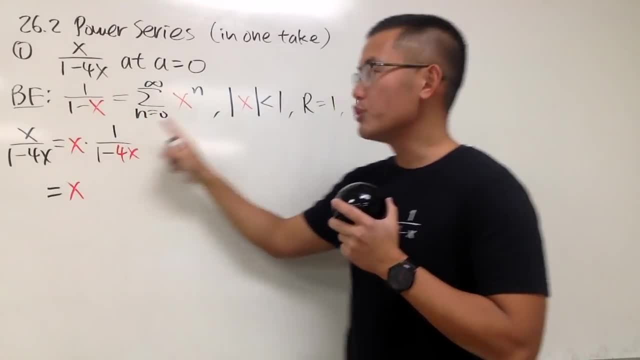 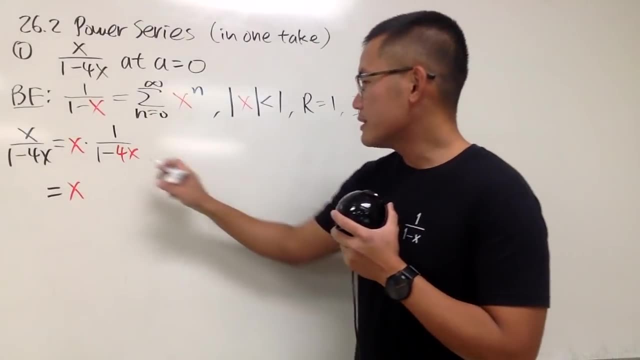 You see, the best friend is 1 over 1 minus 5 for the input. you have just put it here. We can do the same right here, and we're can just do some algebra on this right. So let's see, this is going to give us the series as n goes from 0 to infinity. 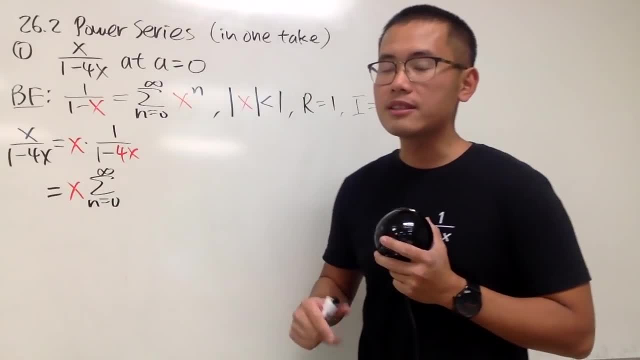 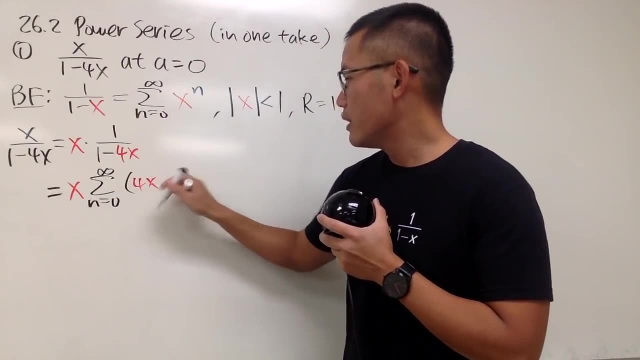 and, by the way, I may say this as a series or I may also say this as a sum. they are interchangeable, right? anyway, you put 4x in here, open the parentheses and Raise to the end power, and don't forget to put the 4x in here. 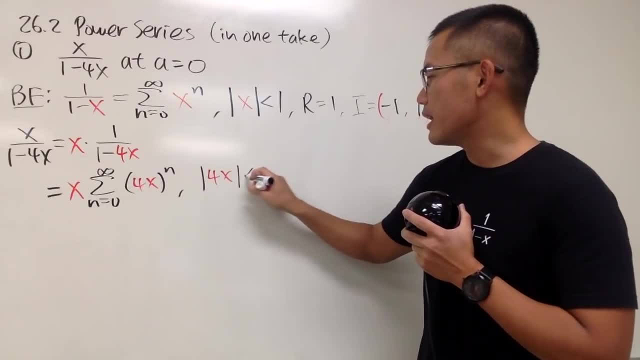 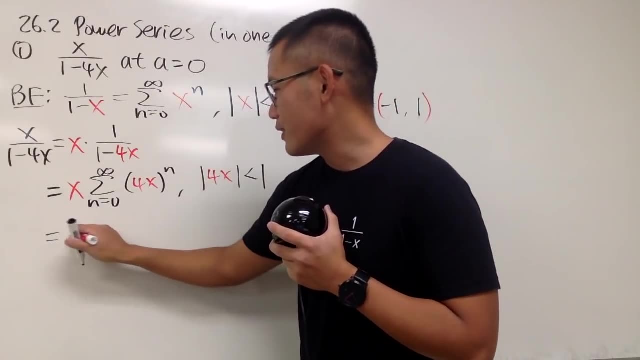 So we have the absolute value of 4x, that has to be less than 1, like this. Then we're just going to fix this pretty quick, that's all. So we have the x in the front, and this is just a series, as n goes from 0 to infinity. 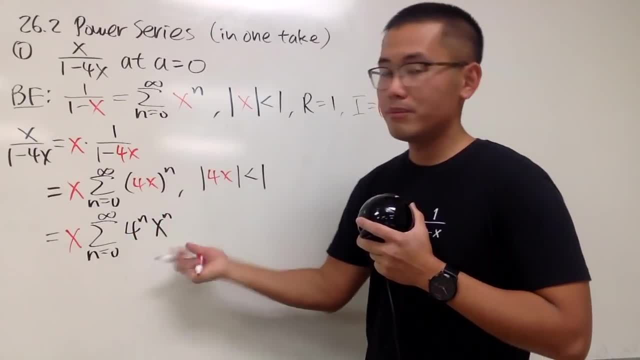 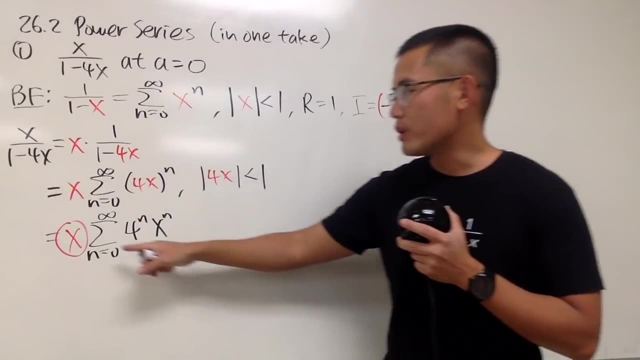 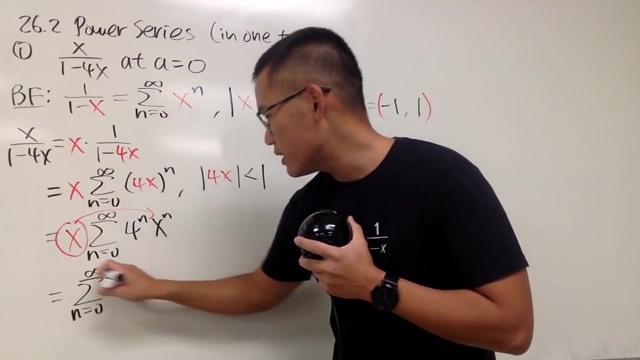 4 to the nth power, times x to the nth power. yeah, And in the end this is x. and don't forget that this, right here, is an infinite polynomial and we can just distribute the x right here. So in the end we get the series as n goes from 0 to infinity. 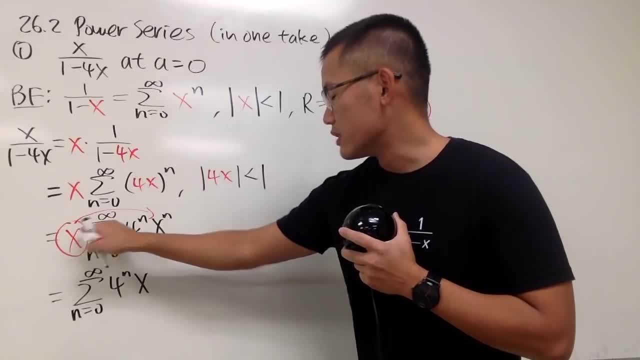 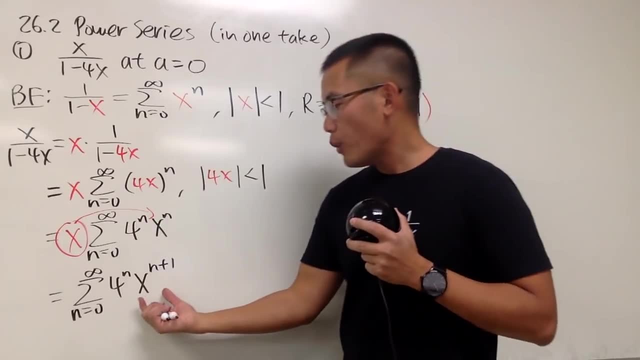 and this is 4 to the nth and this is x to the. this is the first power and this is nth power. so you just add the exponents and that's the form that we have. And I will also recommend you guys always try to put the x to some power at the end, like this: 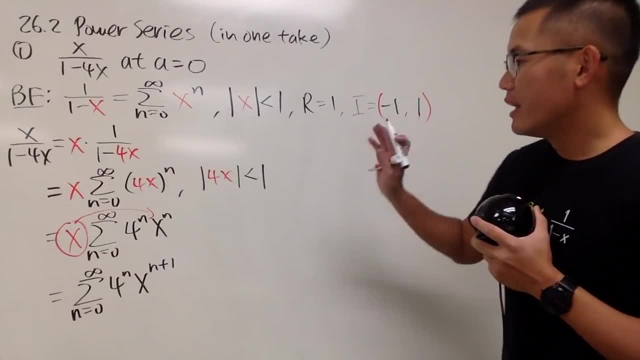 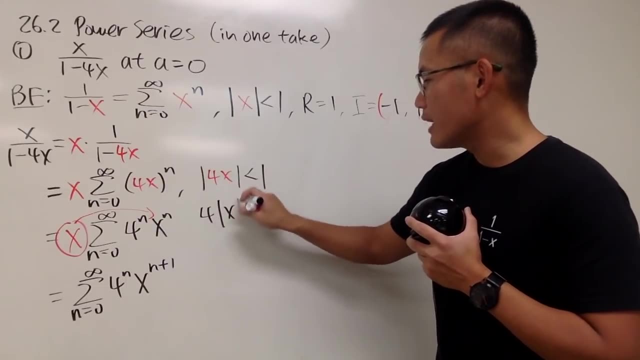 and have the coefficient right here. okay, Then look at this. We have to simplify this a little bit. Absolute value of 4x is the same as 4 times absolute value of 4x. It's less than 1, like this: 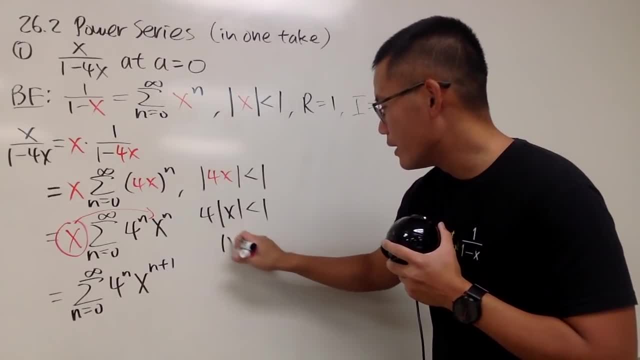 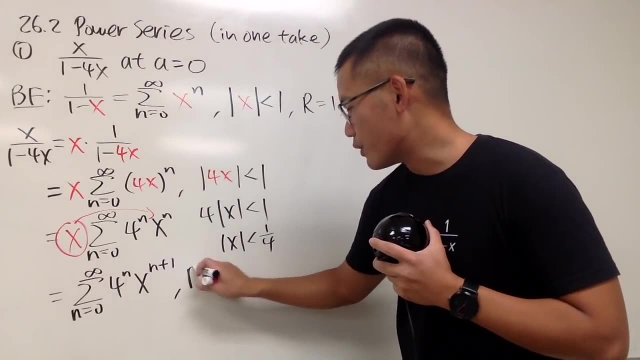 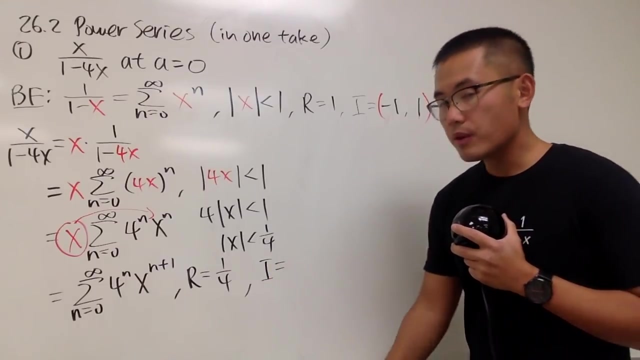 Divide both sides by 4, we get absolute value of x is less than 1 over 4.. With this being done, we know that the radius of convergence is just 1 over 4, and then the interval of convergence is going to be well. from 0, we move to the left and also move to the right. 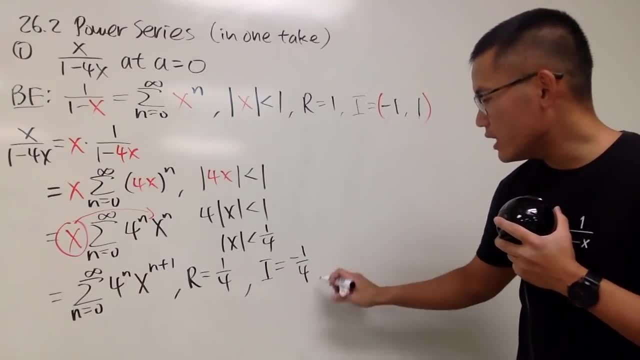 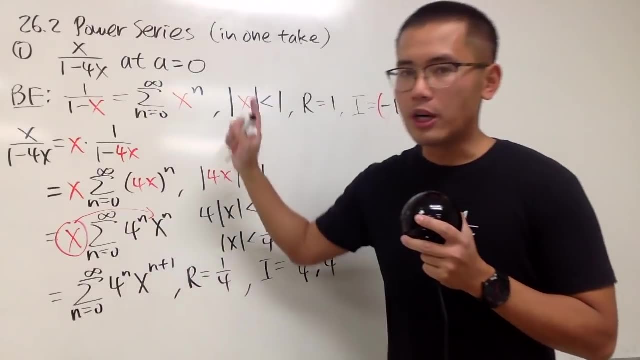 1 over 4 units each time. So we have 1 over 4 negative and 1 over 4 positive. And now pay attention, Pay close attention to this. Notice how we just did algebra with our best friend and end up with this right. 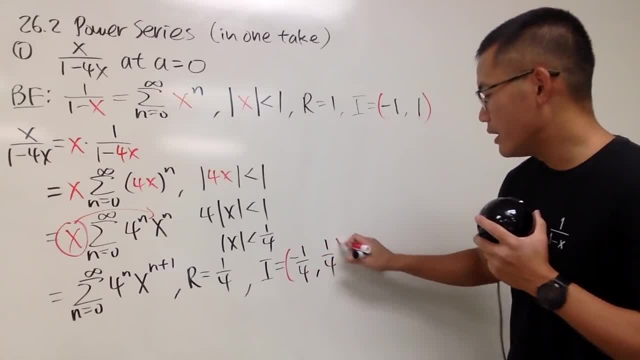 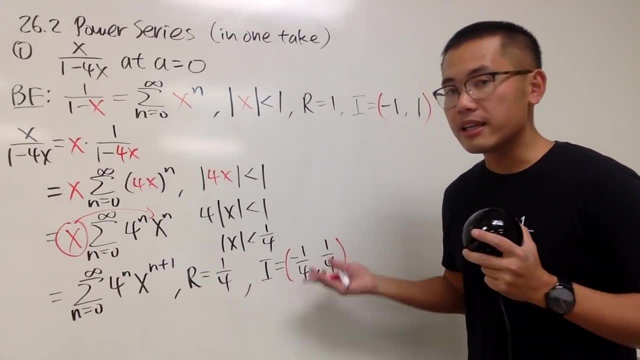 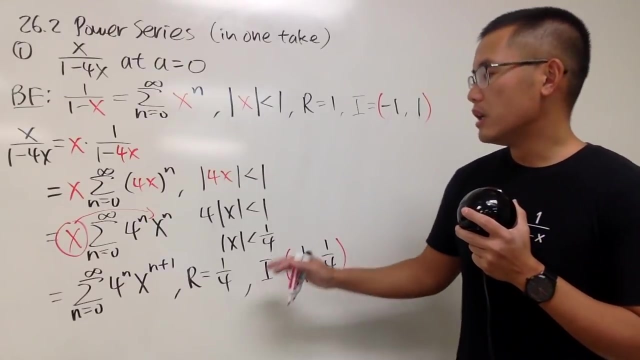 In that case we also do not include the endpoints of the interval of convergence. So this and that, maintain parentheses right, Maintain to be open like this. Only later on, when we are doing like integrations or maybe differentiations, we really have to be careful with the endpoints of the i by. if you're just doing algebra. 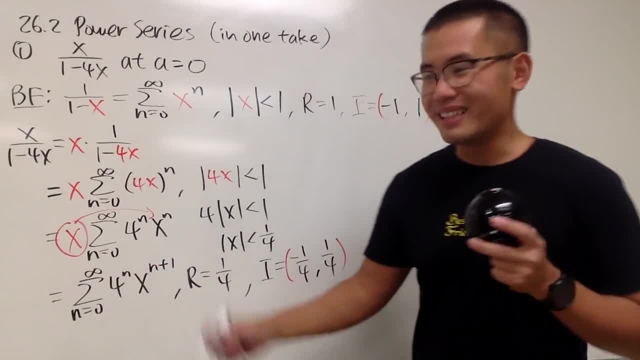 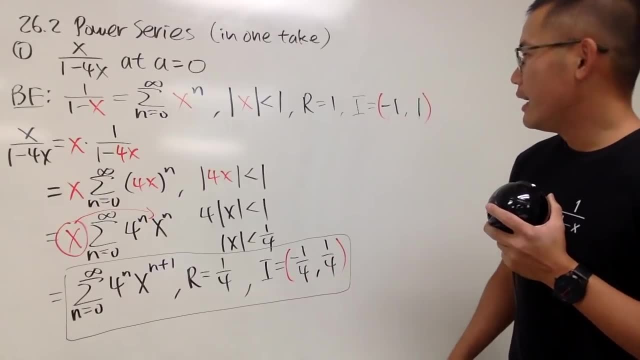 it stays the same kind, Right? So this is it. It wasn't so bad, isn't it? Told you, best friend will help us out tremendously, Right? That's the first one, And let's see, I'm just going to save some space, so I'll just write this down here. 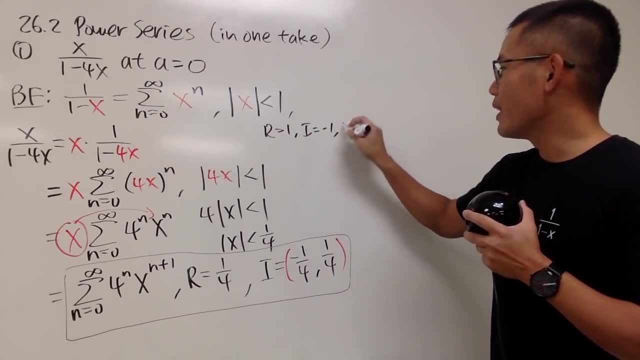 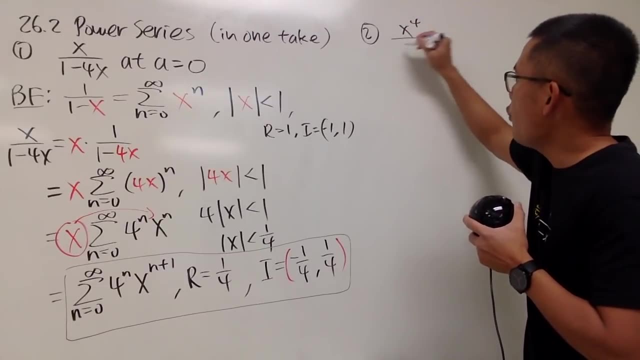 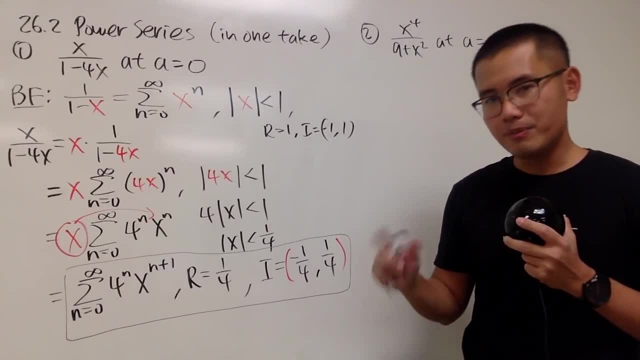 We have x to the fourth, power over 9 plus x squared, and we want the center to be at a equal to 0.. Later on we'll see what if we have a different center, It might be more bizarre, but for now just say 0.. 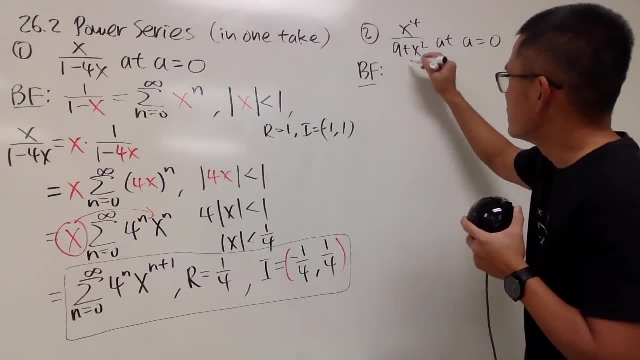 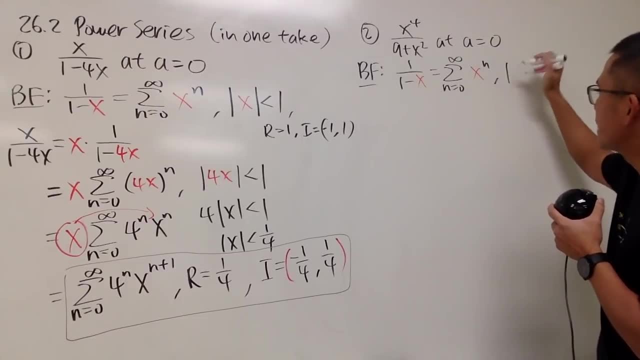 Okay, here we go. Of course, let's write down our best friend first. This is 1 over 1 minus x, and this is the sum as n goes from 0 to infinity, x to the nth power. absolute value of x is less than 1.. 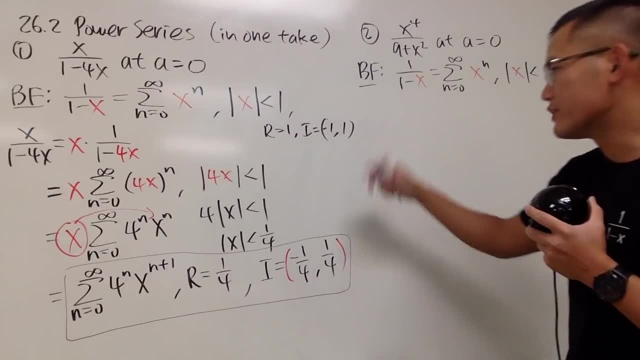 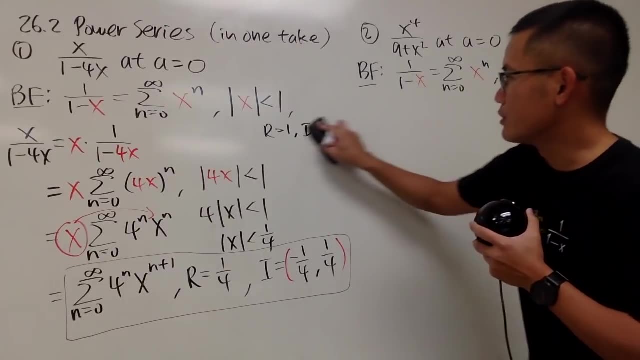 And just keep this in mind. I'm not going to write this down anymore- for the best friend r is 1, and this is the i. Now, this is what we have. Now, this is what we have. Let me just erase this so I have more space, right. 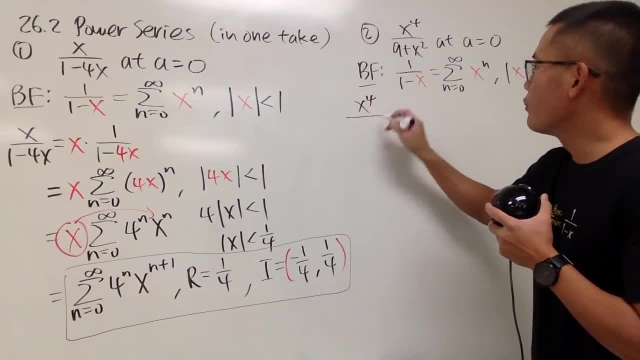 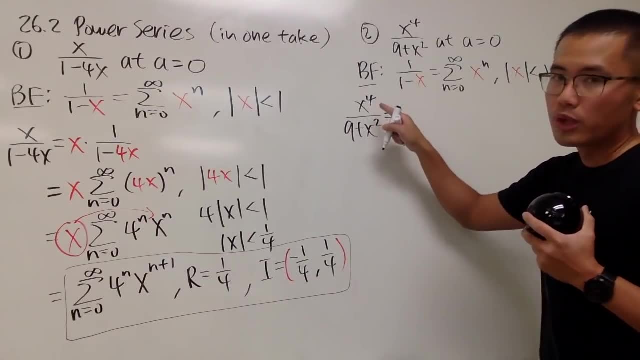 Okay, this is what we have. We have x to the fourth power over 9 plus x squared. We will be doing the similar thing First of all. this is x to the fourth power. We don't like it, It's okay. 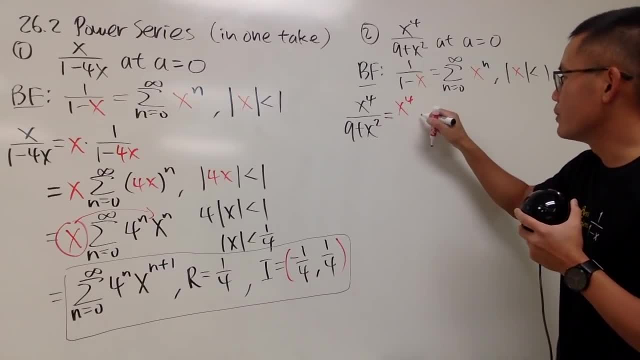 Let me just put it on the side x to the fourth power, so we can look at it like x to the fourth power, times 1.. Now on the bottom we want to have a 1, but this is a 9.. 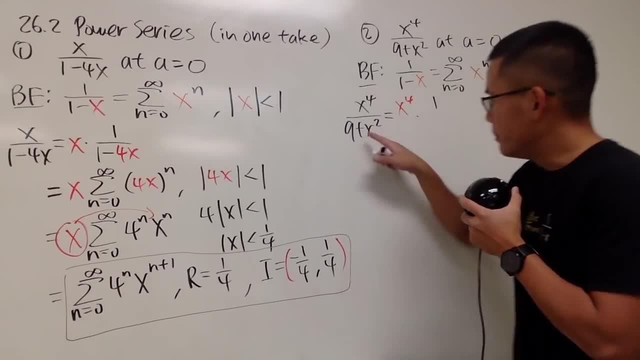 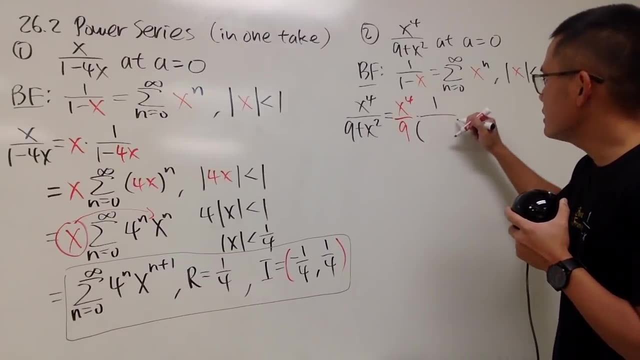 Not so good, but don't worry, Small fix right, Because look at this and that we can just factor a 9.. So I will write it down as this: over 9, and then put down a parentheses like this: 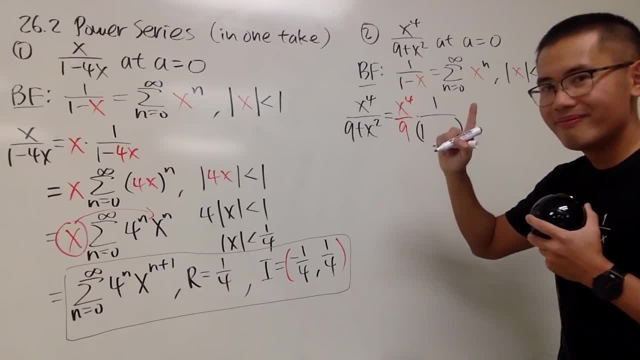 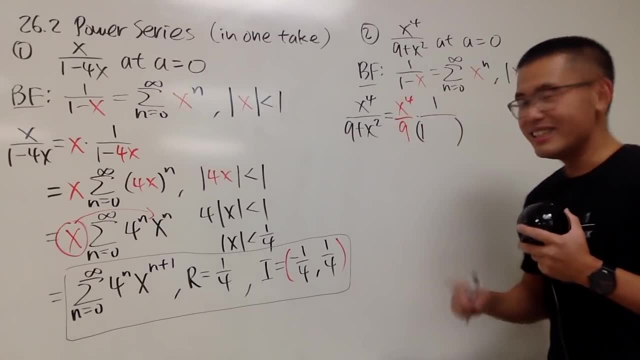 Originally we had a 9.. We factored the l, so we have a 1.. Well, this right here is a plus, but in order for us to use our best friend, we have to have a minus. It's okay, though, because a plus is the same as minus negative. 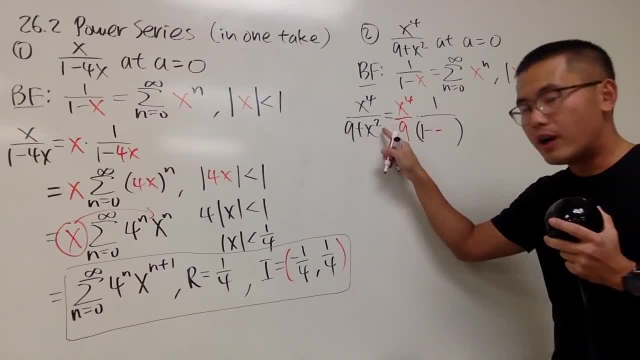 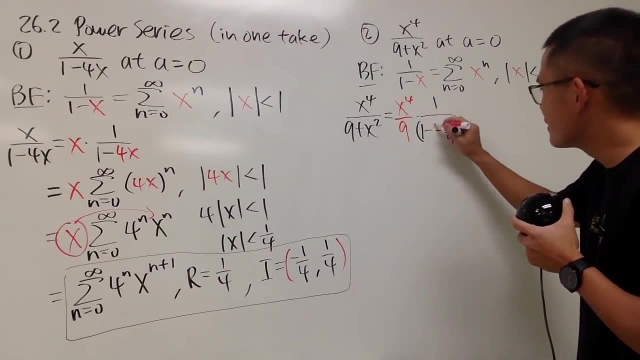 Still the same as that. Then x squared. we factored the other 9, so it's x squared. Don't forget to divide it by 9, like this, right, Very good, Let's put a little parentheses, like so: 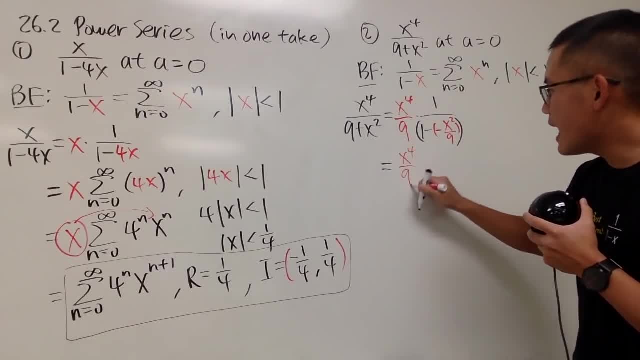 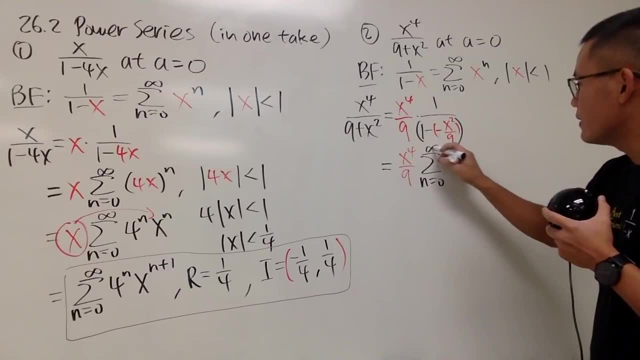 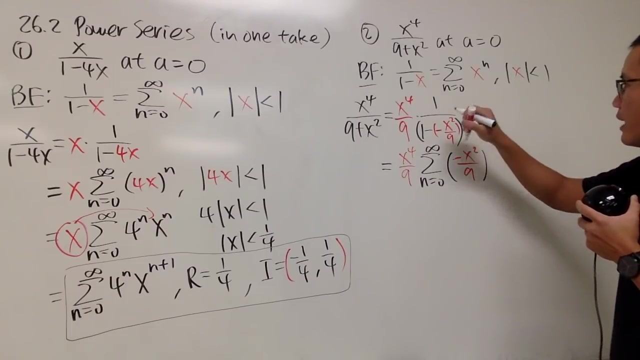 Here we will have x to the fourth power divided by 9.. Same business throwing this right here. So we have the series as n goes from 0 to infinity. Open a parentheses with negative x squared over 9, and raised to the nth power. 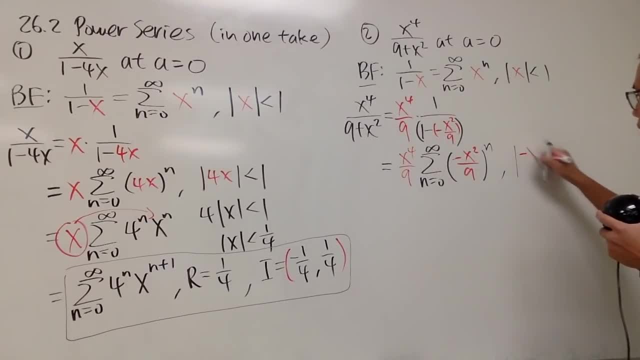 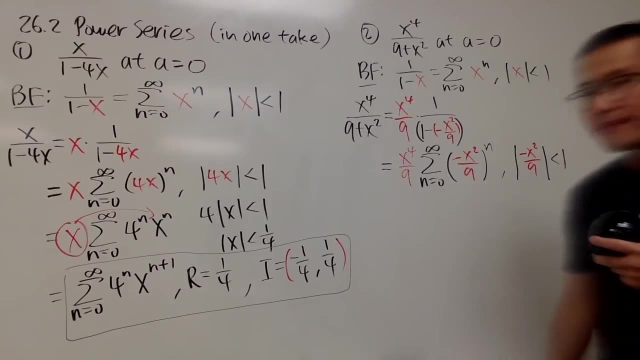 And don't forget to throw this into the output. Add the absolute value negative x squared over 9, and make this less than 1.. And now we just have to fix this real quick. This, right here, is x to the fourth power over 9,. 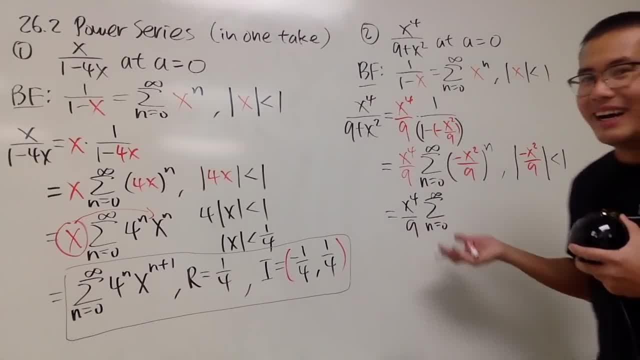 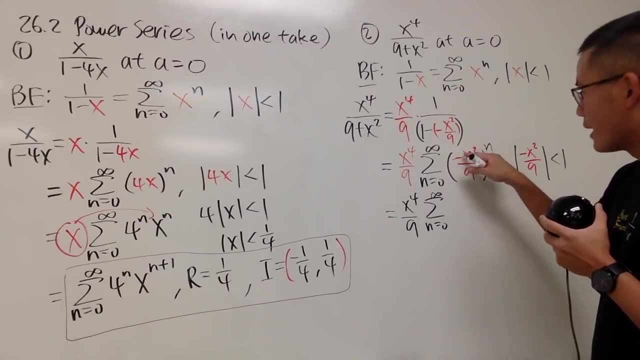 and this is the sum, as n goes from 0 to infinity. Now let's do the following: We have negative 1 to the nth power. Let's write that down first. So here we have negative 1 to the nth power. 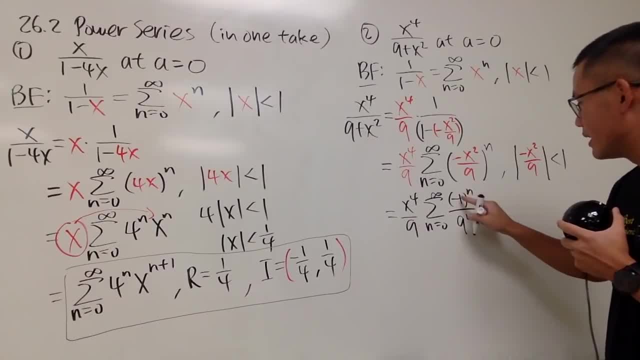 On the bottom we have 9 to the nth power, so our radius is 9 to the nth power. And then this is x squared to the nth power, so our radius is x to the 2n Yep. and then just do the algebra for that. 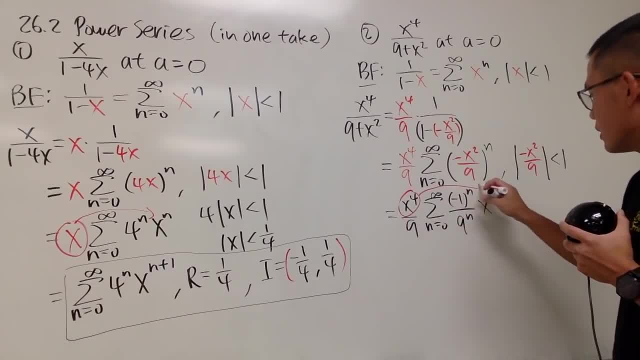 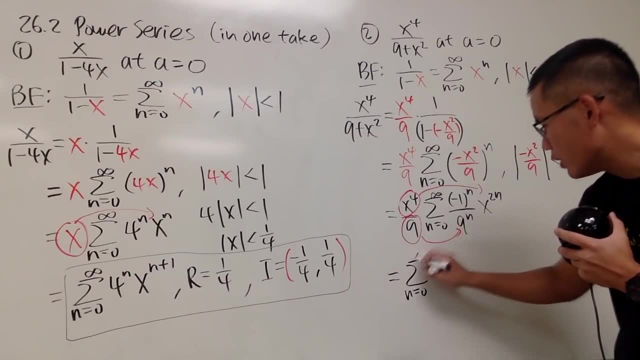 Focus on this. We will distribute the x to the 4 and also the 9.. So it looks like we have the series as n goes from 0 to infinity. This is negative 1 to the nth power over this, and that is 9,. 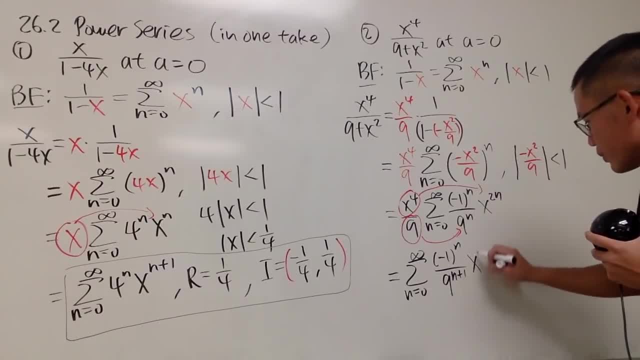 plus 1's power. This and that is x to the 2n plus 4's power, like this: Very, very nice. Okay, now just work this out real quick: Absolute value- the negative doesn't matter inside, And when you have absolute value of x squared. 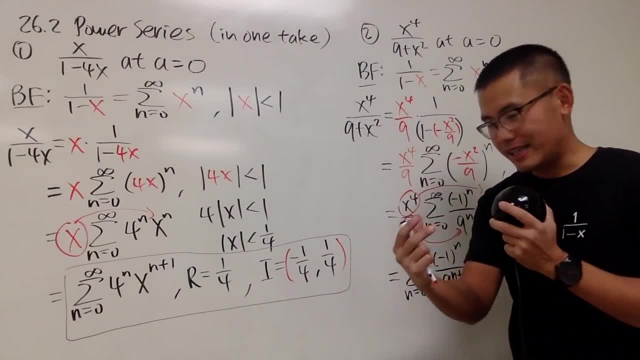 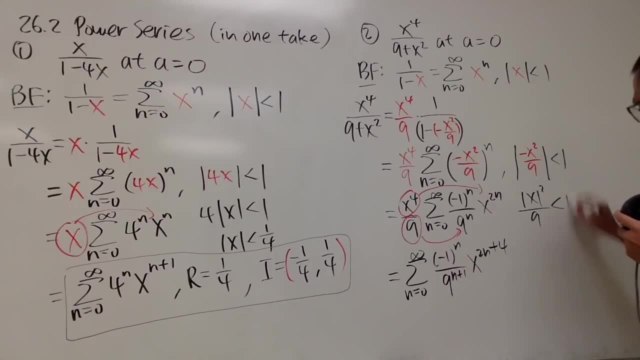 it's the same as absolute value of x and then squared on the other side, right. So this is the same as, say, absolute value of x squared over 9. It's less than 1.. Then of course, we can multiply the 9 on both sides. 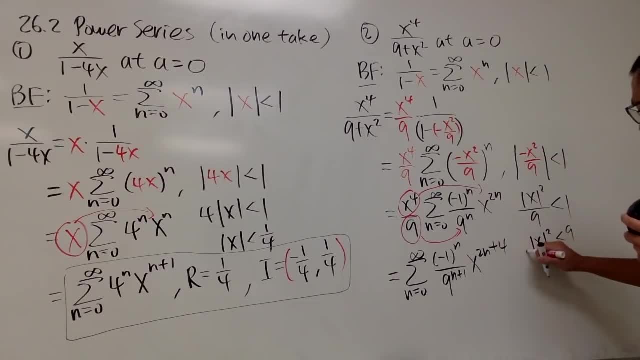 This is absolute value of x. squared is less than 9.. And then take the square root on both sides. Don't worry about the plus minus. And this is legit because the absolute value of x- this part right here- is always non-negative. 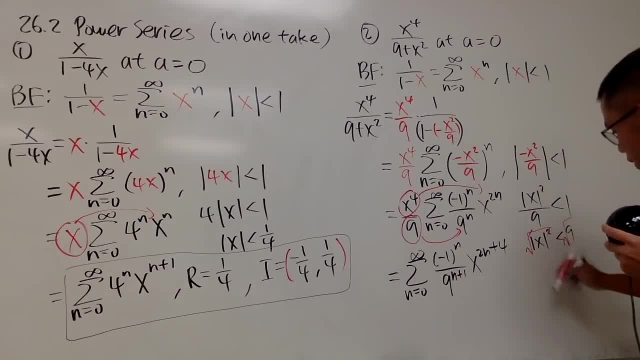 So this is good And in the end, of course, we can just isolate the absolute value of x, which is going to be less than 3.. With this being done, we know that r is equal to 3.. Okay, 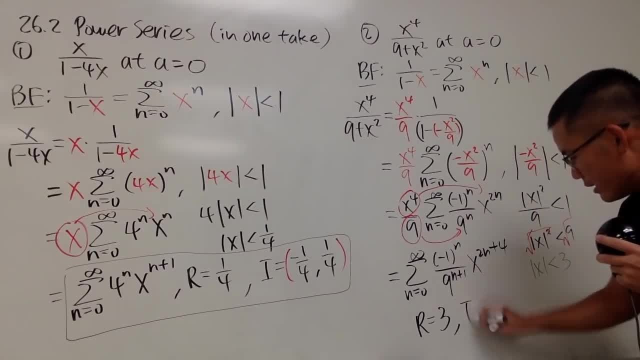 And then, because the center is at 0,, that means the i, the interval of convergence will go from negative 3 to 3.. And again, do not include the endpoints, because we just did algebra with our best friend, So this right here would be the answer for number 2.. 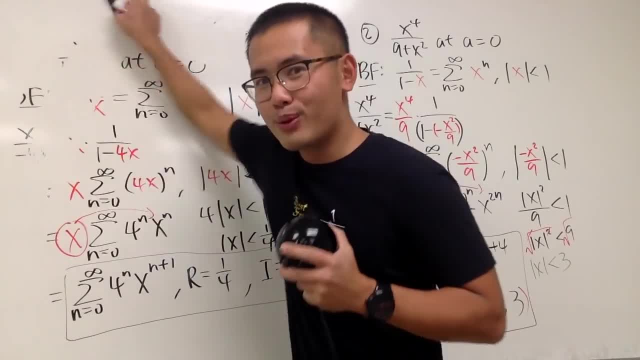 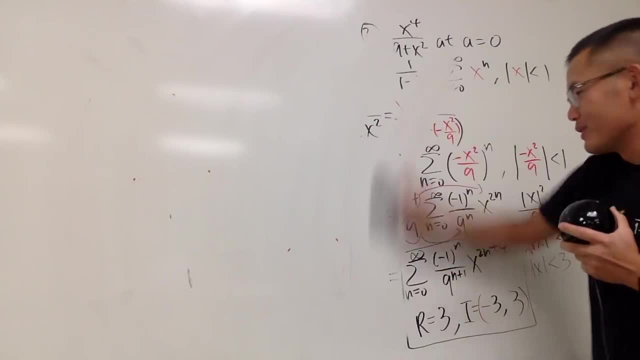 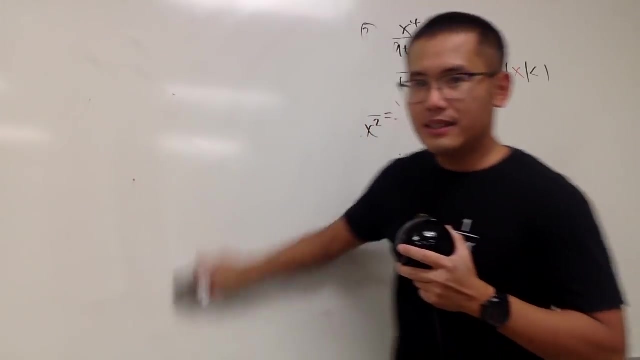 That's it, And we just have 24.2 to go. I'm sorry It's not 100 questions, but you know, I think this right here should be efficient, effective for you guys. So yeah, And I do plan to make 100 calculus 2 questions for you guys. 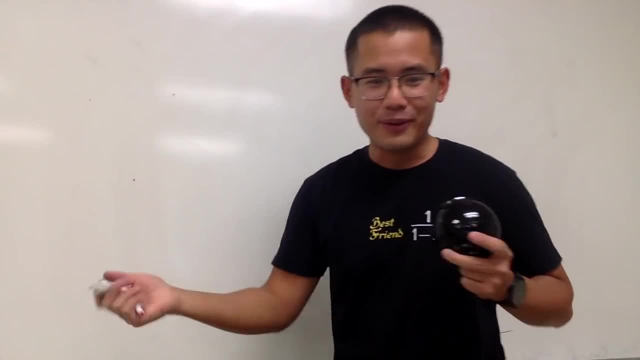 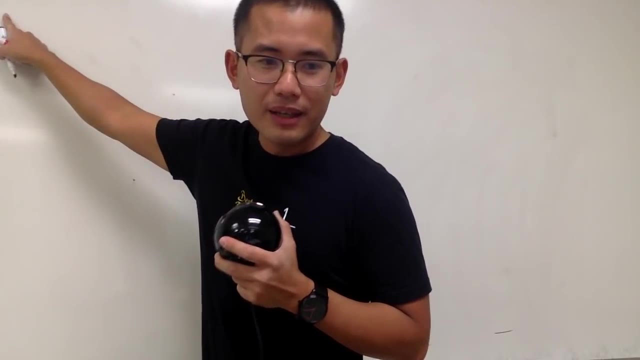 by the end of this year And, of course, by before the final exam. of course, Yeah, So you guys can expect that. I don't know when, but hopefully sometime soon in the next week or so. I should just focus instead of talking. 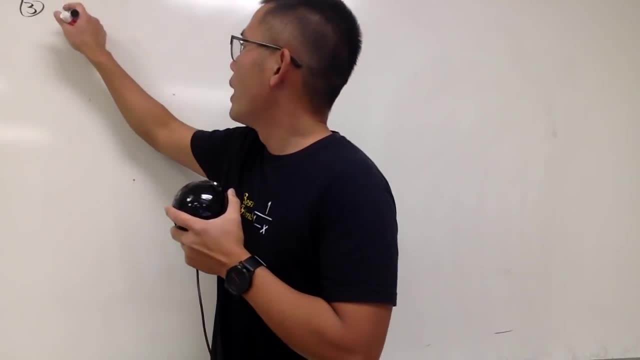 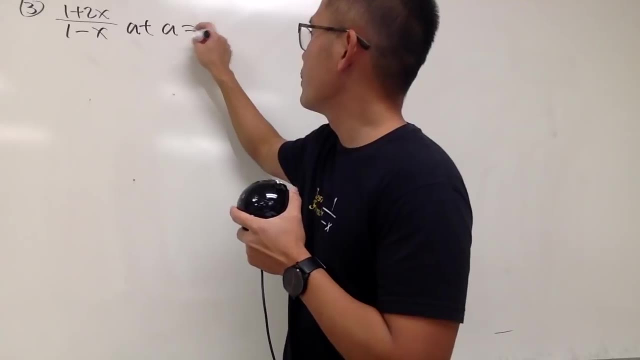 like trying to write. Okay, Number 3, we have 1 plus 2x over man, 1 plus 2x, 1 minus x at a equal to 0.. Hmm, Okay, Let's see how we can do this. 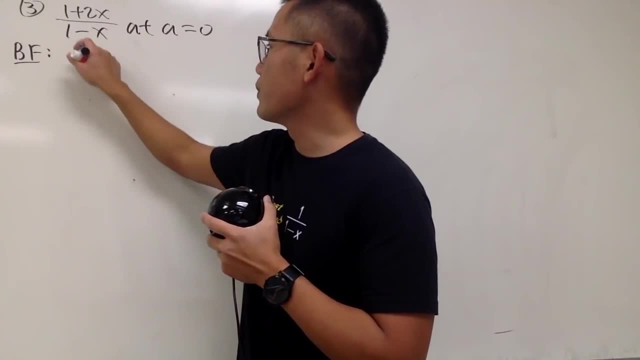 Of course, let's go ahead and put down our best friend, And I'll just write down a few more times for you guys: 1 over 1 minus x. this right here, It's the sum, as n goes from 0 to infinity. 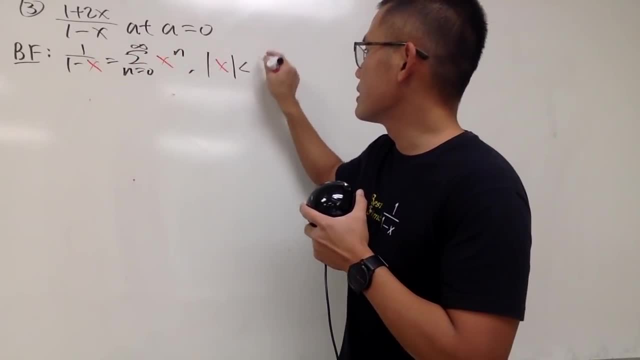 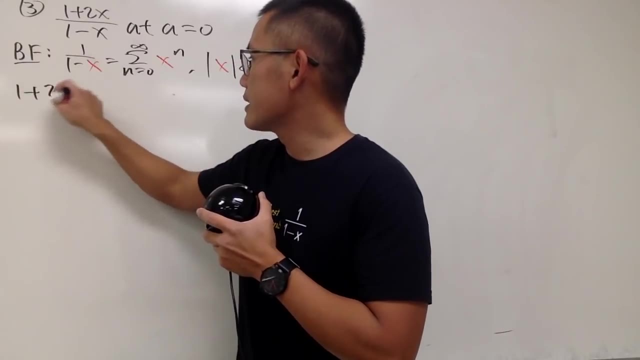 x to the nth power, and absolute value of x has to be less than 1.. Now, this, right here, is what we have. yeah, So let me just write it down: 1 plus 2x over 1 minus x. 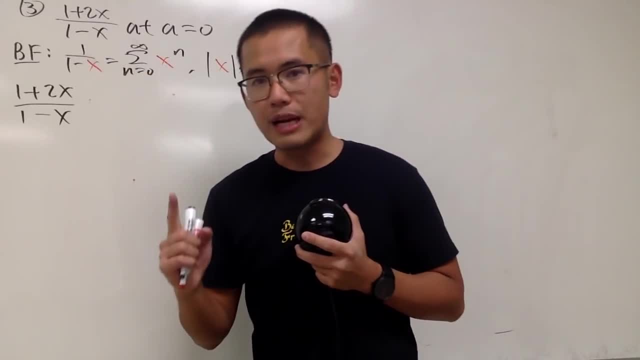 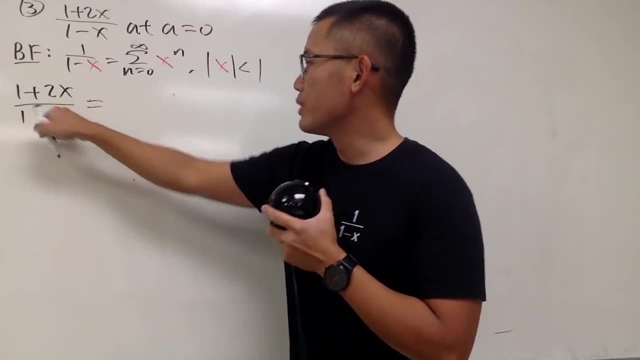 For the best friend. we only have one term on the top, namely just a 1, but we have two terms. It's okay, Just separate them right. So this right here, we can look at this as 1 over 1 minus x for the first fraction. 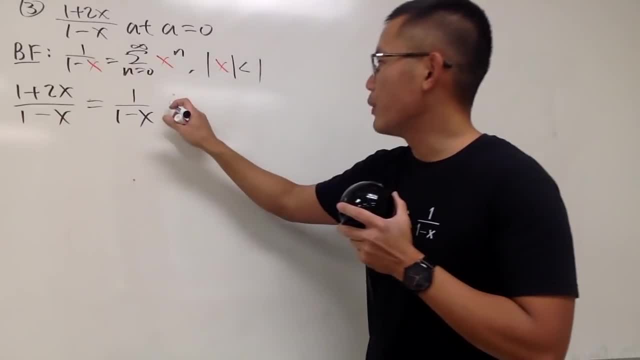 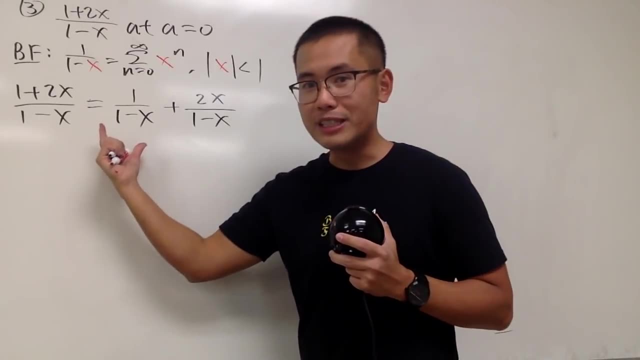 And for the second fraction, we put it as 2x over that and we add 2x over 1 minus x, Like this: Well, this is our best friend, straight off. right, This is not quite, but it's almost. 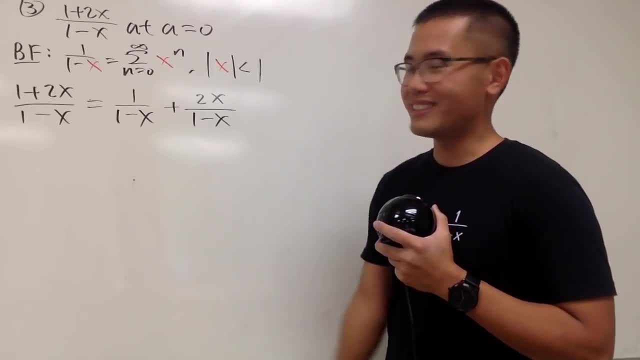 This right here is a small fix, Because you know we can just write it as 1 over 1 minus x here and plus write it as 2x times 1 over 1 minus x. Like this, Very nice. 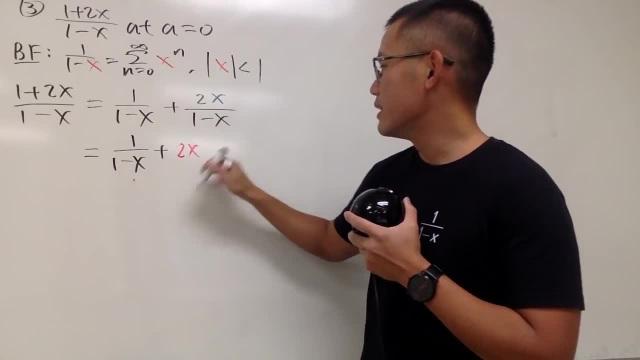 huh, Then we will see this right here- is directly our best friend. So this is the series as n goes from 0 to infinity, of x to the nth power and absolute value of x has to be less than 1.. 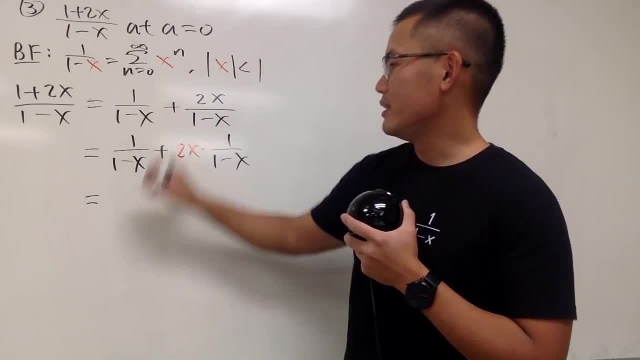 So this right here is our best friend. So this right here is our best friend. So this is the series as n goes from 0 to infinity, of x to the nth power and absolute value of x has to be less than 1.. 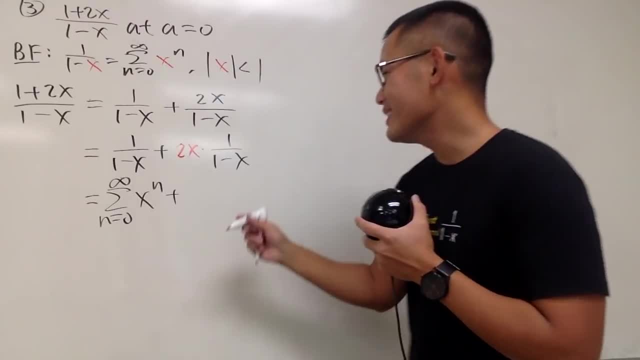 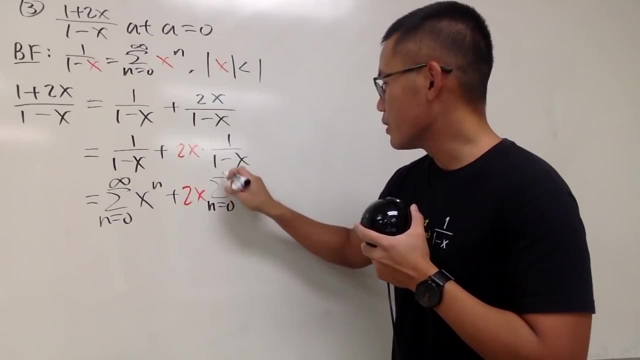 And then this is also our best friend, straight right here, right? So this is just going to be the 2x right here, and we have the series as n goes from 0 to infinity, and this is just x to the nth power. 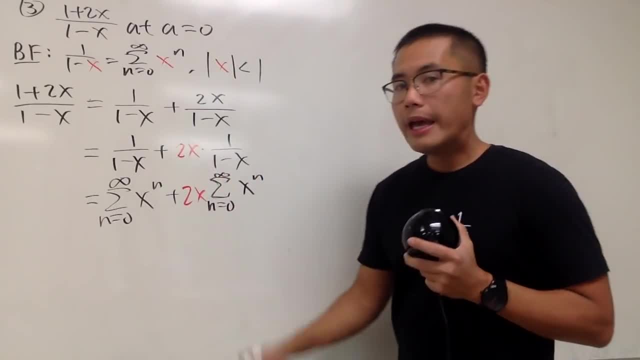 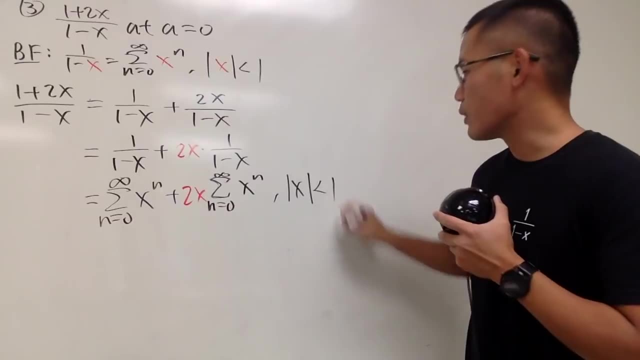 Nothing weird And because we went from here to here by using the best friend, so be sure, now we just enter: the absolute value of x is less than 1, and the input right here is just x, So so it's the same one right here. 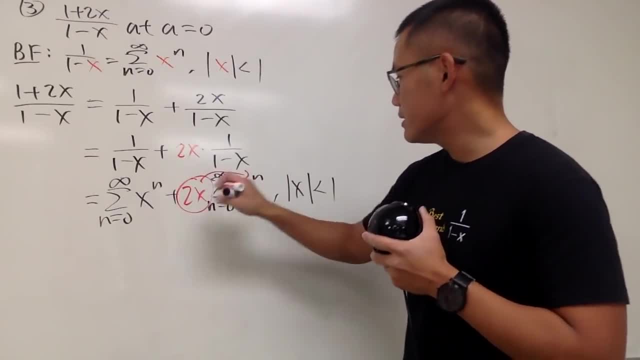 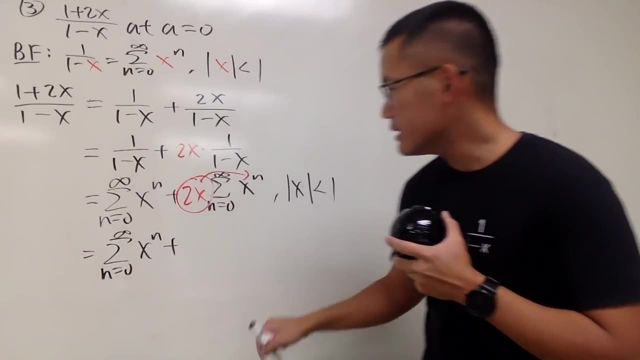 Okay, now multiply this and that, So it looks like we have the series as n goes from 0 to infinity, x to the nth power plus well, I'll write it down as the sum n goes from 0 to infinity. 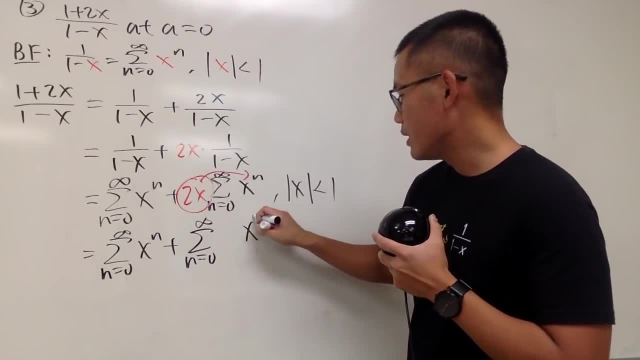 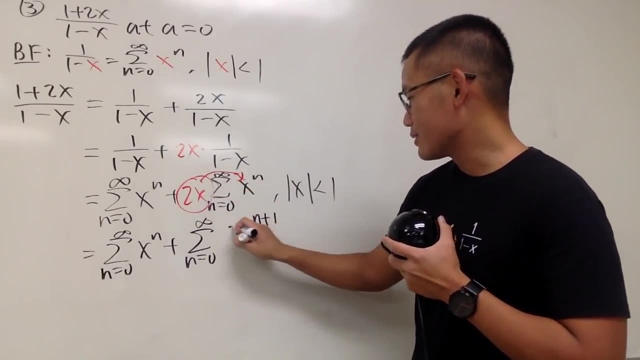 This is x to the first power, so we will have x to the n plus 1, and this is of course, just a 2.. I should have draw the arrow like this, so 2 times that's just a 2.. 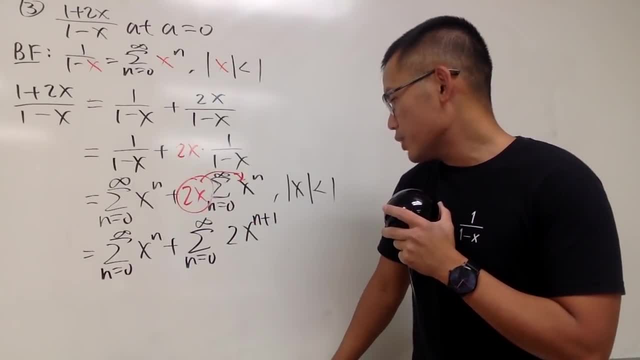 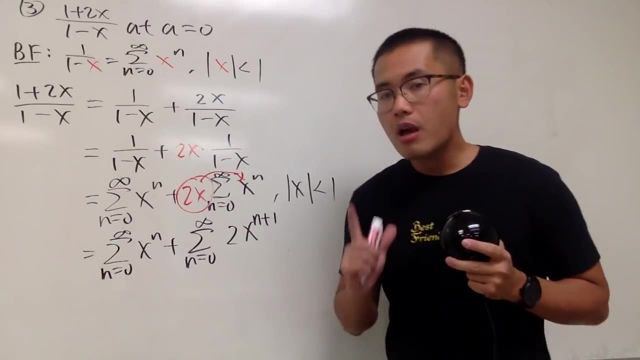 Like this: Hmm, it seems okay, but can we combine the terms? And the answer to that is yes, we can. This is how. So let me show you First thing. first, in order for you to combine anything, the power right here should match. 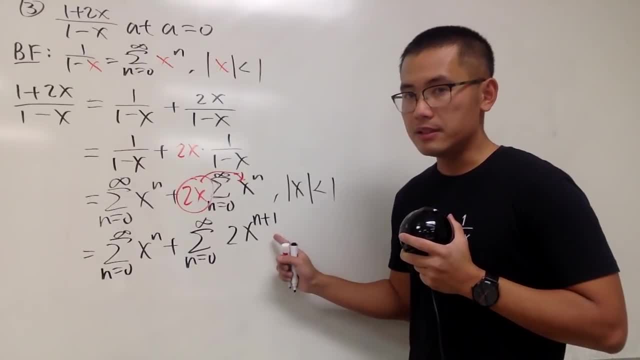 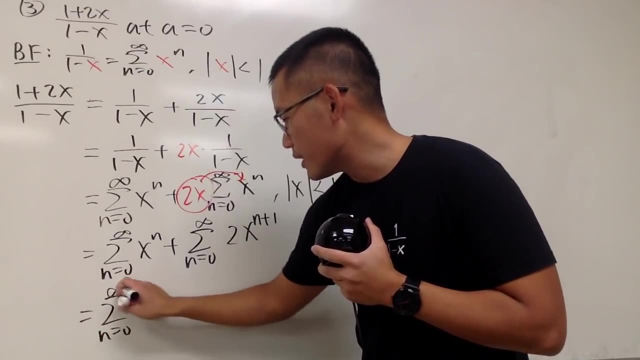 This is x to the n. this is x to the n plus 1.. This is not good. So this is what you do with this series. I will maintain the same one right here. the series as n goes from 0 to infinity. x to the nth power. 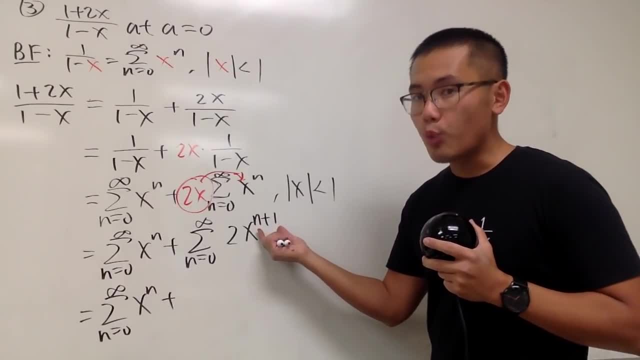 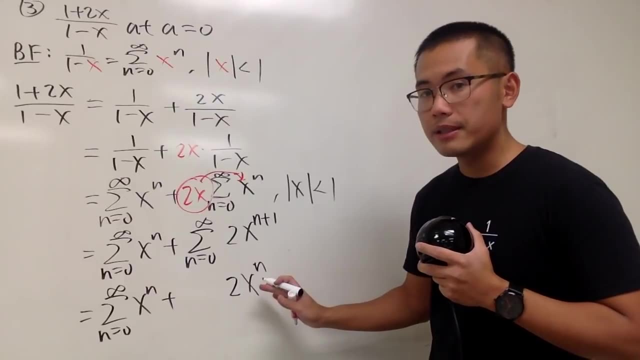 what we are going to do is we are just going to subtract 1 from the n here, so we have 2 to the x, I mean 2 times x to the nth power, only like this, But we subtract the 1, well, how can we balance this out? 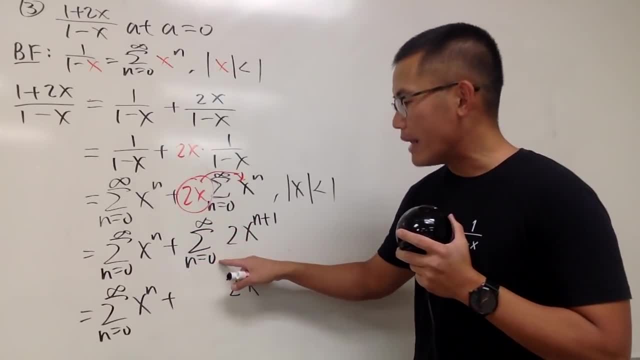 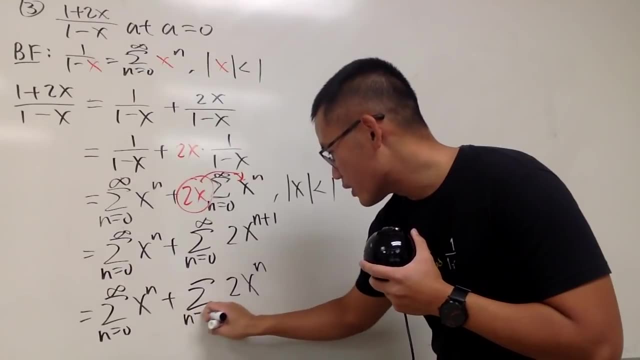 Well, just go here in the sigma notation, we add 1,, we add 1.. That's how we, you know, shift it and keep things balanced. So here we will have the sum, as n goes from 1 to infinity plus 1, still infinity. 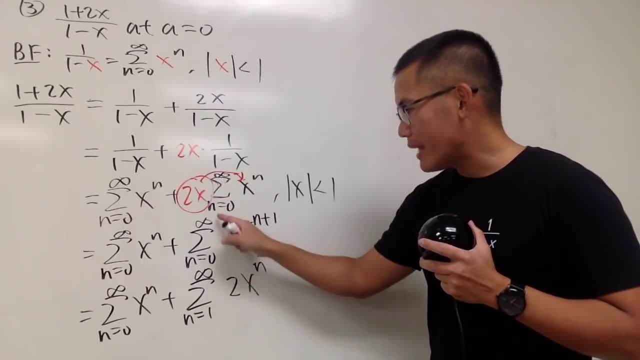 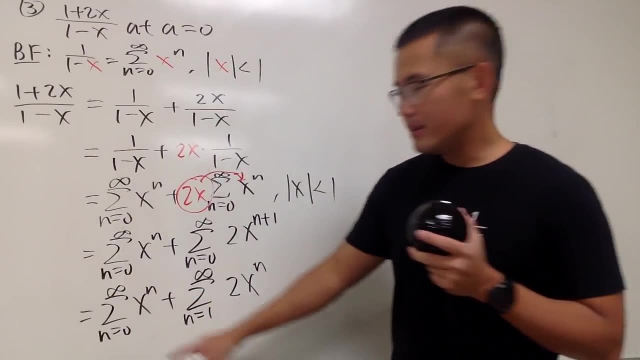 Again, Minus 1 to the n, but add 1,, add 1.. So that's what we have, And now you see that the index right. This is going from 0 to infinity. this is going from 1 to infinity. 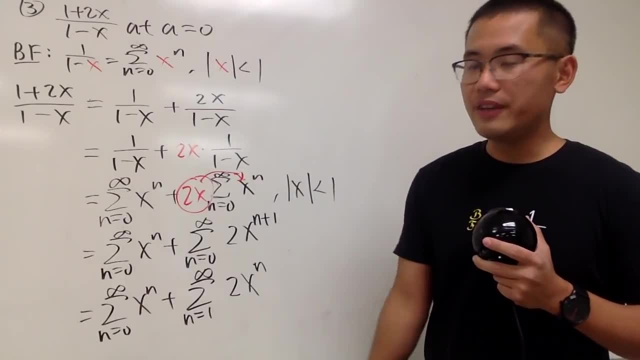 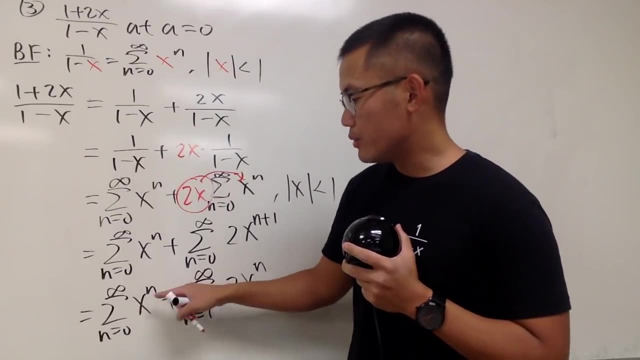 so they don't match anymore. Hmm, it's okay, Easy fix. Remember what this is. This means you put in 0, and you add, you put in 1, and you put in 2, and so on, right. 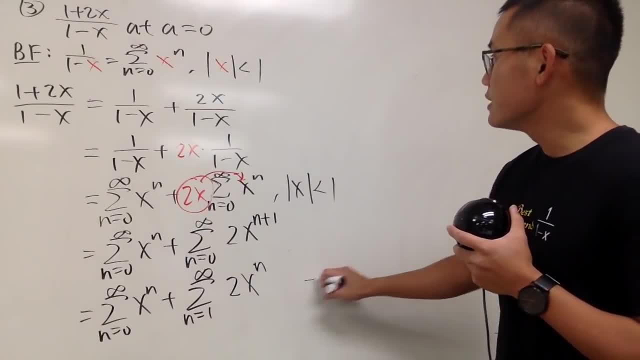 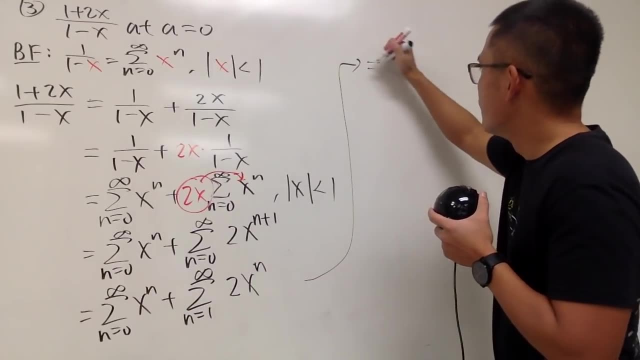 n is equal to 0,, 1,, 2,, 3, and so on. So this is what we'll do. I will just show you if we put, if we put n equal to 0,, well, that's just the first 10, so you just get 1.. 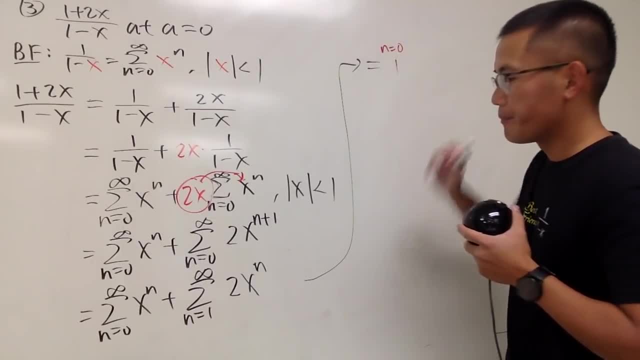 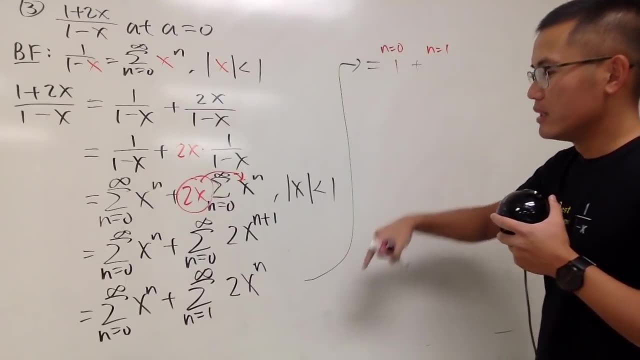 This is when n is equal to 0,. okay, Because x to the 0th power, we get 1.. And, of course, next is just when n is equal to 1, and you get x, And then to the first power, and then the next one is just put 2 in it. 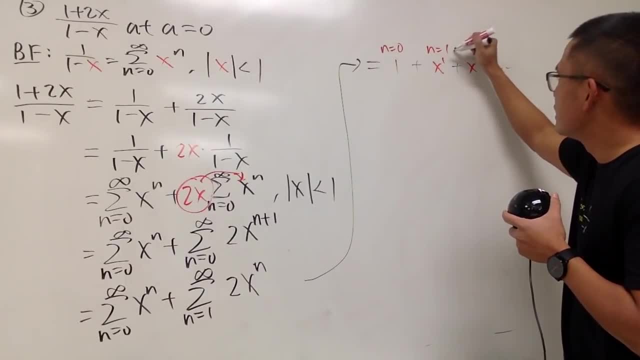 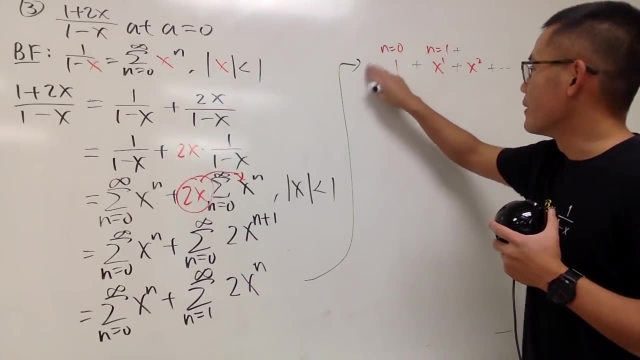 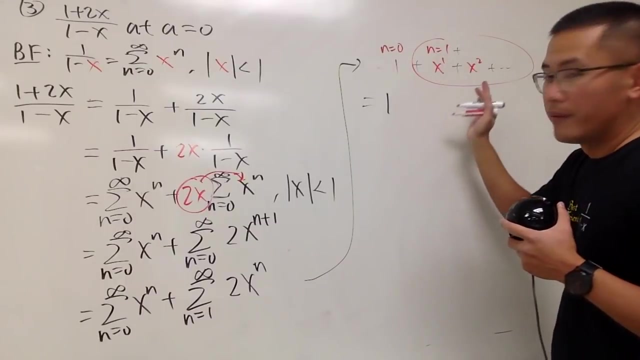 You have x squared, and so on, so on, so on. yeah, And this is what you do. You leave it right here. right, You leave this right here. This one stays, but this, this right here. you put it in the sigma notation. 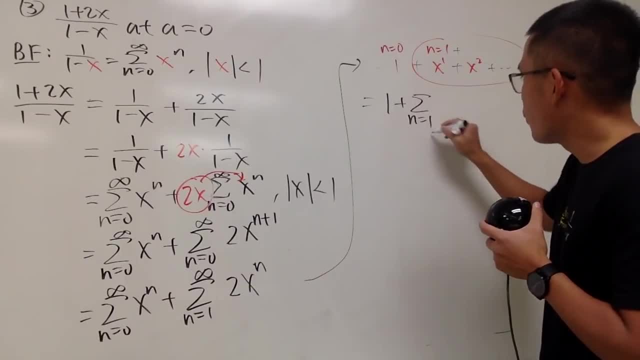 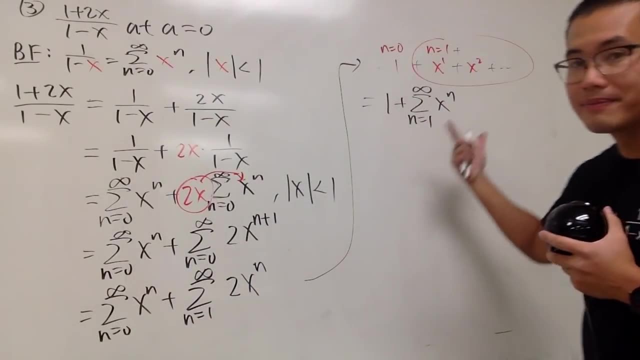 So it's going to look like the sum as n goes from 1 to infinity, x to the nth power, like this, And again, this right here is for the first part, right. I should have done that in purple, but like, let me just indicate that. 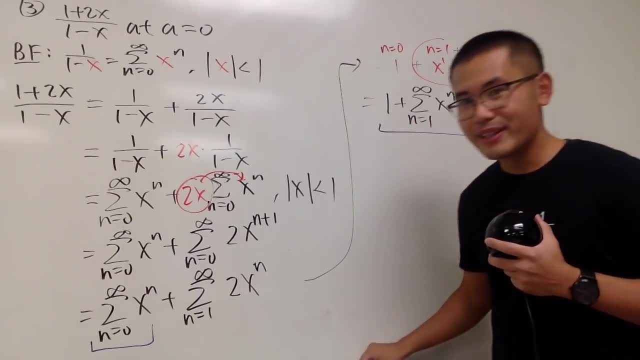 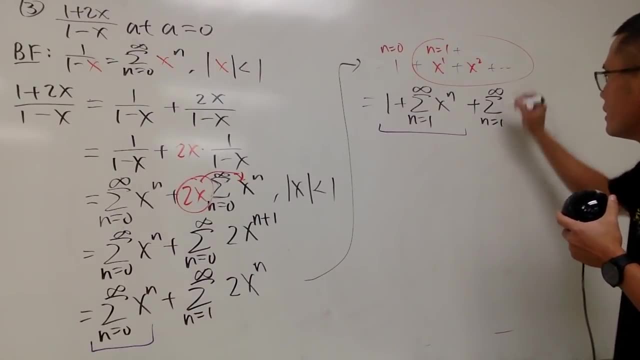 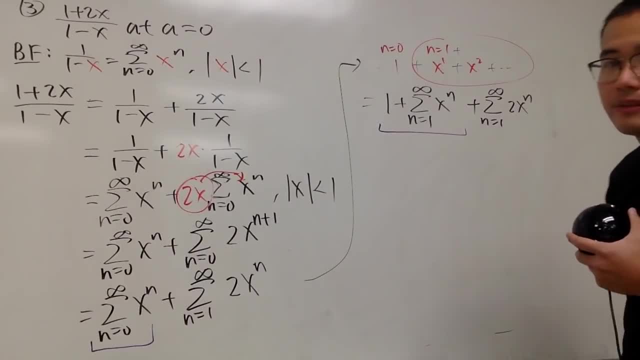 And we have the 2,, x to the nth power like this. And now, when the index 1 to infinity, 1 to infinity are the same, This is x to the n, x to the n. Of course, we can just put things together. 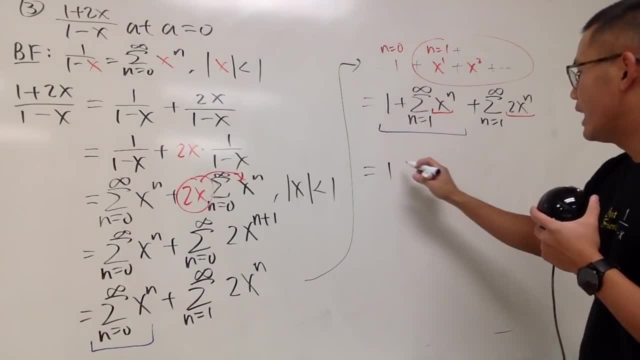 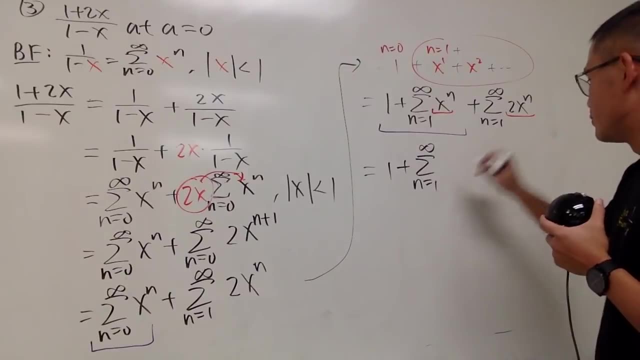 Therefore, we have the 1 all the way in the front and we have the sum, and this is the n goes from 1 to infinity. 1 plus 2 is 3, and then x to the nth power, like this: 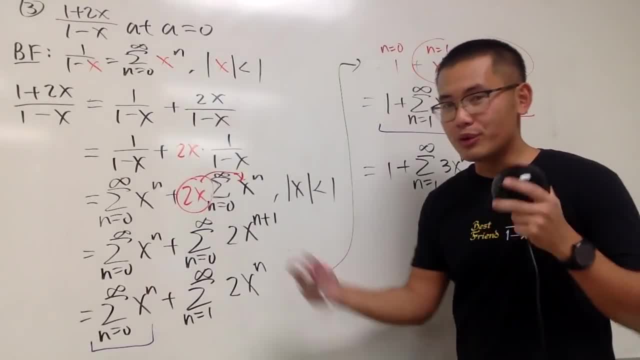 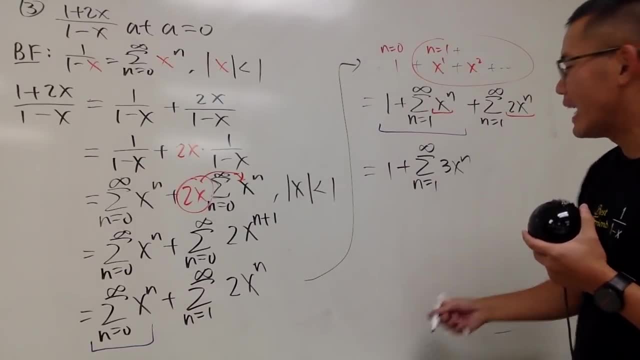 Yeah, So this right here will be the form for that, when you combine as much as possible, okay, And of course we didn't do anything weird. This is all we have. That means r is equal to 1,. 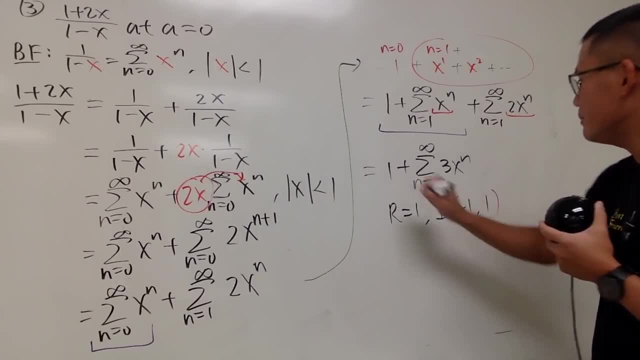 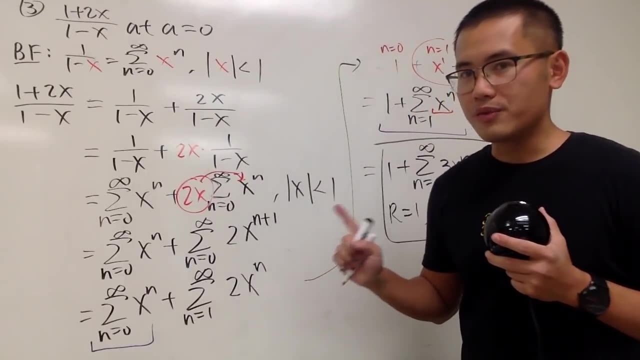 and i is negative. 1 to 1.. Do not include the endpoints, And that's it. This right here. it's actually a pretty good technique if you are doing this for differential equations, Again, you fix the power here. 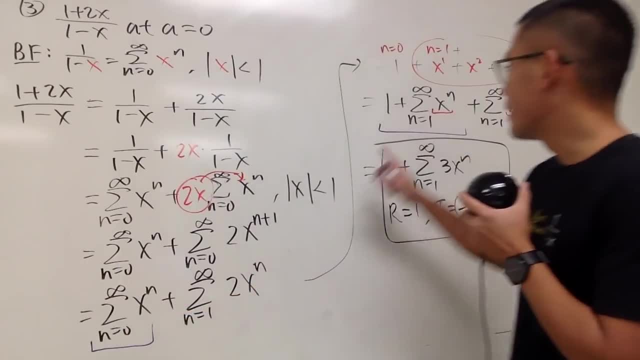 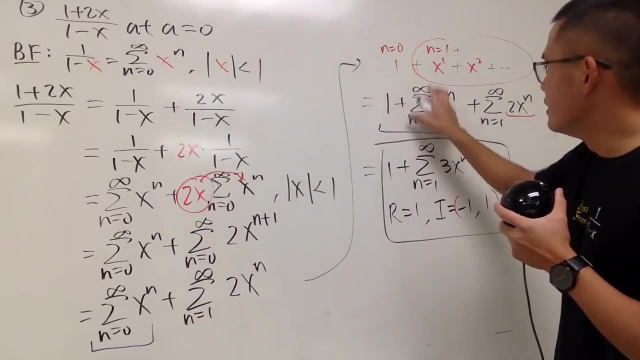 and then you are going to fix the index, And by fixing the index you just write down a few terms, You can just draw in zeros right here, And then this is just going to be from 1 to infinity, all of the same thing. 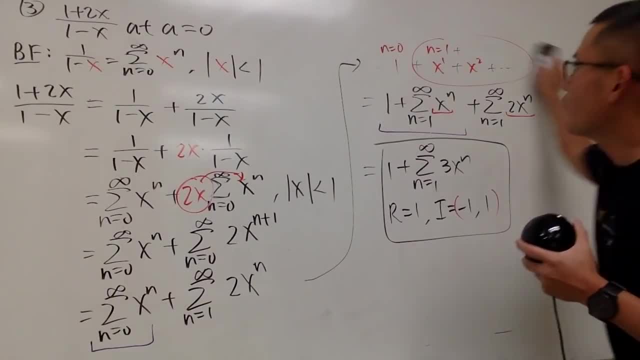 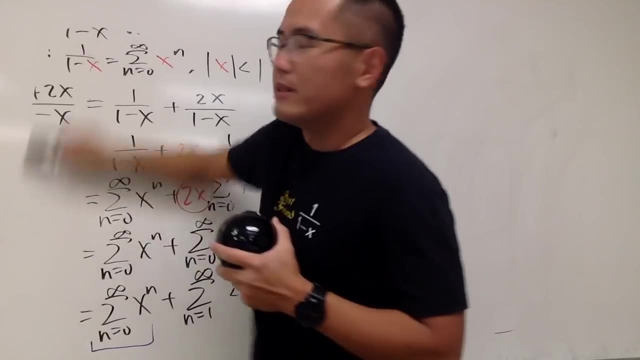 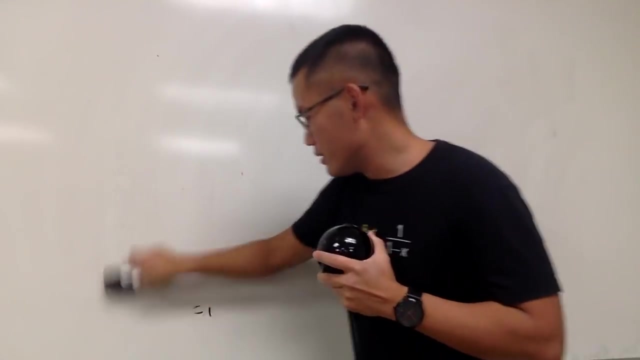 Yeah, like this. Okay, that was question number 3.. Now question number 26. already, No, Still a few more to go. I don't know how long this will take me, though, because I want to give you guys some detailed explanation. 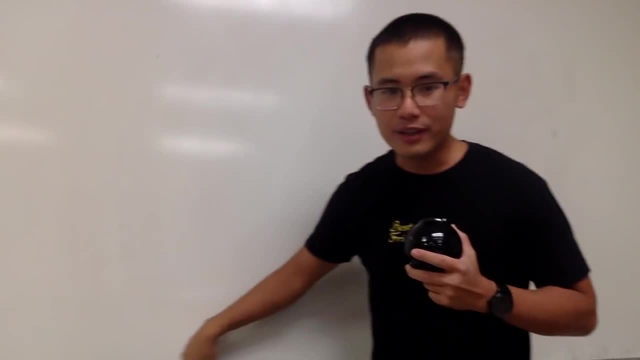 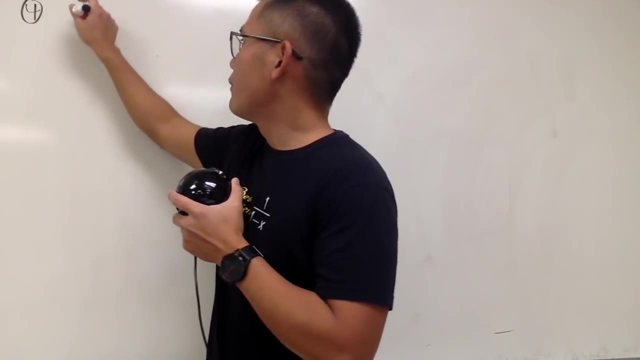 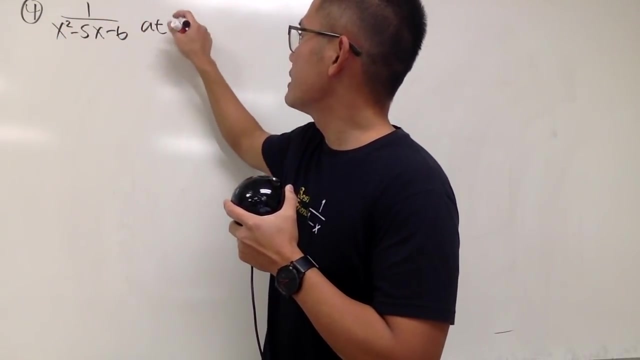 Because I know power series are weird most of the time. so yeah, Next one, number 4.. Let me just show you guys right here. Here we have 1 over x, squared minus 5x minus 6 at the center. 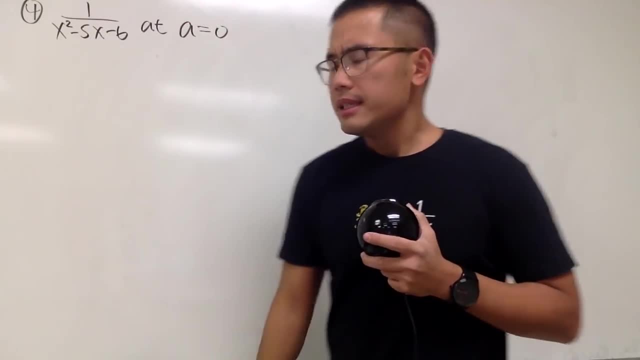 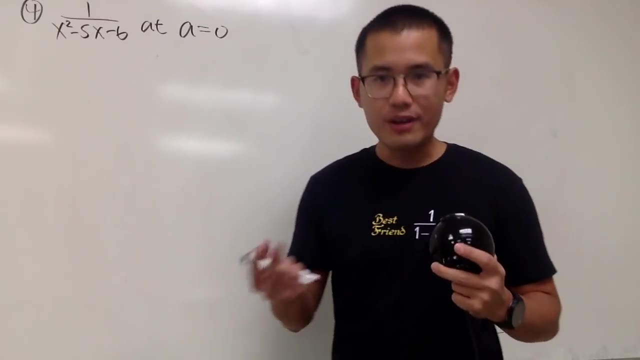 a is 0.. 0.. Man, this is not a best friend. It doesn't look like the best friend at all And the worst thing is that it has 3 terms. Best friend, it also has only has 2, right. 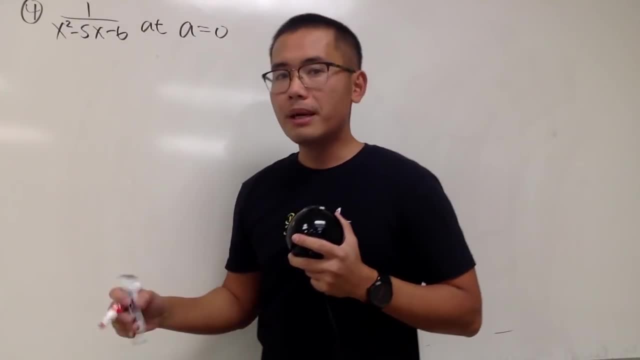 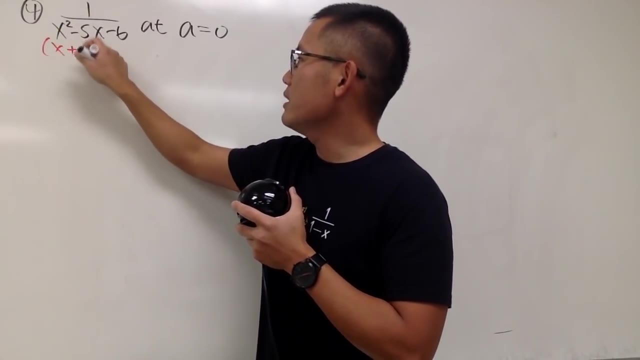 But we do notice that this right here, x squared minus 5x minus 6, we can factor it, isn't it? This right here we can factor: This is x plus 1 times x minus 6.. Looks good. 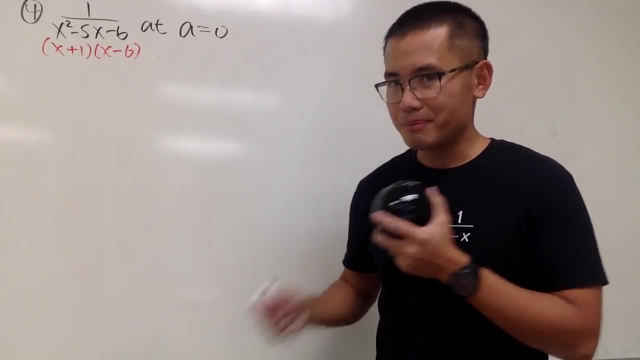 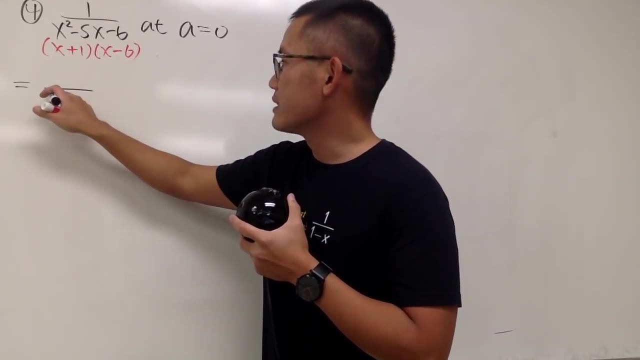 And if we do that, what can we do next? Partial fractions, Yeah, So here we go. Partial fraction for this guy. Okay, for the first one I'll just write this as x plus 1, some number over that, and then 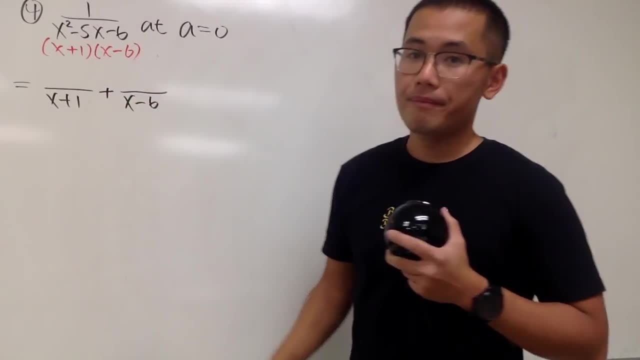 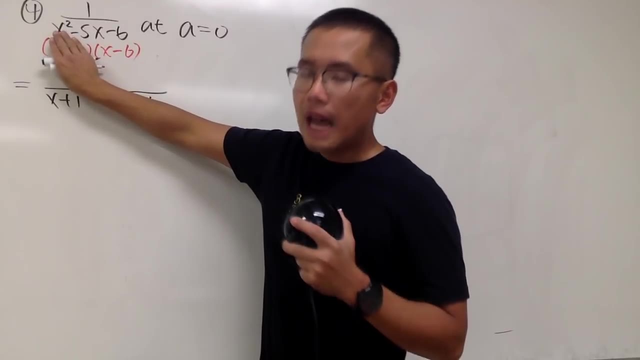 plus this one is x minus 6, and all that. Now here we go To figure out this number. we go back to the original and cover up the same denominator and ask yourself: how can we make x plus 1 equal to 0?? 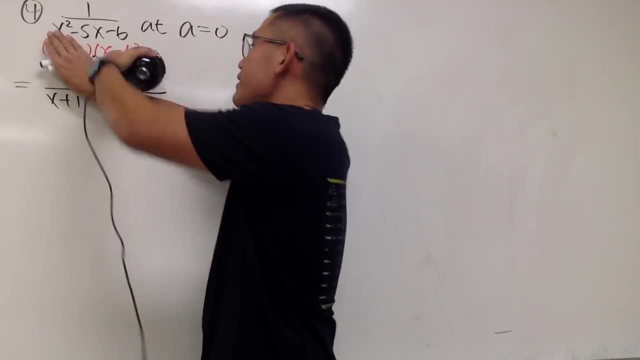 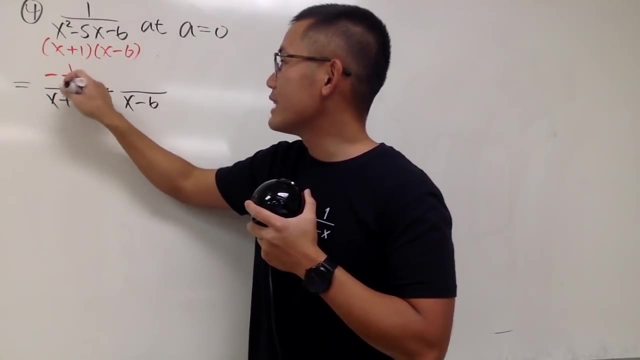 Well, x has to be negative 1. And then we put negative 1 in here. So we have what? 1 over negative, 1 minus 6, namely we get negative 1 over 7, right. And then we do the same thing here. 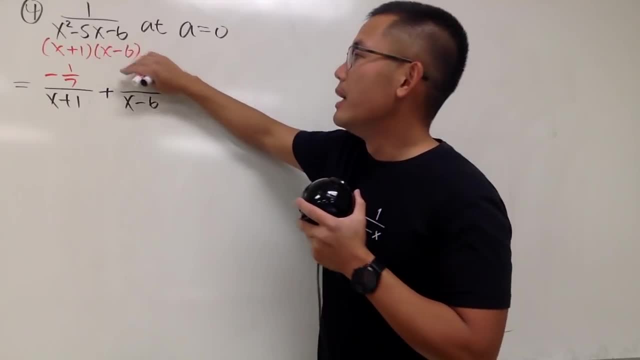 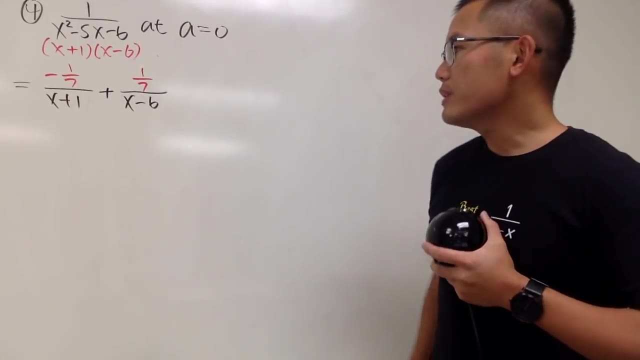 But cover this up. we need to make x equal to 6, put it here, so we have 1 over 6 plus 1, namely we get 1 over 7, like this. Okay, and we know our best friend already. 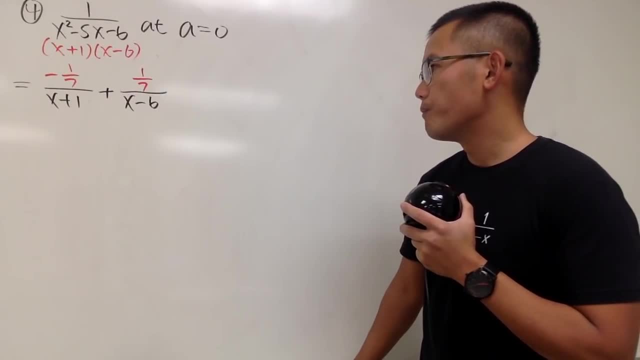 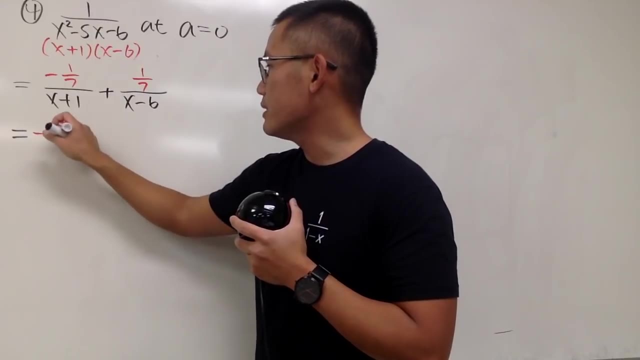 and let's see: Hmm, Okay, we'll just do the change right. Our best friend right here. So here I will just write this as negative: 1 over 7,, all the way in the front, and multiply by this is 1,. no big deal. 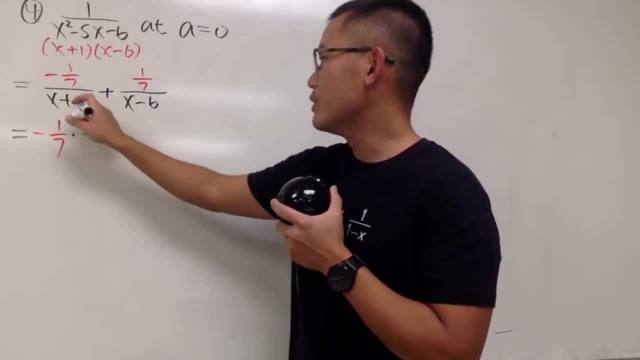 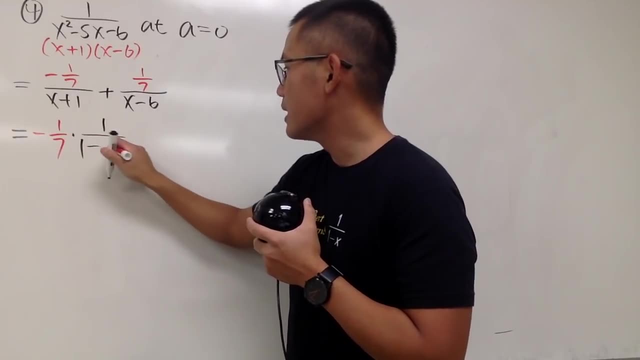 over. of course we can switch the order, no big deal. so we have 1, but this is a plus. No big deal, because plus is the same as minus minus. so we have minus minus x. So that will be for the first part. 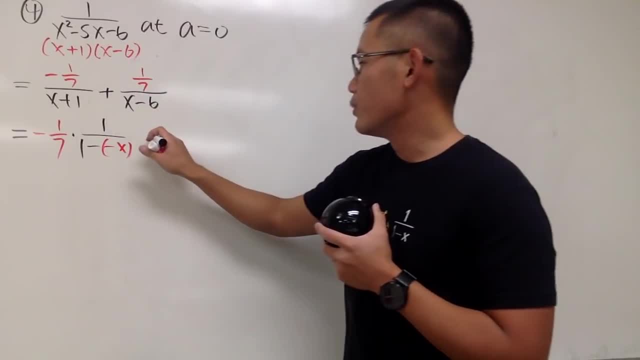 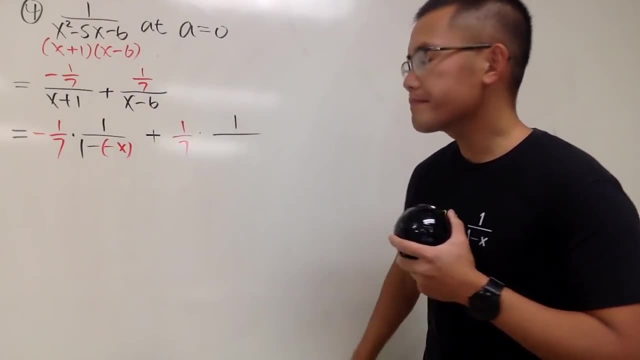 and we're ready for using our best friend. Next we add: this is 1 over 7, let's put it on the side like this: and then we have the 1 over, then we have x minus 6.. 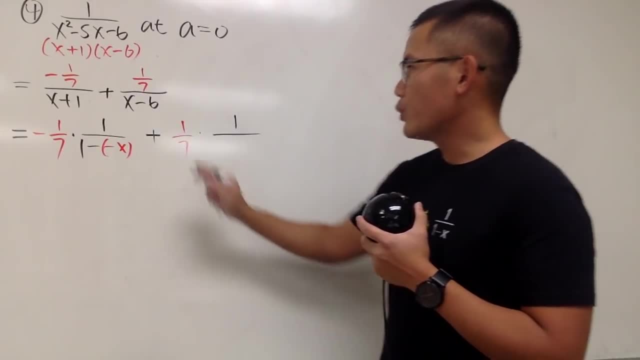 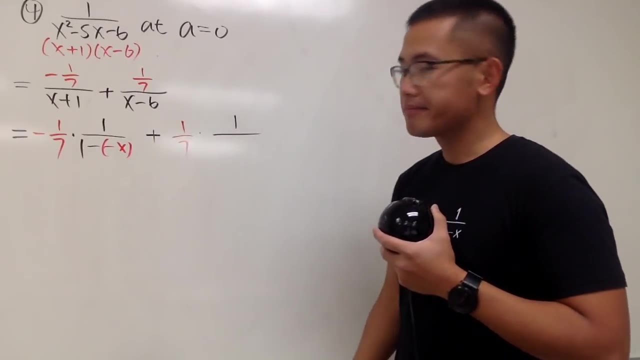 We need to have the number goes first, right, Because it's 1 minus x. So we will have to switch the order of subtraction. In the meantime, I need to make this a 1, not a 6.. It's okay, we will just use a purple pen. 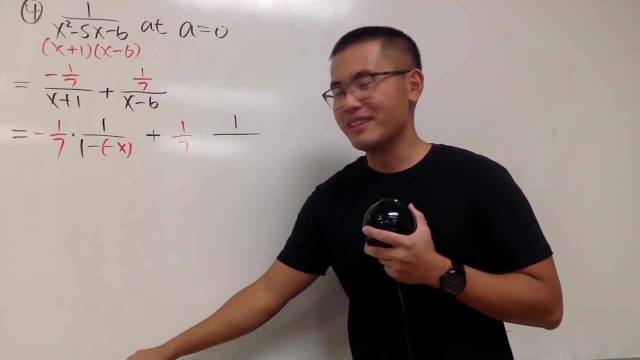 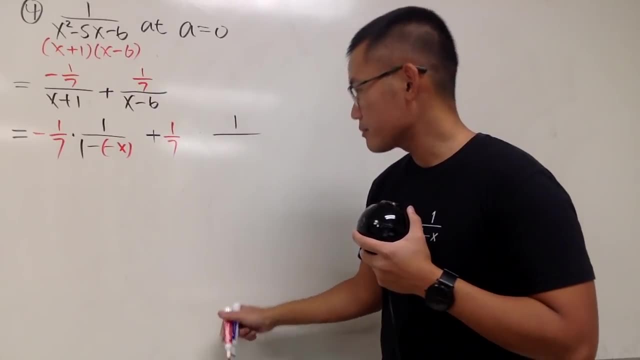 to take care of business. for us, Today is, yeah, purple pen, because unfortunately I don't have a pen of blue pen in my department. so, yeah, 1 over 7.. Okay, here we go. I'm going to just have a 1 over. that looks more better. 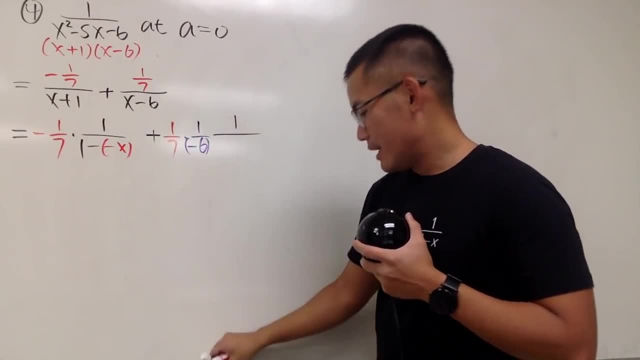 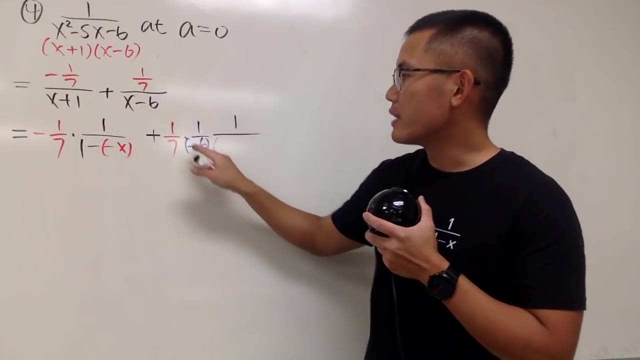 Anyway, we factor out the negative 6 on the bottom like this and we see that. okay, to write this down carefully: originally we had x minus 6, but we factor out the negative 6, so we have 1, okay. 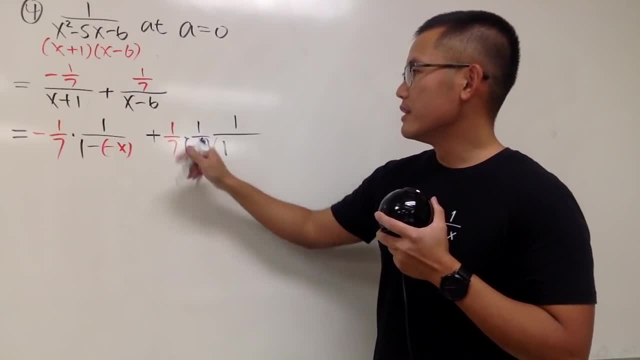 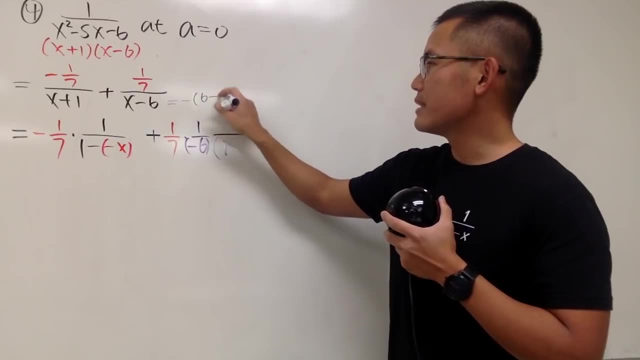 And when we factor out a negative 6, let me just put this down: when we factor out a negative 6, when we factor out a negative, it's 6 minus x. right, But then? yeah, but then I also want to factor out the negative. 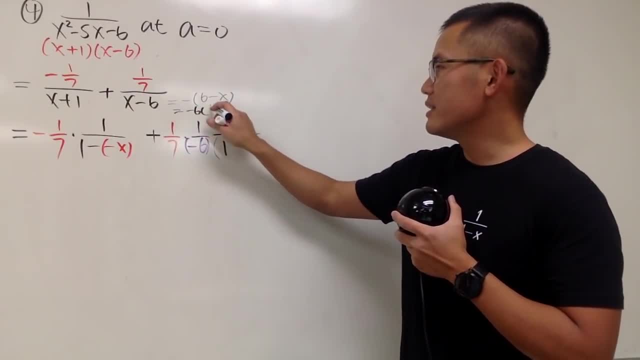 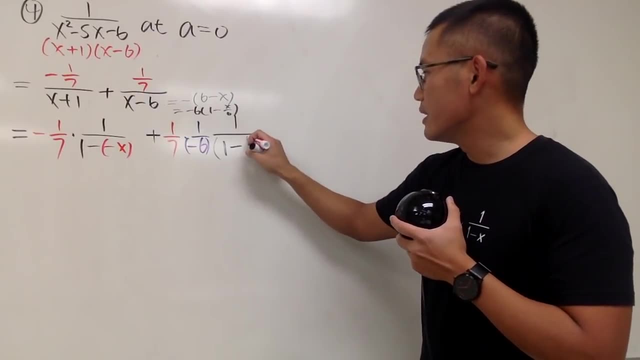 I also want to factor out the 6,, so this is negative 6, and this is 1 minus x over 6,, like this, okay. So this is going to be 1 minus x over 6,, like that, okay. 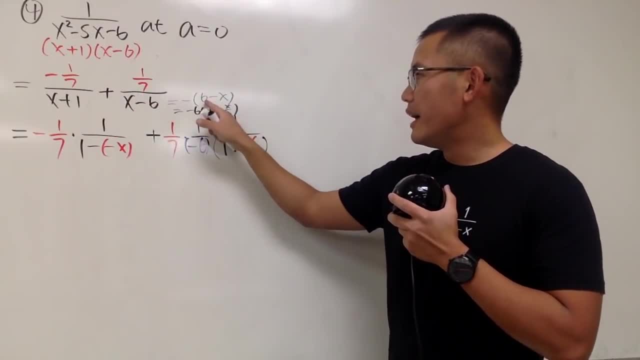 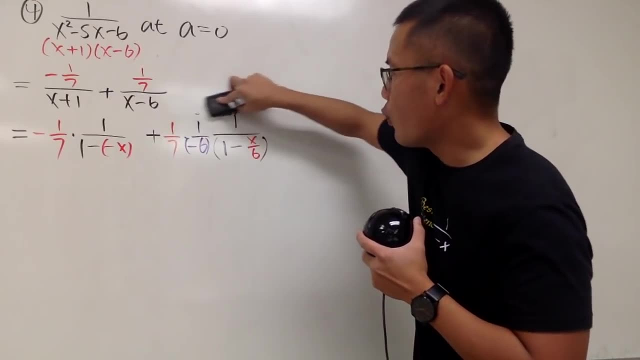 So again, I switch the order by factoring out a negative, and then I factor out the 6, and then it's 1 minus x over 6, and that's what we have. And of course you can always double-check and triple-check. 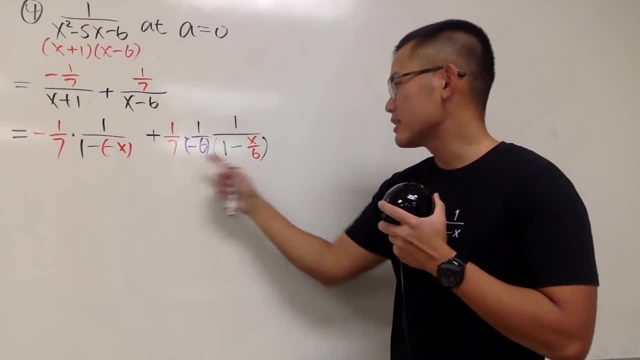 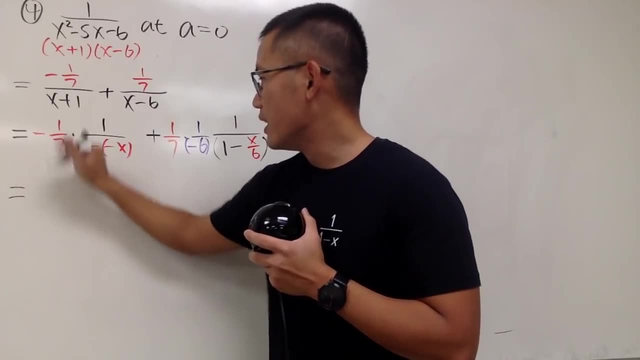 just by multiplying this: in This times that is negative 6, this times that is positive x. so we did it. Okay, now use our best friend. This right here: we get negative 1 over 7 over there in the front. 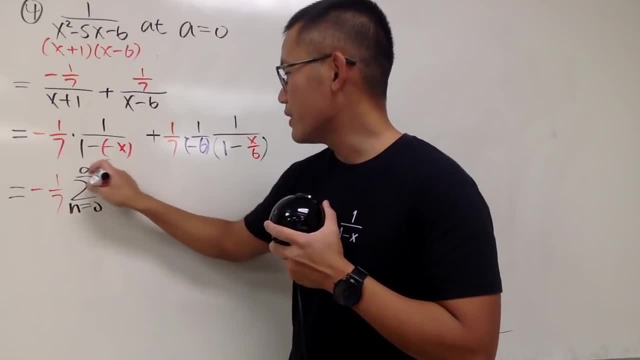 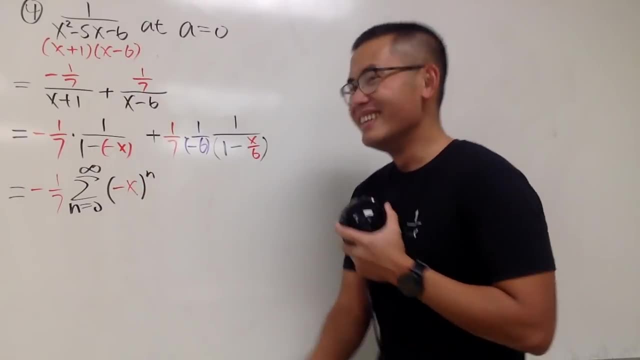 and this: right here we have the sum, and it goes from 0 to infinity. open the parentheses. you enter this into the parentheses that you just opened. yeah, And then right here. okay, multiply this out, we get a minus. 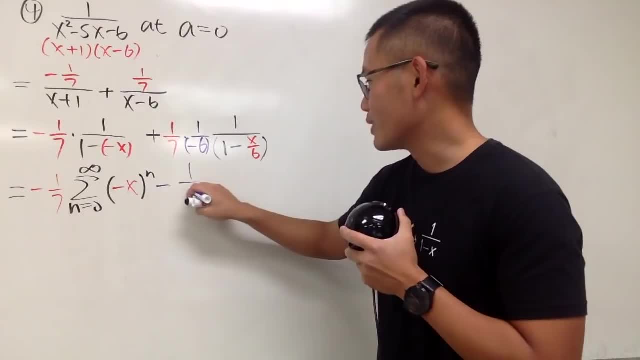 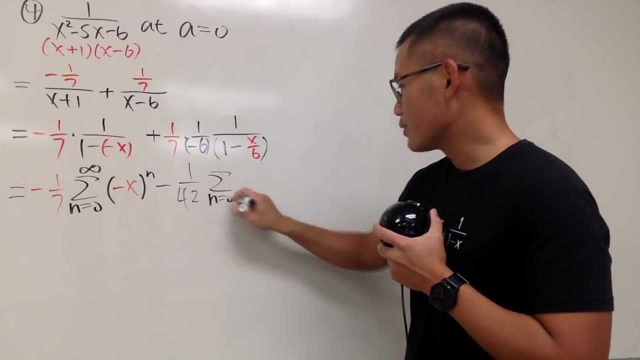 so I'll put this down in purple: minus 1 times 1 is 1, and then 42. And here we join this into that parentheses and it goes from 0 to infinity, and here we have a parentheses x over 6,. 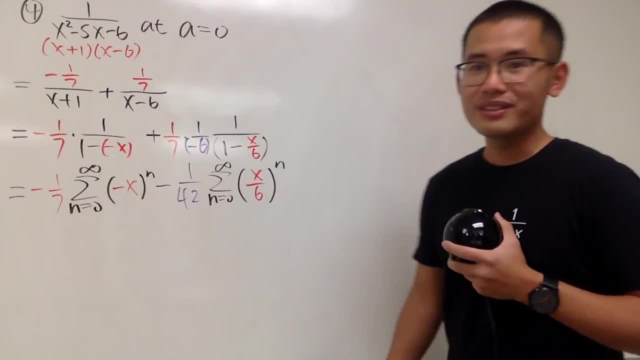 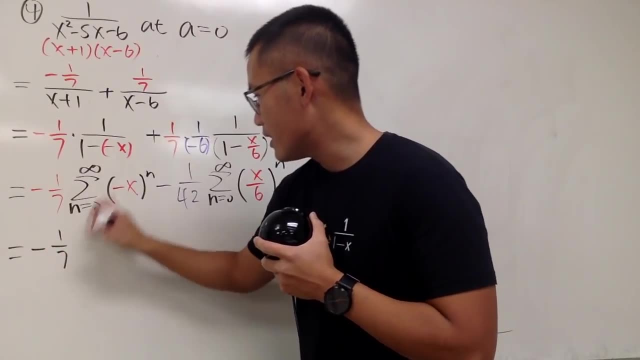 it's just positive. okay To the nth power like this. Pretty good, Now just do the rest. yeah, So here we have: negative 1 over 7, this is the sum, and it goes from 0 to infinity. 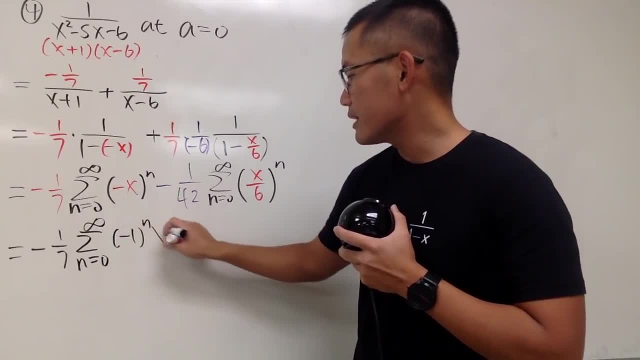 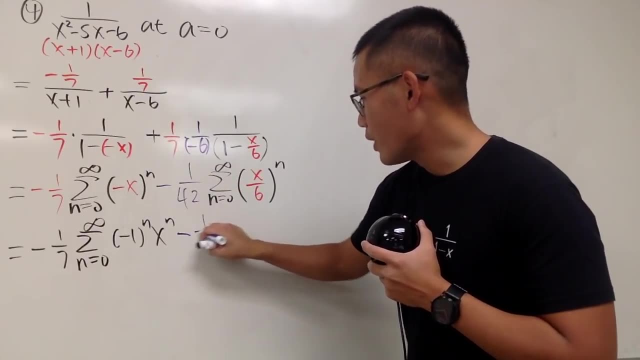 Write this as negative: 1 to the nth power times x to the nth power. like this For this one man, I will still use the purple pen. So this is a minus 1 over 42, and then here we have the sum. 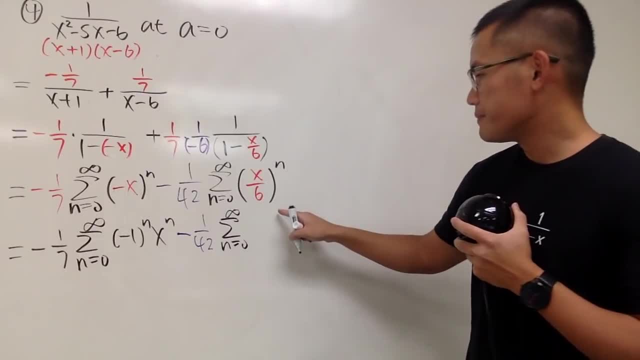 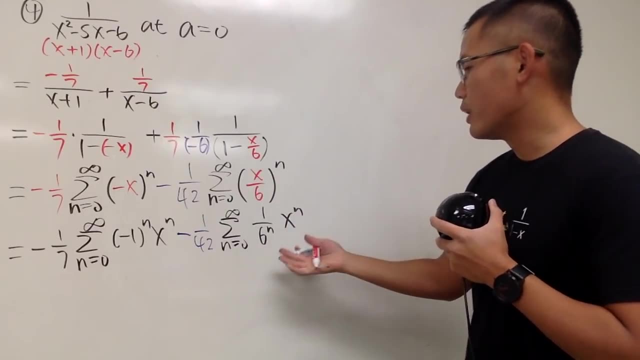 and it goes from 0 to infinity, and this is 1 over 6 to the nth power. You should write down the coefficients first and then write down x to the nth power on the side like that: Yeah And now. 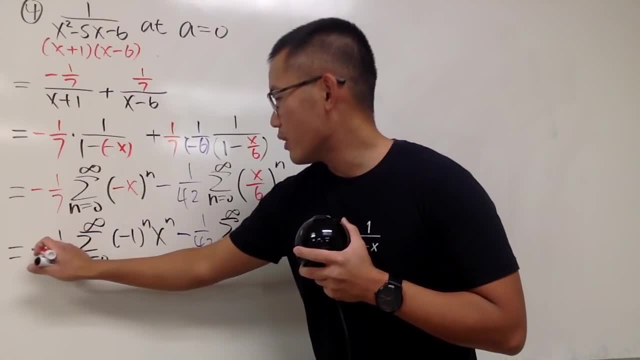 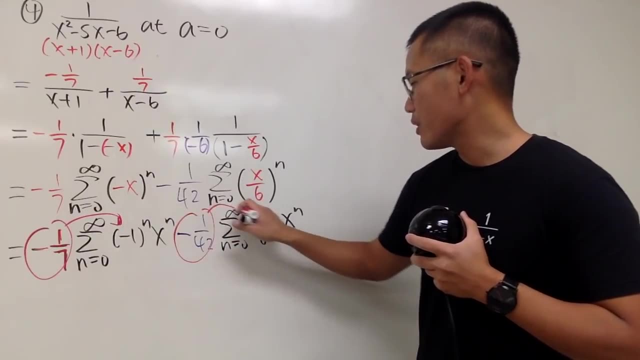 we will just kind of join everything, because this right here, of course we can just change this, put it inside multiply, and then likewise we also do the same right here. Now we do two things in one step. Here we go. 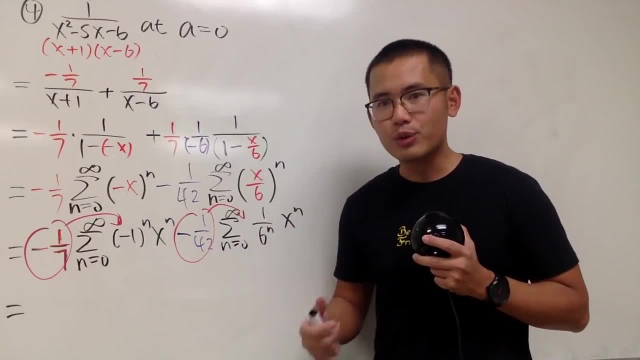 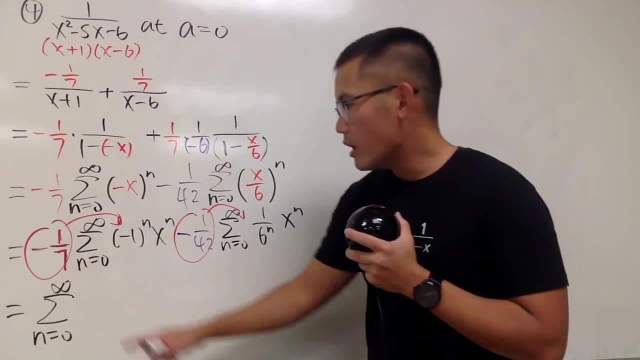 Both of them. they have the sum going from 0 to infinity, so we can just write this down as one series in the one-sigma notation. First of all, we have this, which is negative: 1 over 7 times that: 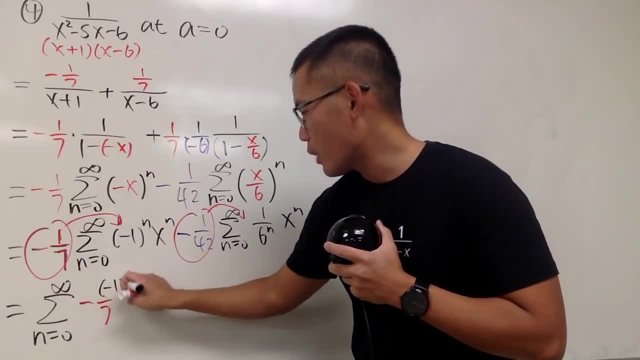 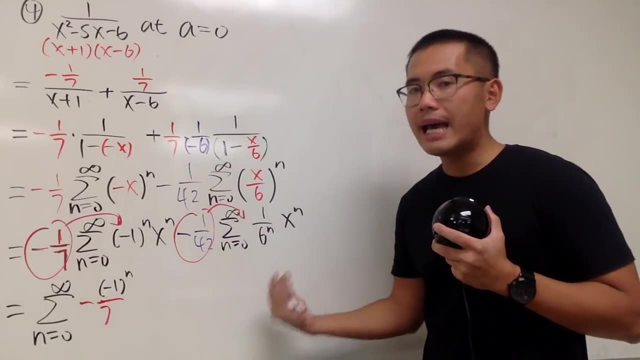 so I should have this right here on the top: negative 1 to the nth power, okay, And then, because both of them will have the x to the nth power, so I'm just going to put that at the end. Next we have this times that: 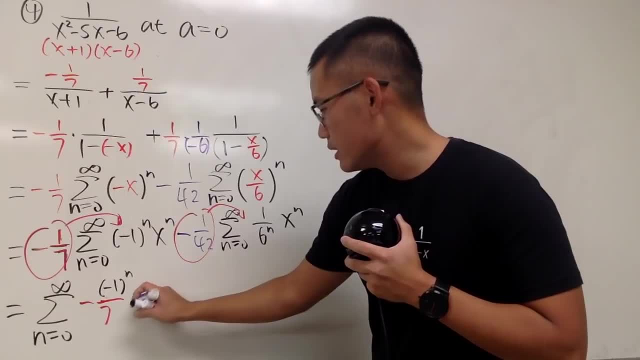 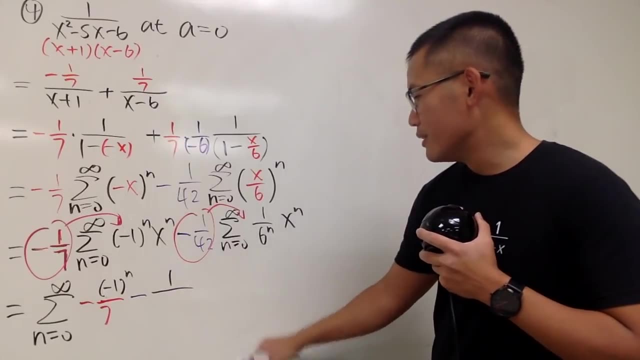 so perhaps I'll just write this as minus in purple, and one on top, of course, let's just put it on in black and then over: This is 42, so we have the 42 right here. times x, times 6 to the nth power. 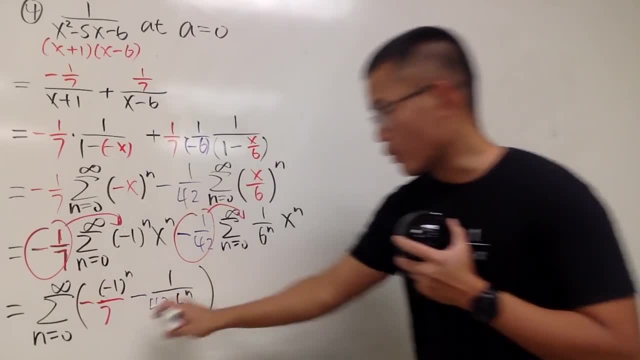 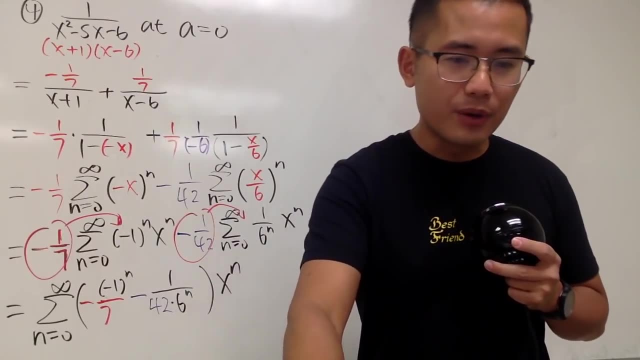 and then, as I said, this is pretty much the coefficient and we multiply by x to the nth power, like this, And I know I haven't put down the absolute value yet, but I just want to make sure that on my answer key. 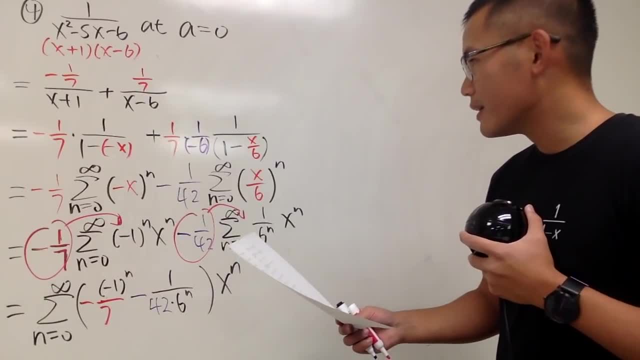 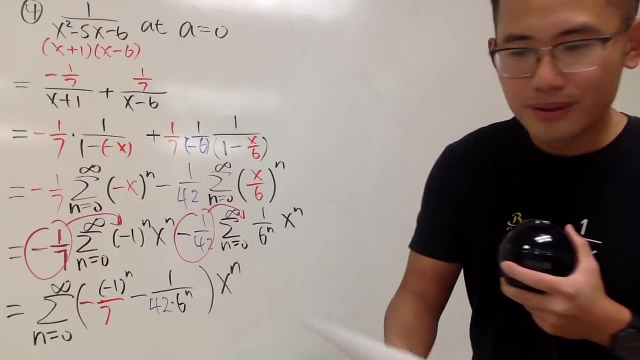 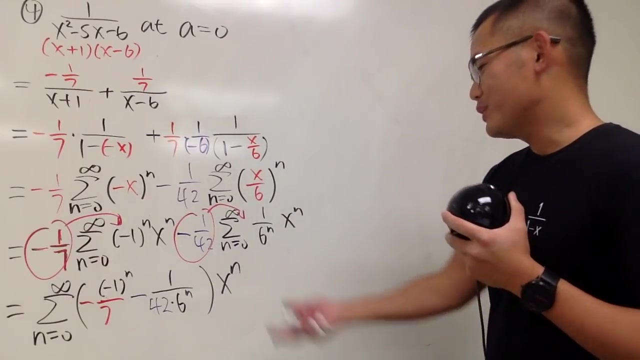 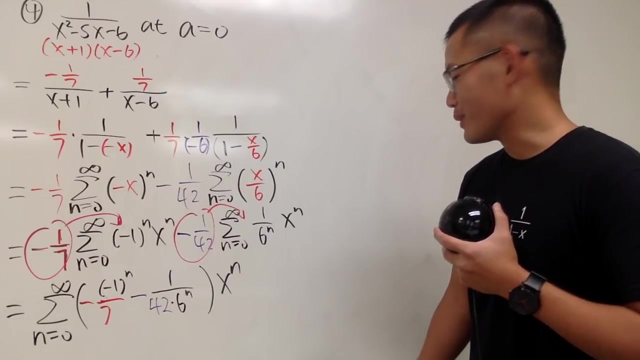 I give you guys some legitimate stuff. Yeah, kind of. You'll see why I said yeah, kind of. but it really depends on how you want to simplify this guy. okay, So just leave it if you don't like it. Man, I don't know. 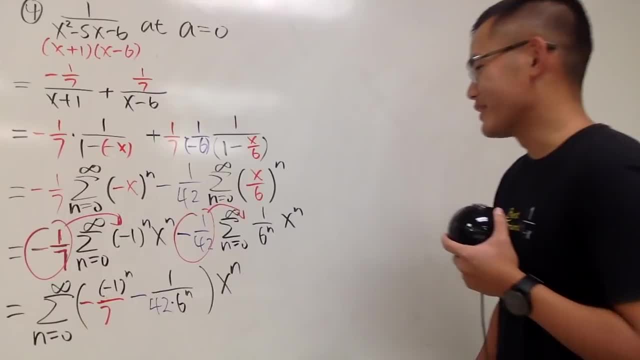 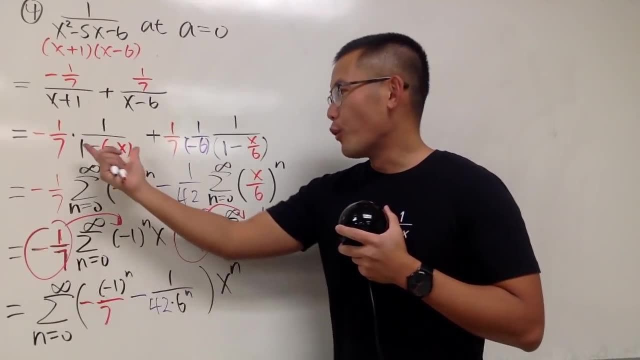 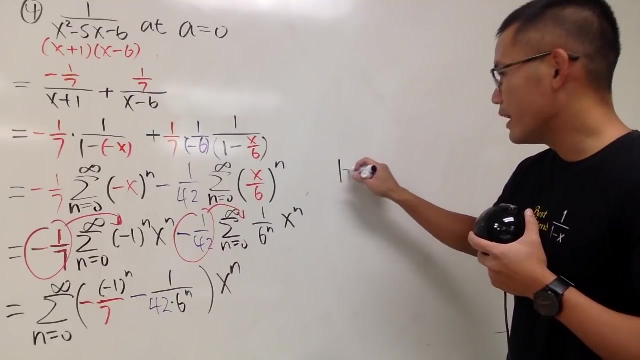 If you leave it like this, it's totally okay, seriously okay. But anyway, right here you need two conditions. The first condition is that from here to here, you enter the negative x Into the best friend, right. So the first thing is that you look at absolute value of negative x. 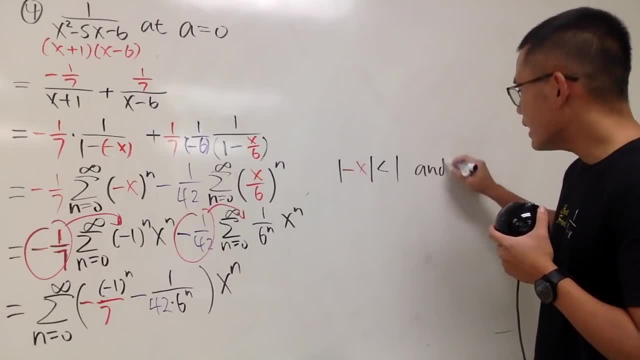 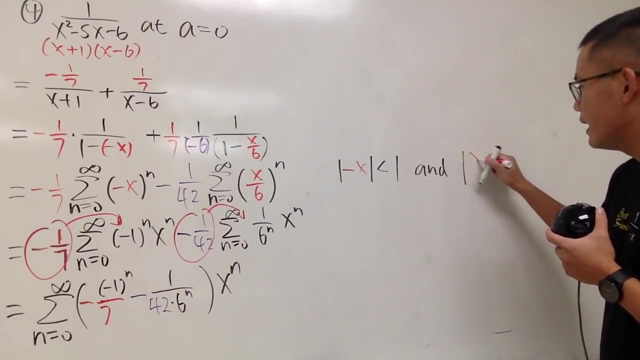 is less than 1.. And you also have to make sure because we entered it x over 6- into the best friend, so we have absolute value of x over 6 to be less than 1.. And of course you are just going to look at this. 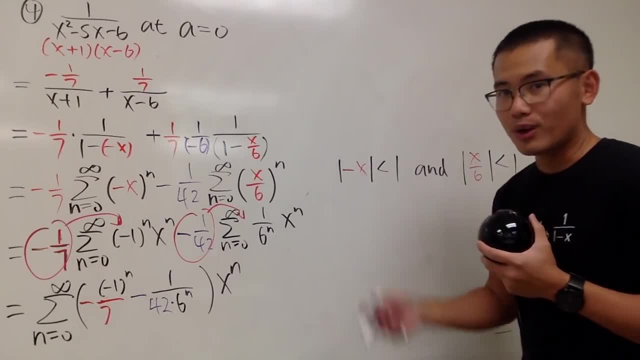 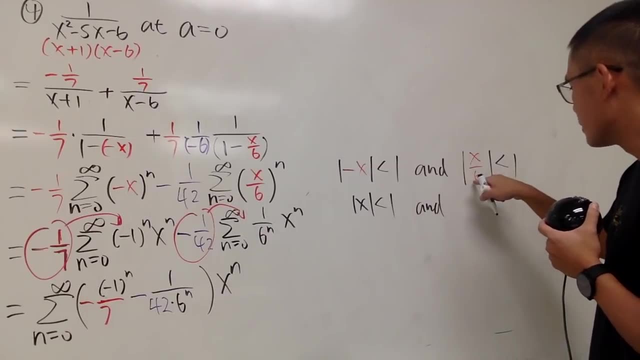 and then just kind of solve to see the inequality. This right here is straightforward: Absolute value of x is less than 1, and this right here, well, multiply the 6 on both sides, absolute value of x is less than 6.. 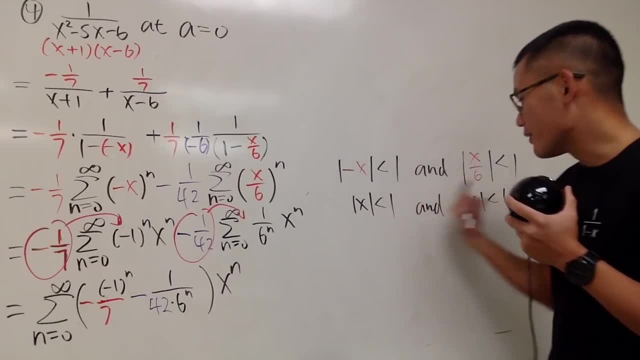 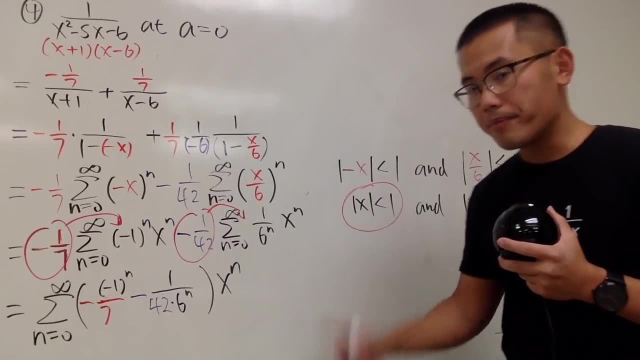 Well, this is smaller, right? This is inside of that, so you just care about this one, because it's an n situation, this and that. So this is it. So that means r will be just 1, because, yeah, this is from negative 1 to 1,. 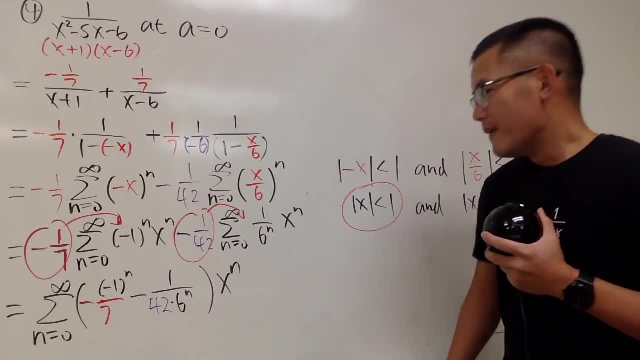 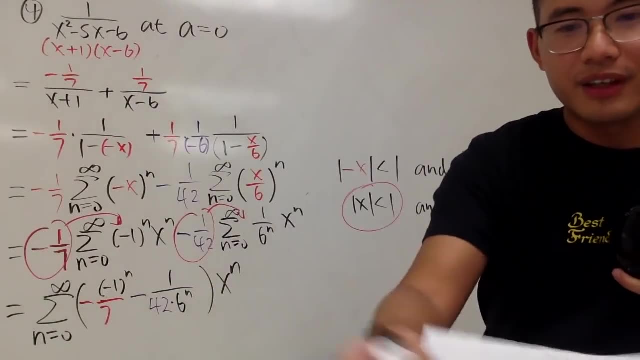 this is yeah, inside, yeah, Hmm. So I'm going to leave it right here, but I do have, perhaps, just an algebra version of the answer on there, so if you guys would like, you guys can try your best to enter that. 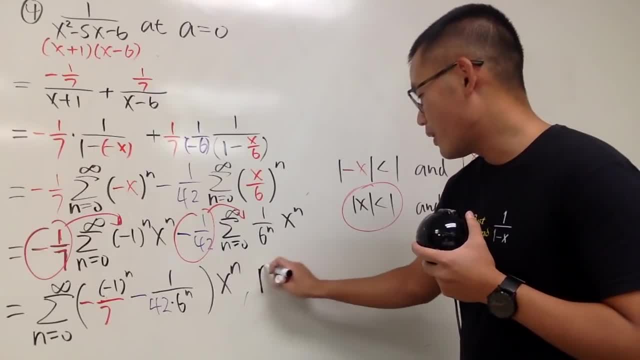 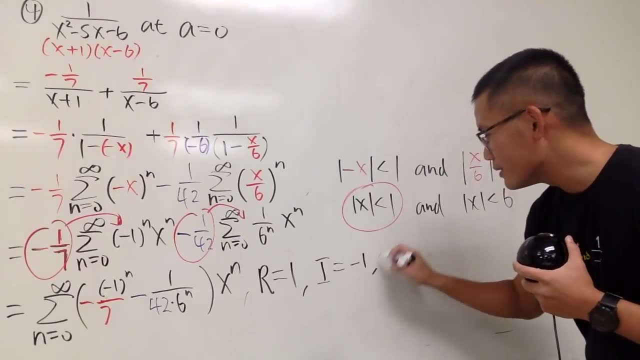 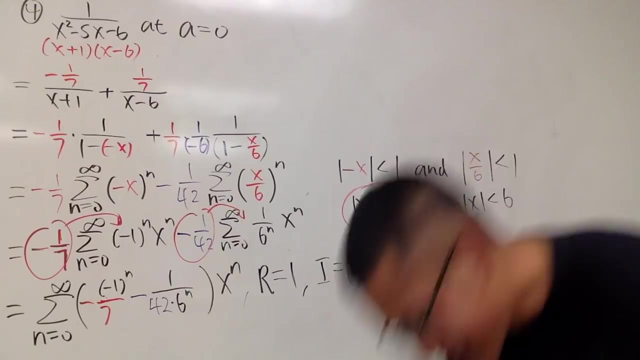 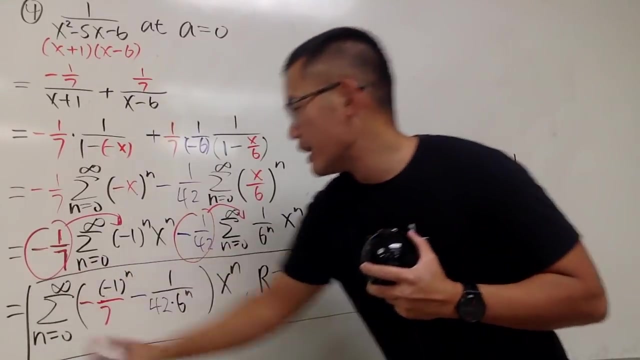 I think I'm done with this, So I'll just tell you r again 1, right, And I will just go from negative 1 to 1.. Oops, Let me maintain the same color, So oops. So this right here, is it right? 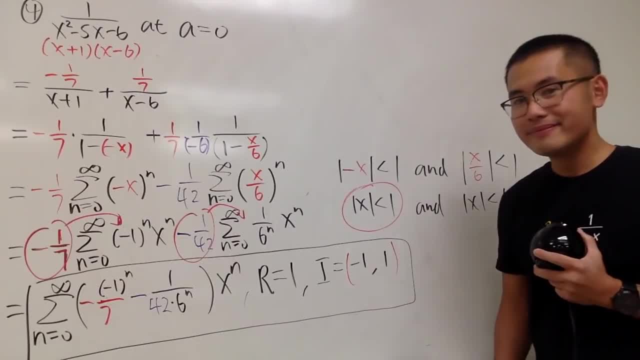 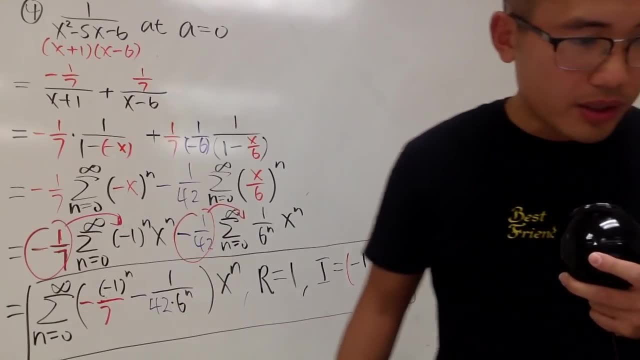 Yeah, Yeah, Okay. so that's question number 4.. And now let's see if I can squeeze in another one, Question number 5.. Okay, I think I can do this one. Okay, 1 over 1 minus x squared. 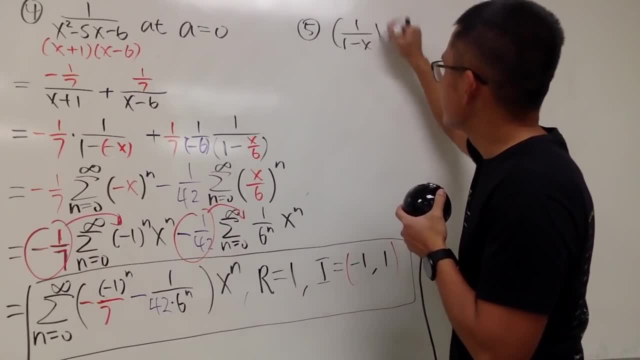 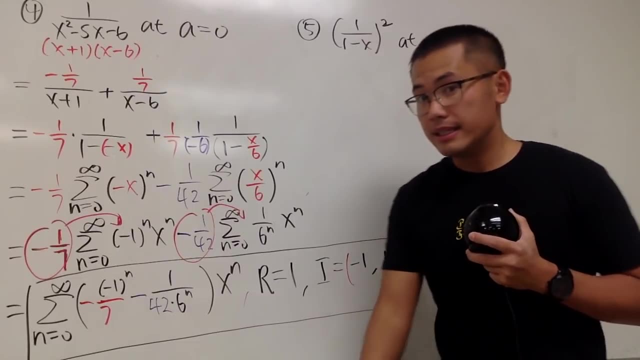 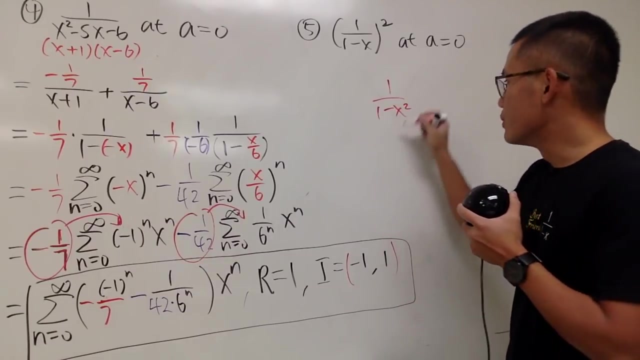 Number 5.. This is 1 over 1 minus x and then squared Center the ad a equals 0.. Man, The question was 1 over 1 minus x squared. This would have been so much easier because all we have to do is to enter the x squared. 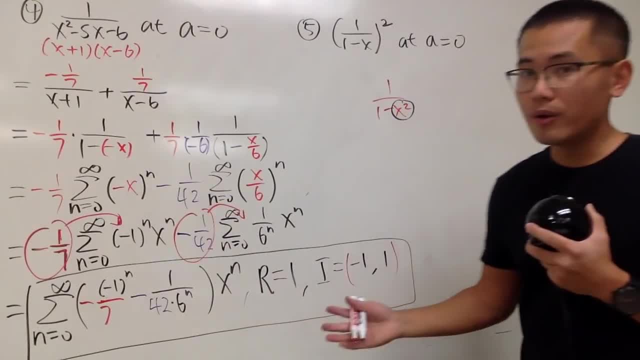 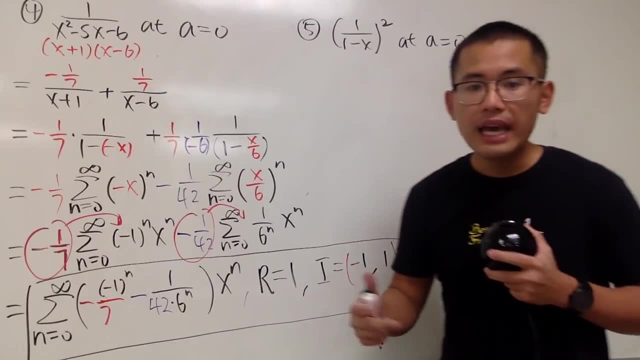 into our best friend, into the summation right here. right, That's all. But unfortunately not. This is what we have: 1 over 1 minus x in parentheses, and then we square that. Of course, this is the same as saying: 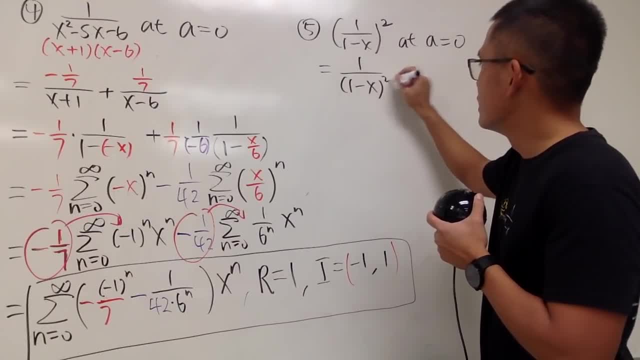 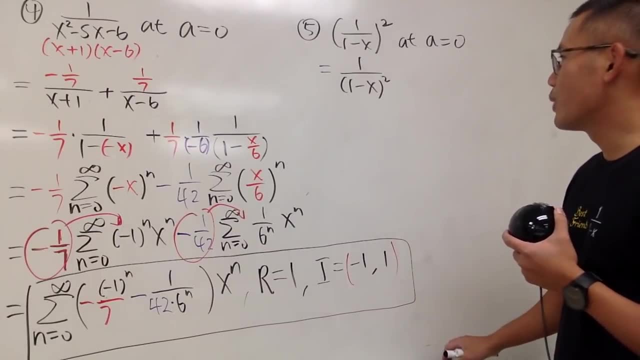 1 over parentheses, 1 minus x to the second power. If you want to expand this, maybe, but maybe not, Don't do it. So now, this is what we are going to do, okay, So let me actually just write this down. 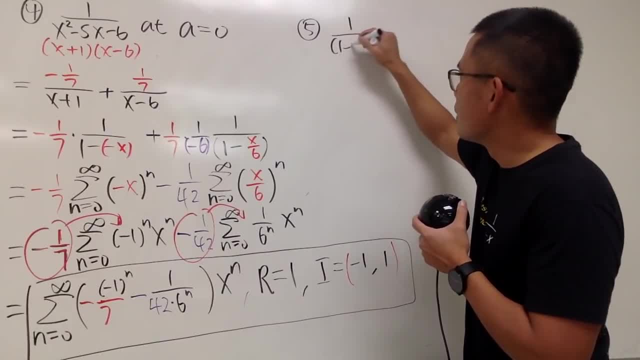 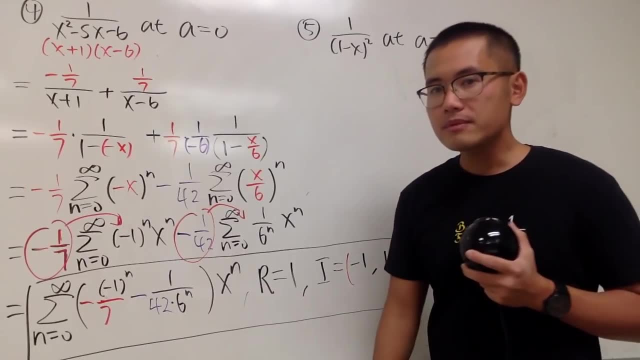 Let me just actually write this down: 1 over parentheses, 1 minus x squared- That's actually how I wrote in the question, actually- And a equals 0. Anyway, Hmm, Let's see what's the connection between our best friend and that. 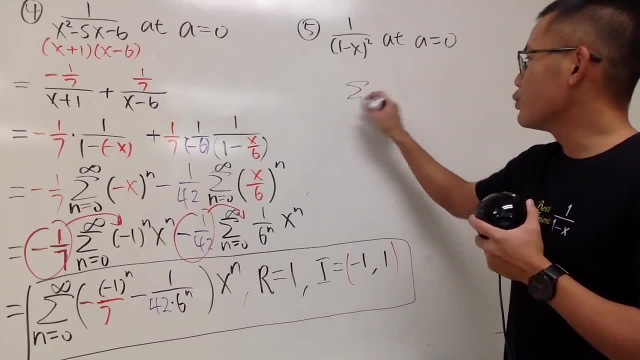 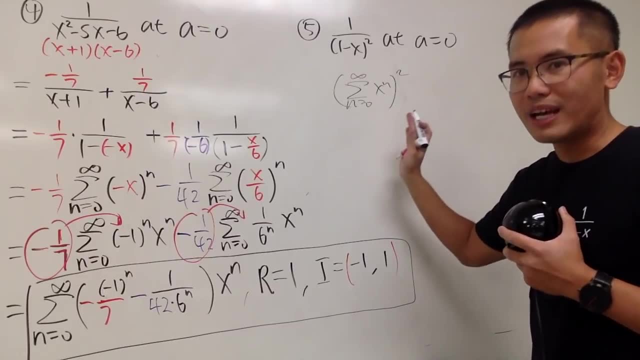 It seems that it's just the best friend squared, But if you put that down, you will have the sum as x. This is the best friend Square. Don't do that. It's much harder. Life doesn't have to be that hard sometimes. 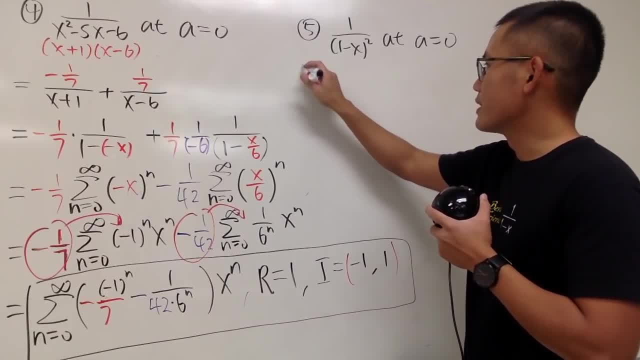 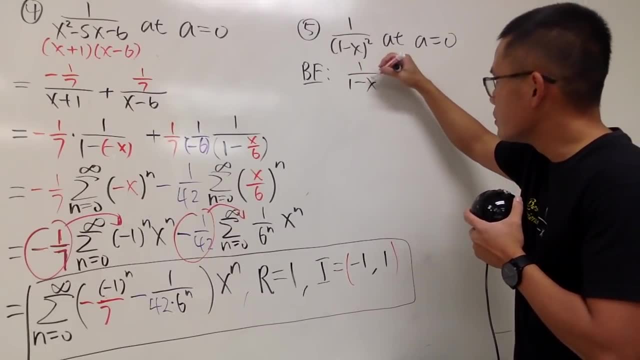 This is how we are going to do it. So here we go. I'm going to write this down again. Again, I'll just write down the best friend, 1 over 1 minus x, which is we know- let me just change this to great. 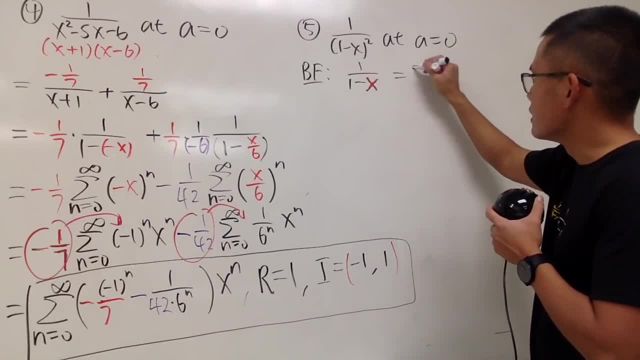 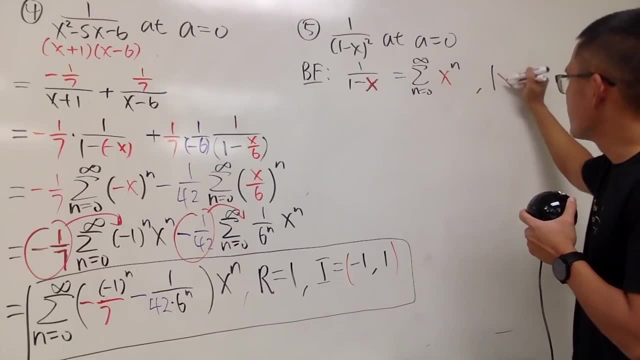 It doesn't matter. in this case, Which we know, this is the sum, as n goes from 0 to infinity. We have x to the nth power and absolute value of x, This is less than 1.. Okay, Well, the bottom is being squared. 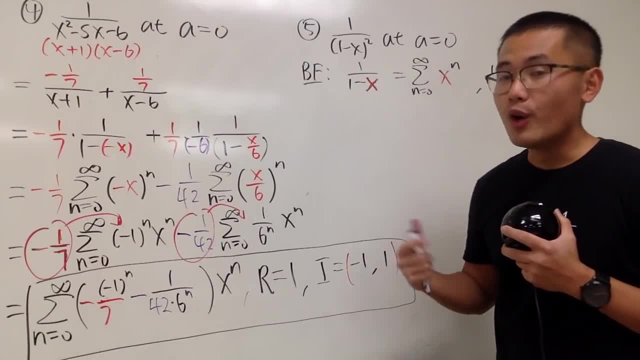 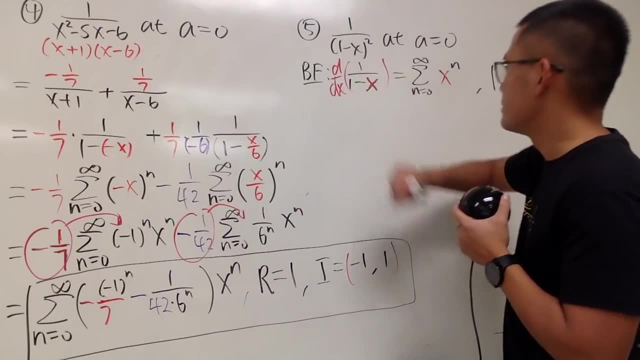 The truth is, if we differentiate the best friend, we can actually get the square on the bottom. Let me show you So. on the left-hand side, I will differentiate the best friend with respect to x. Likewise, on the right-hand side, we also differentiate this. 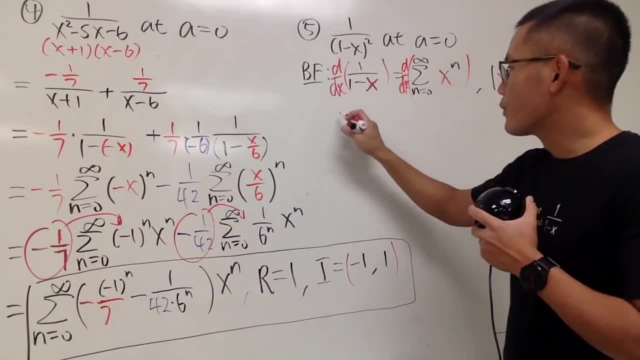 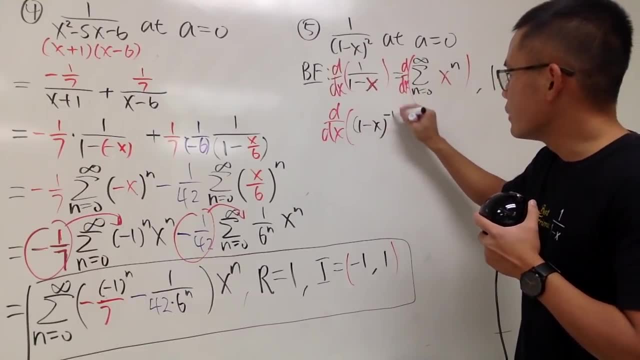 Right, Okay, To differentiate this. of course we look at this as negative power, So we have 1 minus x raised to the negative 1.. It's much easier this way. So let's focus on the left-hand side first. 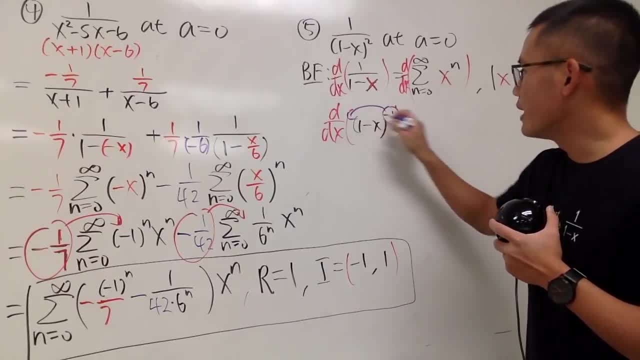 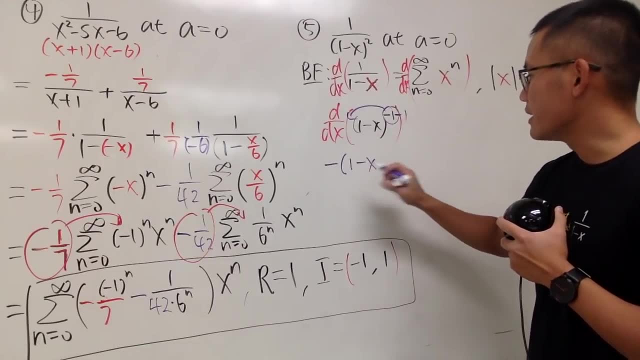 Well, to differentiate this, we can of course bring the power to the front and then minus 1.. So we get negative parentheses with 1 minus x in here, And then that's the negative 2 power. But don't forget the Chengdu. 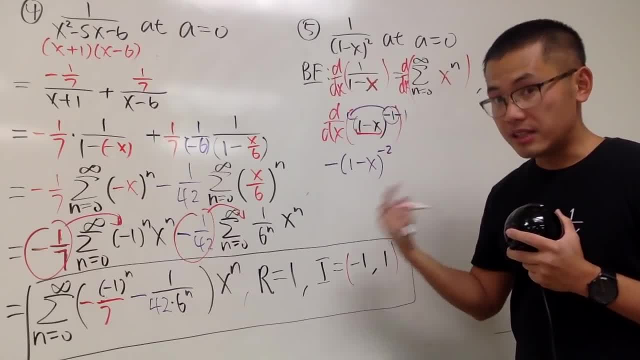 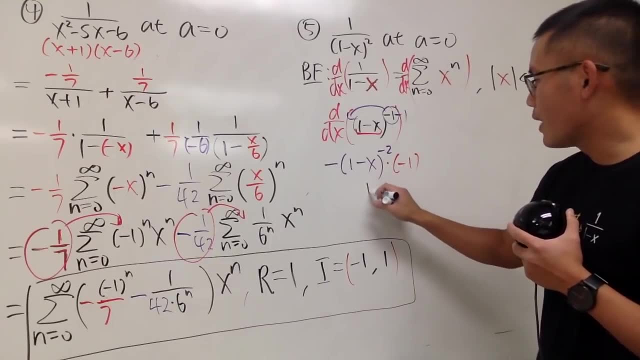 Multiply by the derivative inside. The derivative of 1 minus x is negative: 1. So multiply by negative 1. So in fact negative negative becomes a positive. So we get 1 over parentheses, 1 minus x, squared like this: 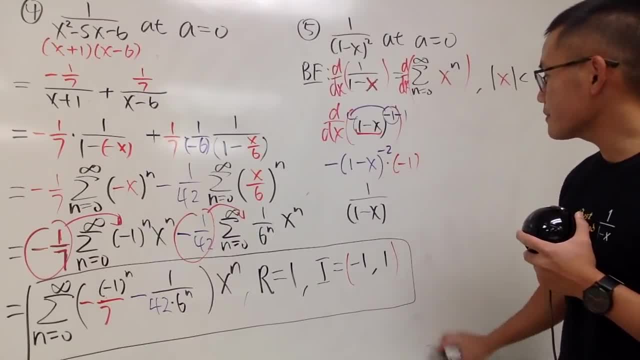 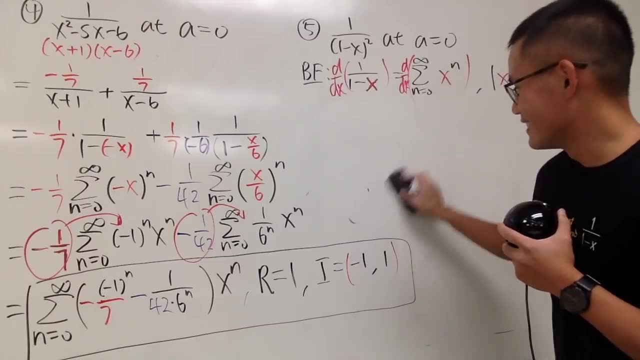 Very nice, Very nice, Right. So that's the idea. When you differentiate this, you get that. Let me just erase this so I have more space. When we differentiate that, we get 1 over parentheses, 1 minus x squared. 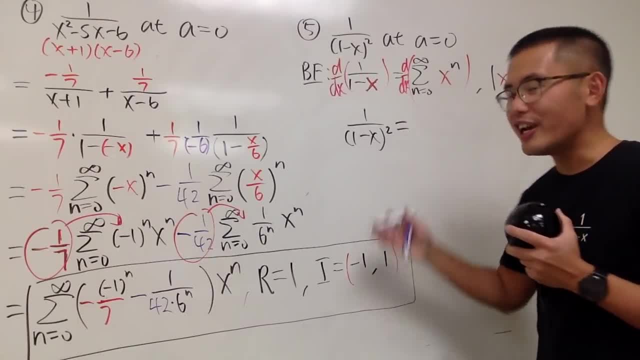 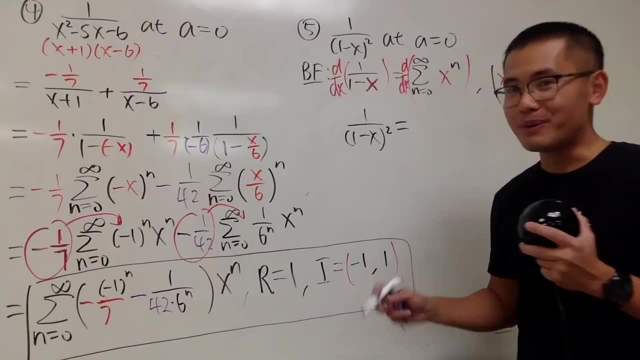 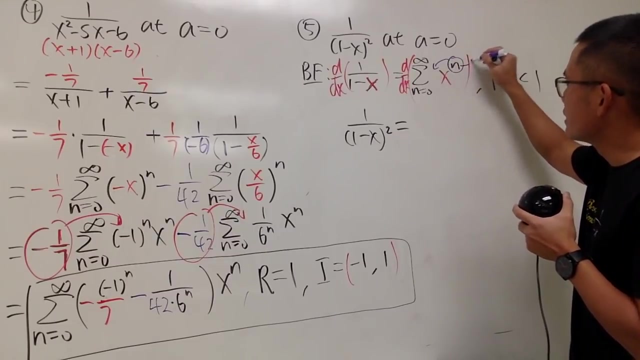 And congratulations On the right-hand side. to differentiate a power series, You don't need to use anything tricky. Unfortunately we can use the Chengdu, but sometimes it's better that way. Differentiating a power series, go ahead and bring the power to the front and then minus 1 and you are done. 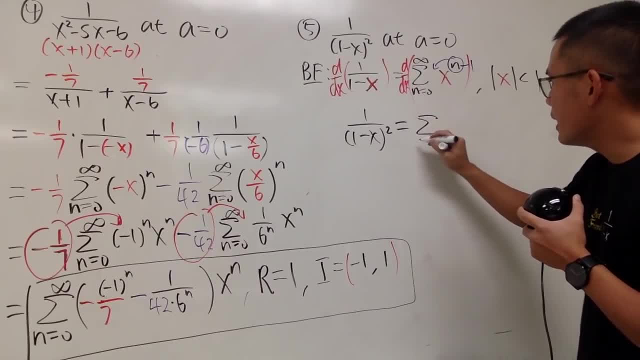 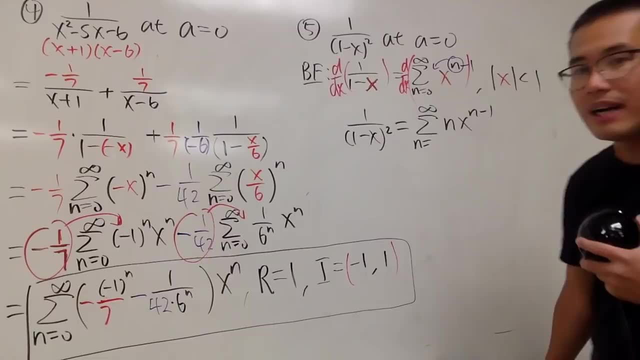 That's all. So I will write this down. We will have the sum as n goes from some number to infinity, And let me just write down n x to the n minus 1 power, like this: Now here is the deal. 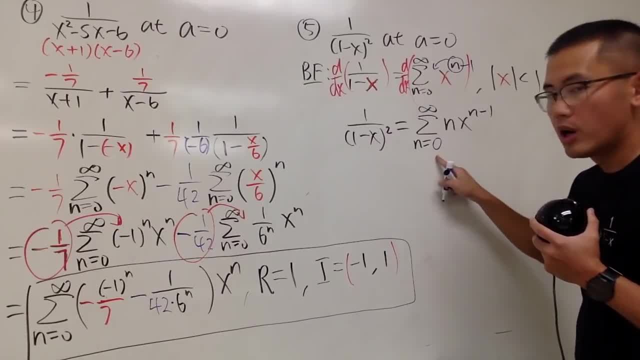 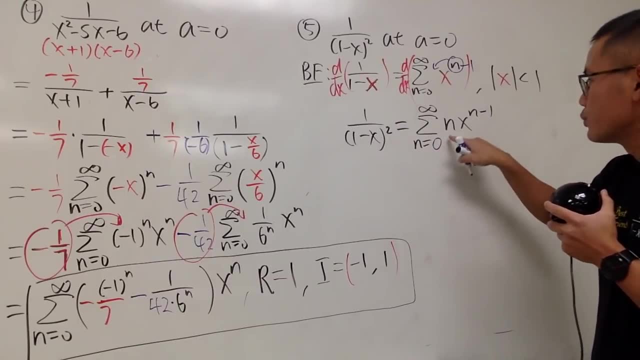 If I put down when n is equal to 0, right, because if I maintain it, well, if we put 0 into the n right here and right here first, we will just get 0 times that, It's just 0, so it's nothing. 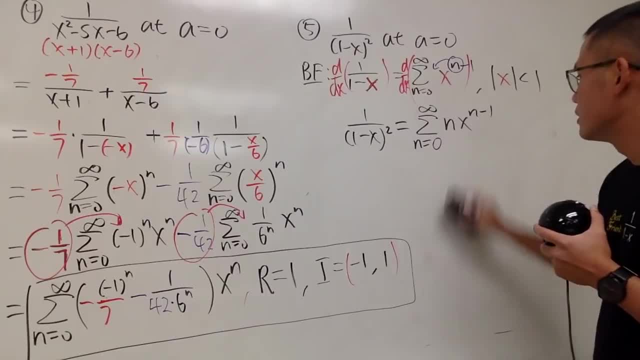 If you put 0 right here, okay, it's not wrong, But change it. We go with 1.. Because the first term matters When n starts with 1, that's the only term, That's the first term that actually matters. 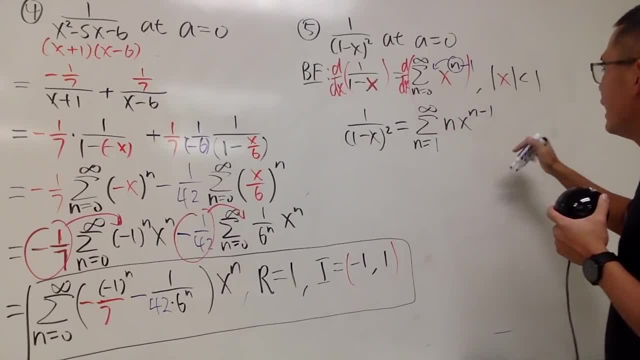 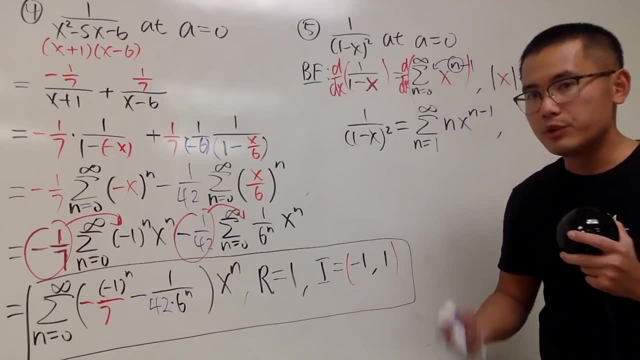 And then of course, 2,, 3,, 4,, 5, and so on to infinity. like this, And right here, I will also tell you. we know another thing that you have to know: When we differentiate the power series, the radius of convergence stay the same. 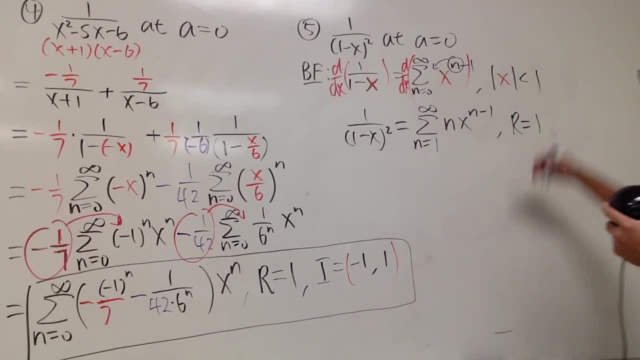 The radius of convergence stay the same right So earlier the best friend of r was 1.. Now r will still be 1.. But for the interval of convergence you will just have to double check. Well, how do we check it then? 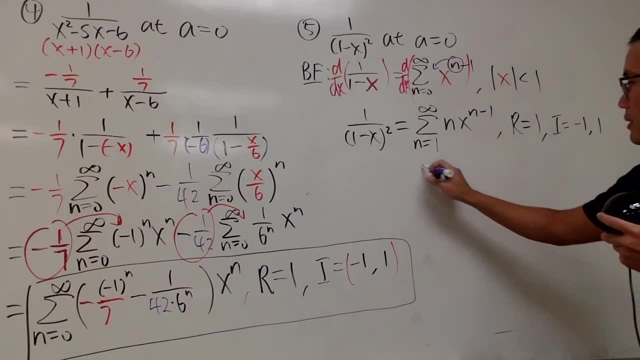 Put in negative 1 in here, So it looks like. let me just show you Check when x is equal to negative 1.. You put it right here. So we are looking at sum as n goes from 1 to infinity, And here we have n times negative 1.. 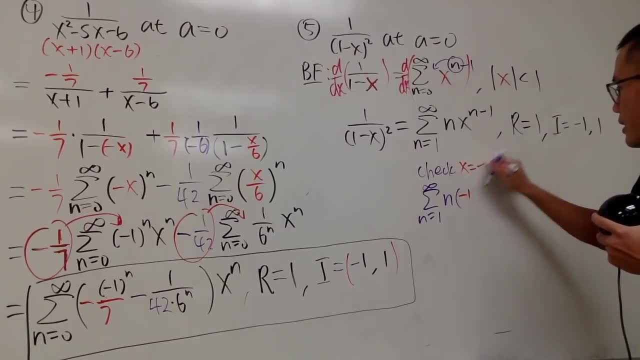 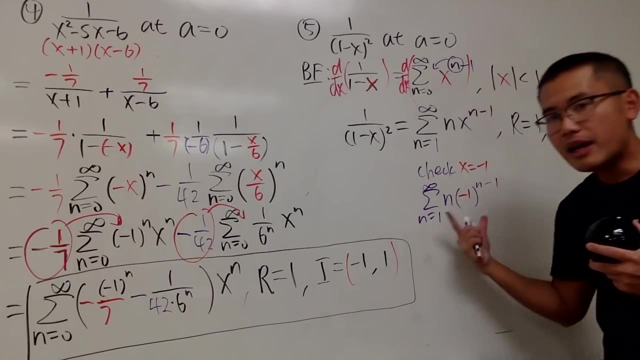 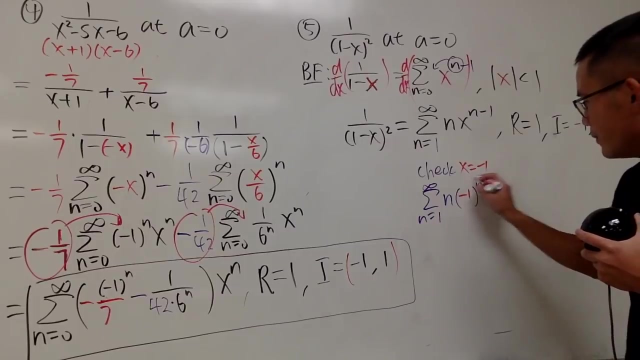 Let me just change this: in red x is equal to negative 1.. Put the negative 1 here And minus 1.. Like this. Now the question is: if n goes to infinity, does this converge? No, Because if you look at the a n part right here, 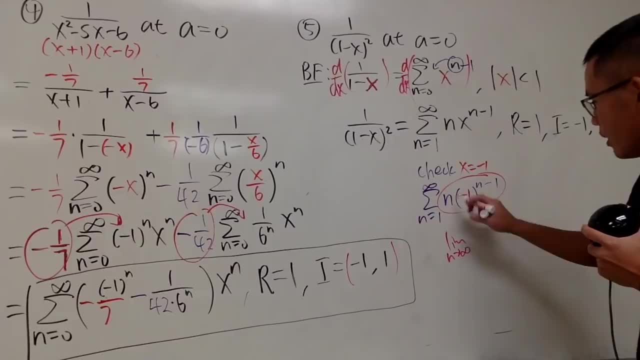 the limit, as n goes to infinity, of n times negative 1 to the n minus 1 power. this right here, well, does not exist. So in fact, this right here diverges by test for divergence. So right here, we still do not include the endpoint. 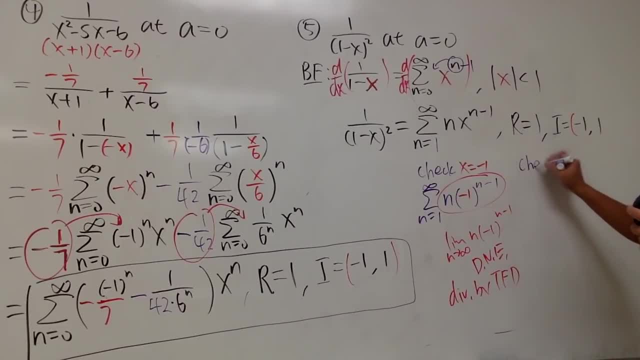 Similarly, we are going to check when x is equal to 1.. Check when n is equal to 1.. You put 1 right here. So we are looking at the sum. n goes from 1 to infinity. n is right here. 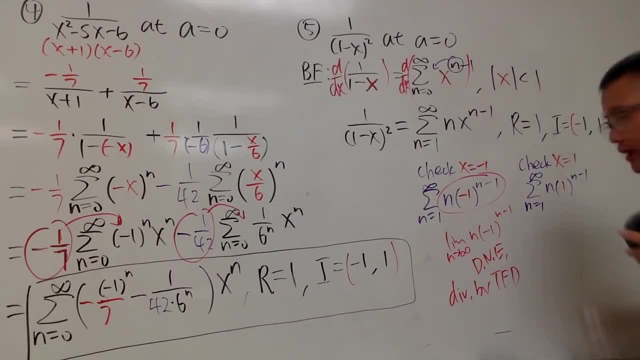 And then 1 to the n minus 1 power, which doesn't matter. And again, this right here, the limit, as n goes to infinity, of just this, this right here again, is not equal to 0.. So, divergence by test for divergence. 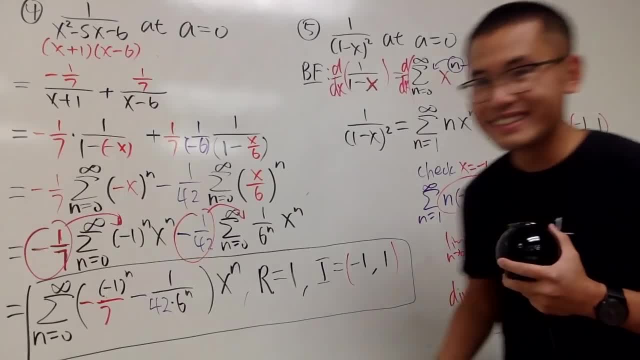 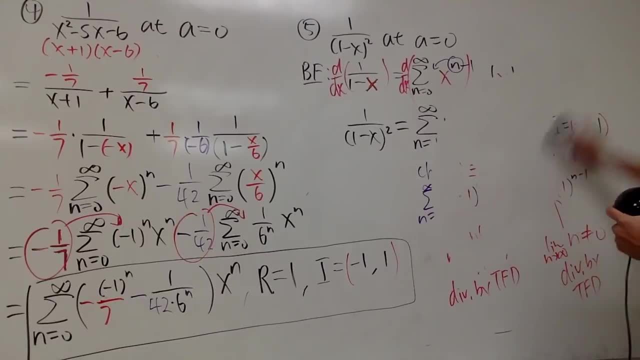 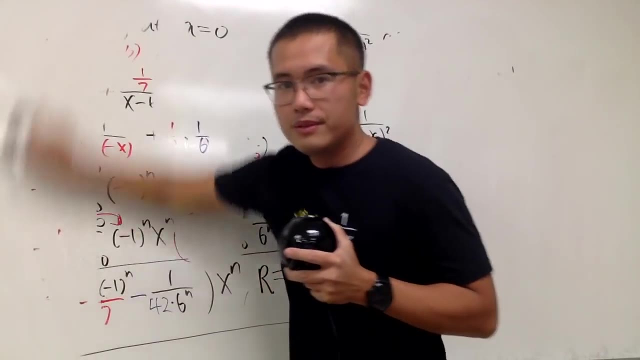 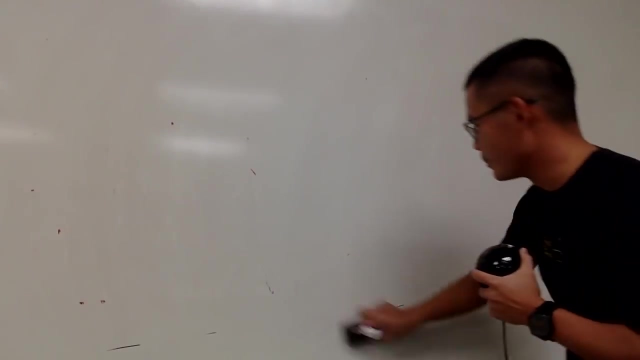 You also don't include the other endpoint Right, So that's number 5.. Yeah, OK, I think the markers are not too well today because it's kind of hard for me to clean the board, But it's OK, I'm doing this for you guys. 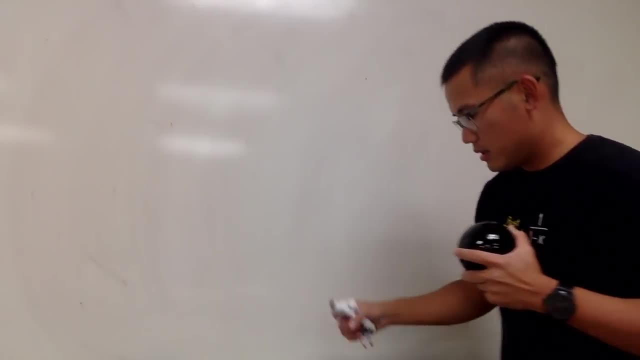 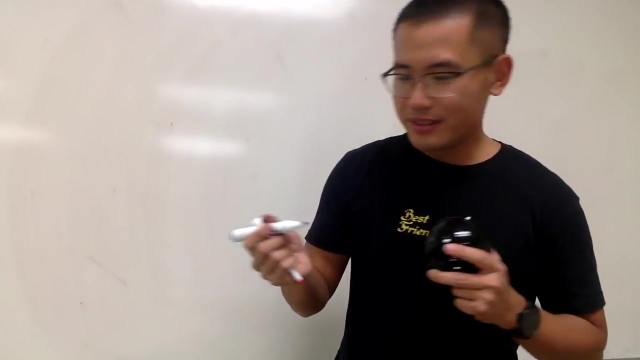 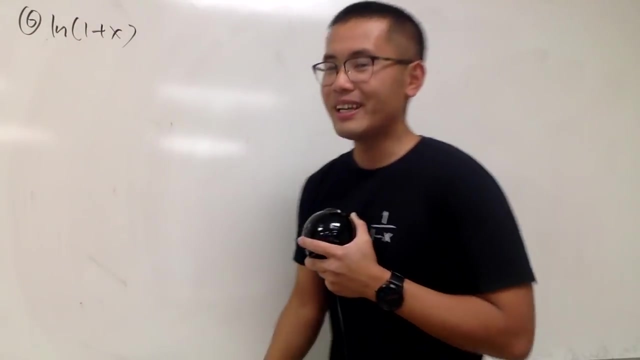 That was number 5, yeah, Now we are going to take this into a different style, Number 6.. Here we go. Natural log of 1 plus x Man. natural log, And this time at the center again: 0.. 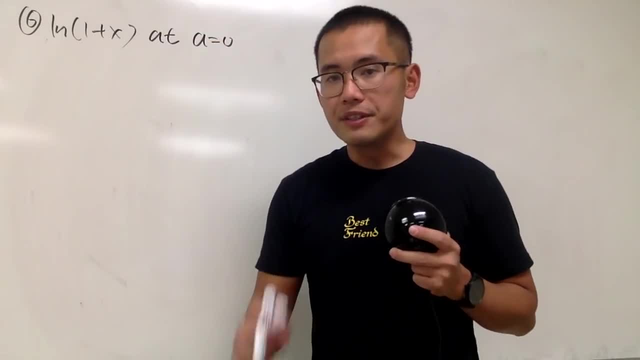 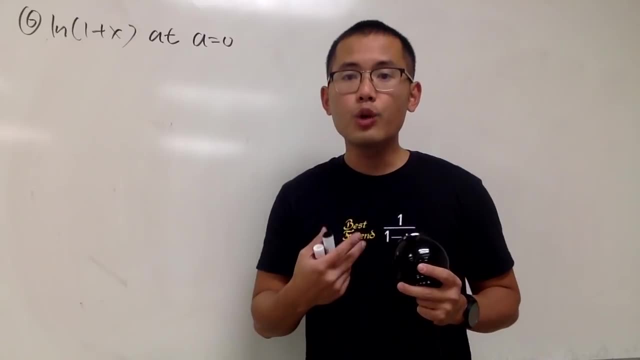 Don't worry, Later on we'll be doing the different center First thing first. Is there any connection between our best friend and the natural log? It seems like it, Because if we integrate 1 over a linear function, we can get natural log. 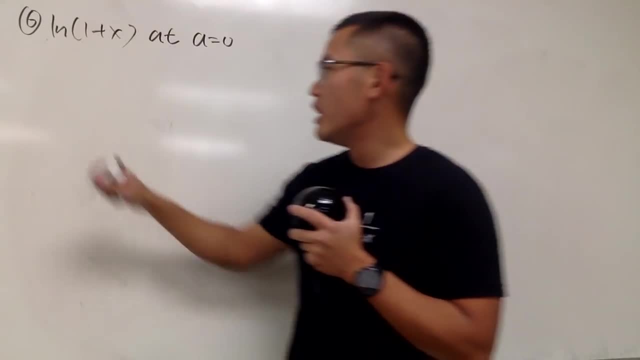 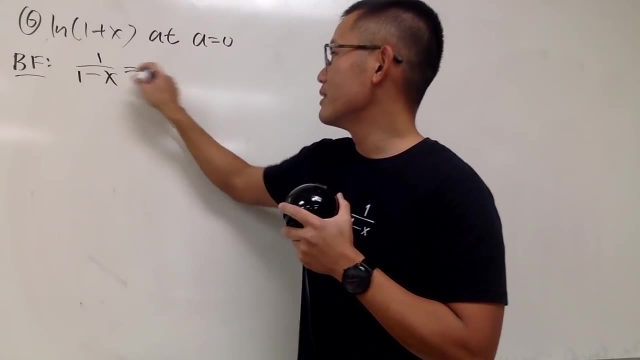 Right, So this is what we are going to do. Let's look at the best friend again. We know that this is 1 over 1.. Let me just write down everything in black. So we have this. Well, actually in this case, I need a red. 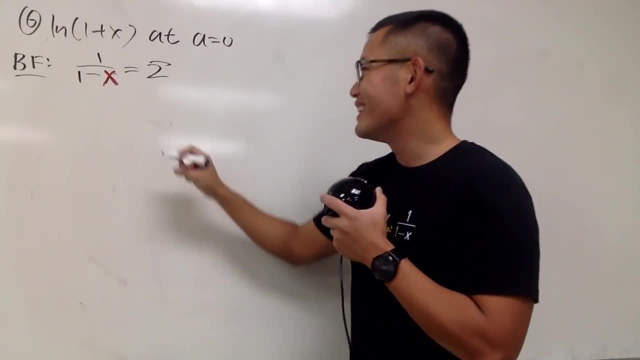 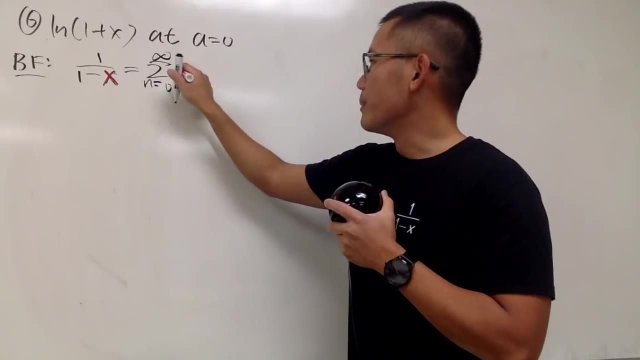 Earlier, I didn't need a red, But yes, this is what I want to do. This is the best friend. n goes from 0 to infinity parentheses. I mean x to the nth power. Like this, Absolute value of x is less than 1.. 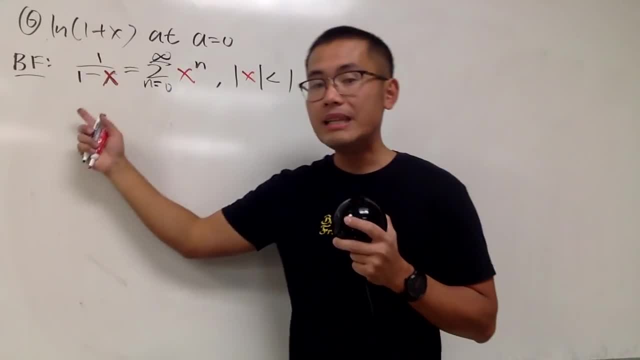 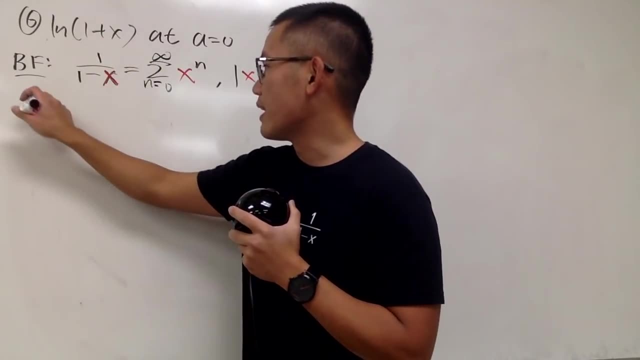 Right Now I need the best friend's cousin, Because the input here is 1 plus x. I'm not going to integrate this right here. This is okay, though I will just write this down: 1 over 1 plus x. 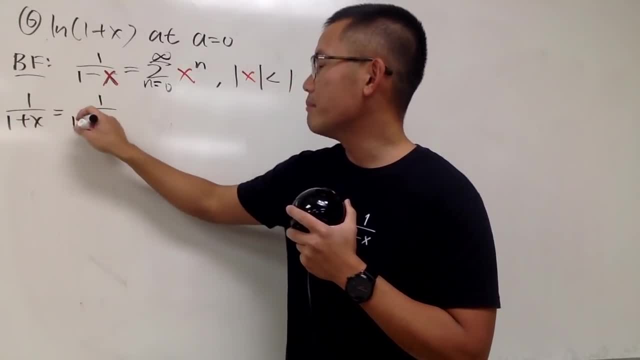 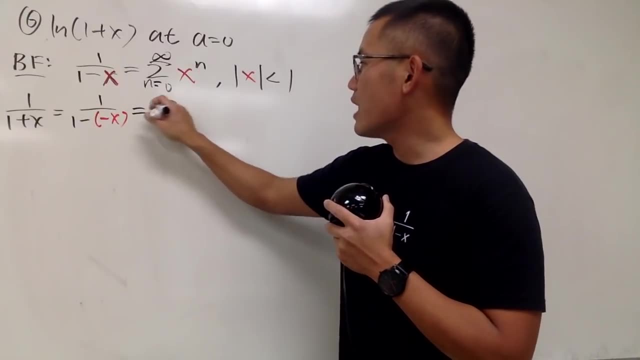 This is the same as 1 over. you know the deal: 1 minus parentheses, negative x. So I can put a negative x in here. This is the sum: n goes from 0 to infinity, parentheses negative x to the nth power. 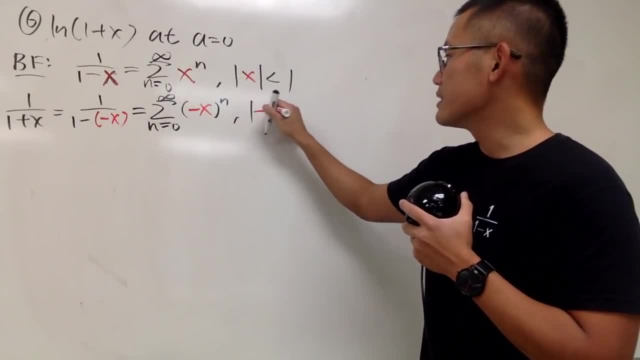 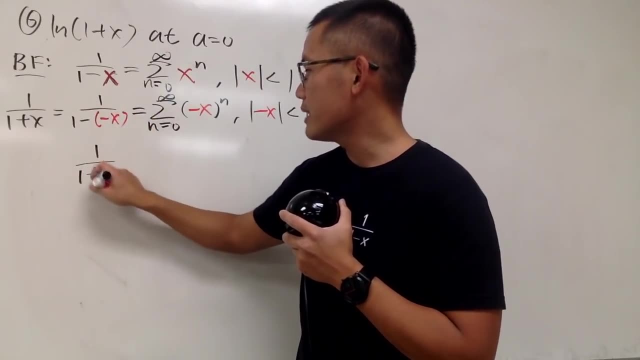 Yep. And then, of course, don't forget to put the negative x in the absolute value to be less than 1.. Now we are going to focus on this. The difference sign is 1 over 1 plus x, The right-hand side. this is the sum. 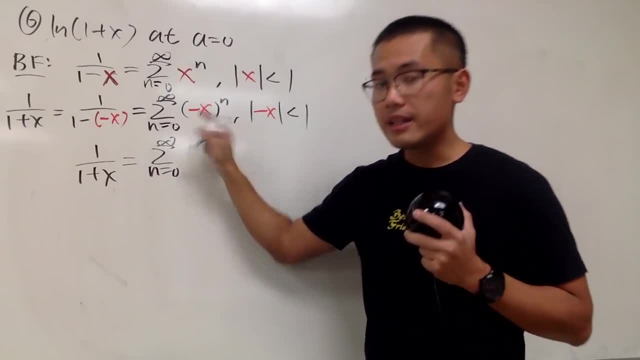 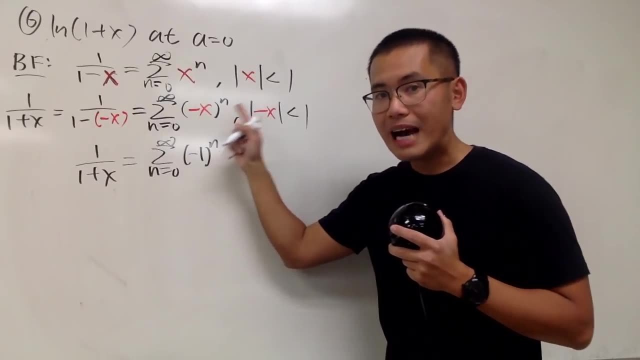 n goes from 0 to infinity And again just kind of separate the coefficients and also x to the power. This is negative 1 to the nth power And we have x to the nth power Like this. Now purple pen's time. 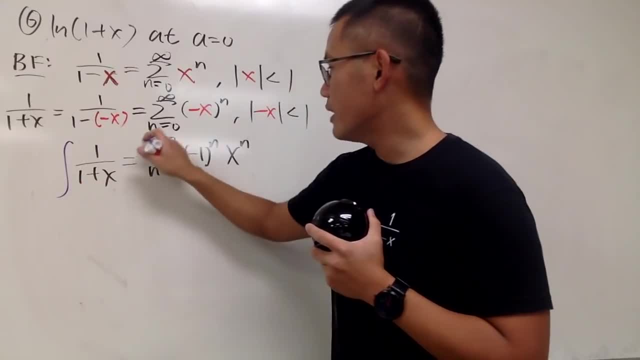 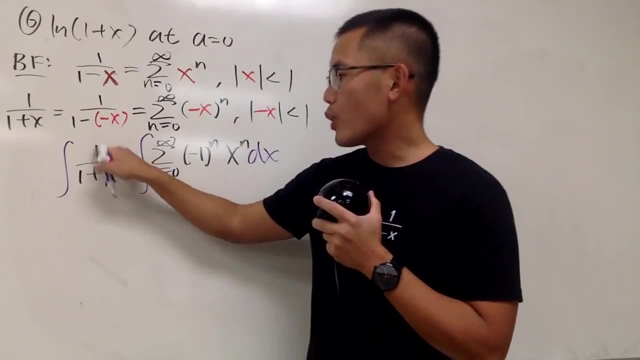 We are going to integrate both sides. Go ahead and do it right here and right here with respect to x, namely in the x world On the left-hand side, when we integrate 1 over linear function, we do end up with the natural log we want. 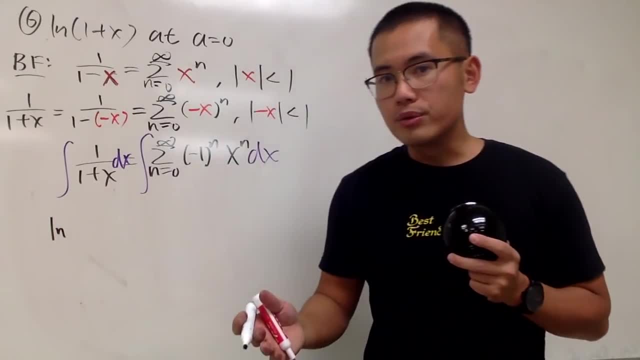 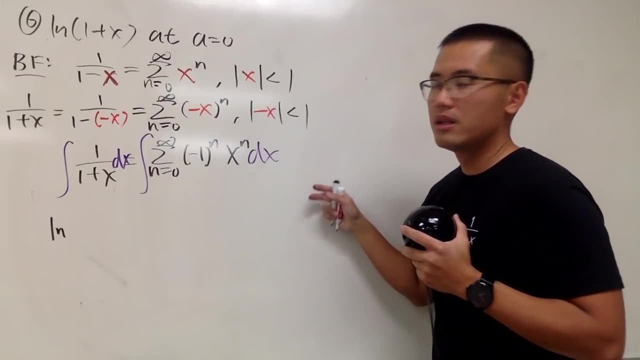 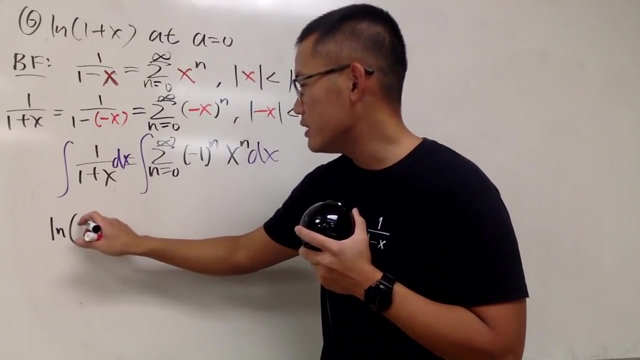 Very nice. We have natural log And you don't need absolute value. because we are on this interval, Absolute value of positive x will be less than 1.. So this 1 plus x will always be positive in that unknown interval. So we just need regular parentheses. 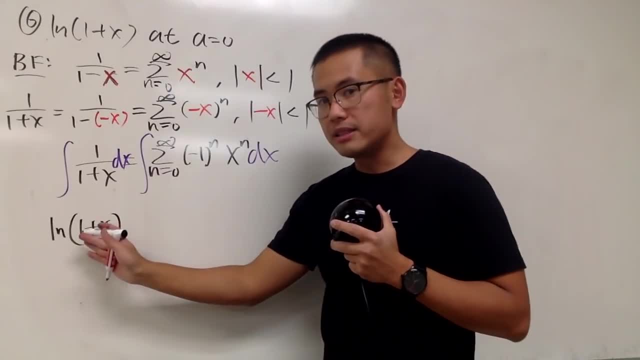 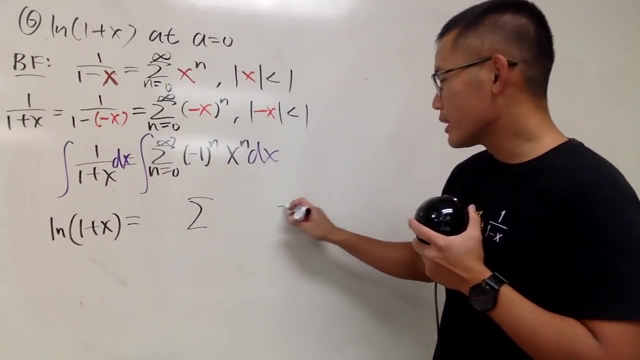 1 plus x, like. so Don't worry about the plus c, Just worry about the plus c on the right-hand side. But you know we are going to get a summation like this, right, I'm not going to put down the plus c at the end. 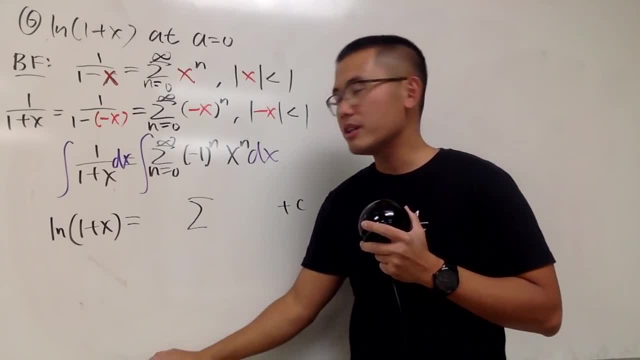 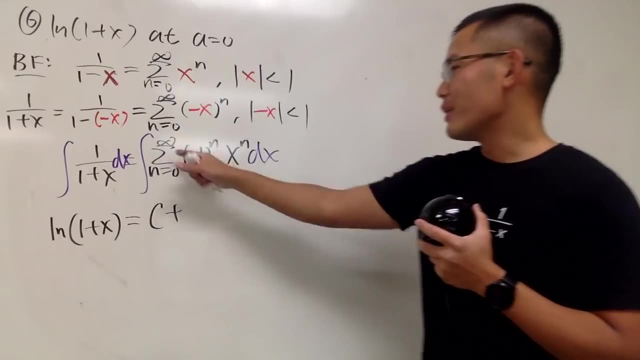 because sometimes this might look like it's belonging inside of the summation. Well, the way to fix that is: you put down c plus first. Okay, Now integrate this guy. We still have the summation. This time we don't lose any terms. 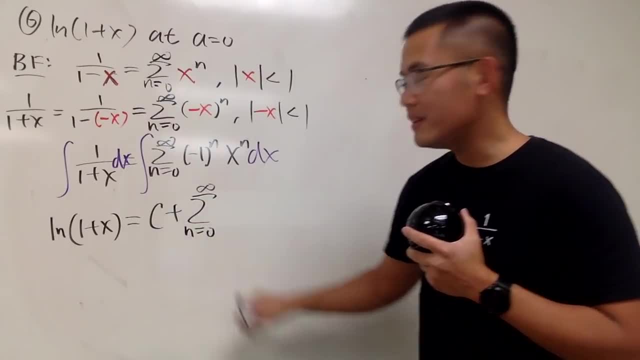 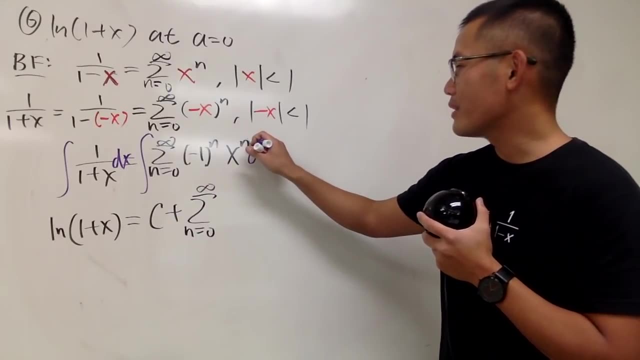 We will still have. n goes from 0 to infinity. Now to integrate a power series: it's just as easy, because all we have to do is look at the power right here. We just add 1. And that's a new power. 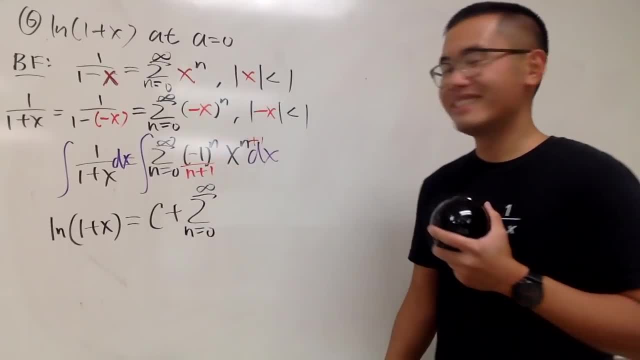 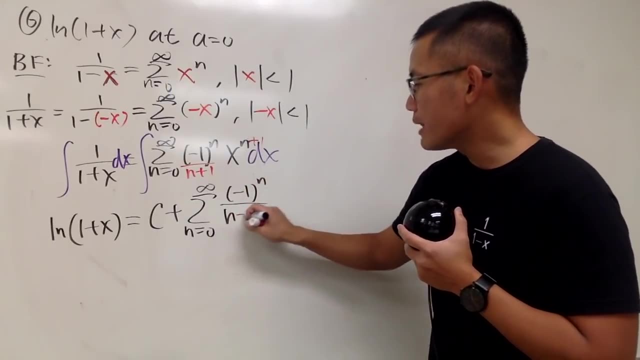 And then come here: divided by the new power, That's it Very nice. So here we have the coefficient, namely negative 1 to the nth power Over n plus 1. And then we have x to the n plus 1 power. 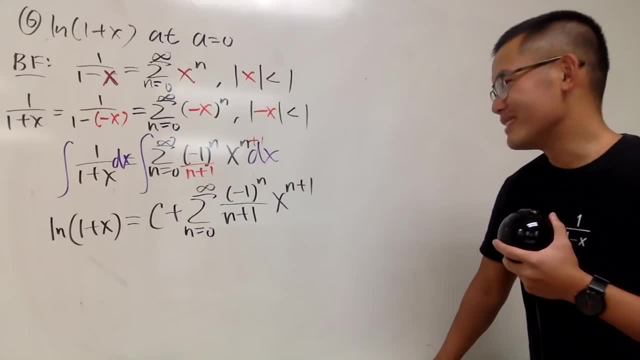 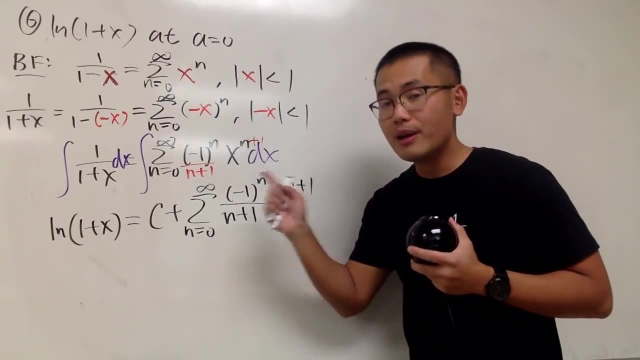 Man Love integrating things. power series. Who doesn't right? Okay, So that's pretty much it, And we will worry about this later. However, though, we still have to find out what the c is To do so. 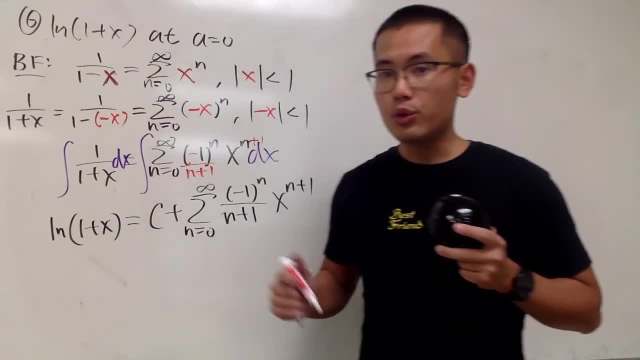 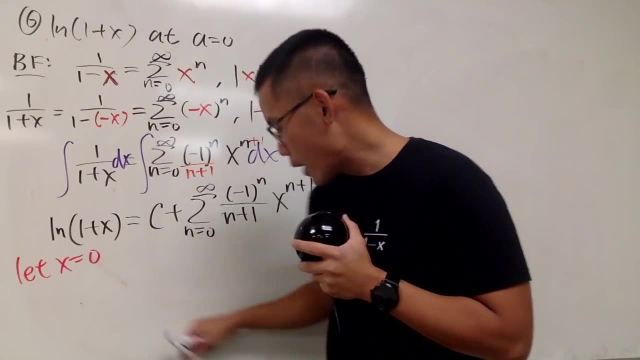 because the left-hand side is a known function. so we can do the following. I'm just going to pick an easy enough x value for us to use: 0,, of course, Because that way the left-hand side is going to be ln of 1 plus 0.. 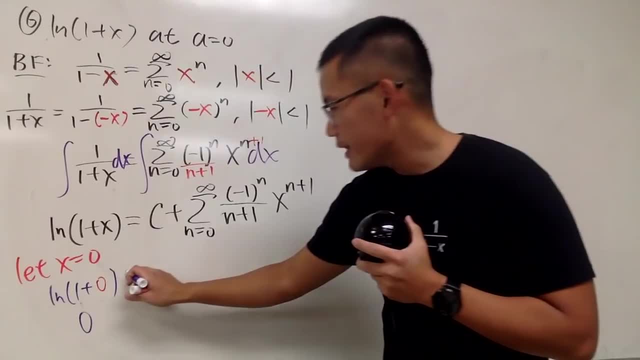 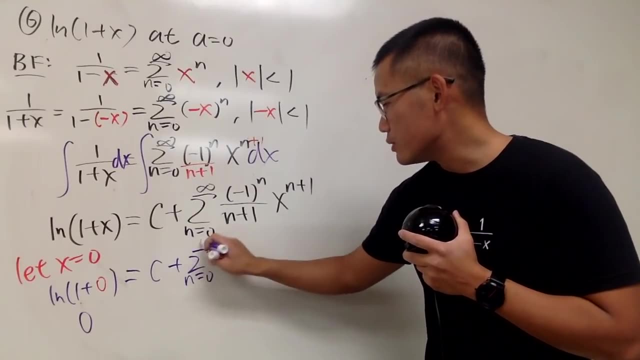 And that's of course just 0.. Now the right-hand side. this is c. I will enter the 0 right here. So we plus sum as n goes from 0 to infinity, write this down: negative 1 to the nth power over n plus 1.. 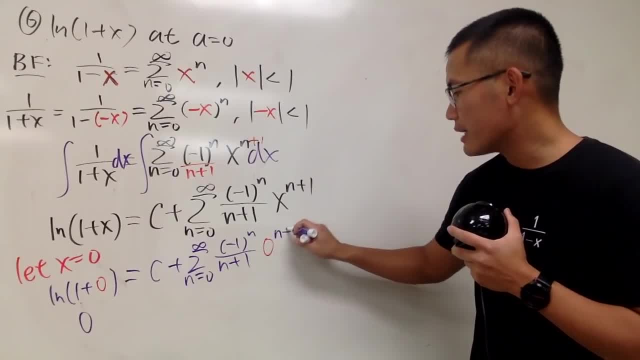 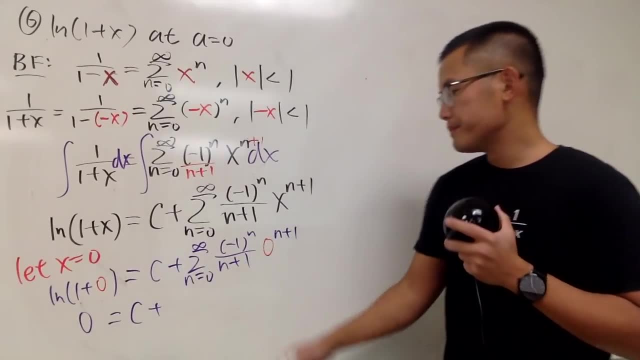 And then put the 0 right here, so we have 0 to the n plus 1 power. The left-hand side is 0 right there already, and this is c plus Well. well, When n is 0, that's the first term. 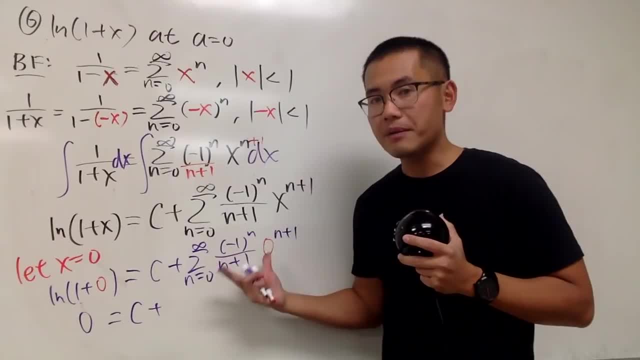 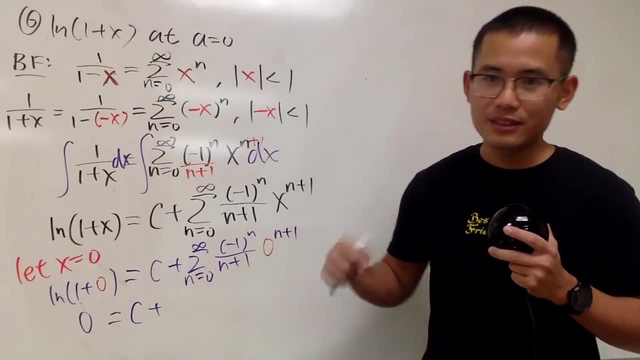 Put it here: you have 0 to the first power, so that means that term is 0. And then, when n is 1, again you get 0. And then so on, so on, so on. You get infinitely many solid, exact 0s. 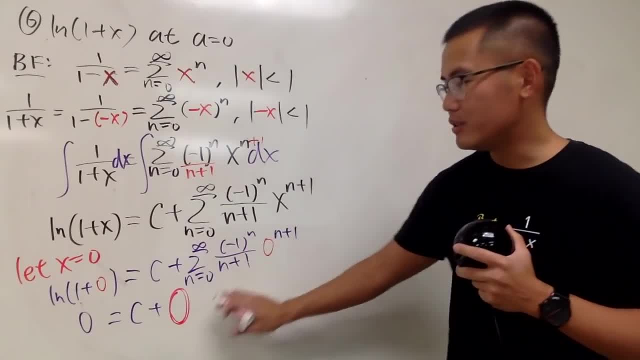 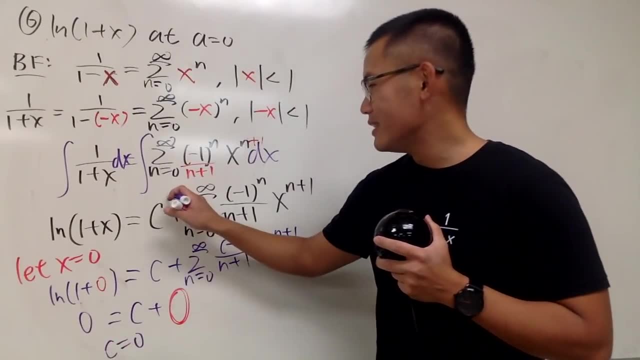 Add them up, you get 0. So this is just going to give you 0.. In another word, c is just nicely equal to 0.. In another word, this c is just equal to 0.. Oops, Well, yes. 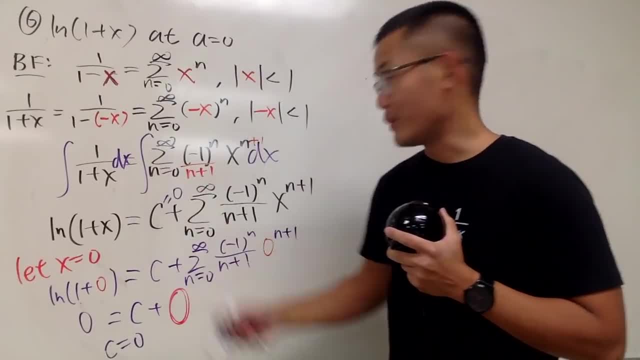 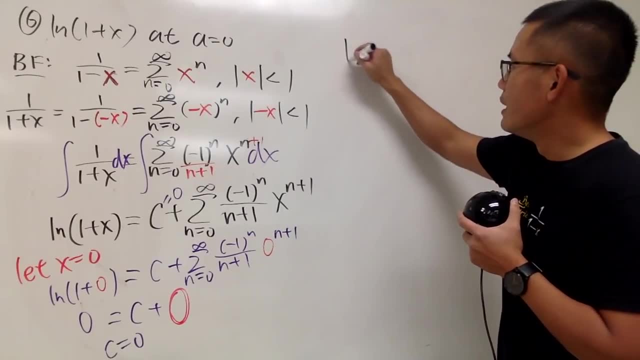 No, no, It looks like c is equal to e. There we go. Okay, so c is equal to 0.. Finally, I can come here and tell you the absolute, not the absolute value, ln of 1 plus x. 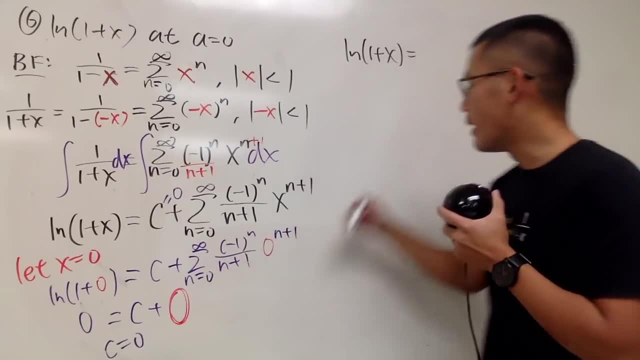 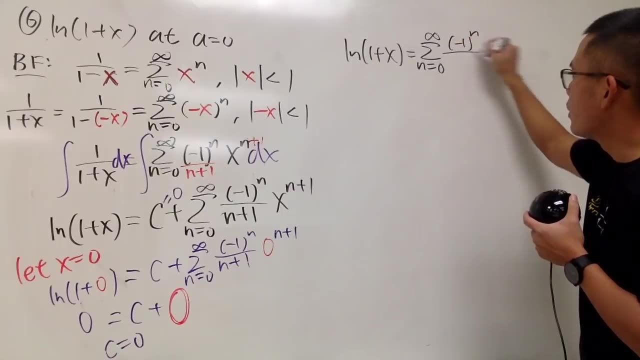 this right here is nicely equal to just this part. The sum as n goes from 0 to infinity and we have negative 1 to the nth power over n plus 1 times x to the n plus 1's power, Like this: 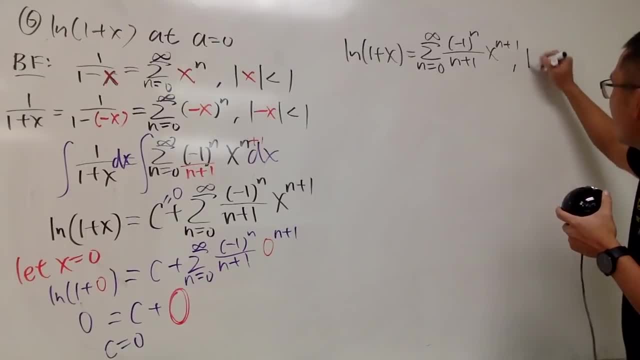 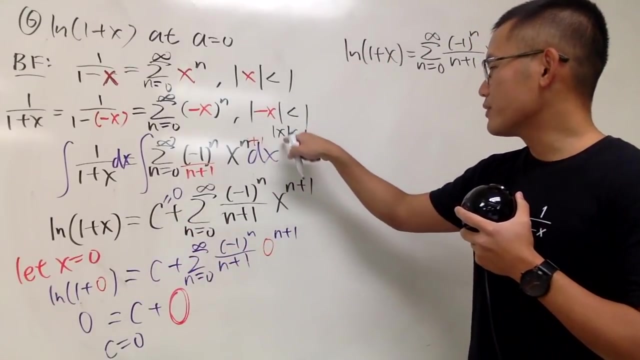 Very nice, Now r. well, when we integrate we'll differentiate power series. the r will stay the same. Earlier we integrate the best friend's cousin, which the r is still. you know less. the absolute value of x is 1,. 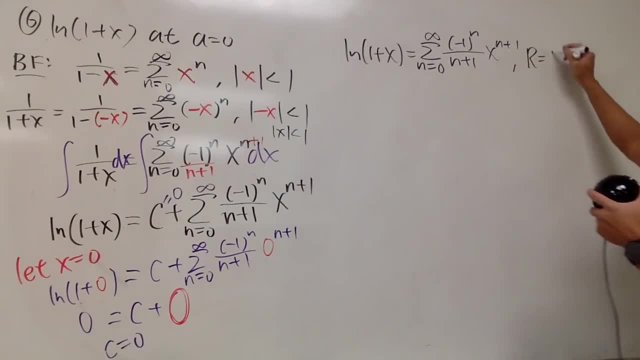 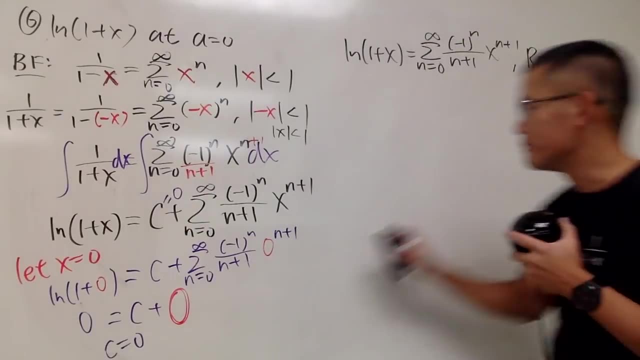 less than 1.. So r is still equal to 1.. r is 1.. Center was at 0, so we go from negative 1 to 1.. For the i let me just write some better. I will be going from negative 1 to 1,. 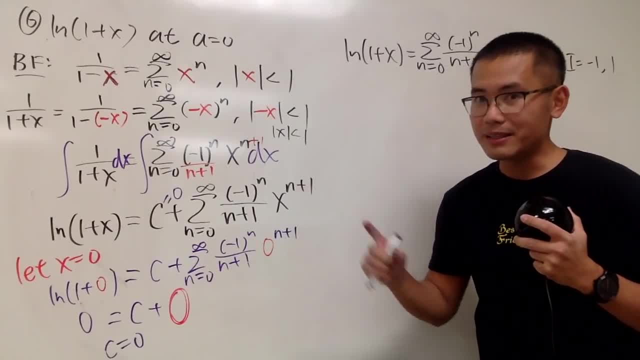 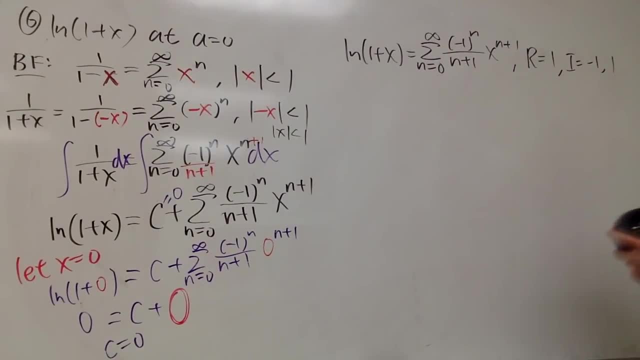 but I don't know about the endpoints. It's not parentheses anymore. you'll see Again, we will have to do what we did earlier for the check. Let me check negative 1, right? So I will just tell you. 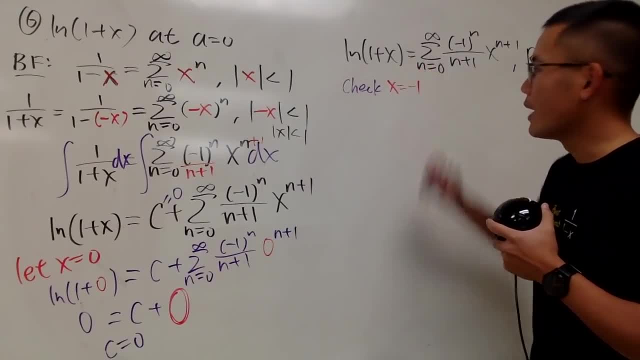 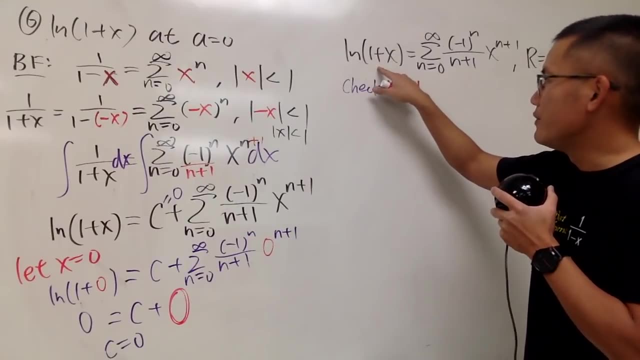 we are going to check when x is equal to negative 1.. Well, well, this is a quick check that we can do. If you put negative 1 into the function right here, ln of 1 minus 1 is ln of 0,. 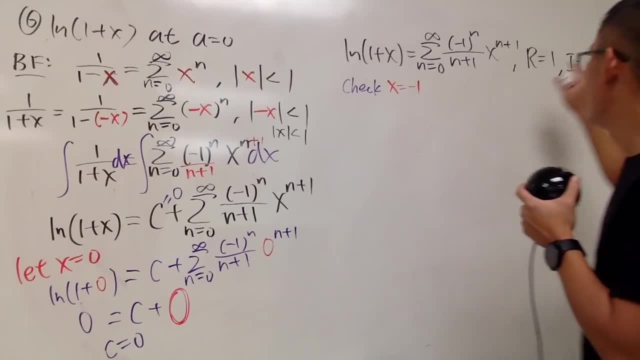 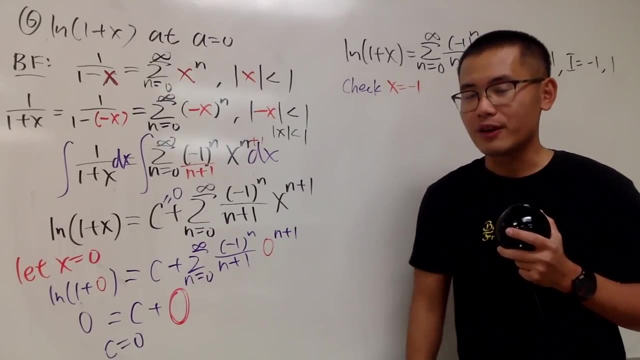 it's undefined, It's bad, So it's not going to converge for sure. But do not just rely on the function every single time. Right, Do not rely on the function every single time, Because if the function doesn't work, 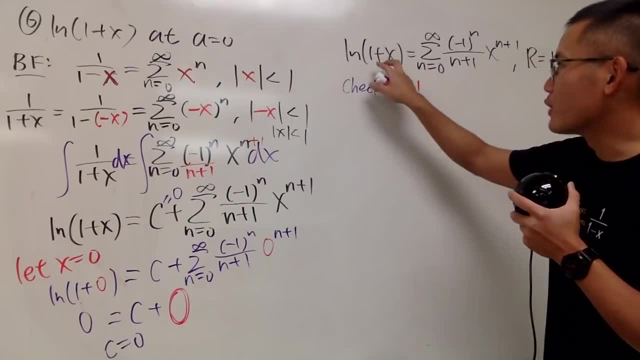 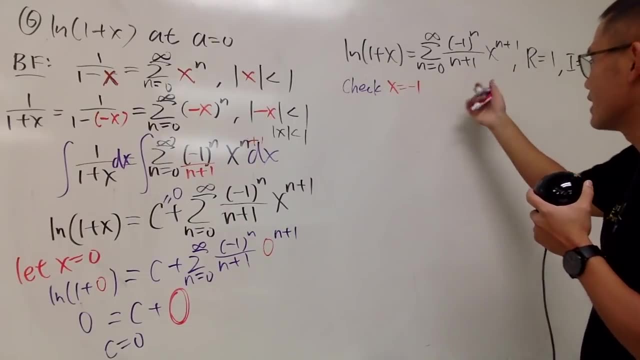 yes, the power series won't work, that's for sure. But if the function works, it does not mean that the power series will work. Okay, So I will still show. you put the negative 1 right here. So let's just look at this. 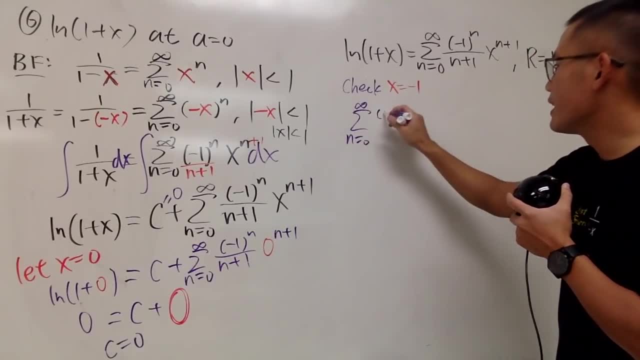 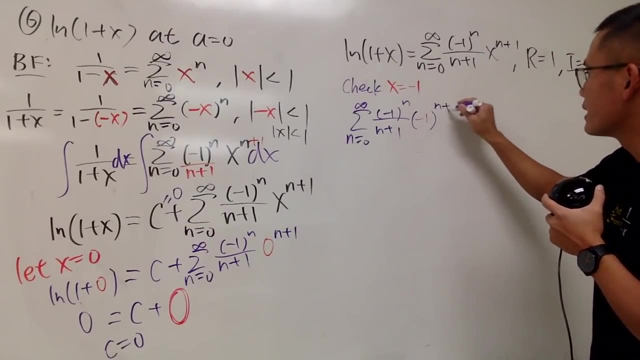 The sum as n goes from 0 to infinity. we have negative 1 to the nth power over n plus 1.. And put the negative 1 here. we have negative 1 raised to the n plus 1's power, like so: 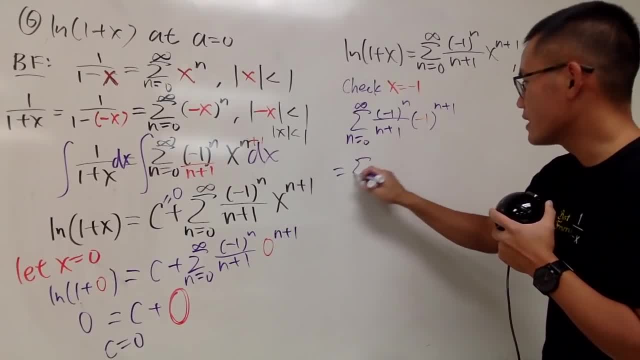 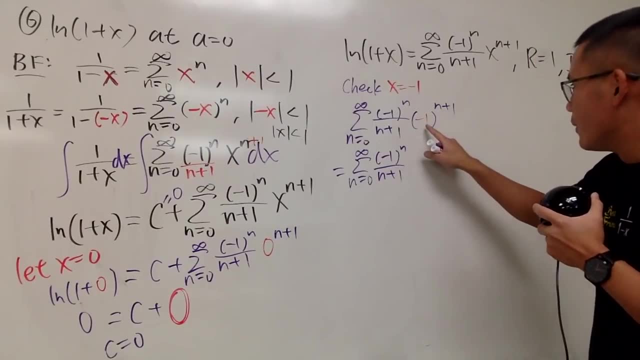 And then just simplify this real quick. This is the sum as n goes from 0 to infinity. negative 1 to the nth power over n plus 1.. Well, well, this right here is what This is: negative 1 to the nth power. 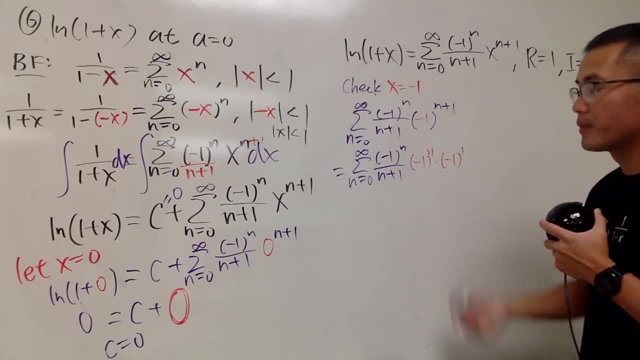 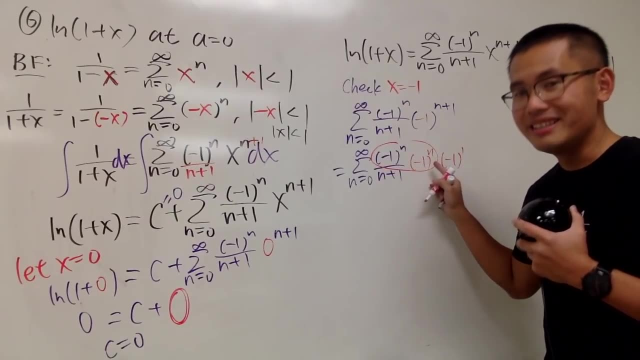 times negative 1 to the first power, right. Good, Now check this out. This part- negative 1 to the n times negative 1 to the n is negative 1 to the 2n. So let me just write this down. 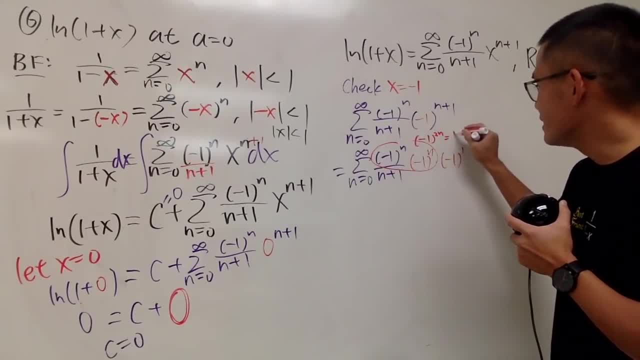 This is negative 1 to the 2n. This means it's always 1.. So they pretty much cancel out. We just always get 1.. But we have the negative right here though: Negative 1 to the first power. 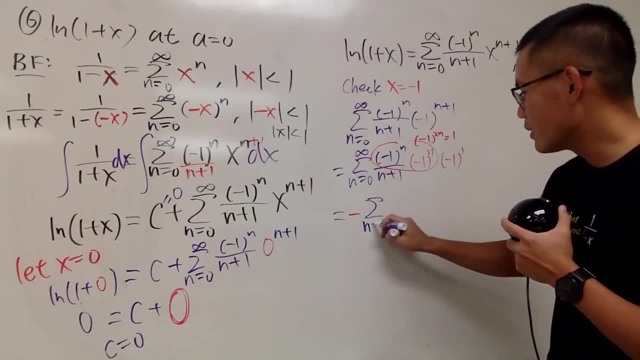 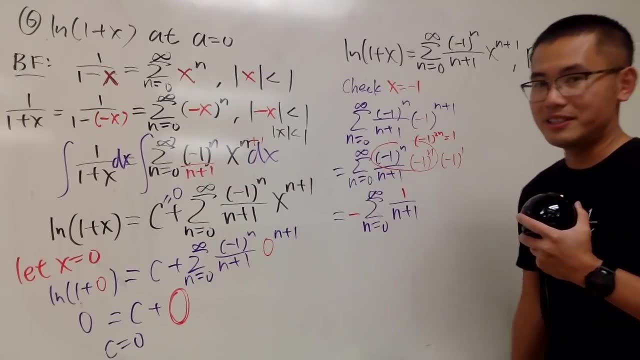 so we have this negative in the front and then we have the sum n goes from 0 to infinity. Again, this is just going to give us a 1, and then over n plus 1, like this. Now, does this converge? 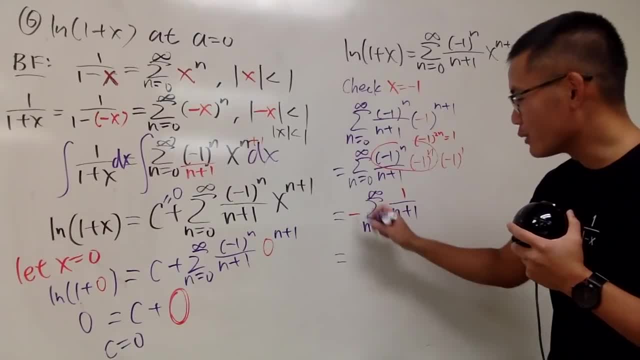 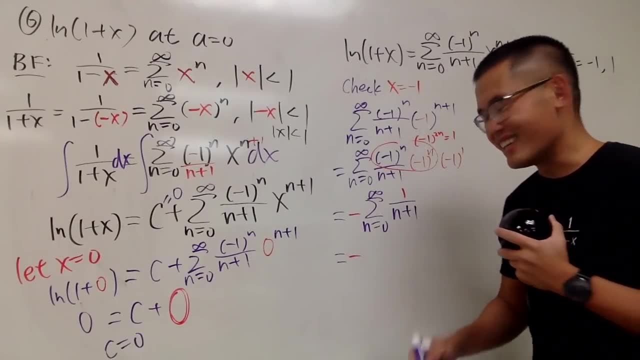 No, it does not, Because if you write it out real quick- this right here is actually- well, you don't need to write it out. you can do the trick that I showed you guys earlier. Let me do that with you guys again. 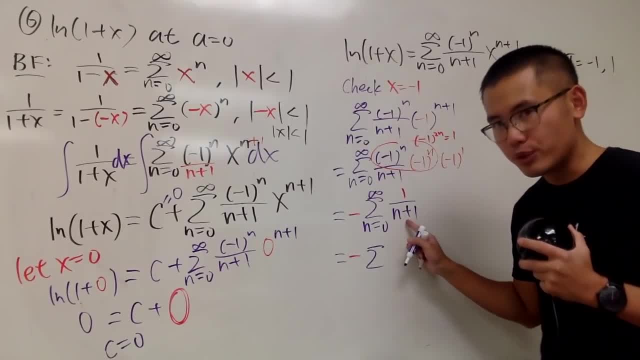 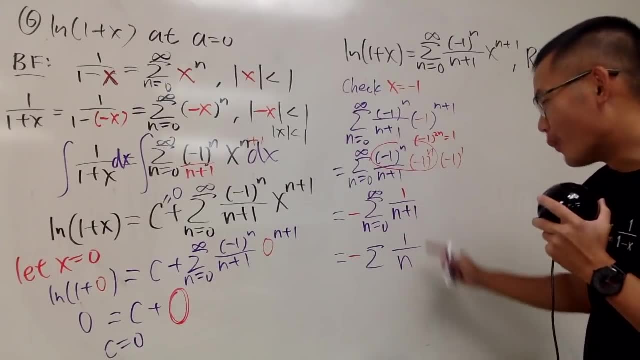 This right here is the sum. Let me minus 1 to the n, so I get 1 over n. only because n plus 1 minus 1, you get n. Well, to balance it, we will have to add 1 here and here. 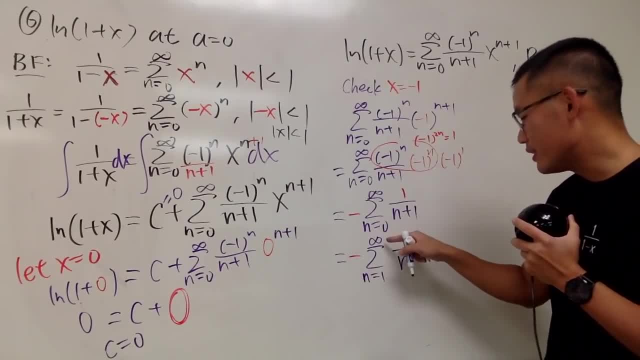 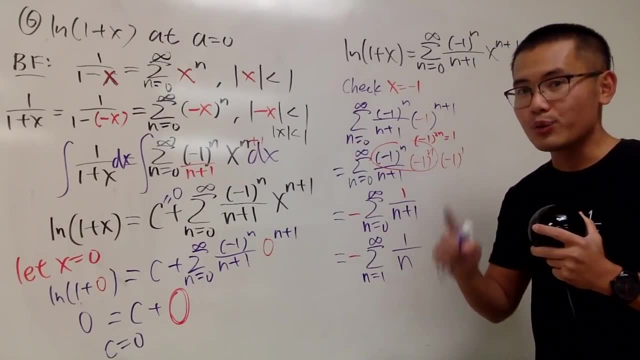 so we get: n is equal to 1, 2 infinity plus 1 is still infinity. Now does this look better? Yeah, this is the what p-series when n is equal to 1.. Or you can also say: this is the harmonic series. 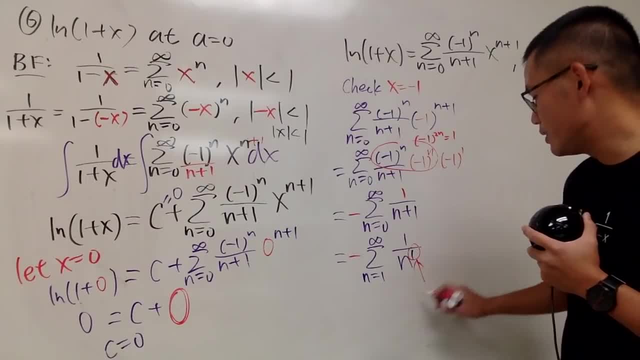 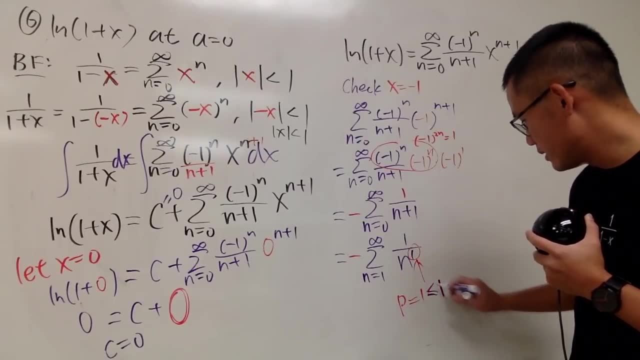 Well, this right here, I will just call this to be the p-series You just use that p is 1, which is less than or equal to 1.. Like this. Well, of course, it diverges. and when you have negative times. 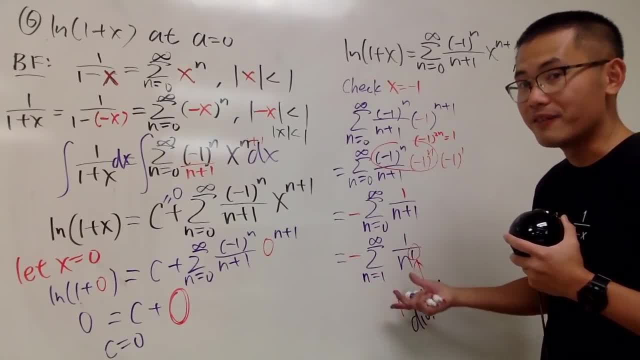 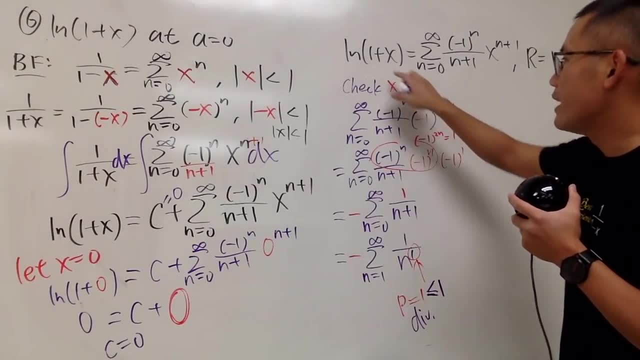 this actually goes to infinity. so you actually get negative infinity. But it doesn't matter. Right here, do not include negative 1. Again, you could have just say: because the function doesn't work, of course the series doesn't work, right. 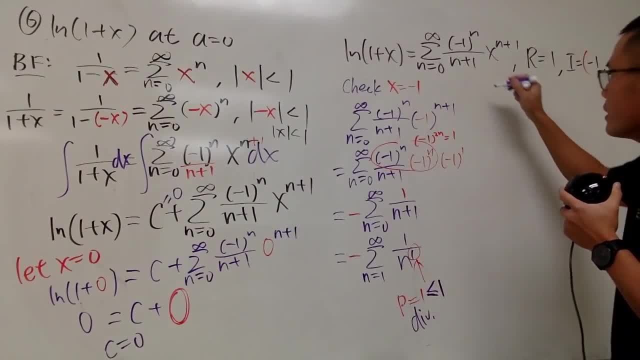 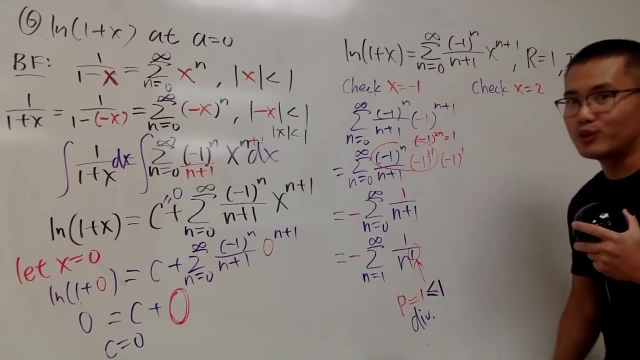 In that case. But let's check the next one. Check when x is equal to 2.. Well, does it converge when x is equal to 2?? I put the 2 right here, I get ln of 3. It works. 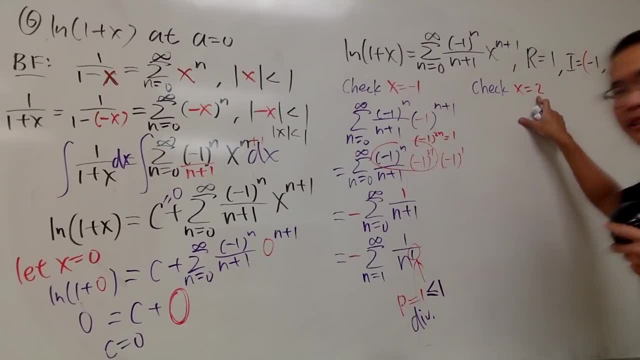 But no, Because this is outside of the interval of convergence already. So do not just use the function. Do not just use the function. I will put a 1, not only in the function but actually right here, So be sure you really use the series. 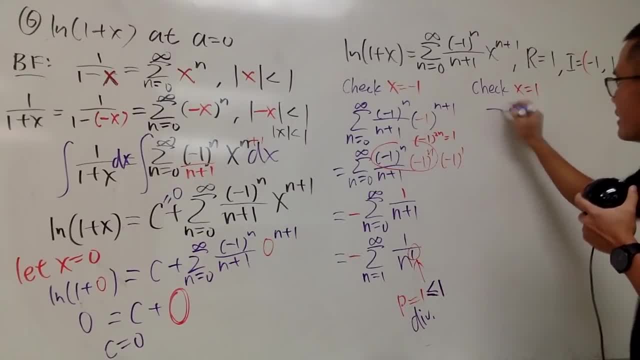 Put a 1 in here. So we are looking at this. one is the series as n goes from 0 to infinity And this is negative. 1 to the nth power over n plus 1 times 1 raised to the n plus 1th power. 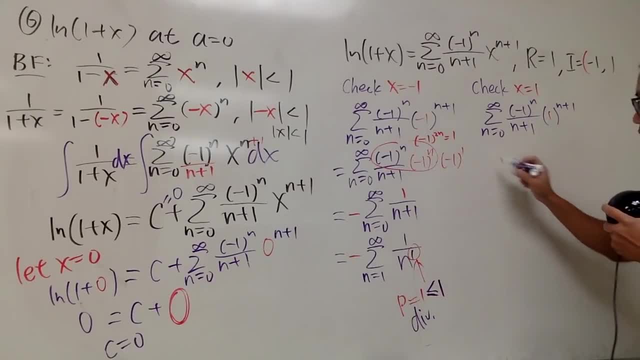 The good thing is that this is always 1.. So that's good. So we have the series as n goes from 0 to infinity. Put this on the side, Because I like that- And then right here we have the 1 over n plus 1.. 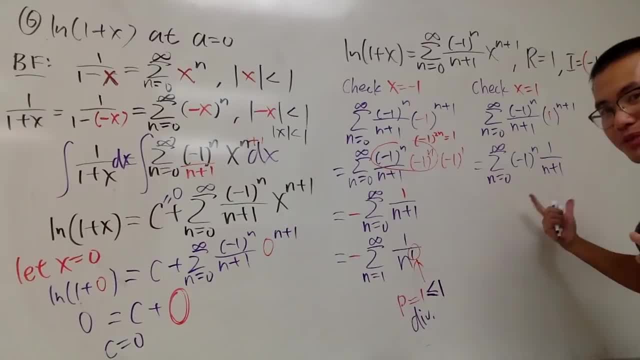 Like this, In fact this right here, we get the alternating series Right Because we have this. So I will call this to be the bn To check, The first check. I don't know why I put down 2 first. 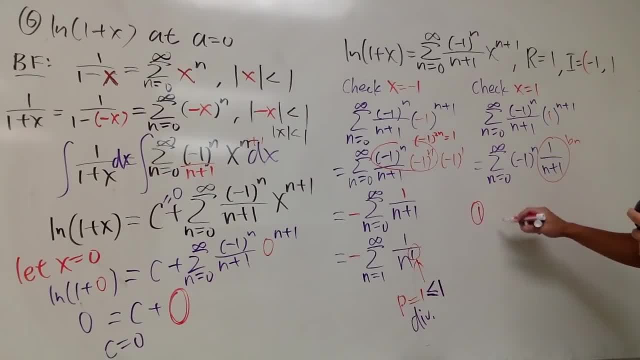 First check: Does bn go to 0 when n goes to infinity? So let's go ahead and say: as n goes to infinity, bn which is 1 over n plus 1, does this go to 0? It sure does. 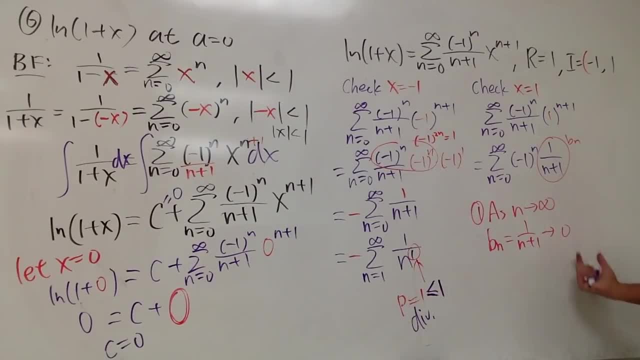 Because if you put infinity on the bottom 1 over infinity, it's clear that it goes to 0. So the first check checks: Secondly, do we have bn plus 1, less than or equal to bn? Namely, does bn decrease? 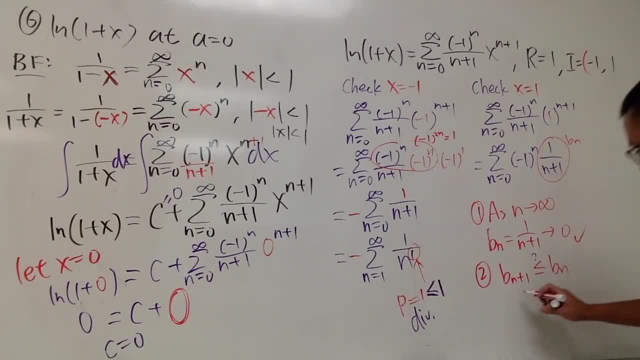 Well, if you put bn plus 1, n plus 1 in here, we get 1 over n plus 1.. Again, for this expression, just enter n plus 1 into this n. so we have that. But don't forget, we still have the plus 1 after this. 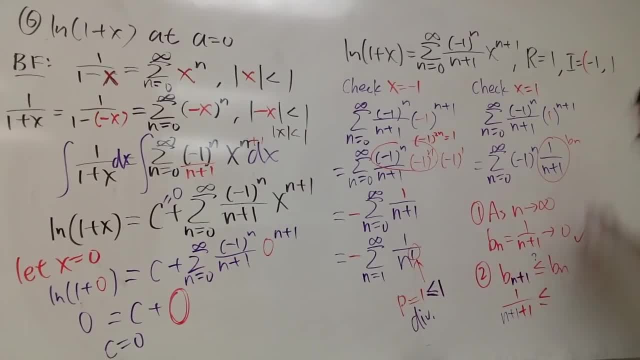 And this right here. is this less than or equal to the original bn, Namely 1 over n plus 1.. Well, you can cross multiply if you would like. This times that is just n plus 1.. Is this less than or equal to? 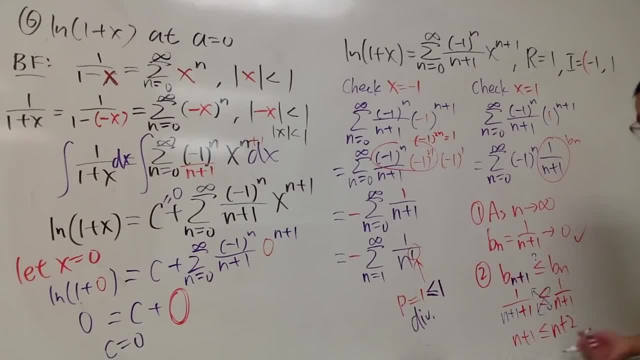 well, this times that is just n plus 2. And this is so true, isn't it? So checks. Therefore, this right here converges, this series, right here converges. let me actually put this down: right here converges. 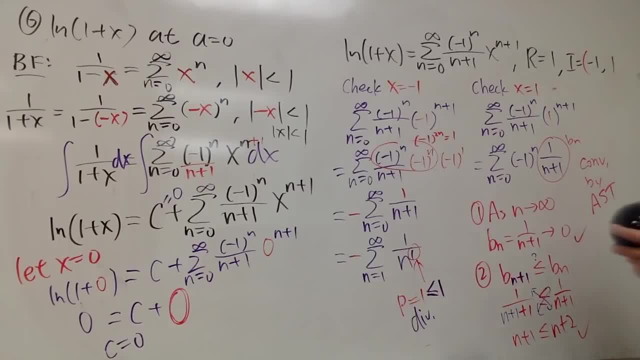 by the alternating series test, And perhaps this is what you have to show. I know it's a long question. Anyway, right here it converges. so you come here, you put down a bracket. That means you include the endpoint right here. 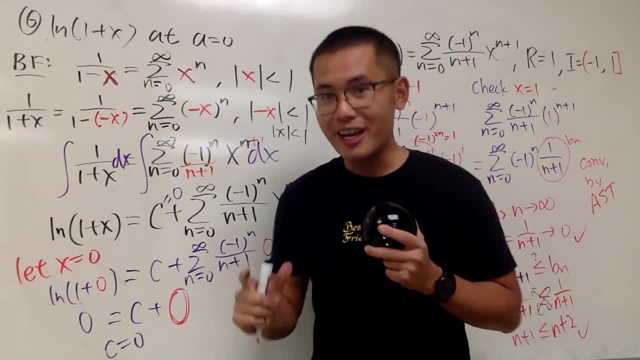 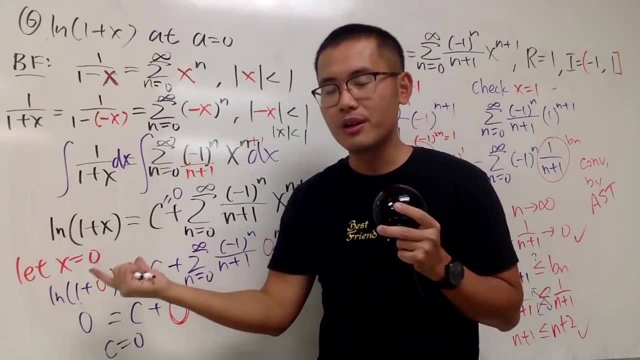 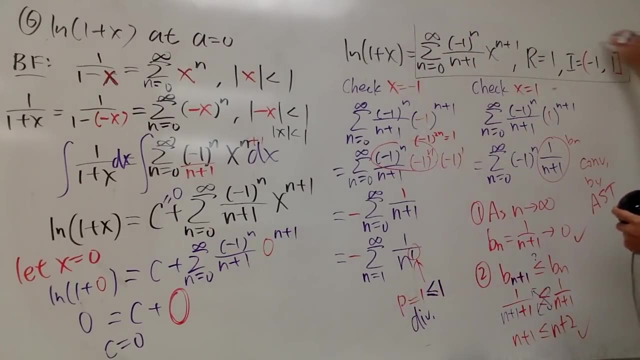 This is why I told you guys that you really have to check the convergence at the endpoint when you do calculus. with the best friend, We did the integration, which is the calculus step, so be sure you do this. Okay, so box this for the answer. 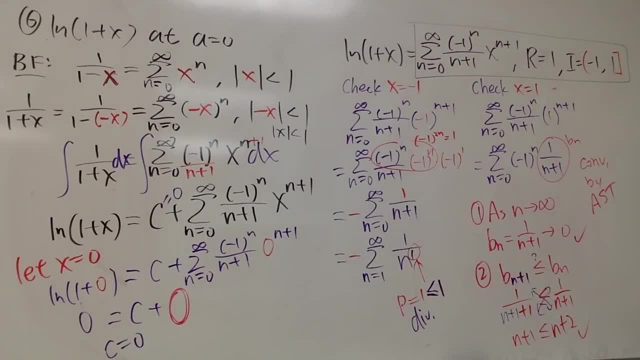 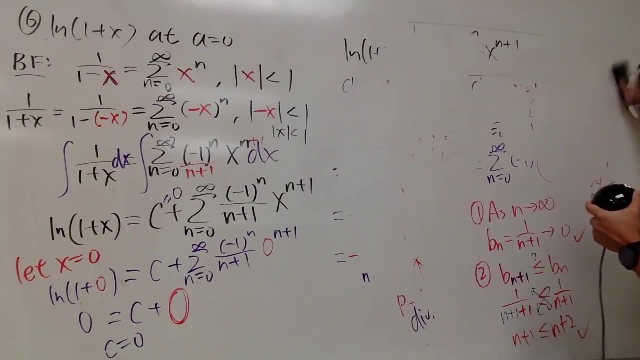 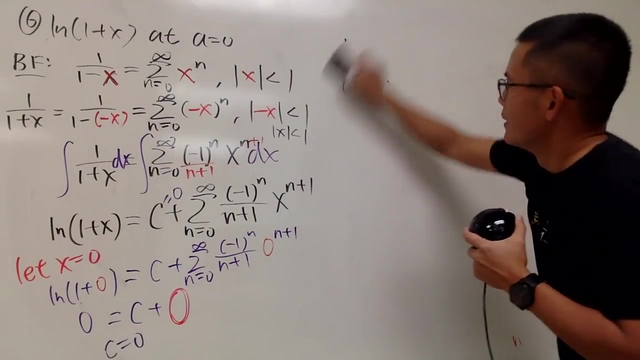 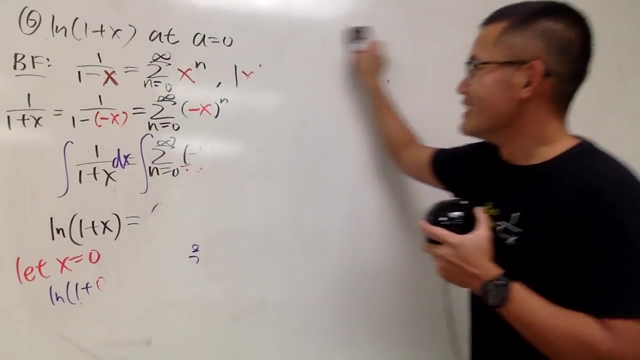 So take a look, take a look, take a look. Okay. so yeah, continue, continue, continue. We just have 20, something more to go. It shouldn't be taking too long. I don't know What's the next question. 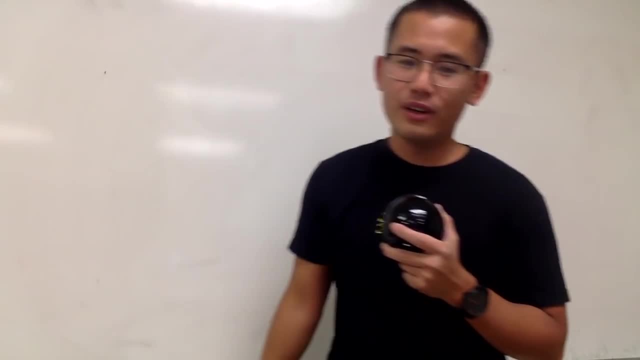 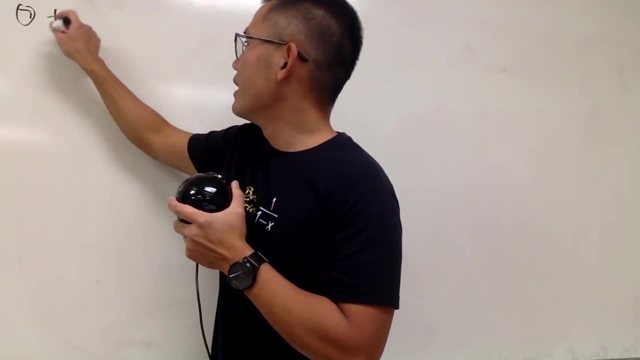 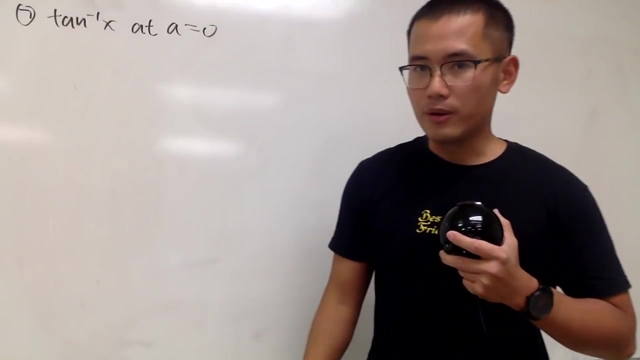 Let's see what's the next question: Inverse tangent. Oh my god, it's going to be another long one. Anyway, number 7, here we have the inverse tangent of x and the center is at 0.. Well, well. 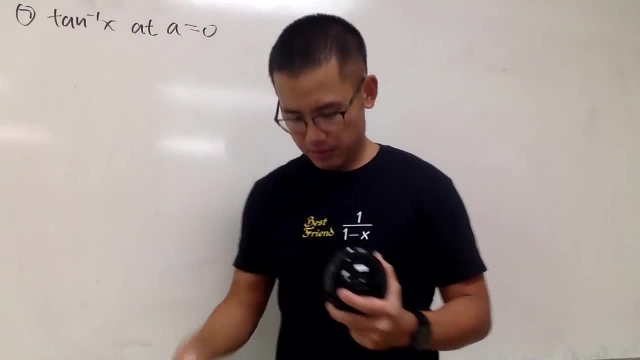 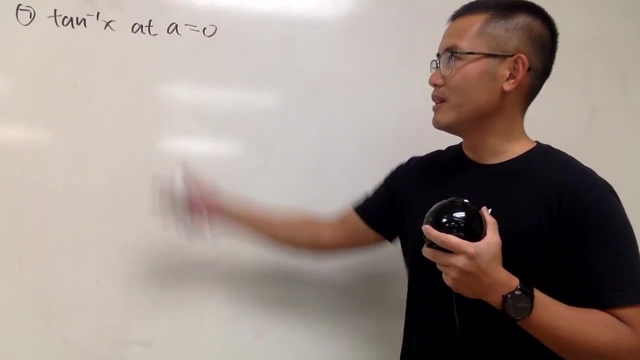 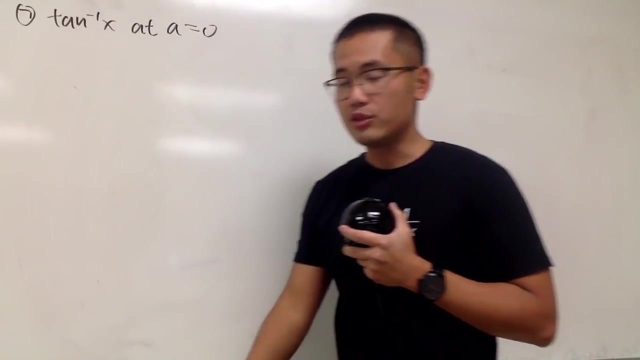 what's the connection between inverse tangent and our best friend maybe? Well, it doesn't have like direct connection, but it's like a long distance relative. you'll see, Because we know that if we differentiate inverse tangent we get what. 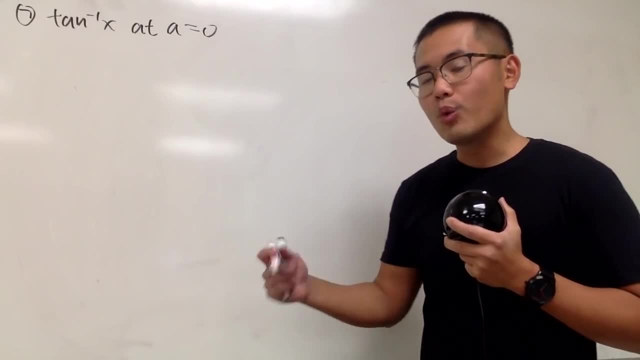 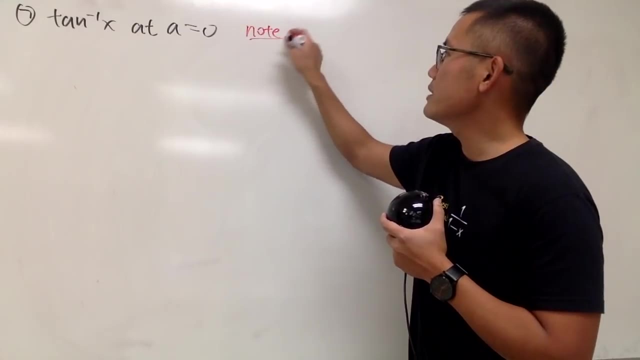 1 over 1 plus x squared. So if we integrate 1 over 1 plus x squared, we get inverse tangent. So the strategy is- I'll just put down a note right here on the side for you guys- If we integrate 1 over 1 plus x squared. 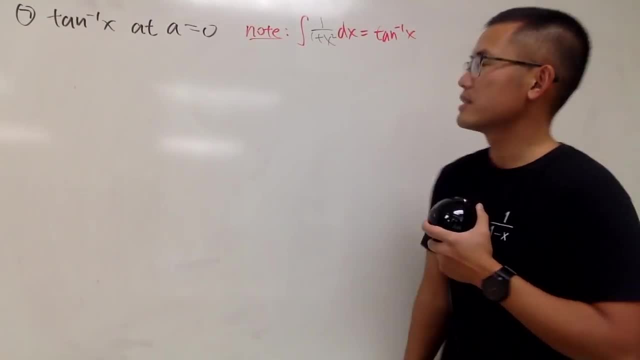 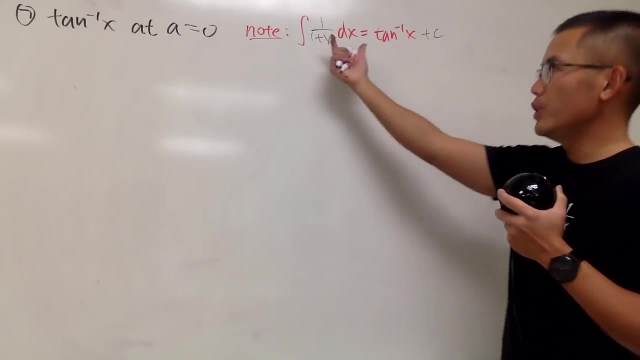 this will give us inverse tangent of x. Alright, And yes, I do know to put a plus c, Alright. so we'll just come up with a series for the 1 over 1 plus x squared and integrate that Yes. 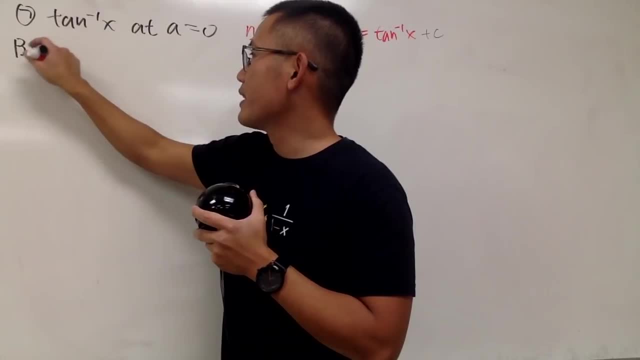 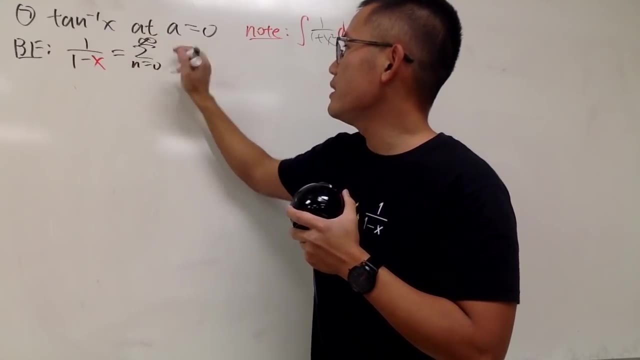 Alright, so go ahead. perhaps I'll just write down the best friend again: 1 over 1 minus x. This right here is the sum as n goes from 0 to infinity, x to the nth power. absolute value of x is less than 1.. 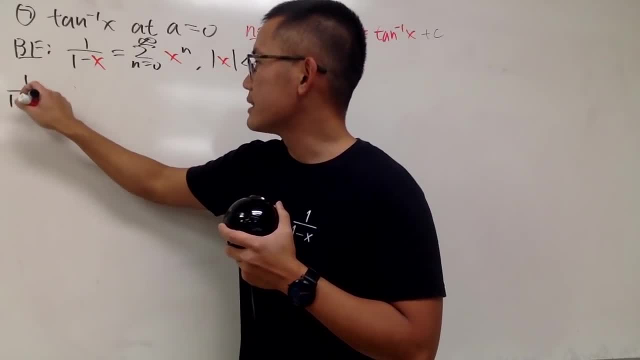 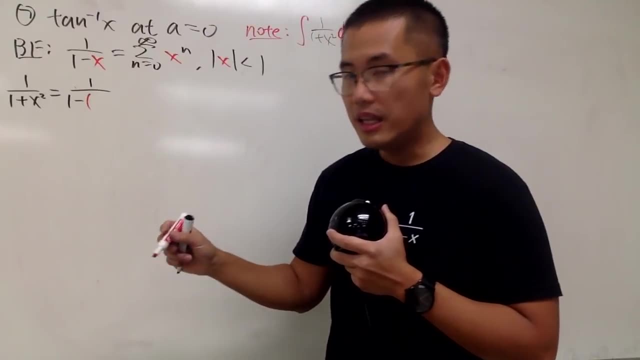 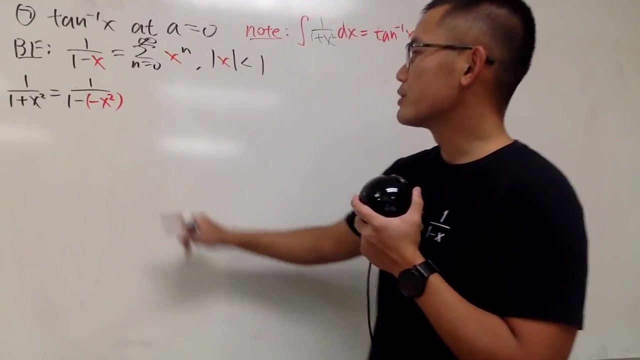 And now 1 over, 1 plus x squared. This is the same as saying 1 over, 1 minus parentheses, negative x squared like this: Okay, And then I'm just going to enter this right here, So we have the sum. 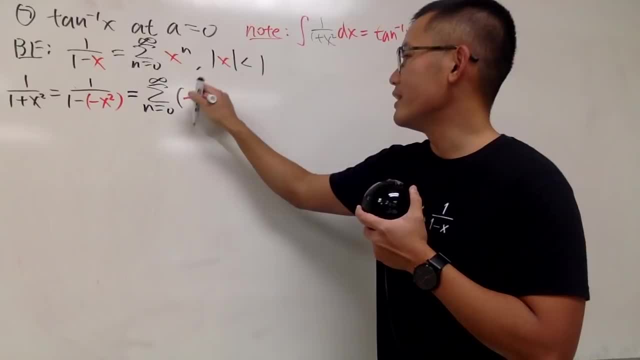 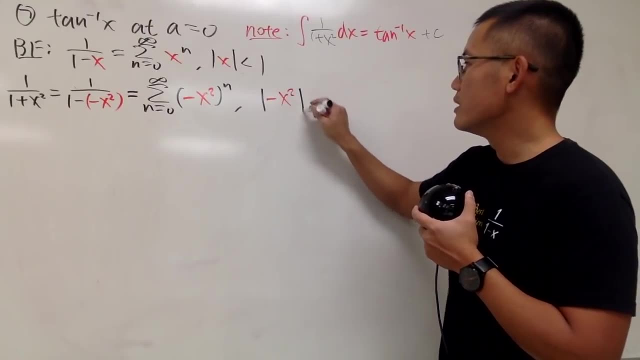 as n goes from 0 to infinity, parentheses that, and we have the negative x squared To the nth power. enter this into the absolute value. Absolute value of negative x squared is less than 1.. Good, Now work this out. 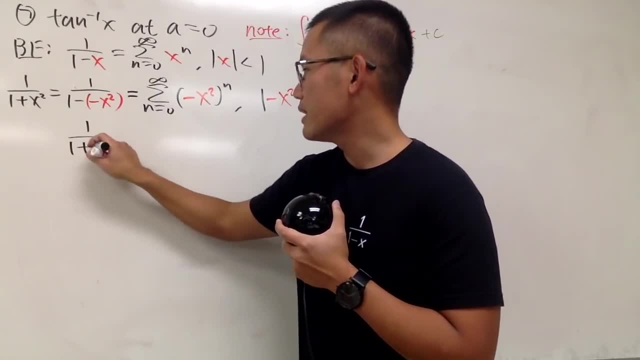 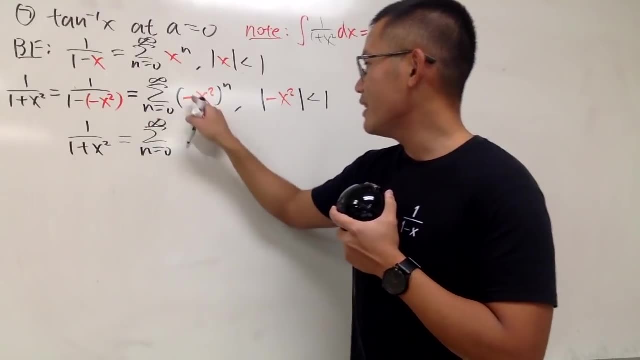 You see that this is, of course, 1 over 1 plus x squared, And simplify this a little bit. This is the series as n goes from 0 to infinity. We have negative 1 to the nth power, So I'll put this down nicely. 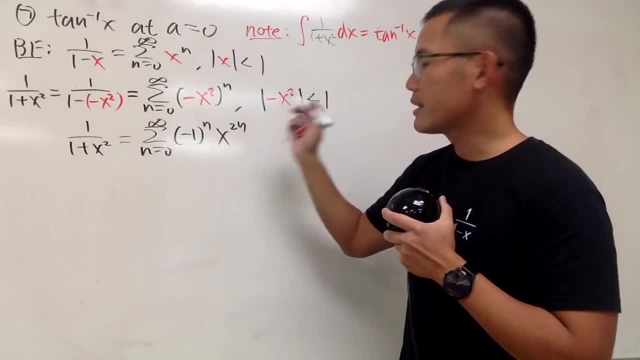 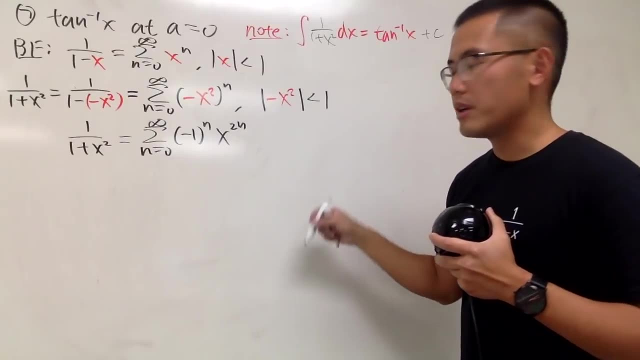 And then this is x to the 2 nth power like this, And, of course, when you have the absolute value of negative, it doesn't matter, And then you can take the square root, like what we did earlier. So, all in all, 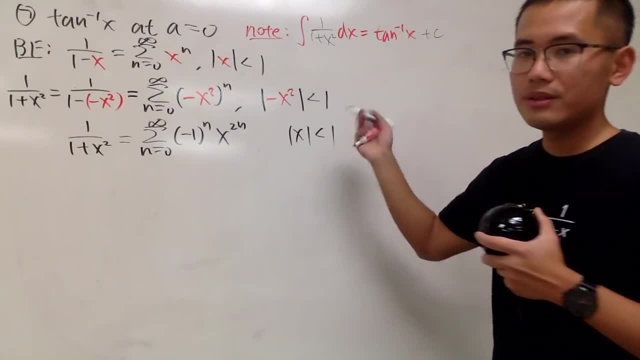 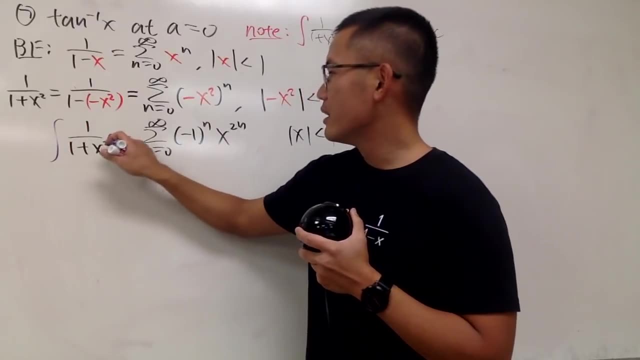 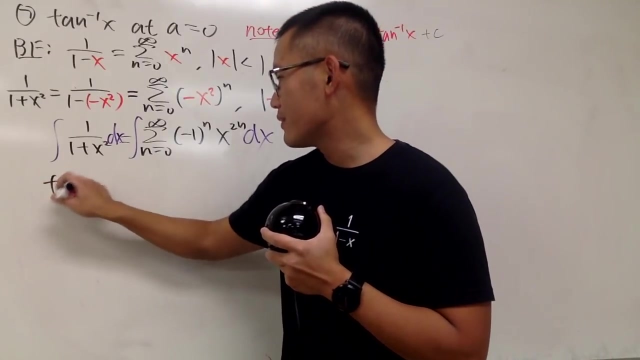 we get: the absolute value of x is less than 1.. Okay, So just some simple algebra for that. Now it's time for us to integrate. We will just integrate: integrate- Left-hand side inverse tangent. So here we have the inverse tangent. 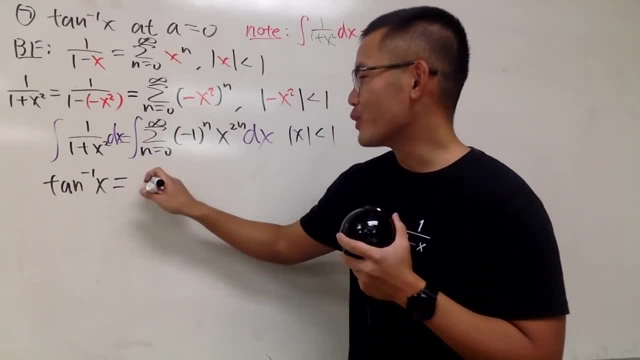 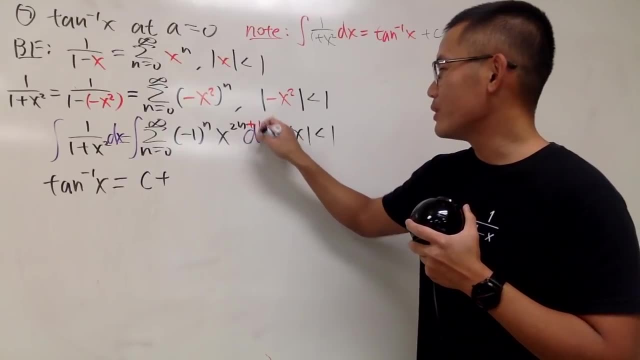 Right-hand side. first of all, put on c plus. Unfortunately, we cannot say plus c, in this case c plus. And here, don't worry, Go ahead and add 1 to the power. This is the new power. Divide it by that. 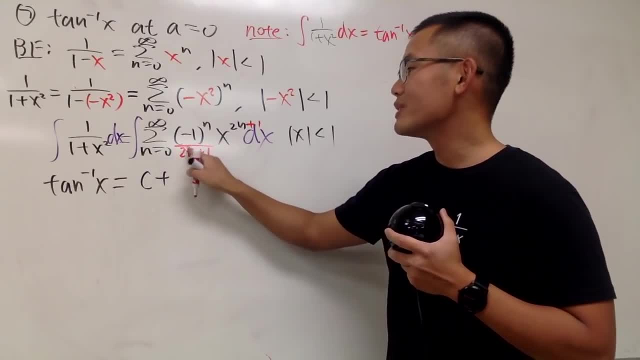 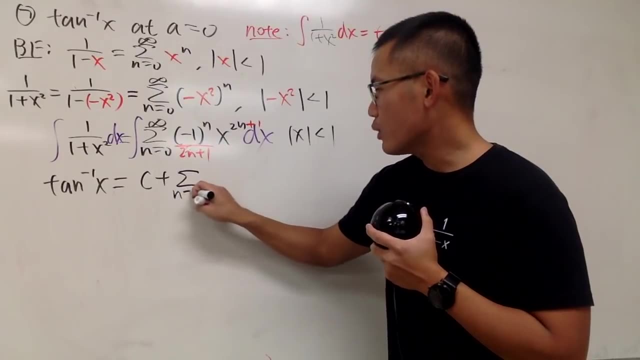 And man, we can integrate power series all day, all night long, Right? Okay, So here we have the sum, as n goes from 0 to infinity. Again, when you integrate, you don't lose any term, Right? 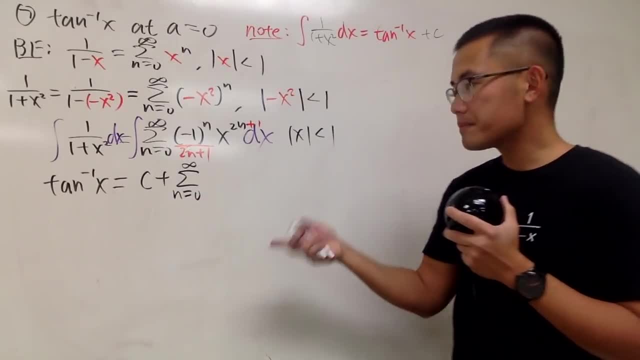 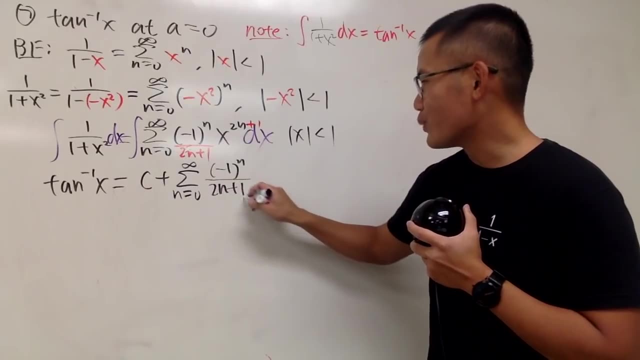 When you differentiate, maybe sometimes you want to start with: n is equal to 1,, et cetera. Okay, Anyway, here we have negative 1 to the nth power over 2n plus 1.. And then this is x to the 2n plus 1th power. 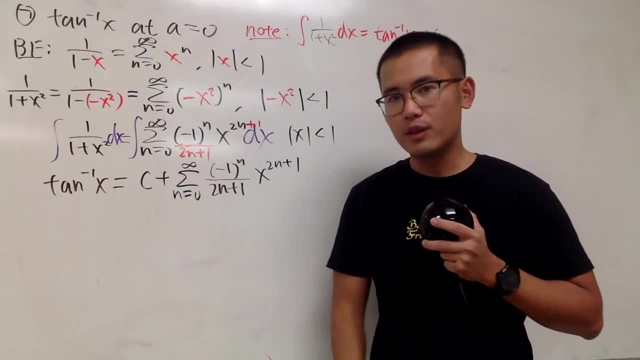 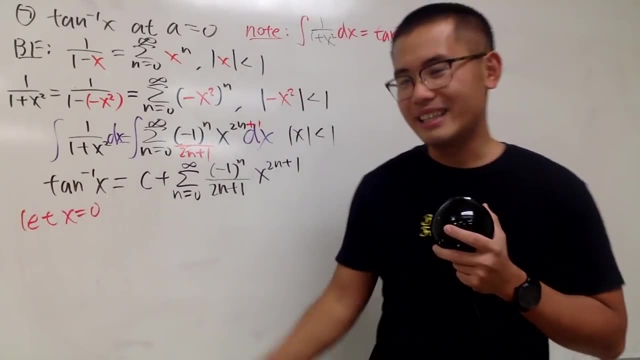 like this: And yes, you know it, We have to find out what the c is. And, yes, you know it, We are going to pick x equals 0. And then put it here. We get to use the purple pen now. 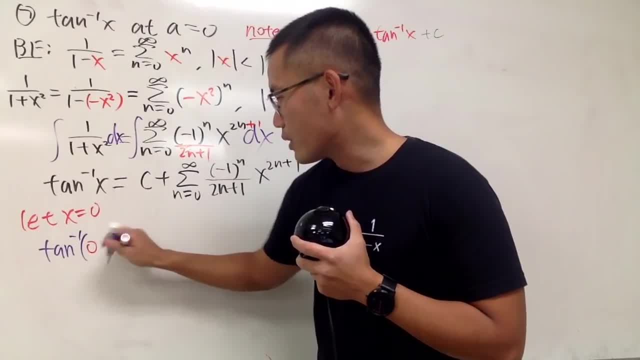 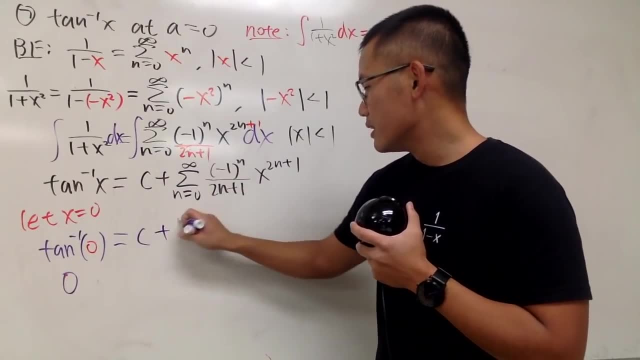 this right: here is the inverse tangent of 0. And of course that's going to be 0. No big deal. Put the c plus series n goes from 0 to infinity negative, 1 to the n over 2n plus 1.. 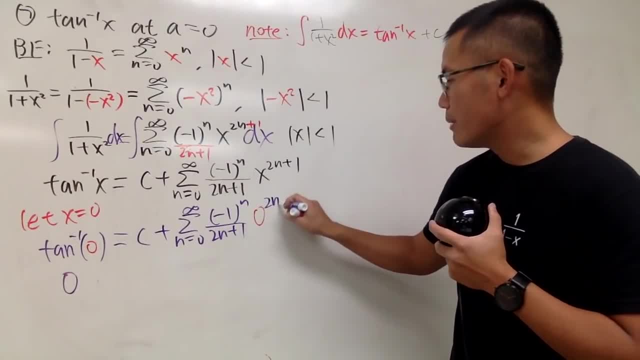 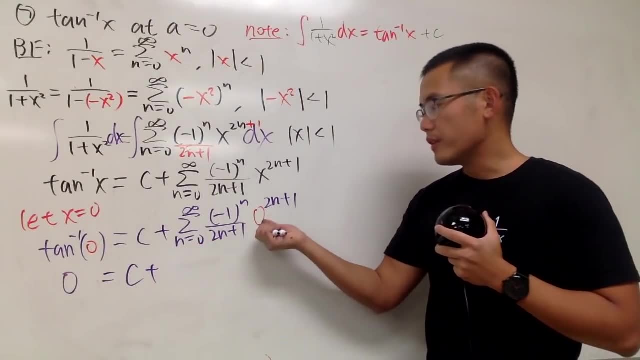 You put the 0 in here, so you have 0 to the 2n plus 1th power. This right here is equal to c plus. well, when n is equal to 0, the first time is 0 to the first power times, all that. 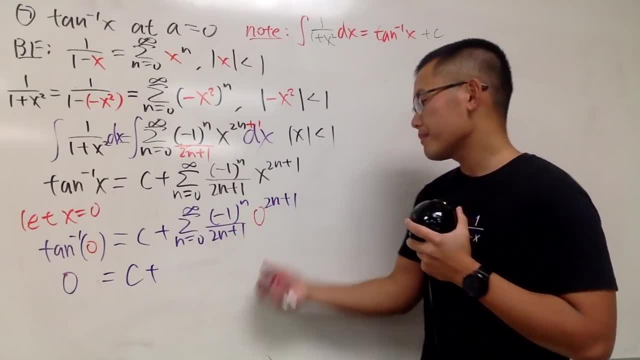 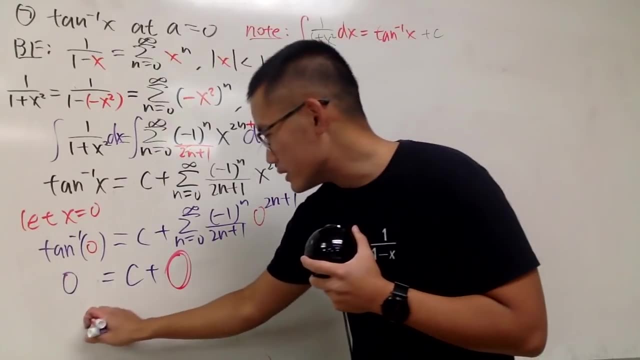 which is 0.. Likewise, the next time, when n is 1, you get 0, and so on, and so on, and so on. So you get 0 for this series. In other words, c is of course equal to 0. 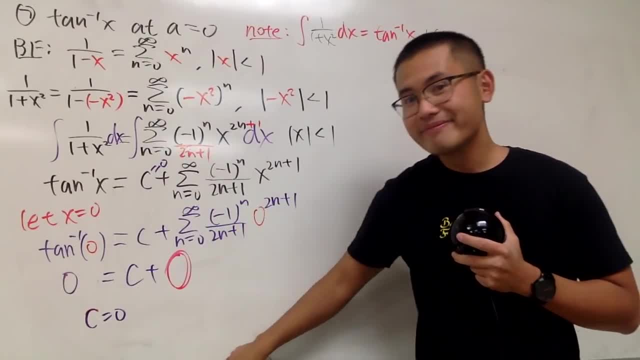 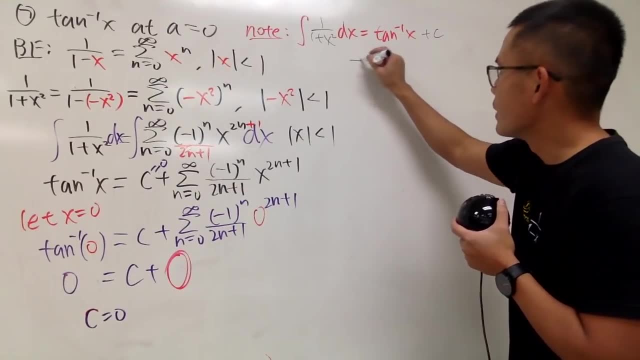 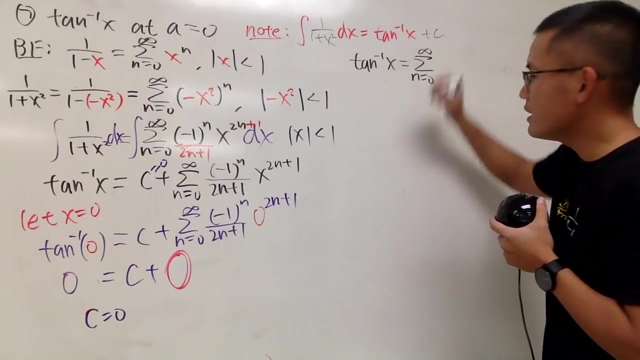 That means right here, is equal to 0. Okay, so we are going to do what we did earlier, so just kind of stay strong, okay? So let me just write this down Here we have the inverse tangent of x, which is that we have the sum as n goes from 0 to infinity. 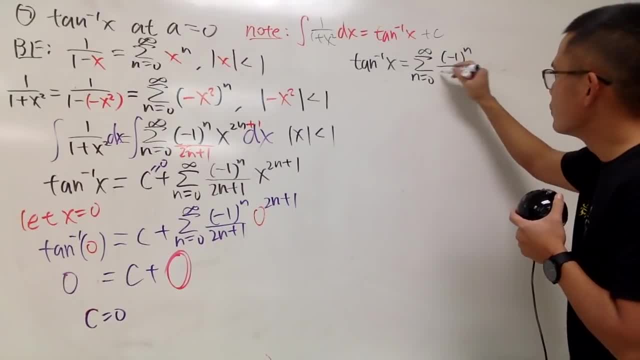 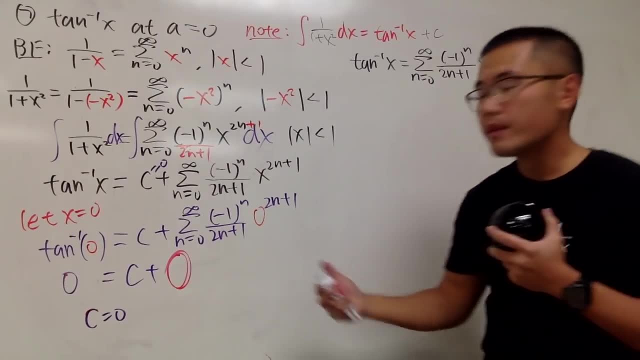 and we have negative 1 to the nth power over 2n plus 1.. And we have x to the 2n plus 1th power. Well, the radius of convergence will stay the same because we just integrate this thing right here, right. 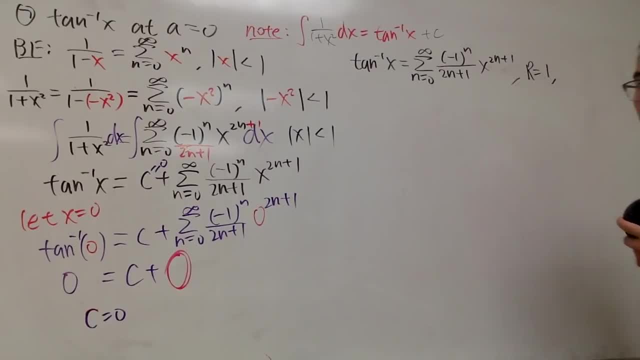 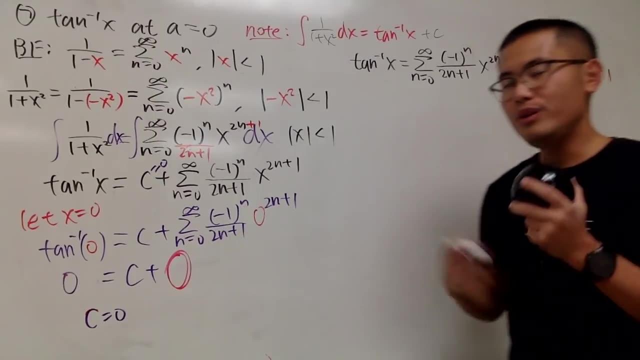 So r will still be 1. And that means I will be going from negative 1 to 1.. But this time we don't know what will happen at the endpoints, So go ahead and do the check. Here we go. 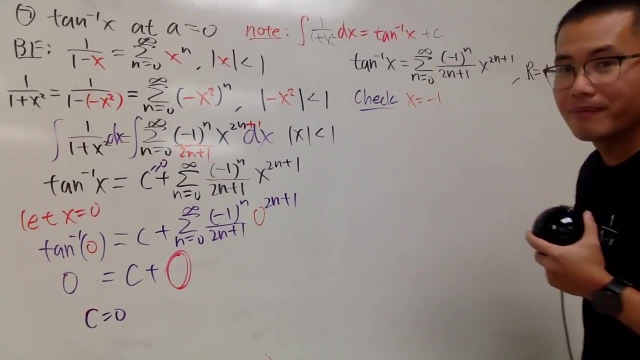 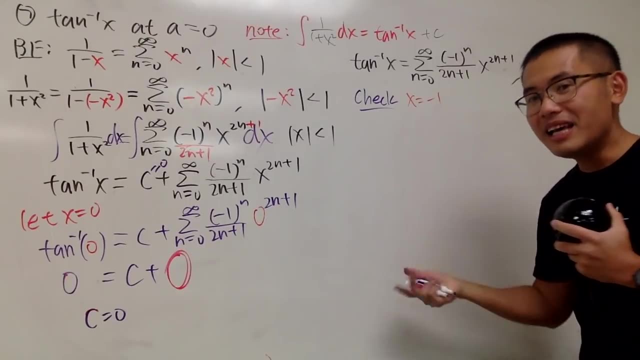 This is the check. When x is equal to negative 1,. again, do not just put in the function okay. You always have to put in the series and just observe. Unless you can say, okay, the function doesn't work. 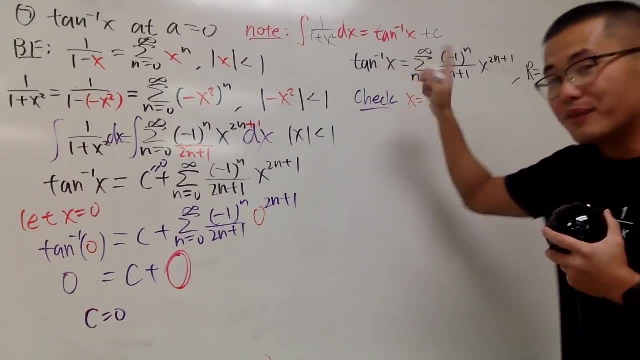 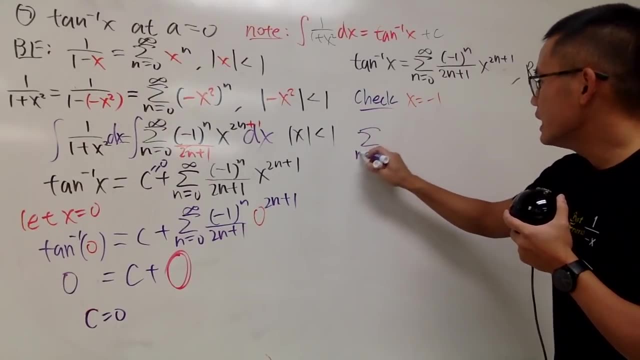 the series doesn't work, But you know, in this case, inverse tangent- it always works. So don't do that. So put this right here. So here we have the series. n goes from 0 to infinity. 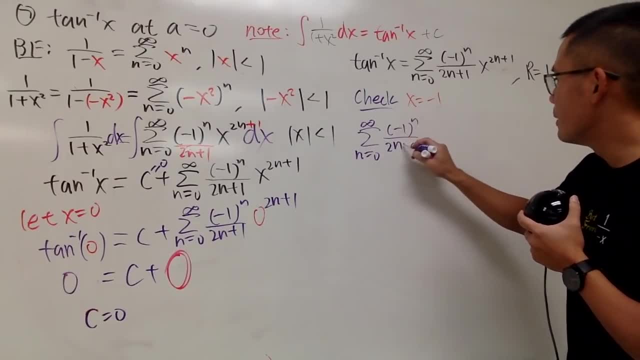 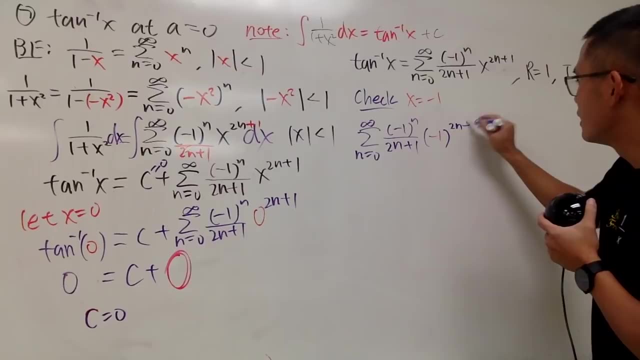 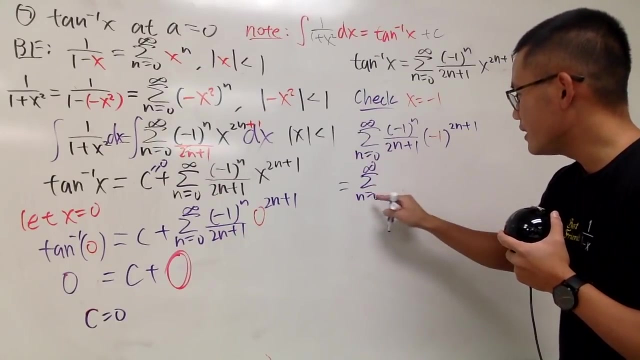 and this is negative 1 to the nth power over 2n plus 1.. And here we have parentheses- negative 1 to the 2n plus 1th power, like this: Okay, Here, what do we have? This is the sum n goes from 0 to infinity. 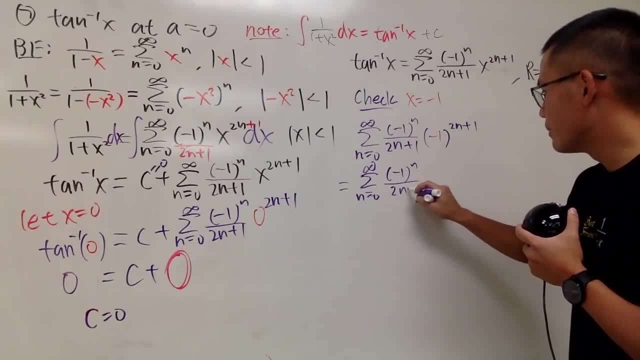 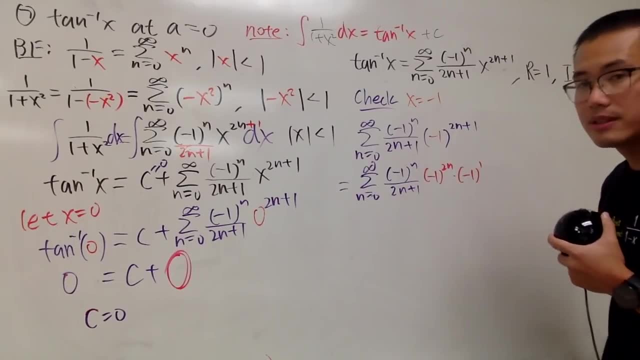 This is negative 1 to the n over 2n plus 1.. And of course we can separate this. This is the same as negative 1 to the 2n times negative 1 to the first, But this right here is nicely equal to just 1.. 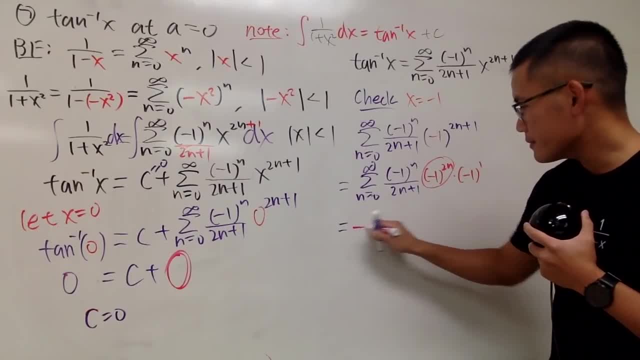 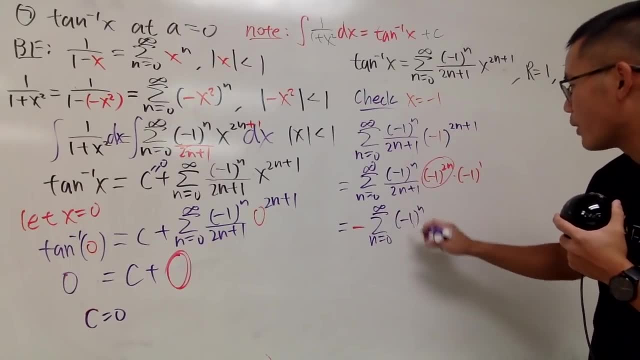 This is a negative 1.. I can put it all the way in the front And this is the sum: n goes from 0 to infinity. So we have negative 1 to the nth power and this is 1 over 2n plus 1, like this: 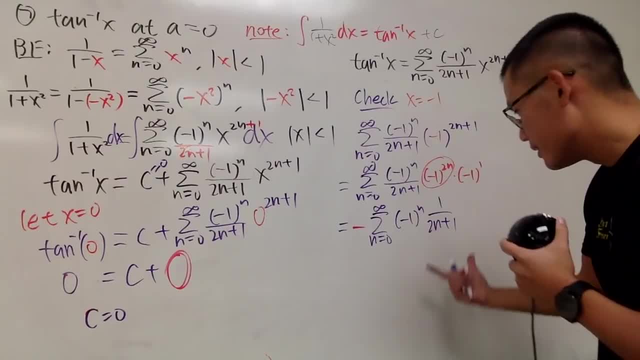 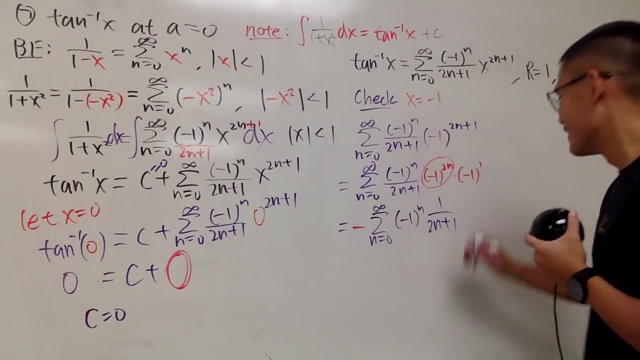 Right, So that's how you do it Then. does this converge or diverge? What kind of series is this Alternating? Okay, Good, So take this to be the bn and let's just go ahead and do the check. 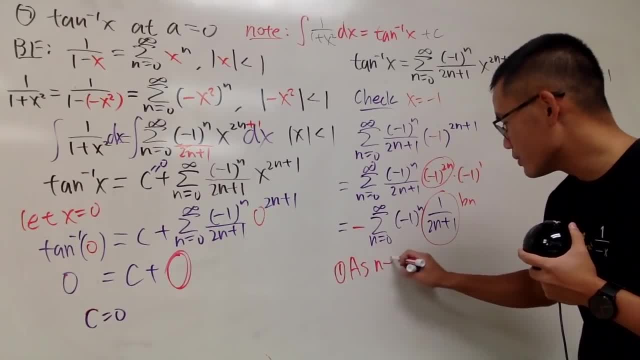 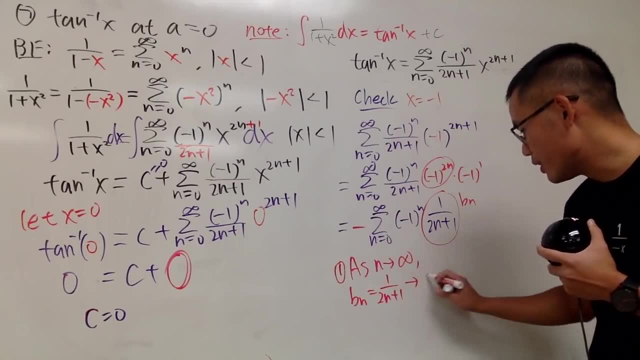 First check: does bn go to 0?? So as n goes to 0, it goes to infinity bn, which is 1 over 2n plus 1, put infinity to here. does it go to 0?? Yes, it does. 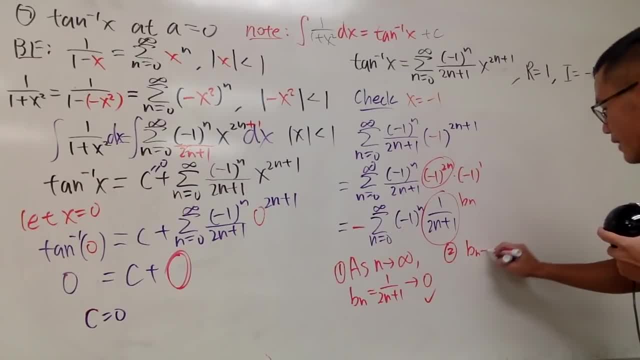 So, of course, checks. Secondly, do we have a decreasing bn? Well, we don't know yet. so let's put this down: Put n plus 1 here. So notice, put n plus 1 here, okay. 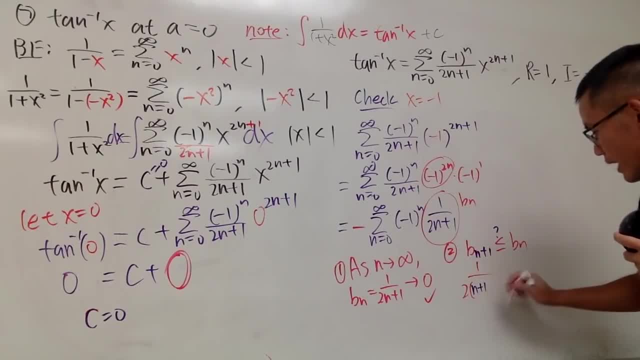 1 over 2 times n plus 1, and then plus 1,. is this less than or equal to the original bn? Well, just work this out real quick. So here you get. just cross-multiply if you would like. 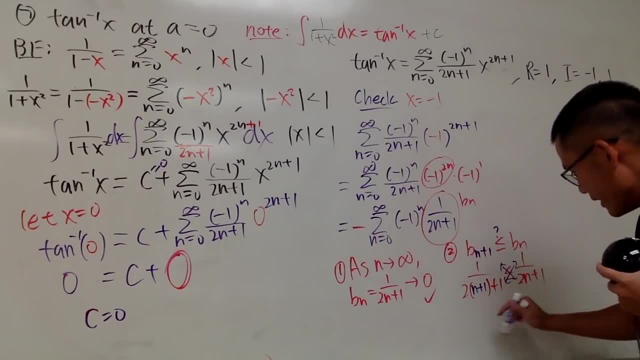 I find students like to cross-multiply, so this times that is 2n plus 1.. Is this less than or equal to this? right here is 2n plus 2 plus 1, so it's of course plus 3.. 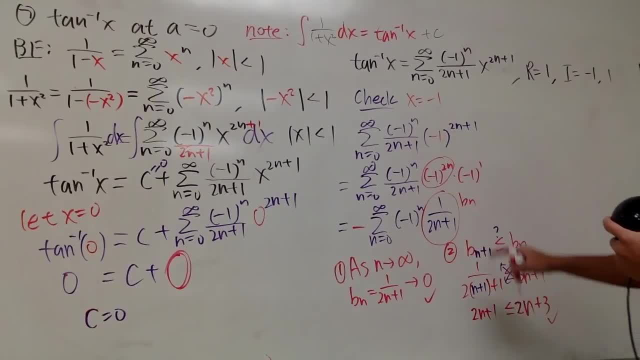 And if you look at this, of course it checks. So again this right here. let me just write it down here: it converges by ast. okay, So it converges by ast. okay, So we can come here. 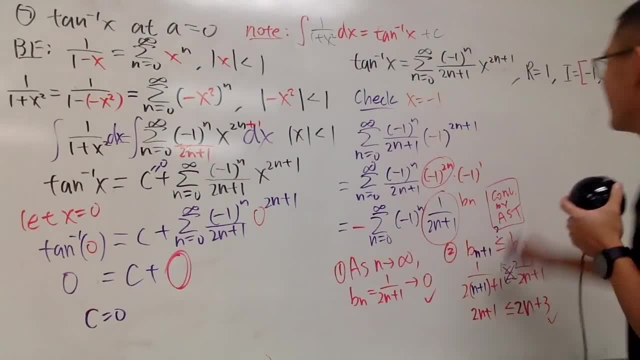 and include negative 1.. Very good, Now don't forget to check when x is equal to positive 1.. Yeah, Anyway, put a 1 in here. So we are looking at the sum as n goes from 0 to infinity. 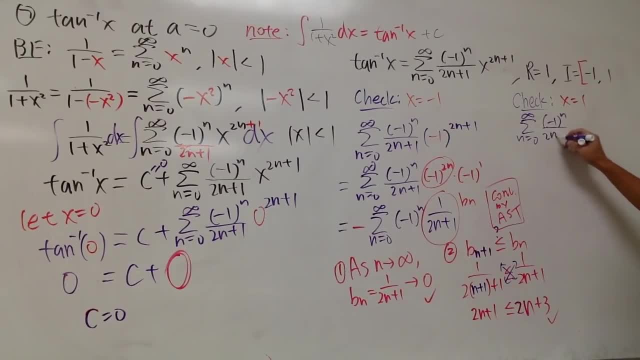 and here we have negative 1 to the nth power over 2n plus 1 times 1 raised to the 2n plus 1 power. The good thing is that this is always 1.. Yeah, So we are looking at the sum. 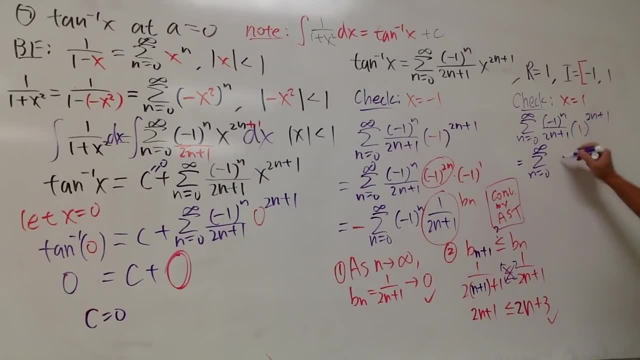 as n goes from 0 to infinity, I will just write it as negative: 1 to the nth power, and then this is multiplied by 1 over 2n plus 1, like this: Yes, this is exactly the same as that part. 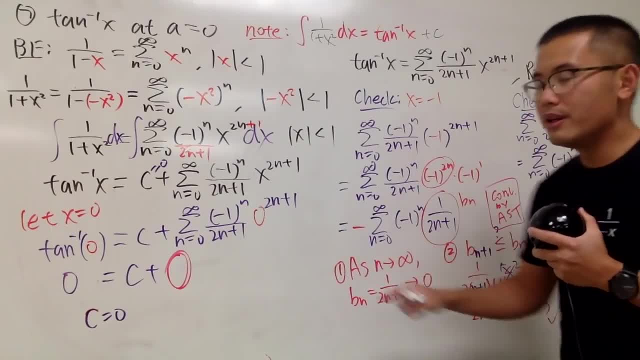 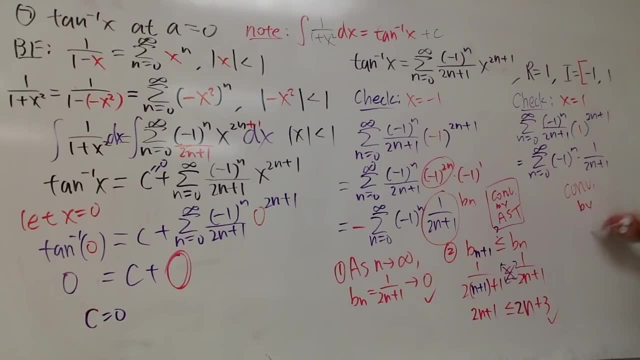 This right here has a negative. It's a negative of finite value. This is just a positive. So I will just tell you this right here. converges as well, of course, because we can do the same thing. converges by AST, right. 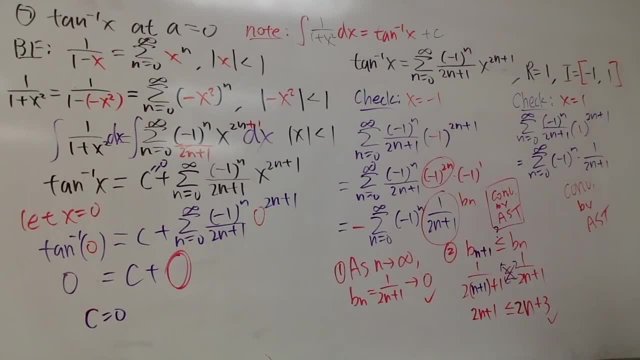 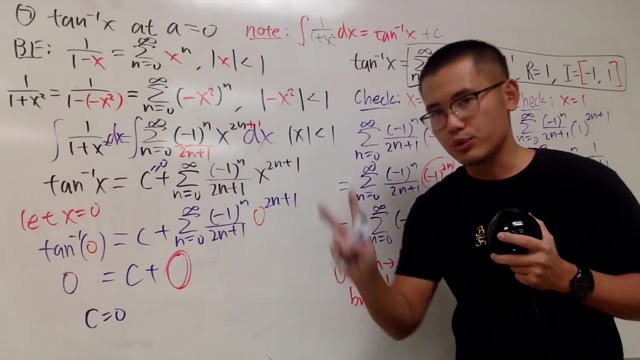 Therefore, we come here and include positive 1 as well. Right, So we are done. Ladies and gentlemen, this is the inverse tangent of x. Take a look, I know another monster question, but this is what we have to go through in Calc 2.. 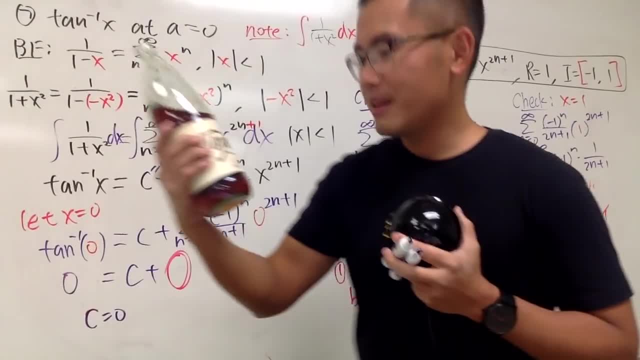 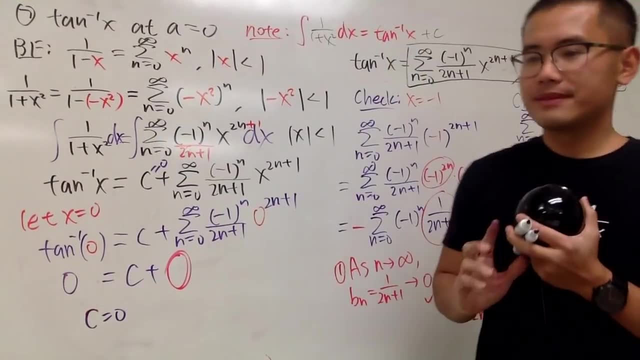 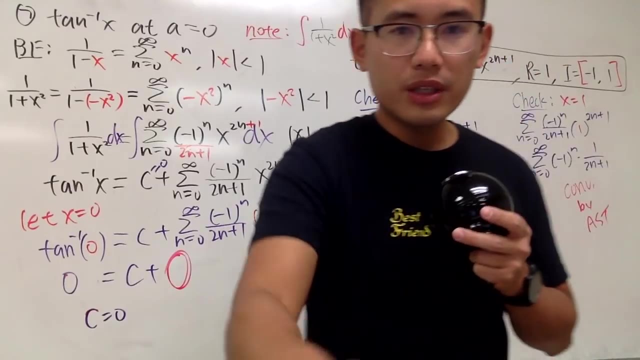 Right, So have a look. In the meantime, let me tell you guys why I'm drinking this thing. okay, Just black tea. Okay. Now, of course, we are going to continue with the next question. We have a couple more to go. 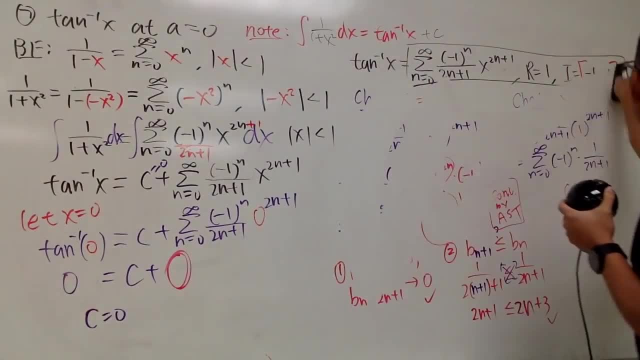 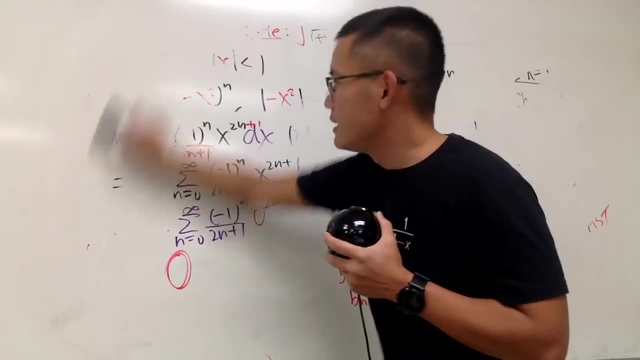 This is an hour already, man. Seven questions took me one hour. Oh my God, It's at 55 minutes, So almost an hour. Yeah, Hopefully this time it will be better. And yeah, I picked some questions. 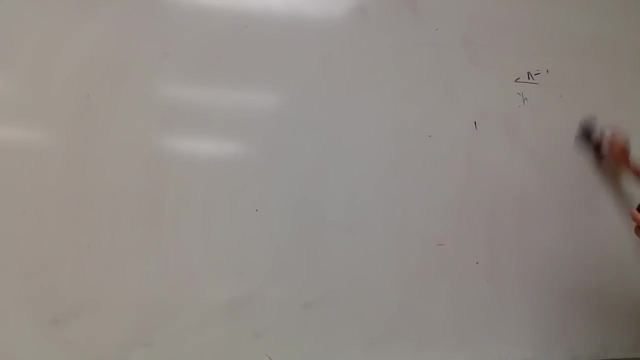 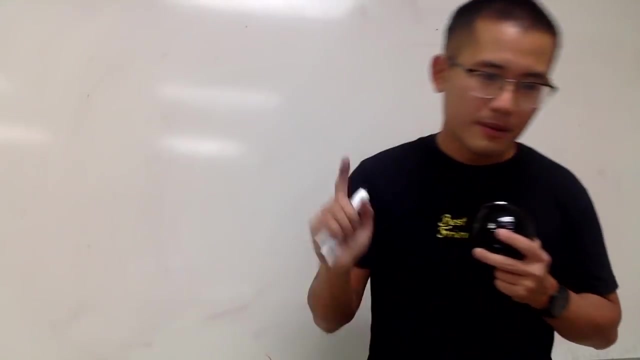 that I know you guys will have to know for Calc 2 classes and questions that you know- typical questions- And I think I covered pretty much everything that you have to know. So, yeah, Now we'll be talking about the best friend. 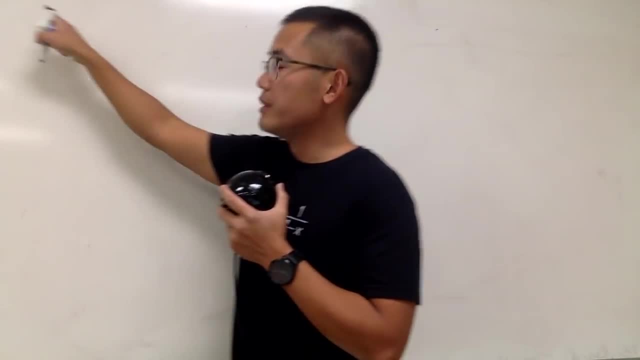 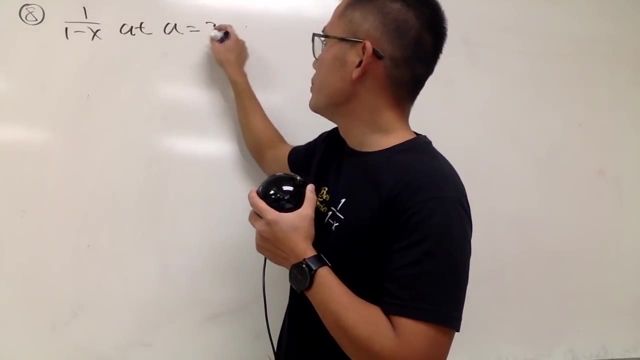 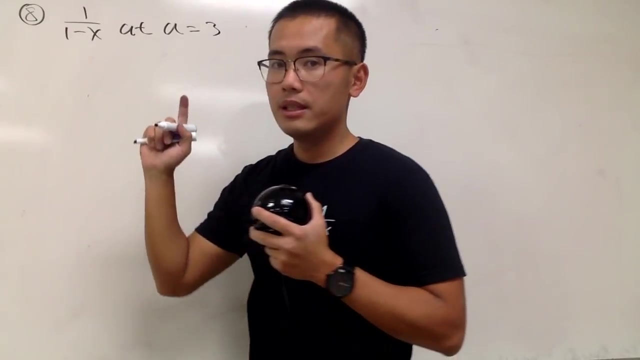 at a different center. So here we go. This is number 8. I'll kind of work this out carefully with you guys. Add a equals 3.. Okay, So this is what we are going to do. Let me just write down the best friend. 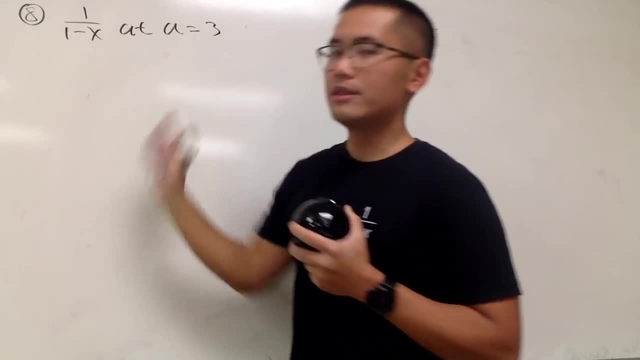 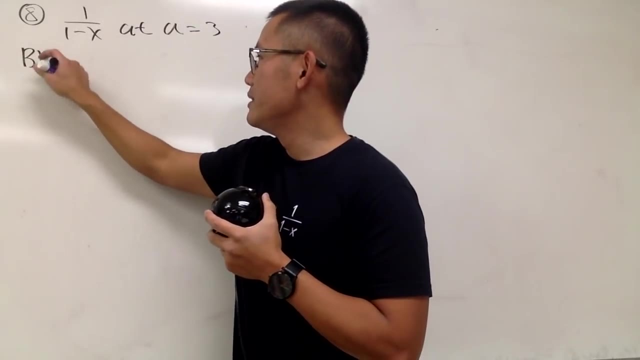 This is the best friend for you guys, right? So while it's on the board, I will just do this. I will still write it down for you guys. This is the original best friend: 1 over 1 minus x. 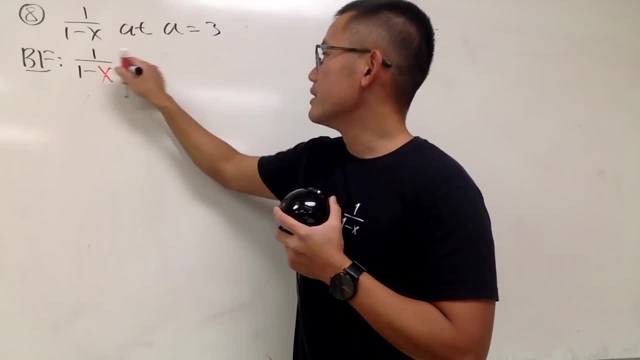 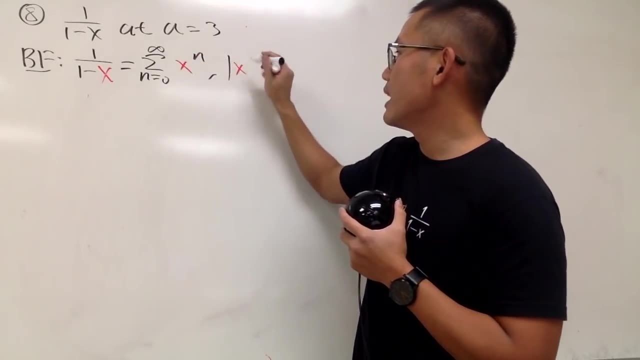 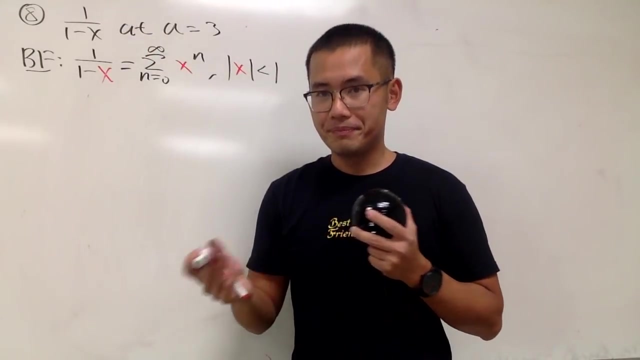 Okay, The original best friend. This is the sum as n goes from 0 to infinity, x to the nth power. absolute value of x has to be less than 1.. Okay, The original best friend. Now this is our best friend. 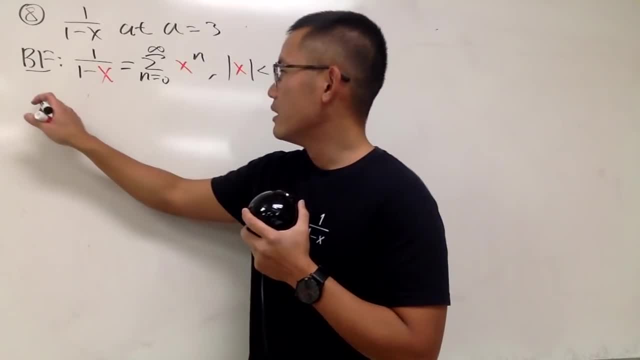 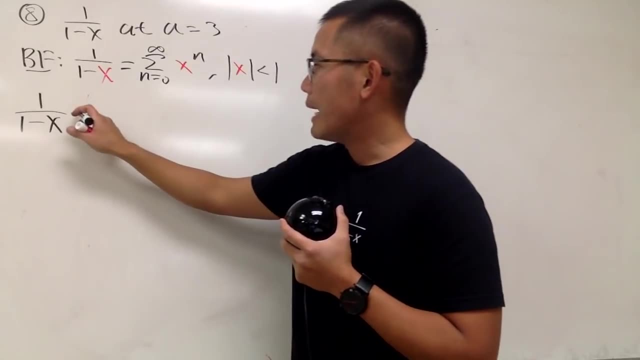 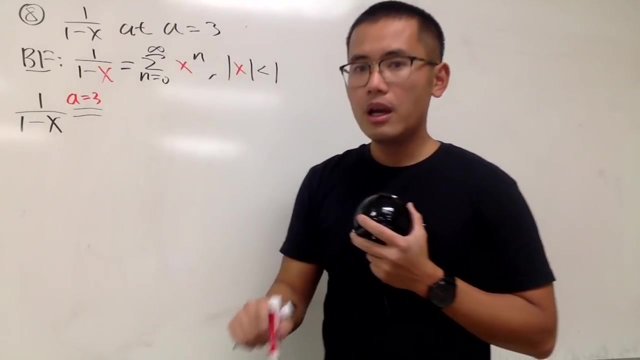 but he moved to a different center. So this is what we do: Start with 1 over 1 minus x. That's exactly the one that we are doing, But here is the deal. Here is the deal If the center a is equal to 3,. 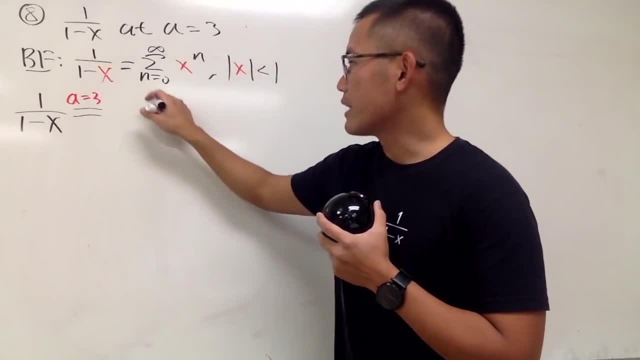 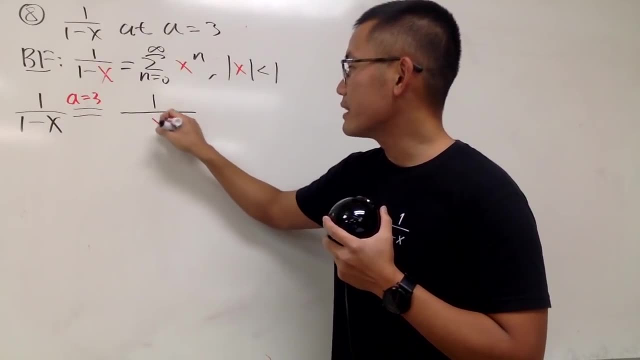 then what you want to have is this: I still have a 1 on the top, That's okay, But if you have the, a right here is 3,. what you want to have is you want to have x minus 3 as your input. 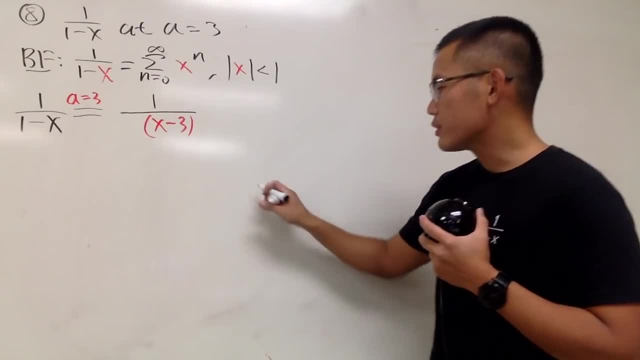 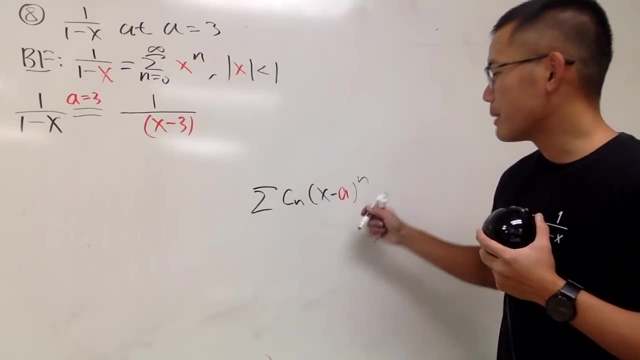 They have to be together. Why? Because, remember, for the power series, it's going to be the sum of the coefficients times x, minus a to the nth power, or so like this Right. So you want to have this as your input. 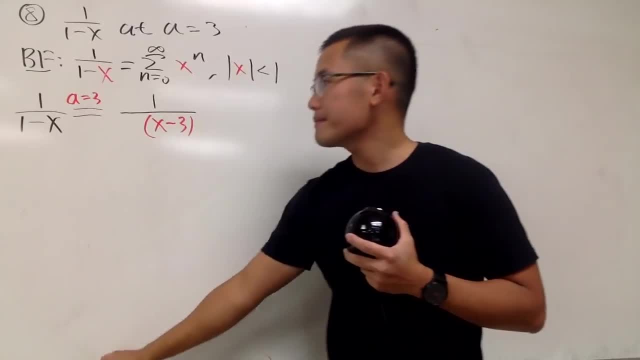 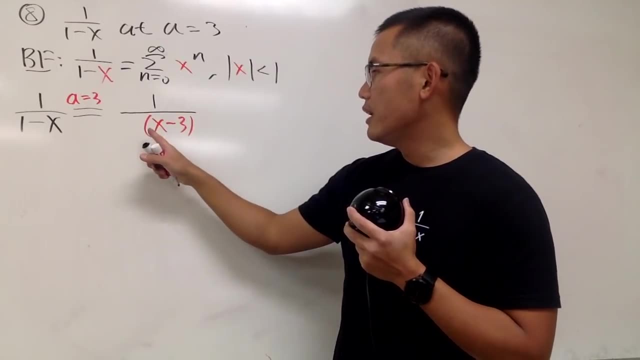 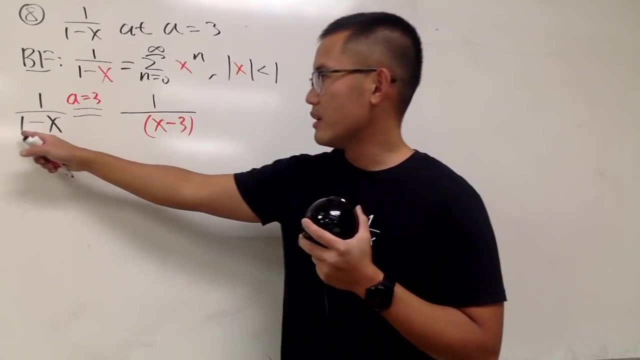 That's the idea. Now we are going to make sure this is the same as that, algebraically, of course. So now, if you look at this, we have x minus 3.. That's no good, Because originally I have a 1.. 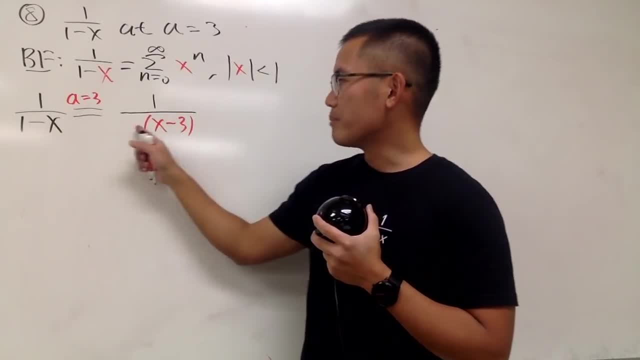 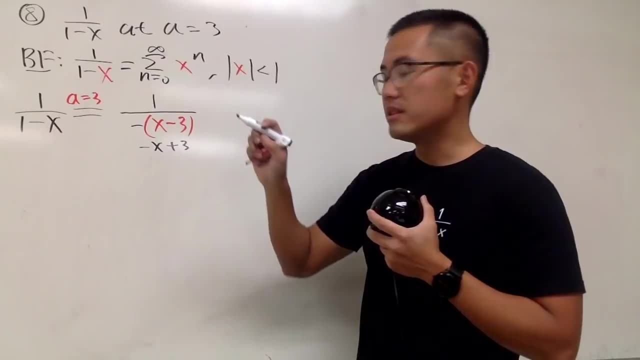 That's x minus 3.. And, by the way, I want to maintain the minus though. So let me actually put on a minus right here. So, technically, right here, I actually have negative x plus 3,, isn't it? 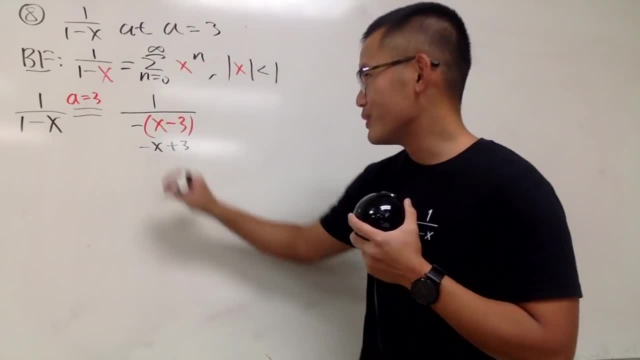 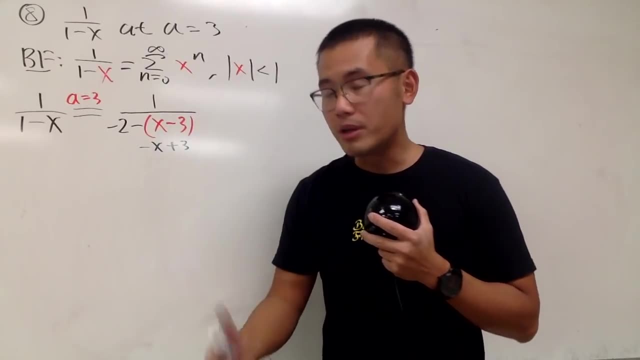 In that case, how can I get a 1 back? Well, we can just put down a minus 2.. Like that Again. this is just the algebra word that you want to do. And remember, if you have, x is equal to 3,. 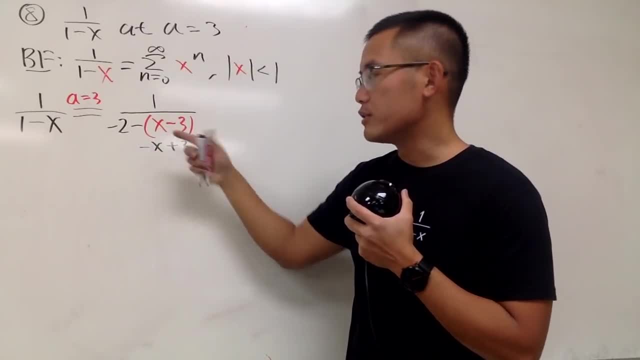 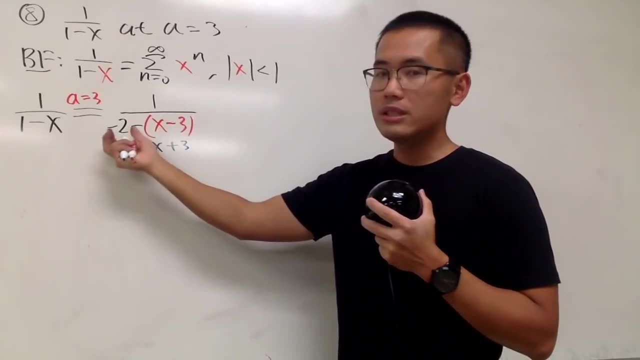 if you have a is equal to 2 for the center, you must have x minus 3 as your input, And later on you'll see what I mean by that. So always put this down right away And just try to see if you have to add or subtract. 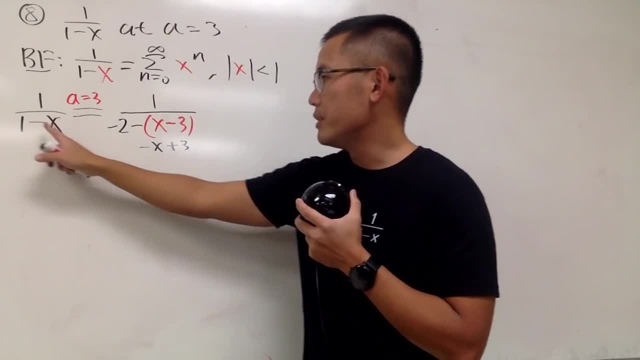 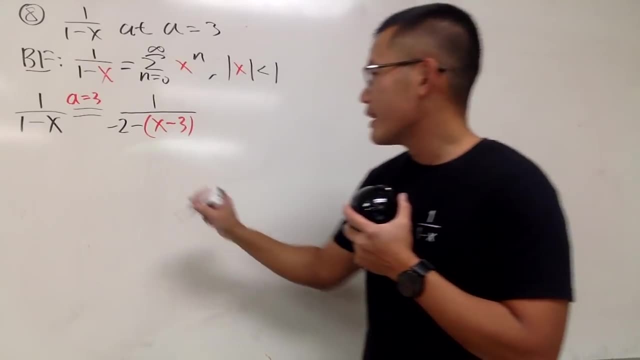 so you can match the original. And again, I put down the minus here because we want to subtract this right here. Okay, So that's the idea. I'm going to erase this now, And then we do some more algebra. 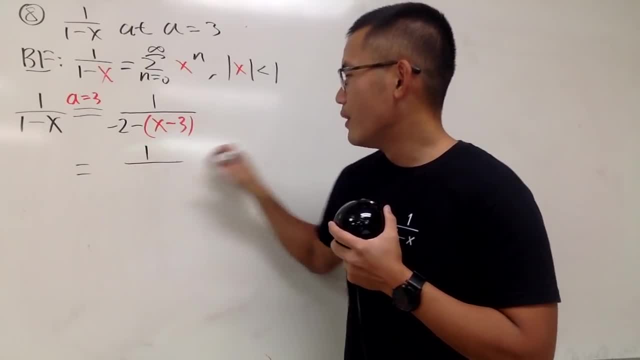 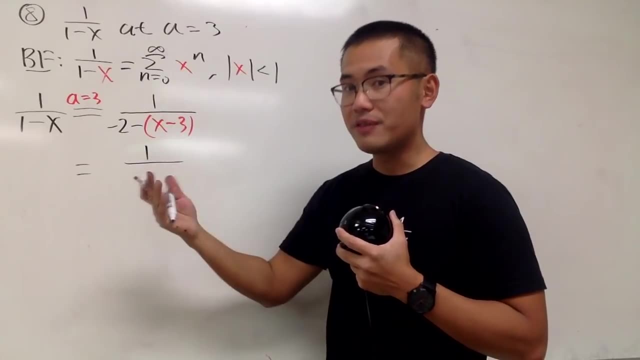 Here 1 is a 1 on the top, of course, Over, But I don't want a negative 2. I want to have a 1. So what we can do is just factor things out. So here I will factor out a negative 1 half. 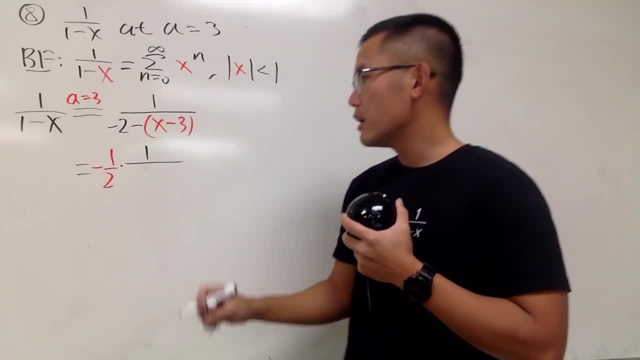 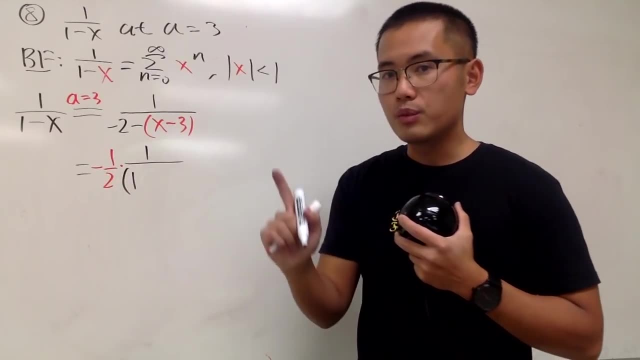 Like this. I'm going to factor out a negative right here as well, Okay, And then I'll open the parentheses. Originally I had a negative 2, but I factored it out right here. That means I have a positive 1.. 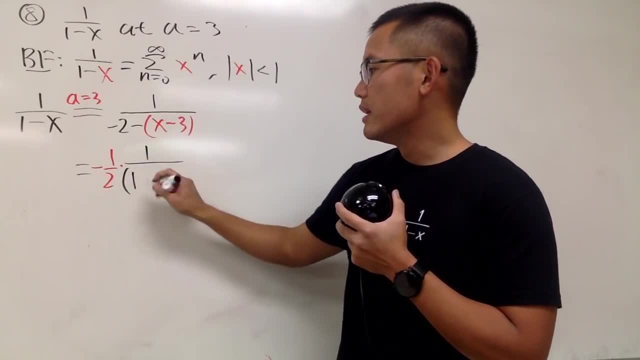 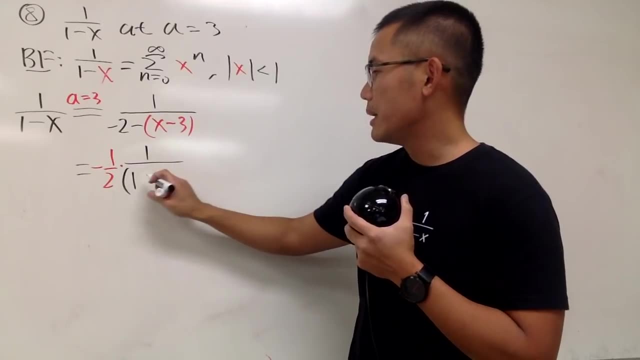 Originally I had a minus, but I factored out a minus. It's a plus, But that's no good because I want to use the best friend. It's a minus, It's okay, I'll look at this as minus, minus. 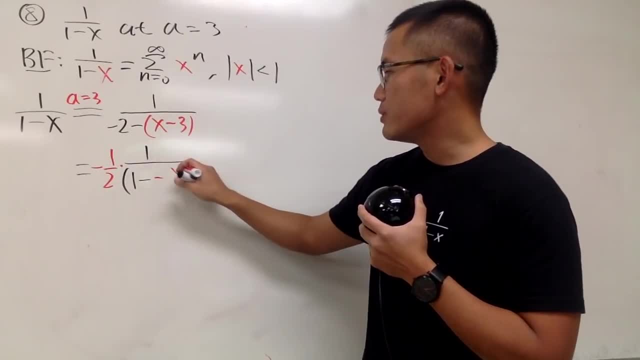 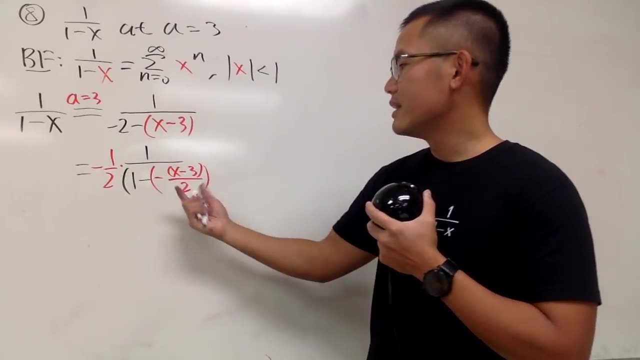 Okay, And originally we have the x minus 3 in the parentheses, but we factored the other 2.. So be sure, we divide this by 2.. So, in fact, this will be our input. Yeah, Crazy right. 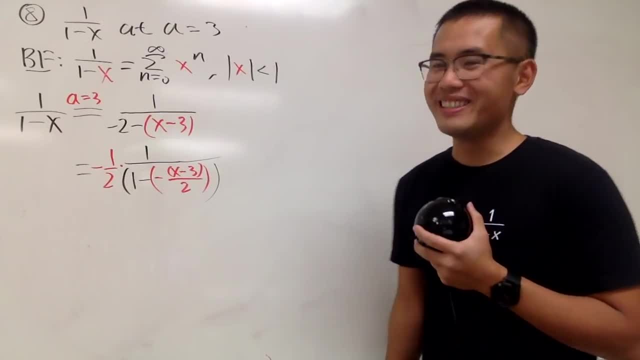 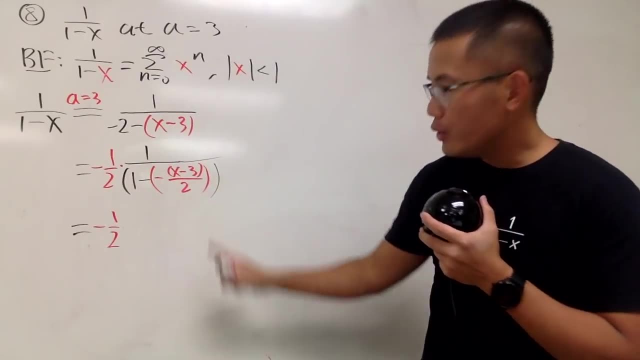 Crazy, huh Yeah. when the best friend moves away it's crazier, But it's okay, Don't worry, We can always find it. This right here is negative 1 over 2.. This right here, you enter this thing in here and in here. 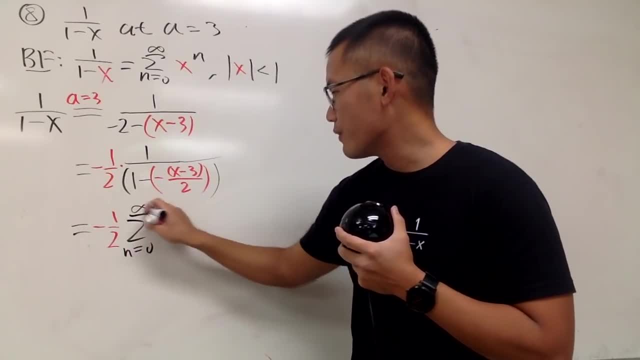 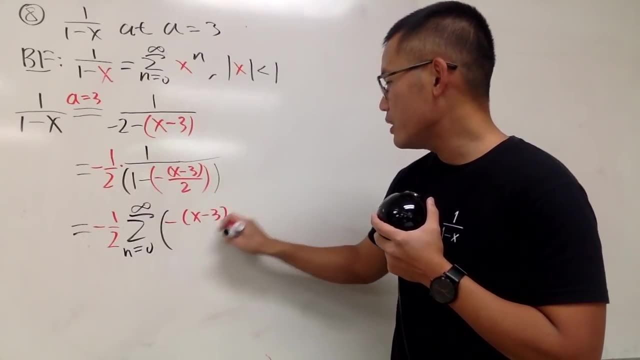 So we have the series as n goes from 0 to infinity. Open the parentheses and just enter this in here: Negative parentheses, x minus 3 and then over 2 and then raised to n's power And then absolute value of that. 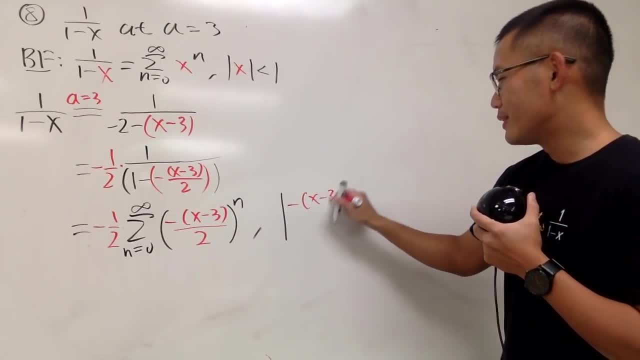 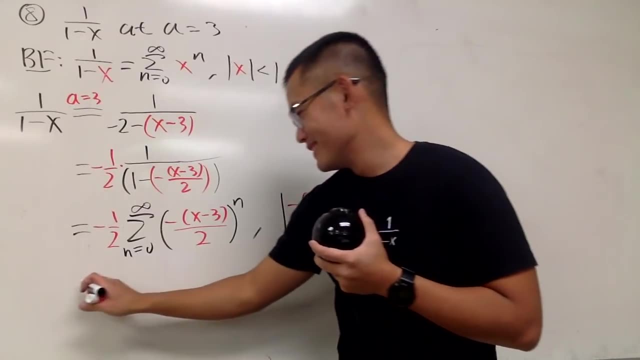 And then open this right, Put it in here, And then yeah, And then, and then, and then It's always, and then, of course, All right, And then just work this out. This is negative 1 half. 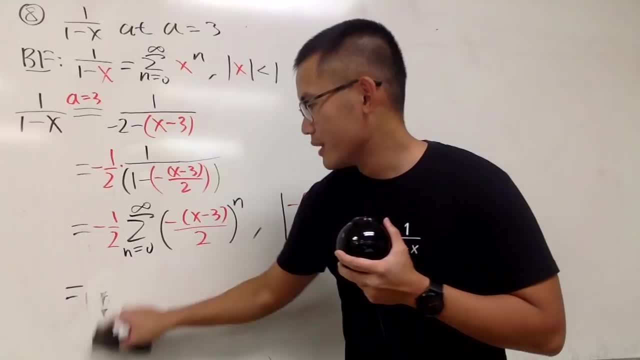 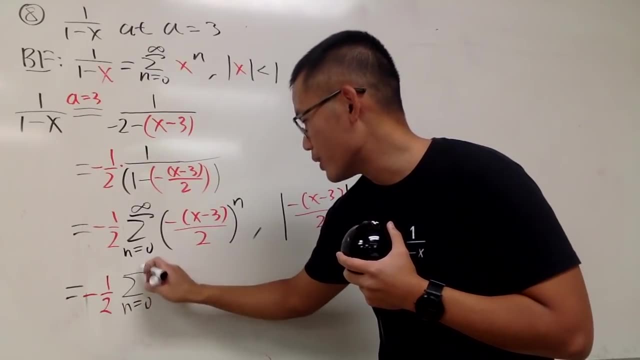 No big deal. Yeah, Perhaps I'll still keep that in red, Why not? All right To continue. this is the series as n goes from 0 to infinity. Now, this is what I would like to do. Negative 1 to the n's power. 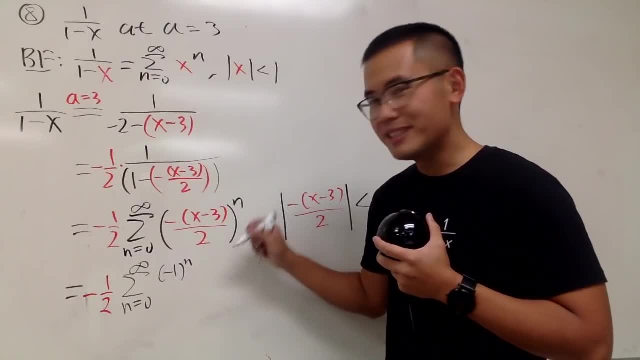 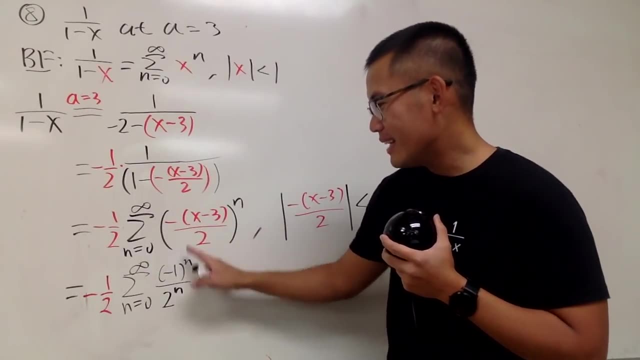 Let me write it down first, And then 2 to the n's power. Maybe you guys can keep track of how many n's I'm saying right now. So we have negative 1 to the n and then 2 to the n's power. 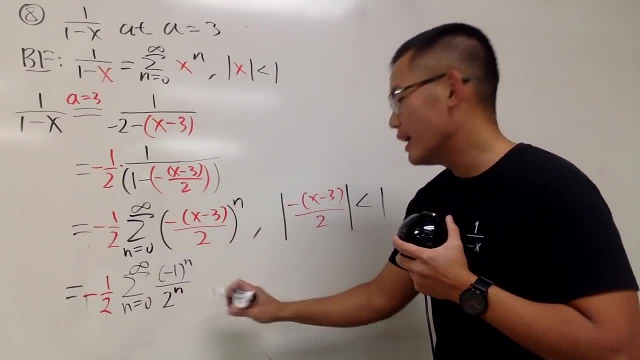 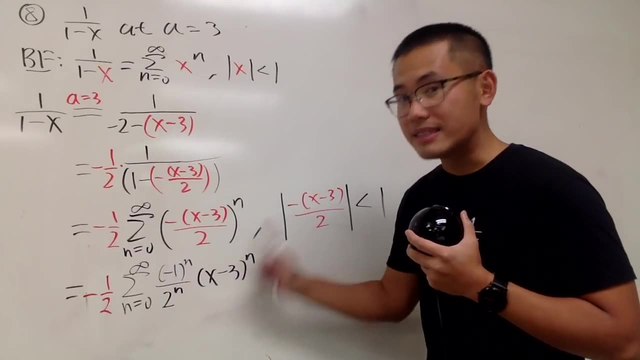 And we will have x minus 3 to the n's power. So, as you can see, this is what I mean: A coefficient times x minus the center, which is the a, is 3. And then 2 to the n's power. 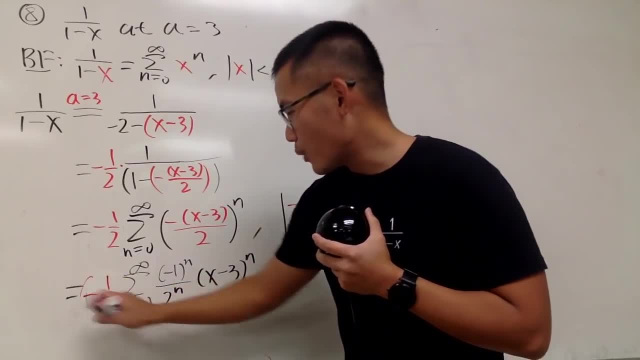 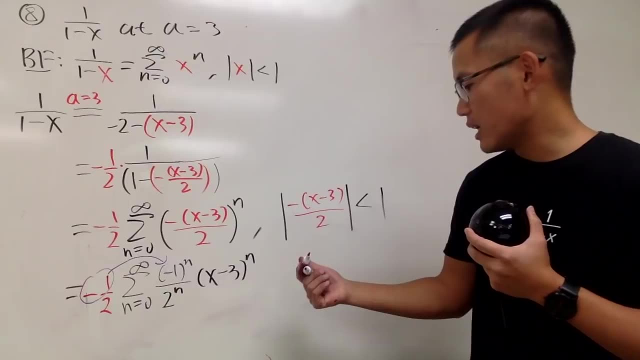 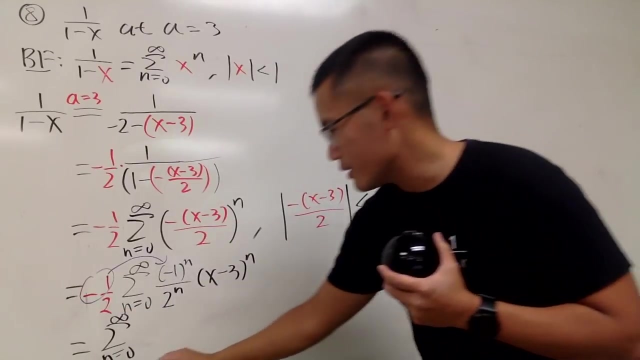 like so. Finally, this is negative 1. I'm just going to group this and multiply with that, So perhaps I will write it down here. Can we see? okay, n is equal to 0, to infinity, Yeah, kind of. 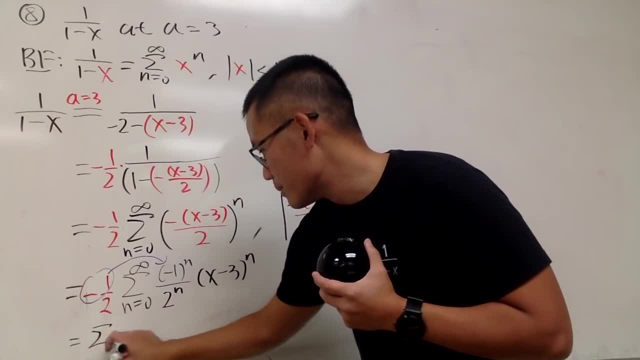 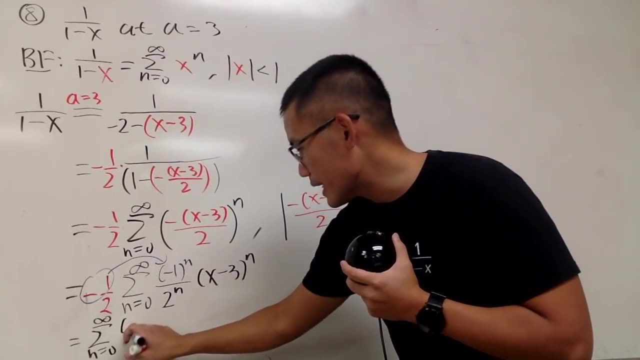 Let me see The sum as n goes from 0 to infinity. Okay, good, Okay, So this is negative 1 to the n. Of course, we just add the exponent. So this is negative 1 to the n plus 1's power. 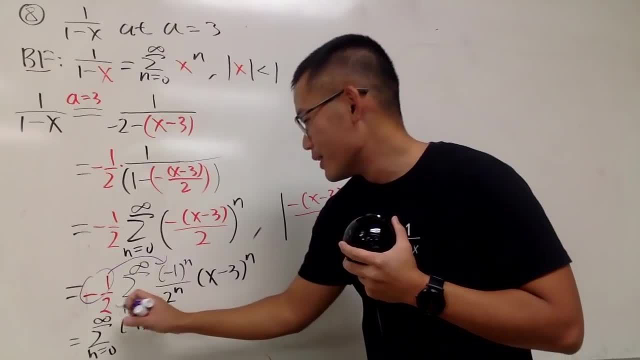 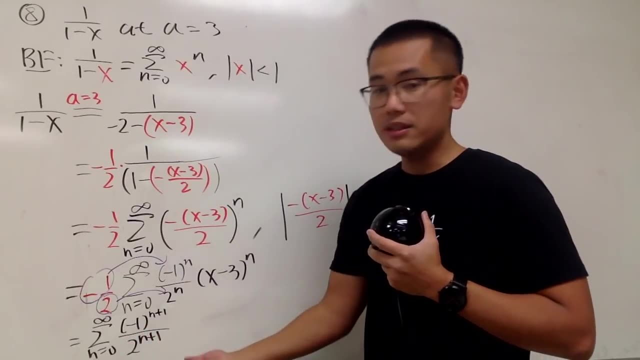 Then 2 times negative. sorry, what am I saying? 2 times 2 to the n's power. We will just divide this by 2 to the n plus 1's power, like this. Then this right here stays: 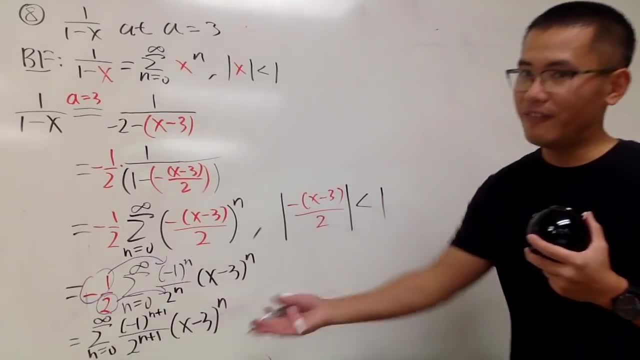 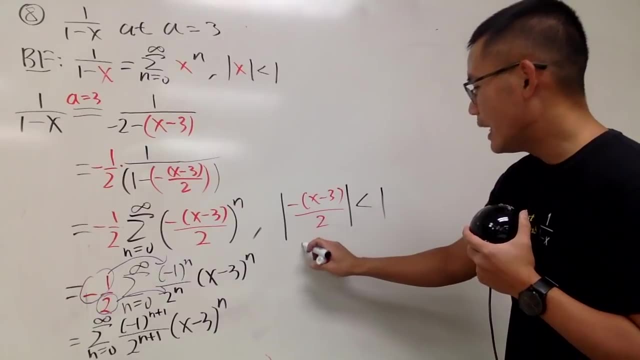 x minus 3 to the n's power like so: Very good, huh. Now we just have to work this out Absolutely. the negative doesn't matter. Multiply the 2 on both sides, So we see absolute value of x minus 3. 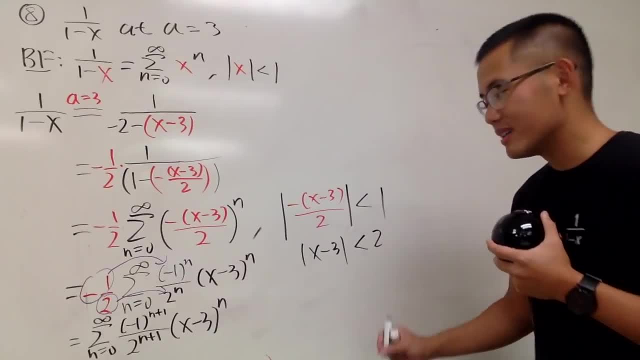 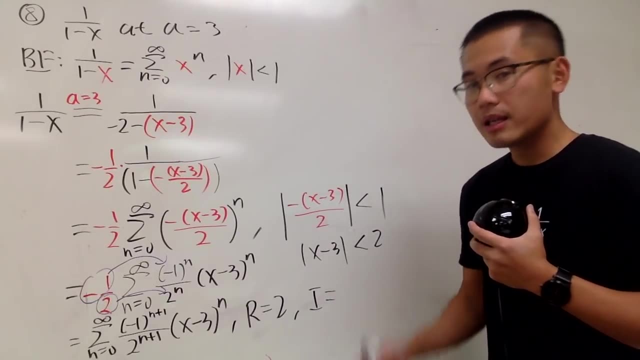 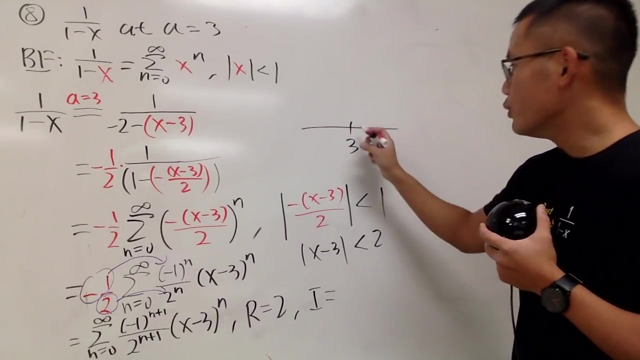 is less than 2.. That means the r is 2.. Well, where's the i then? This time the center is x3.. So let me just draw the little picture for you. And what we do is move to the left twice. 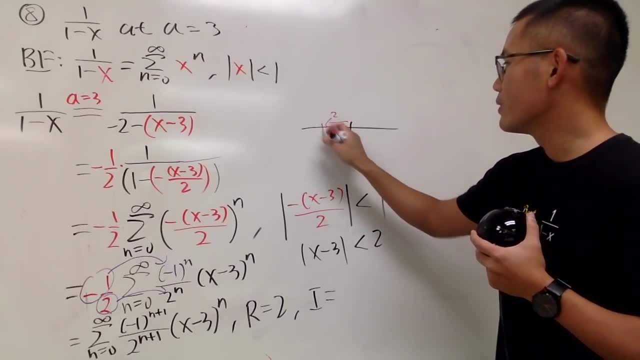 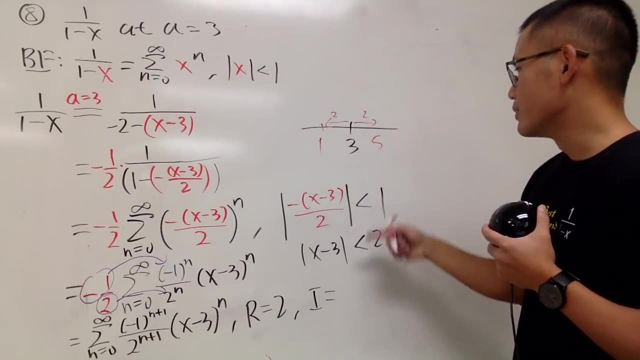 So if you just move to the left twice, you get 1 right here right. And then if you move to the right twice, you get 5.. So minus 2 and then plus 2. So we have 1 to 5.. 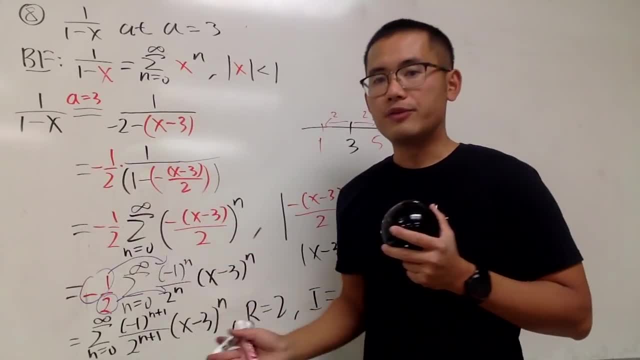 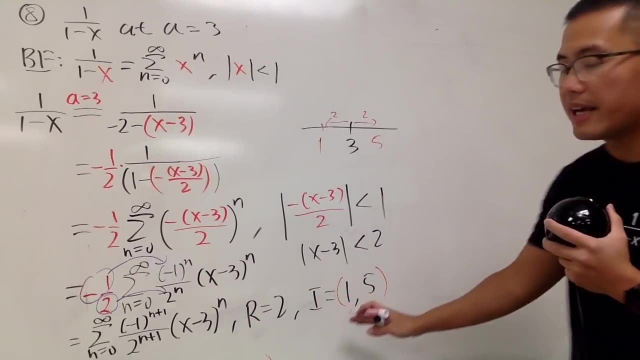 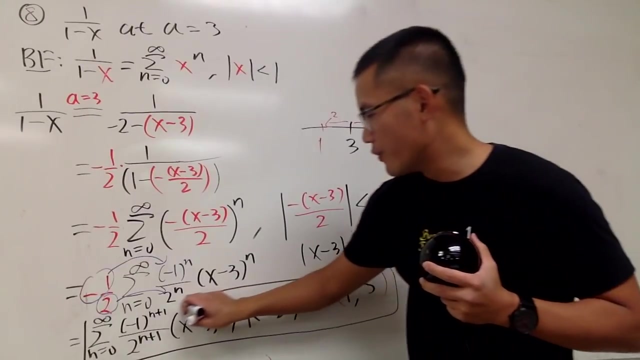 Now notice what did we do with our best friend? Just technically algebra, right. Therefore, you do not include the endpoints for the. i just like the original best friend. Okay, so this right here is the answer for the best friend. 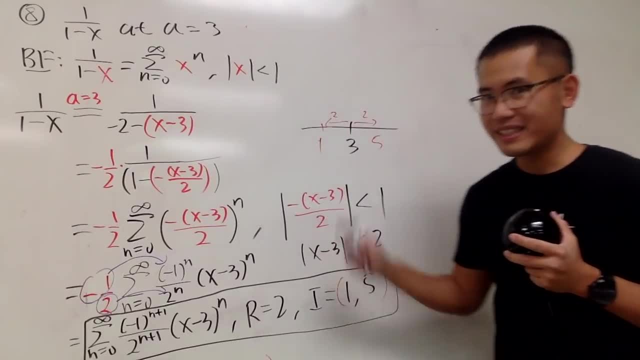 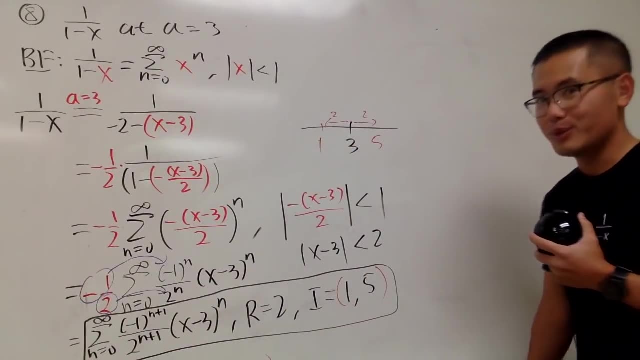 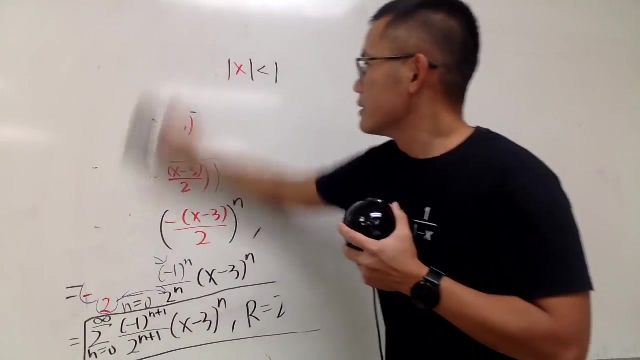 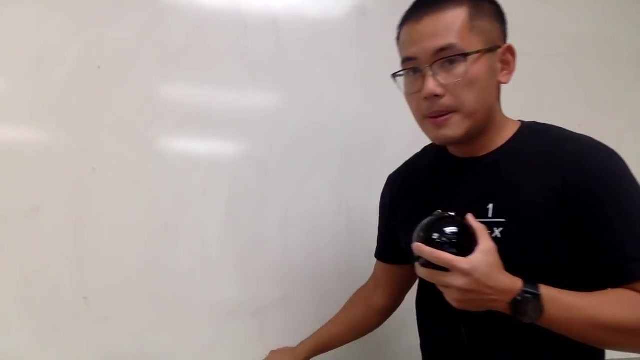 if it moves to the new center 3.. That's it, Okay. Perhaps I need more space for the next one, so I'm going to erase that. Erase this question, okay. Okay, Now we are looking at 1 over x squared. 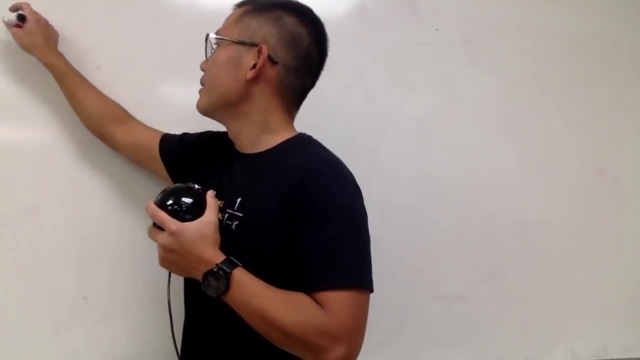 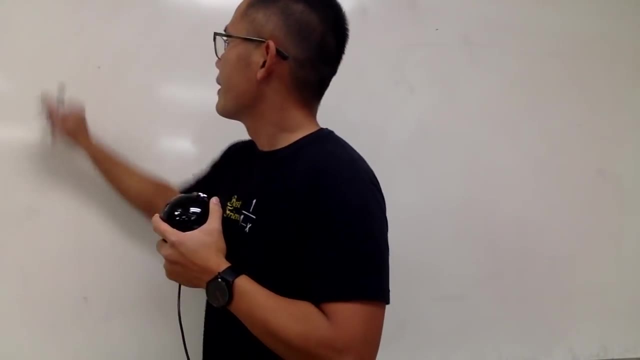 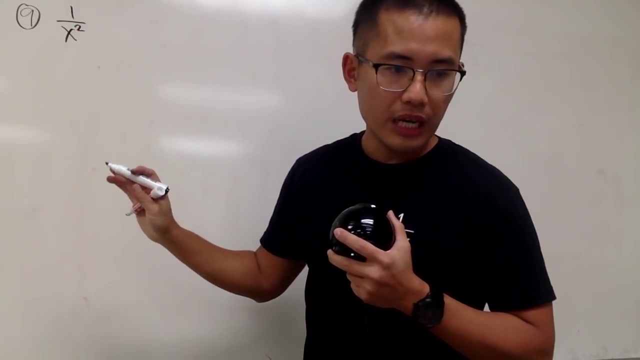 when the center is a negative 2.. Number 8.. No, that was number 8.. This is number 9.. Yeah, okay, Number 9.. Here we have 1 over x squared and we have the center at a equals negative 2.. 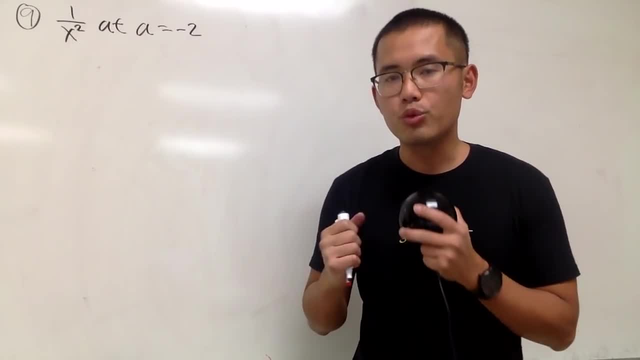 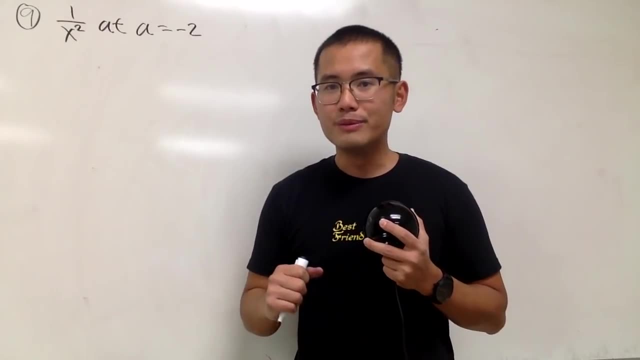 You have two ways to do this. The first way is you can still use our best friend, And the second way is that you can actually use the father of the power series, Namely Taylor. Yeah, you can use the Taylor formula to get that. 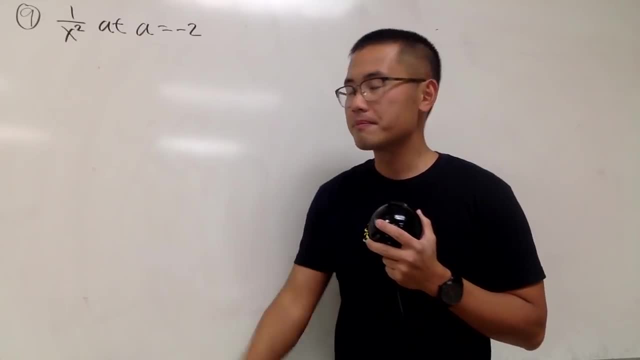 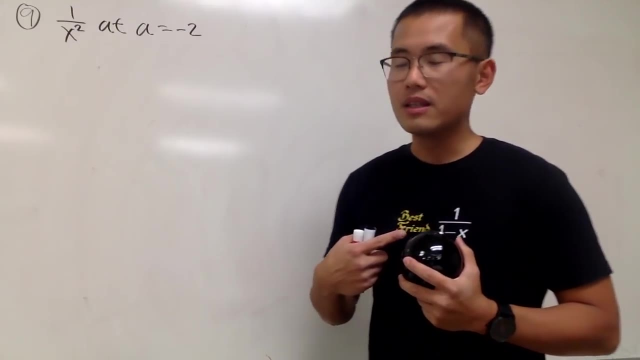 But I will show you guys how we can use our best friend for this. Hmm, Well, for the best friend is x to the first power on the bottom. huh, This is x squared on the bottom. But we know if we differentiate the best friend. 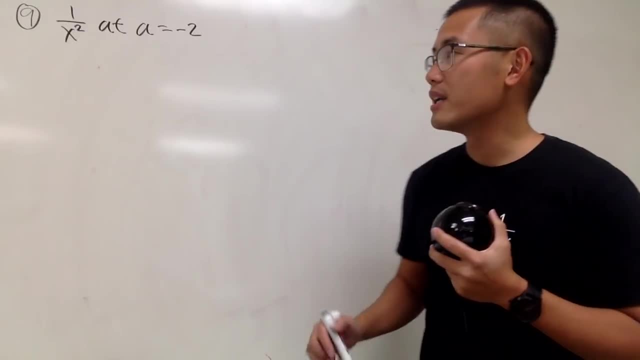 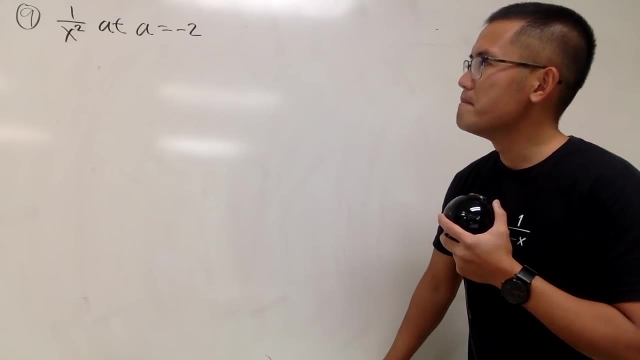 we can get the x squared something like that on the bottom, So we'll do that, But the input here is just x. Let's see how we can do it. Hmm, Well, this is how we are going to do it. 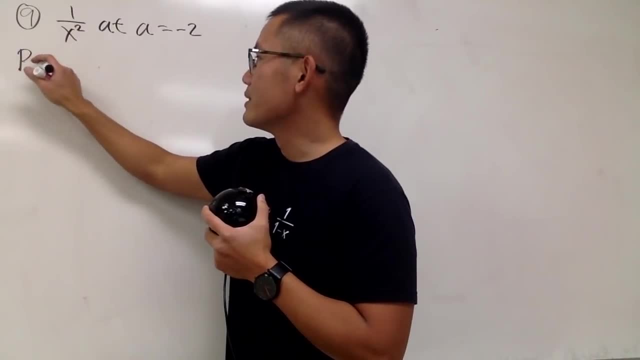 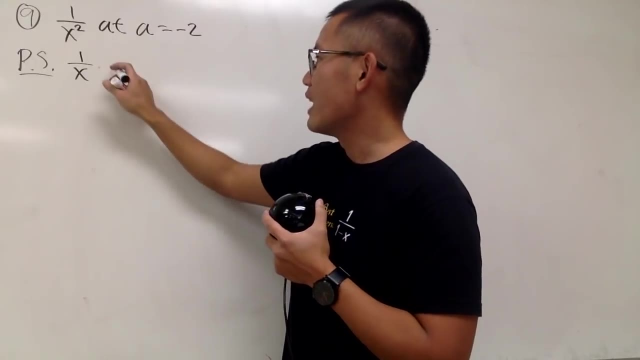 First of all, we need a power series. This is just a power series of 1 over x. I want to differentiate this guy later on. I want to look at this guy, I want this. Let me just write this down for you guys. 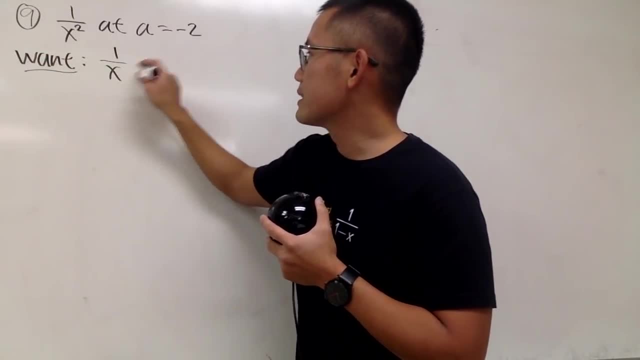 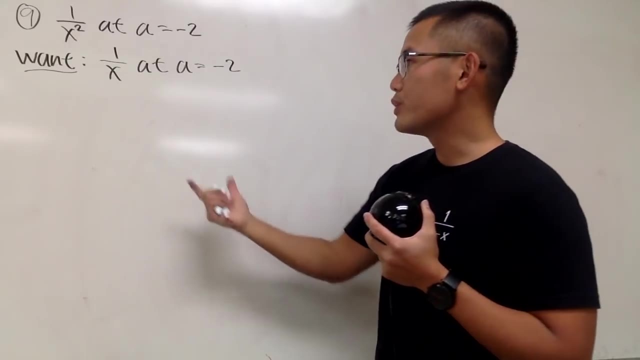 This is what you want. first, You want 1 over x at a equals negative 2.. Again, why? Because we want to just differentiate this so we can get that and it's going to be pretty fast, Okay, So let's see how we can make this happen. 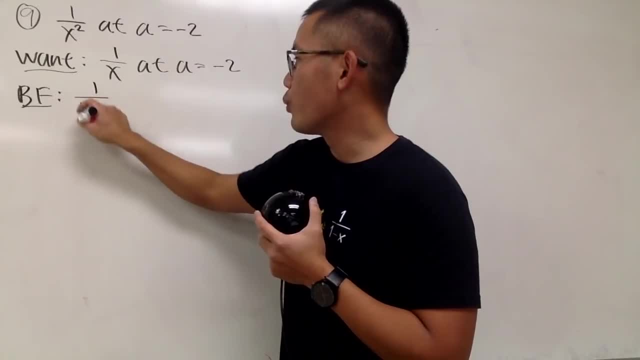 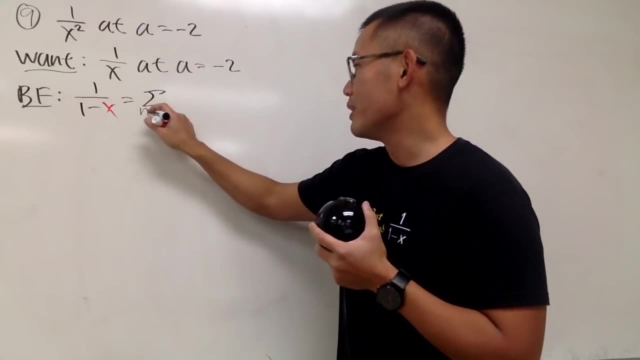 Again, here is our best friend, So let me just write this down: 1 over 1 minus x. This is some dedications. Seriously, I write down the best friend. I don't know how many times already, But I will continue to write down the best friend. 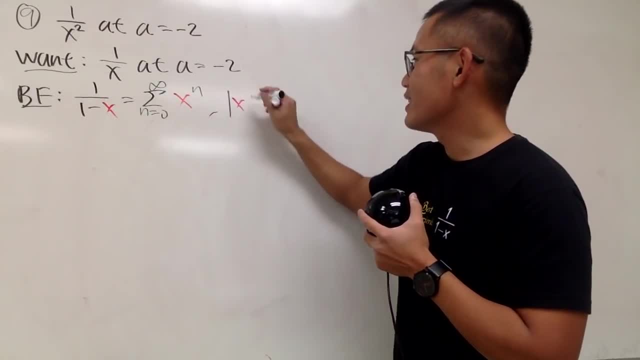 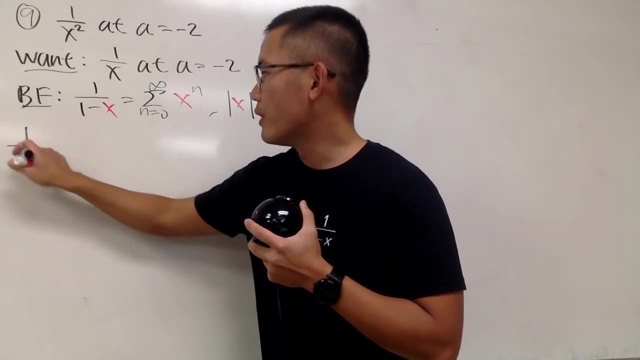 for everybody. So this is our best friend right here. Now write down the things that you want to do, which is this: Okay, So write down 1 over x, like, so This time a is at negative 2.. 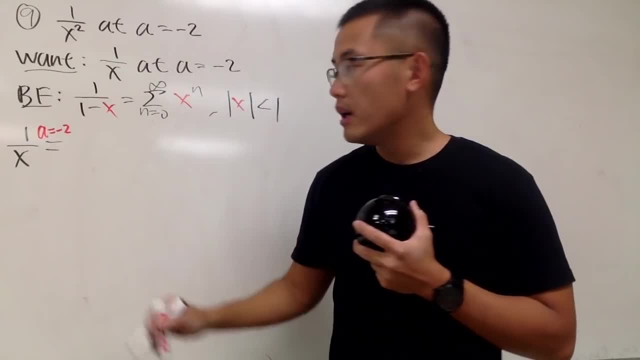 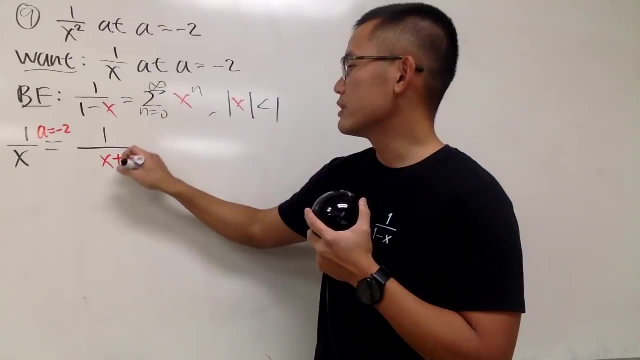 We want a to be a negative 2.. That means what That means. I need to look at 1 over. I need the input here to be x minus negative 2, which is x plus 2 like this: Hmm, Okay. 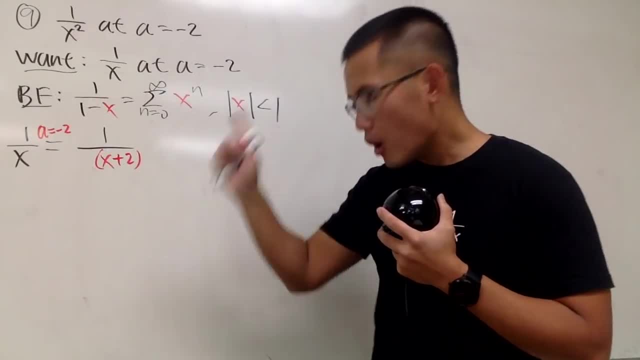 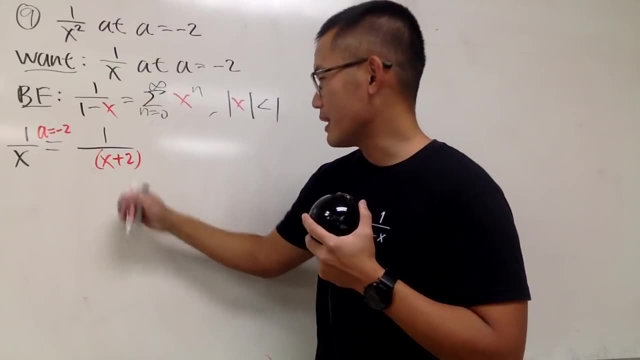 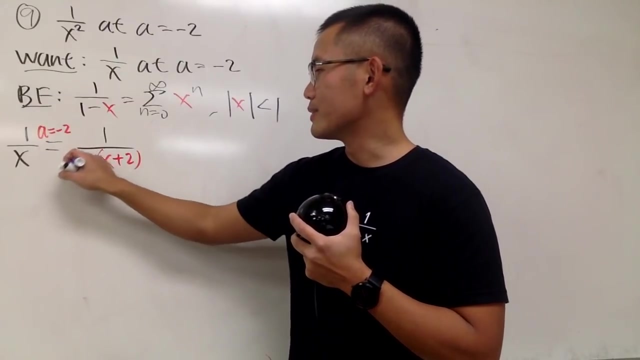 Well, this and that are totally different. but it's not bad at all because, first of all, well, I can put down as a plus: Yeah, Let me just put this down in purple, And we can just minus 2 right here. 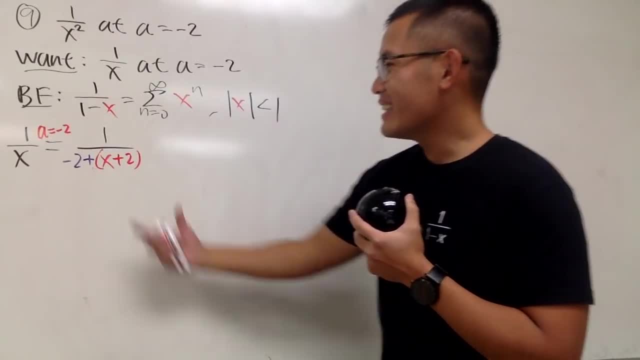 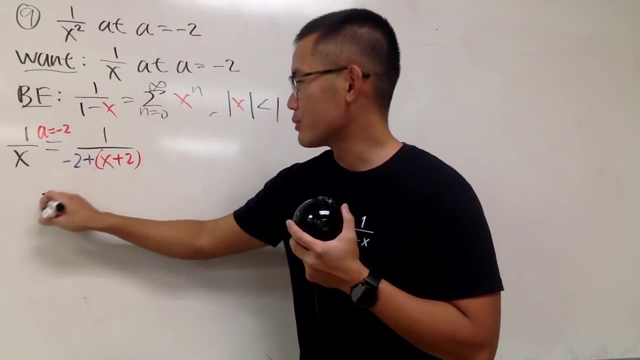 That is very good, isn't it? Again, if you work this out, you just get the x back. Yeah, So that's what we have. Then let's see. I will just do one more algebra. I will just do the algebra here. 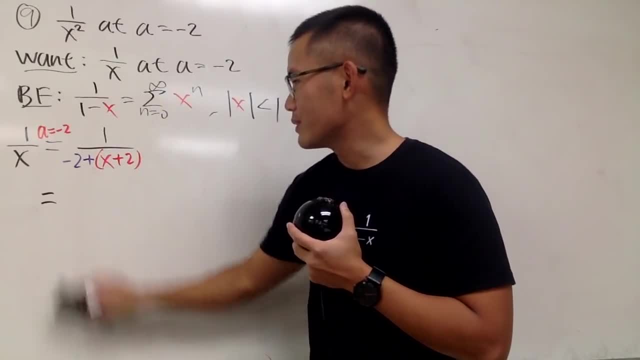 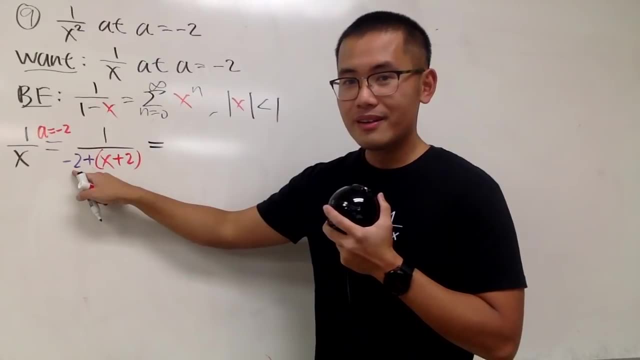 Okay To use the best friend. in order for us to use the best friend, we will use the. actually write it down here. Okay, here we go. In order for us to use the best friend, we need to have a 1 right here, right. 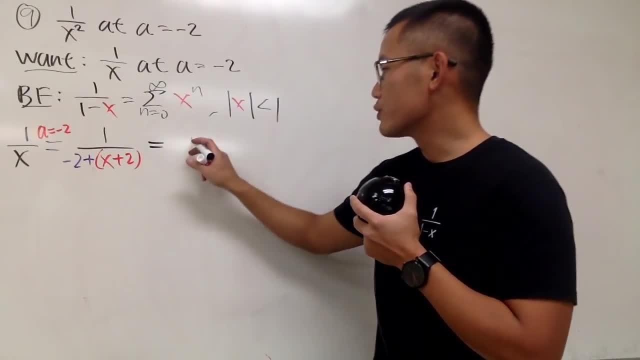 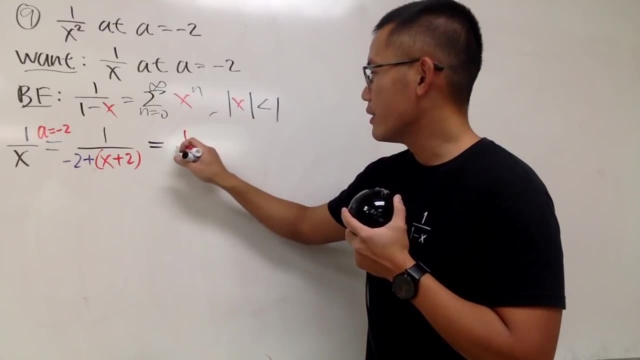 So this right here. I will just write it as 1 over. I will factor out the negative 2 right there. So I will write this down as 1, negative 1 over 2, like this: okay, Times 1 over parentheses. 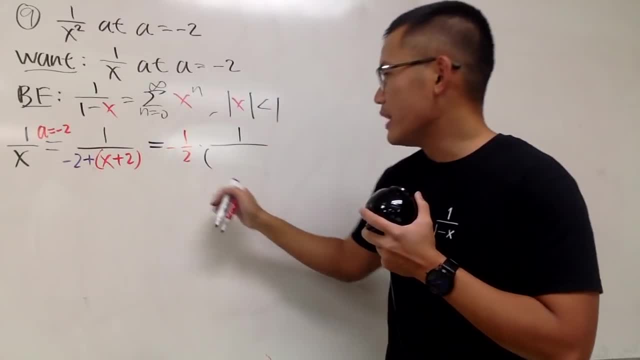 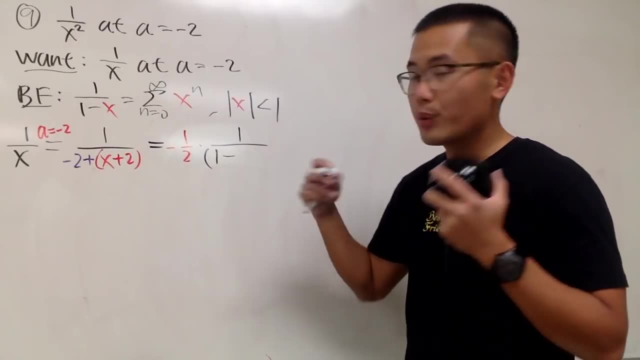 Here we go. Originally you had negative 2. We factor the out, so we just have a 1.. Then, originally we have a positive, but we factor the out a negative. so this is minus, which is much more preferred anyway, right. 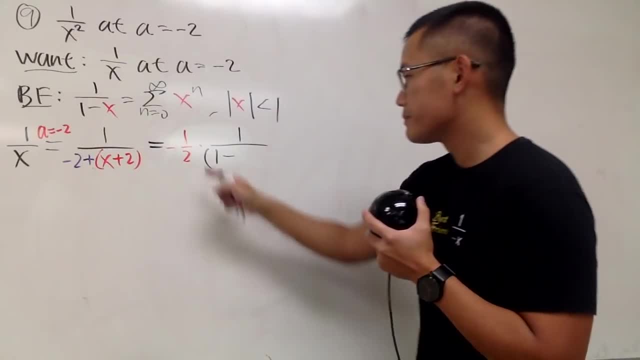 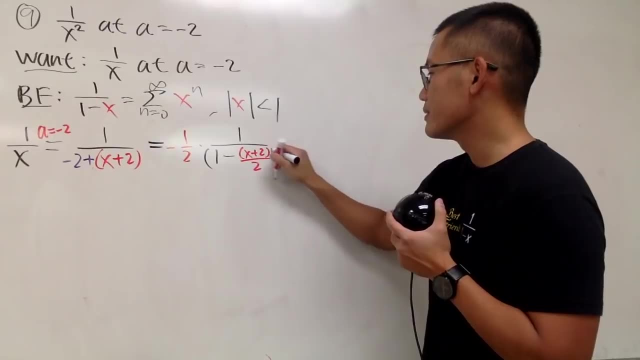 And this is what we had originally. but we factor out the 2, a negative 2, technically, and then we will just have parentheses x plus 2 divided by 2, like: so, Yep, Then we can use our best friend. 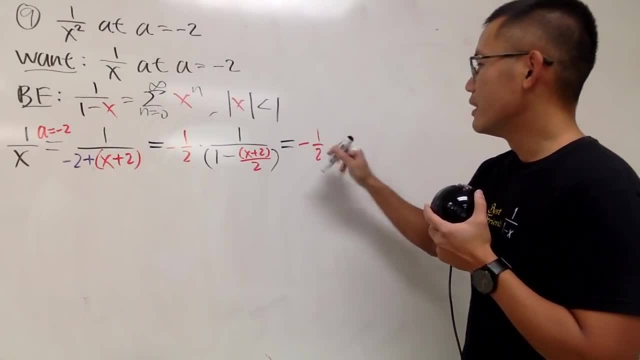 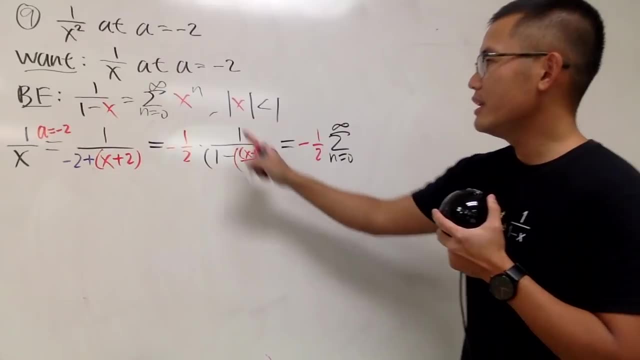 This right here is negative 1. half This right here is the sum as n goes from 0 to infinity. We just enter all this right here in, here and here, So let's go ahead and do that. So we see that this is going to be. 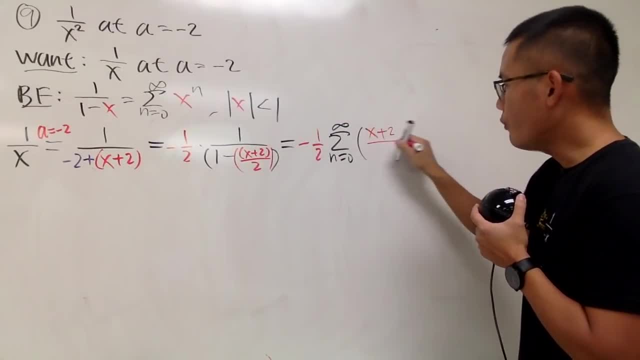 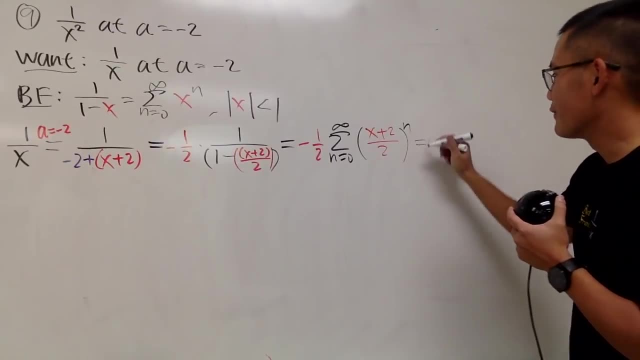 parentheses x plus 2 over 2, raised to the nth power like this, And perhaps I'll just write it down a little bit more: Here we have negative 1 over 2, and this is the sum as n goes from 0 to infinity. 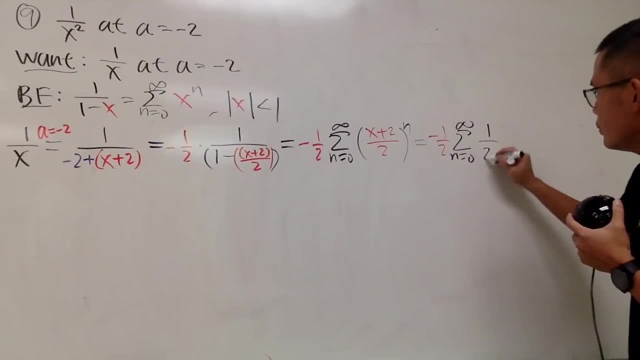 And let me write it down like: 1 over 2 to the nth power, and this right here is parentheses x plus 2 to the nth power, like this: And finally, I'm going to just write this down for you guys, I'm just going to multiply the negative in: 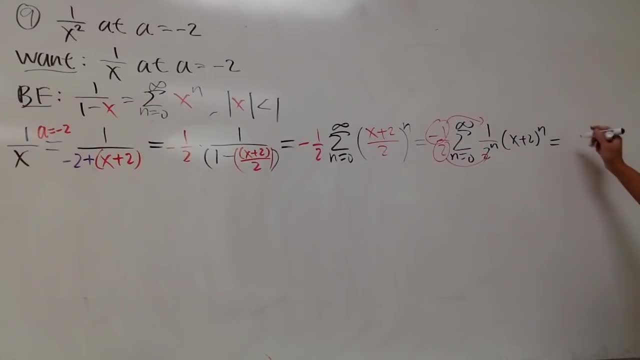 and then distribute this here, so we get the sum as n goes from 0 to infinity and we have negative 1, so it's negative 1 over 2 to the n plus 1's power, and then we have this: 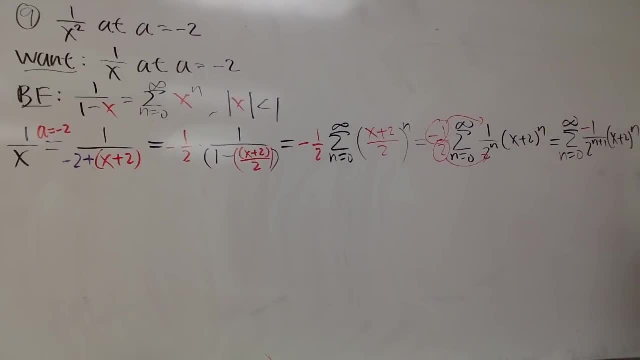 which is x plus 2 to the nth power. like this right, I know you guys might not be able to see, but don't worry, I will write it down over there again anyway. Then why did I write it down here? 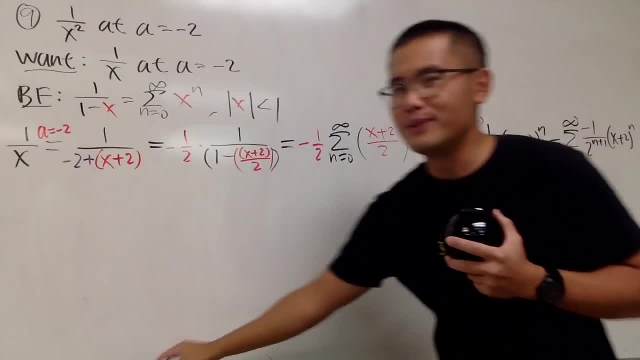 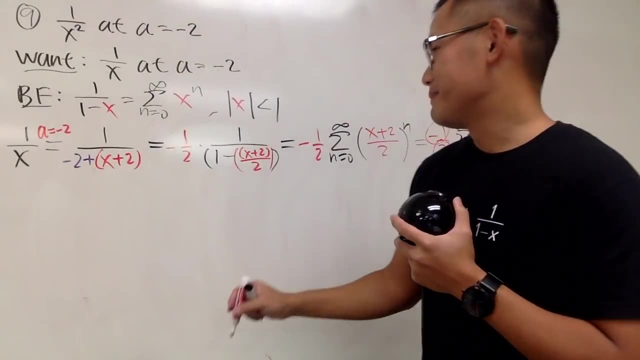 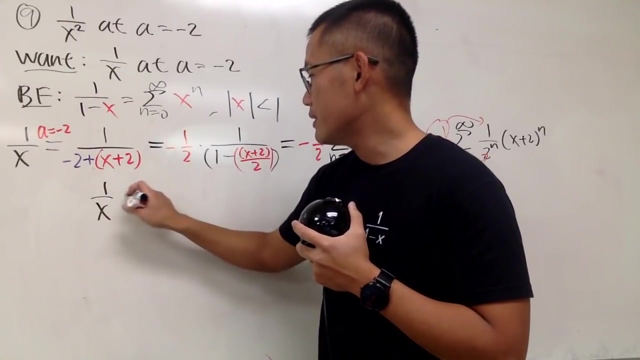 I don't know, I don't know. Okay, So I'm just going to write it down over here. Anyway, what this is doing is the following: We know that 1 over x is going to be this. We have the series. 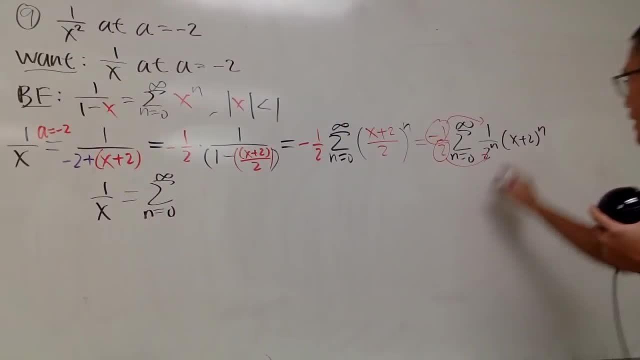 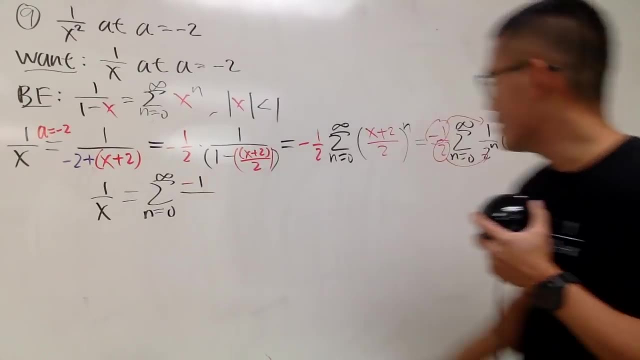 n goes from 0 to infinity. Again, do the algebra that I was doing, but it's raised for no reason. Here we have the negative 1 over 2 to the n plus 1 power right here, so I'll just put that down. 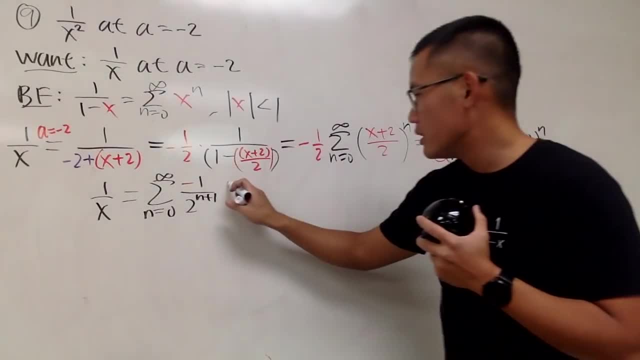 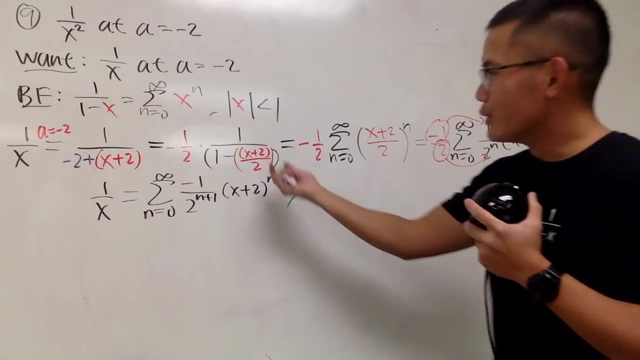 and that's the coefficient. and then here we have the x plus 2 raised to the nth power, like so, okay, And don't forget to enter this right here in the absolute value as well. So I'll do that right here, real quick. 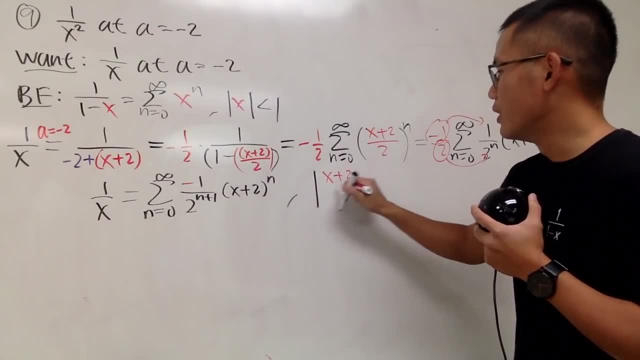 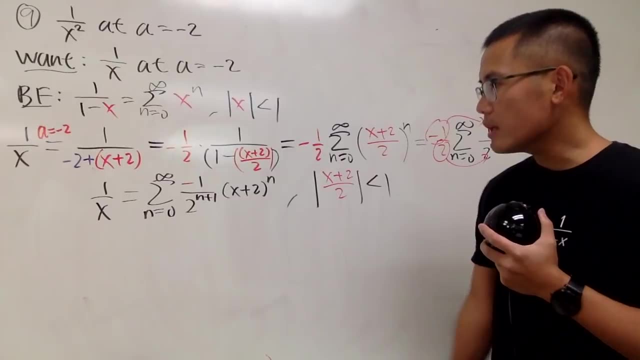 Absolute value and x plus 2 over 2 is less than 1.. So again, multiply both sides by 2, we'll get the answer for that. Anyway, this is not the main deal. The main deal is that we will differentiate both sides. 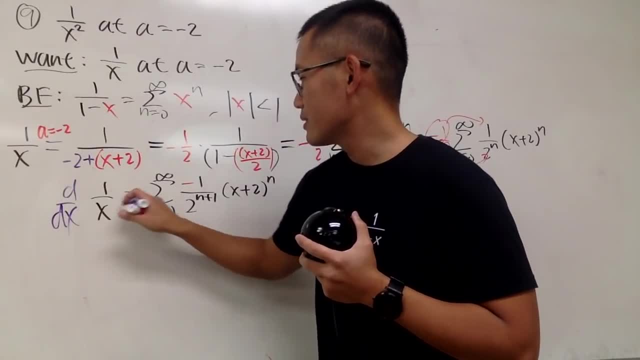 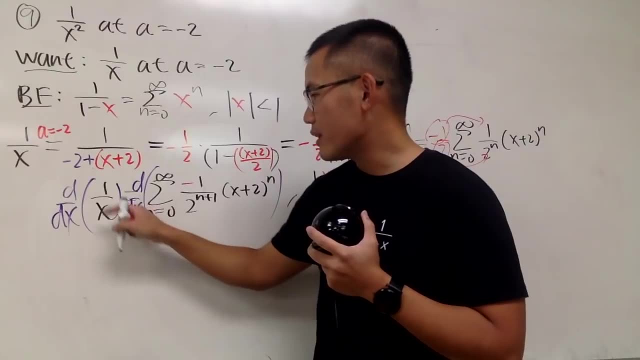 So d? dx, let's just put on d? dx and d dx. Okay, so differentiate the left-hand side, this right here, this radius x to the negative 1 power, bring the negative 1 to the front and you get negative. 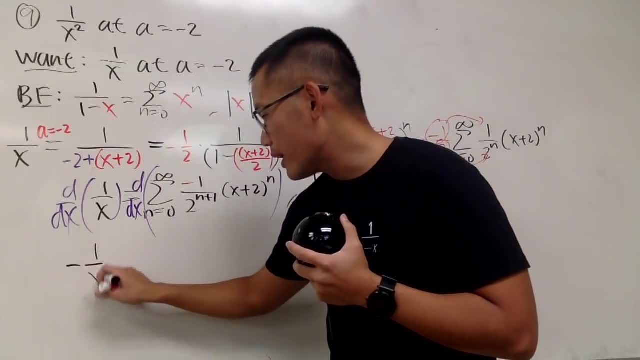 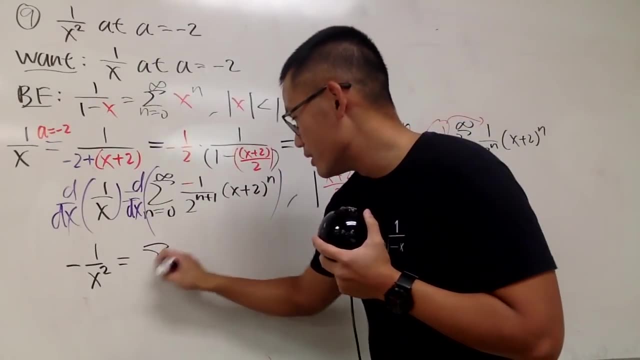 and you get x to the negative 2 power. so you get 1 over x to the 2 power. like this Right-hand side man, I love differentiating power series. Very, very fun, You'll see. Oh, by the way, 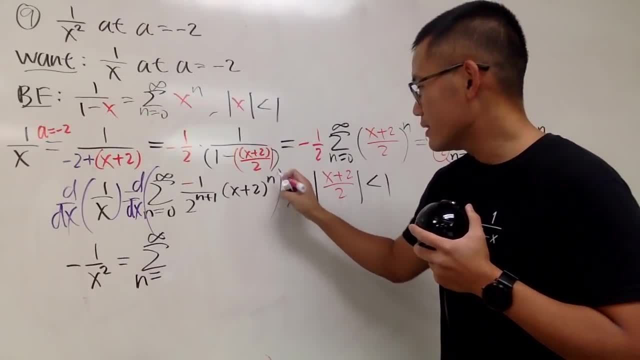 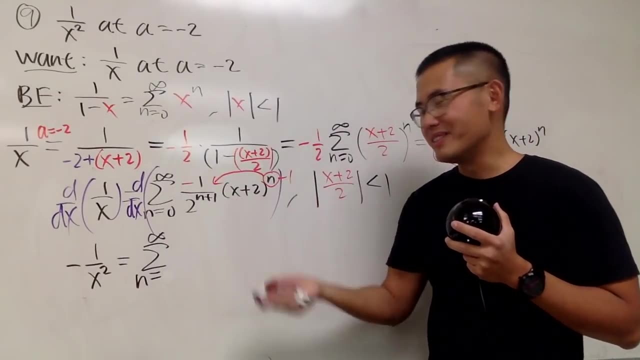 okay, here we go. First of all, you bring the power to the front, and then minus 1, and you are done The Chengdu right. here it's always going to be 1, because, remember, it's always going to be x minus a right. 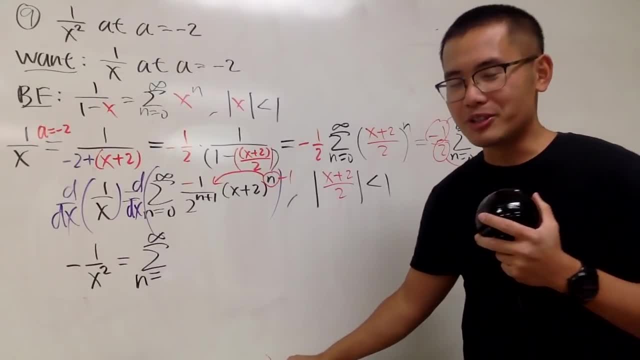 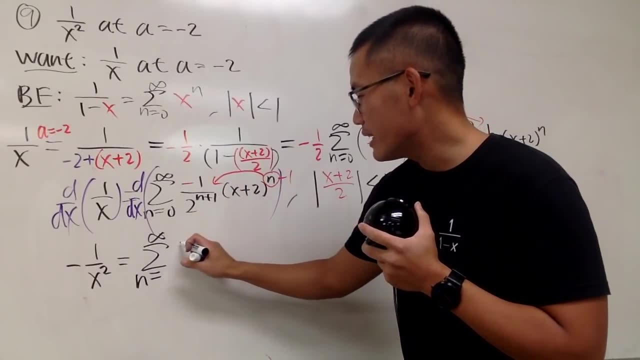 So the Chengdu is just always going to be 1.. So if you forget about the Chengdu, you know you are safe. this time, Anyway, bring the 1 to the front This time. this is just a negative n okay. 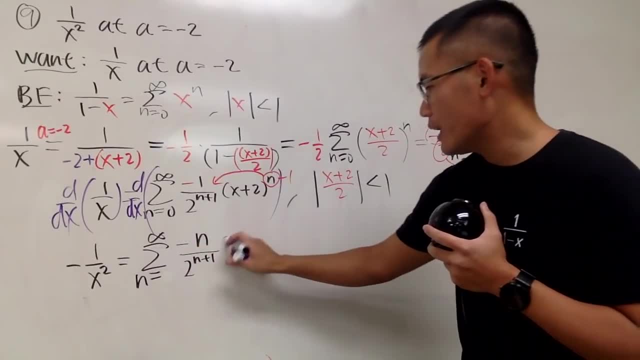 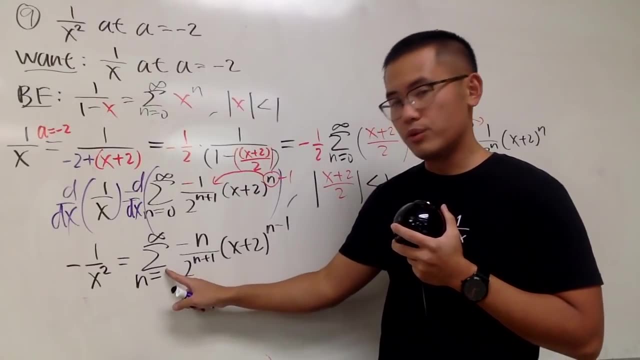 And then over this is 2 to the n plus 1 power, and then we have the x plus 2 raised to the n minus 1 power. But now, if you put n is equal to 0 in here, the first term will be 0.. 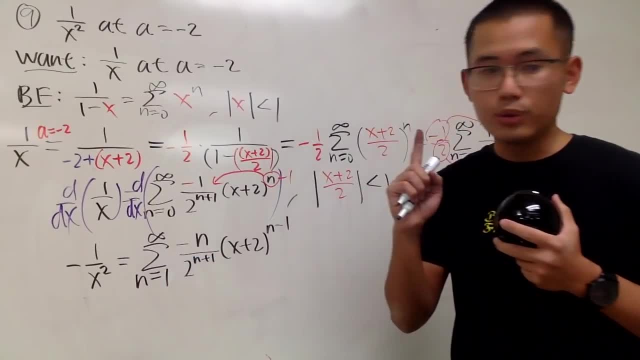 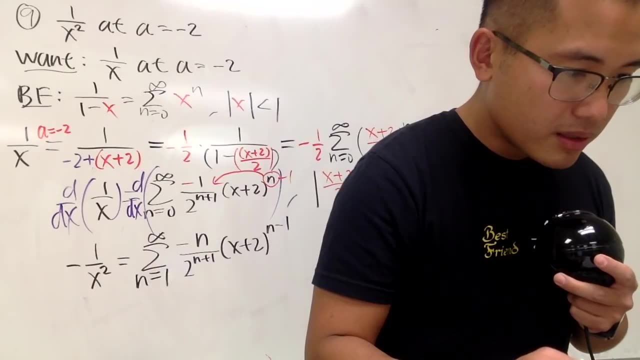 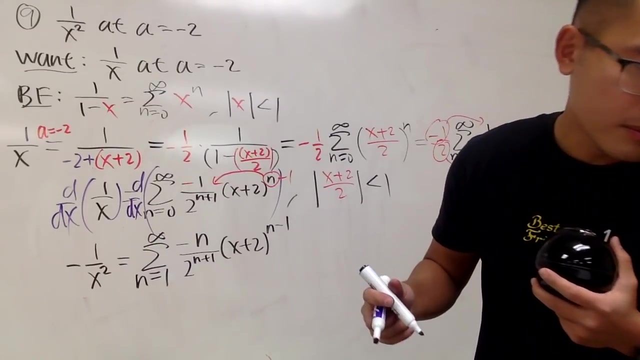 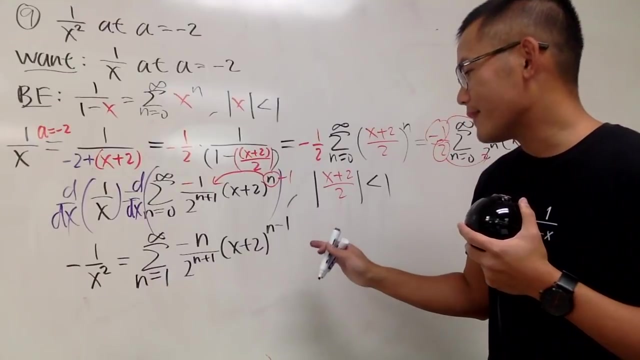 So you can skip that. You can just start with: n is equal to 1.. And let me just double check: my answer key had that. Oh, let's see. Oh, yeah, Now, this is the first and a half. 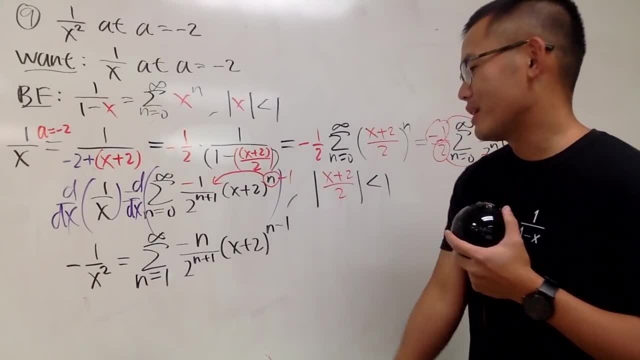 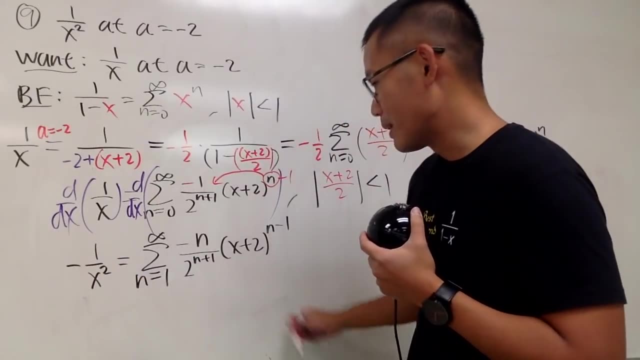 This is not the first and a half on the answer key, but I'll tell you guys what I mean by the one and a half n on the answer key. Anyway, not done yet. This is negative. That's negative. Of course. we can just multiply both sides by negative. 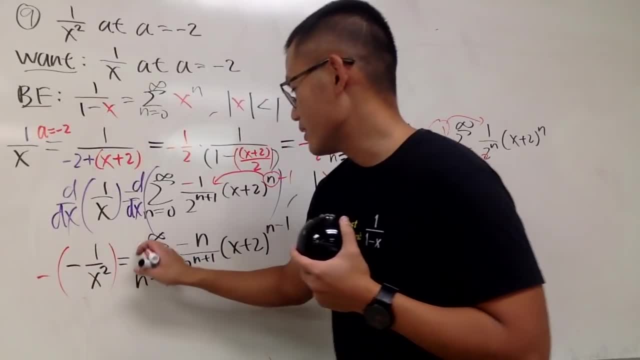 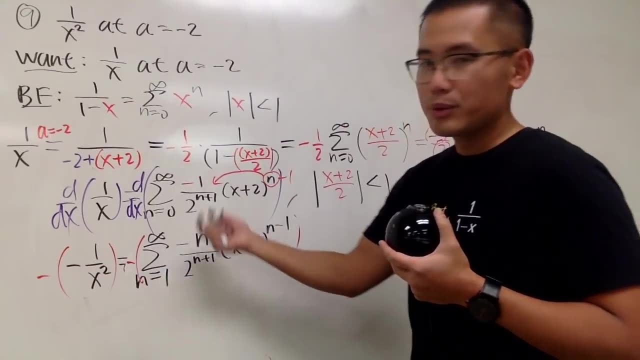 So just multiply, Man. multiply both sides by negative. however you want to write it, Yeah, So that this and that cancel Man. I will just write this one more time. So this is 1 over x squared. 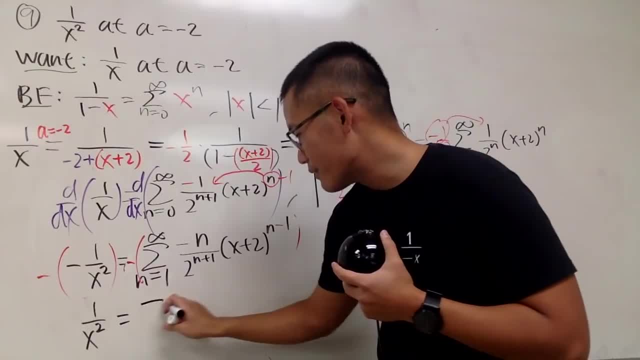 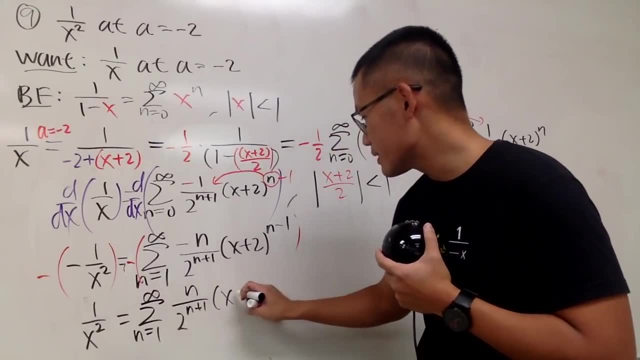 and this is equal to next time. this times that cancel. So you have the sum: n goes from 1 to infinity, n over 2 to the n plus 1 times x plus 2, raised to the n minus 1's power, like this: 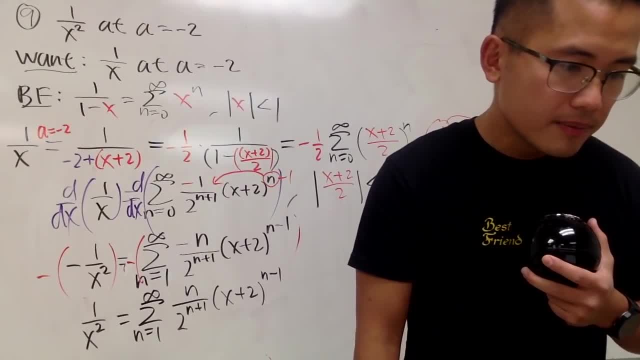 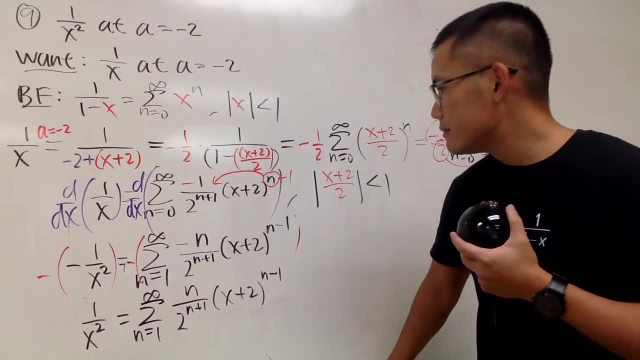 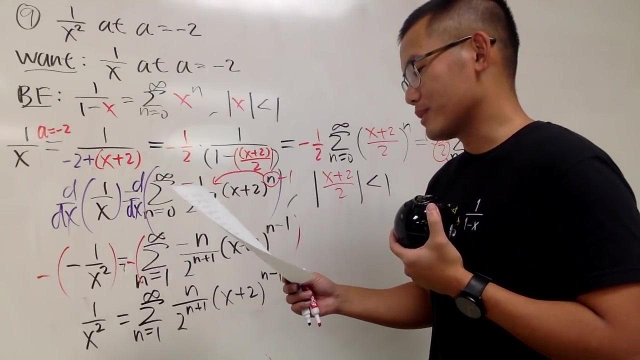 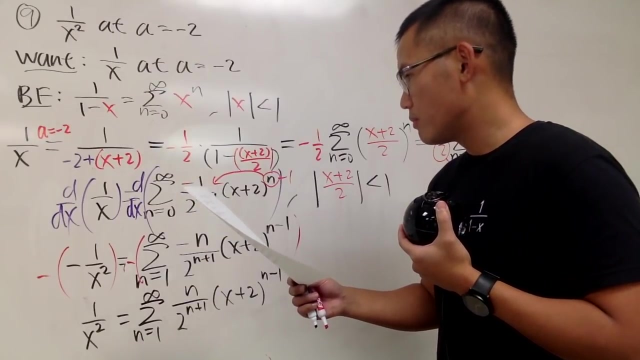 Okay, Then let's see. Wait, let me just double check my answer key. Most of the time it looks like the one I'm doing is correct. My answer key is not correct, So that's the one I'm trying to fix. 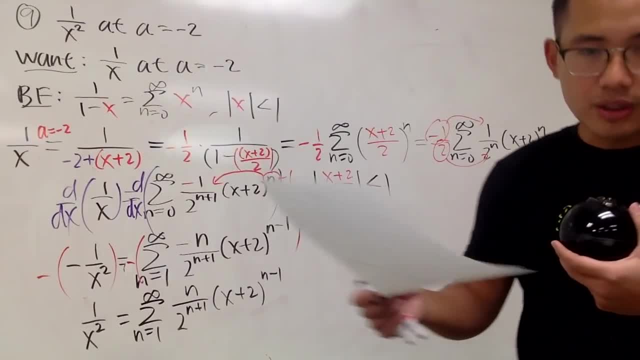 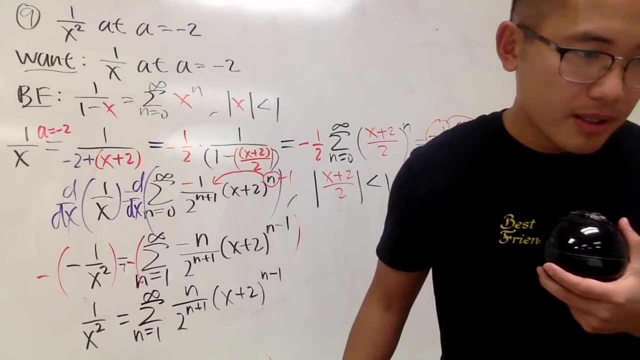 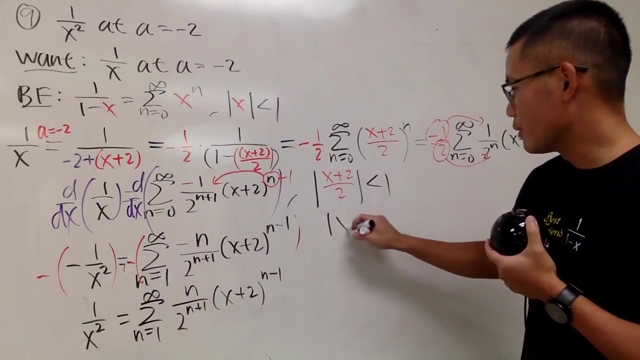 Let me just double check, triple check, Yeah, So I will just triple check the answer key later, right here, Yeah, Anyway, though, right here, just work this out real quick so you get the absolute value. So if you multiply 2 on both sides, 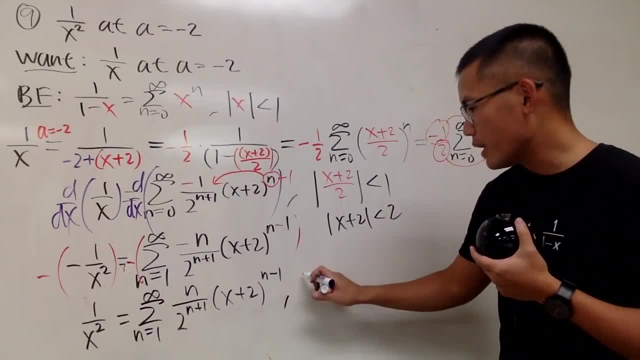 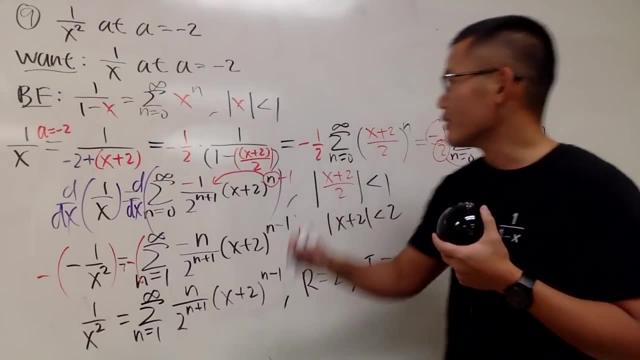 so x plus 2 is less than 2, so you know right away: r is 2.. Now the i, the center this time is 2.. So let me draw a picture for you guys real quick. Oh, the center is a negative 2.. 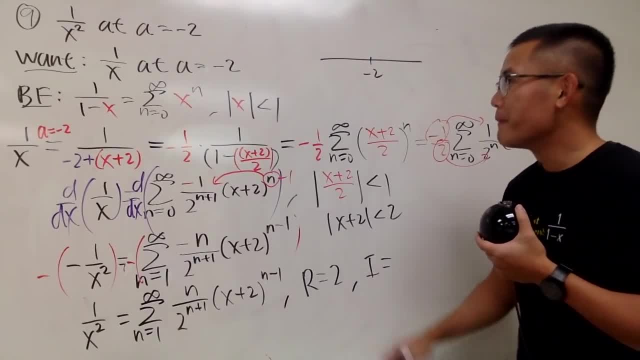 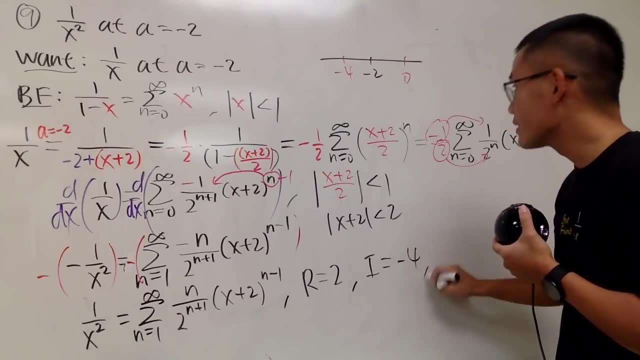 My bad, The center is negative 2.. Yeah, And you go to the left twice, which is going to be negative 4, and you go to the right twice, which is 0. So you actually get negative 4, comma 0,. 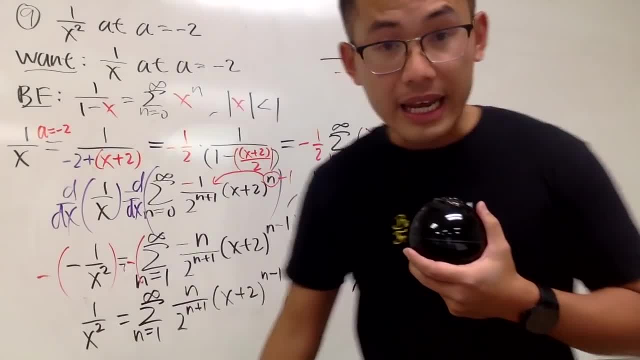 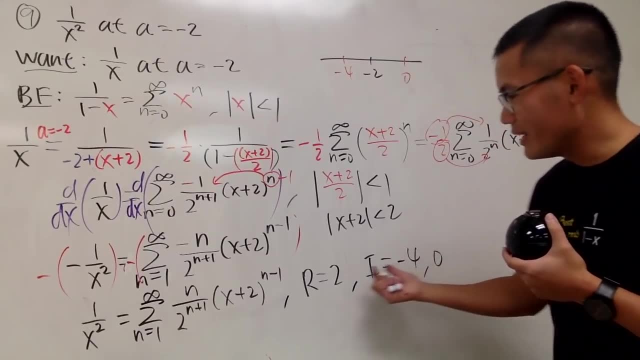 like: so, Yeah, Okay, And what you are going to do is: hmm, well, again, you should plug in negative 4 in here to see if it converges or not. But if you plug in negative 4 in here, 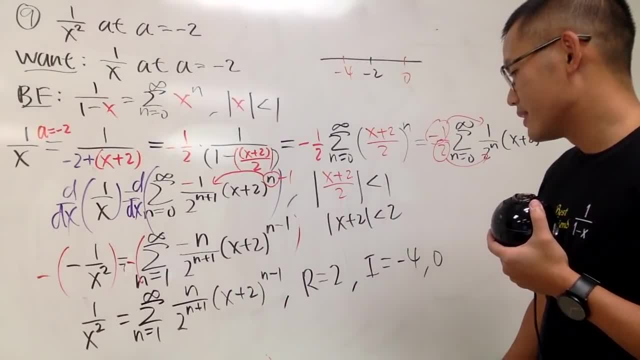 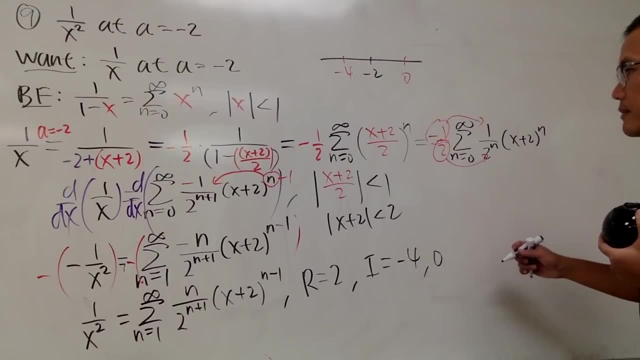 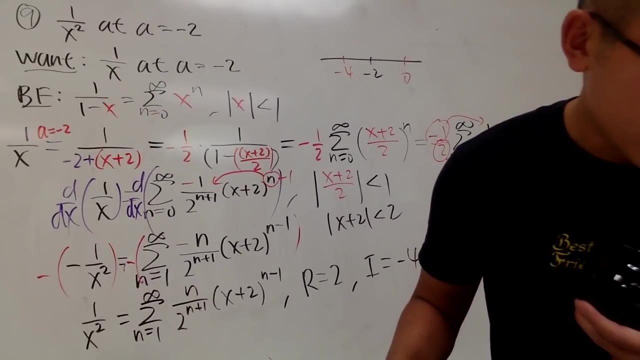 then you will see. let me see check negative 4, man, Let's see, let's see. I just want to make sure, why did I do that? I think I got this answer from Wolfgang Alpha also, then that's why I'm like: 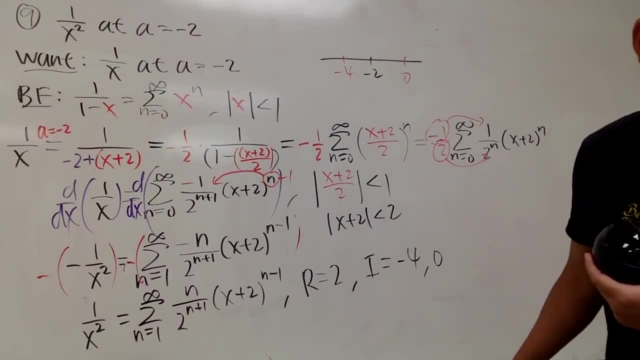 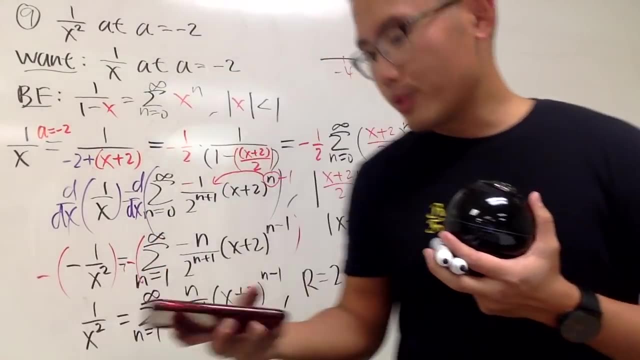 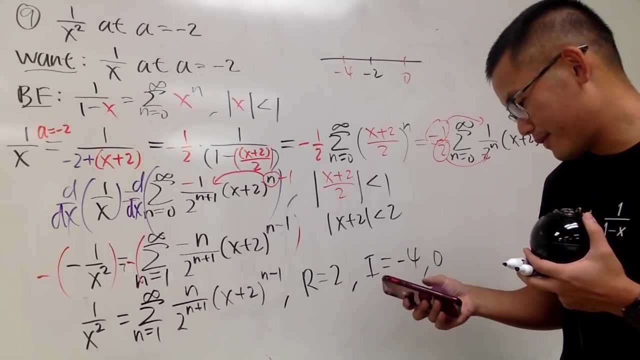 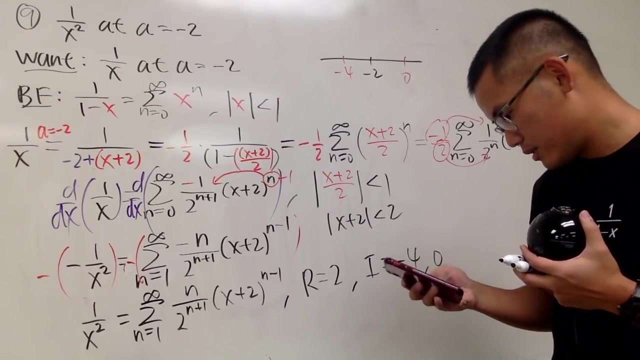 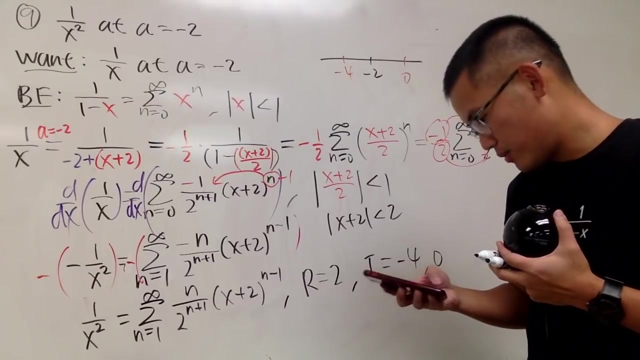 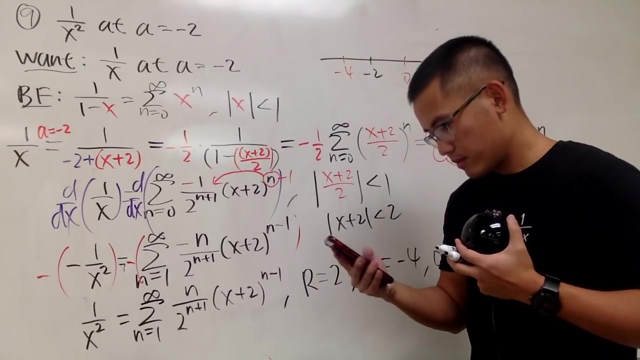 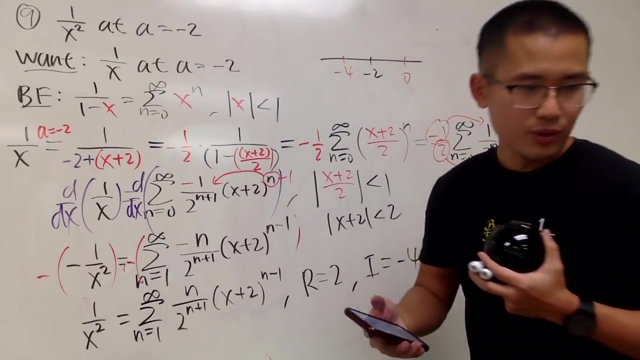 hmm, Let me just double check on Wolfgang Alpha real quick. Nothing wrong with this. I just don't let me see power 1 over x greater, yet negative 2.. Oh, so I do have a typo on my answer key. 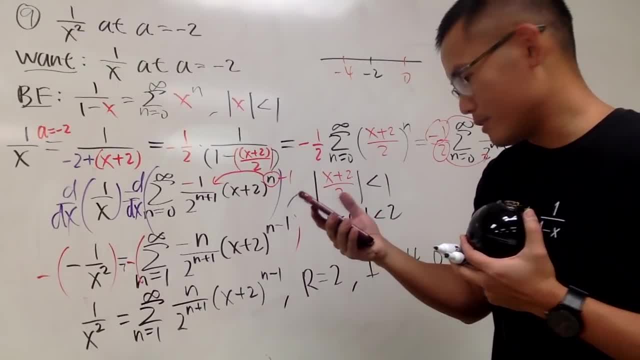 so I will fix that for sure. I don't know why I'm saying that five times already, but let me just see: 1,, 2,, 3,, 4,, 5,, 6,, 7,, 8,. 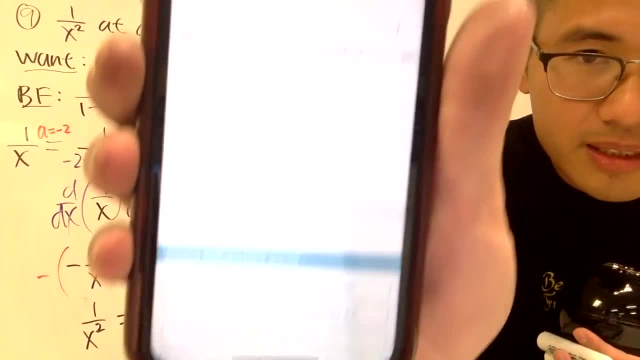 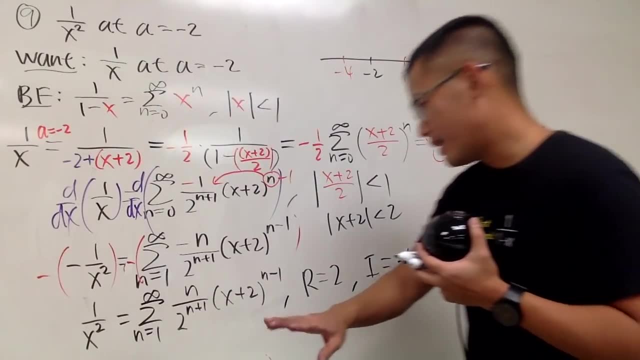 9, 10.. Yeah, So on Wolfgang Alpha, you can see. that's the answer. Maybe you guys cannot see, But it's just that I fixed the index, So sometimes it's annoying, but this is okay, All right. 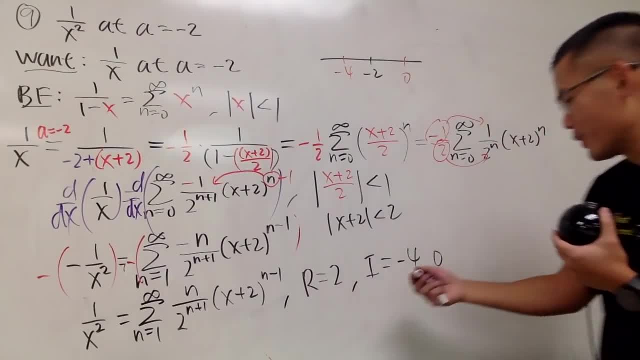 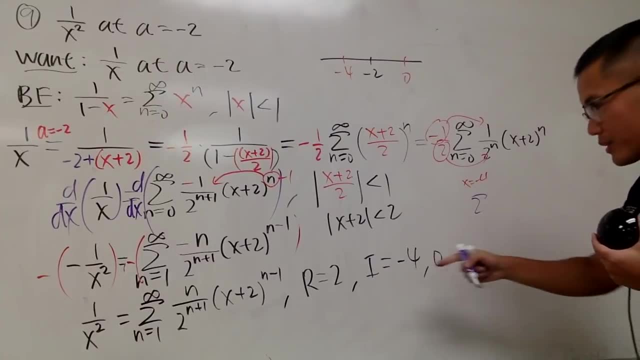 So what you are going to do next is just go ahead and do a quick check. When x is negative 4, check this, okay, So you get the sum. This is when x is equal to negative 4, okay, Just go ahead and do that real quick. 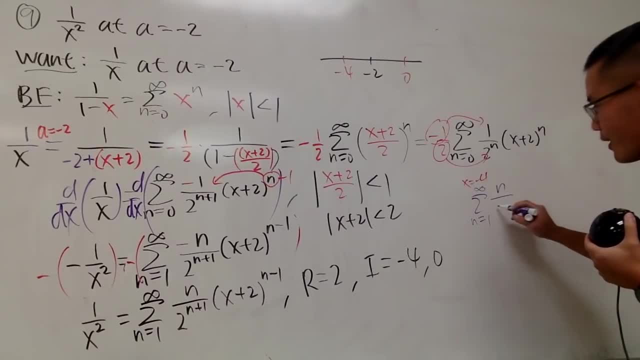 n is equal to 1 to infinity, and you have n over 2 to the n plus 1.. And when you put negative 4 in there, you get negative 4 plus 2, and you have the n minus 1's power. 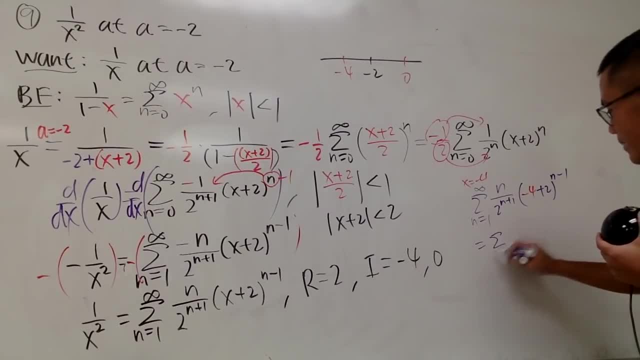 All right, And what you do is this. This right here is going to be: the sum: n goes from 1 to infinity, n over 2 to the n times 2 to the first. This right here is going to be negative 2.. 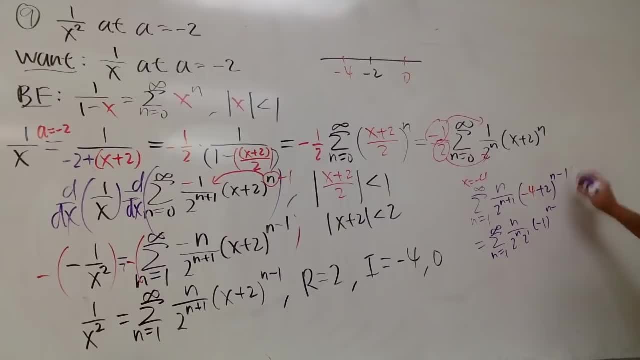 So I will have negative 1 to the n plus 1's power times, and if you do negative t1 already, so this will be 2, and then you have the n times 2 to the negative 1.. You see this and that will cancel. 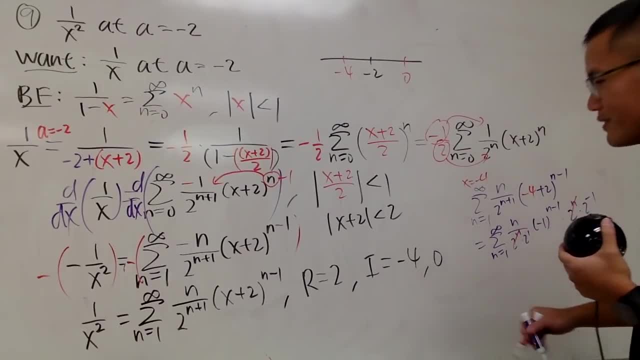 This right here diverges because similar to what we did in the previous question. So this right here is parentheses. If you have 0 here, it's going to be a similar situation, So you will have this n. that will be bothering you. 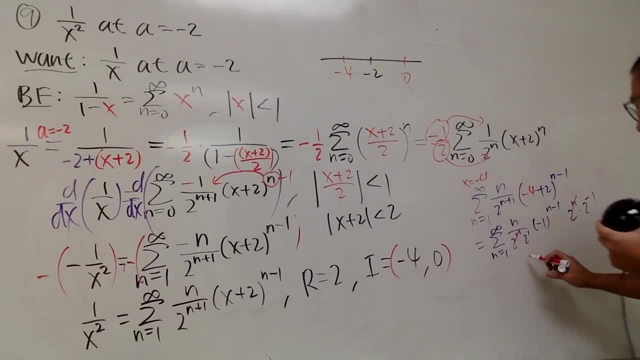 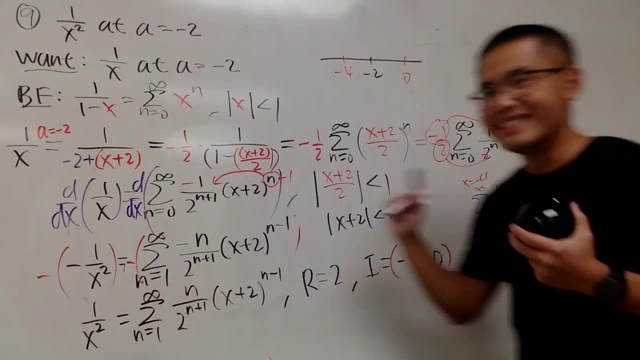 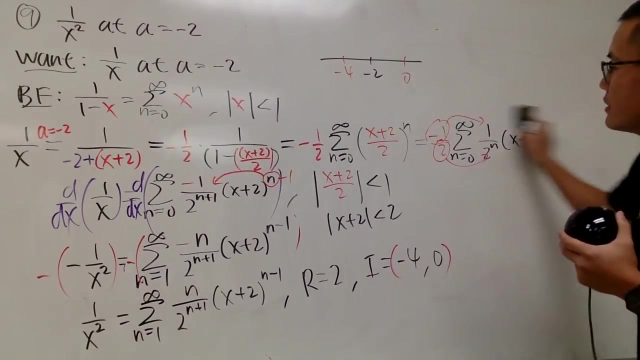 and that will not be convergent. So just use the test for divergence. So the limit doesn't exist. Anyway, I will leave this to you guys for that part. Okay, so that was number 9.. It took some time for that. 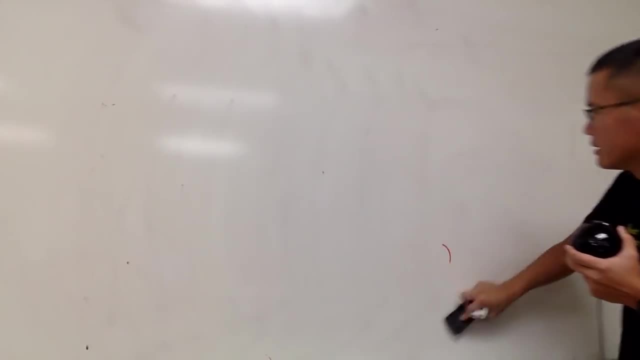 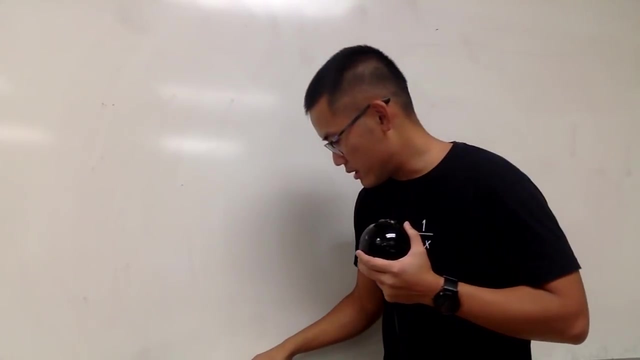 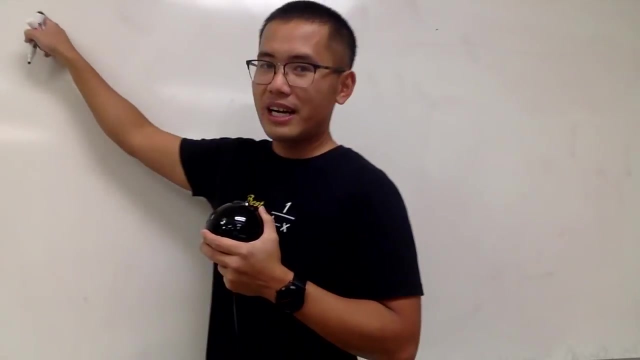 Now I will fix the typo on my answer key And yeah, let's see. Okay for the next one. man, let's see, let's see. Still kind of like best friend. you will see why, though, This is number 10.. 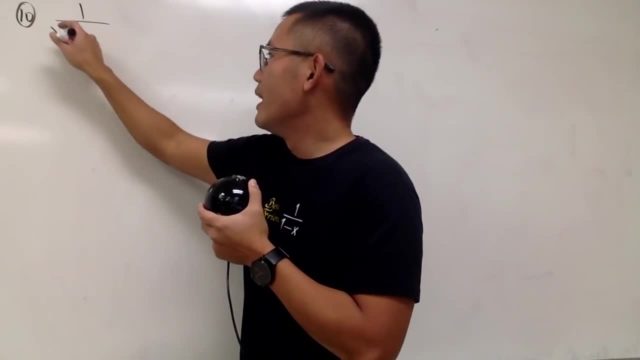 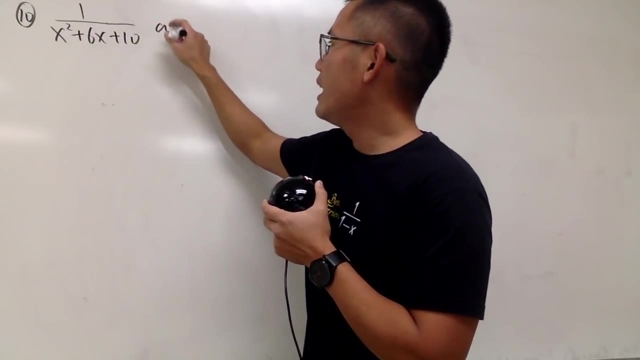 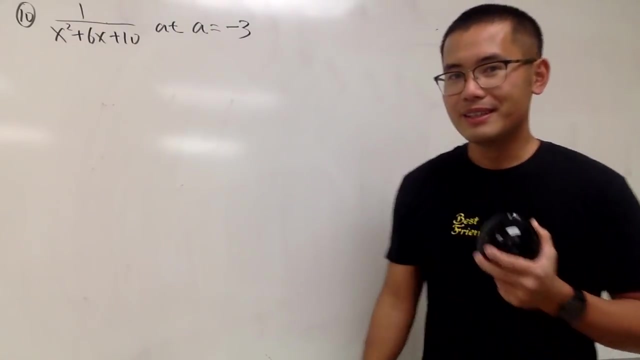 We have 1 over. and here we have a quadratic again, but this time it's three terms: x squared plus 6x plus 10x, Add the center negative 3.. Okay, What do we do? Can we factor it? 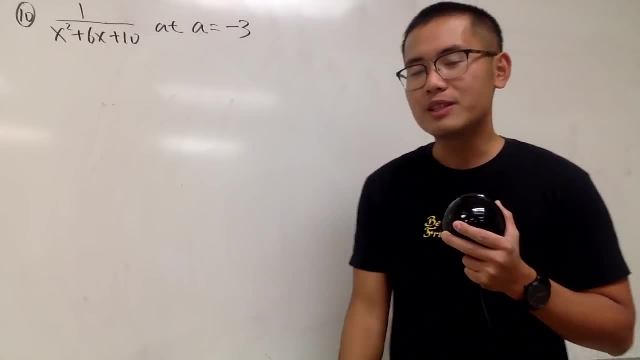 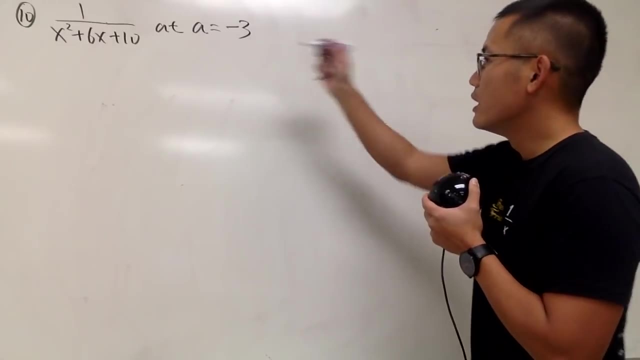 Unfortunately not. Can we complete the square? Yes, we can, So let's go ahead and do that. So perhaps I will just put on the completing square on the side for you guys real quick. If you look at x squared plus 6x: 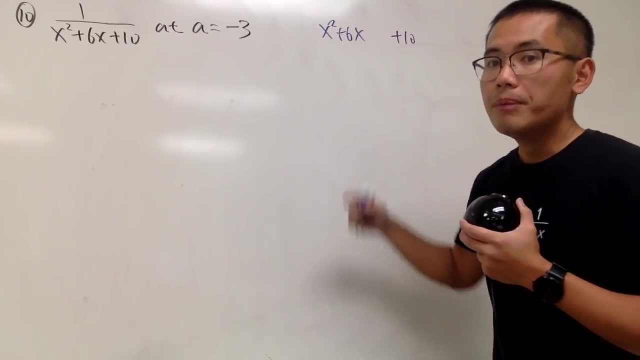 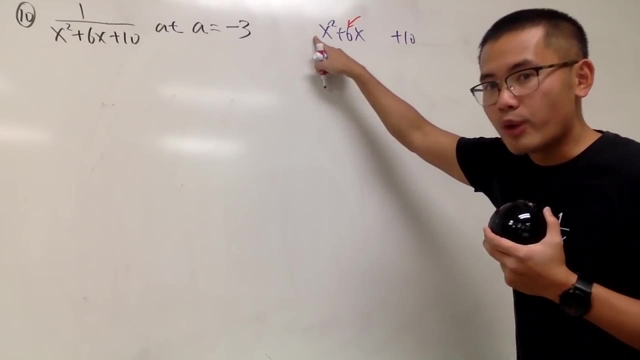 and let's leave a space. Let me just put on plus 10 right here, because for this we will have to use the magic number To do so. you look at this number. Be sure that you have the 1 in front of the x squared. 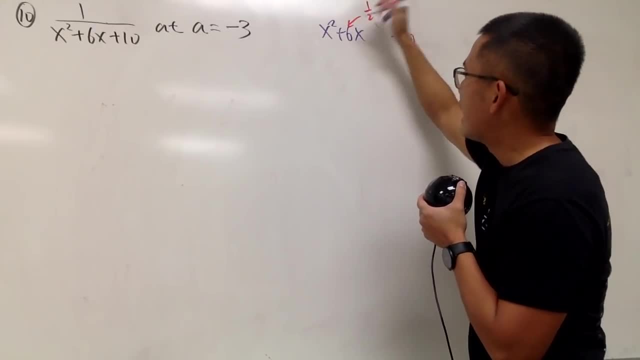 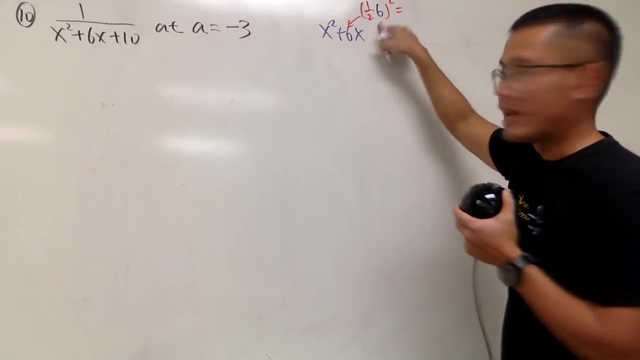 which we do. So take 1 half times the coefficient of x and then square that. This right here is 3 squared, which is 9.. So go ahead and just add 9, but we will have to minus the 9,. 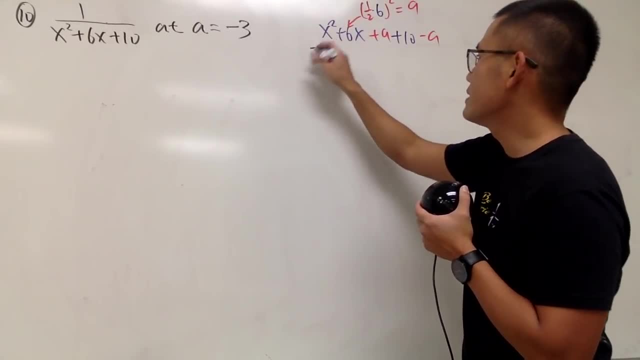 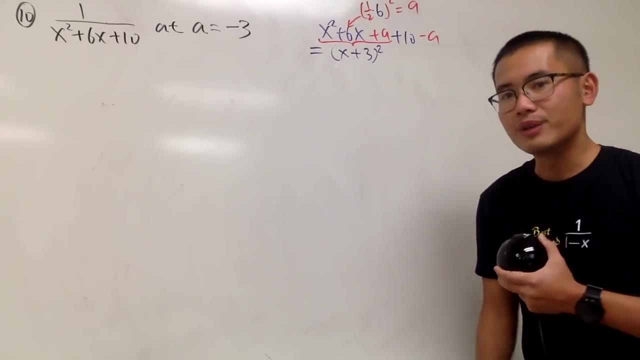 so that you don't change anything. The left-hand side- well, not the left-hand side, this side, this 3 terms- is just going to be x plus 3 squared. If you complete the square, if you factor, you get x plus 3 squared. 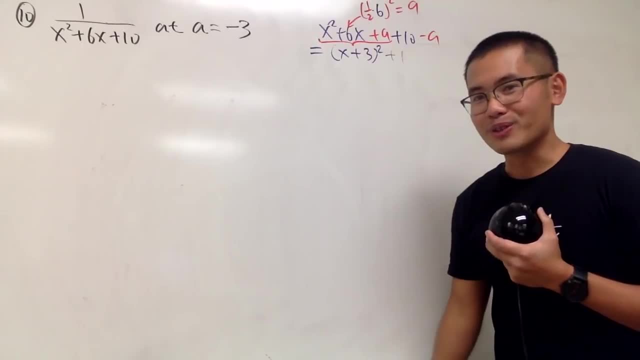 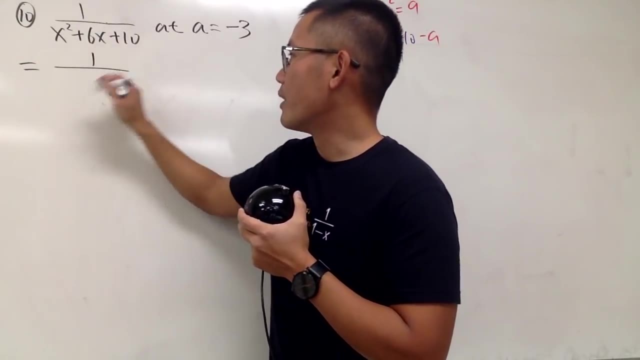 And this and that is going to be plus 1.. So this is an irreducible quadratic, But it's actually pretty good. You'll see why This right here on the bottom now is 1 over. I will just put down 1,. 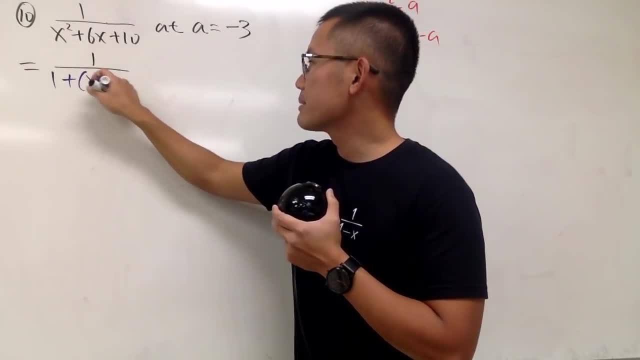 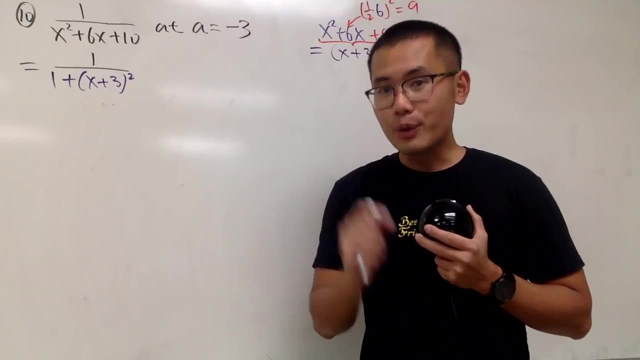 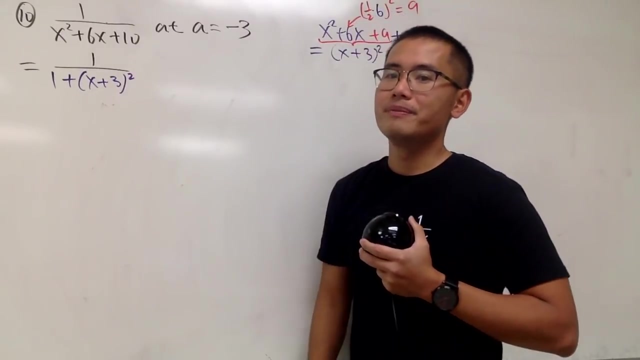 goes first, okay, Plus parentheses, x plus 3, squared like. so Here is a really really good part, Unlike the questions that we did earlier. you have to kind of get like weird stuff right. You see, the input here is already x plus 3.. 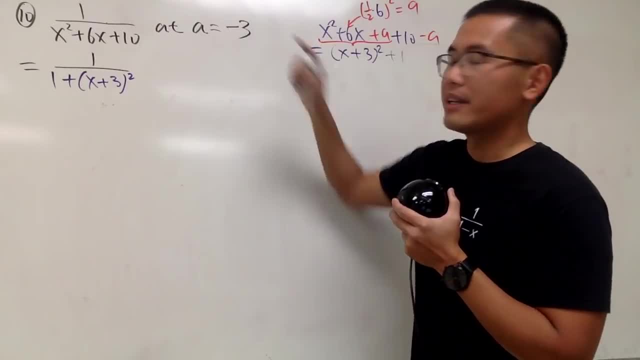 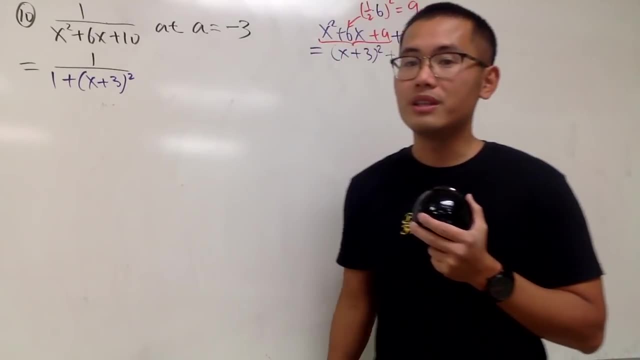 When you have the a, it is at negative 3.. That means you have to have x minus negative 3, namely the x plus 3, which we do already. And yes, you might be wondering what if you have this? 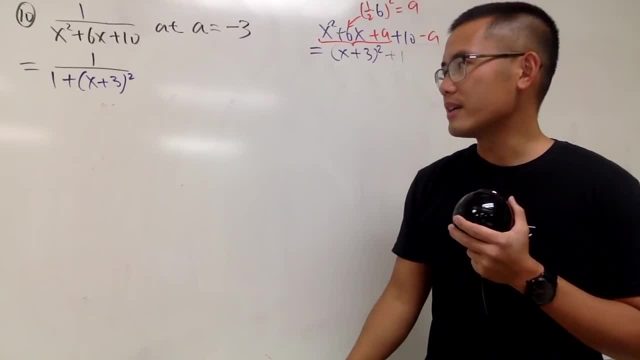 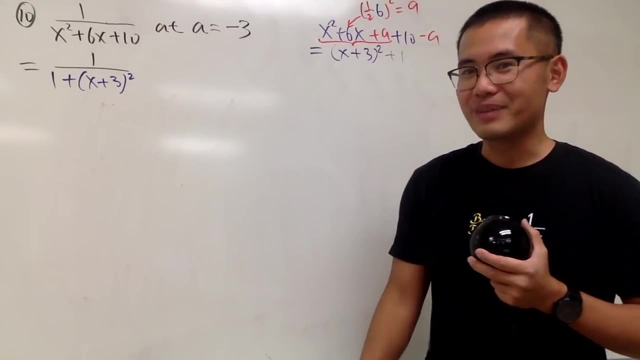 and you want the center to be a 0, or you want the center to be at like 5? I will tell you, the question might be much more difficult than this, But that's not the plan for today, so maybe next time or so. 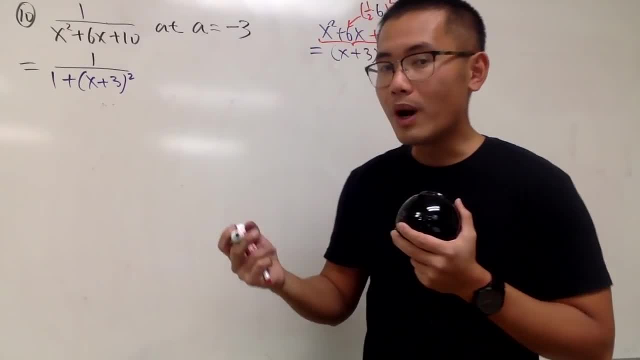 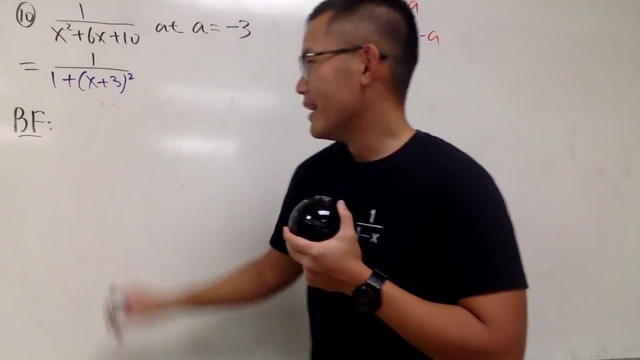 Alright. so to do this now, what we want is the following: Again, use our best friends, Do our cousins' cousin or so. Anyway, put down the best friend one more time: 1 over 1 minus x- This right here is equal to the sum. 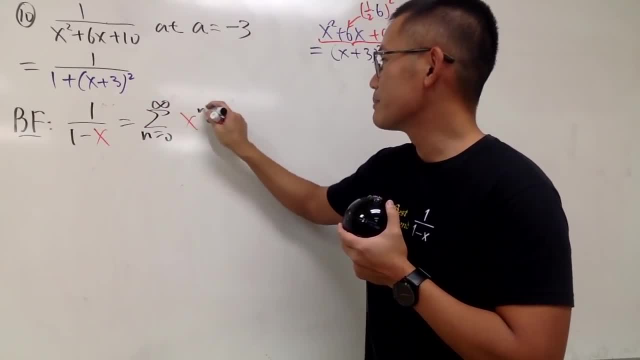 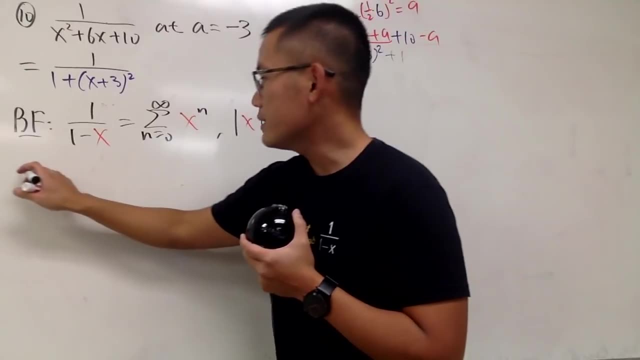 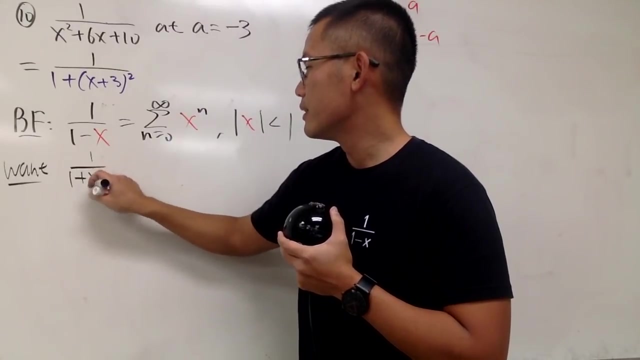 as n goes from 0 to infinity, x to the nth power, absolute value of x is less than 1.. Well, if you look at the big picture, this is what we want. We want 1 over 1 plus x squared. 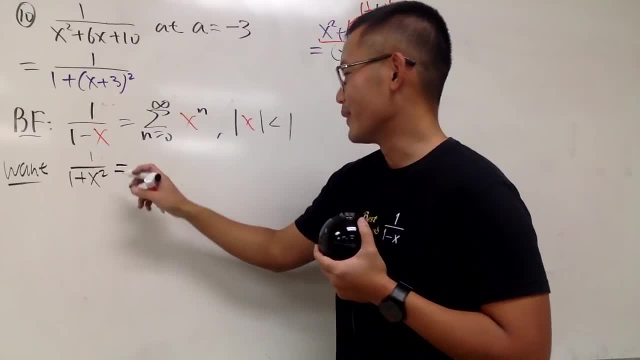 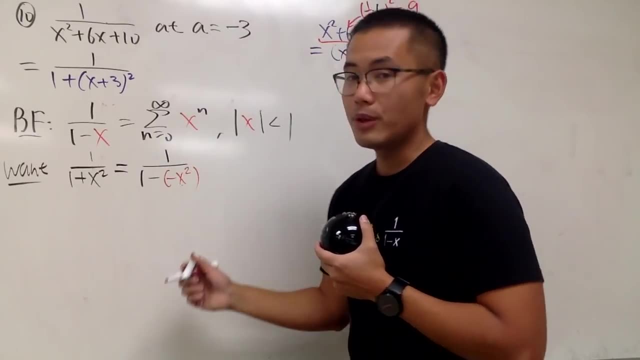 Which is actually not so bad. Why did I make that noise? I don't know. This is actually not so bad. This is 1 over 1 minus negative x squared. We did that a few times already And I can just put this right here and here and here. 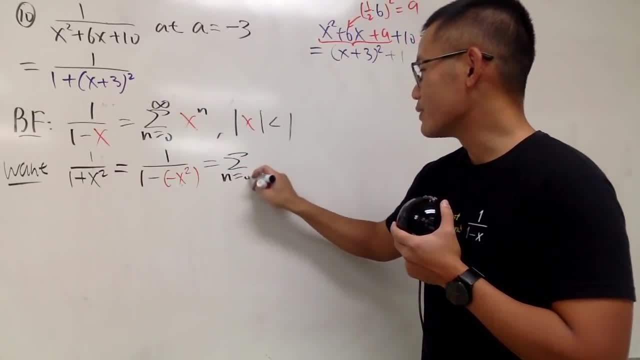 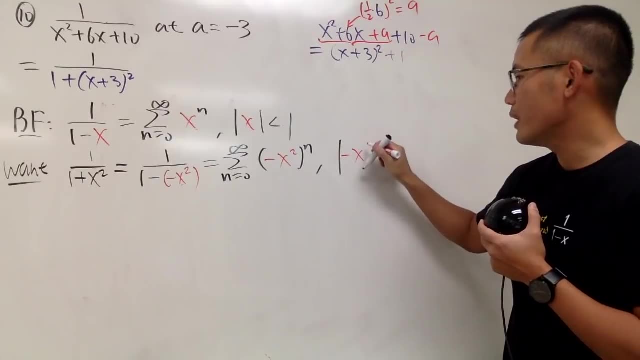 and all that. So this is the sum and goes from 0 to infinity. parentheses that Enter negative x. squared Negative 1 to the nth power. Put this in the absolute value as well. Right, And if you look at this, 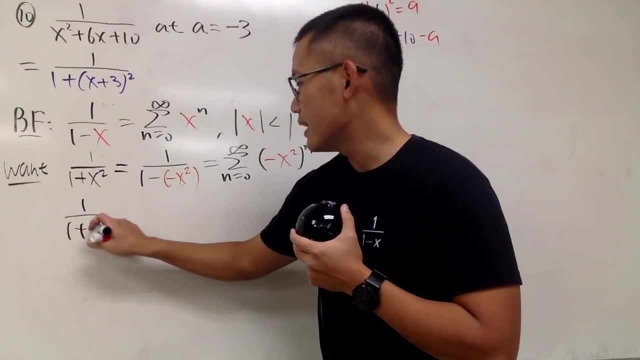 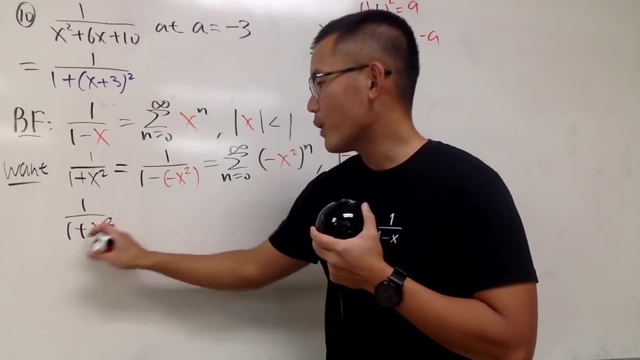 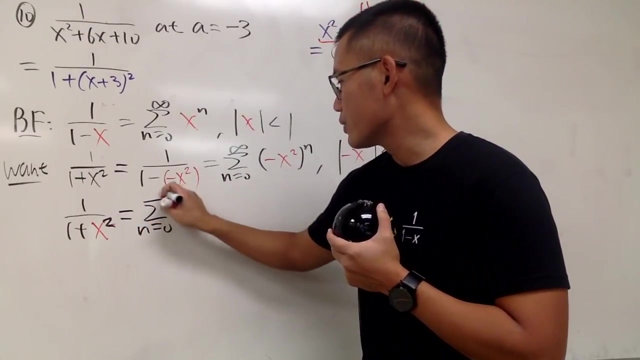 we get 1 over 1 plus x squared, 1 plus 1 x squared, 1 over 1 plus x squared. This right here is nicely equal to this. We have the sum, and it goes from 0 to infinity Negative 1 to the nth power. 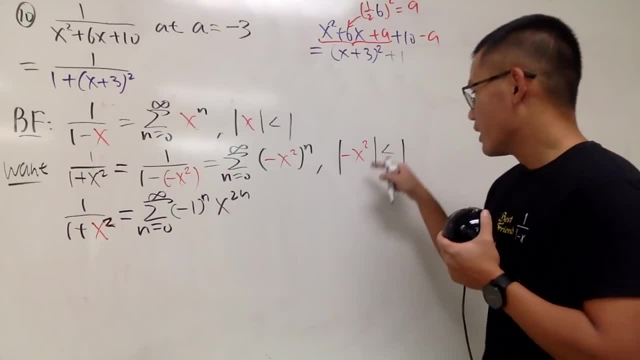 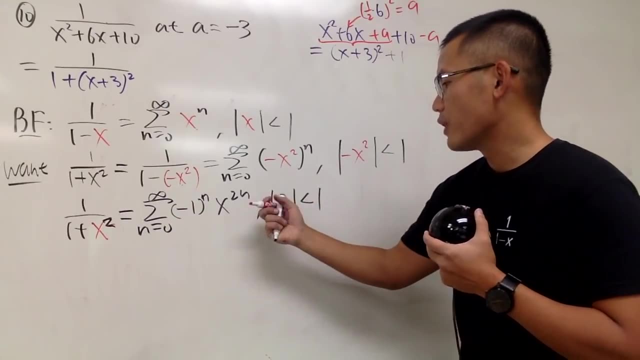 times x to the 2 nth power. Like so Negative doesn't matter. Take the squares on both sides and you end up with absolute value of x is less than 1.. So this is actually the 1 that we are going to use this time. 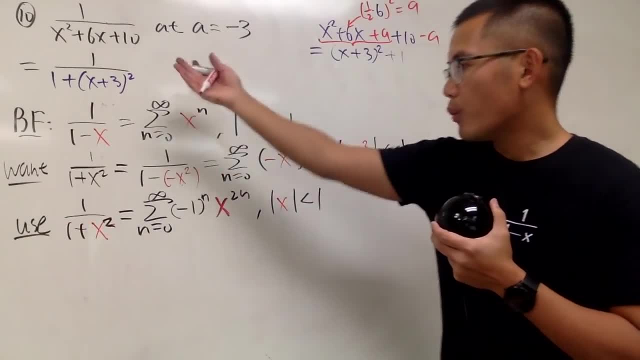 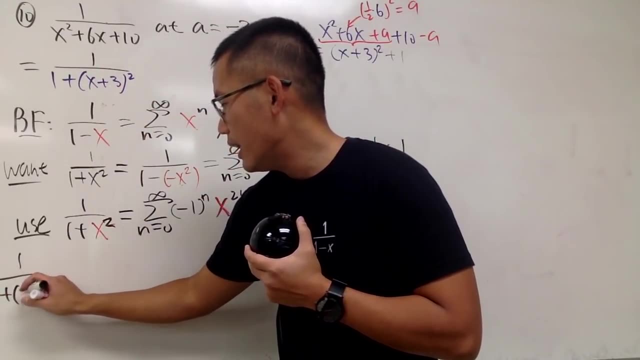 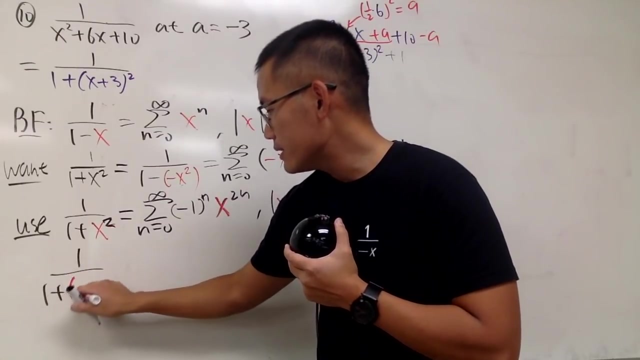 Okay, Because now we have this, We have 1 over and we have this right here, which is 1 plus parentheses x plus. let me just write this down: We have the 1 over, 1 plus parentheses x plus 3 and then square like so: 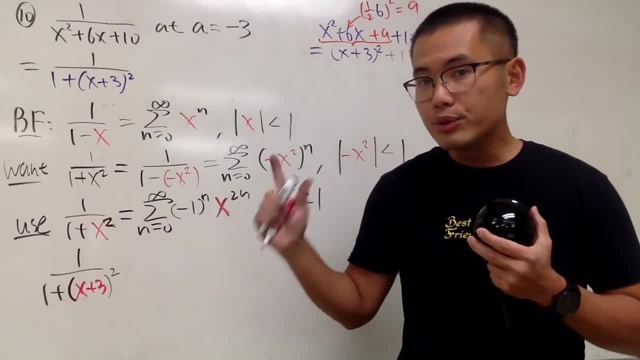 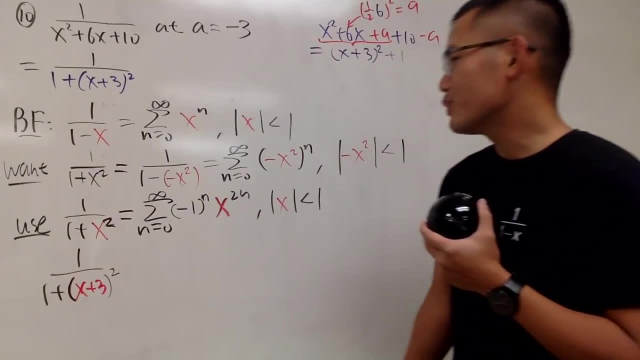 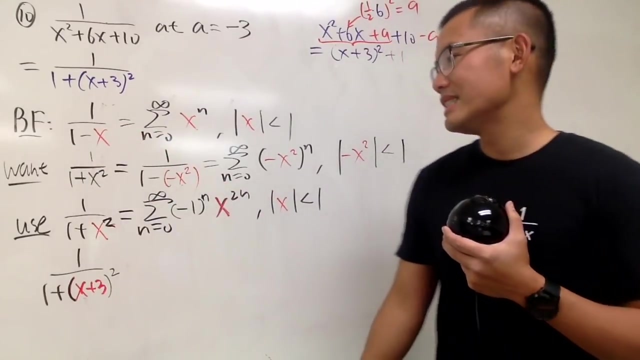 Right, All we have to do is enter x plus 3 in here, in here, in here. Well done, And in fact you could have entered. Oh, you could have used the best friends because of 1 over 1 plus x. Yeah. 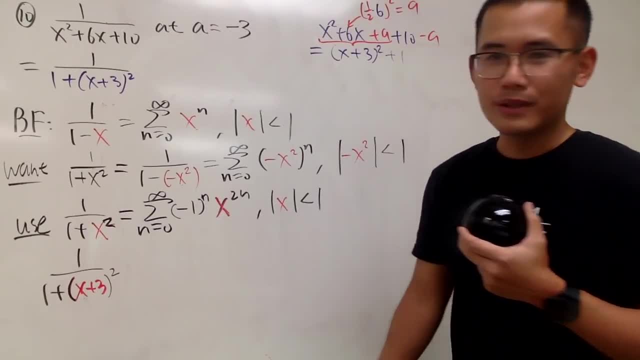 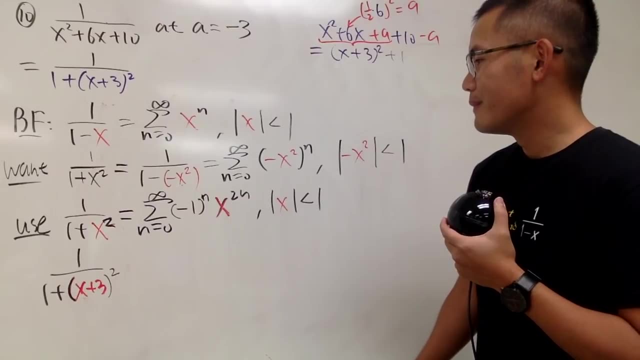 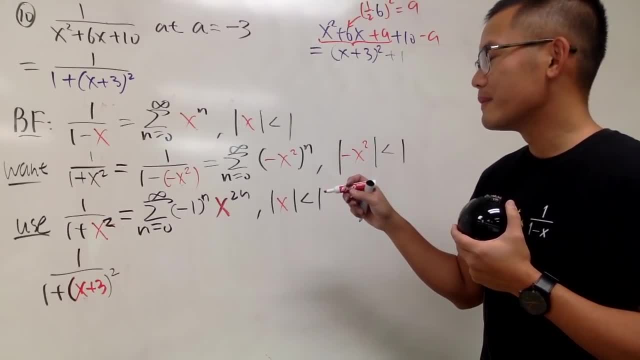 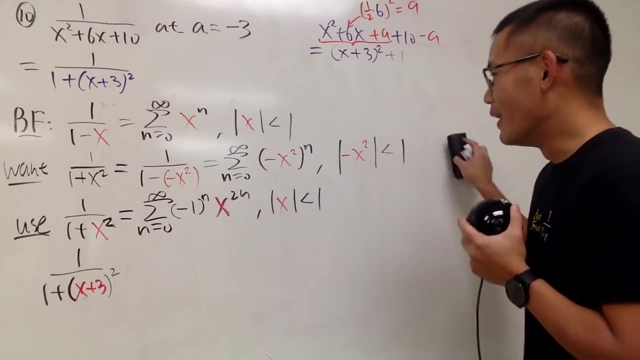 And let's see if I want to do that for you guys or not. I don't know, Let's see. let's see. I don't want to complicate things, so I will show you guys the quickest way to do the power series for all this. 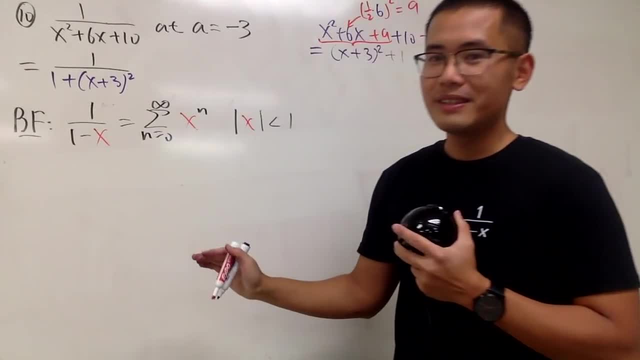 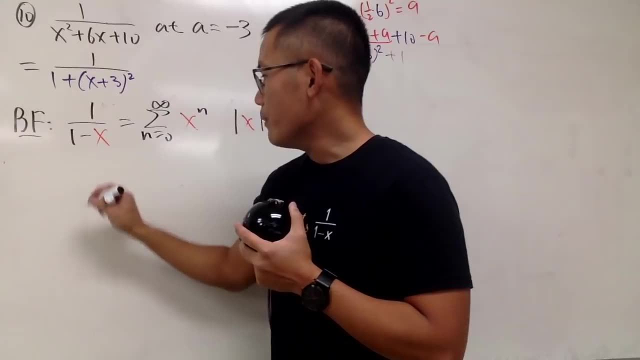 So I will look at this, I will look at this And perhaps let's just make the timestamp right here. Okay, So 121.. So let's see, Well, if you have this, you can just look at 1 over. let's do 1 over 1 plus x. 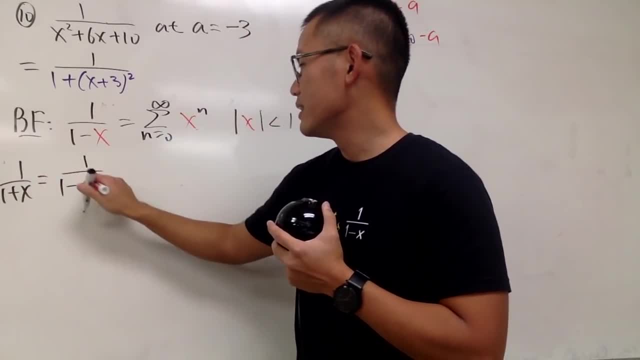 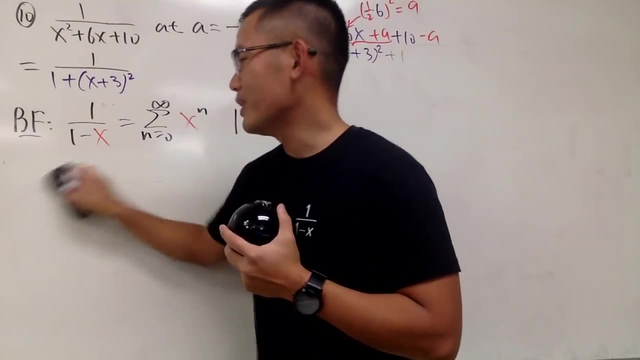 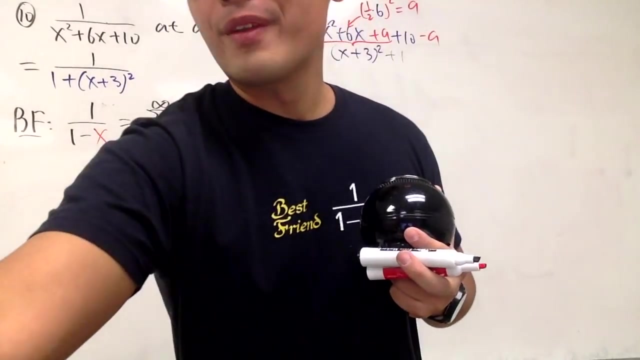 which is 1 over 1 minus negative x. I know it's going to be really similar, but you know this right here is actually No, No, no, no, no, no. What am I doing, seriously? No, I'm just doing one step. 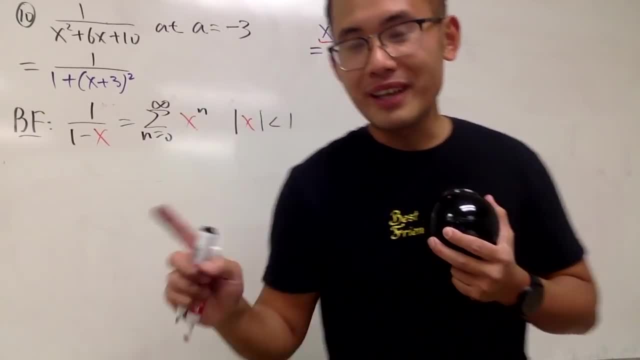 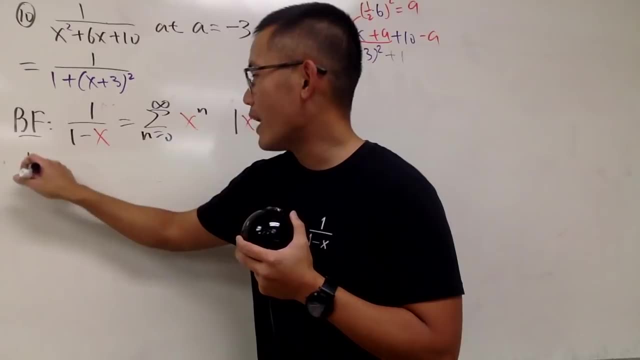 Right, Maybe I'll just make a cut. But yeah, I said one take, But I didn't say I will not make a cut, or not? Anyway, 1.. Now this is what we have. So we have 1 over 1 plus. 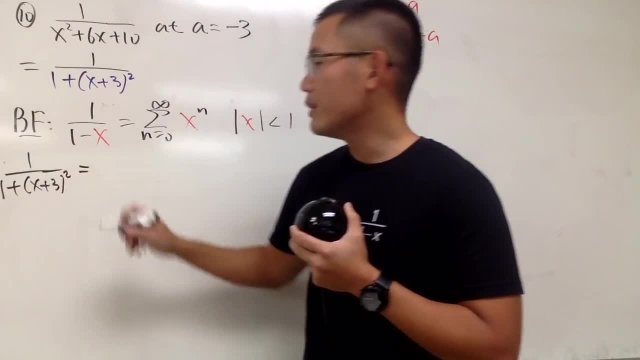 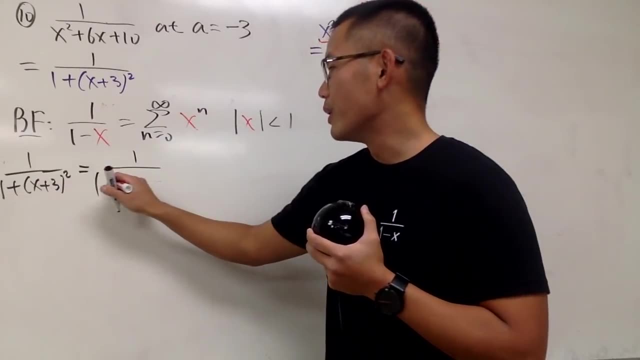 parentheses, x plus 3 squared. And now, in order to use our best friend: Okay, We have the 1 on the top, This is the 1. That's good, But this is a plus, So we do minus, Sorry. 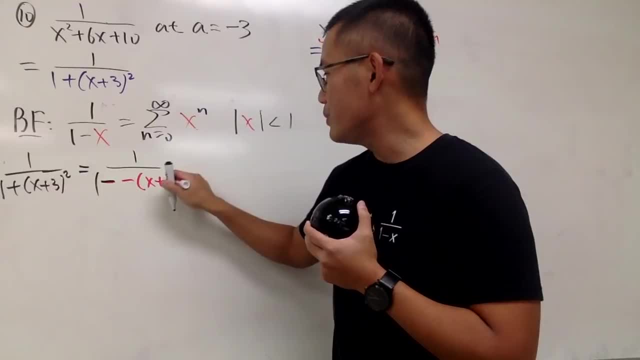 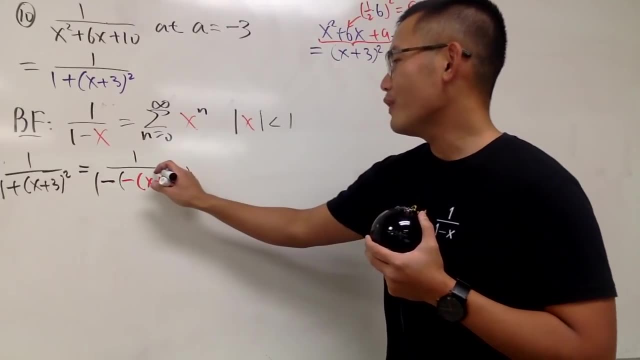 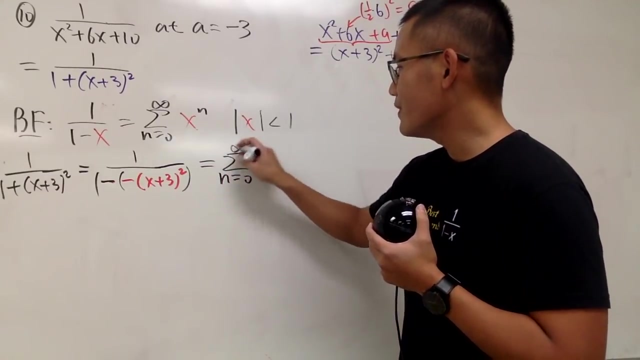 We do minus, Minus parentheses, x plus 3 squared like this Right, So what we can do is, of course, enter this into here. That's it Much easier. So we have the sum and goes from 0 to infinity. Enter this right here. 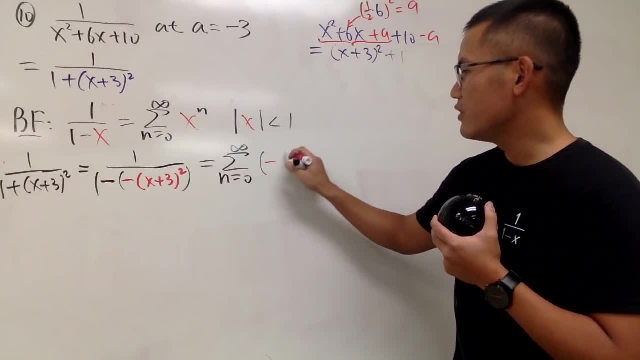 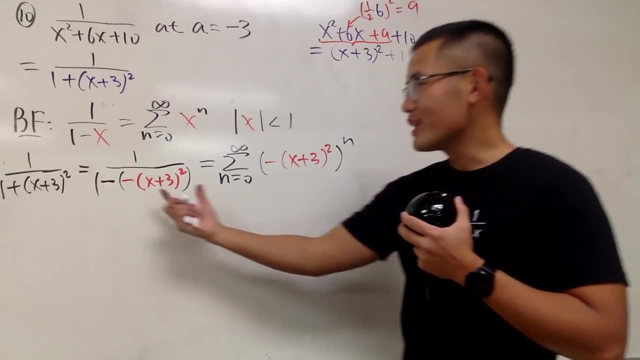 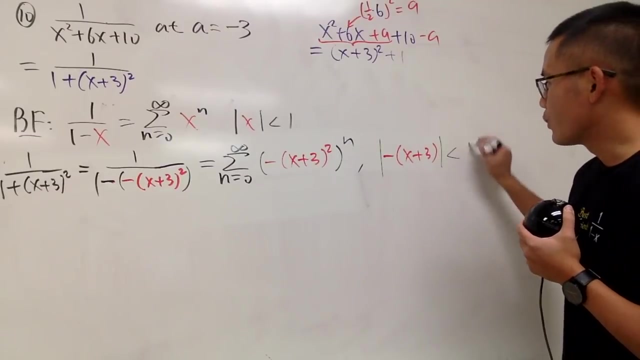 So we have a parentheses with negative parentheses, x plus 3, squared, And to the nth power, And don't forget to enter this into the absolute value as well. So we have the absolute value: negative x plus 3, less than 1.. Yeah, 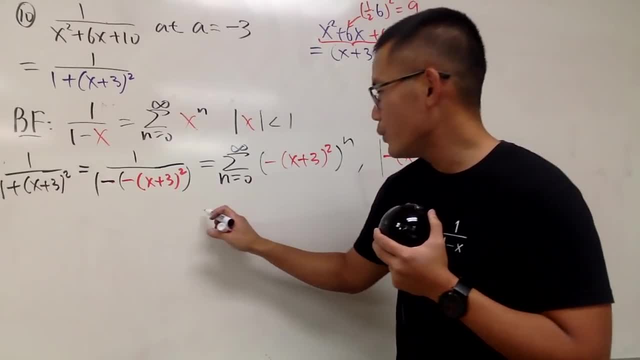 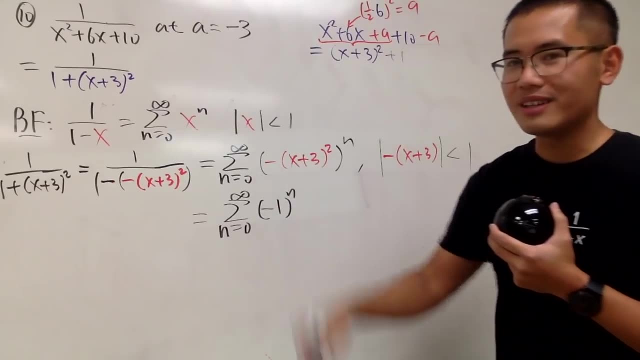 And then work this out. So finally we will get the sum as n goes from 0 to infinity. This is negative 1.. See, this is much faster. I don't know why I did that earlier. Negative 1 to the nth power. 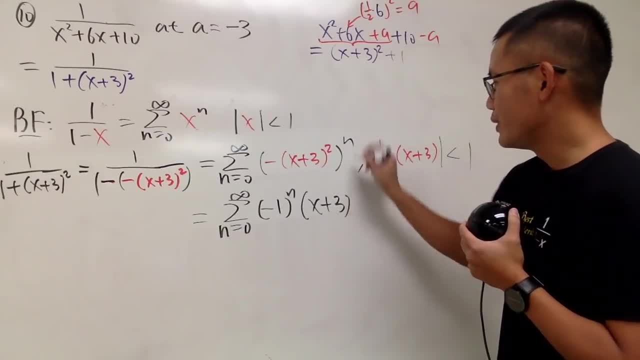 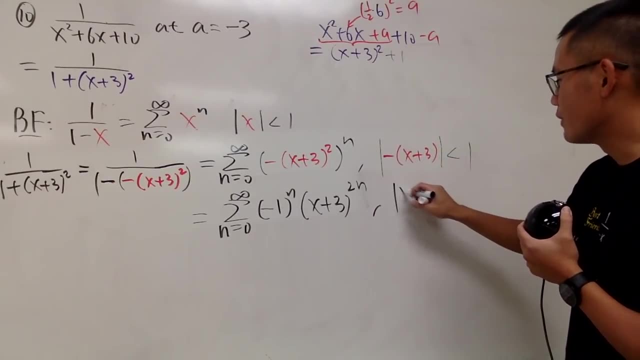 And then this is x plus 3 to the 2 nth power, Like this, And we're done, And of course this is nice. Absolute value of negative doesn't matter. So we have absolute value of x plus 3 is less than 1.. 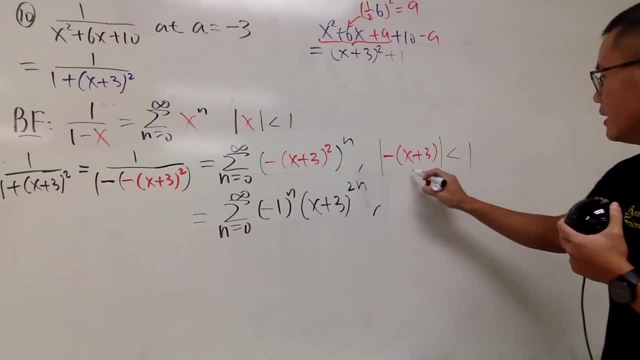 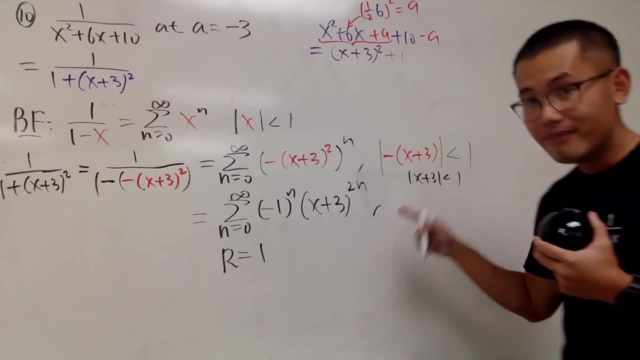 And this is absolute value of x plus 3 is less than 1.. So this will mean r is equal to 1.. r is equal to 1.. And the interval of convergence? Well, don't forget, We start at 3.. 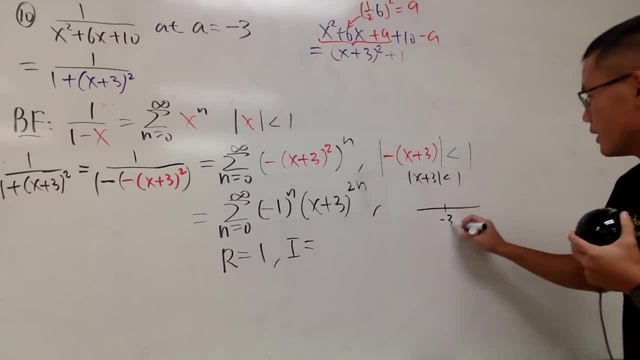 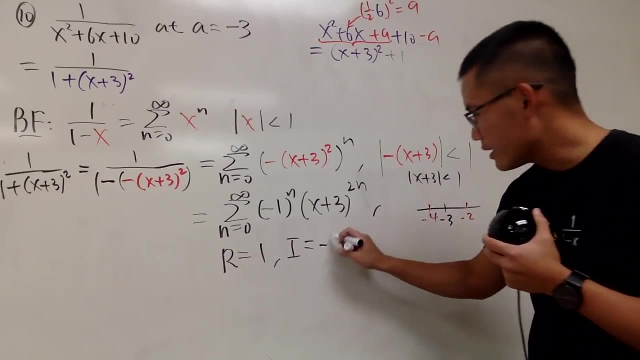 We start at negative 3.. Move to the left one time, which is negative 4, and 1. Right, which is negative 4, and move to the right one time, which is going to be at negative 2.. So we go from negative 4 to negative 2.. 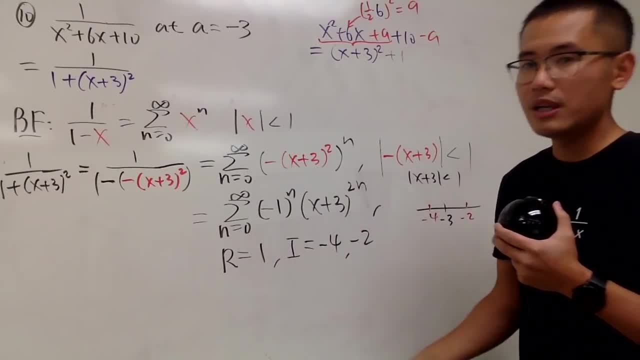 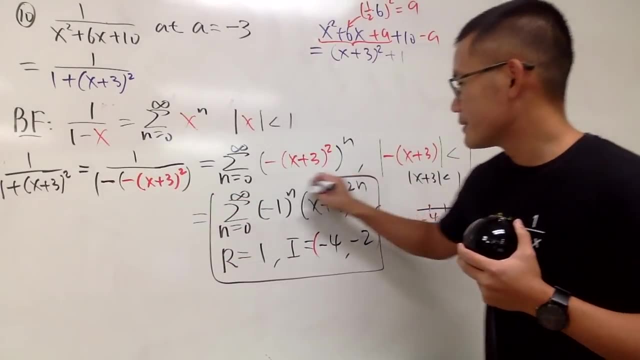 And we do not include the endpoints because, again, we're just the algebra. It's the best friends and its cousins and all that stuff, All right. so this right here, is it Okay? so let me just double check. Yeah, just like that. 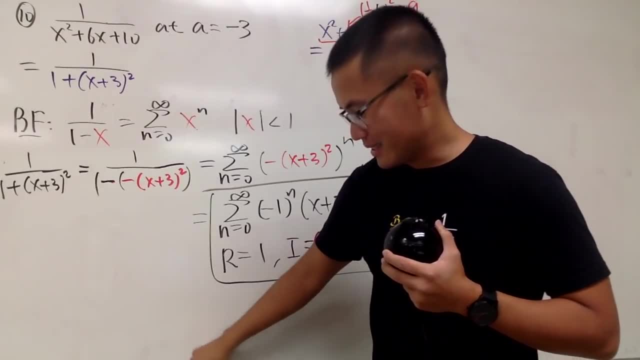 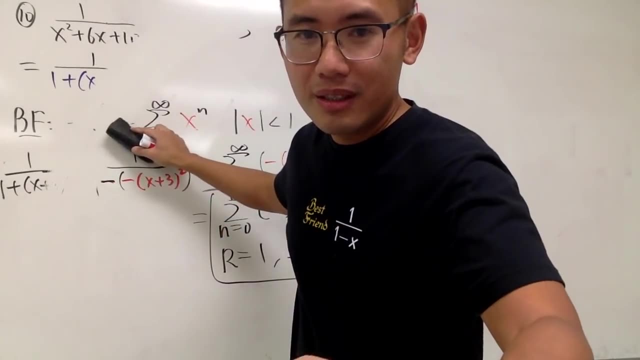 It's actually pretty fast. I don't know. I just come with the cousin earlier, but you don't have to, You can just do this right here. Okay, so that was 10 questions and it took me 84 minutes to explain all this. 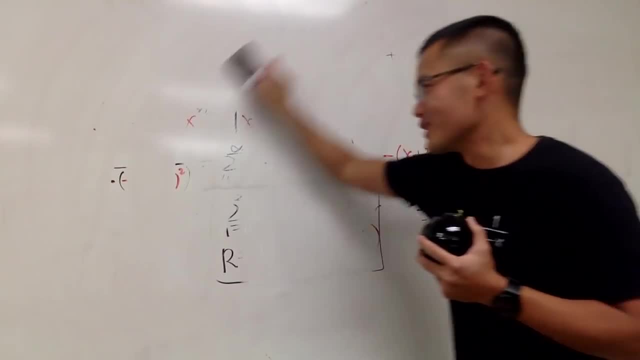 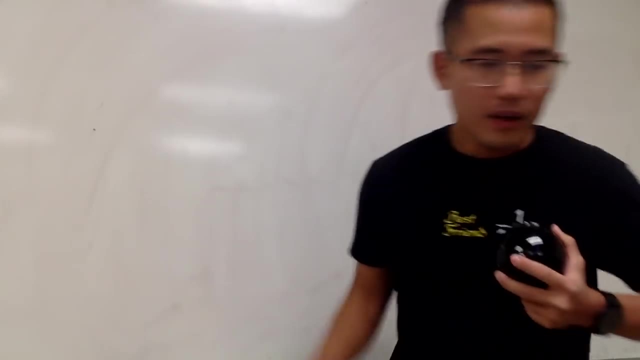 Hopefully you guys are finding this helpful. okay, And if you guys do, please just let me know. That way I will know what kind of materials I should make for you guys. Okay, Man, number 11.. Here we go, number 11.. 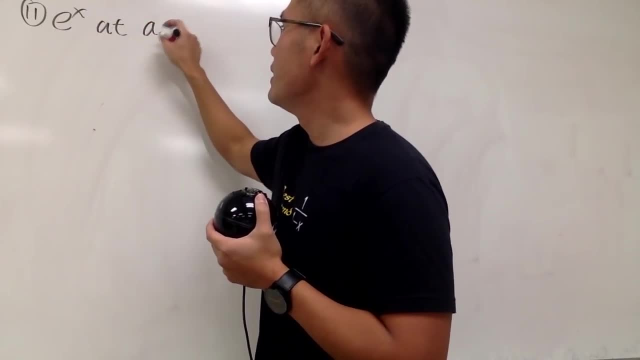 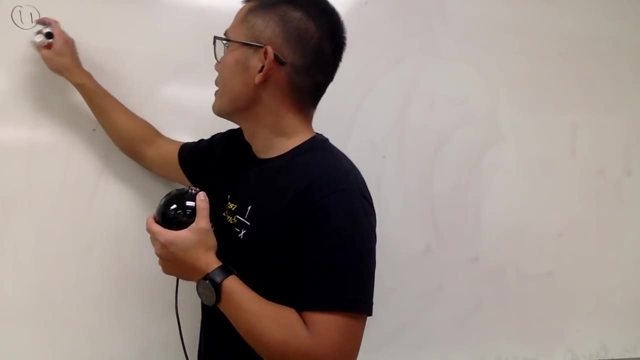 e to the x center d at a equals 0.. All right, e to the x center d at 0.. That looks like a face. Let me just write it down again. Number 11 still looks like a face, but whatever. 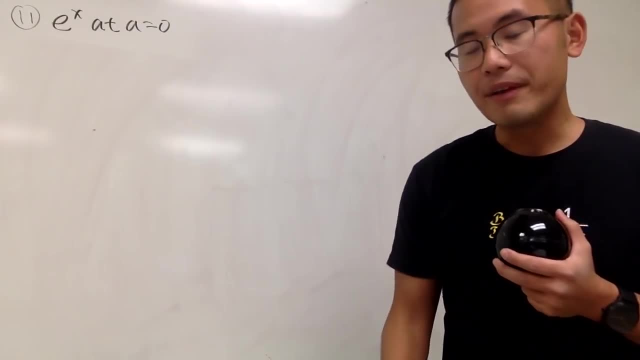 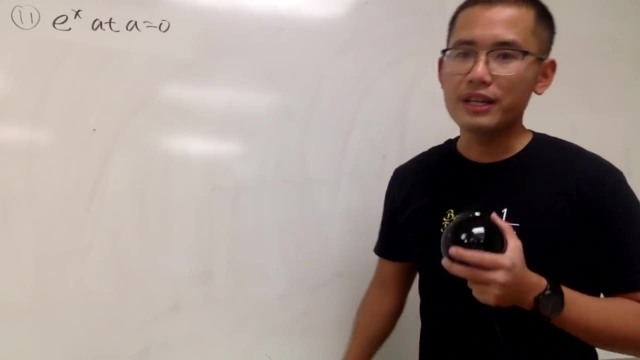 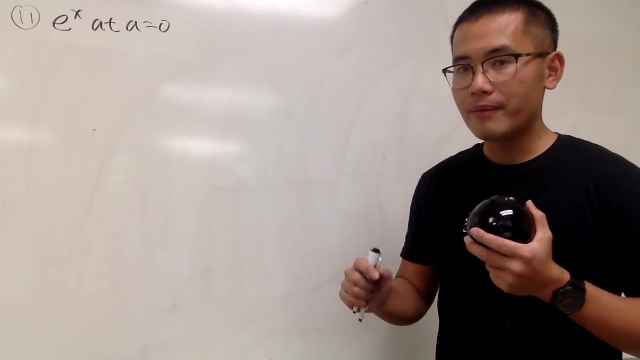 All right, okay, so this time, unfortunately, we cannot use our best friend anymore. We cannot integrate this, We cannot differentiate this to get e to the x, nor doing any algebra. so no, But it's okay because we can use the Taylor formula. all right, the father of the power series. I will say: 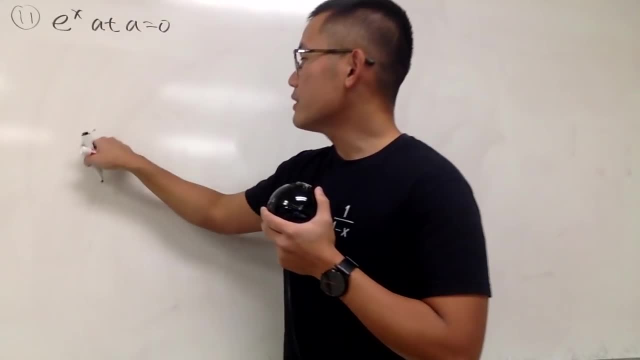 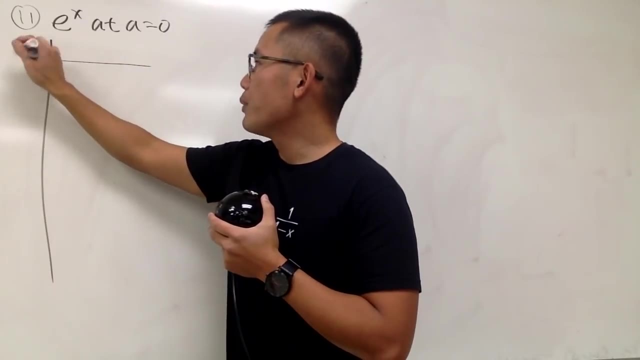 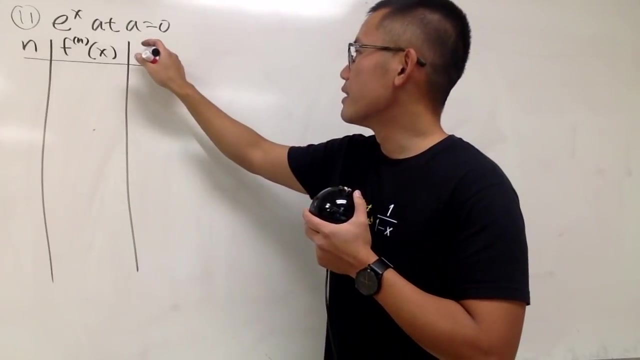 Okay, and this is what you do. First of all, I will just write down this for you guys. We'll make a table, Set this up. We have to have n and then the nth derivative of the function right, And then the third part, right. here you write down the Taylor formula, which is the thing you have to remember. 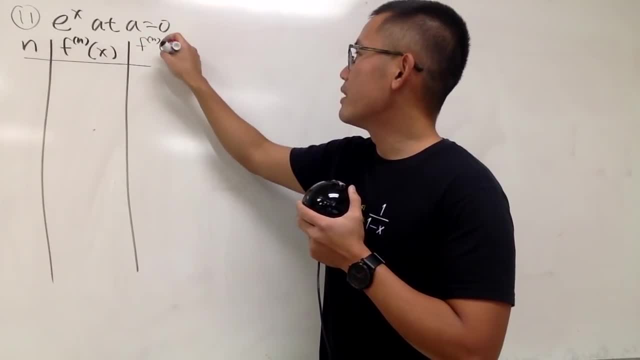 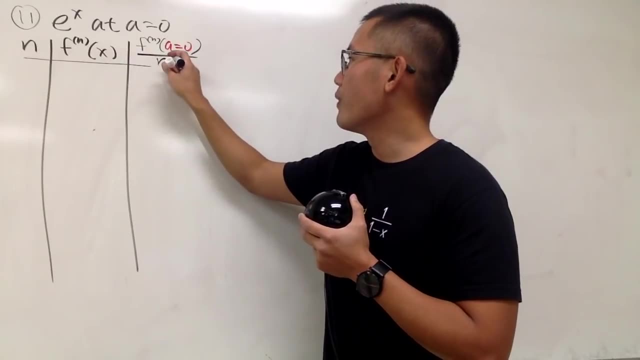 This is f, the nth derivative of f, And you enter: in this case, a is equal to 0,. okay, And then divide it. Divide n factorial, Okay. Now let's go ahead and do a few of this. 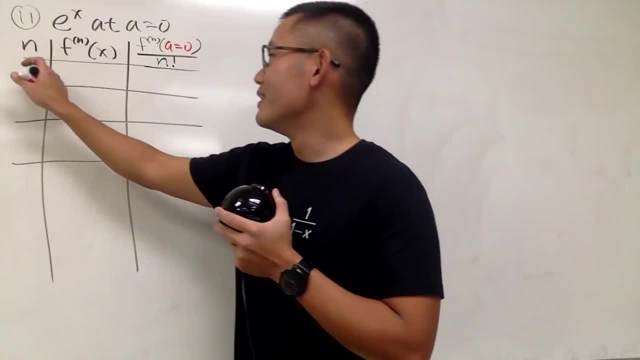 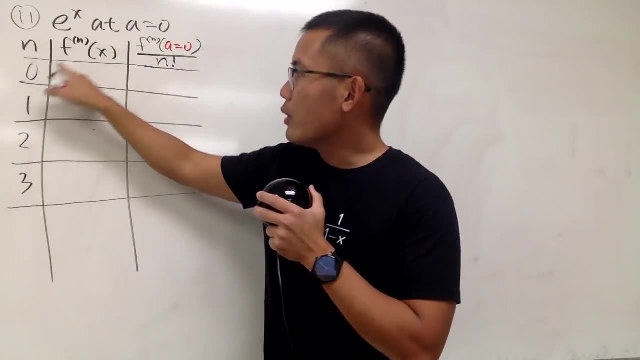 Is your 2 enough? As long as you can see a pattern, that's good enough: 0,, 1,, 2,, 3.. And in fact you will see, this is actually enough. First thing first, When n is 0, you don't do any derivative. 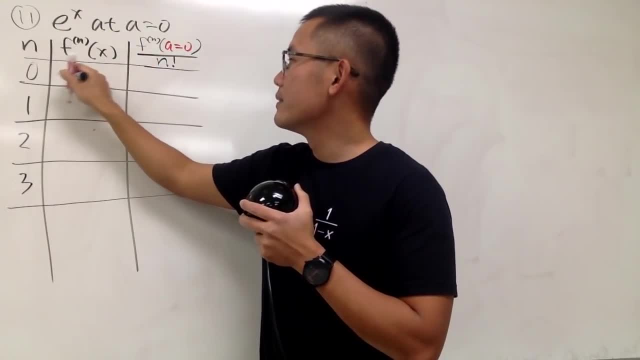 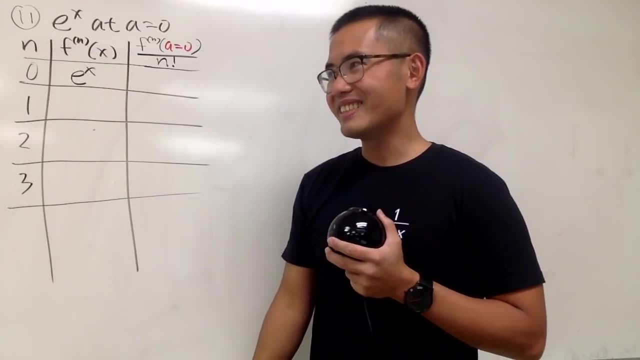 It's just the original function. So you write down e to the x And this is just the original function. And now here we go, Differentiating e to the x. Yes, we still get e to the x, That's perfect. 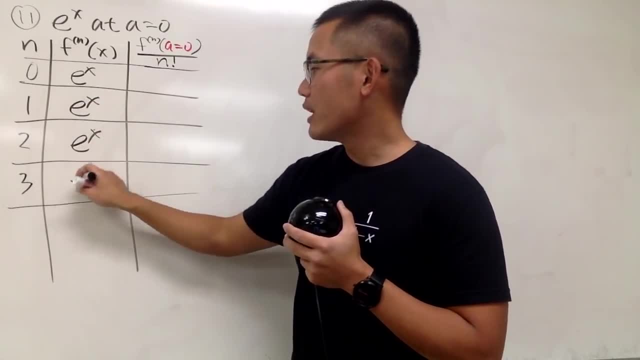 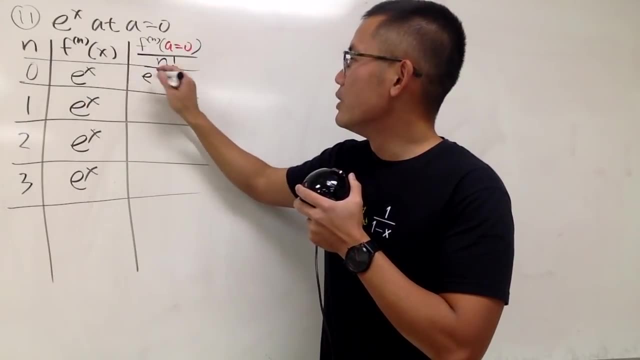 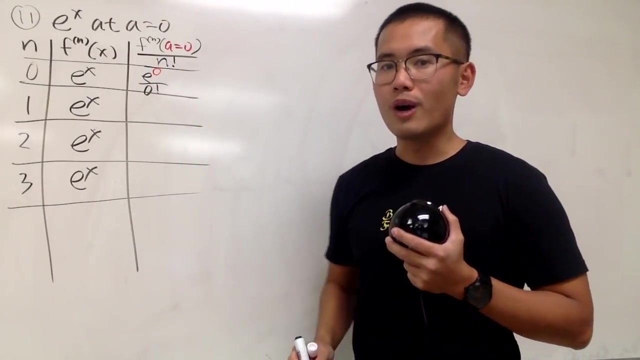 And then you take e to the x And you still get e to the x, And so on. Now I'm going to enter 0 into here. So we have e to the 0's power over 0 factorial. And remember, 0 factorial, by definition, is equal to 1.. 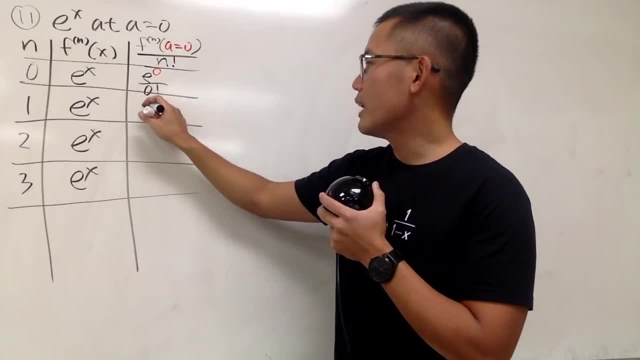 So this right here is what we have, And of course, let's just do the rest. We have e to the 0's over 1 factorial, And then again we have e to the 0's power over 0 factorial. 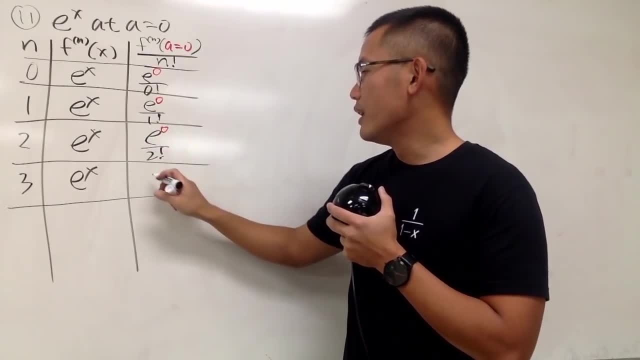 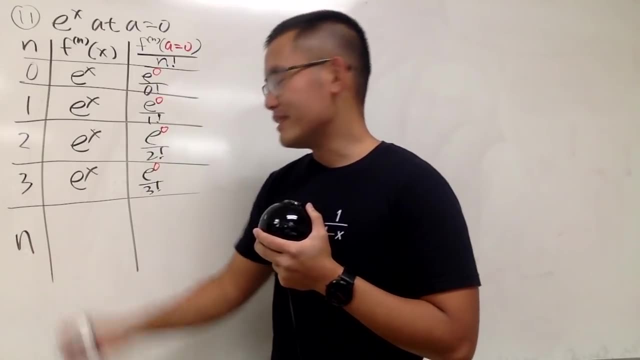 And then again e to the 0's power over 2 factorial, And then e to the 0's power over 3 factorial, And if this is just any n that you want, of course you always get e to the x. 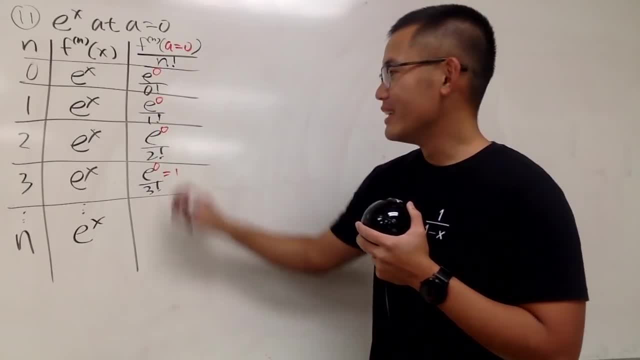 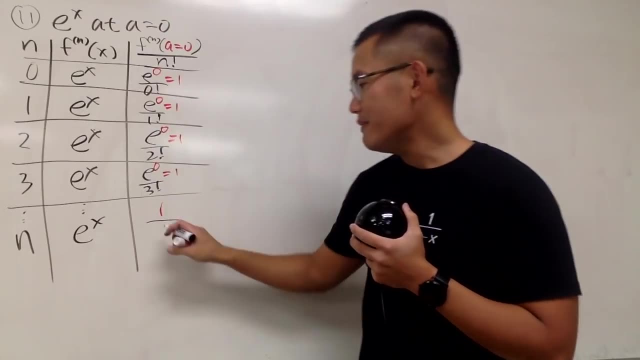 And notice that e to the x is just equal to 1.. That's very nice. So on the top it's always equal to 1.. We can just put that down. If this is n, just divide it by n. factorial. 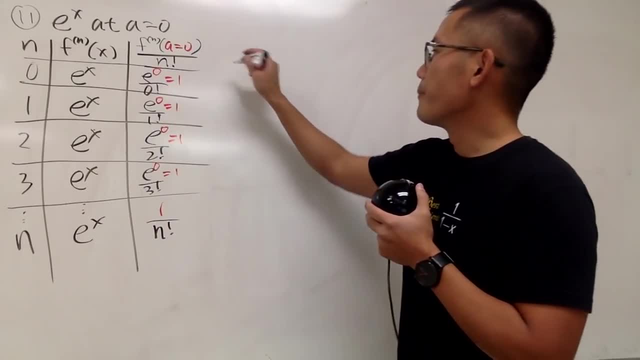 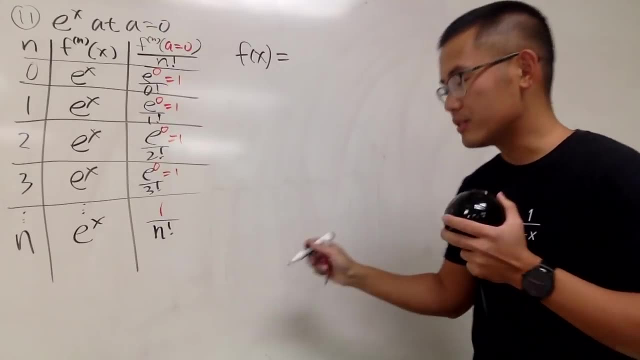 That's all we have. Okay, that's it. So here we go. Let me just write this down again, at least for the record. Any function that you want, as long as you can differentiate that, that means it's good enough. 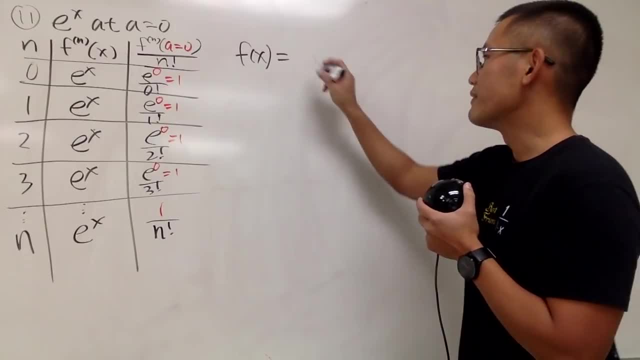 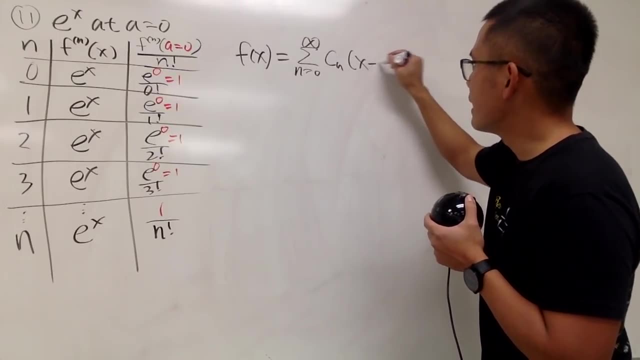 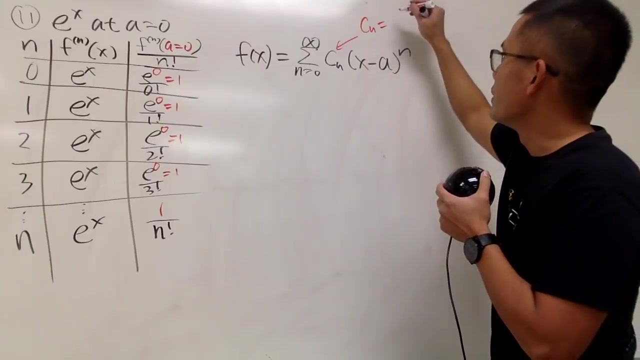 You can have the power series expansion thanks to Taylor. You have the following formula: It's the series as n goes from 0 to infinity, cn times x minus a to the n's power, And Taylor says the cn here is exactly the one that we did. 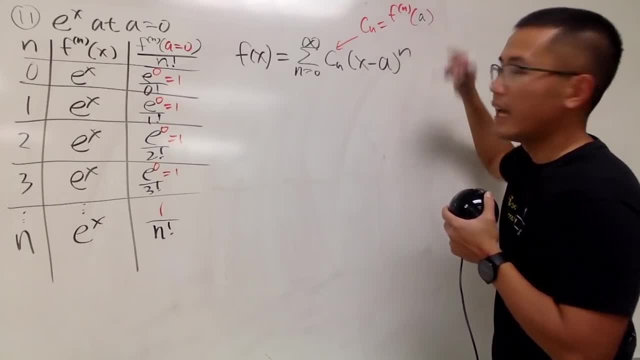 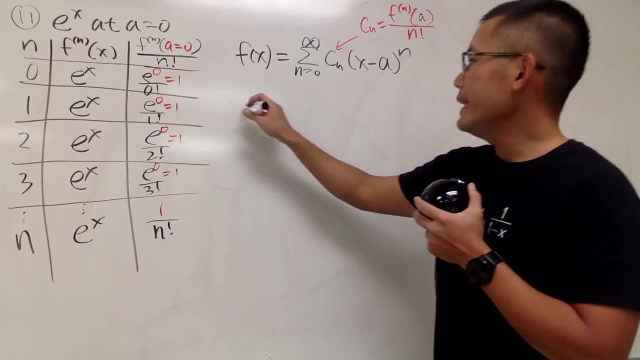 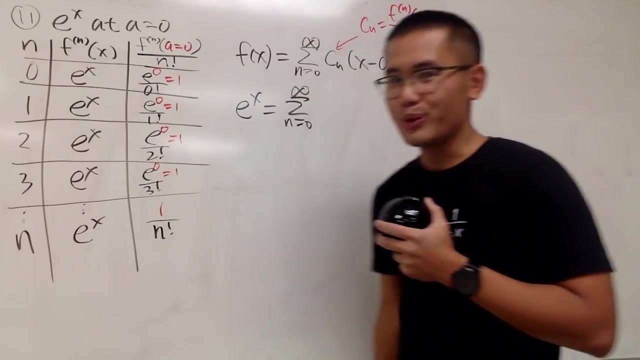 The n's derivative of f, evaluated at the center a And then divided by n factorial. Okay, So I will tell you: e to the x is actually equal to the series. as n goes from 0 to infinity, The coefficient is nicely equal to 1 over n factorial. 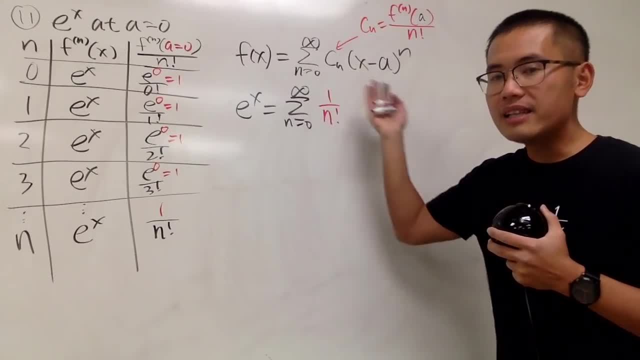 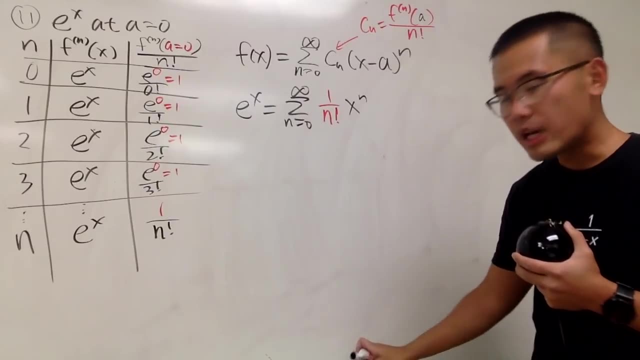 So I'll just put that down. And in the case right here, a is equal to 0. So we just get x to the n's power, like so, And that's pretty much it. And now you might be wondering: how do we find the radius of convergence? 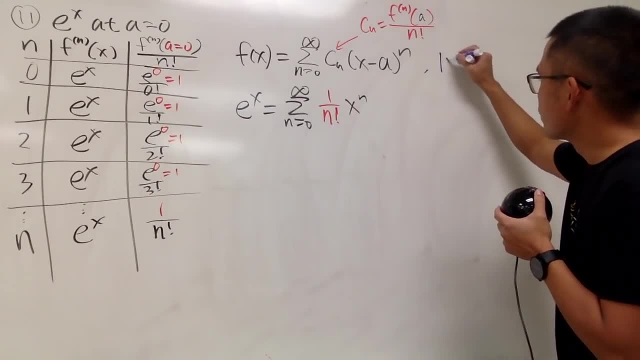 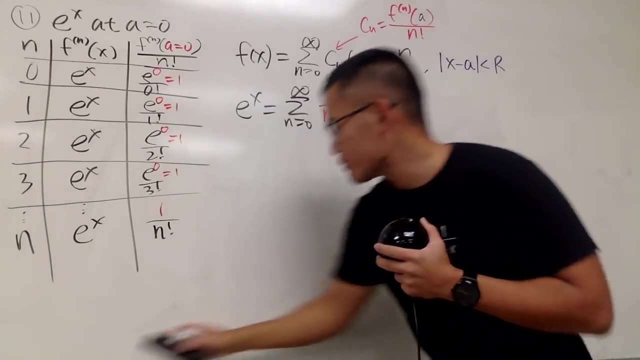 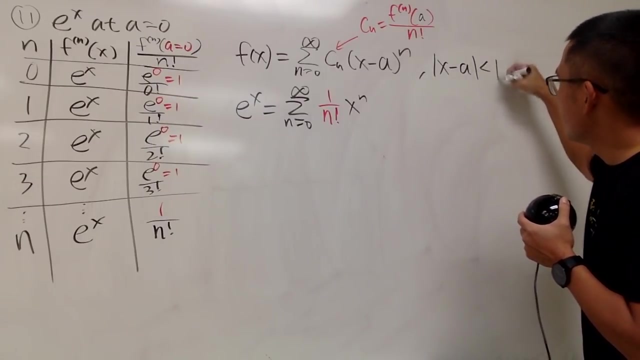 Good question. Well, we still want to have the absolute value of x minus a to be less than r. And let me tell you, Let me tell you- Actually, let me change the color a little bit- We still want the absolute value of x minus a to be less than r. 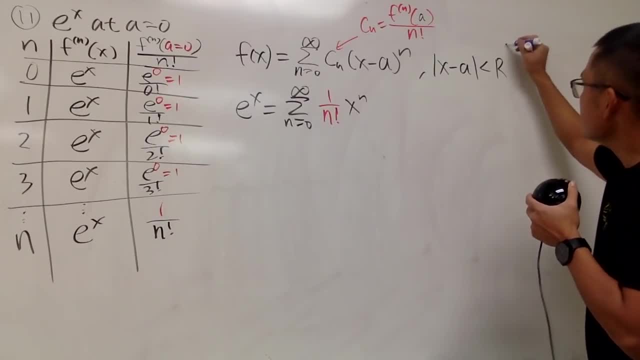 And let me tell you, this is a nice formula for the r, This r. What you do is go ahead and take the limit as n goes to infinity, And then you do this, And then you do this, And then apply the absolute value. 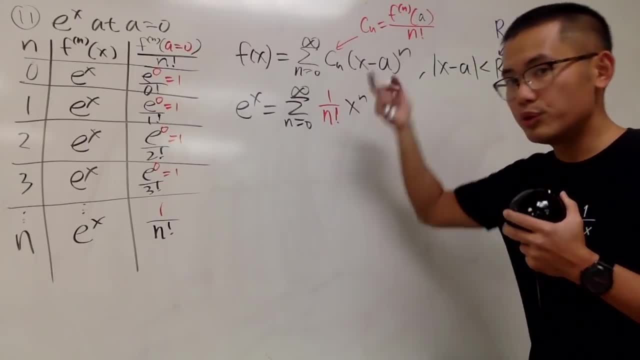 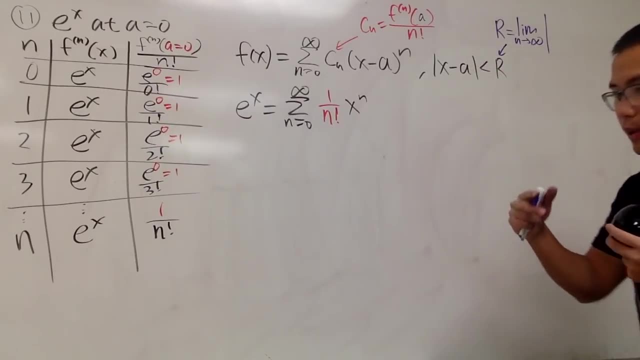 Okay, Look at the coefficient sequence, which is the cn, And this is pretty much derived from the ratio test. But you don't do the original ratio test. if you want to use the formula right here For the r, what you do is you do cn divided by cn plus 1 in that. 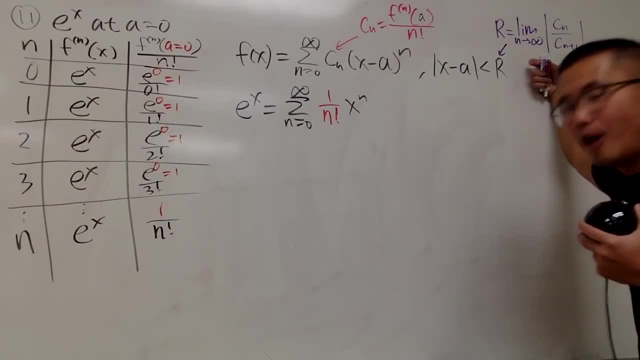 Just compute that If the limit exists, you get the r for free. Well, I actually do the work, so it's not for free. Anyway, that's it. That's all you have. So this is what we have. 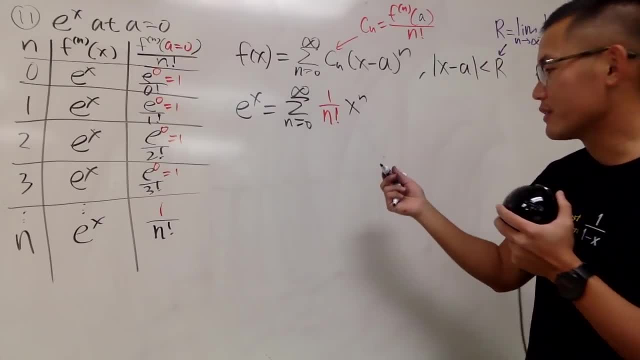 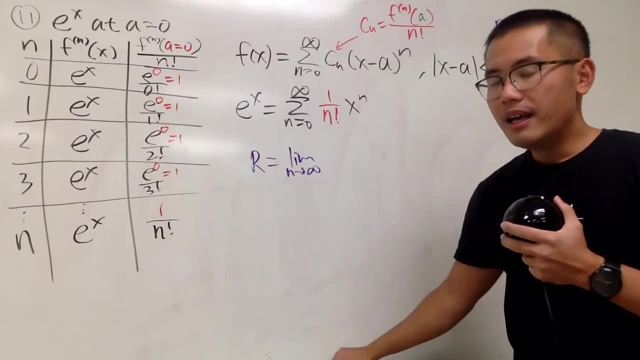 Then we are going to go ahead and do our radius of convergence. So here we go. r is equal to take the limit as n goes to infinity. And sometimes you can also say as n goes to infinity. Up to you. 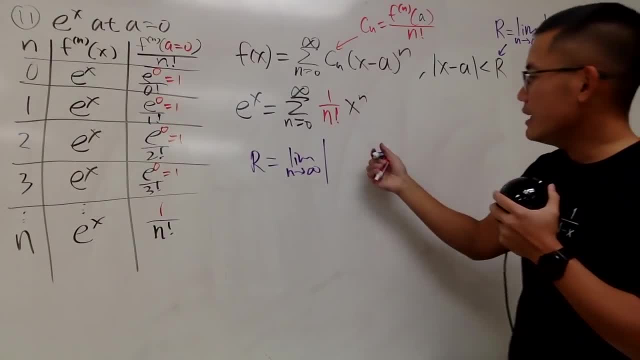 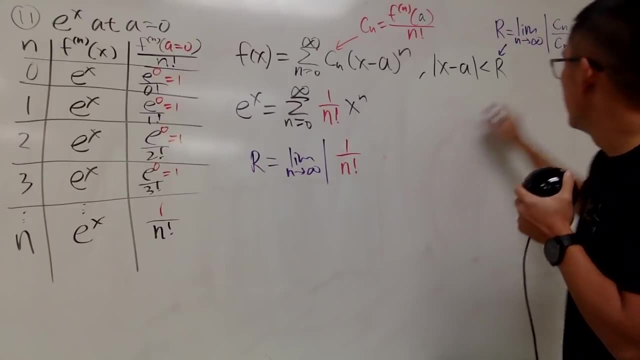 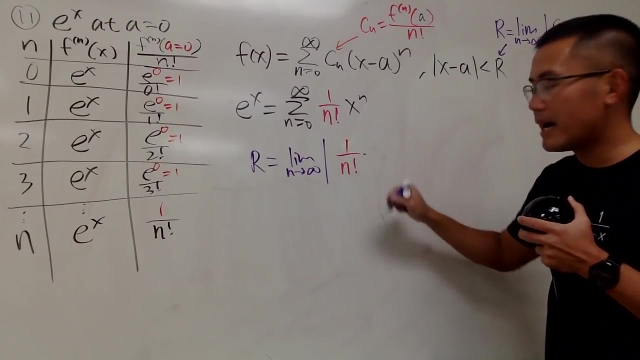 Anyway, here we go. Cn, which is this: First I will have 1 over n factorial, 1 over n factorial, That's this part. And then, notice, we have the 1 over cn plus 1.. So we can just multiply this by the reciprocal. 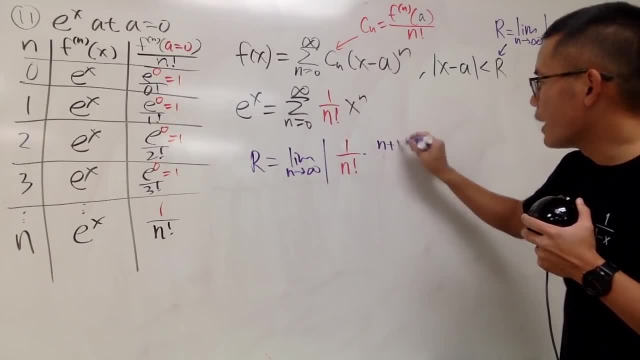 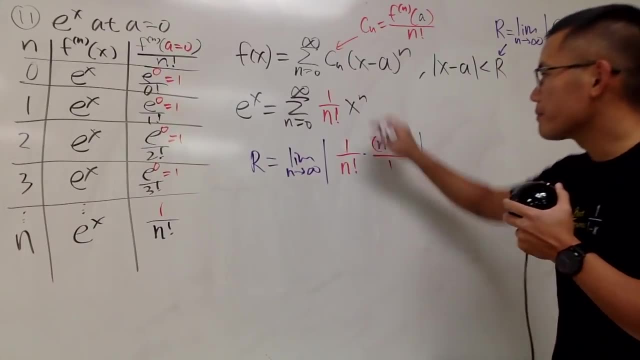 And n plus 1 means we have the n plus 1 as the input, And then factorial that, And then divide it by 1.. Like this Again, this is the cn, And then when you have the cn plus 1 on the bottom, 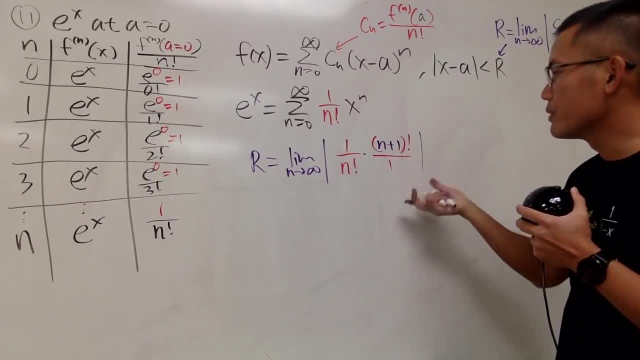 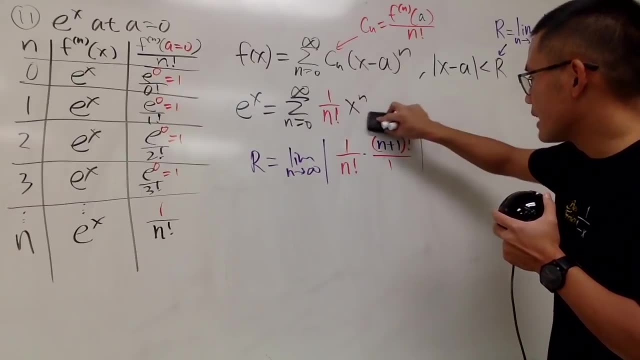 you can just flip that And you have the n plus 1 right here, factorial. So that's what you have. Simplify: the big factorial, Bigger factorial, which is n plus 1.. Let me just write it as n plus 1 times. 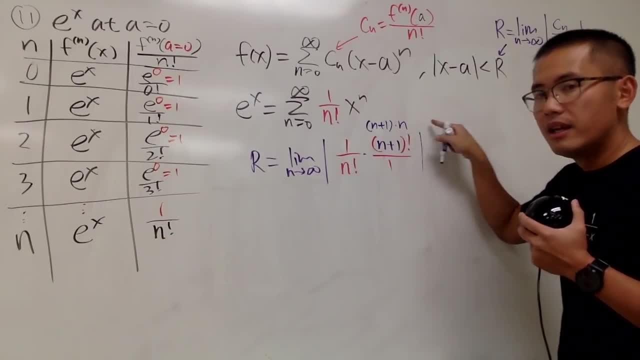 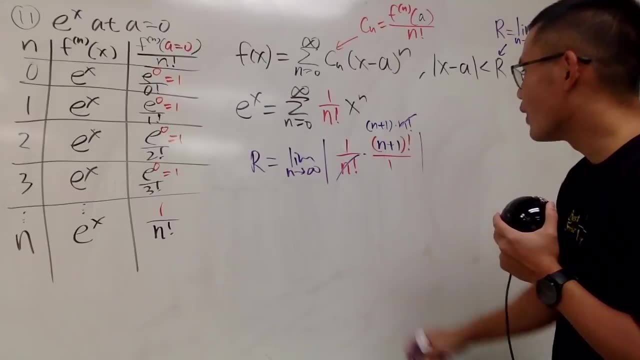 The next is going to be n, And the next one is going to be n minus 1.. And then n minus 2, and so on. So you can just include all that and say: that's n factorial. Very nice, because this and that will cancel. 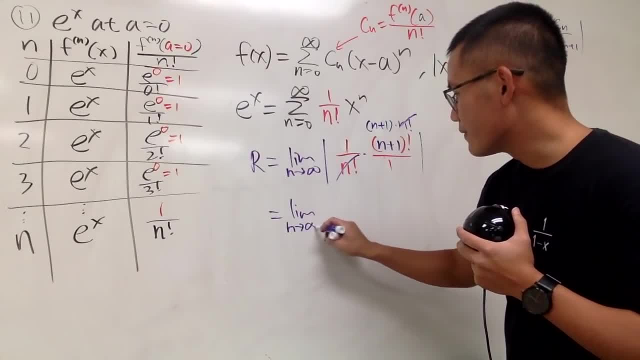 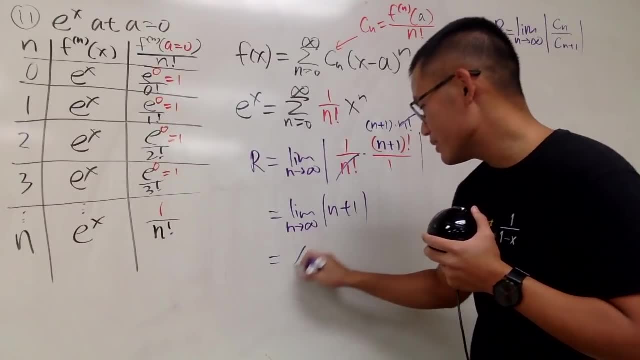 And you are looking at the limit, as n goes to infinity And this is just n plus 1.. When you take n goes to infinity, this is, of course, equals infinity. Congrats, this is the first one that we have today. r is equal to infinity. 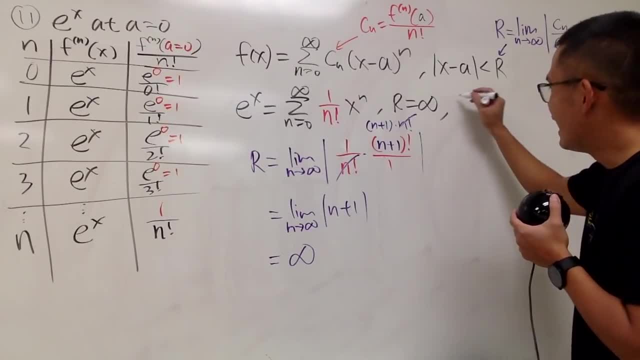 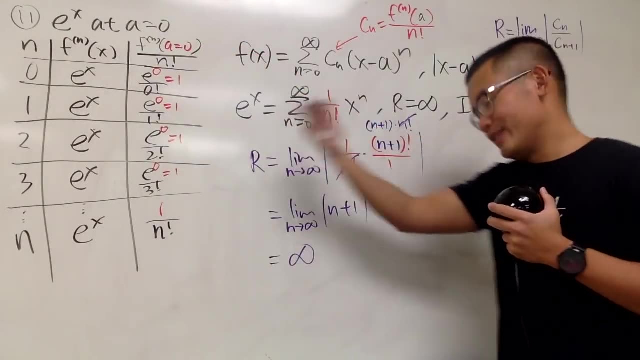 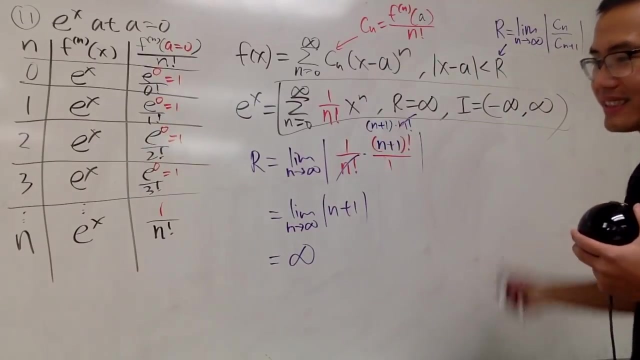 Why do I say congrats? Because if r is equal to infinity, i is automatically negative. infinity to positive infinity Doesn't even matter where the center is. All the way, all the way. So, ladies and gentlemen, this is e to the x as a power series. 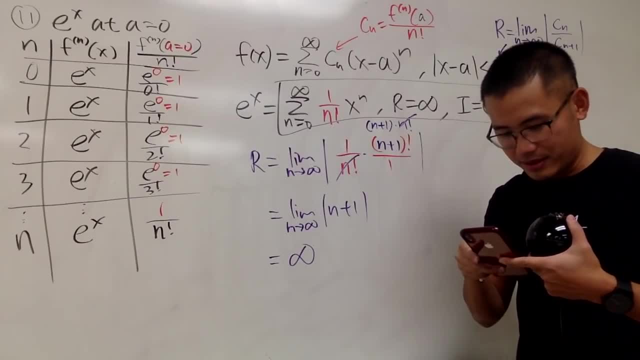 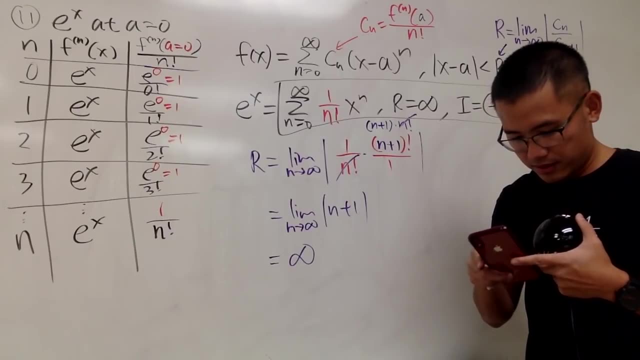 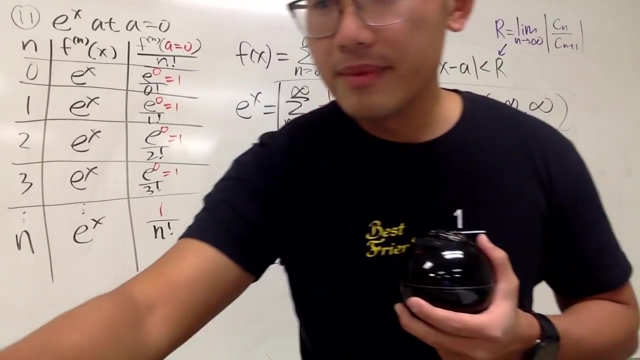 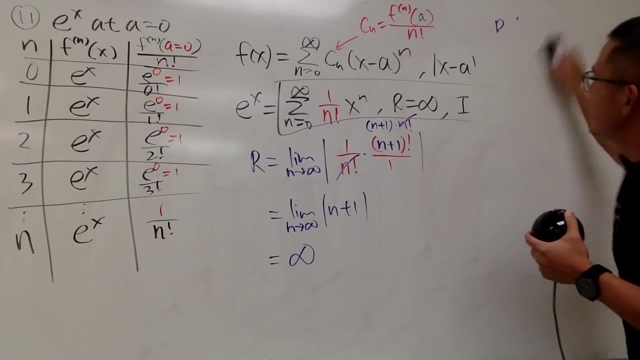 Let me just check any messages. I saw someone. I saw some messages of you. Yeah, All right, So this is e to the x And we'll be using this Same thing for the other ones, And, of course, you should know the e to the x by heart, right? 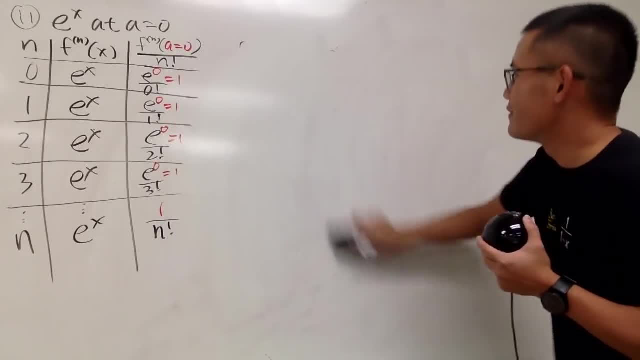 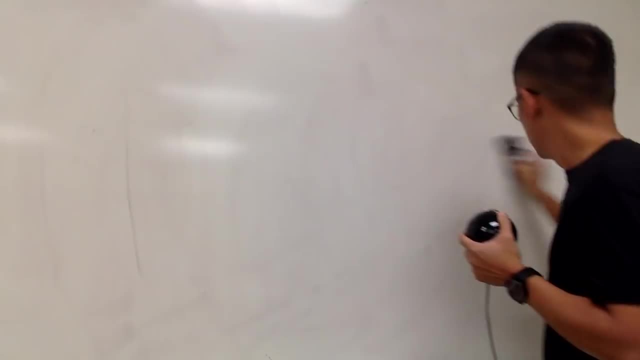 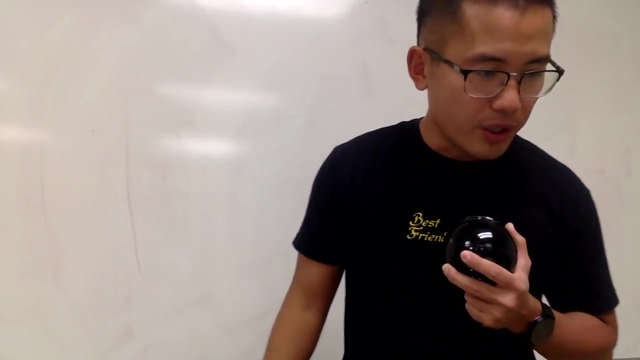 This is another friend that you have to know. It's a standard function that you definitely have to know. Now for the next one. we have sine x. So here we go, Number 12.. Number 12.. Sine x. 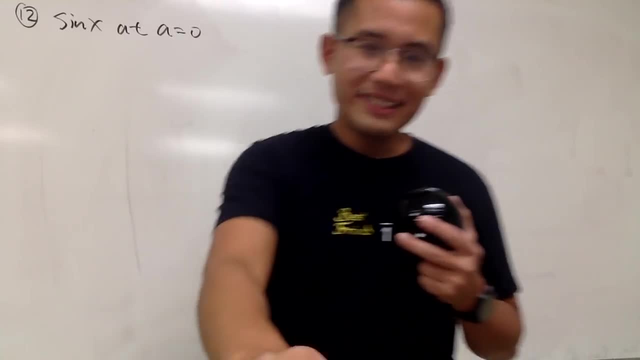 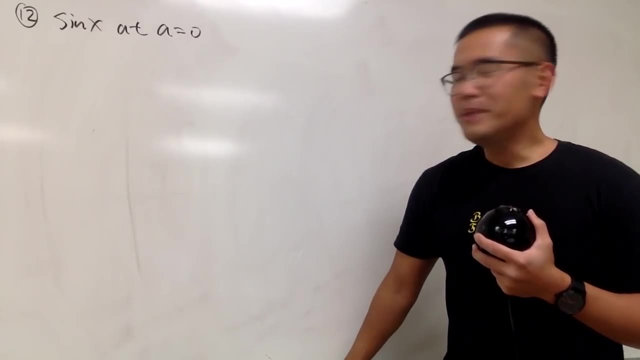 At a equal to 0.. Man, this power series, business 12 questions took me an hour and 30 minutes. So you multiply that by 10. That would be equivalent to do like 100 differential equations. man, Seriously. 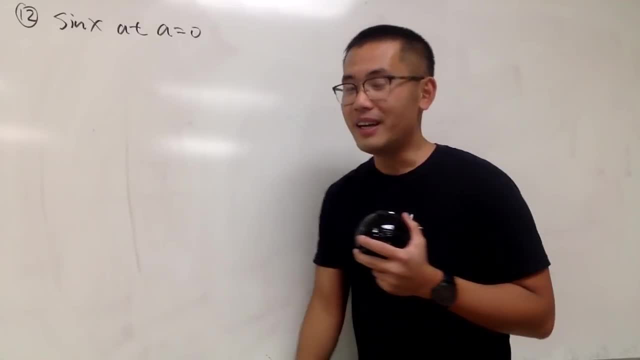 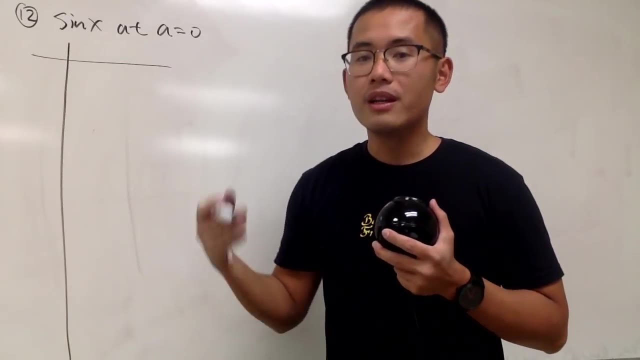 So I don't know if I should ever do that. 100 differential equations. Anyway, I will, And then do the work. All right, So again for sine x, we will be using the Taylor-Fulmer to help us out. 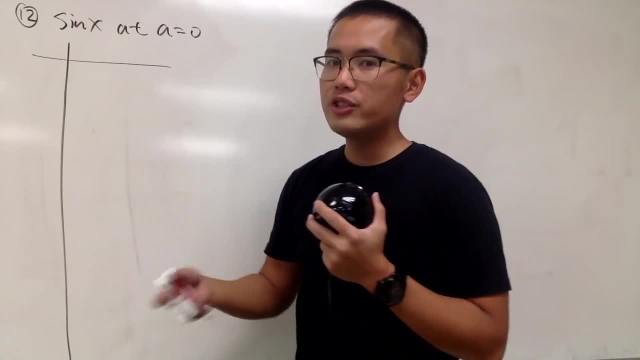 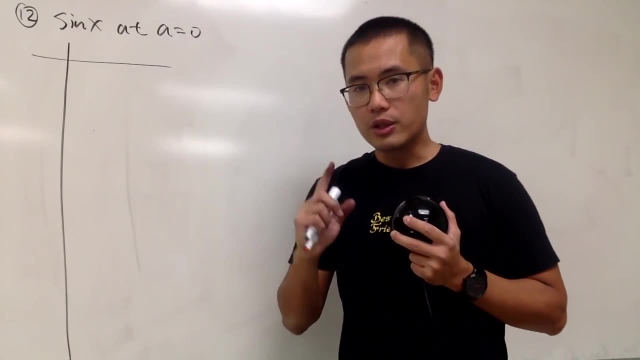 But you know, if you differentiate the sine, you get like cosine and all that, and especially when a is equal to 0, you get some 0s. So instead of using n, I will be using k, And you guys will see why later. okay, 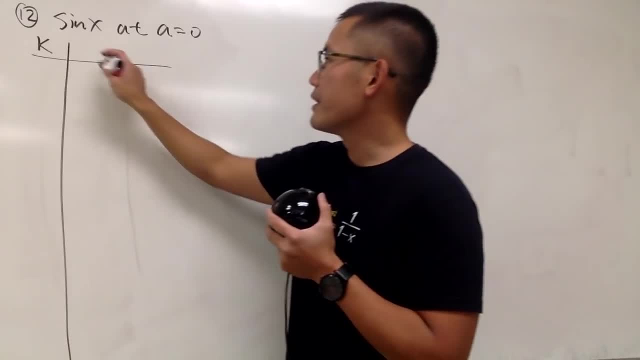 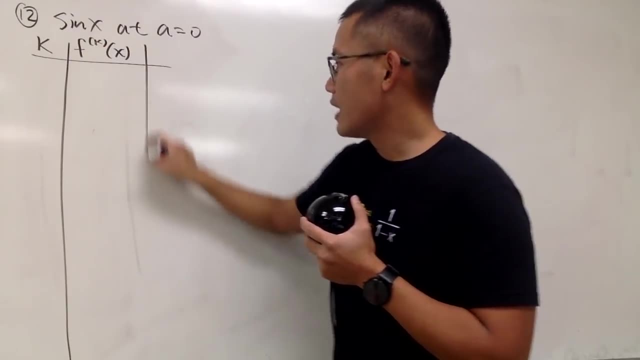 So let me just use k, And right here I will be writing down the k-th derivative of the function. Just differentiate that however many times that we need to, And then here we have the k, And then enter: a is equal to 0.. 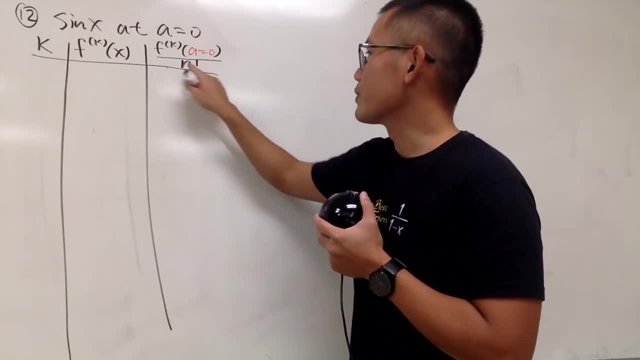 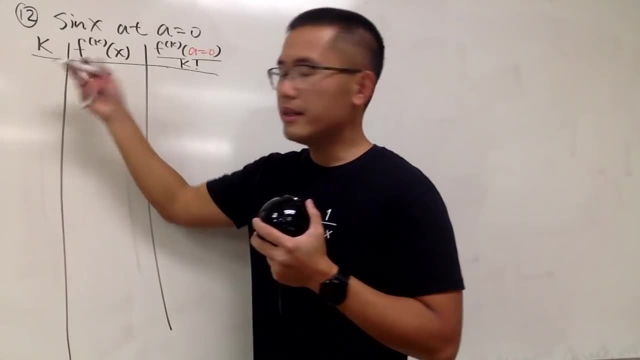 And then divide it by m- factorial, Sorry, divide it by k- factorial, All right. And again, like k and n, they are the index. They are just like dummy variables, So it doesn't matter that much, All right. 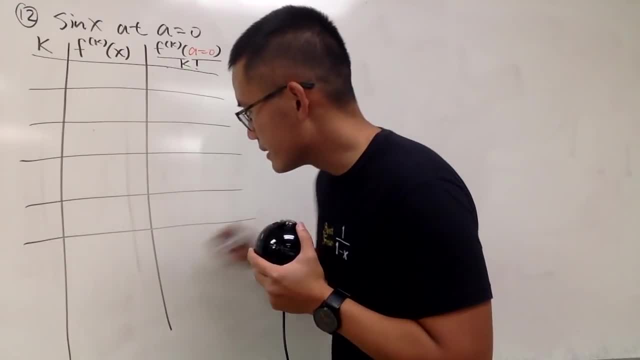 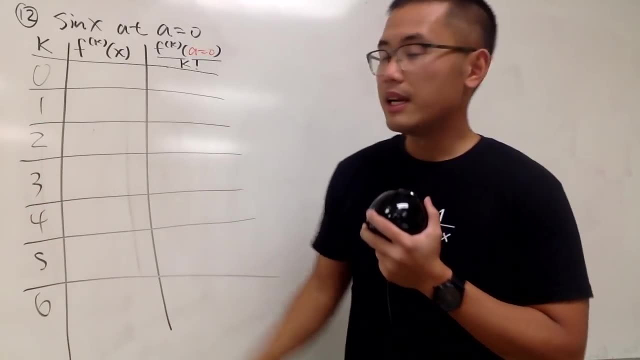 So let's see, I will do a few of them. I'll show you guys real quick. Go ahead: 0, 1, 2, 3, 4, 5, 6.. First we get sine of x. 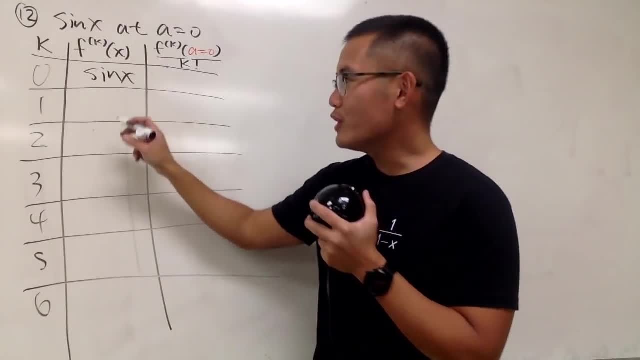 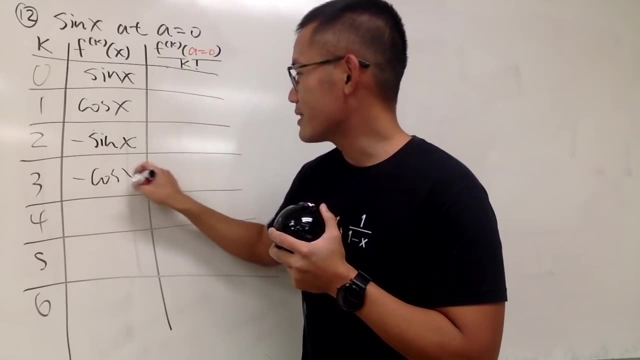 And here we go. This is the derivative function. So differentiate this sine of x. We get cosine of x. And then do it again: We get negative sine of x. And then do it again, We get negative cosine of x. 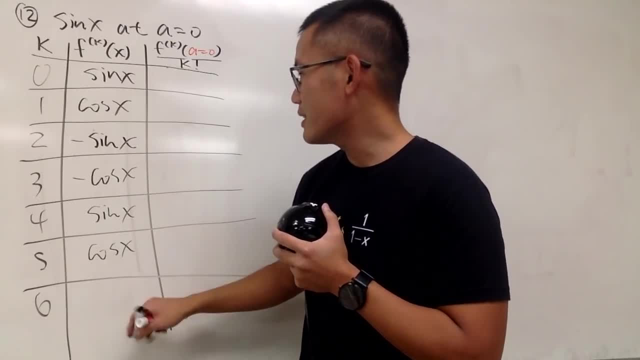 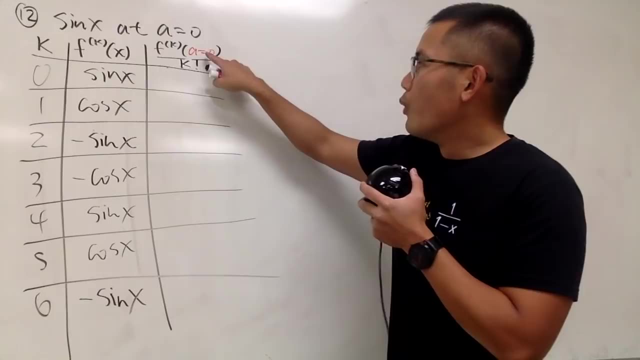 And do it again. We get positive sine of x, And then do it again. We get cosine of x, And then do it again. You see that it starts to repeat: Yeah, And so on, so on, so on. Now putting 0 in here. 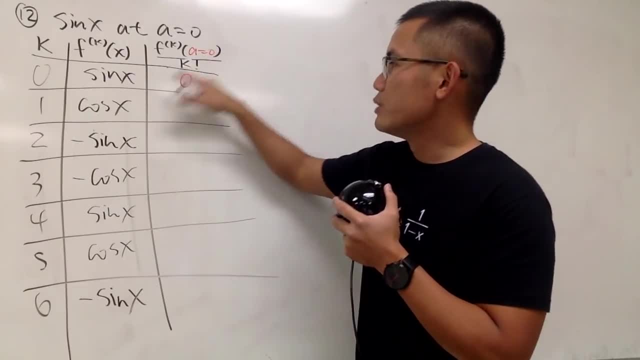 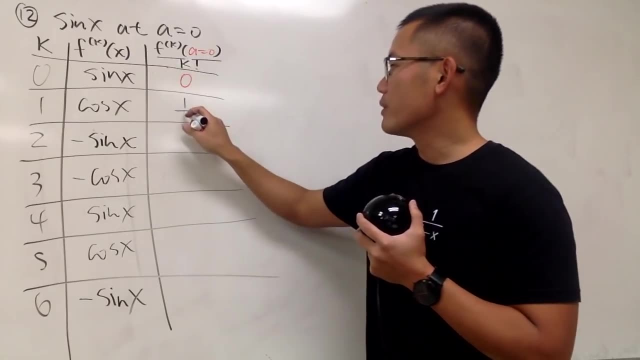 divide it by whatever, we still get 0. So that's gone. Putting 0 for cosine, we get positive 1. So it does matter, So we have 1.. And then over 1 factorial. So let's write that down. 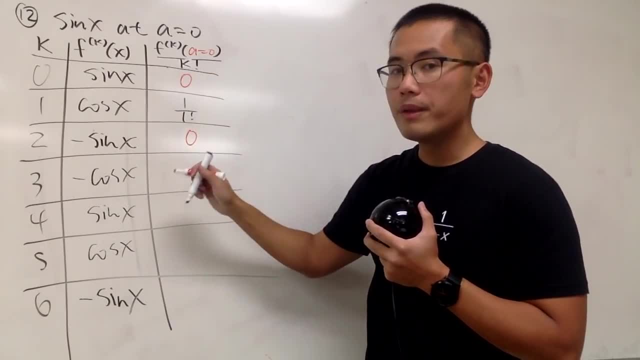 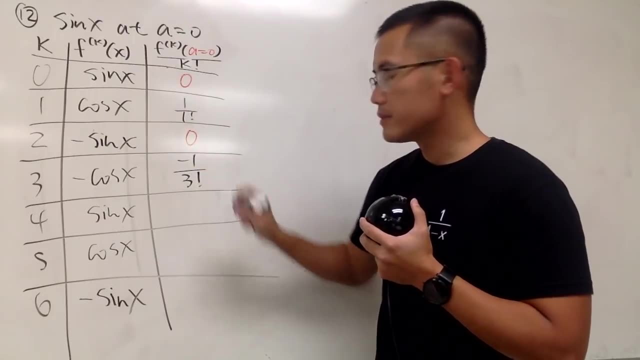 Next, when we put 0 in here, when we have sine, we get 0.. Well, next one: when we put 0 right here, we get negative 1. Divided by 3: factorial. Next, putting 0 into sine, we get 0.. 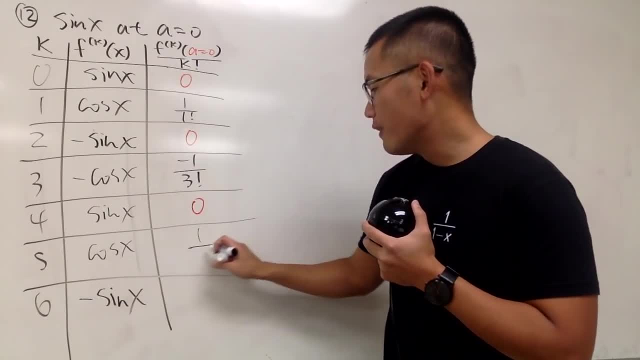 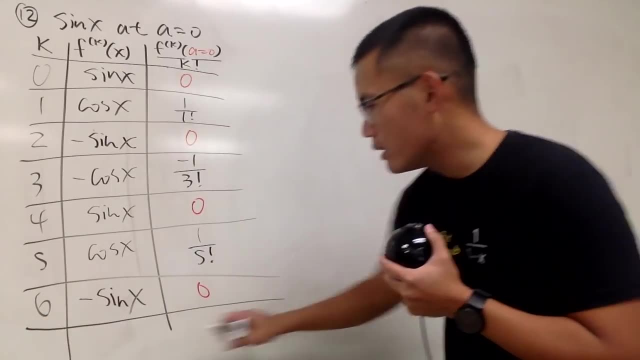 And next we get positive 1 again, And that's over 5 factorial. And the next one, if you're putting 0, you get 0. And if you would like to see one more, 7 is going to be negative. cosine of x. 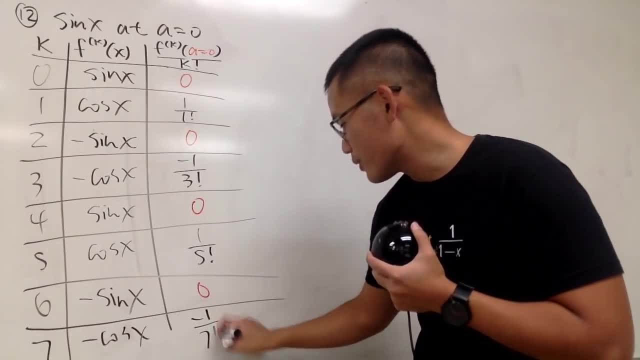 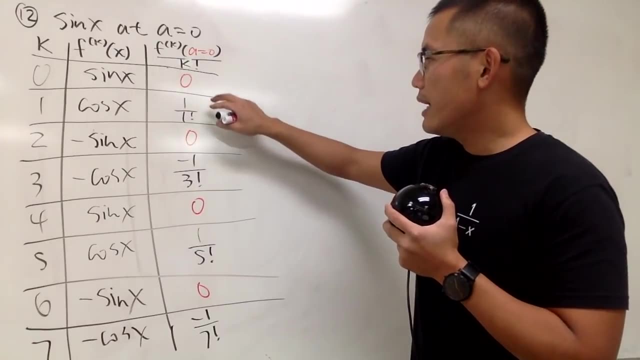 And you can guess that it was going to be negative. 1 over 7, factorial anyway, And so on. right, So here is the DEO. You see that you have 0. And this 0,, that 0, that 0, run. 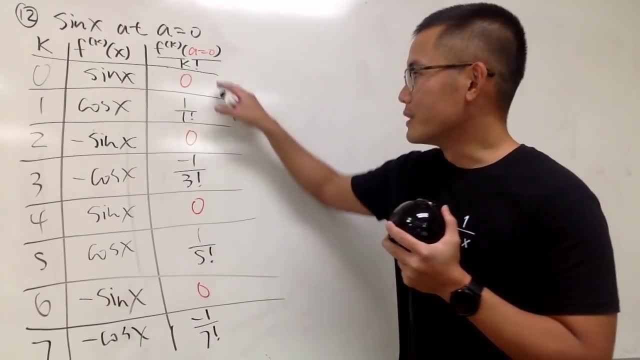 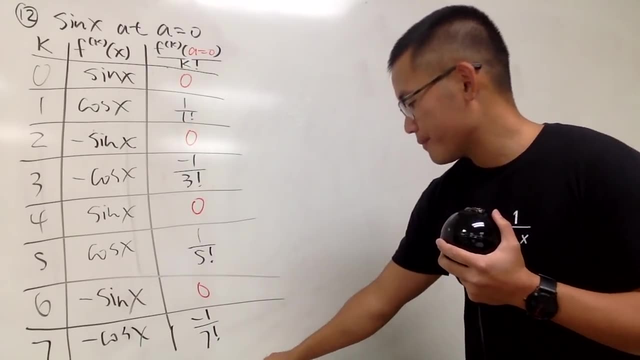 What you want to do is: do not try to write a formula with the 0s being included, Because that's like overkill. Just don't worry about it. Try to focus on a formula. Right, Try to focus on a formula. 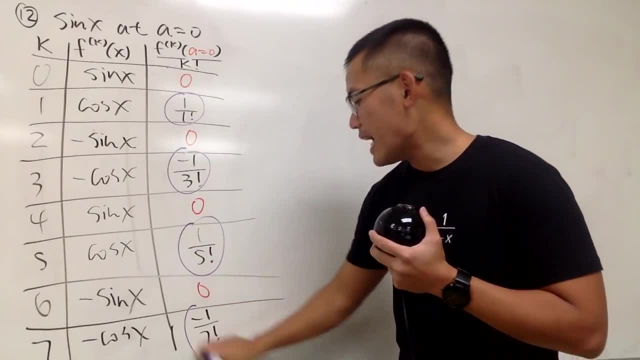 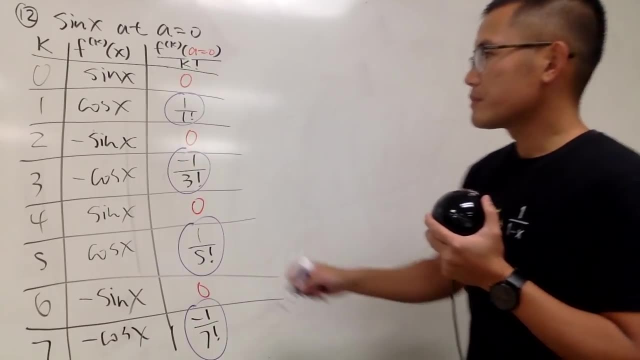 With this, this, this and that, only Right. So that will be the coefficients that we really care about. Well, when k is 1, we get this. When k is 3, we get that. When k is that, we get that. 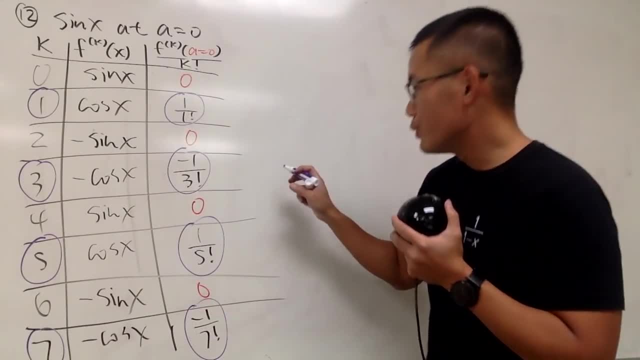 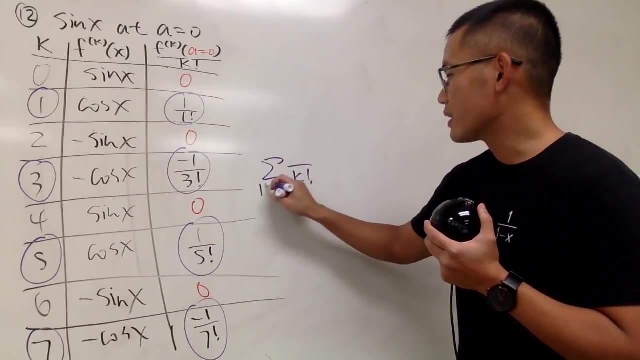 Right. But here's the trouble, though: We cannot do not just say over k factorial here, Because if you put down over k factorial, if you look at the k goes from 0 to infinity. if you put this down, you will be including these guys. 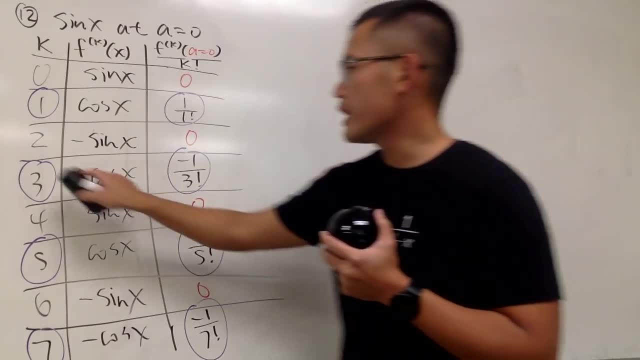 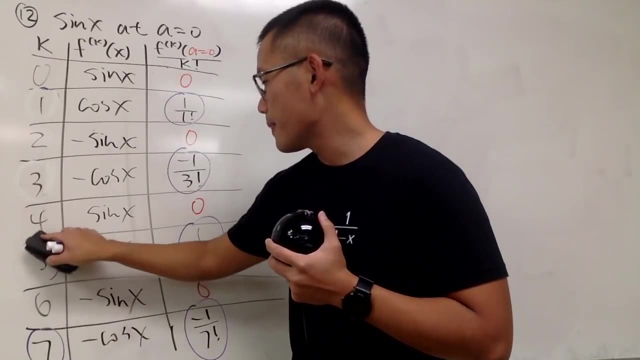 And that's no good. So, seriously, that's no good. So again, do not look at the k right here. This right here is just for us to set up the table Right. I shouldn't have circled the left-hand side. 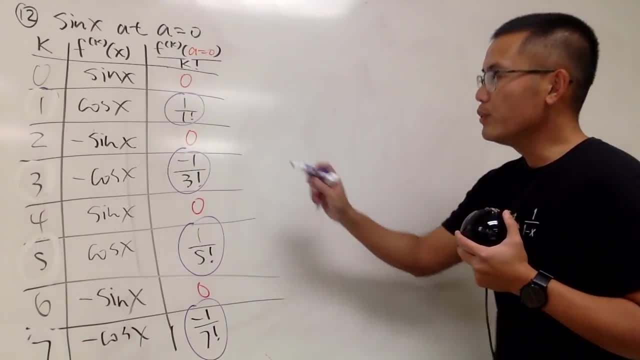 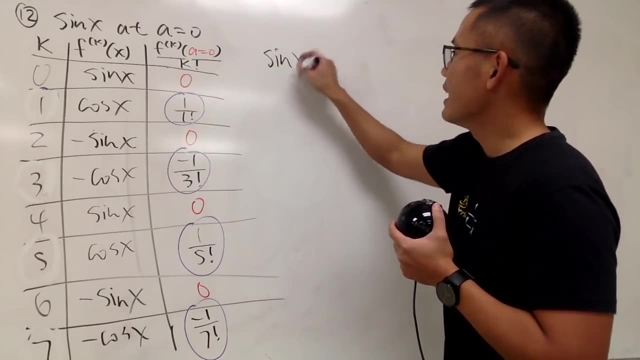 I just noticed that. But if you look at this, and now we'll be using n, So let me show you what we'll do with it. Here is sine x. I'm going to write down the terms For you guys. 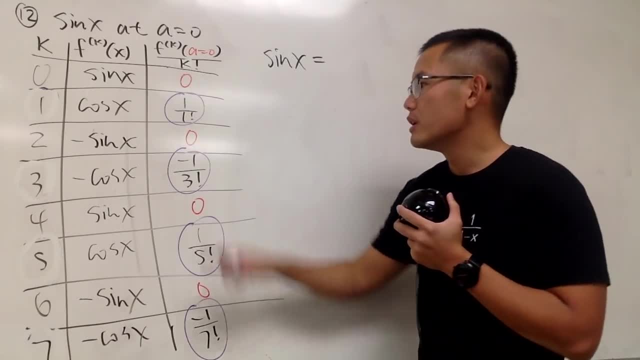 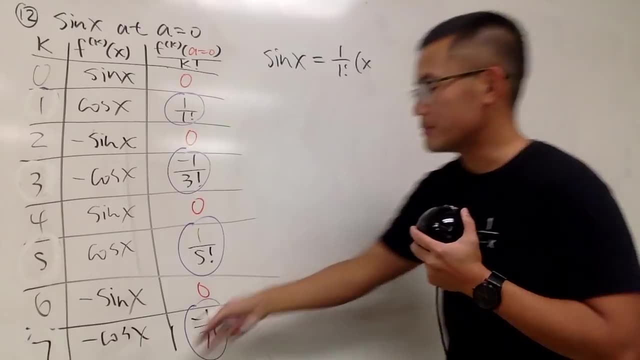 First Right. For the first time, this is the expanded version. This is what we have. We have 1 over 1 factorial times x Minus 0, so it's just times x By itself. Right here To the first power. 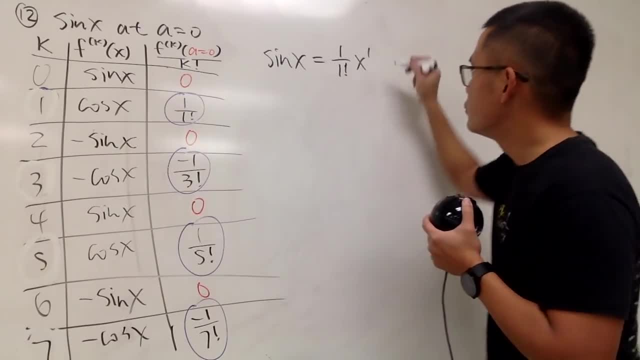 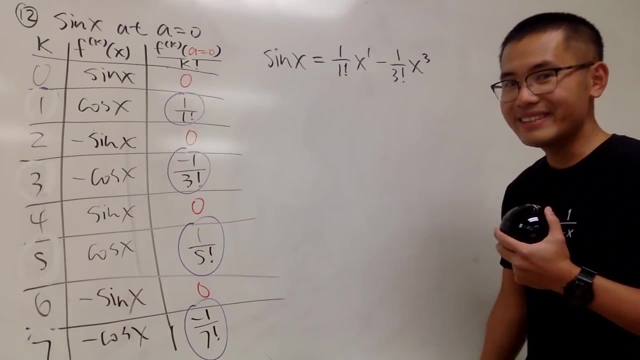 Okay, That's okay. Next we have this which is minus 1 over 3 factorial, And we have x To the third power: Okay, And then next we have that which is plus 1 over 5 factorial: x to the fifth power. 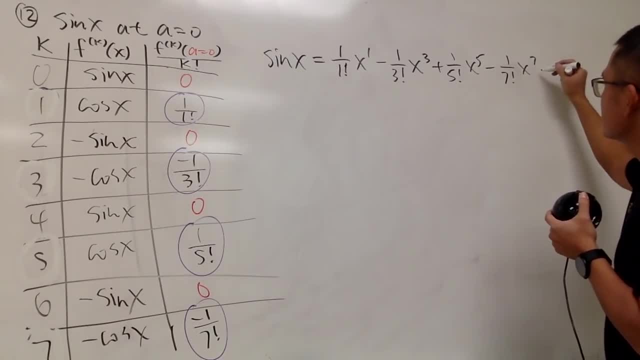 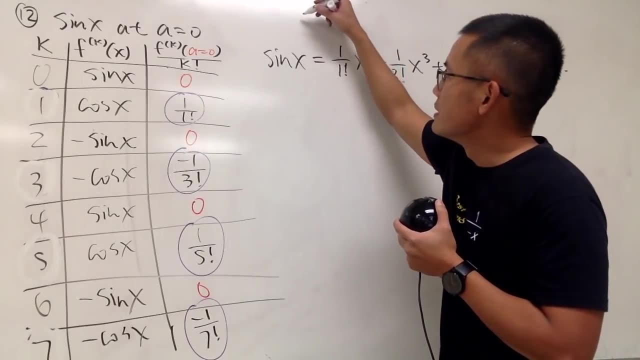 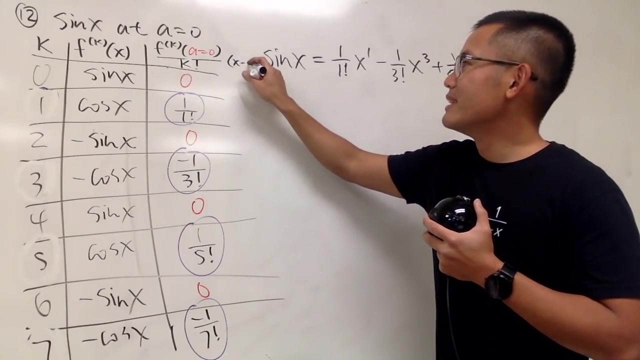 And next we have minus 1 over 7, factorial x to the seventh power, And so on, so on, so on, Like so Remember. remember. the formula Is this: And then times x minus a to the kth power. 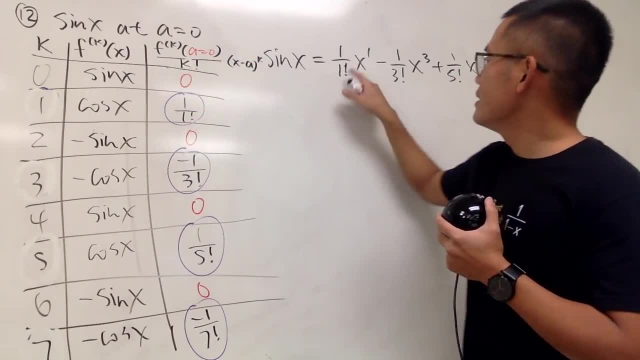 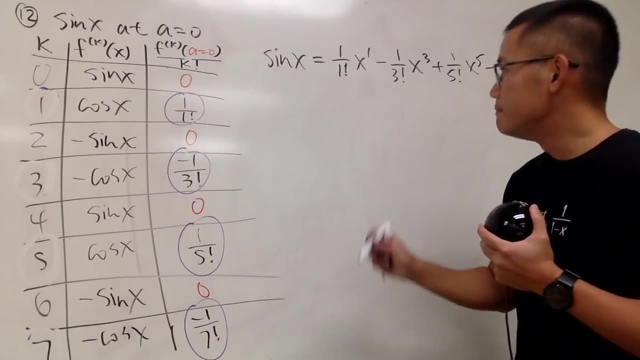 Right, That's the formula for that. So if you have 1, that part matches, That matches, That matches. That's okay, So that's okay. But now here is what we are going to do. We are going to be writing a formula down right here. 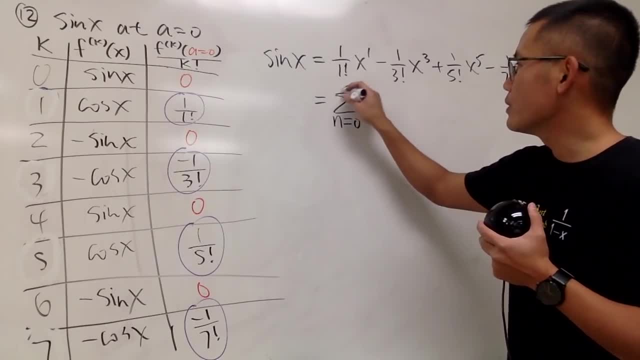 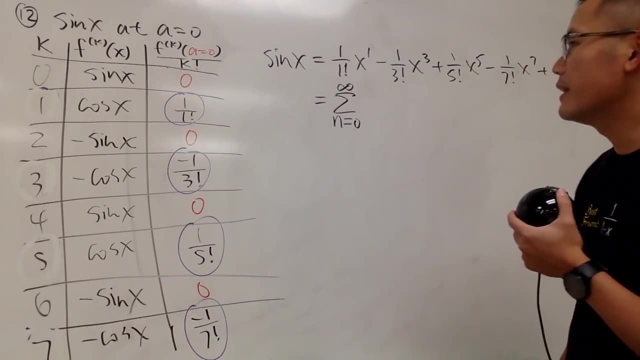 With n, With n, Which is equal to 0 to infinity. Again, we are just going to look at these things and then write a formula with a sigma notation for this. Alright, One more time. This and that match, This and that match. 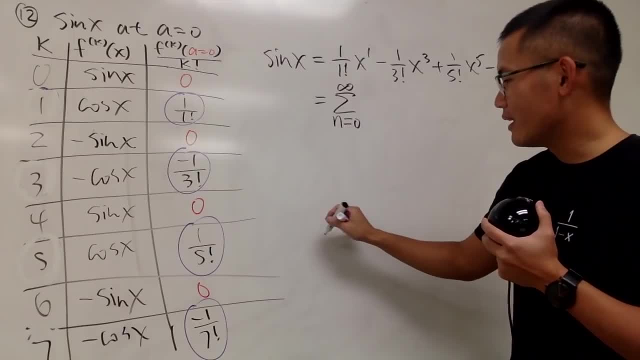 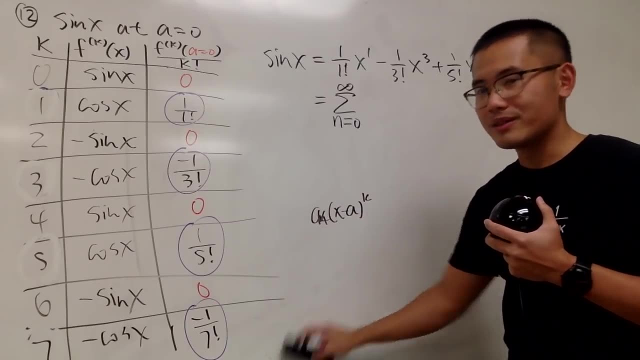 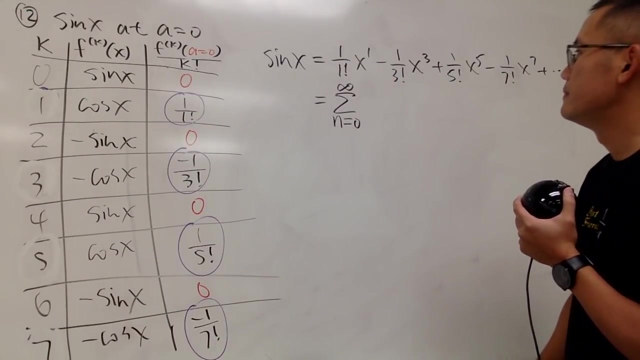 This and that match Because of the formula of the cn times x minus data formula, The k. I use k, So it's that one, Okay, Alright, Anyway, So n start with 0. Hmm, Okay. 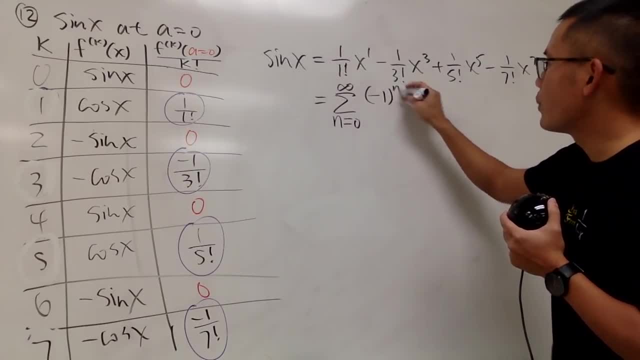 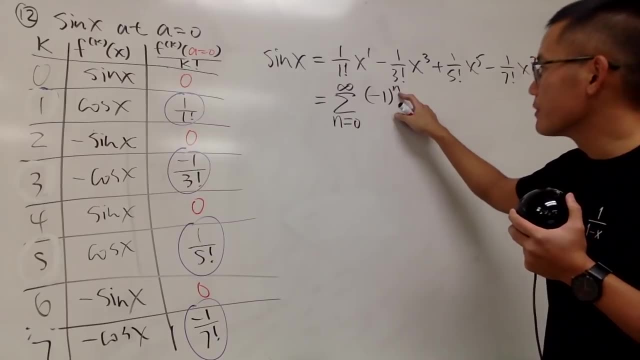 First of all, it's alternating, So I should have negative 1 to some power, Because n start with 0 and this is positive, So to the nth power works Right, Because this is when n is equal to 1.. 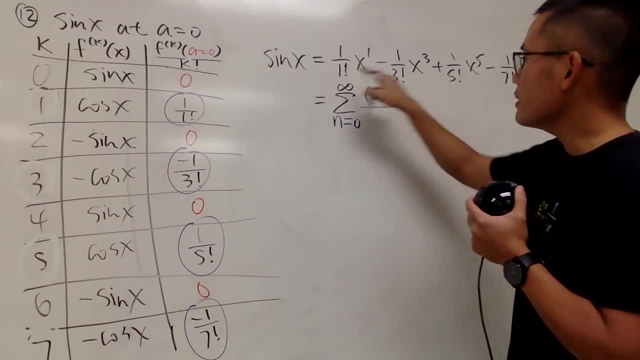 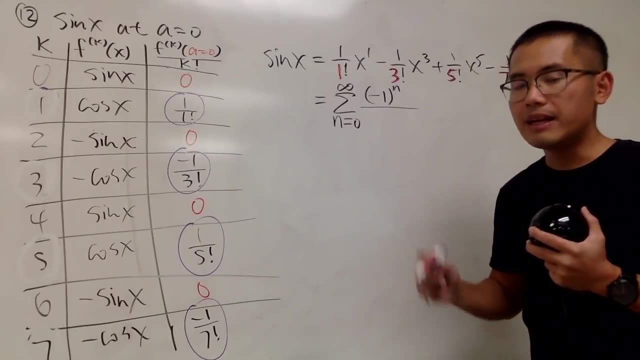 And you get negative. So that works. Next On the bottom here, if you focus on 1,, 3,, 5, 7.. That's just the r numbers. Well, r numbers is 2n. Either plus 1 or minus 1, depends on your starting value. 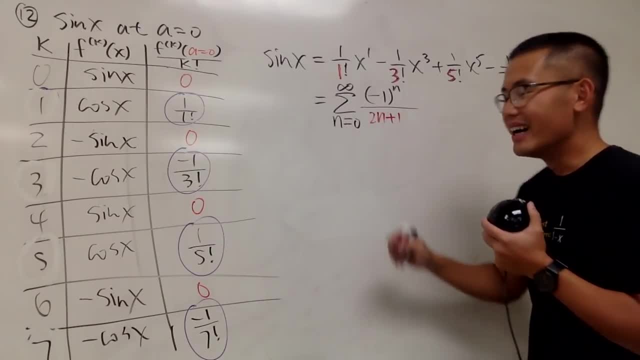 Because n start with 0, it will be plus 1.. Again, you see 1 to 3,, 3 to 5,, 5 to 7.. The difference is 2 every single time. So that's a coefficient of n. 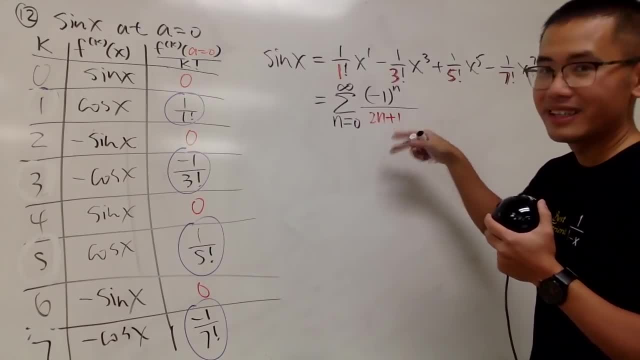 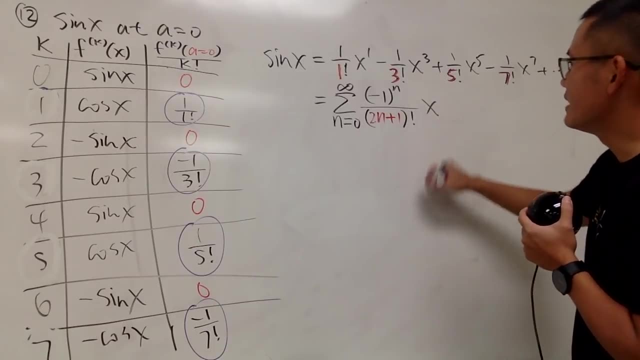 Because n start with 0, so you have to add 1.. See, So you get 2n plus 1 for these numbers And then you factorial that Right. Then you see this is x And again this, and that match. 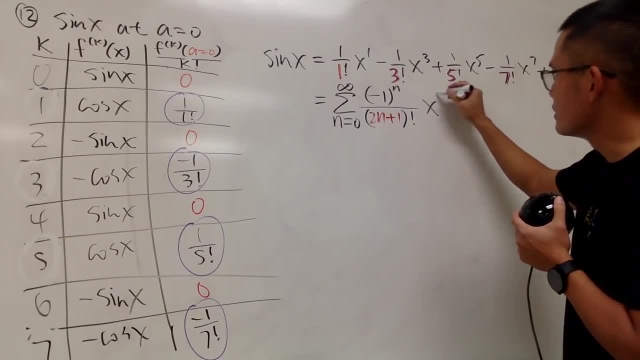 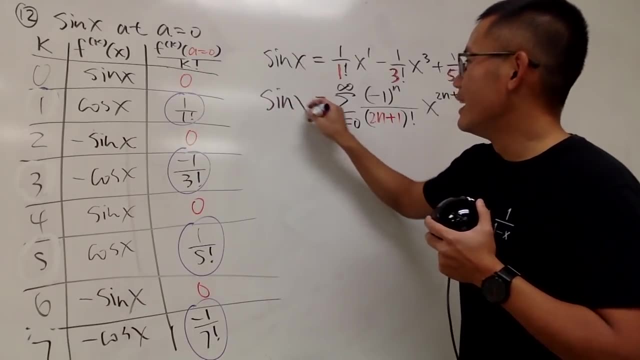 So this will become the power right here. So this is 2n plus 1 power. So that's it Right. So this is sine x. And again, the reason I use k over there, it's because we have the zeros in between. 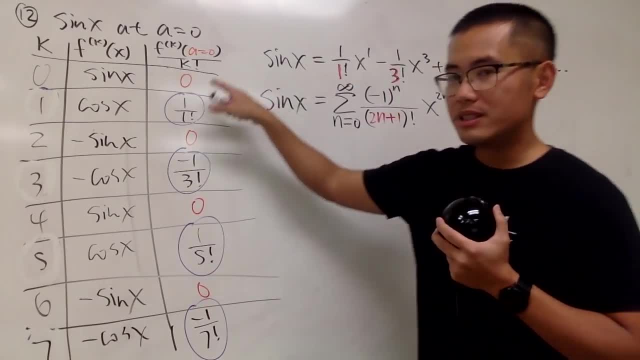 We don't want to write a formula with sine x. We don't want to write a formula with sine x. We don't want to write a formula with sine x. We don't want to write a formula with the zero being included, because that will be redundant. 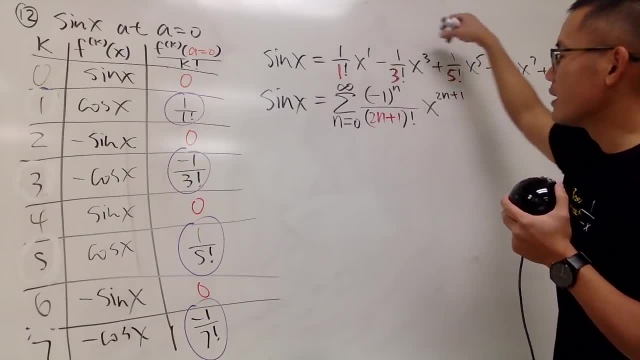 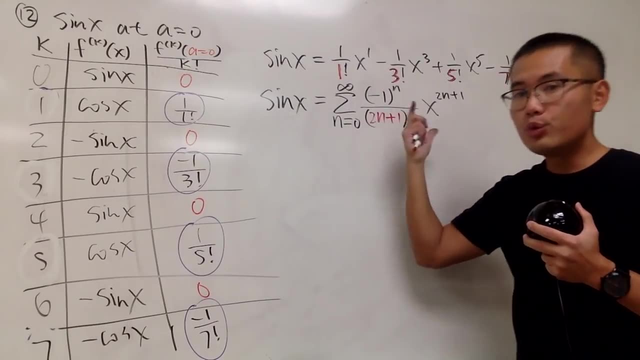 That's why I use k on purpose, And then I just write down the remaining terms, the actual terms with all the zeros, And we look at the remaining terms and write them down into the sigma notation And finally I use n. So that's the idea. 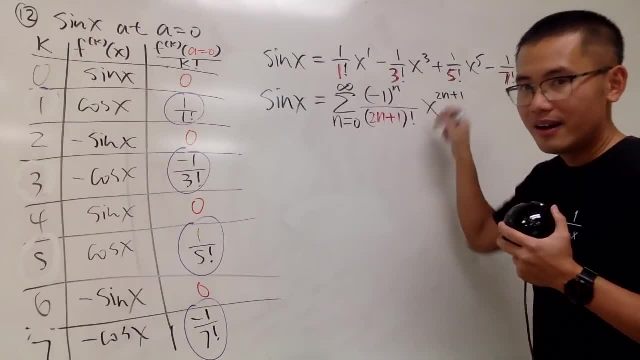 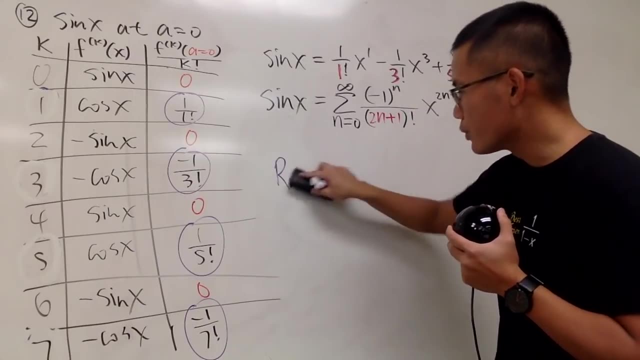 All right, Here is the cn, So I will compute the r real quick. So here we go. So here we go. So the cn is equal to the limit, as n goes to infinity. So here we go. 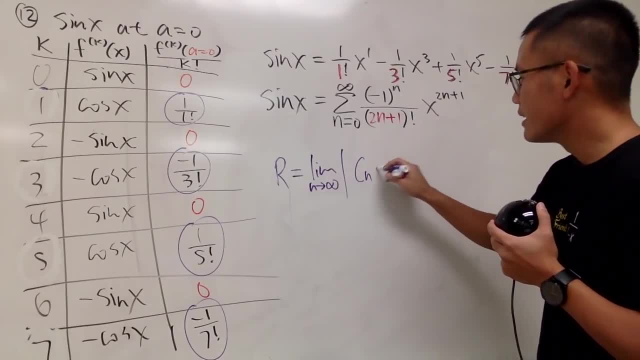 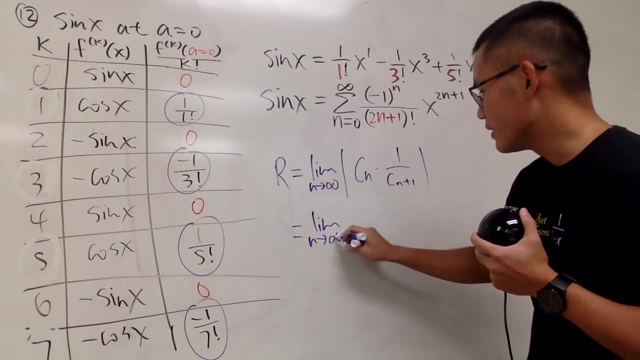 So here we go, And again, I will just write this down just to emphasise: it's cn times 1 over cn plus 1, right. So let me just emphasise, If I didn't emphasise clear enough earlier. 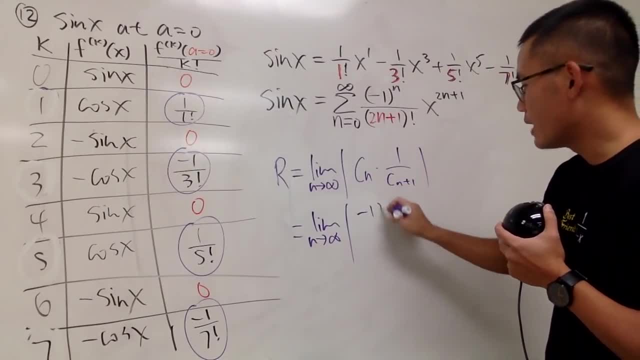 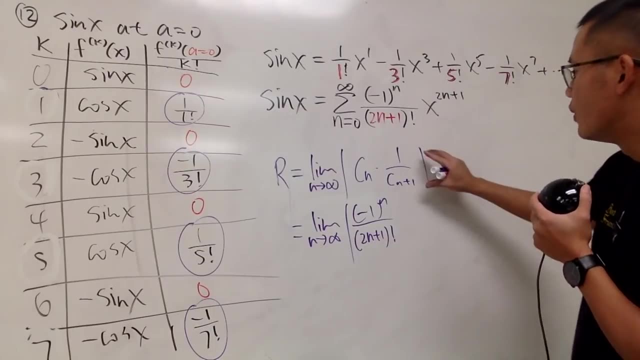 cn is all this. So I will just write down negative 1 to the n-th power over 2n plus 1 factorial that. 2n plus 1, factorial that, And for the cn plus 1, I'll just put n plus 1 in here and do the reciprocal. 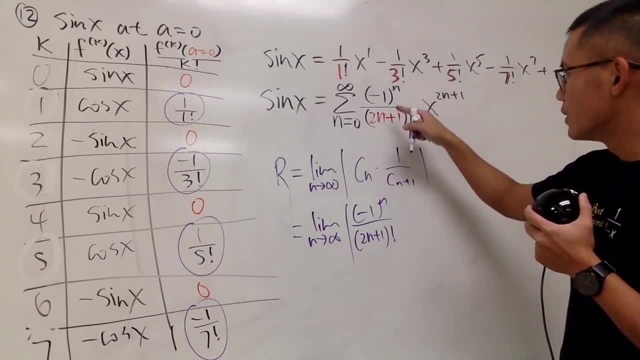 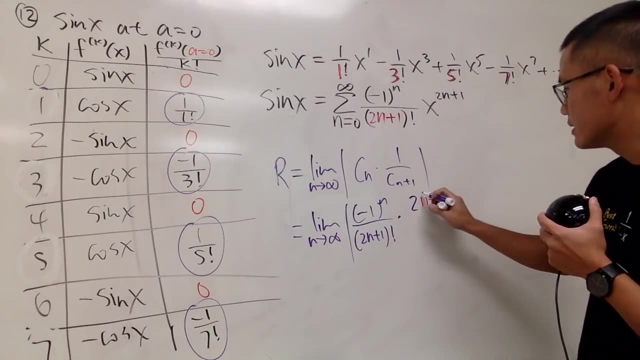 Remember it's the reciprocal right. So I will just put n plus 1 in here, So we will have 2 and then n plus 1, like this in parentheses, and then plus 1.. And then factorial that And divide it by negative 1.. 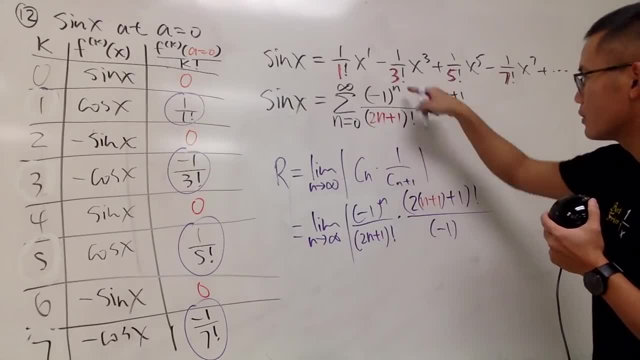 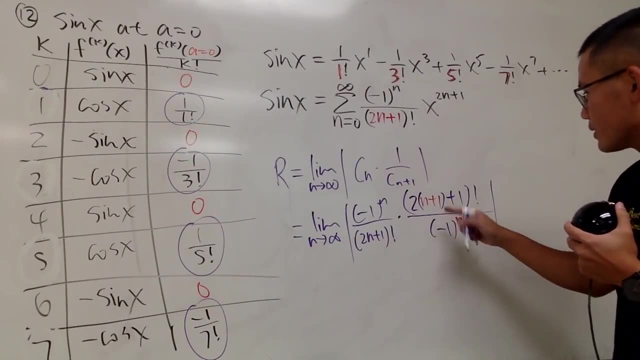 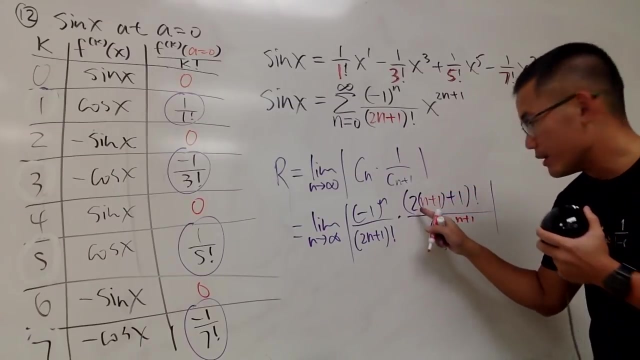 And I have the cn plus 1, so this right here should be n plus 1 as well. Like this, Close that. Now I will work this out in detail for you guys. This is the cn plus 1.. This right here, 2n plus 2, right. 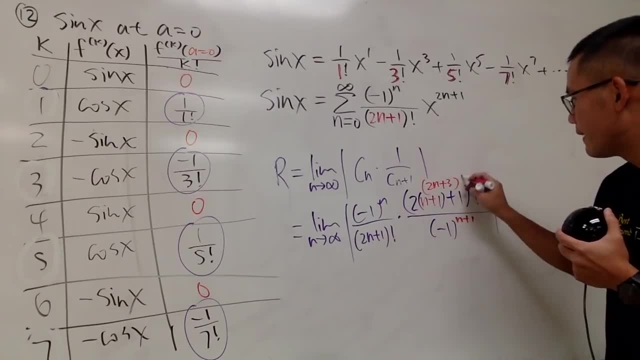 And then plus 1, so you have 2n plus 3. Factorial that. So if you expand this, you get 2n plus 3. That's the first term, And the next term is 2n plus 2, because you just minus 1.. 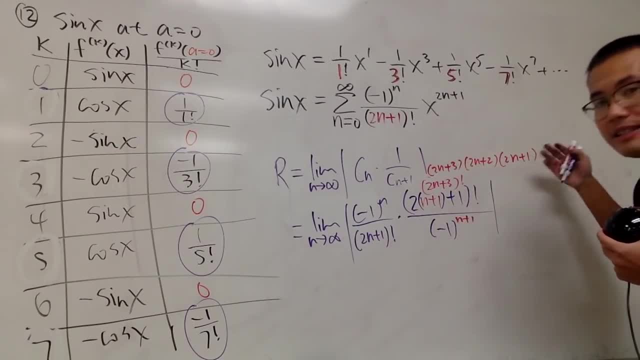 And then the next term is 2n plus 1.. And then 2n, and then 2n minus 1, and so on. But you can just factorial this guy and you stop. The good thing is that this and that can be cancelled here, which is very nice. 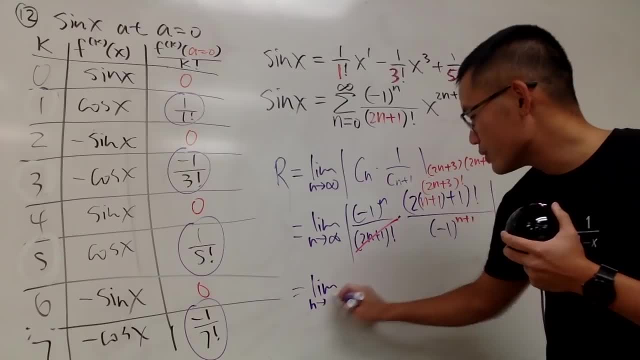 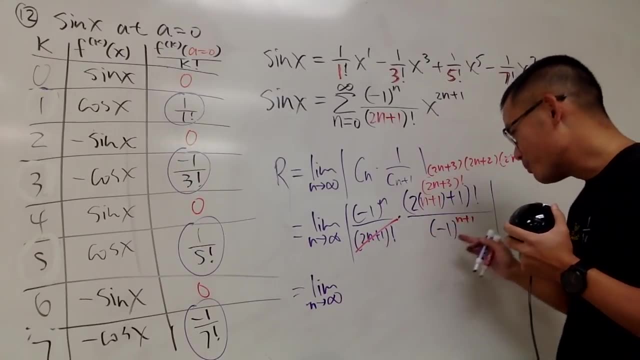 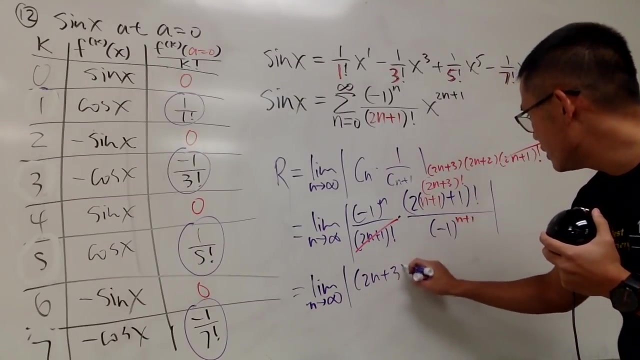 And now we are looking at the limit as n goes to infinity And we just have this. And, by the way, the absolute value right just pretty much make all the negative positive. So this and that don't matter. So we get absolute value of 2n plus 3.. 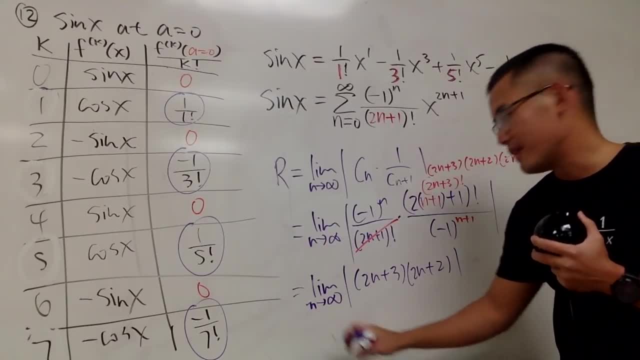 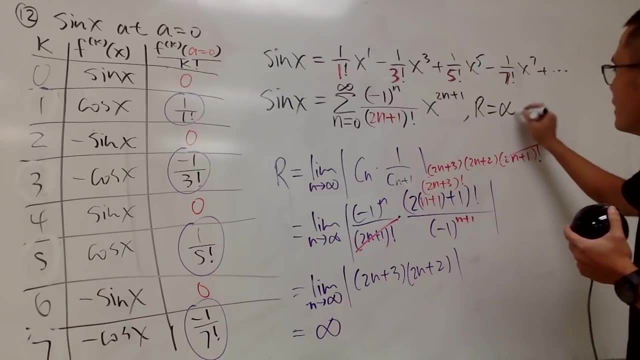 2n plus 2.. Yes, it will be infinity when n goes to infinity. So this is just as nice. We get r equals infinity. Likewise, i will be negative infinity to positive infinity as well. Do not include infinities. 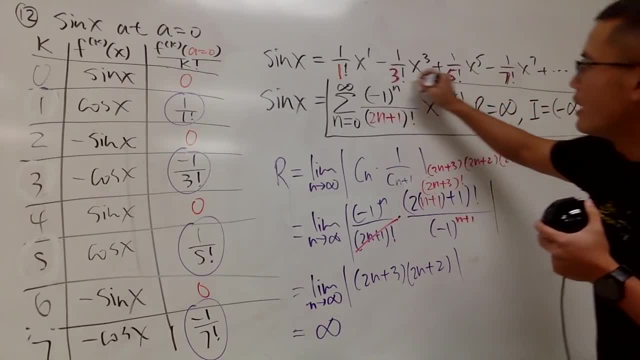 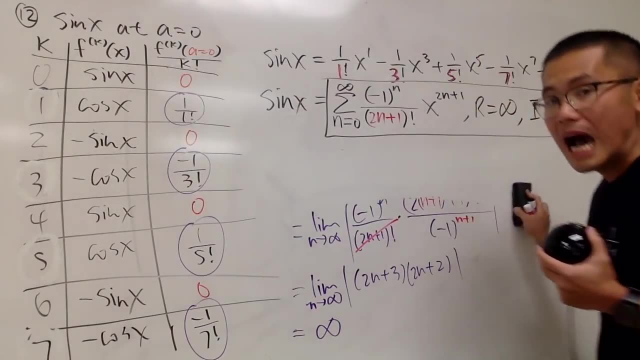 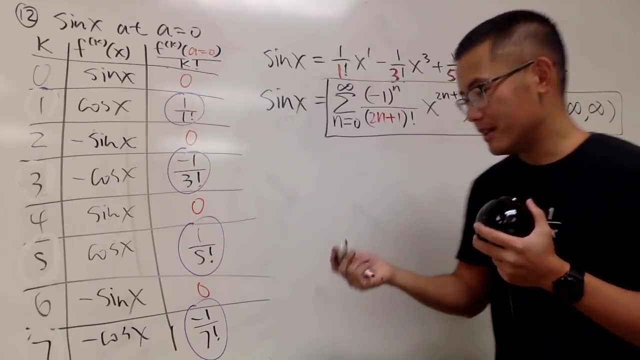 That's why I just put down parentheses right away. Okay, So it's just like this one, Cool huh. Now I will show you how we can find out the next one Within this little box right here. Okay, So the next one, number 13,. we will be dealing with cosine, right? 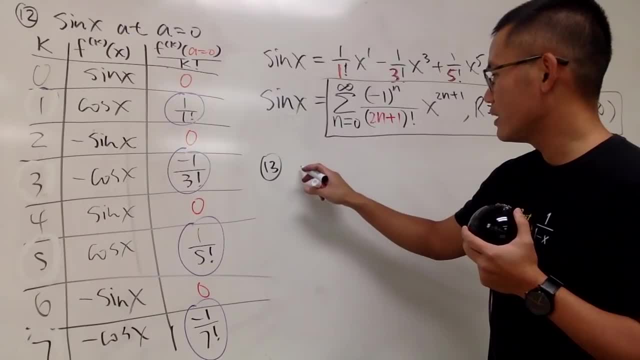 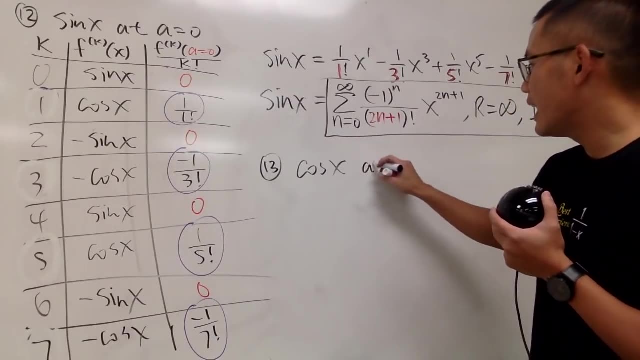 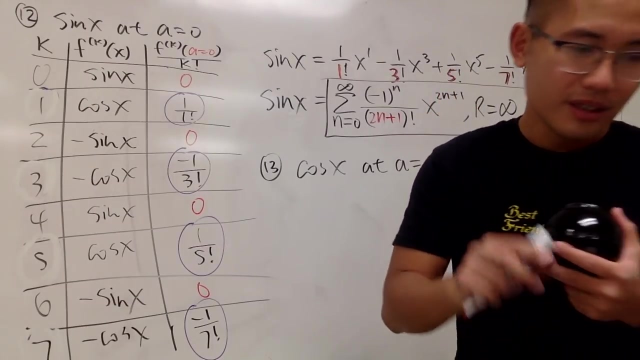 So for cosine, I will just put this down right here: Cosine x, And again centered at a equals 0.. Don't worry, I will be dealing with different centers in the next few questions. All right, So just hold on. 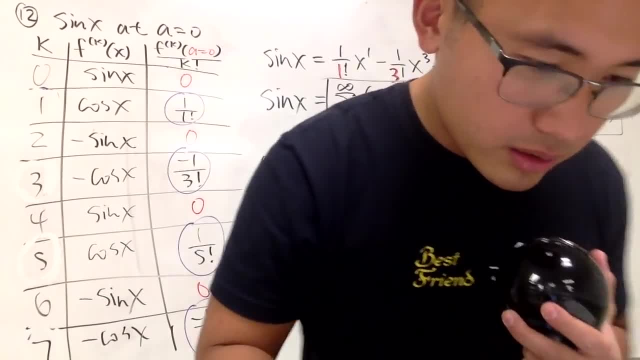 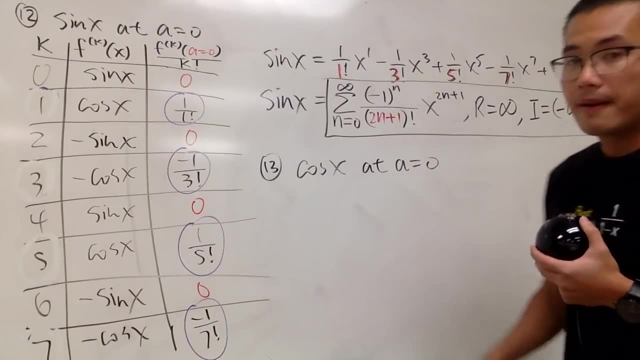 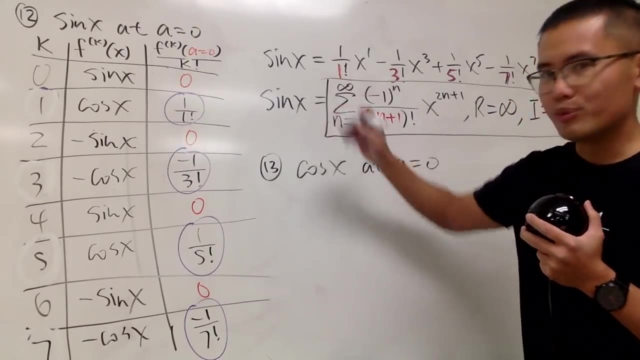 Hold on to that And let me see if I go All right. So let's see if there's any connection between sine and cosine. Yes, there is. There are a lot of connections that I won't miss, But the best connection is, of course, if we differentiate sine, we get cosine. 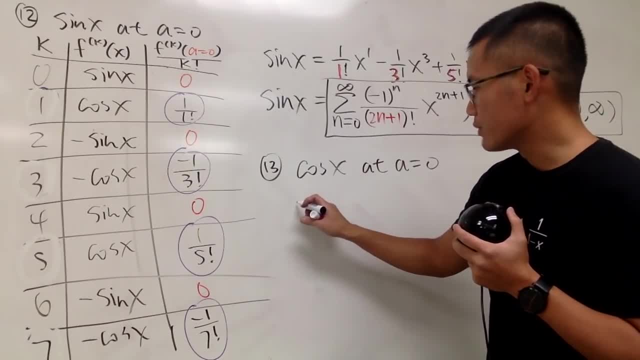 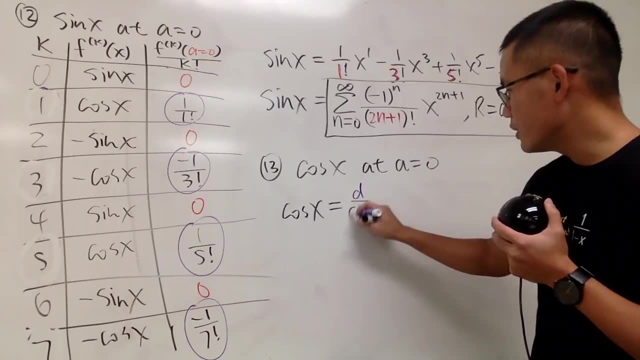 And that's very nice. So I will just go ahead and do this for you guys. We know cosine x. This right here is equal to. We can just differentiate. I'll put this down: We'll just differentiate sine x. That's pretty much it, right. 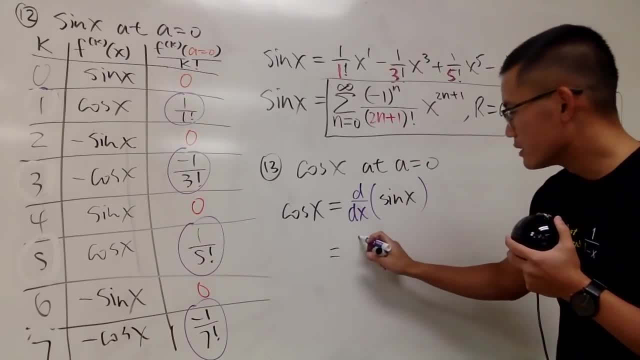 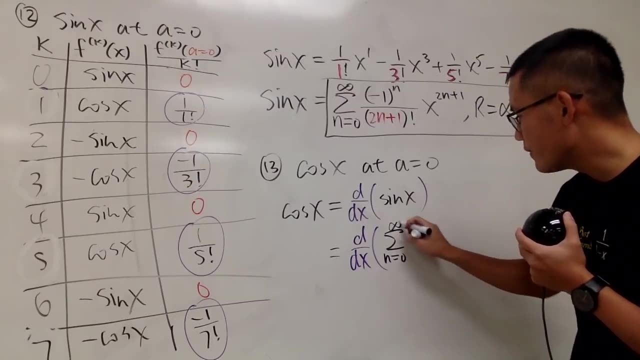 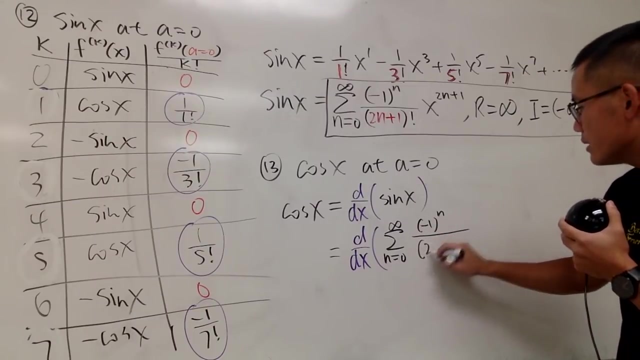 And of course we will be looking at the power series. So let's go ahead and say: differentiating sine is all this. So we have the series as n goes from 0 to infinity And we have negative 1 to the nth power over 2n plus 1 factorial that 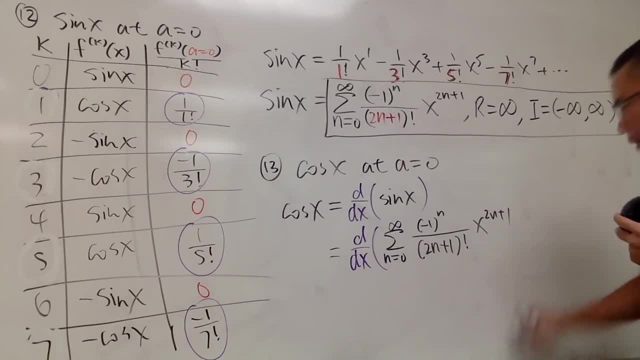 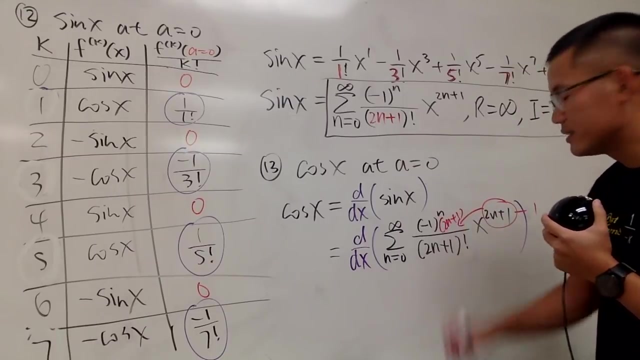 And then x to 2n plus 1 power like so right, and do not put down the x. this is for differentiation. now check this out. take the derivative this, go ahead, bring this to the front and then minus 1. well, when you bring this to the front, you have the 2n plus 1 here, isn't it this right? here it's the same as 2n plus. 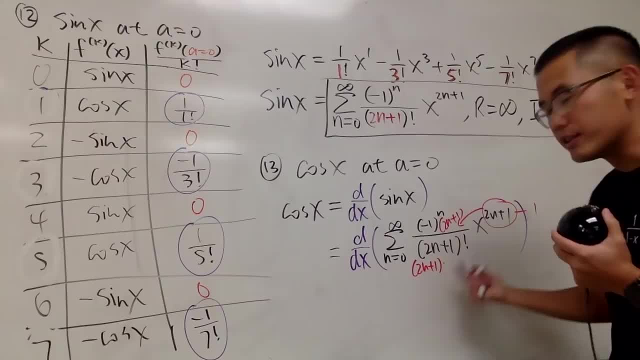 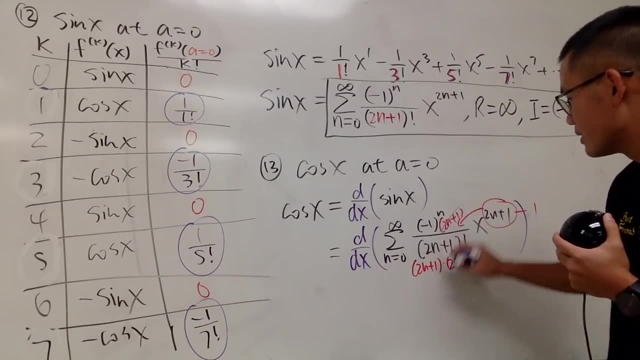 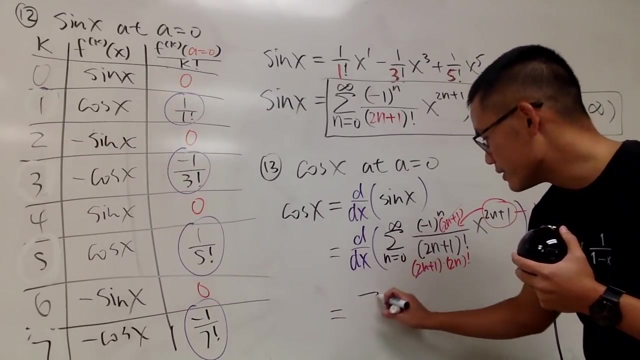 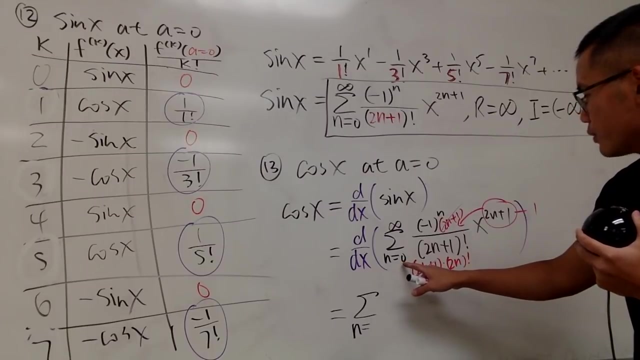 1 times 2n times 2n minus 1 and so on. in another word, 2n in parentheses, factorial. that best thing is this and that will cancel nicely. so i will write this down for you guys. this right here we get a series as n goes from. well, notice this, and that cancel if you put 0 into the n. 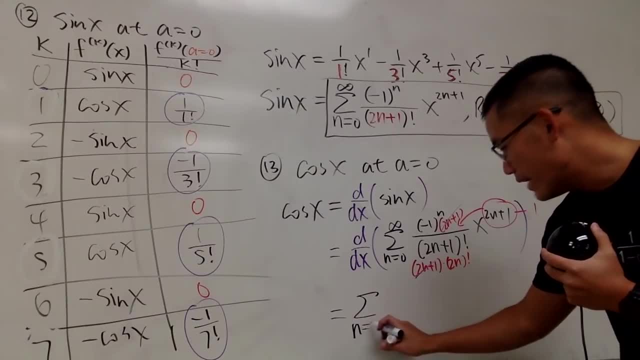 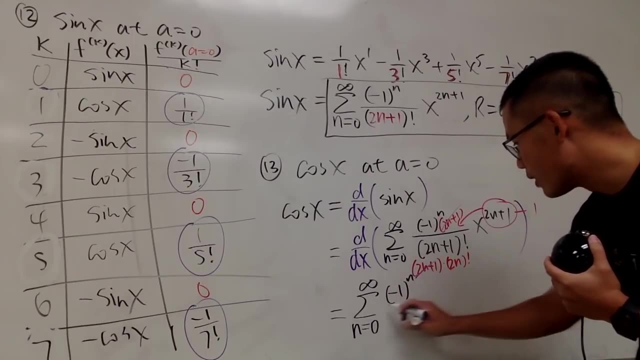 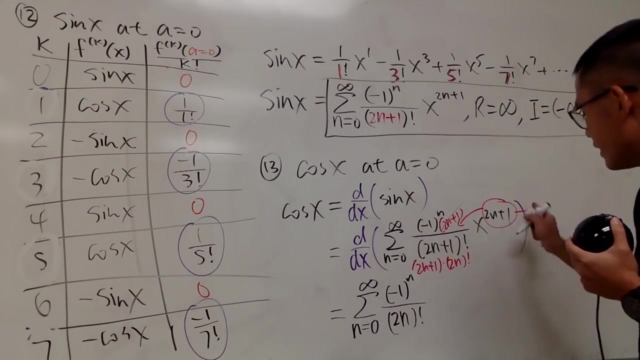 the first test states there's no 0 term, so n will still go with 0 to infinity. this right here is negative. 1 to the nth power over this is just 2n factorial. now and here we will just have x to the 2nth power And again n still start with 0, because 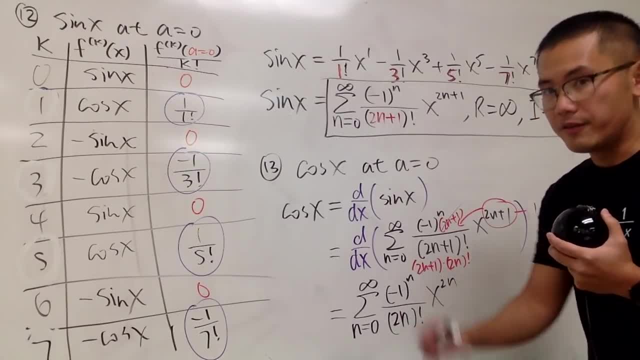 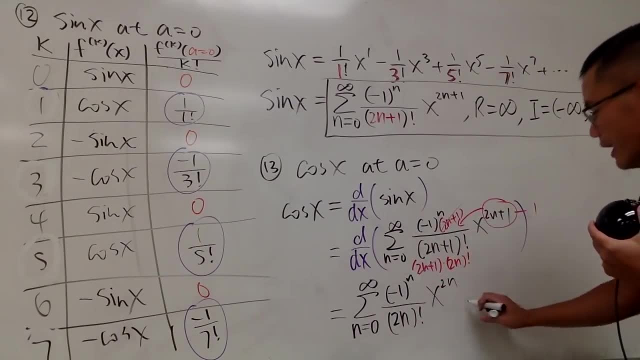 if you put 0 right here and right here, 0, factorial by definition is 1, so you do have to start with. n equals 0 in this case. This right here is a series for cosine, and the good thing is that r will stay the same because we just differentiate the power series and 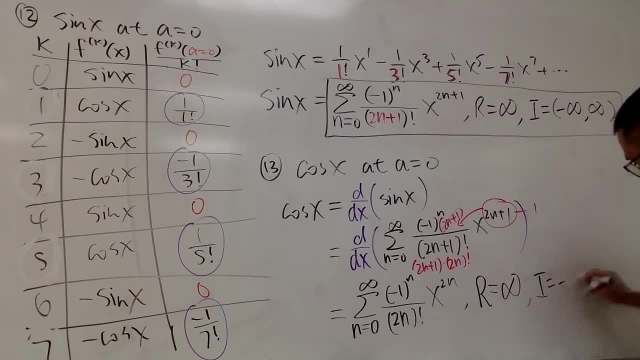 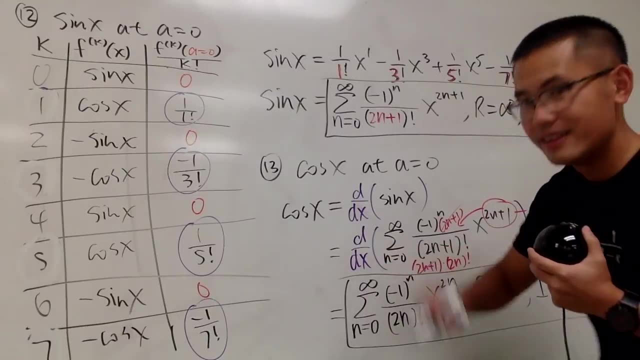 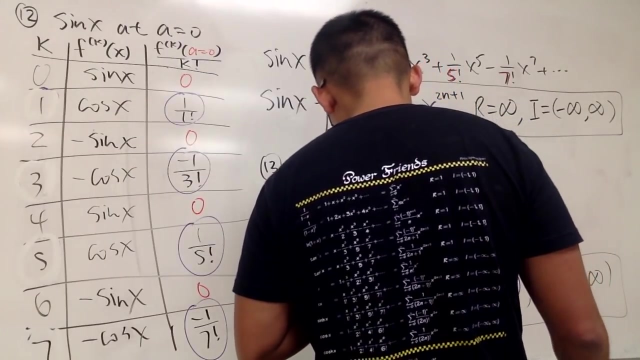 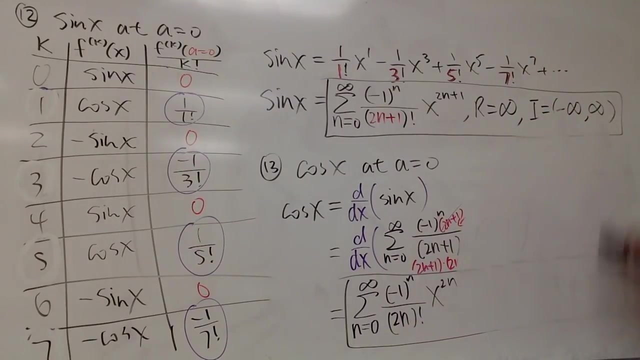 if r is infinity, well, I will be going from negative infinity to positive infinity. so this is it. This is for cosine x, like this. Very good, right Man. there are so many power series. I don't know if I can learn all this or not. Alright, anyway, this is 13,. so we. 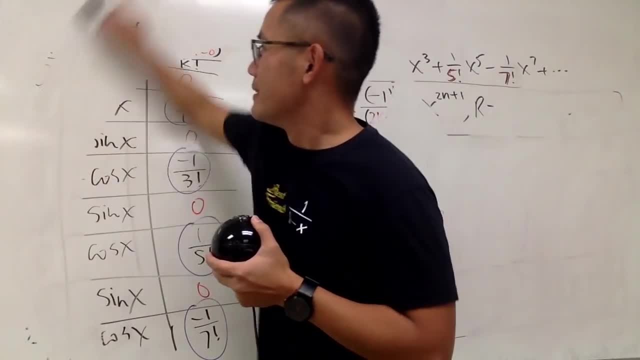 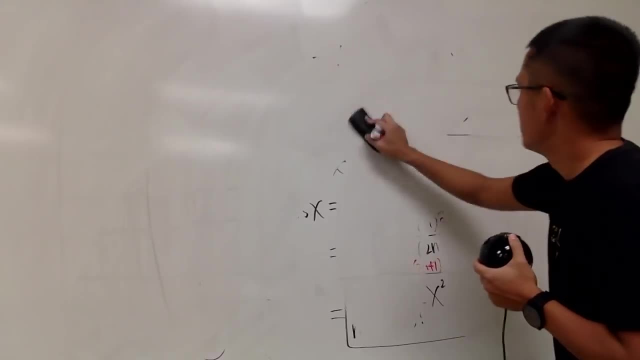 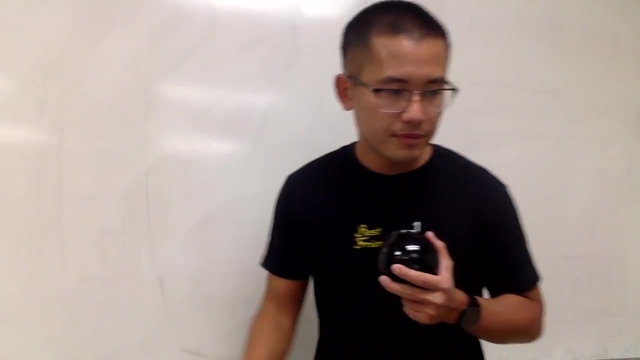 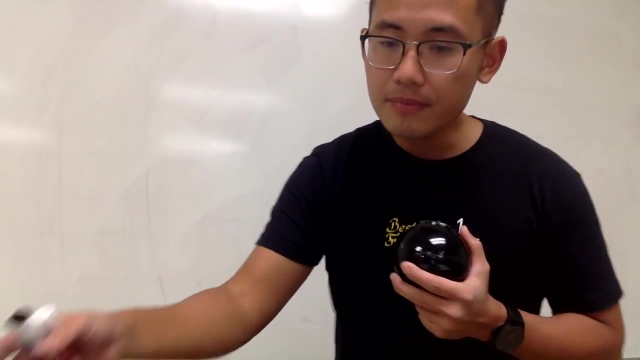 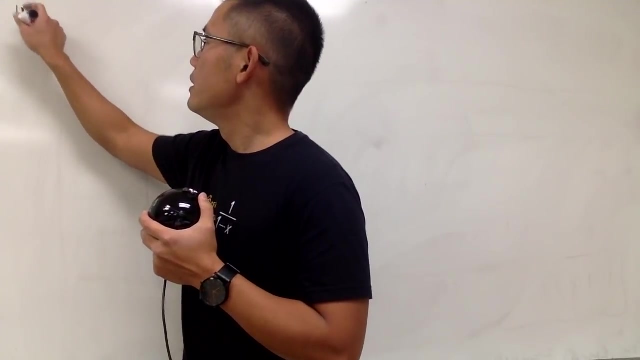 did half marathon already. Now, number 14 is the time that we are going to kind of play around with the center. So, as usual, here we go. Number 14 here is right here. Wait, that was number 14.. 12,, 13,, 14,. 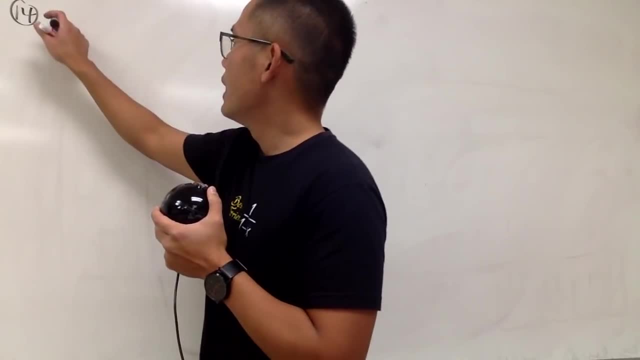 12, 13,, 14.. 12, 13,, 14,, 14.. 12, 13,, 14, 14.. 12, 13,. that was 13,. yeah, So number 14,. we have e to the 3x, but this time the center. 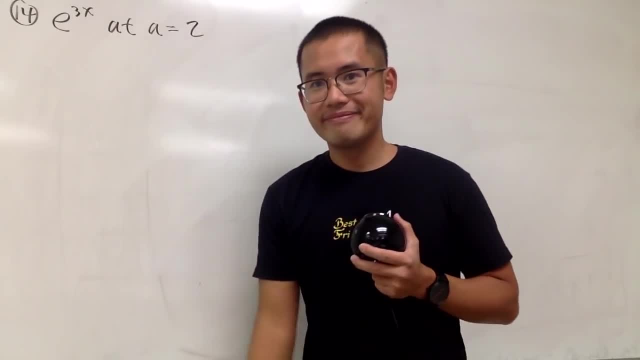 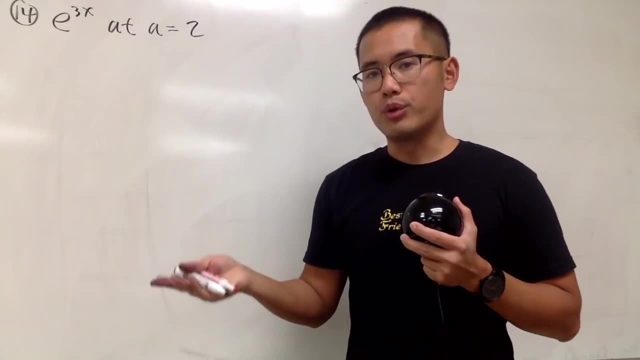 is going to be at 2.. Two choices: One, you can still do the table, and this time you have to plug in 2, and you can produce that. I did that before, so if you want to check that out, you can check that out Here. I'll show you how it gets a different way. Write. 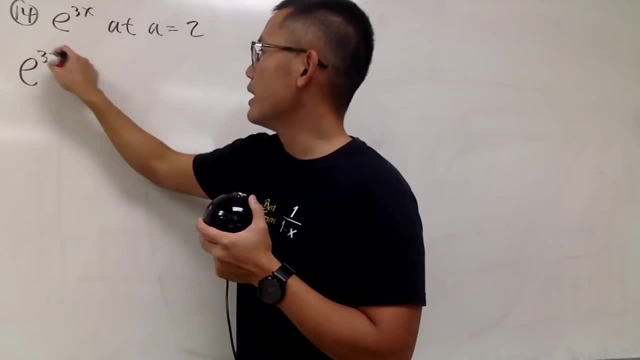 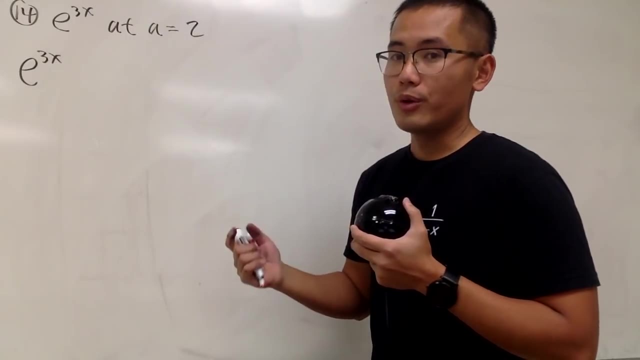 down what you are working with, which is e to the 3x. This is the 1 that you are trying to get right, And you should also put down the 1 that you know, but that's a little later. This is e. 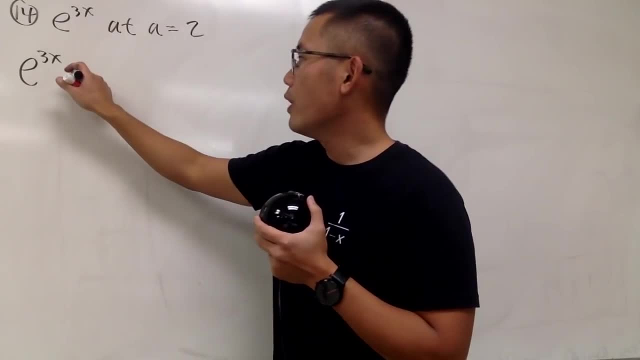 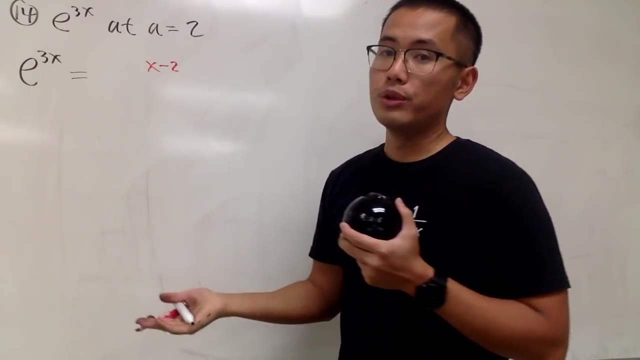 to the 3x. What you want to do is: well, if the center is at 2, then that means you should have x minus 2 as your input. okay, And because we have this 3 in the front, so of course, 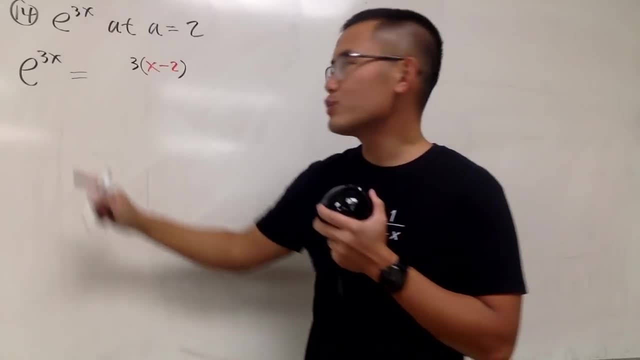 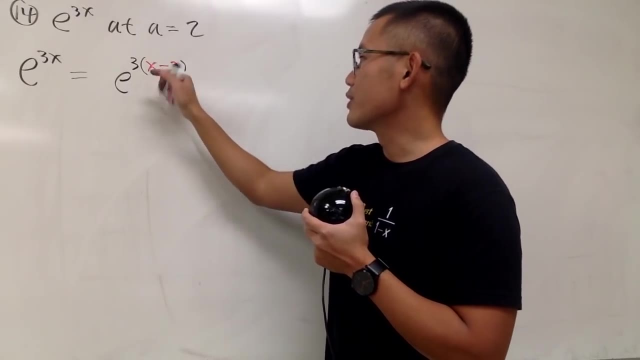 don't forget, we have the 3 in the front, like so, And of course we have the e. so we have e to that power, okay, And of course, if you distribute the power to the center, you will get the power. This is going to be 3x times well. this is going to be negative. 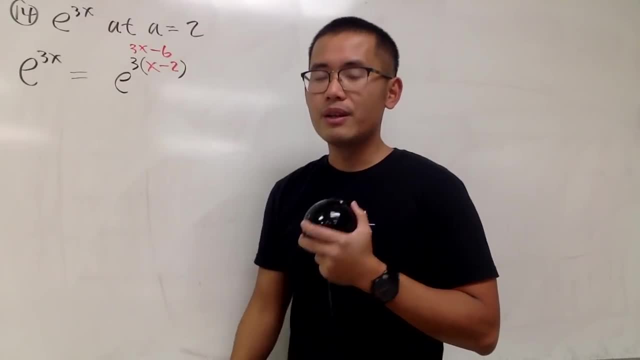 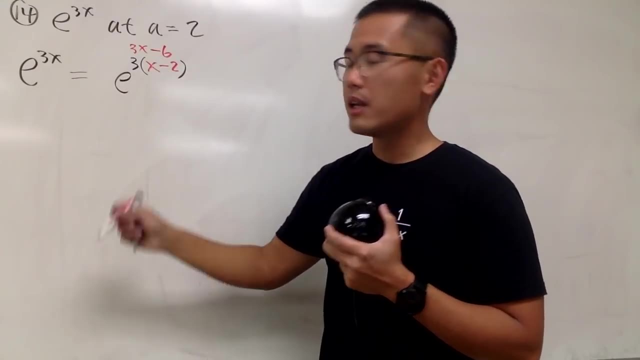 6,. right, This is, of course, not the same as that. You just have to make it the same thing, you'll be happy. We need the negative 6, and this is e to the negative 6 power. We're going to cancel that, So it's just going to be multiplied by e to the positive 6, because 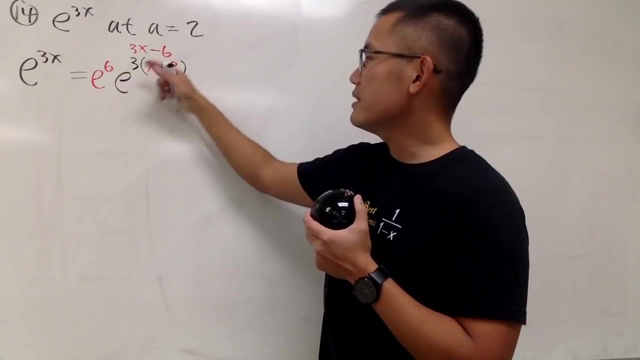 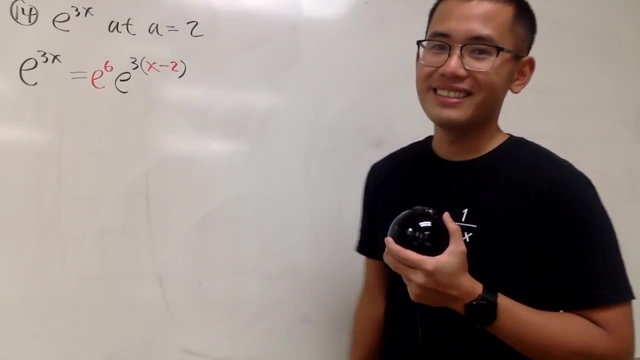 if we have e to the positive 6 times e to the negative 6, you just add the exponents, just kind of introduce new things. That's it. Okay, That's it. And now, which one are we going to use? Of course we're going to use. 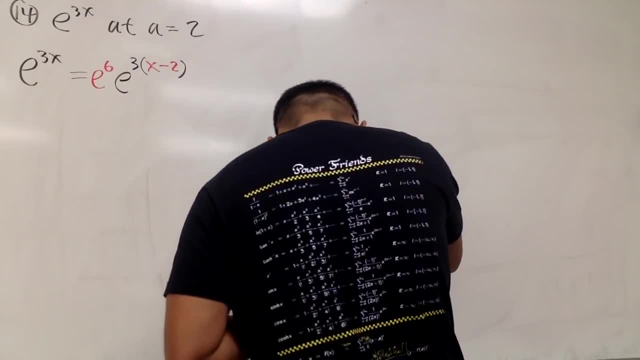 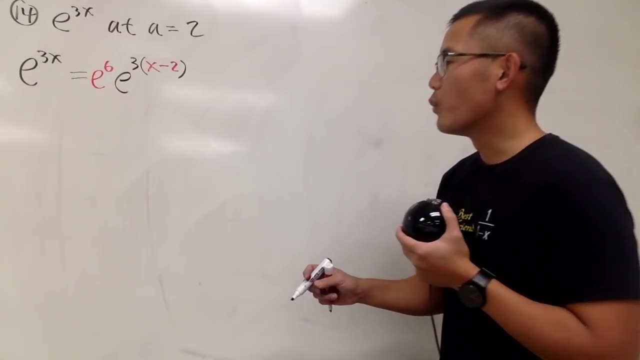 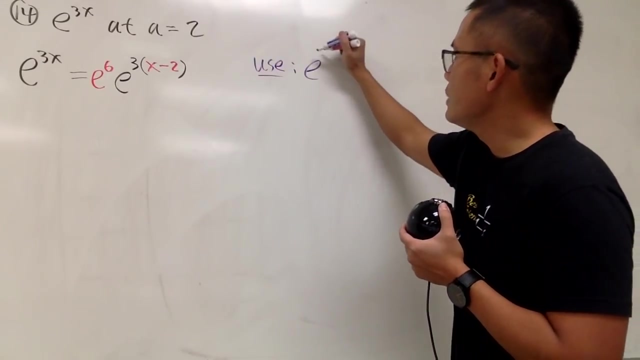 our other friend Man. I don't know which one is my other friend, Of course. e to the x is our other friend. all right, So this is the one that we are going to use. I will just put this down right here. I'll just say: use e to the x. This is equal to the series. 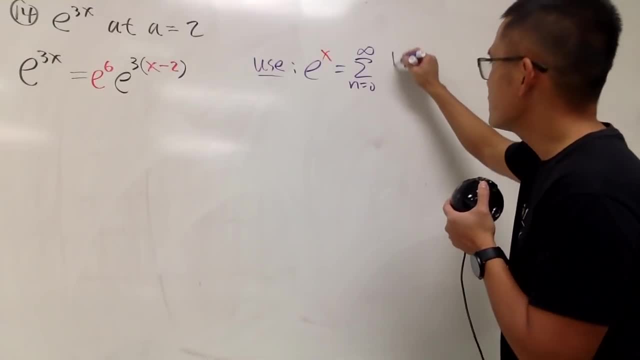 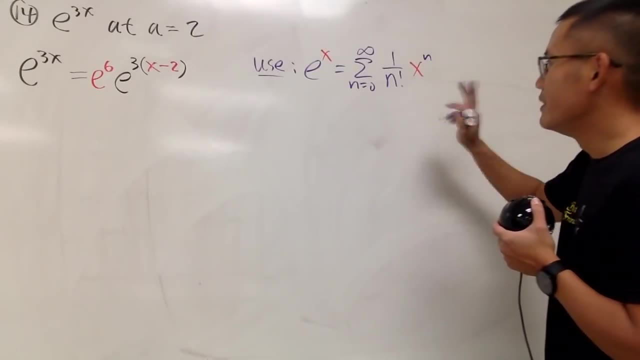 as n goes from 0 to infinity, And again you just have to make sure that you have the same one. So remember this: 1 over n, factorial. Better yet, you can just derive it real quickly, right? Anyway, x to the nth power, This right here works. And because r is infinity, so 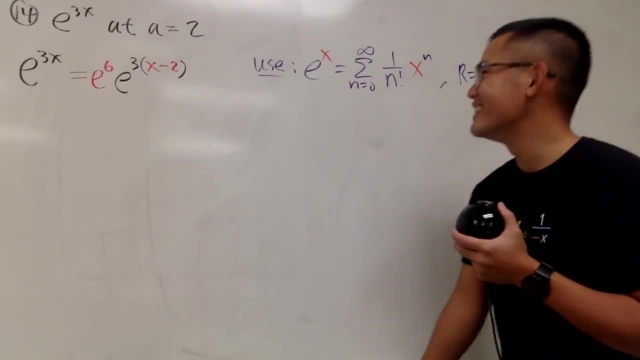 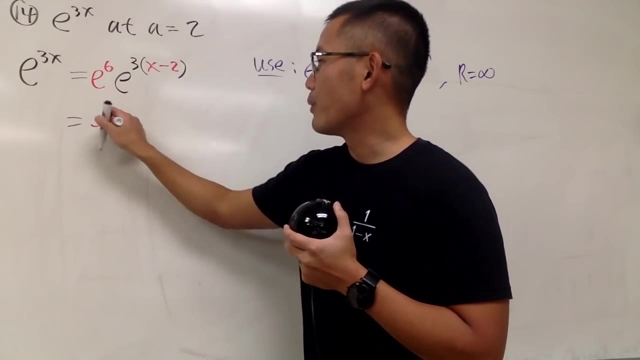 no worry, no whatever. You don't need the absolute value, you don't even need that. All right, So here we go. This, right here we have e to the 6th power. That's great. This, right here, we'll be using that. 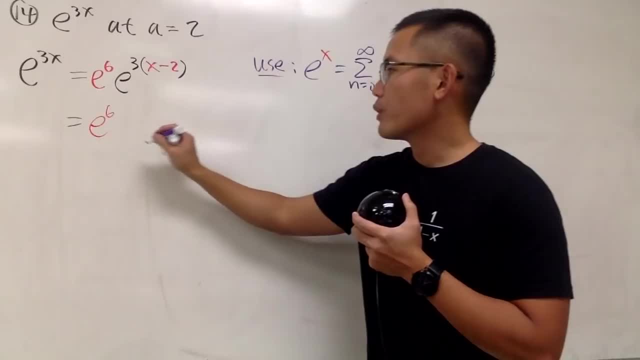 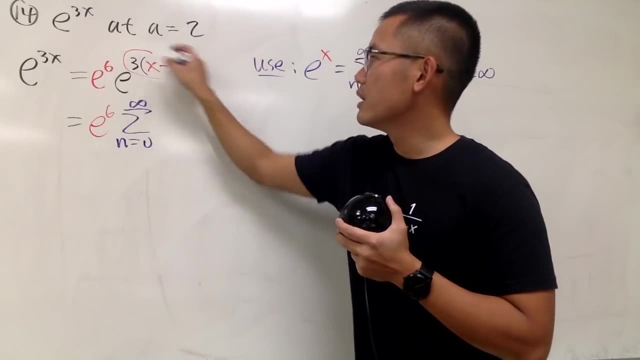 So, Alright, do is, of course, we have the sum n goes from 0 to infinity, and all we have to do is put everything in here, right? That's how we get that, that's the idea, and then just put everything. 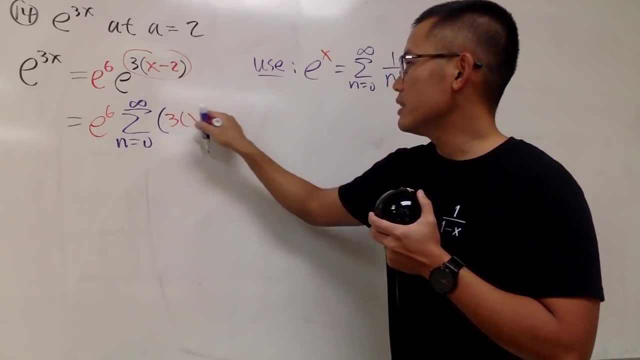 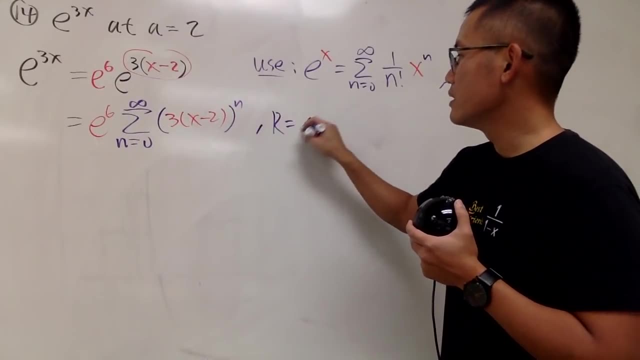 here. So open the parentheses with 3, parentheses x minus 2, and then raise n's power like this: That's it, And then the best part is: r is infinity and i is negative infinity to infinity. so you don't have to worry about the endpoints, There's no endpoints anyway. 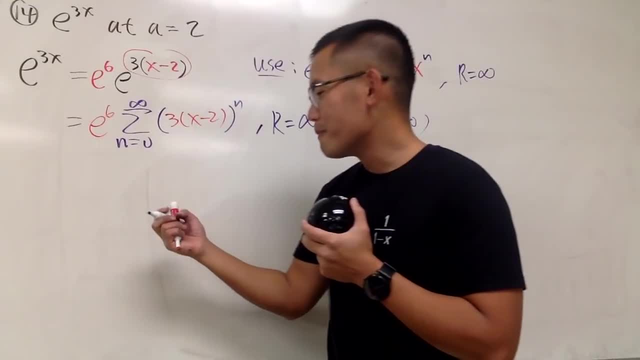 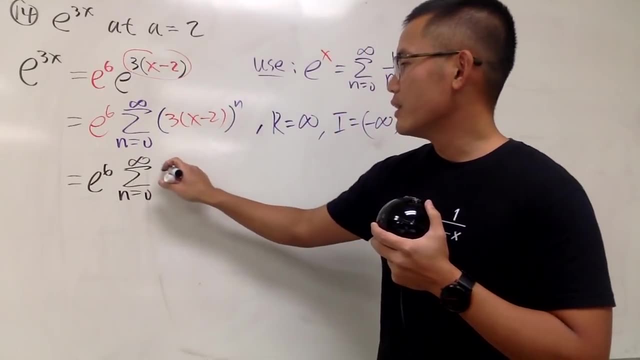 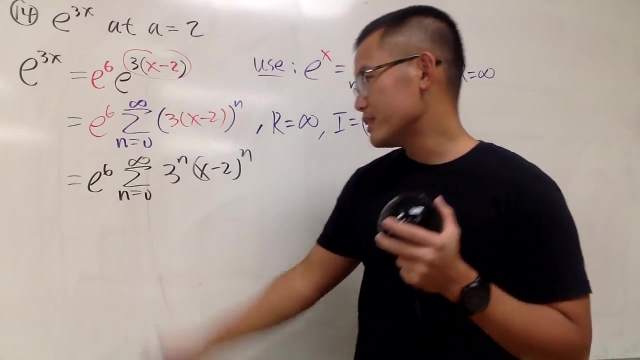 All right, we'll still kind of simplify this a little bit, though. So this is e to the 6th power and this is the sum, as n goes from 0 to infinity. Let's write this as 3 to the n, and this is x minus 2 to the nth power. multiply in, but there's nothing we can combine. 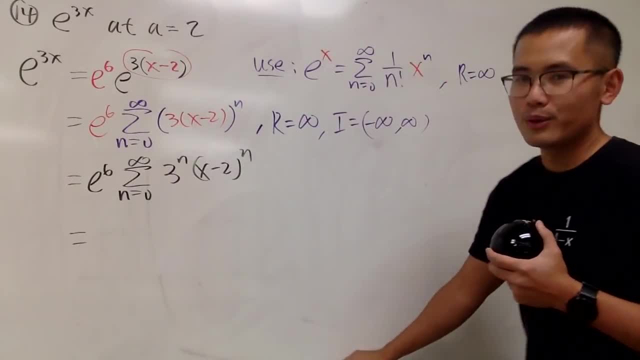 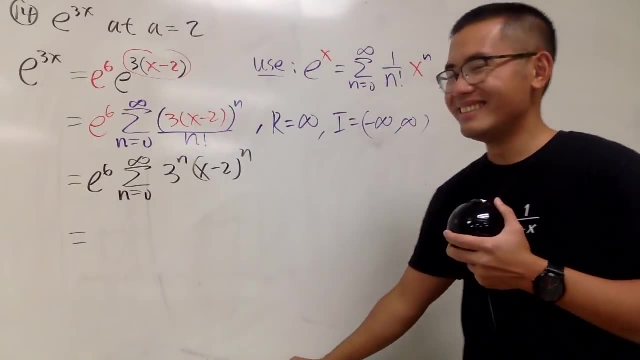 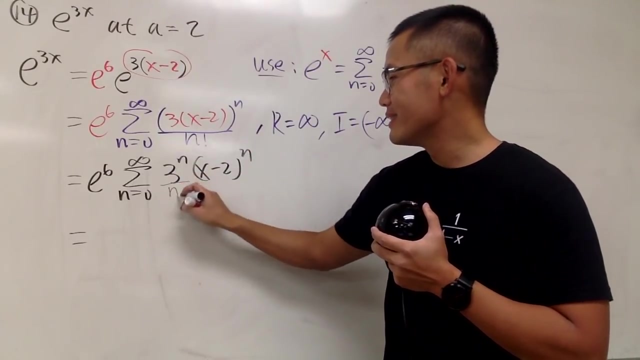 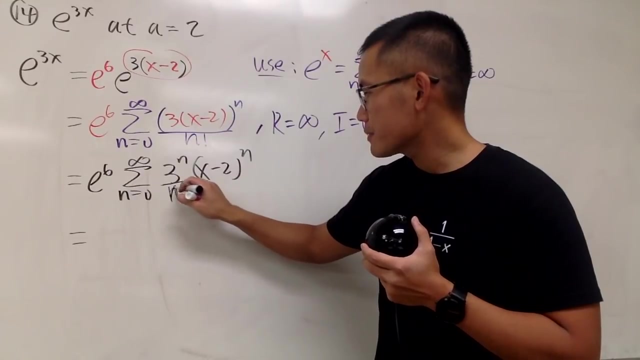 so I will just write this as: oh, I forgot the over factorial, my bad, I put this in here, but I forgot to write it as the over n factorial, my bad. All right, so 3 to the n and this to the n, and then over n factorial right, And finally, we are just going to multiply. 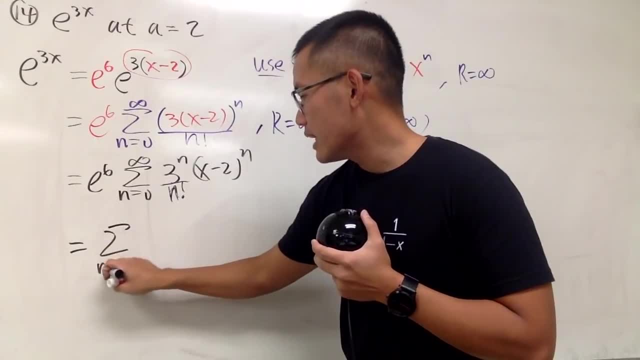 this in. So we end up with the series, as n goes from 0 to infinity and depends on how you want to write it. I will write it as e to the 6th power, times 3 to the nth power. So that's it. 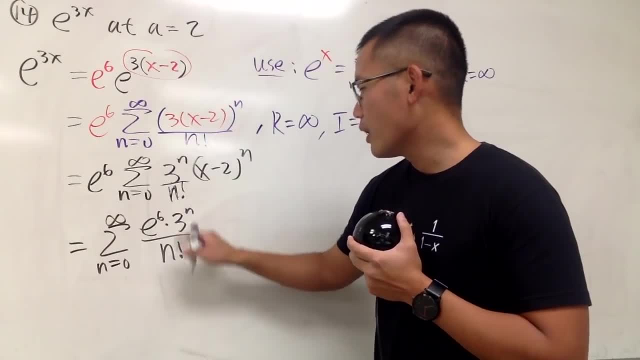 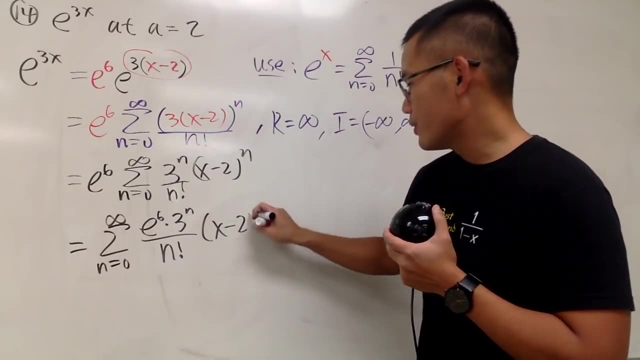 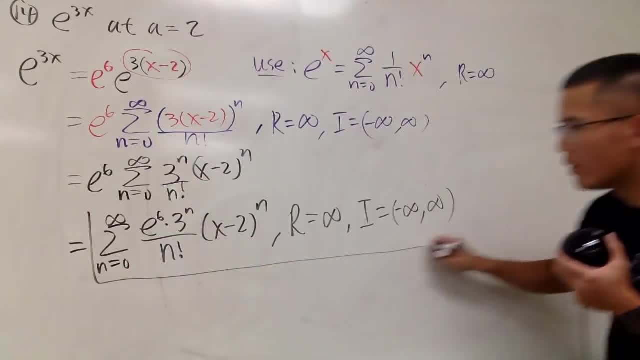 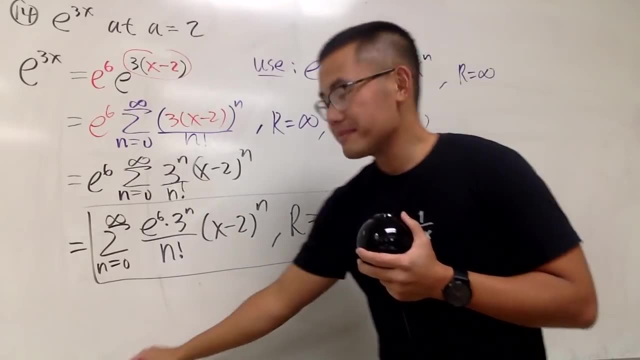 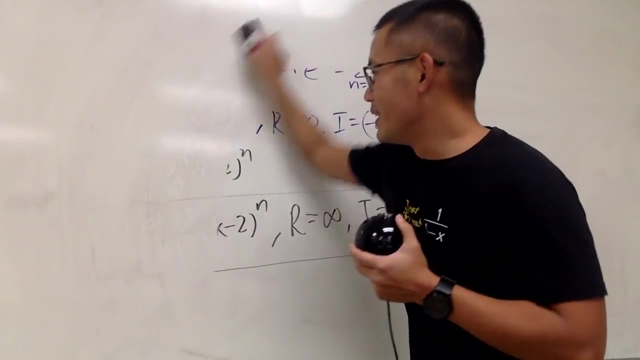 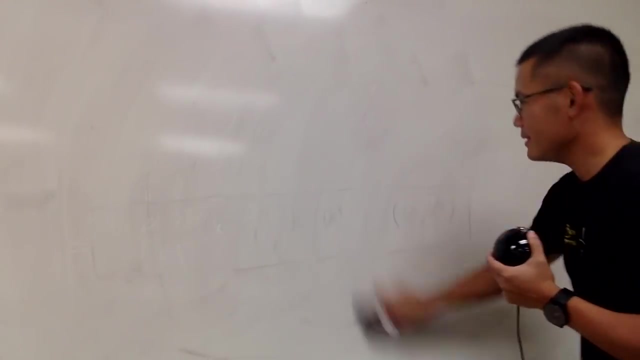 to positive infinity and we are all done Like this right. Very nice, huh Realize that. So I have to erase this every single time because I just want it to be clear. so I have to write it pretty big and all that, And hopefully the board is not so dirty. 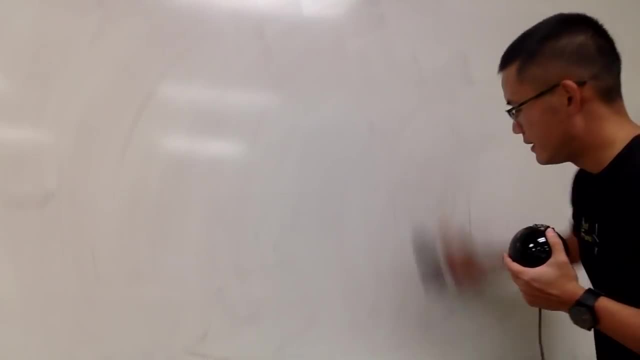 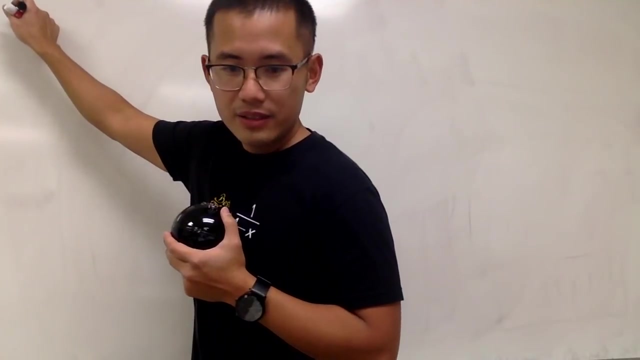 It looks okay right here, right, And let me know if you get a study for your calculus too, Midterm or final whatsoever, right? So anyway, number 15.. Mile 15, man, Let me tell you, You guys don't know how it works. 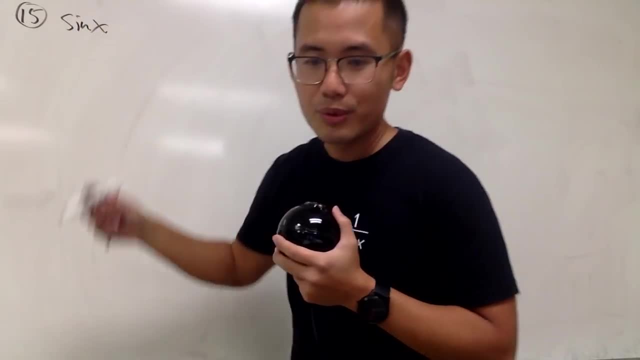 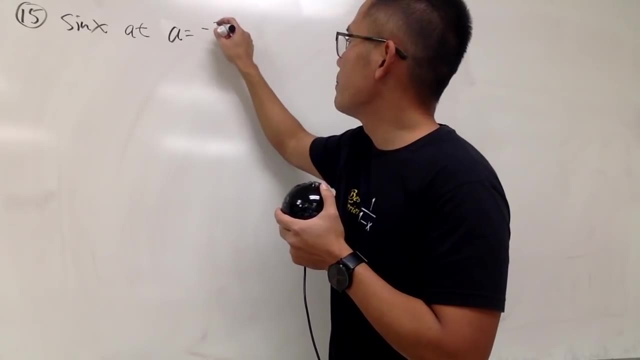 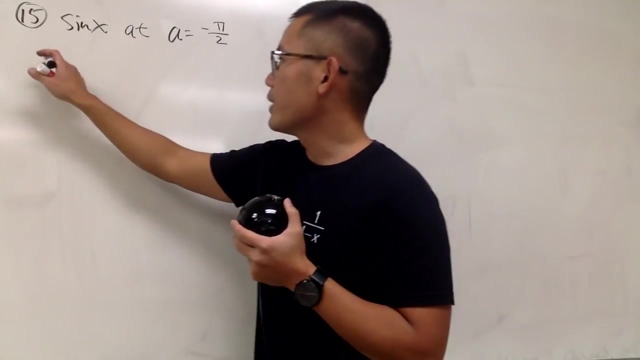 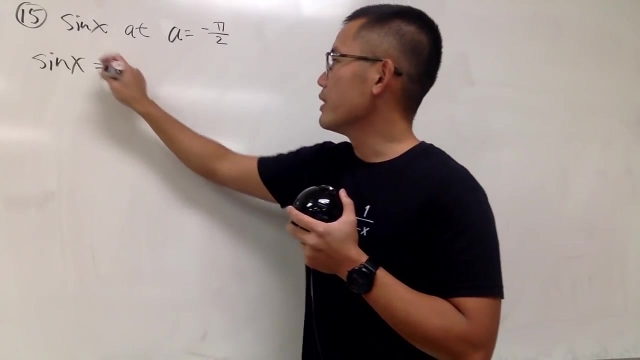 I should seriously just shut my mouth and just do the work. sine x at a being negative pi over 2, like that, Okay, Okay. so here we go. Sine x, and again, this is the most important part, Whenever you're looking at. I forgot to write this down. 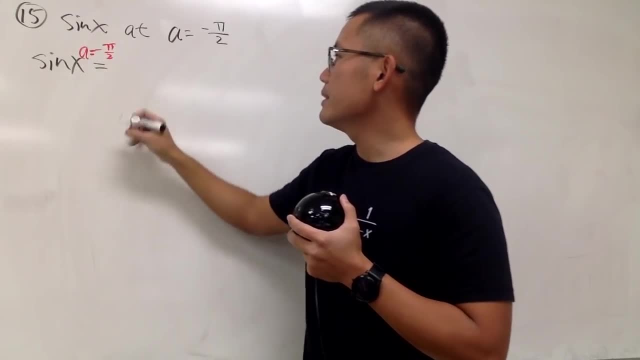 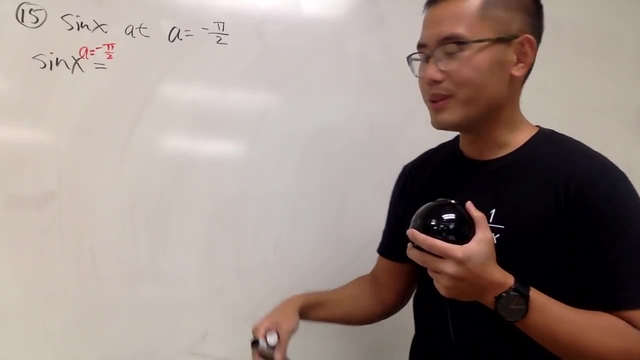 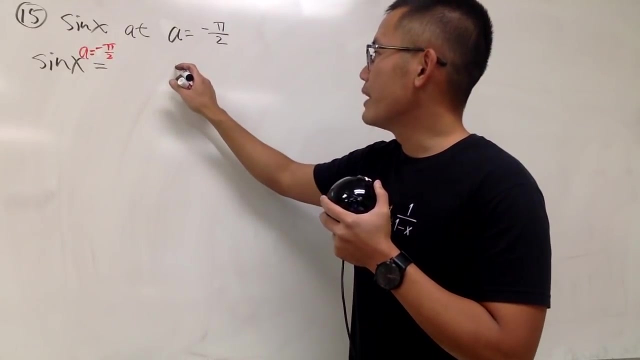 a is negative, pi over 2.. I forgot to write it down earlier, but it's easier. Okay, whenever you have the a- anything besides 0, be sure you write it as x minus the a, which is going to be plus in this case. 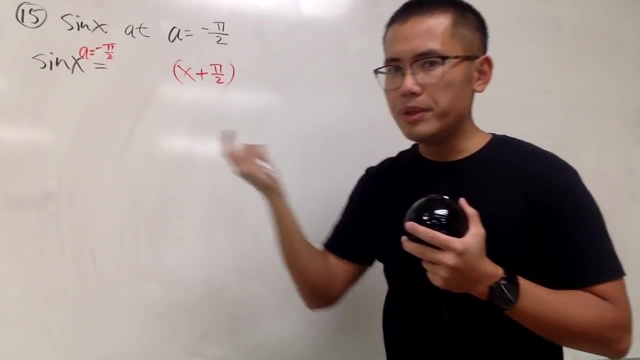 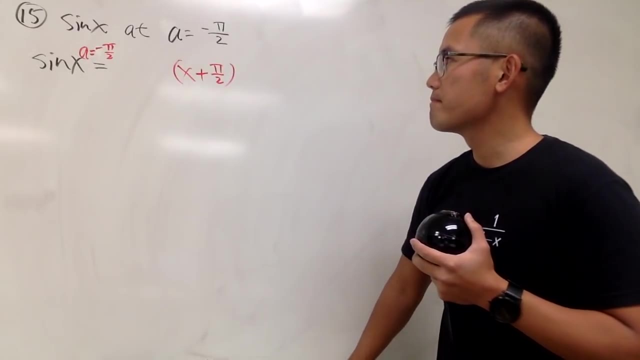 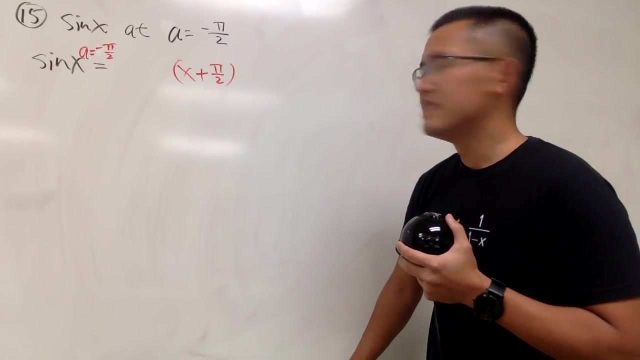 and the pi over 2.. So this will be your new input that you want so that you can use the other things to help you out. Okay, But we have the sine at pi over 2.. Wait, My bad. Sine of pi over 2.. 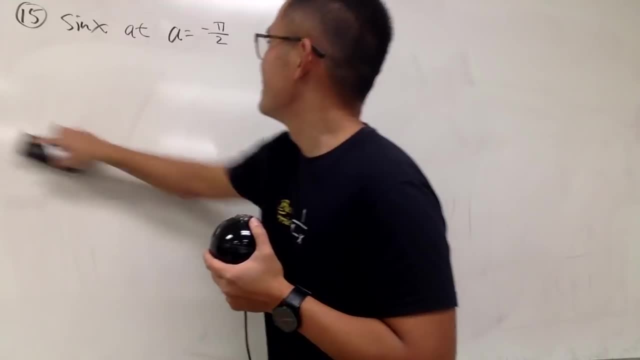 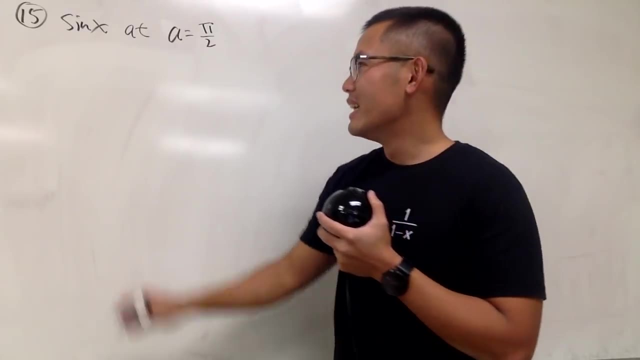 I have plenty of sine of pi over 2.. So so, so let me do it again. All right, Sine at a equals pi over 2.. All right, here we go. Question number 15.. Okay, so here we go. 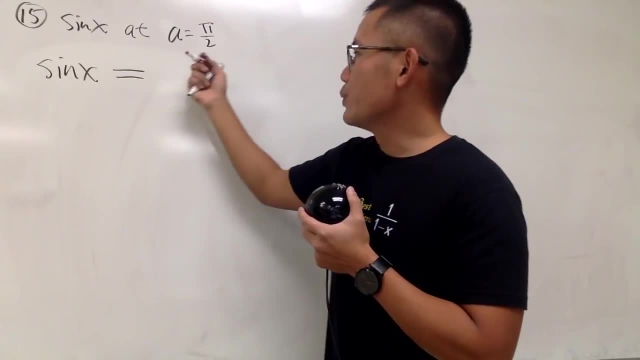 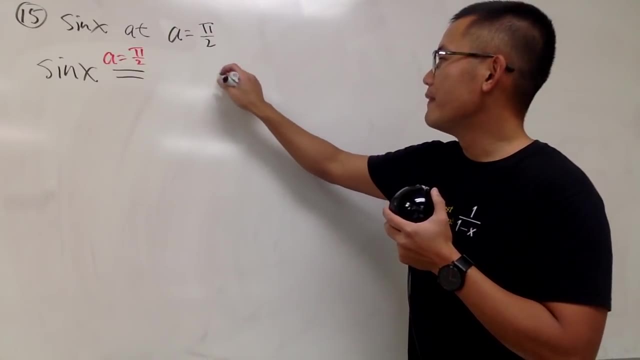 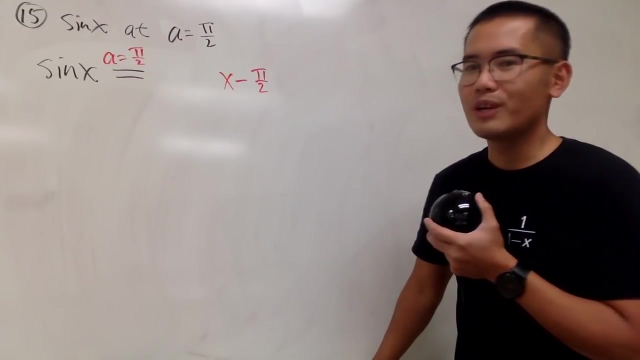 This is sine x. Well, in this case we want the a to be at pi over 2.. This means we want to have a factor x minus pi over 2. And hopefully we can build up some connections between whatever. Now here's the deal. 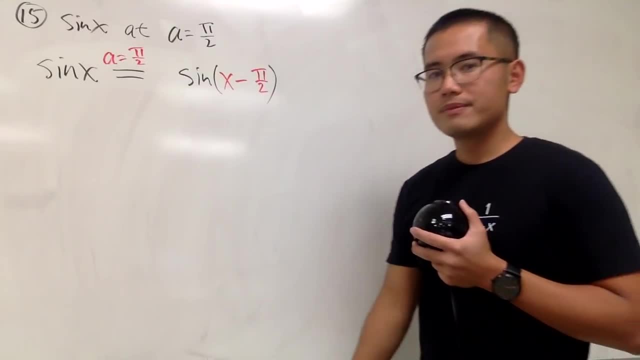 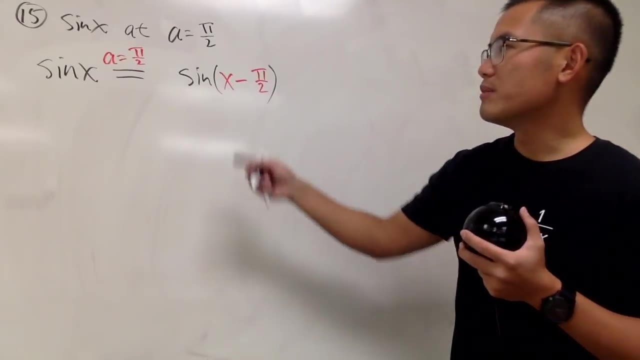 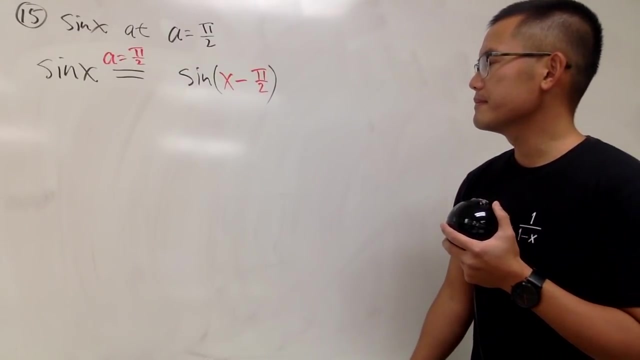 Can I just put in the sine right here. Is this true? No, unfortunately not. Yeah, Sine x is of course not the same as sine of x minus pi over 2.. Unfortunately, this is not correct. What can we do, though? 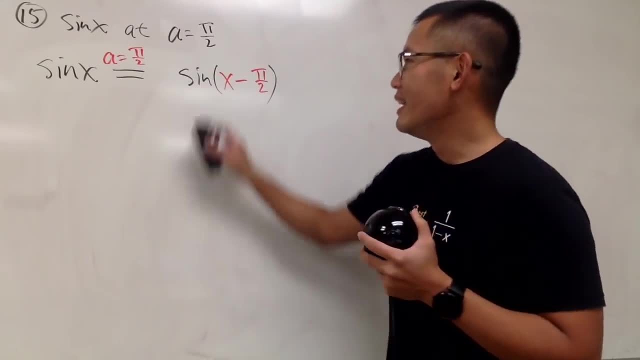 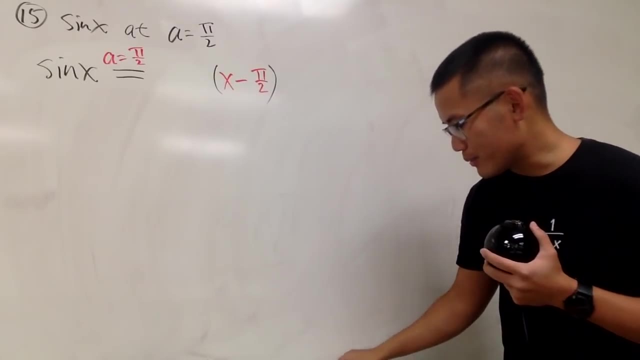 Well, don't worry, If you cannot use sine, maybe cosine will help us out. And the truth is, cosine can really help us out, And let me just write this down right here for you guys. okay, So it's just hard to see how to use the identities in order to help us out. 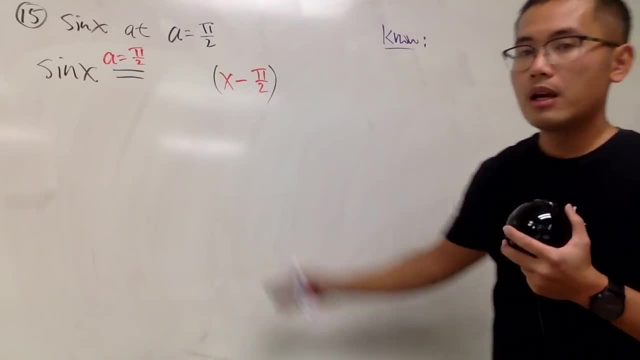 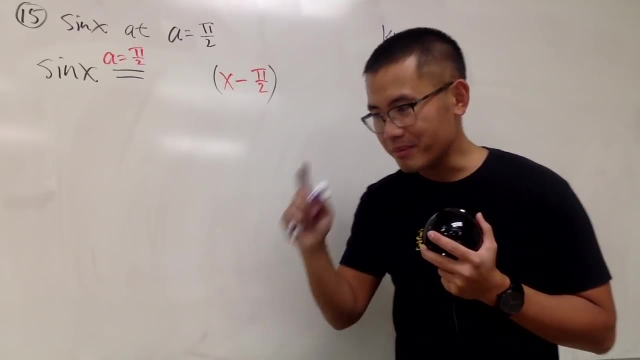 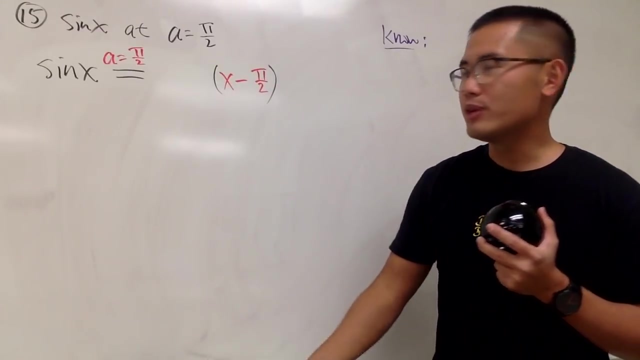 So I will just put this down right here. If you're looking at pi over 2, well, because sine and cosine, the cos stands for cosine, The cos stands for complementary. If you have sine of the angle, well, cosine of the complementary angle of that x is the same as cosine. 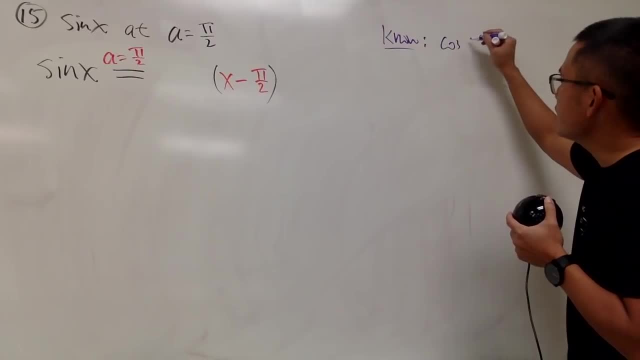 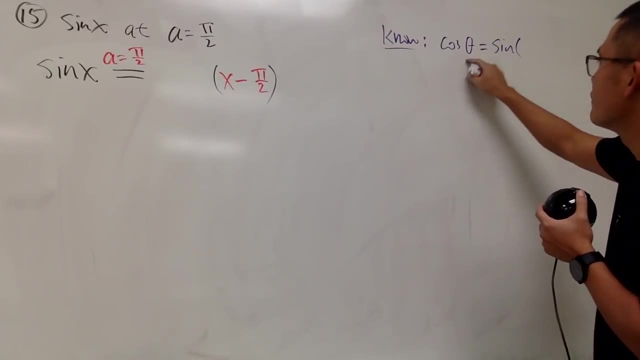 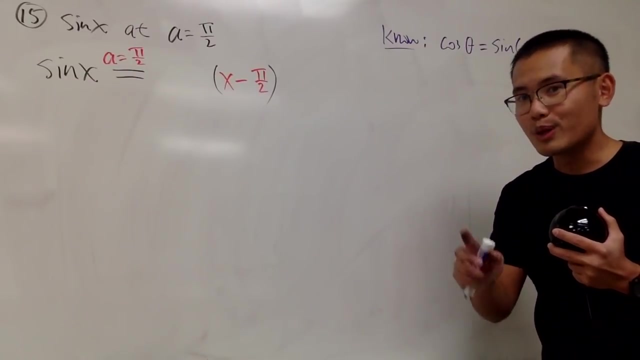 Let me write it down for me. So the idea is that cosine of theta- this right here- is the same as saying sine of the complementary angle of that. So remember: complementary means that two angles add up to be 90 degrees. But we are all adults now, so we have to use pi over 2.. 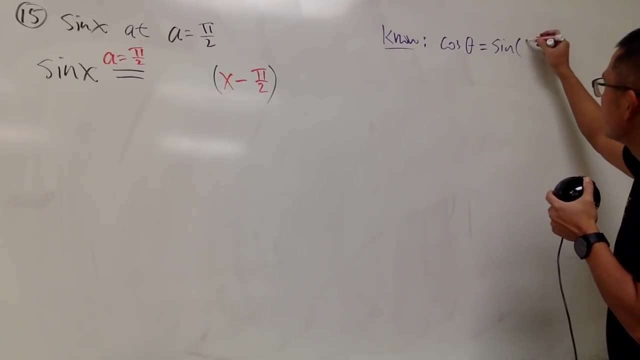 Well, this is theta already. That means the input. right here I would need to have pi over 2 minus theta. So this is the connection. Similarly, you can also write it as: sine theta equals cosine of pi over 2 minus theta. 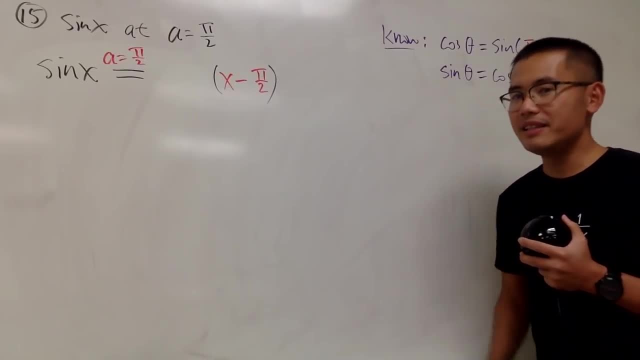 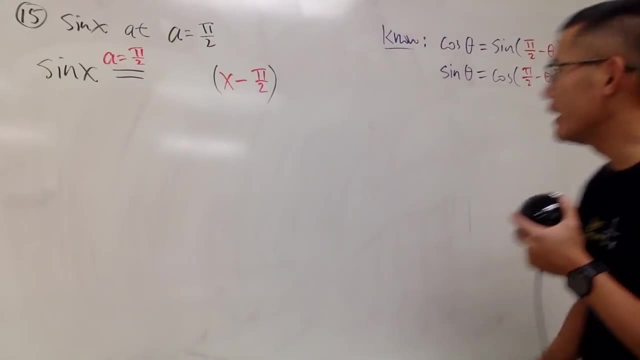 Like this. So this is the co-option, This is our identity. that will really help us out. Well, in this case, we are looking at sine, We're looking at sine theta, sine x over there. So it looks like we have the cosine to help us out. 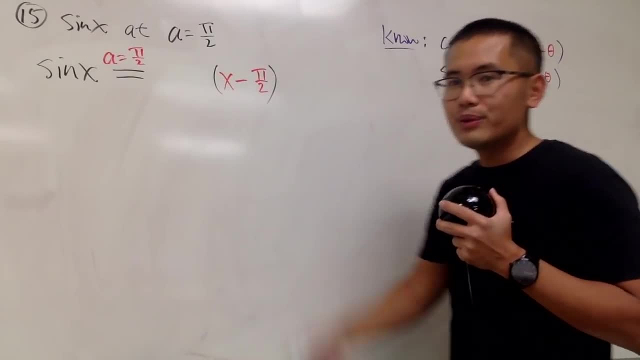 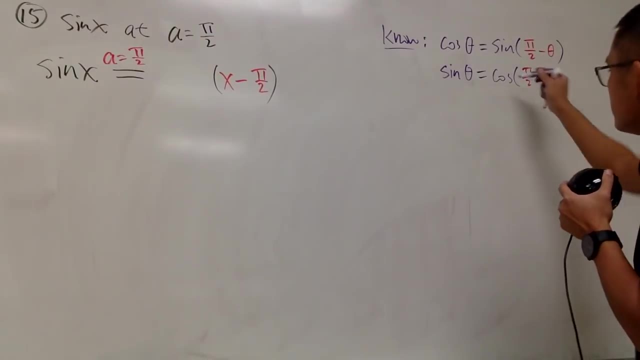 Well, I need to have a factor of x minus pi over 2.. By the definition, this is pi over 2 minus theta. Don't worry, This is cosine. This is all. This is actually really good Notice, So let's put on notice. 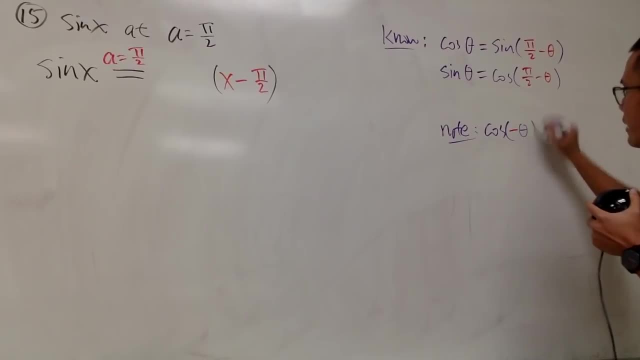 If we have cosine of negative angle, thanks to cosine being an even function, this is the same as saying cosine of theta. So what we can do is, in fact, this is the same as saying cosine of- we can switch this, and I'll just negate that. 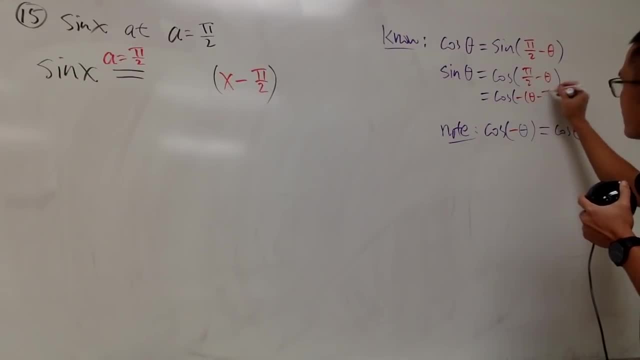 Negative, and I'll put this down first: theta minus pi over 2.. Right, I'll just do some algebra here, But this negative can be negative. This negative can be disappear because cosine is even So. we have cosine of theta minus pi over 2, like this: 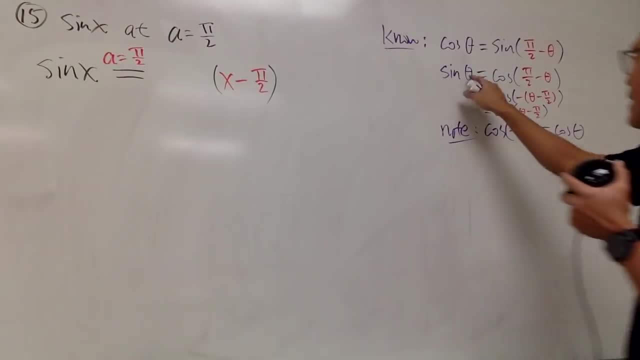 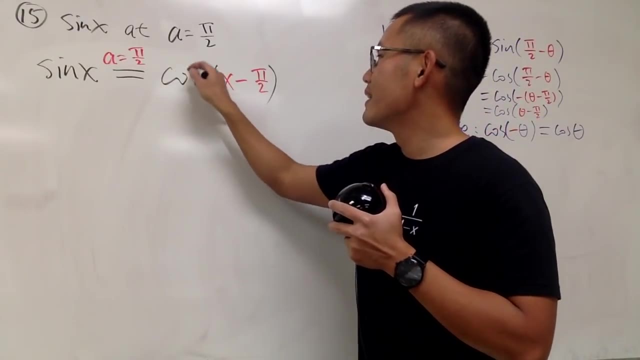 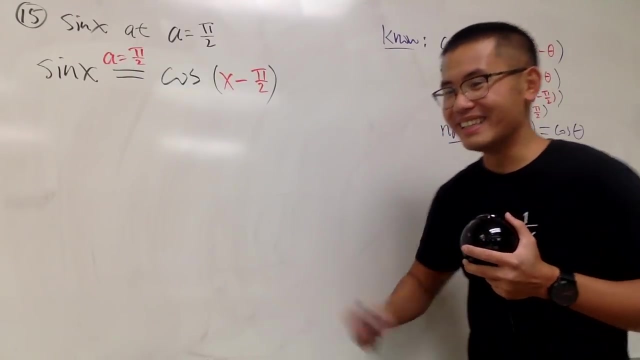 So sine x. of course I'm using theta, but the same as x. This right here is in fact the same as cosine of x minus pi over 2.. So this is very, very powerful. I will say Very, very convenient. 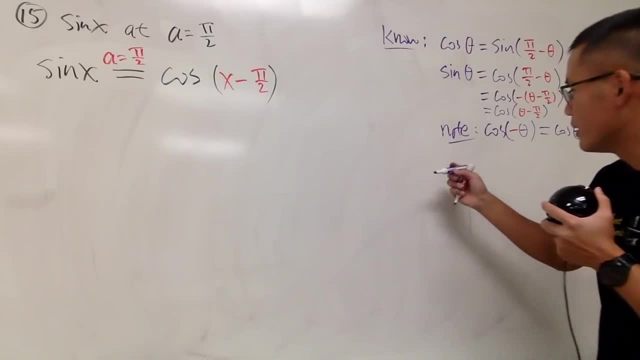 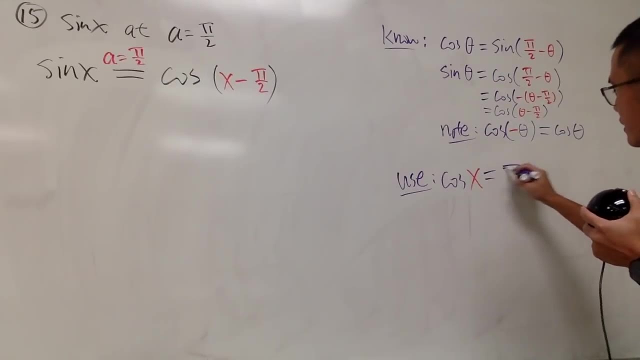 And now what we are going to do is, I will just tell you we can now use cosine of x as the power series, which we did earlier. the sum as n goes from 0 to infinity negative. 1 to the nth power over 2n factorial times x to the 2nth power, like this: 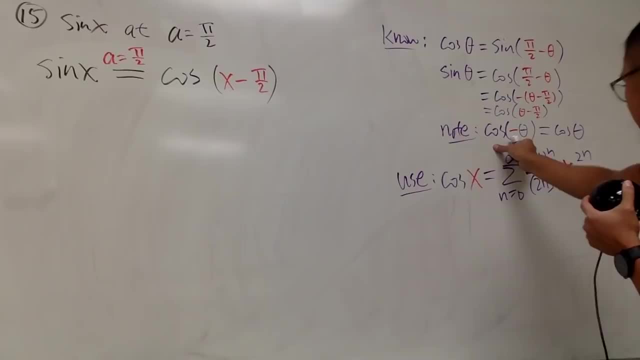 Right And notice that we mentioned that cosine is even and we have this property And you see that in fact we have the even power in the Taylor expansion or the power series expansion for cosine. That's why you know: even, even. 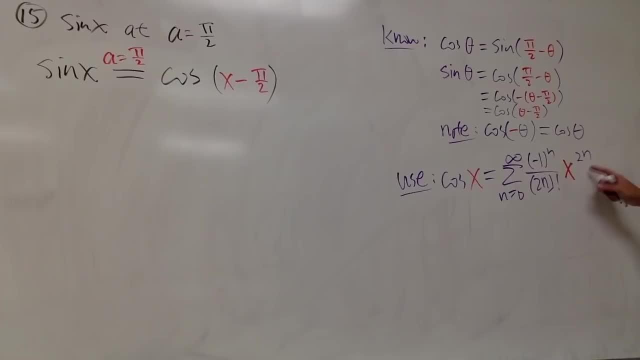 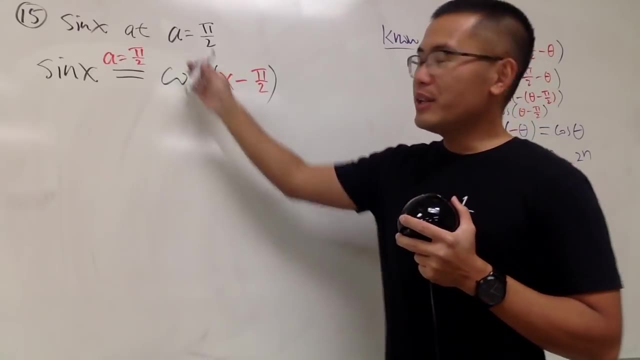 When you have an even function, you get an even exponent in the power series expansion- Very, very nice. So this right here we're almost done. Again, you can do a table, but sometimes using identity will be much quicker. So here we go. 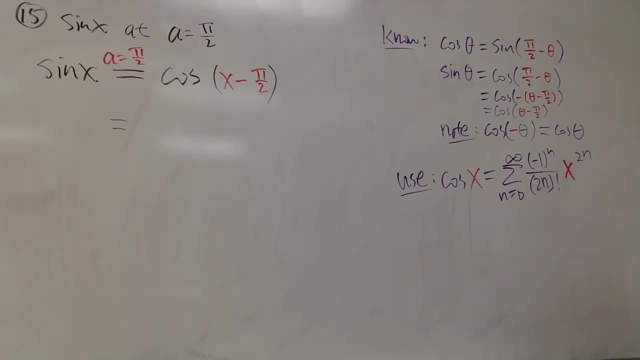 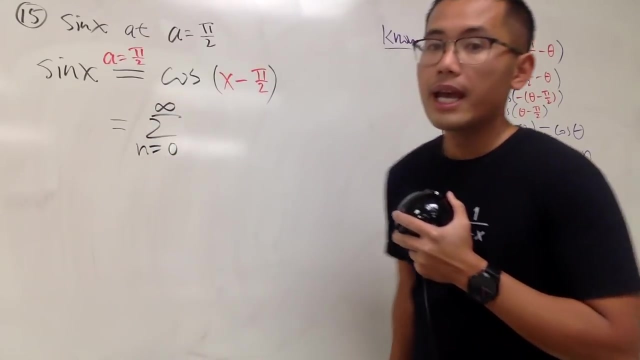 All we have to do is enter this here here, Right? And, by the way, you know that I will put this down here. I'll just write this down: r is infinity. Anyway, put this down here. so we have the sum. n goes from 0 to infinity. 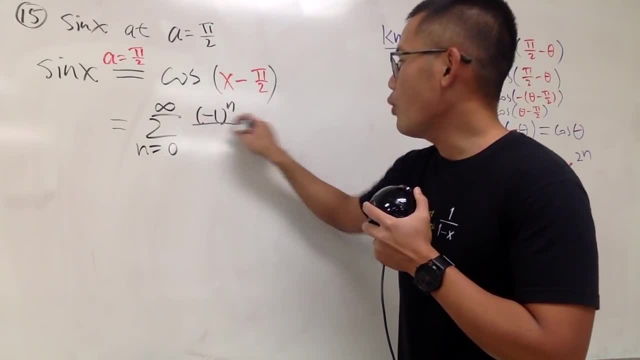 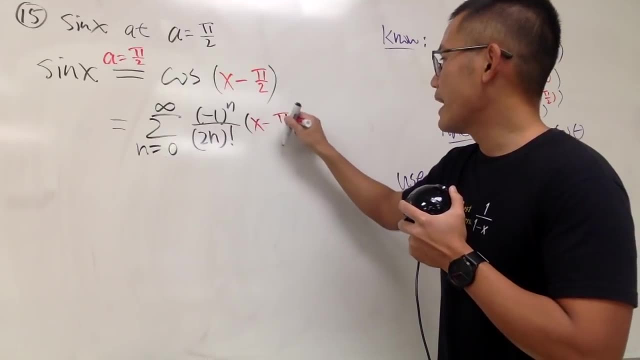 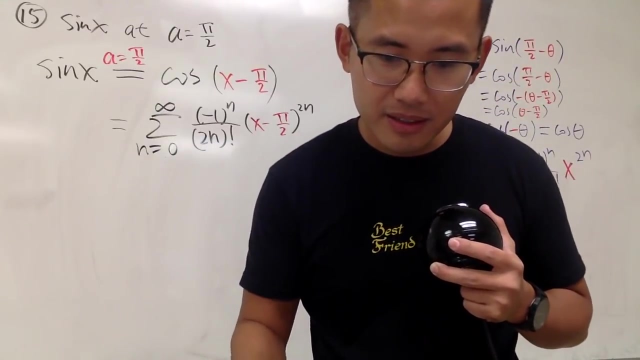 And we have the coefficient being negative, 1 to the nth power over 2n. parentheses, that factorial, that, And then here is just x minus pi over 2 raised to the 2nth power. Very, very clever Convenient, Isn't it? 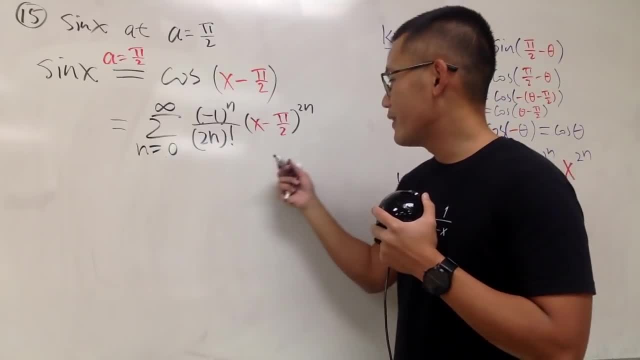 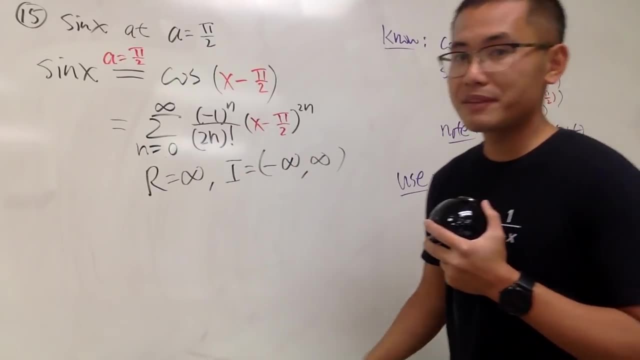 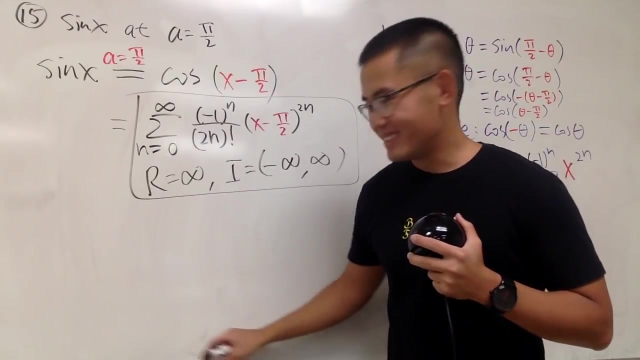 And that's it. That's it, And very quick. r is infinity. That means I will be automatically negative infinity to positive infinity. Done, Done, deal Right. The more we know, the easier our life will be sometimes. So that's the idea. 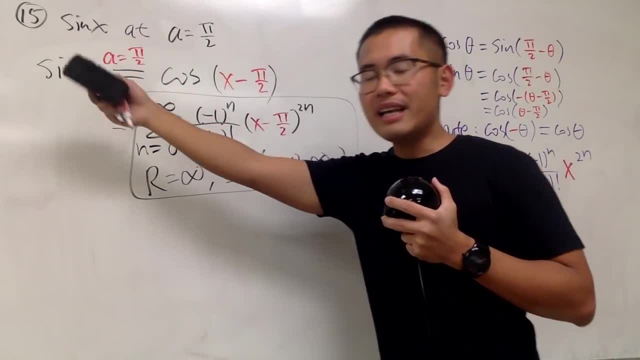 And I wrote this down just for you guys. Sometimes you might be looking for like cosine and like pi over 2, maybe this right here will be helpful, But you will have to use sine being an add function to fix that. 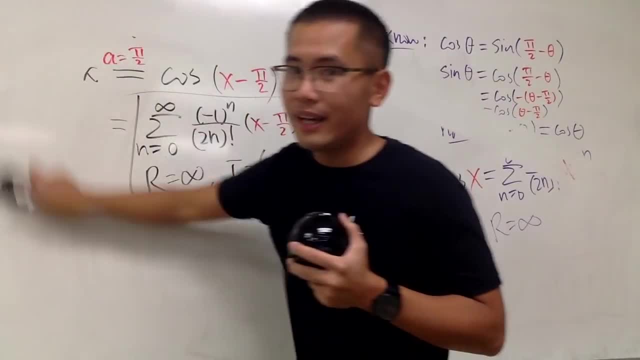 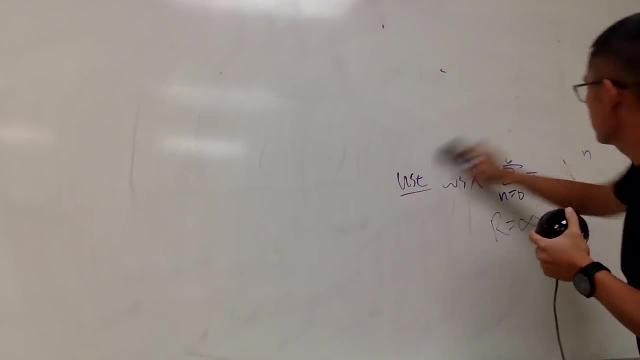 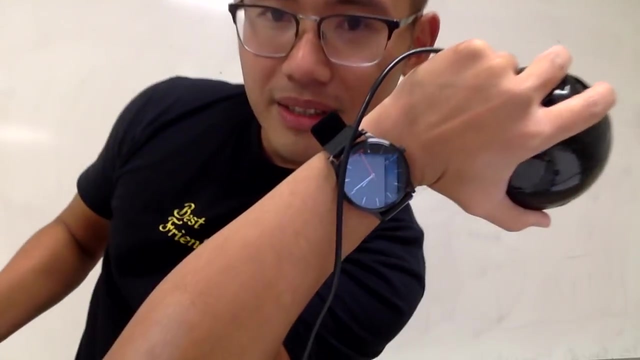 Okay, So that's number 15.. And man, this is exciting. We are kind of almost done. All right, Just to show you the time. okay, Right now is 8.45.. 8.45 pm. 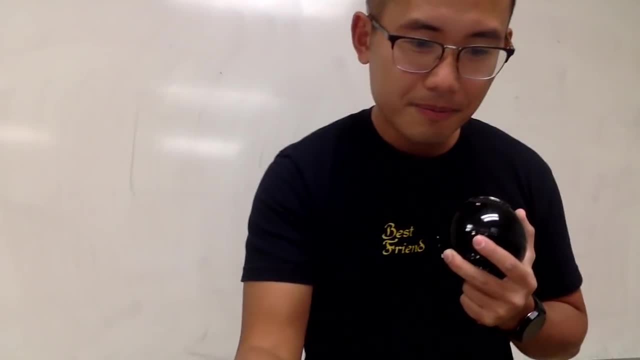 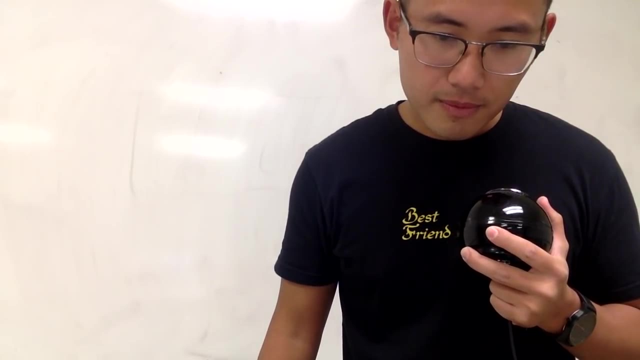 The date is wrong on my watch, So don't worry too much about that. All right, Next one. Oh yeah, Next one, Number 16.. I'm going to space out a little bit. Number 16.. Again, we are looking at sine of x. 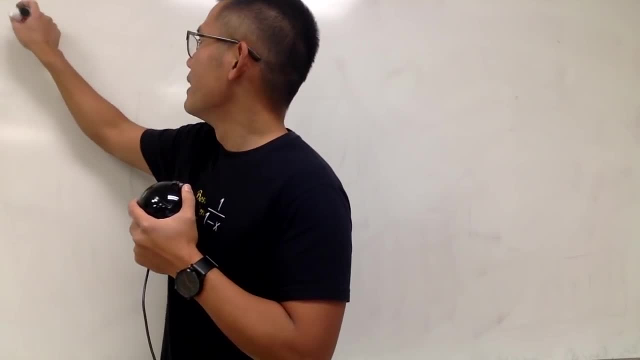 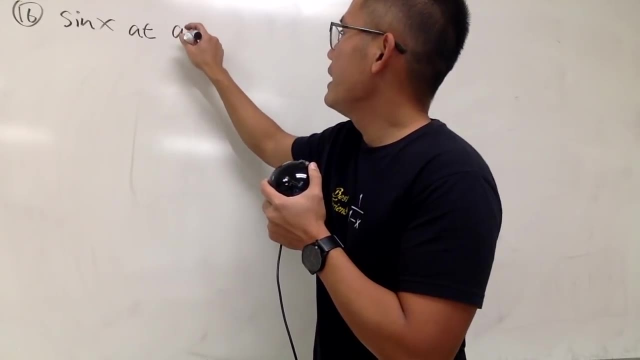 But this time at a equals negative pi Man, Negative pi. So you know the deal. We will be using identity right here again. So let me just put this down: We have sine of x, Hmm, Okay, All right, All right. 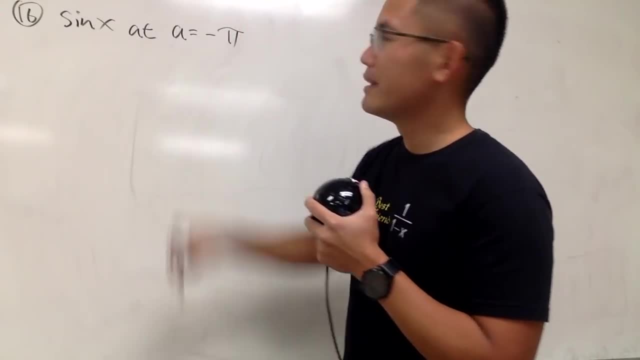 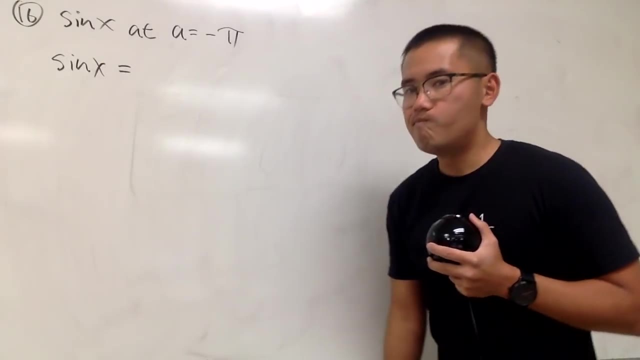 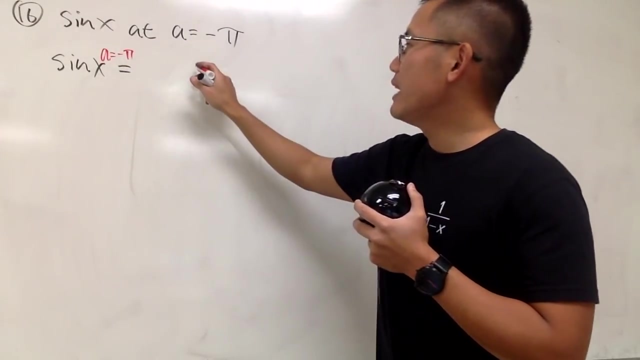 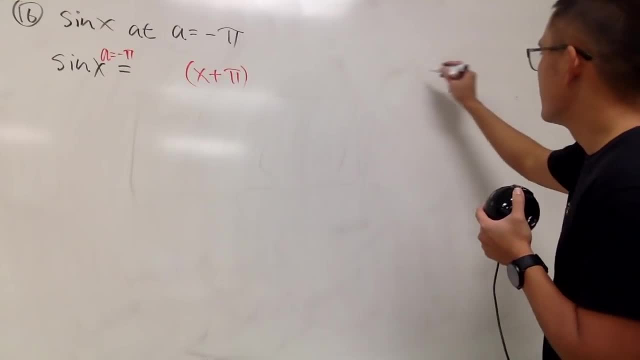 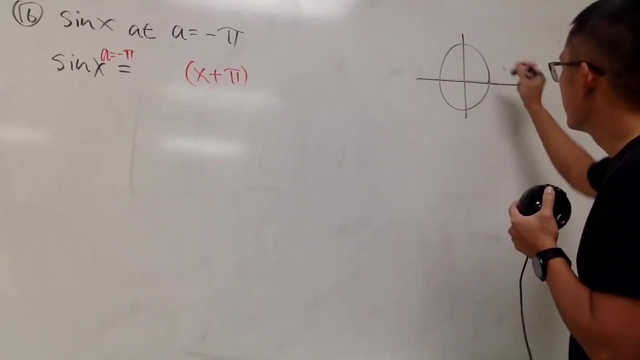 Okay. Hmm. Well, let's take a look right here. Let's say we are on the unit circle, Let's say we have the point right here, And, of course, remember the sine is the y value. This is right here. 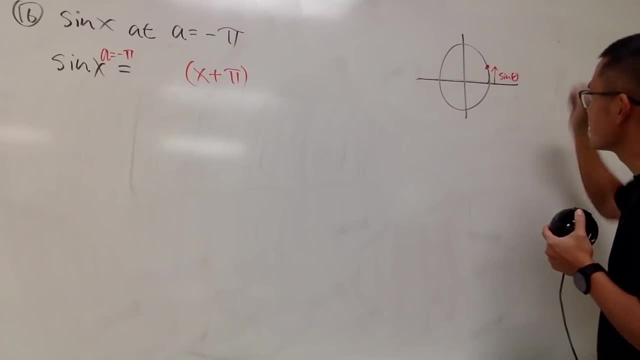 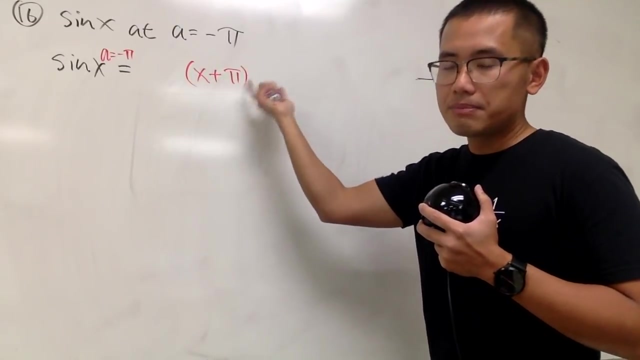 It's the sine value. Okay, So that's the sine of the angle, That's the sine of the angle theta. Well, if you have an angle x plus pi, that means you just go 180 degrees. So just phew, go, look right here, directly down here. 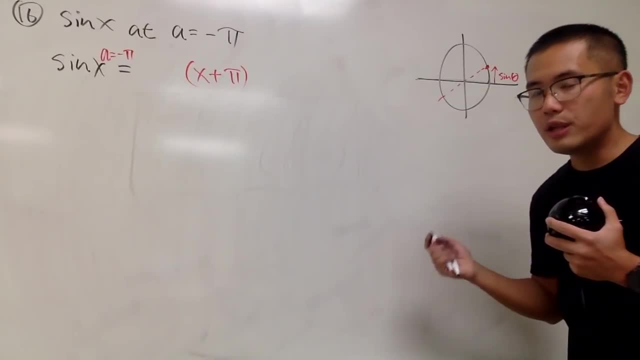 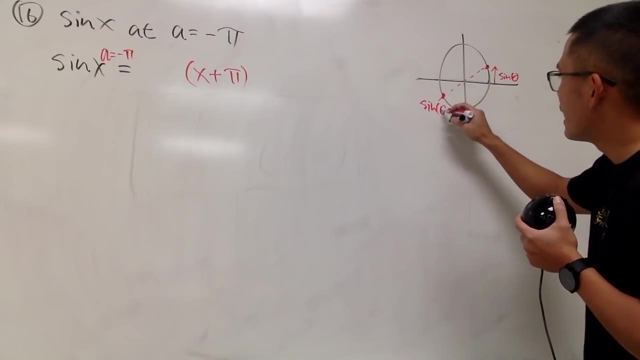 And this is actually a really nice reflection What this is. you just come here and this is going to be sine of pi plus so theta plus pi. But the problem is that it was positive and now it's negative, so you just have to negate that. 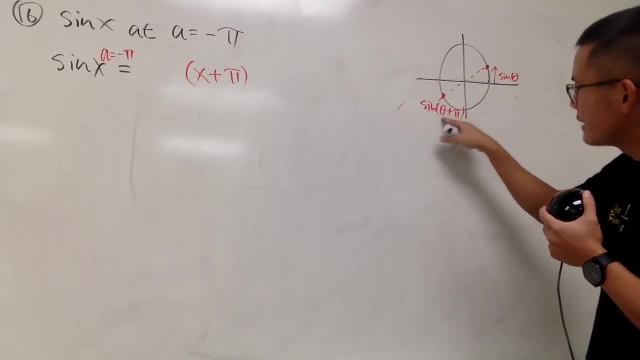 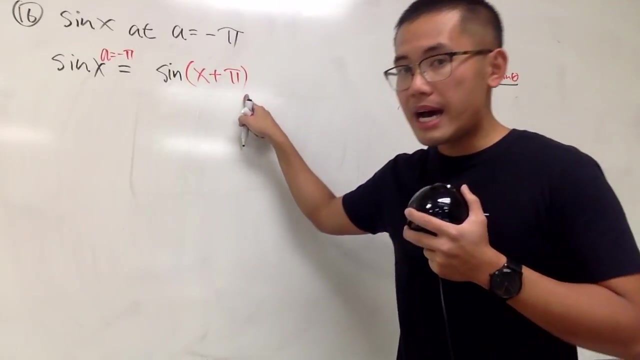 So this is the sine of π, this is the sine of θ plus π, But this is just going to be the negative value of that. That's it. Yeah, so very nice. sin is equal to sine of x plus π, but it's the negative. 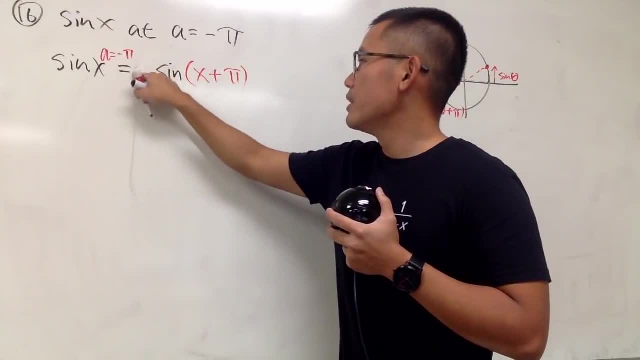 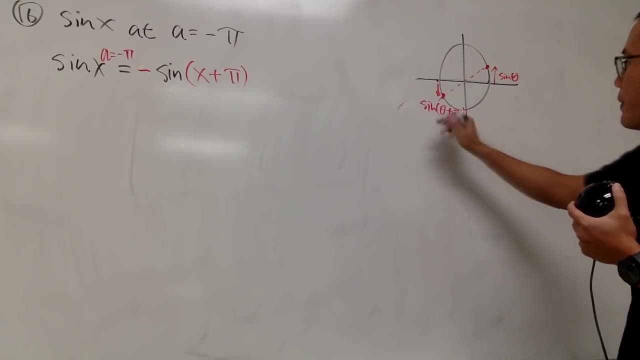 So it's a negative right here. let me just emphasize that it's a negative Why? Because again they have negative sine, And again this angle here is: I should put a negative here. why not? Yeah, if x is, let's say π over 3, and then you add π, yeah. 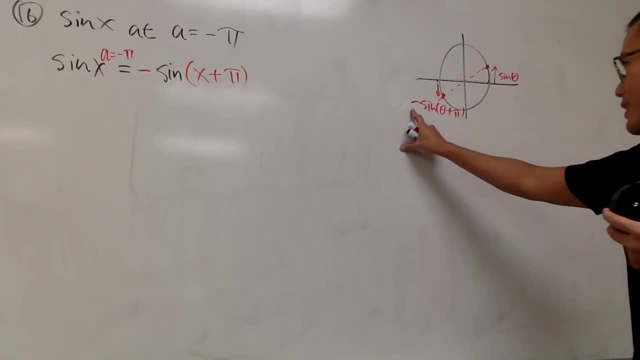 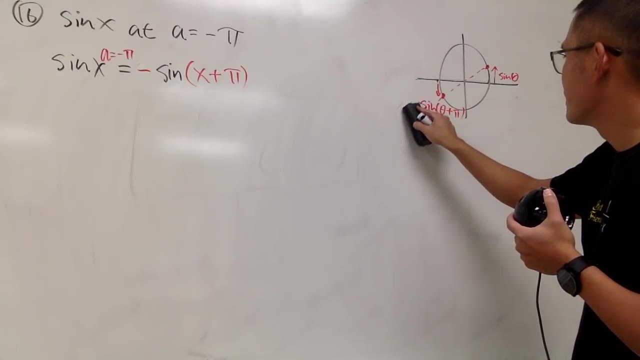 Yeah, the y-value is the same, but just opposite the sine For this picture. I'm not sure if I should put a negative there. I don't know if it does make sense or not, but No, No, no, no, no, no, no. what I mean is this right here? is this distance right? and that's the distance. 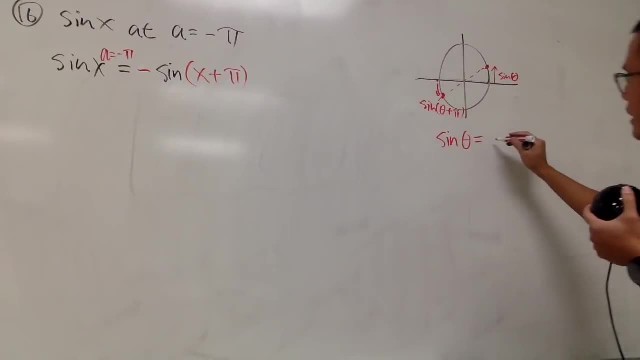 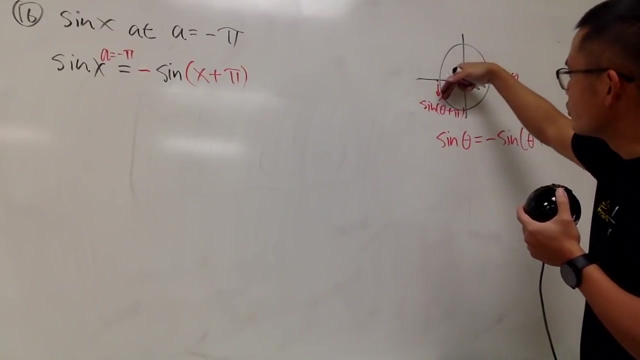 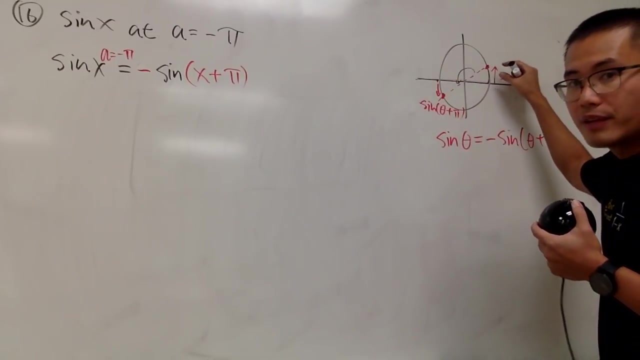 but the connection is: sine of θ is equal to negative sine of θ plus π. And again, what I mean by that is if you just go 180 degrees more, which is π radians, this distance, the y distance, is just the opposite of that. so that's why you have a negative right. so that's the idea. 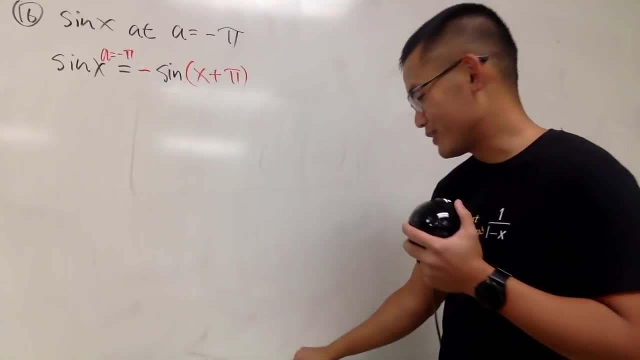 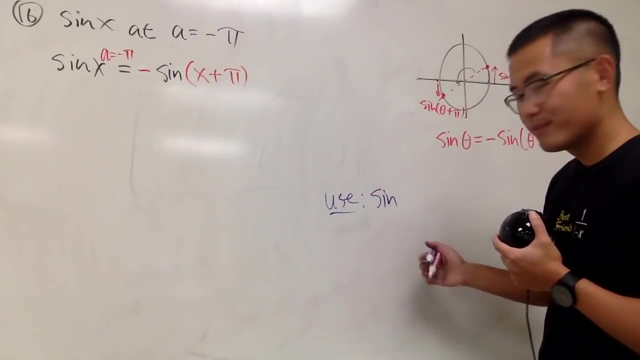 Okay, so that's what we have, Then, what we're going to use. I'll just write this down again. let's see if we remember this or not. We'll be using sine, of course. So we have sine of θ. well, let's use sine x, of course. 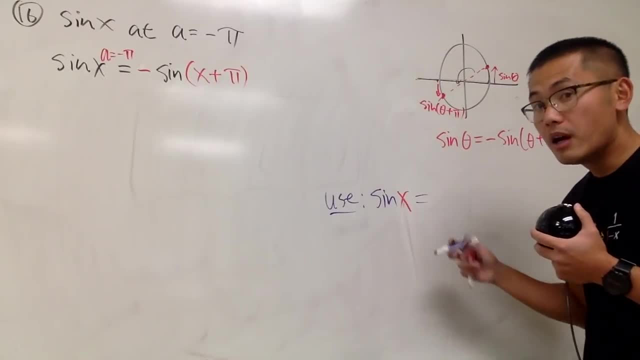 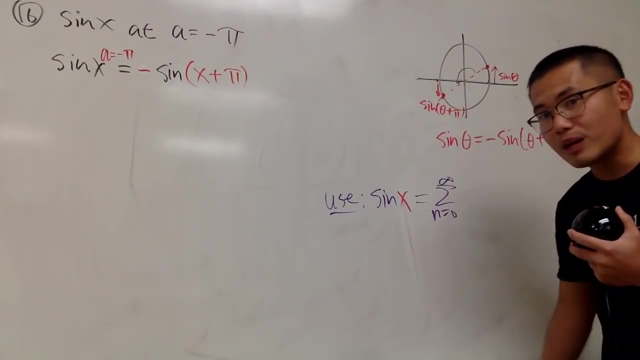 For identities, I like to use theta, of course. Alright, here we go, Because right here this is sine, so we're looking at sine. We have the sum, as n goes from 0 to infinity, and what do we have next? 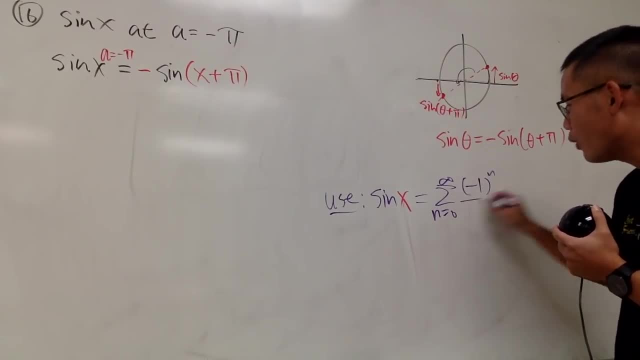 Yes, it's alternating negative. 1 to the nth power over sine is an odd function. so you see the odd numbers and it's 2n plus 1, good, And then factorial that x to the 2n plus 1th power and the radius of convergence is infinity. 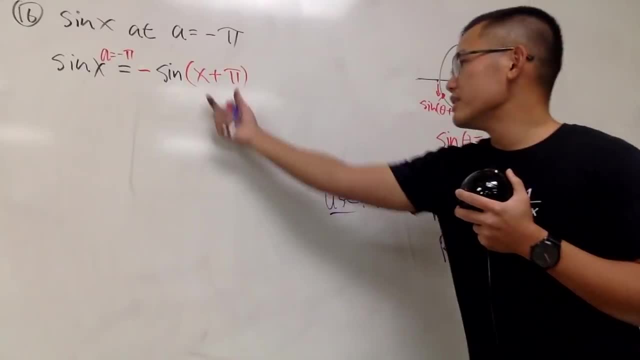 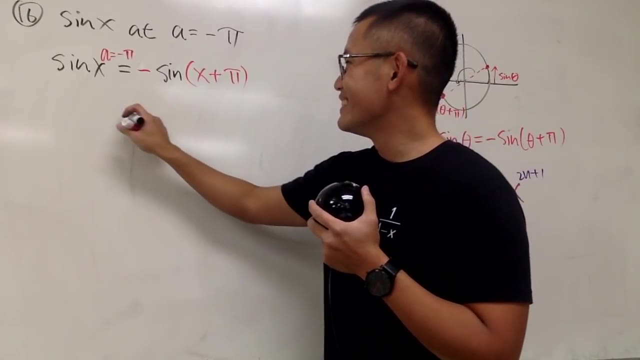 In this case. well, again, we just enter this right here and that's pretty much it. So we have this, This is negative and this is: This is going to be the sum, as n goes from 0 to infinity. 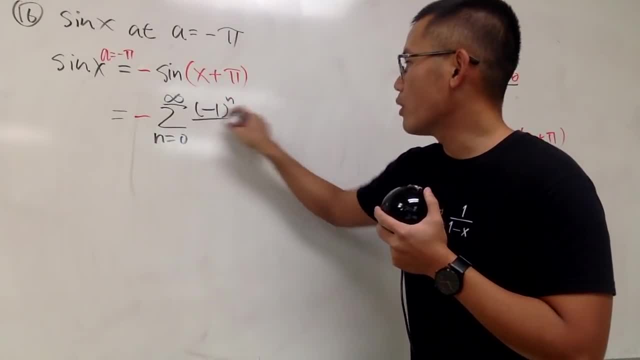 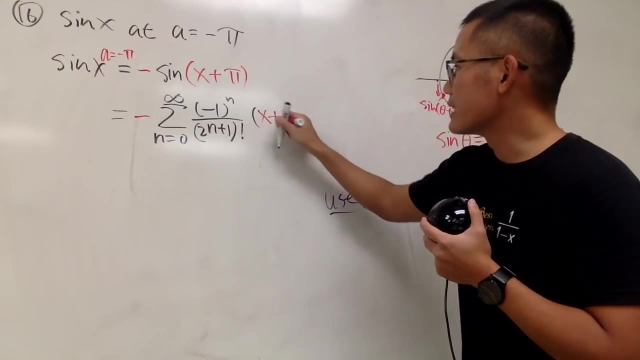 Just write this down: pretty much Negative 1 to the nth power over 2n plus 1, factorial this guy. and then enter this for the input x plus pi raised to the 2n plus 1th power, like so: 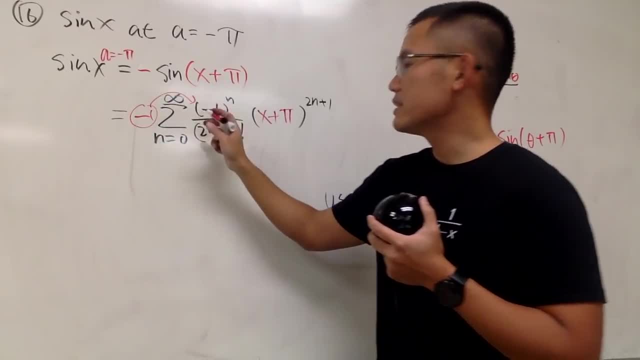 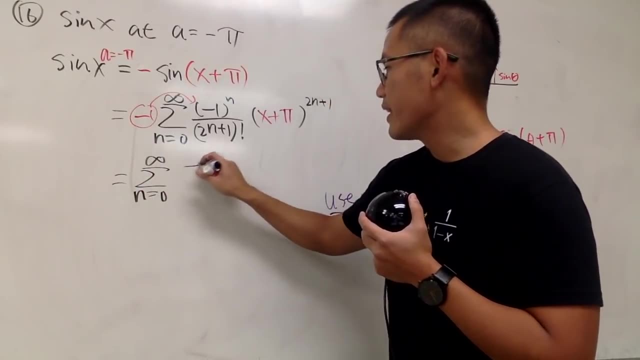 And if you would like, you can just say this is negative 1,. multiply with this negative 1 to the nth power. so finally you can simplify this to be: the series n goes from 0 to infinity. negative 1 to the nth plus 1th power over 2n plus 1, factorial that. 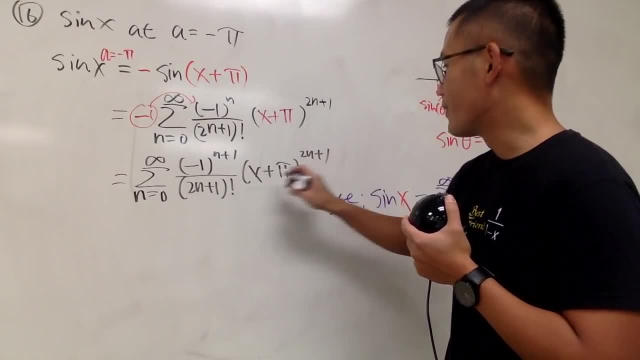 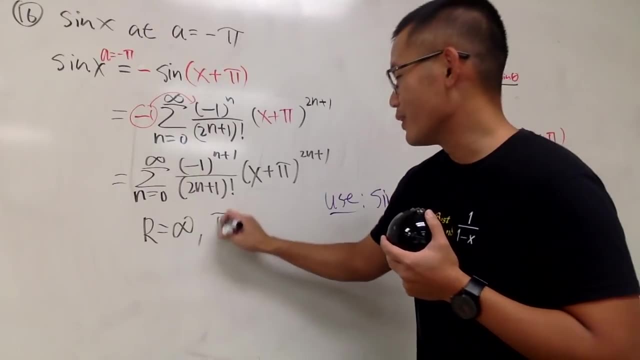 Man, I know it's like it's not so bad, but it's just hard to write the same thing over and over. It's worse than integral sometimes, right? Anyway, r is infinity because you're just plugging, and of course still, i is negative infinity to positive infinity. 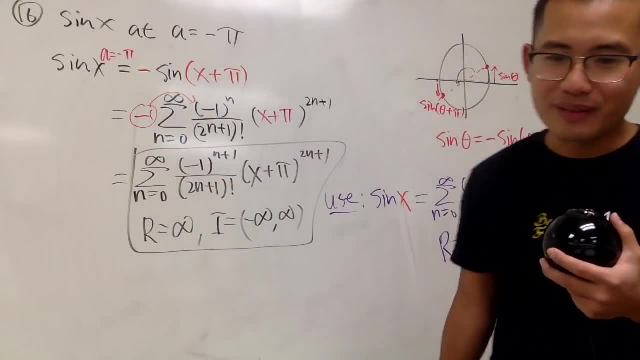 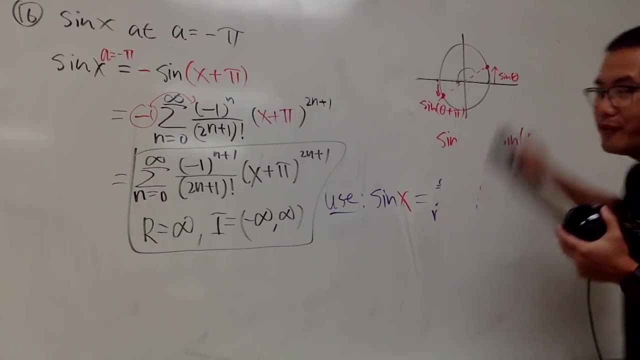 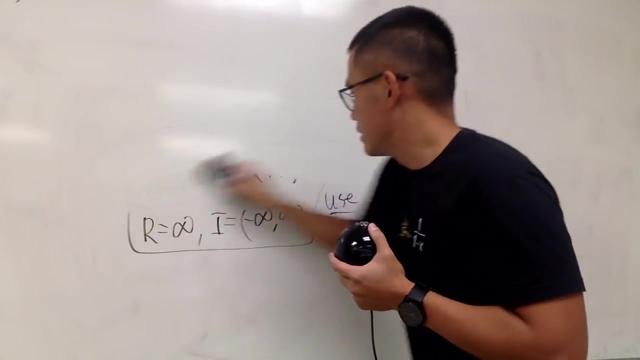 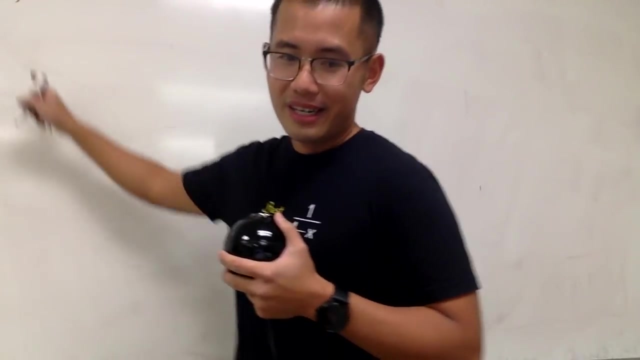 Pretty nice, huh, This is not boxed, but whatever Got it. yeah, Okay, so far, so good. Oh my god. next we have the sine squared. Oh my god, man, this is number 17.. Man who chose all these questions? 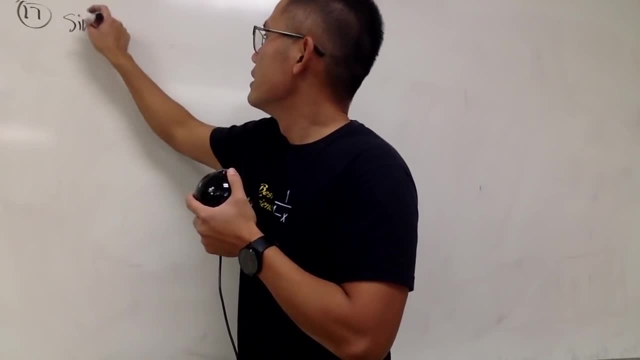 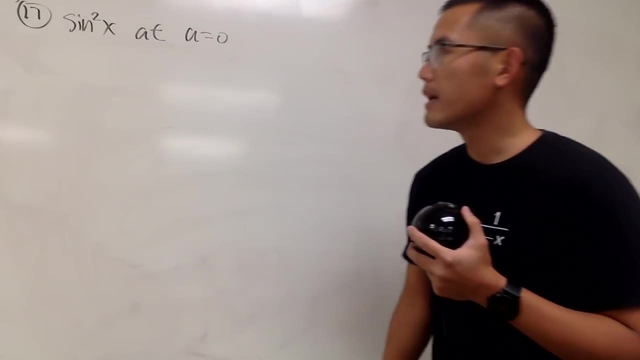 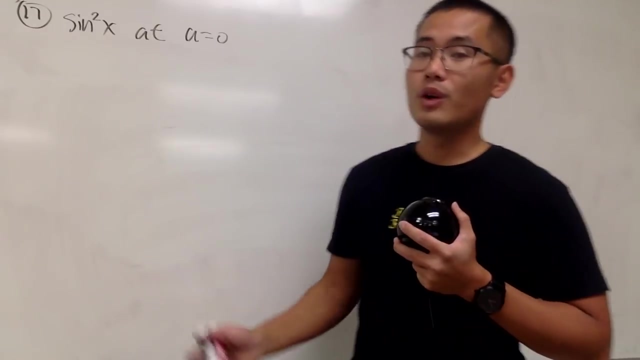 Yes, that person is me. Okay, sine squared Square x at a is equal to 0.. Remember integrals? how do you integrate sine squared? Yes, we should use the power reduction, So in here we do the same as well. 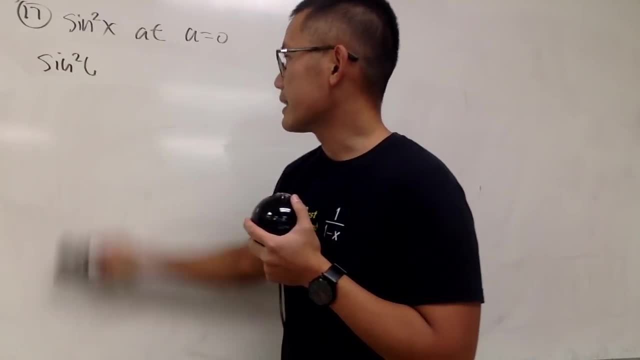 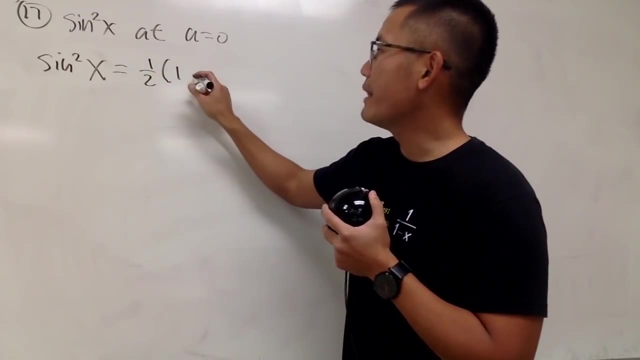 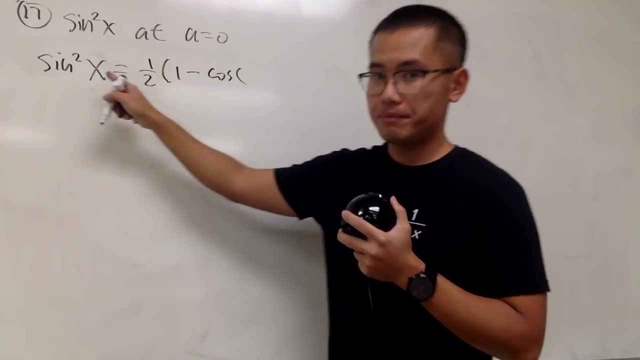 So here we go. Sine squared x. This right here is the same as 1 half times 1, minus. okay for sine squared. if you do the power reduction, it's minus And you will have cosine of 2x. 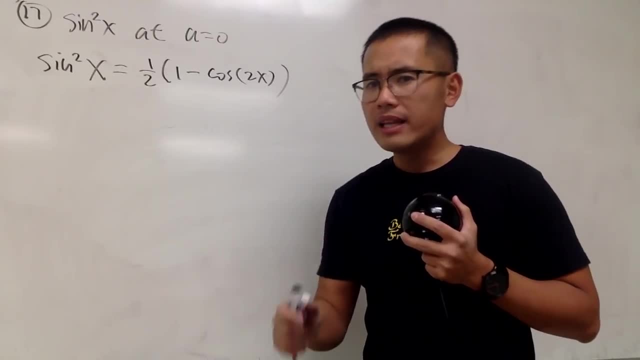 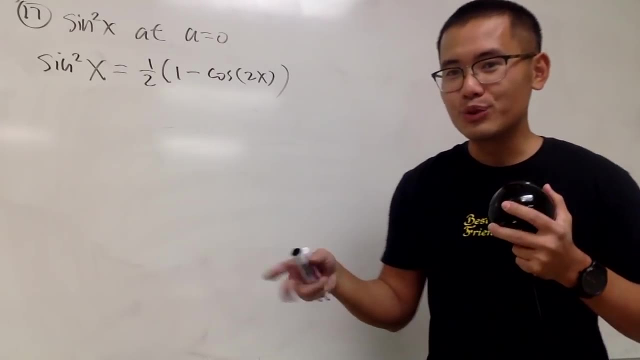 Just like how we do the integral- And luckily we just want to have a is equal to 0. So we don't have to see that x minus pi over 3, or whatsoever. This is all we need. Very, very nice. 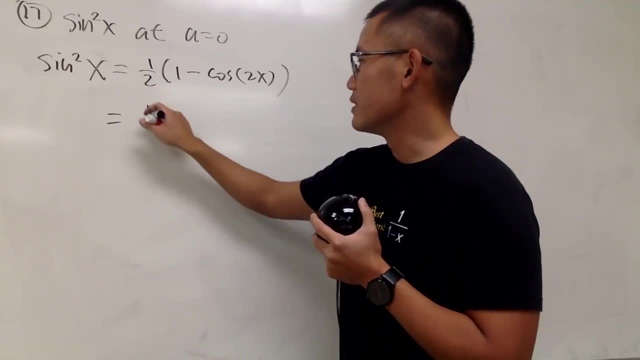 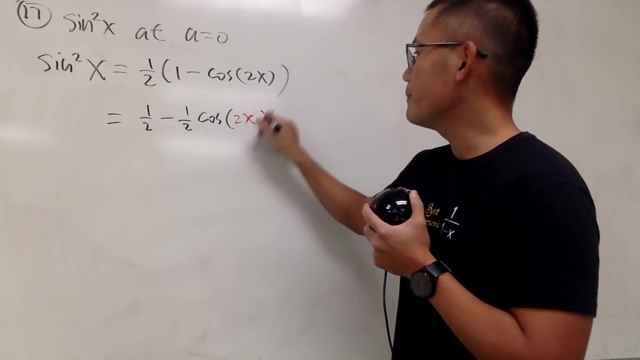 And now we'll just distribute this a little bit. This is 1 half and this is minus 1 half Cosine of 2x, And 2x is our input now, And now let's see what we can do with this. 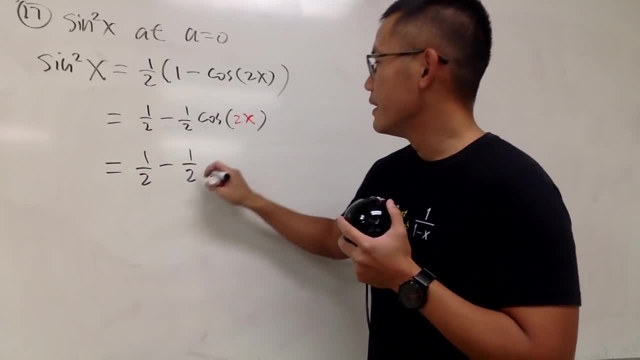 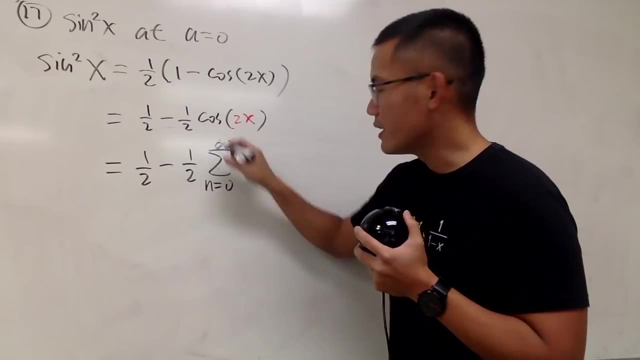 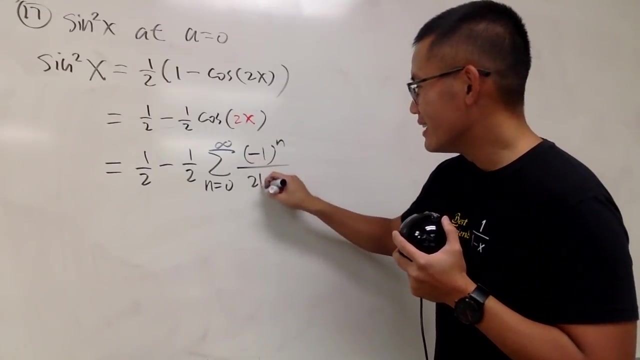 This is 1 half, This is minus 1 half. And for cosine? well, let's remember this, Let's do this in our head. This is the sum. n goes from 0 to infinity. What's the coefficient? We have negative 1 to the nth power over 2n, factorial this: 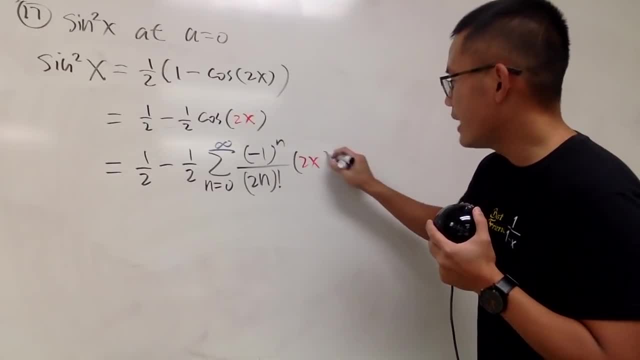 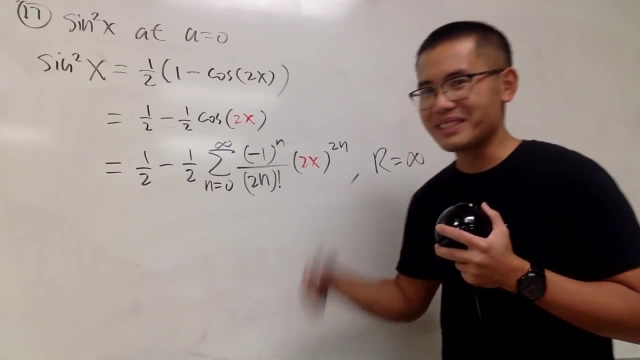 Yeah, And then the input goes here Here 2x, and then raised to the 2nth power, And again r is infinity. You can just write that down. You don't even need the absolute value, because r is infinity. 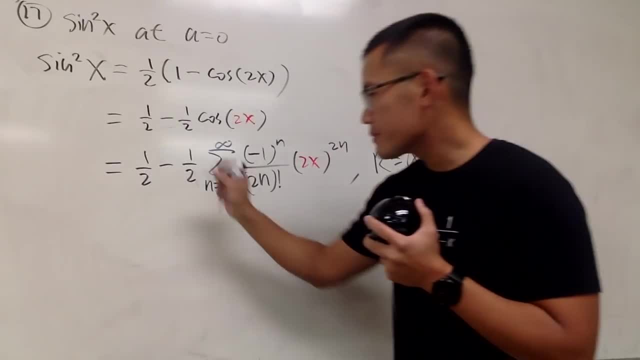 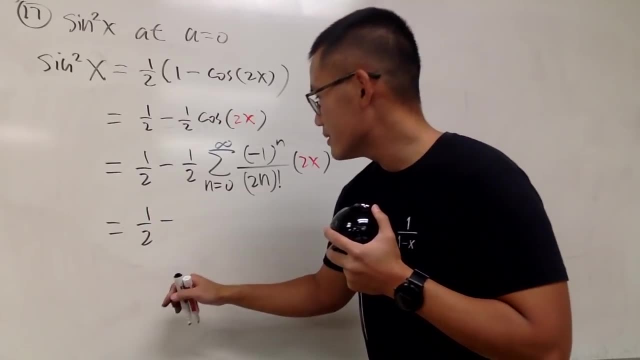 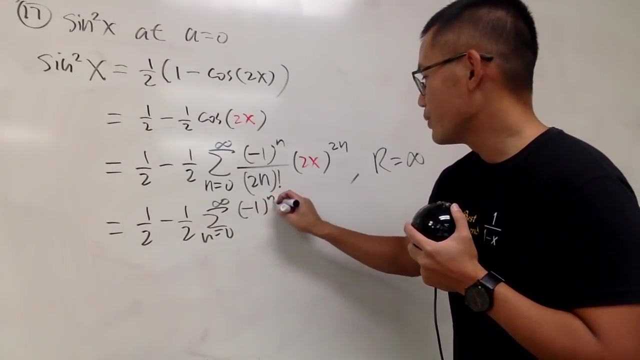 That's very nice. Now simplify this a little bit. Again, this is 1 half minus. Yeah, let's just write it down like this: Sum n goes from 0 to infinity. This right here stays Negative. 1 to the n over 2n factorial. 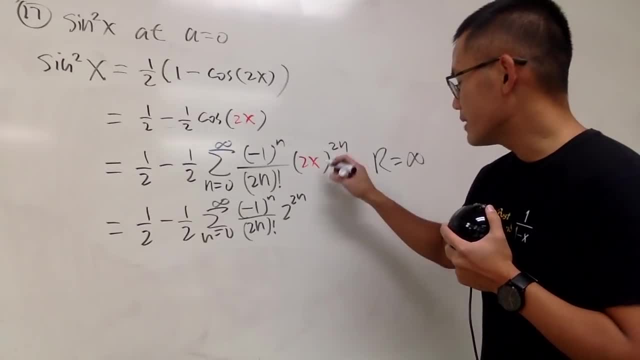 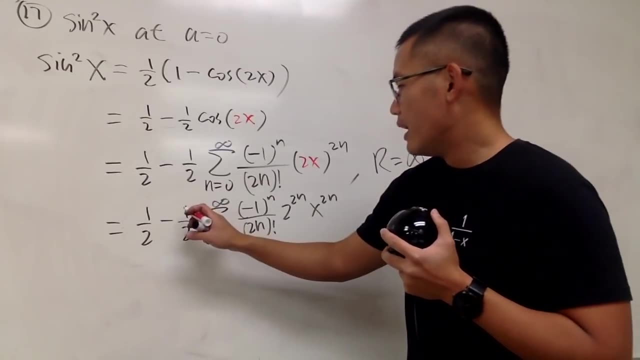 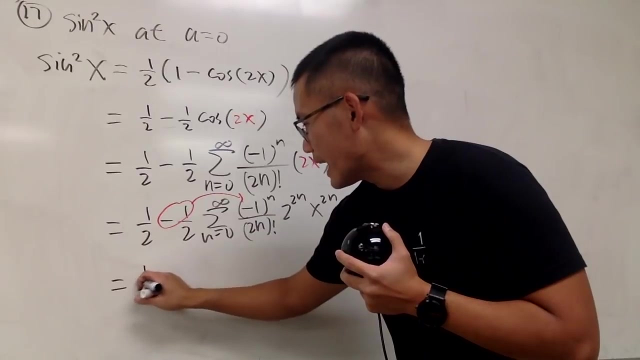 We can write this as 2 to the 2n times x to the 2n, Like that. Okay, now check this out. I'm going to pair this and that, So I will just multiply this and that together. So it seems that we have the 1 half all the way in the front. 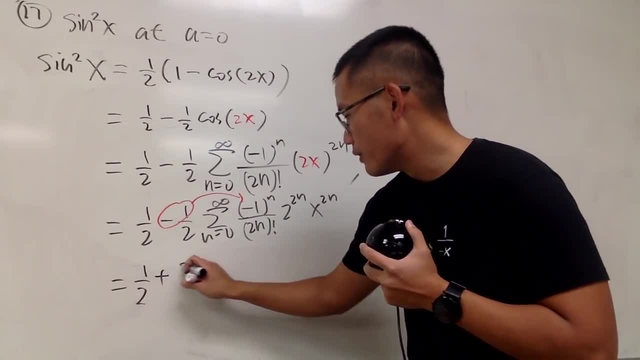 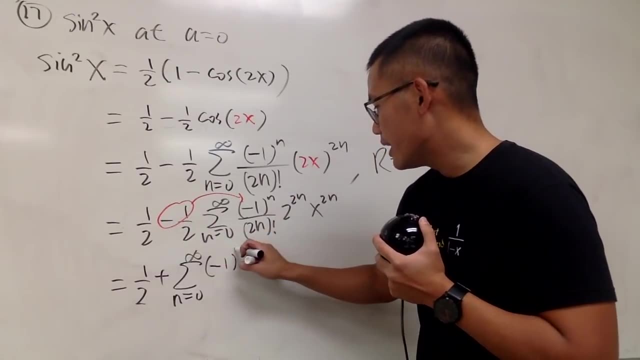 And I'll be adding because I will be multiplying this and that. So first I will have the sum: n goes from 0 to infinity Negative 1 times. this is going to be negative 1. To the n plus 1 power. 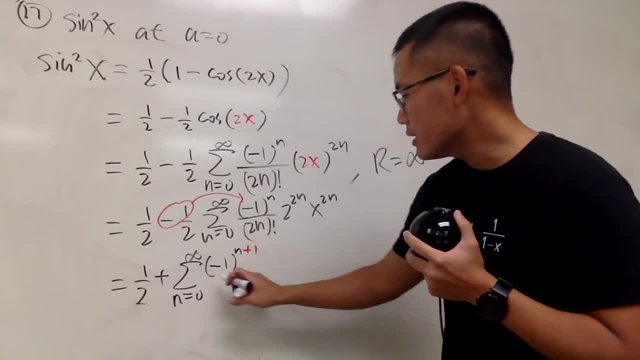 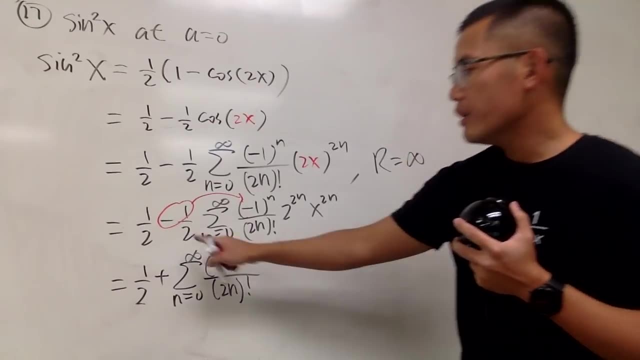 Okay, So that's that part, And then over 2n factorial. It should be outside of the parentheses And notice how this is divided by 2. So we just divide this by 2. Then we can just do 2n minus 1.. 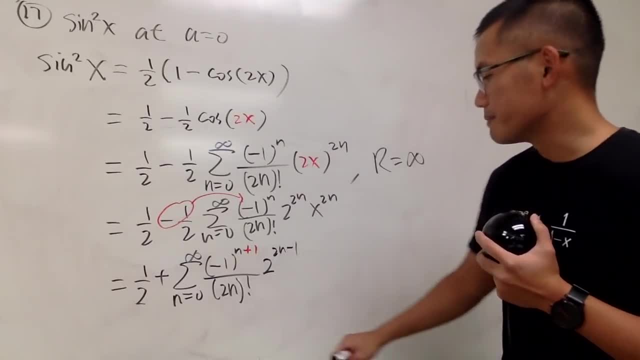 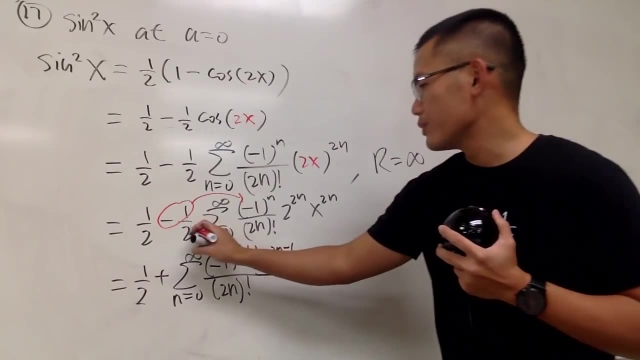 So this is 2 to the 2n minus 1 power, like, so 2 to the 2n minus 1. Because again, you divide it by 2.. Right, So you also have to consider this. So it becomes divided by 2.. 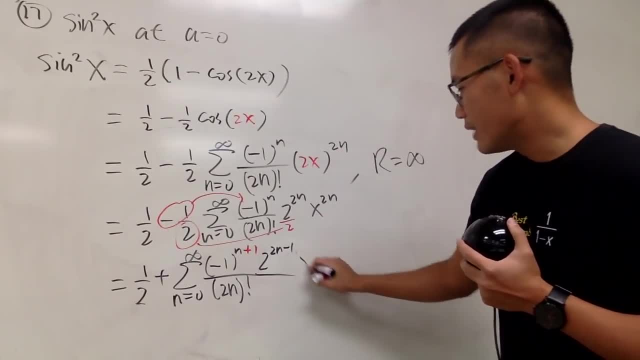 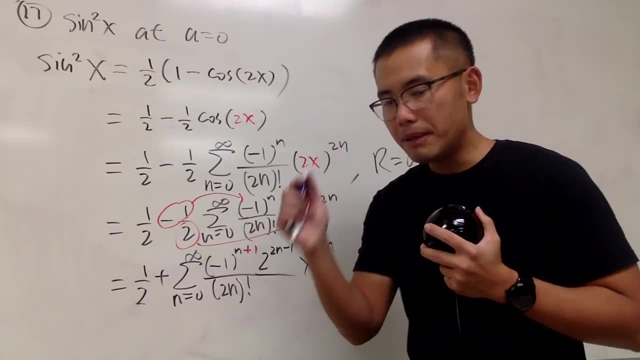 Like that. Okay, So that's the idea. And then you have x to the 2n power, like this. So it seems okay, right, But in fact we can do a little bit better, Because the deal is that, if you look at this expansion, 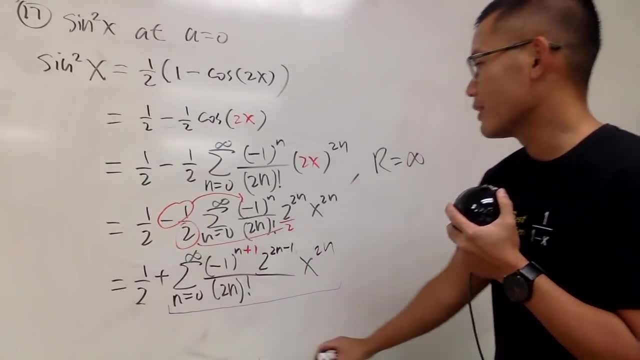 when n is equal to 0, let's do this in your head. Okay, Let's do this in your head When n is equal to 0, okay, this is going to be negative 1. So we'll have negative. 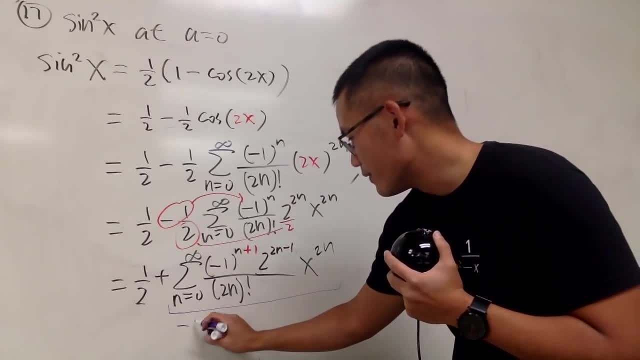 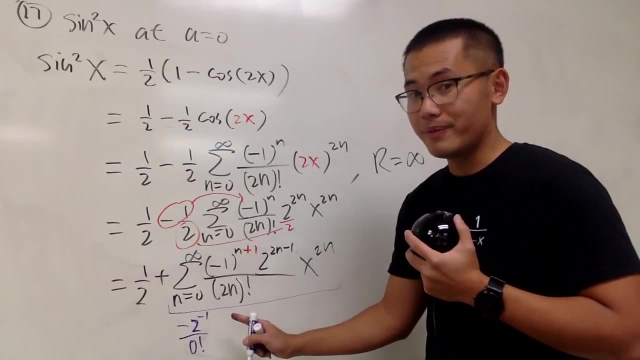 When n is 0, we have 2 to the negative first power. So we'll do 2 to the negative first power over 0 factorial. This is when n is equal to 0.. Okay, And then x to the 0th power. 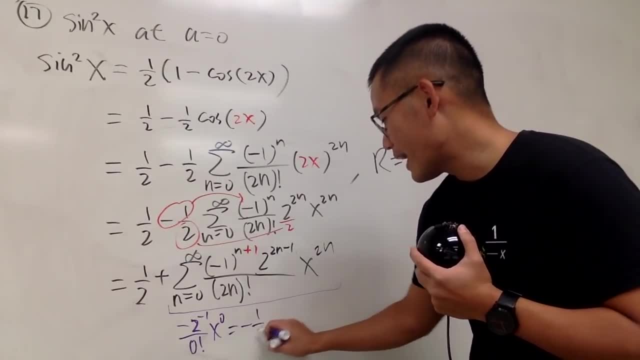 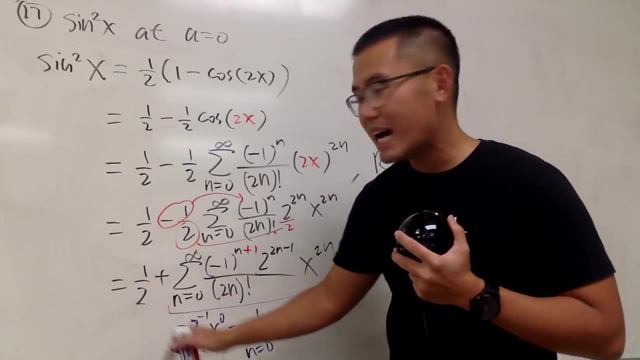 So this is just that. So that means you get negative 1 half. This is when n is equal to 0.. But when n is equal to 0, you get this And outside you have 1 half. So in fact we can cancel this out. 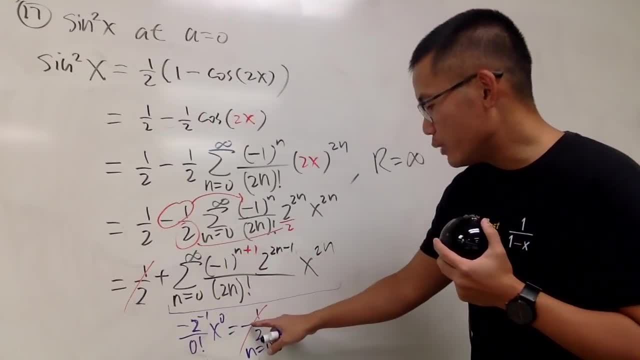 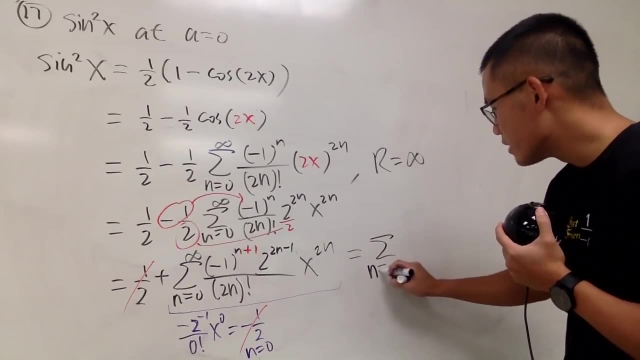 So The first term here is negative 1 half. That can be canceled out with the positive 1 half Altogether. we can just write down the sum as n, starting with 1.. Right, Because the first term we'll cancel with that. 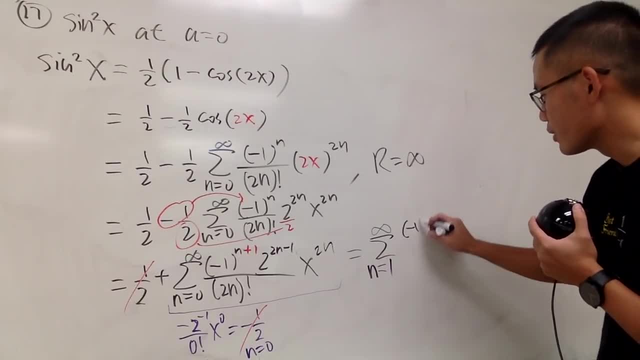 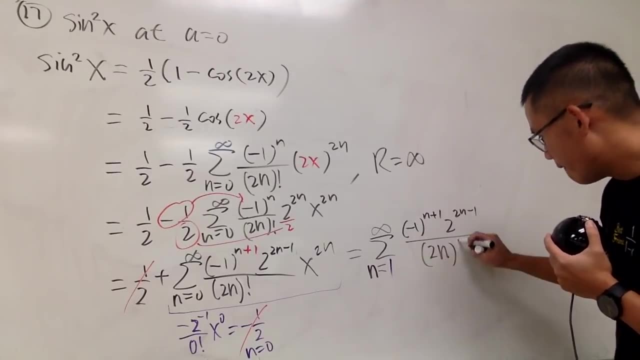 And then you just go to infinity and just write down the rest: n plus 1,, 2 to the 2n minus 1, or over 2n, factorial that, and then x to the 2n, like this: Yeah. 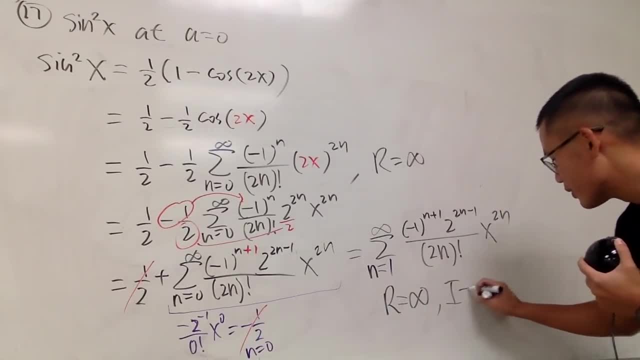 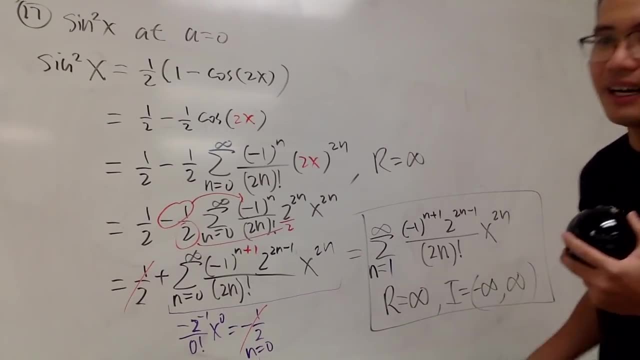 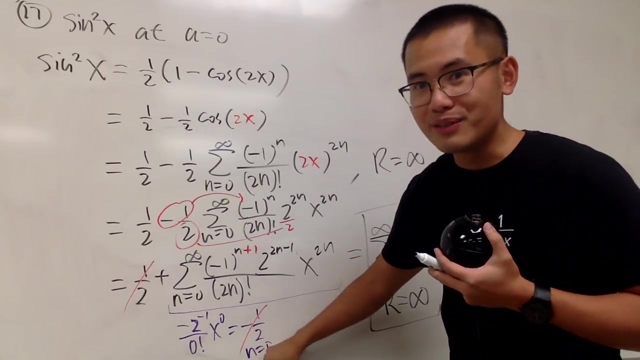 And then, of course, r is infinity. That means i is going to be negative infinity to positive infinity. Man, this marker is almost done, But I have another one. By the way, this marker isn't so bad. If you guys watch my 100 series video, you guys know that. 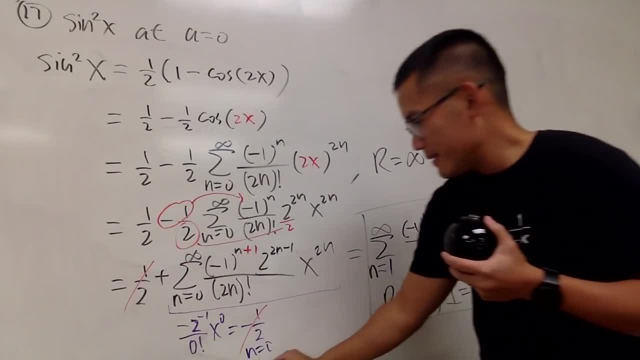 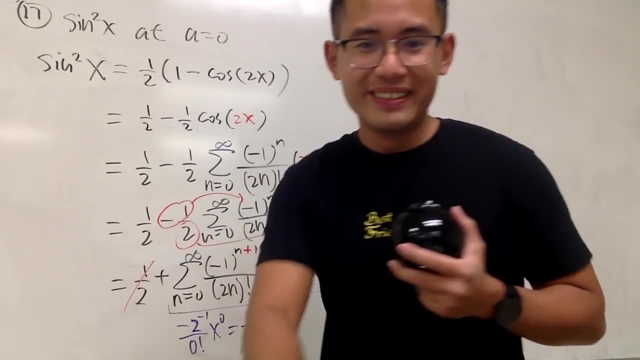 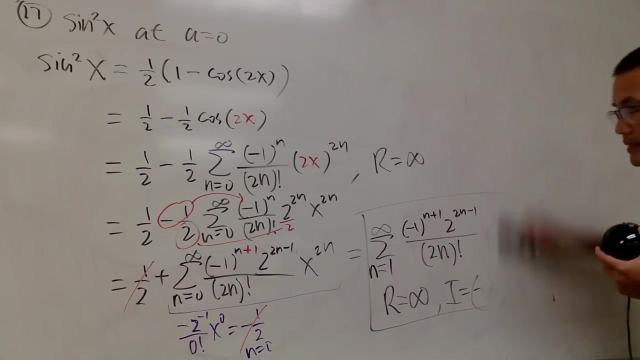 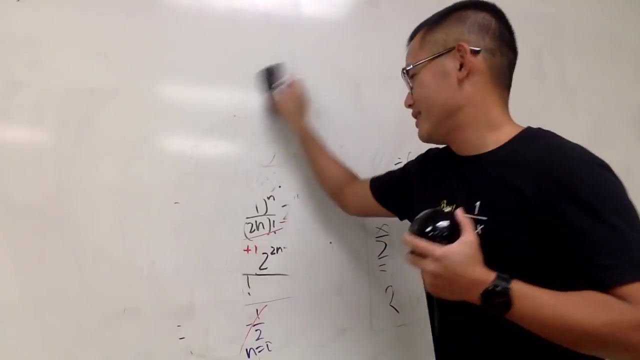 This marker is another one I like. Okay, So that was number 17.. Whoo, Okay, now take a look, take a look, take a look Right. Do you guys miss the Taylor formula? Maybe I heard some people say miss the Taylor formula. 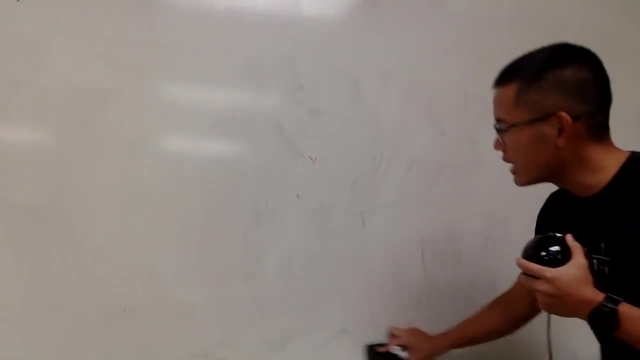 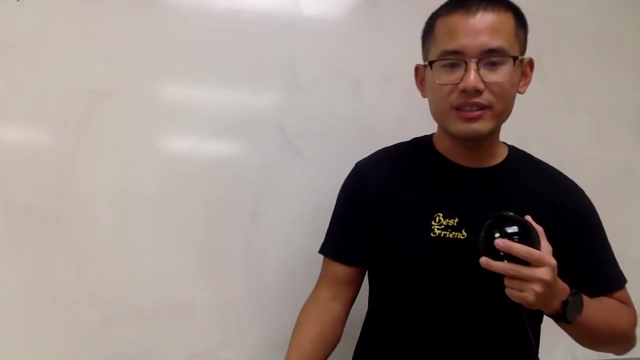 Sometimes we have to do that Right. Sometimes we have to do that Just like: if I'm trying to do something new that we have not seen before, then we have to do that. If not, then just try to make connection. Then that's how we can make things. 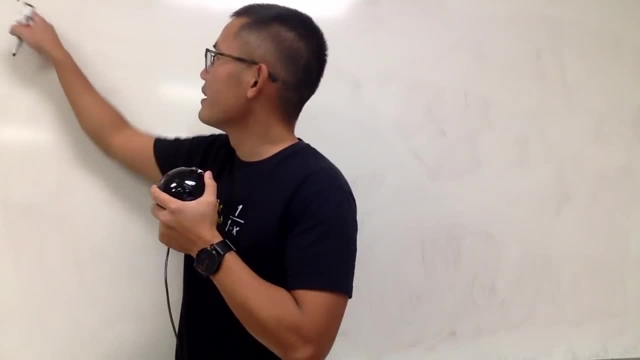 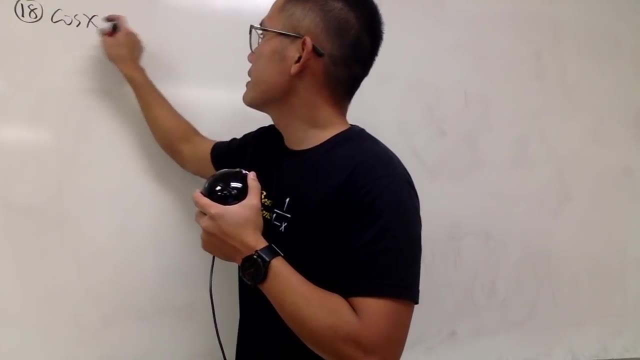 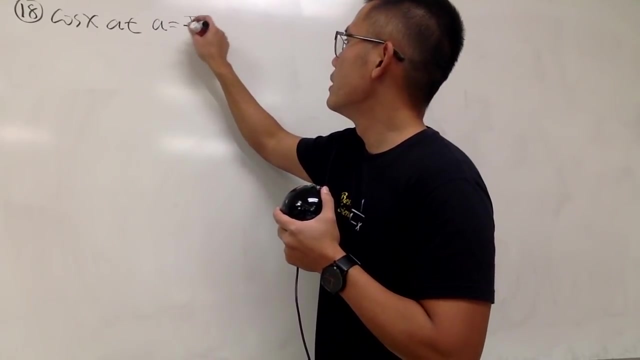 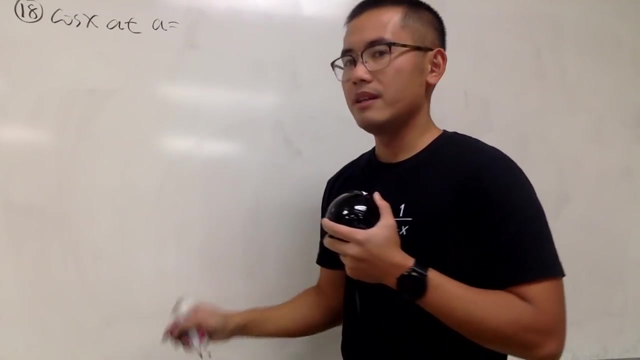 Ha, That's what's going to happen. Okay, number 18, right here, Number 18.. We have cosine x at you guys ready. a is pi over 4.. Okay, think about how you will actually do this. 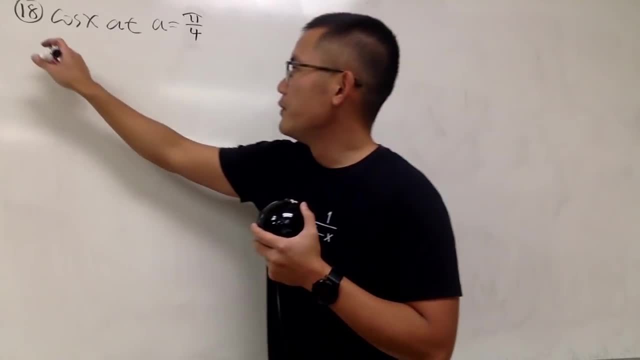 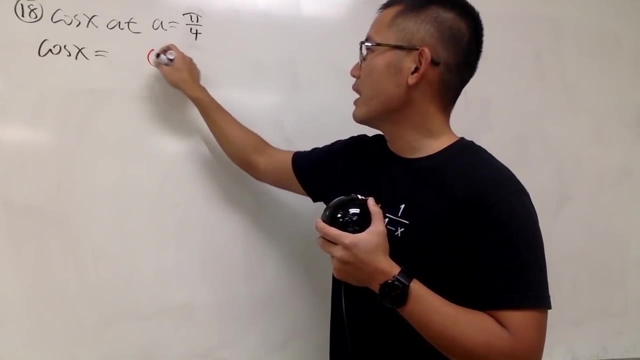 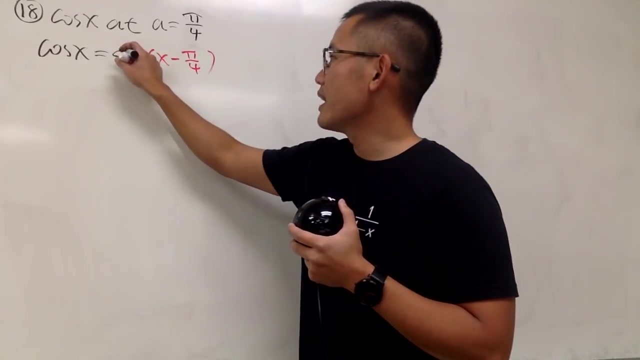 Hmm, Well, if you want to do what we did earlier, this is cosine x, And maybe you can end up with some kind of function with x minus pi over 4.. Is that true? Can you just do like sine or cosine to help us out? 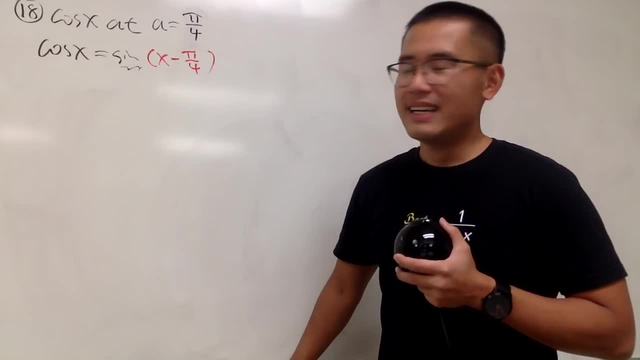 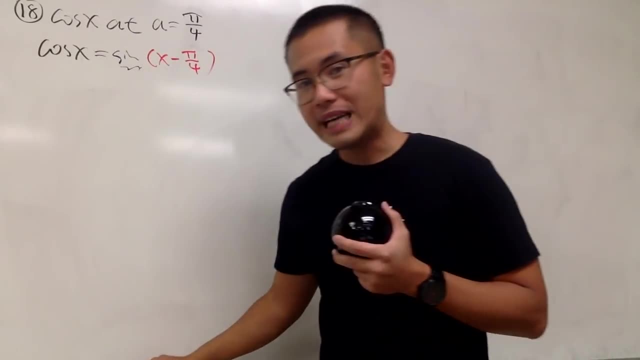 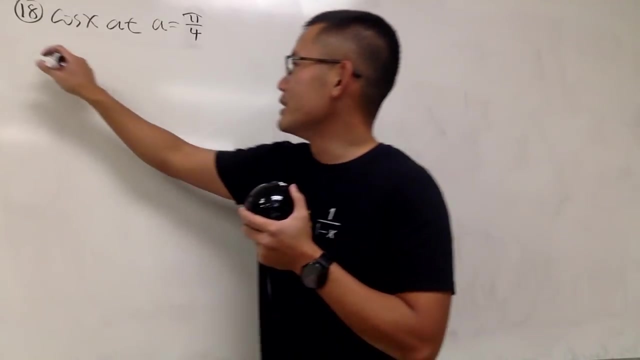 I don't think so, unfortunately. So here we'll go back to the Taylor formula. If you know how to use identity to do this, please comment down below, because I would like to know that myself. I didn't know how to do it, but it's okay, because the father of the power series can always back us up real quick, right. 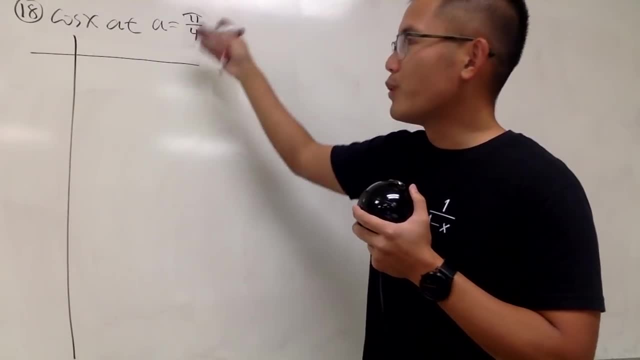 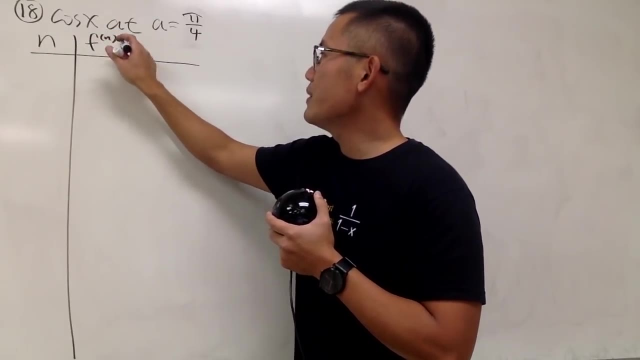 So here we go, Because at pi over 4, we don't get 0,, so I'll just use n. Doesn't matter, So we have n right here. And then do the derivatives, And then the formula which is the nth derivative. 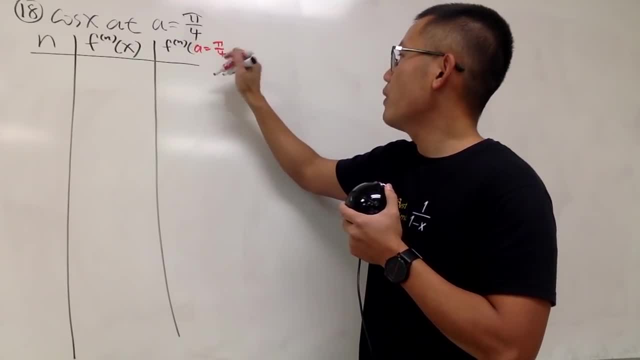 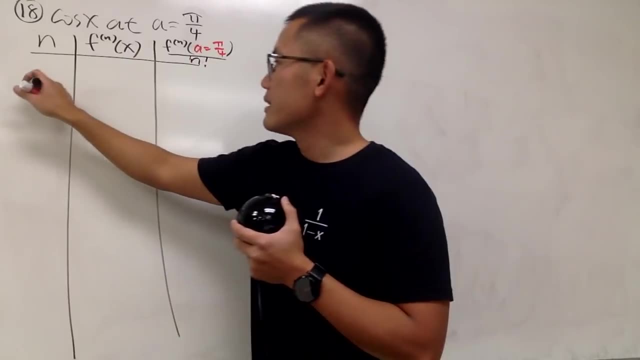 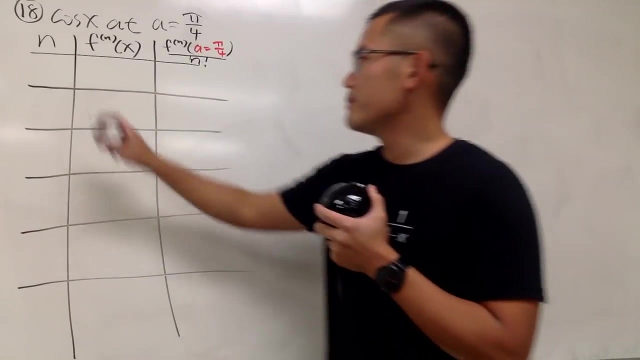 So we get at pi over 4, then divided by n, factorial, that guy, okay. All right, let's see 1,, 2,, 3,, 4, 5.. Hopefully you should see the pattern already, right. 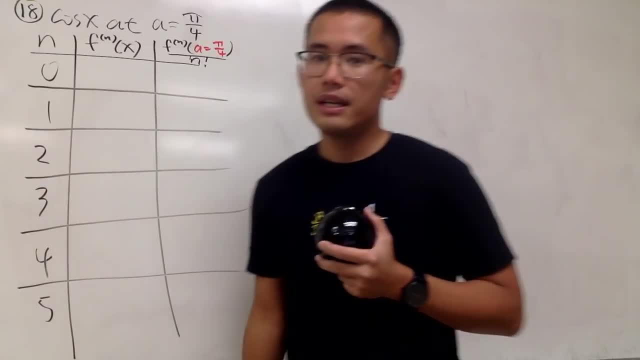 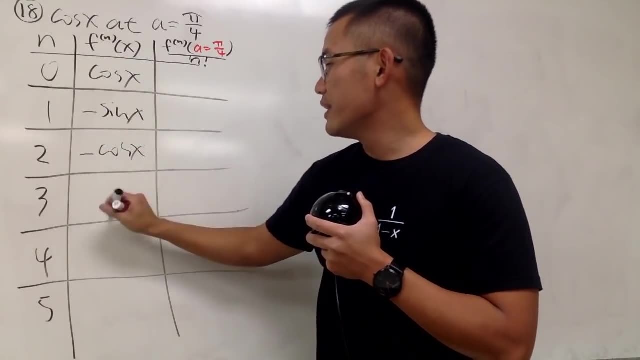 0,, 1,, 2,, 3,, 4, 5.. Here we go. Cosine is the original. Next we get negative sine, Next we get negative cosine. Next we get positive sine And then we get cosine. 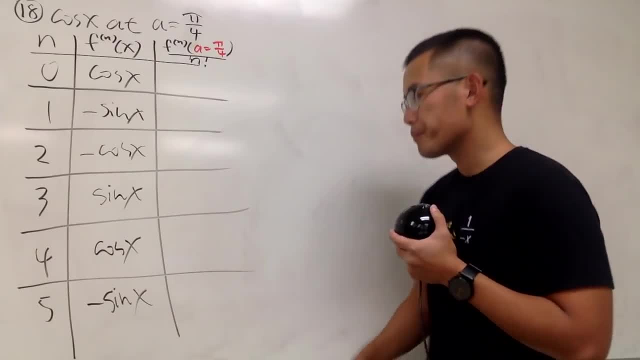 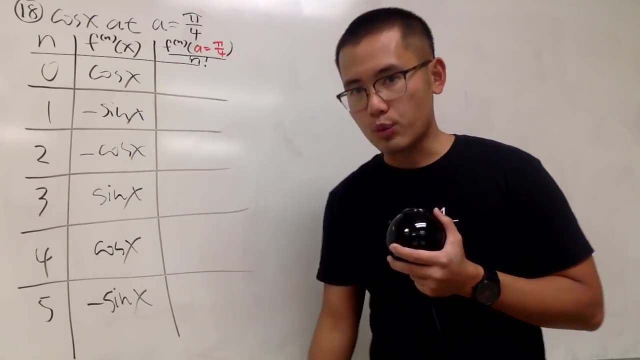 And then we get negative sine. So of course we see the repeat. So that's good. Now I will tell you. when we put pi over 4 into cosine, what do we get? 1 over square root of 2, all right. 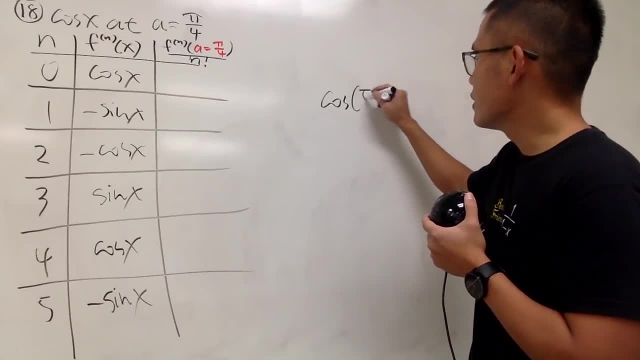 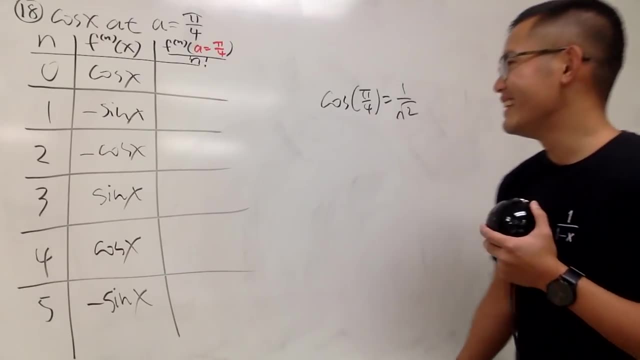 So I will just write this down right here on the side: Cosine of pi over 4.. This is 1 over square root of 2. And we are all adults now. We don't have to rationalize the denominator, And the beauty of this question is that sine of pi over 4,. 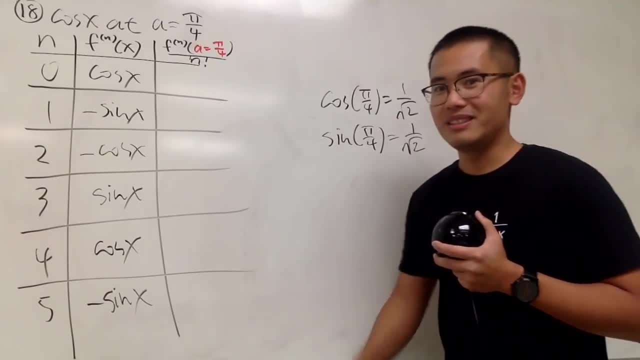 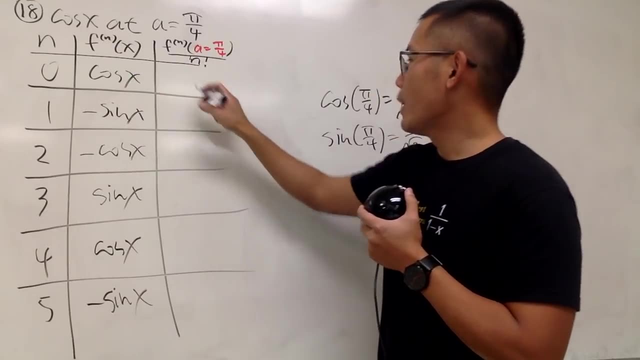 it's also 1 over square root of 2.. So this is the beauty for that, Anyway. so I will write this down: When we put pi over 4 in here, we get 1 over square root of 2.. I will just put it down right here. 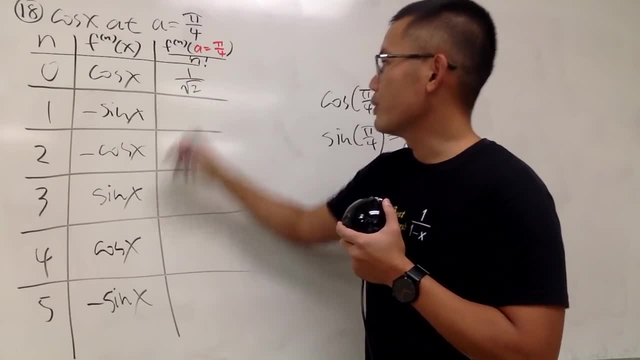 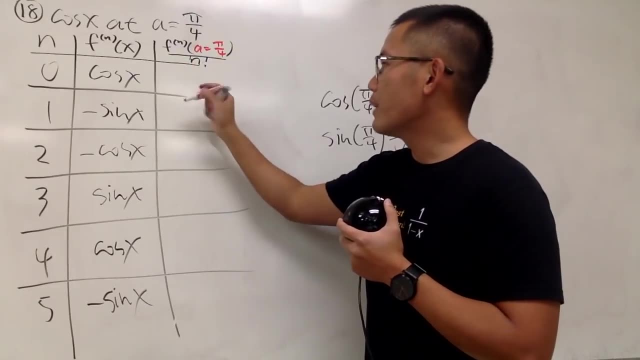 And 1 over square root of 2. And we have the factorial. Let me just put this down in red. actually, Let me put down these numbers in red. So when we do that, we get 1 over square root of 2 times 1 over 0 factorial. 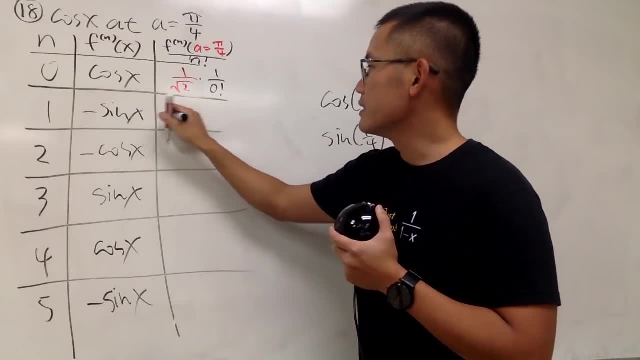 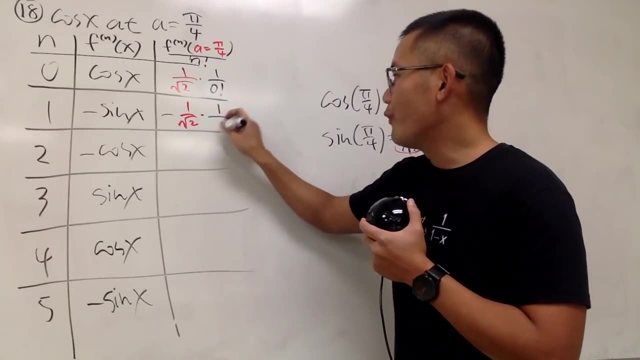 Like this: okay, Next we get negative. So this is negative: 1 over square root of 2. Because sine of pi over 4 is also 1 over square root of 2.. Times 1 over 1 factorial And you just continue. 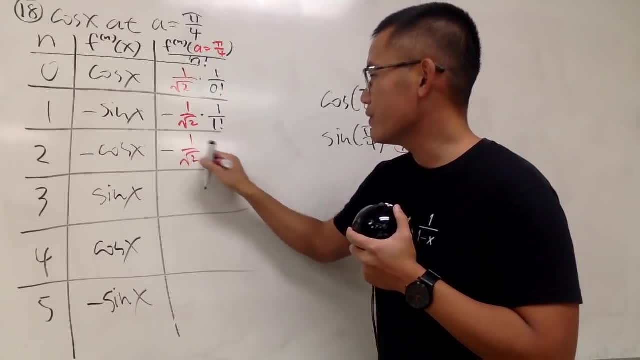 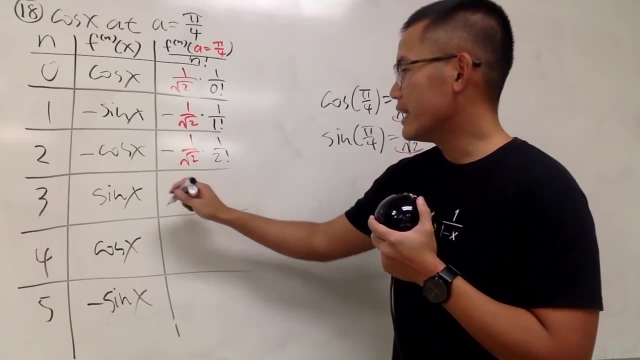 Next you have negative. So this is negative. And again 1 over square root of 2.. Everybody has 1 over square root of 2.. That's pretty nice Times 1 over 2 factorial. And then negative: 1 over square root of 2 times 1 over 3 factorial. 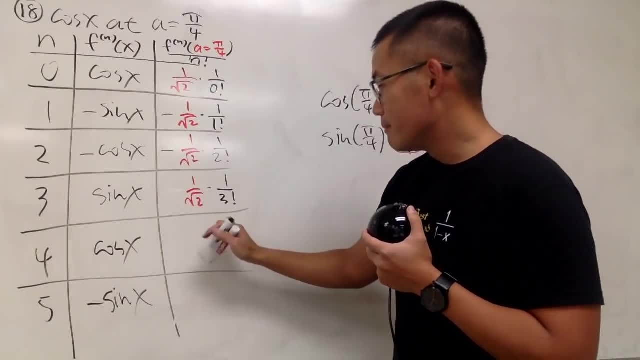 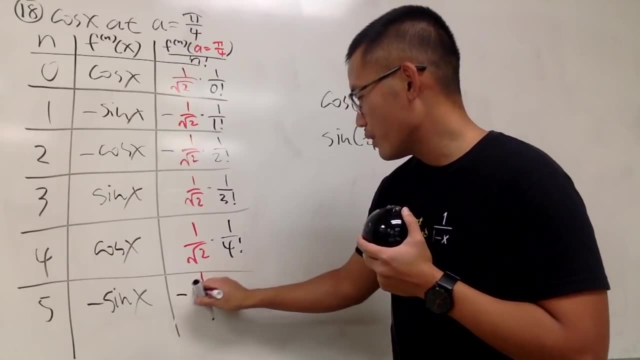 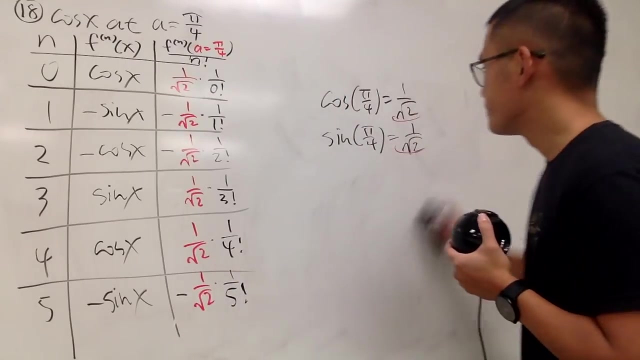 Oh no, this is positive Positive And then negative. Positive: Positive: 1 over 4 factorial. Now it's negative: 1 over square root of 2 times 1 over 5 factorial. So it doesn't seem so bad. 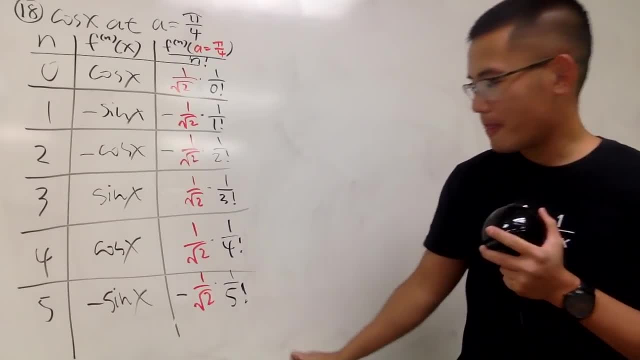 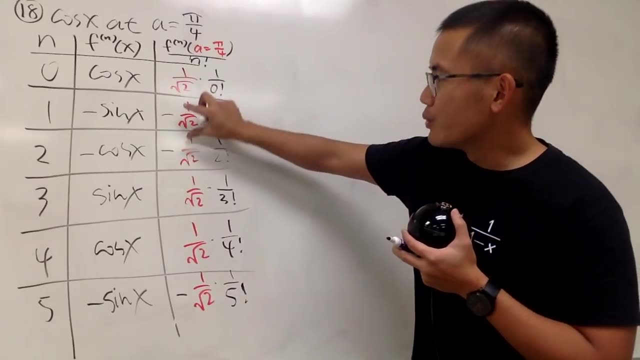 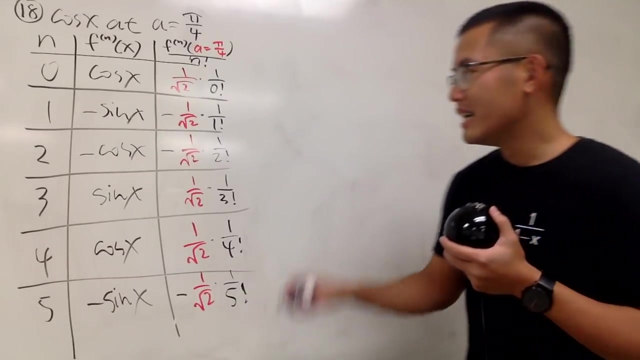 But here is the trouble. Here is the trouble: Positive, negative, negative, positive, positive, negative, negative. So it's like two negatives here, Two positives here And then two negatives, Two positives. Is this alternating? Unfortunately not. 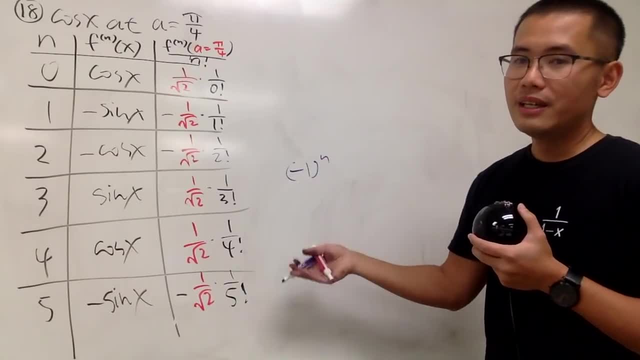 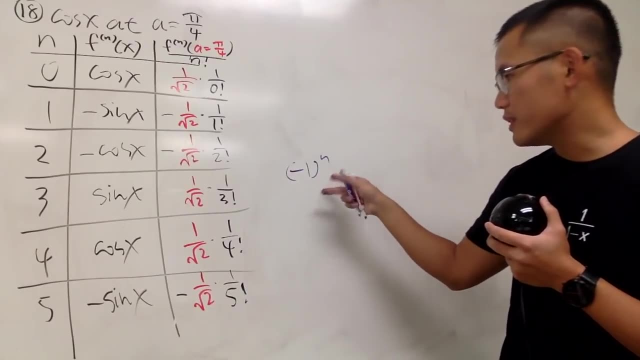 This is not alternating in the usual sense. like this: Again, it's negative, negative And then positive, positive And then negative, negative, And so on, so on, so on. So this factor of a revision of this might not help us out. 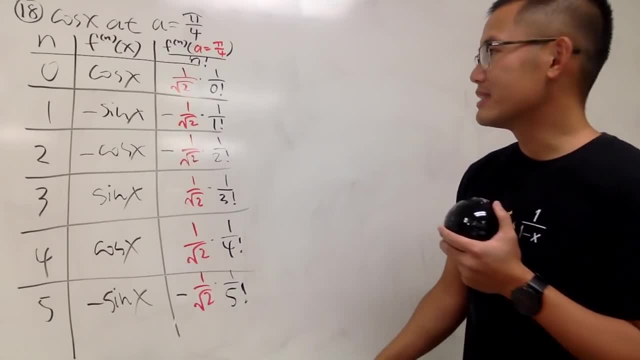 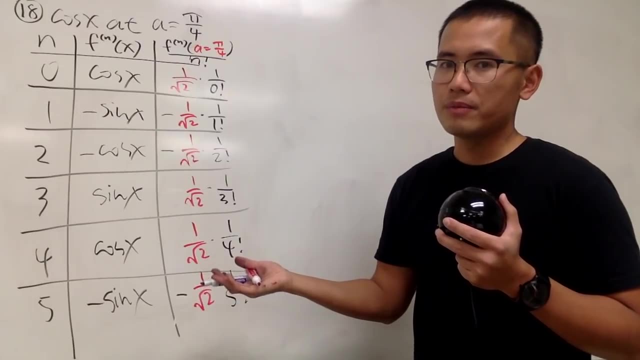 Well, we have to think better than this. I will put this down in purple Notice: everybody has 1 over square root of 2.. So that's the pattern. That's no big deal, And you can just write down: 1 over n factorial. 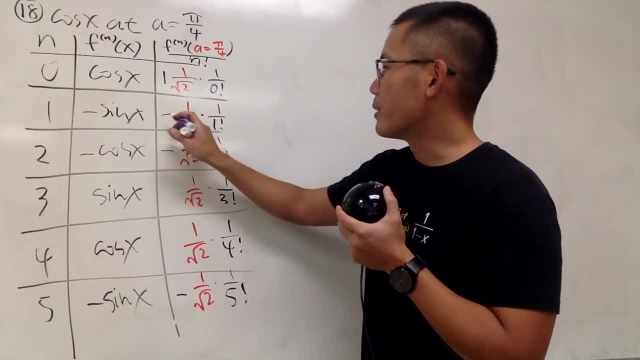 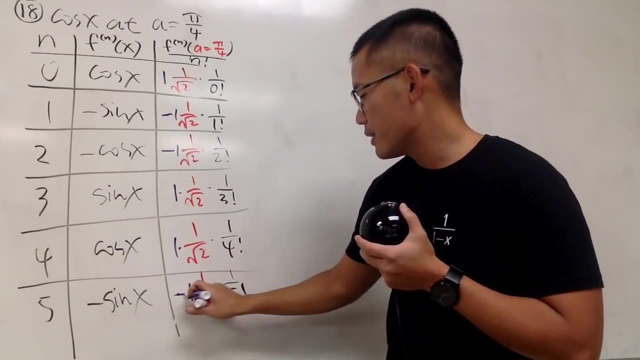 Again, no big deal, But I want to look at 1 in purple, negative, 1 in purple, negative 1 in purple, and then 1, and then 1, and then negative 1.. Right, In fact, let's look at these numbers. 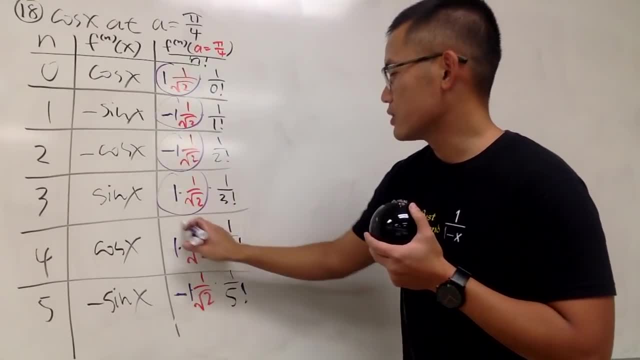 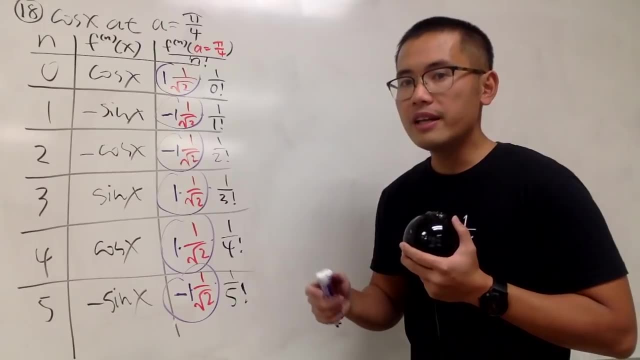 This, this, this, this and so on. You guys will see this is actually a really nice way to do this. It does repeat. So it's a good idea to visit the unit circle And, by the way, if you want to check out my unit circle on Merge, 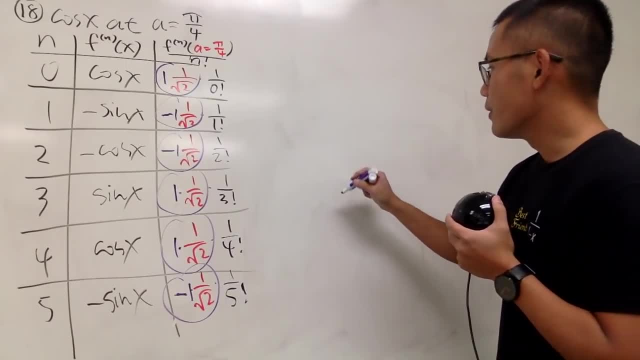 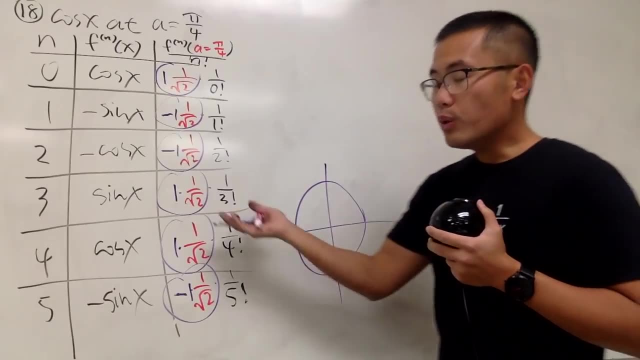 you can just go click on that, OK. So now we'll just put this down right here. Here is the unit circle, And we're always talking about 1 over square root of 2. That means the angle is pi over 4.. 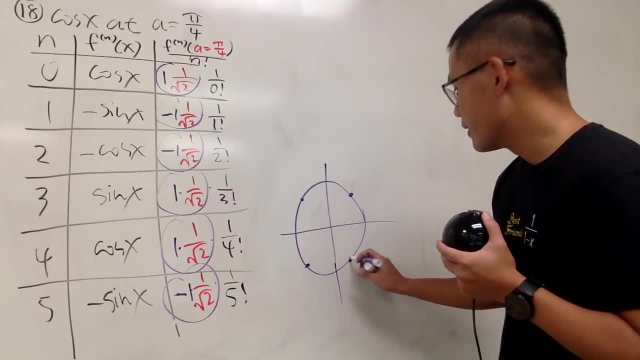 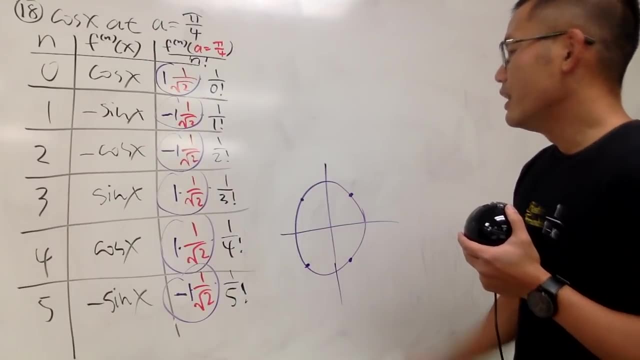 Or maybe right here, Or maybe right here, Or maybe right here. Right, And it depends if you want to like to use, if you like to use sine cosine Or whatsoever, In this case it's a good idea to use cosine. 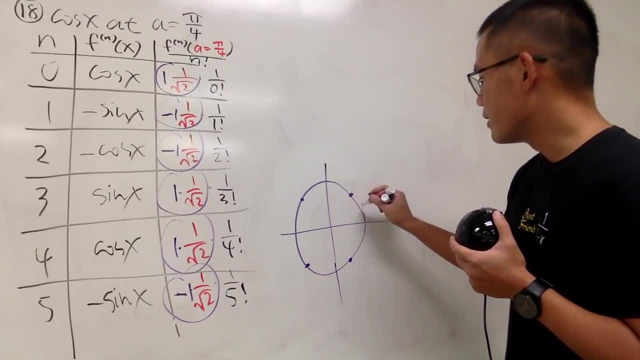 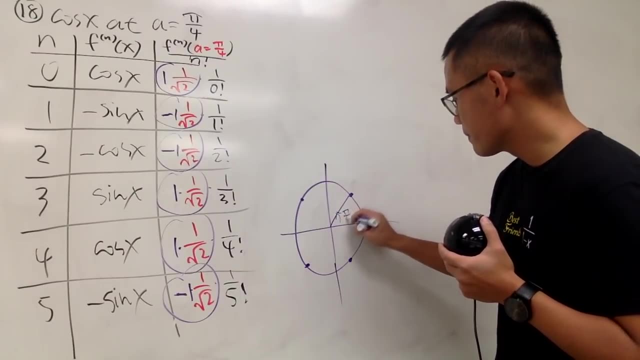 Check this out, This right here. if you look at cosine right here, this is pi over 4.. And this is pi over 4.. So let me just write this down for you guys real quick. Cosine of pi over 4. 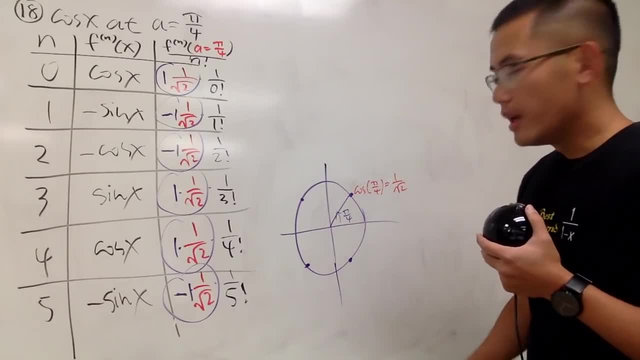 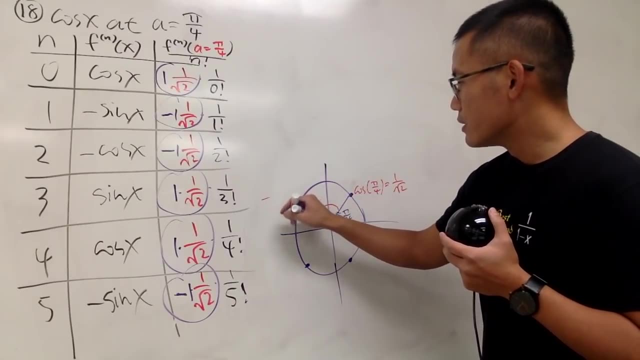 is positive: 1 over square root of 2.. And the moment that we reach to here, so you just have to rotate here. the moment we reach here. this is negative cosine of pi over 4, if you want to do that. 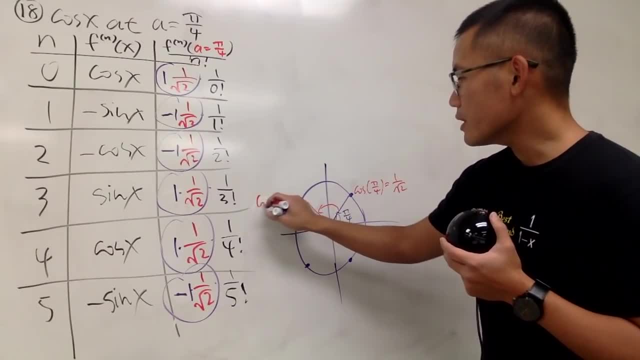 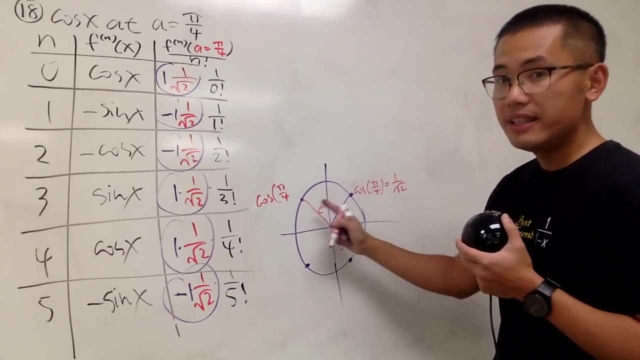 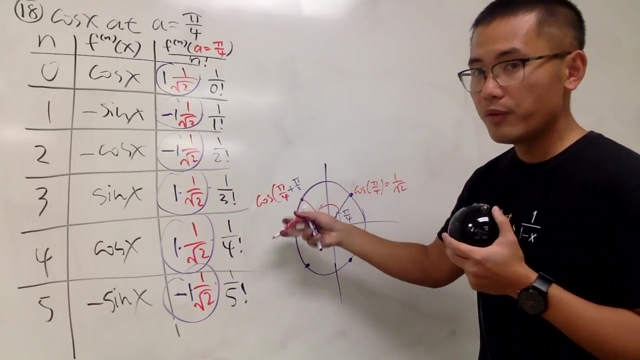 But you can also look at this Cosine of pi over 4, and if you want to go from here to here, this is actually a 90 degree angle, So you just have to add pi over 2, which is going to give you 5 pi over 4,. 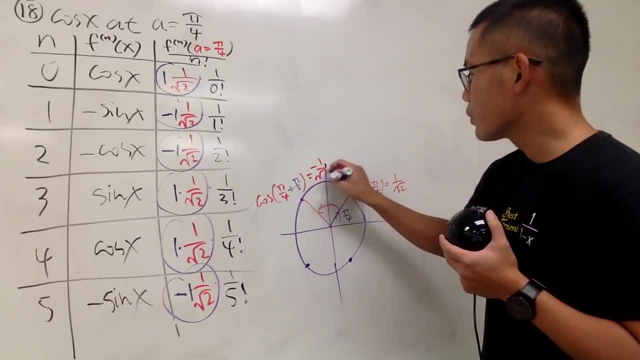 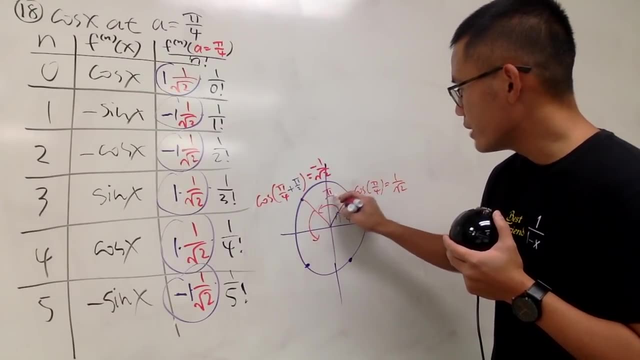 instead of cosine. This is going to give you negative 1 over square root of 2, isn't it? And then, if you keep going, another pi over 2, this is rotated pi over 2,, rotated pi over 2,. 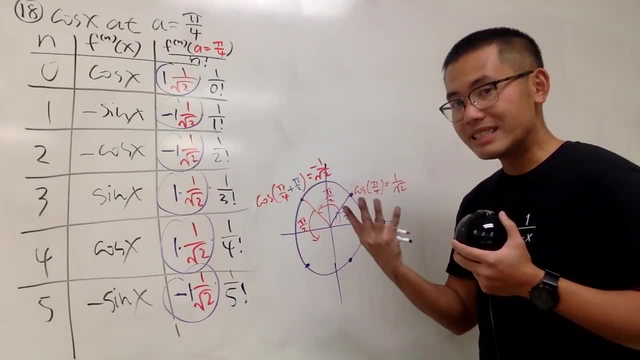 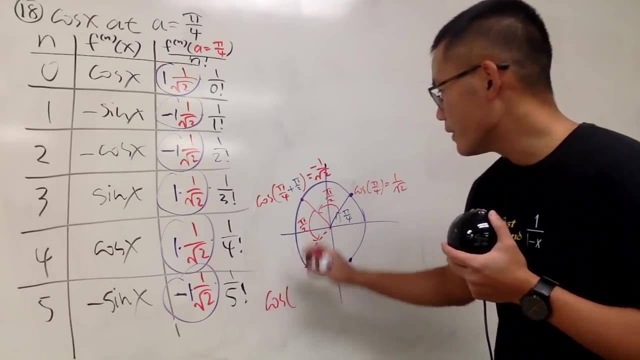 because you have the whole circle cut into 4 pieces. So 2 pi divided by 4 is pi over 2.. That's all that's done. This right here is going to be cosine of pi over 4, I'm looking at the starting. 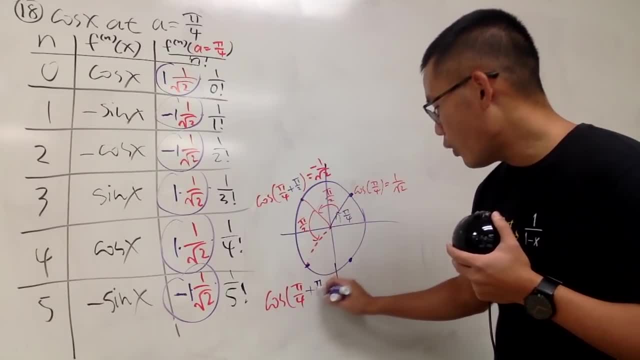 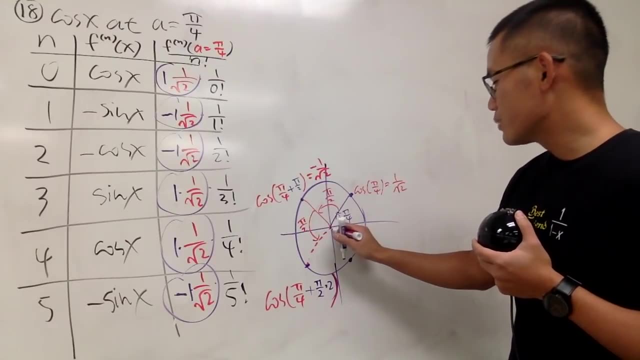 and then I just have to add pi over 2, but twice Right. That's the idea And you can imagine what I will do next. This right here. I'll just make it like a different dash line, like: so, Just add the pi over 2 one more time. 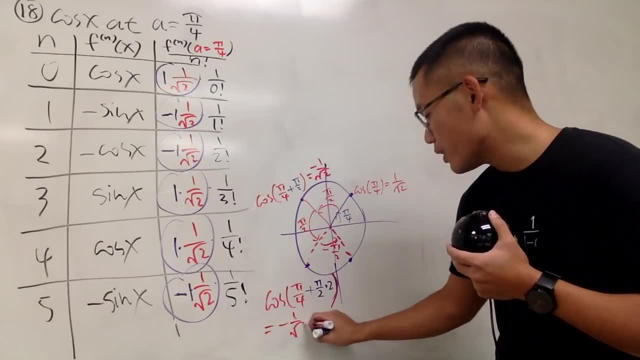 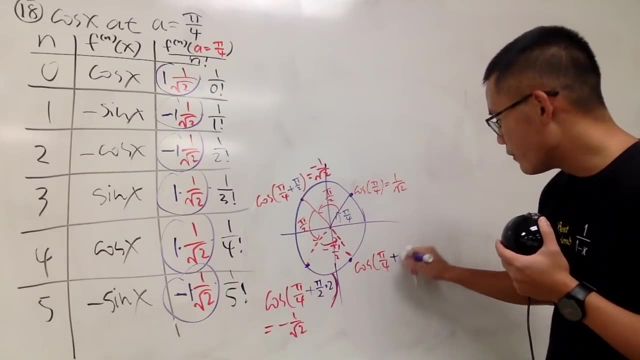 And notice this right here- does give us negative 1 over square root of 2, right, And for this point, this is going to be cosine of starting at pi over 4, and then you add the pi over 2 three times, like this: 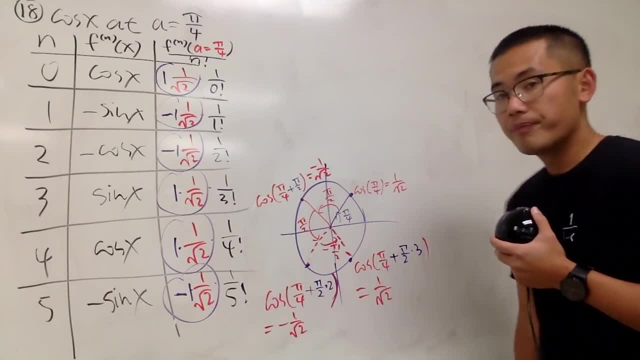 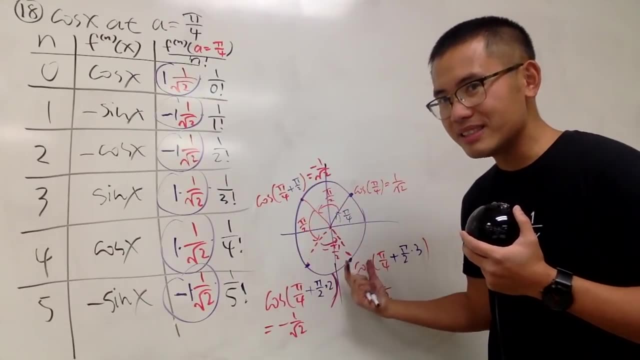 And you end up with positive 1 over square root of 2.. Because right here you're talking about positive x value and then negative x value, and still negative x value, and then positive, positive, negative, negative and so on. 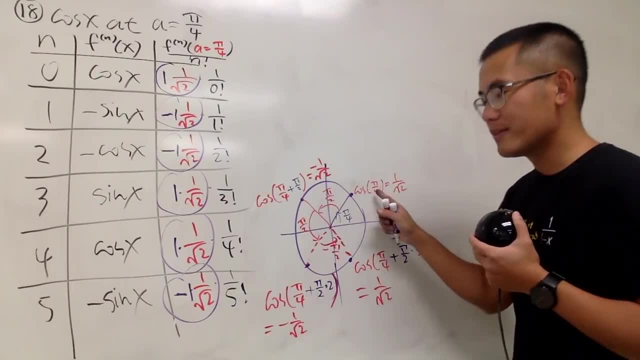 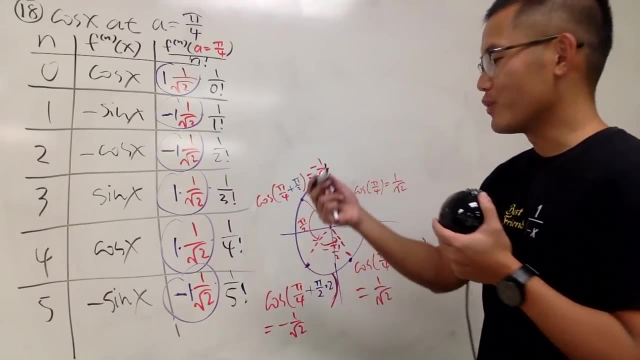 So for all the numbers in purple, it's just cosine of pi over 4, plus pi over 2 times n. Very nice, So here we go. We can write down the formula: Cosine x equals the sum. n goes from 0 to infinity. 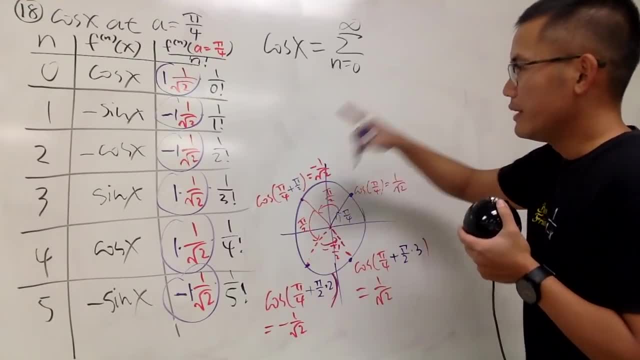 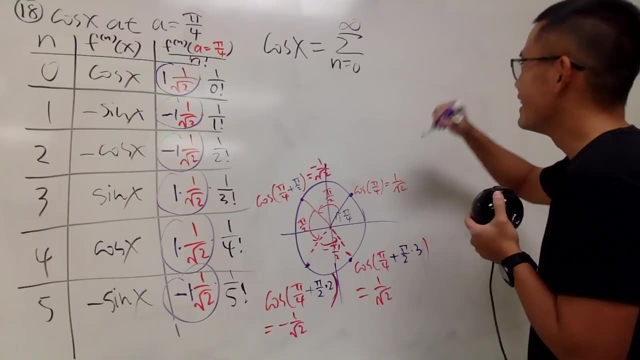 Let's write this down. In fact, I include 1 over square root of 2 because of 9th D. we have the cosine right, So that's why it's very nice. Anyway, we have cosine starting at pi over 4,. 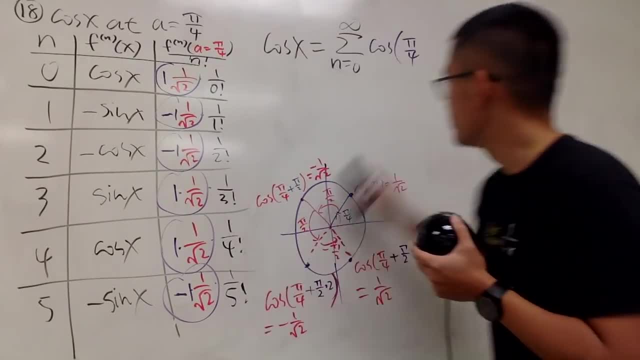 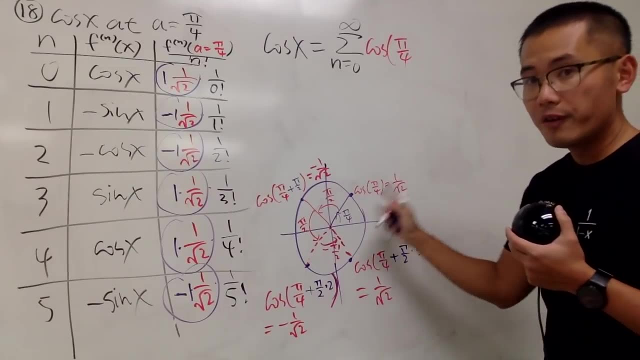 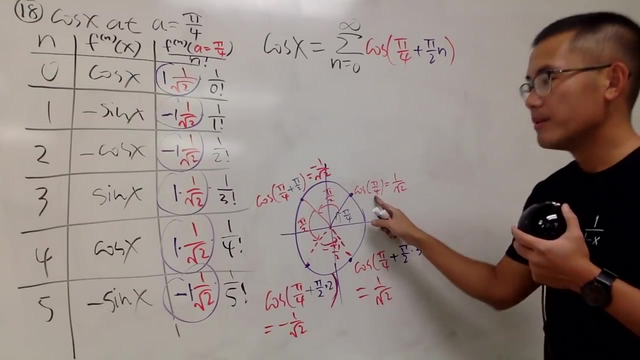 starting at pi over 4.. Actually, let me match the color Cosine of starting at pi over 4, and we are going to just add pi over 2, n like this, Because n start with 0, so if you put 0 here, 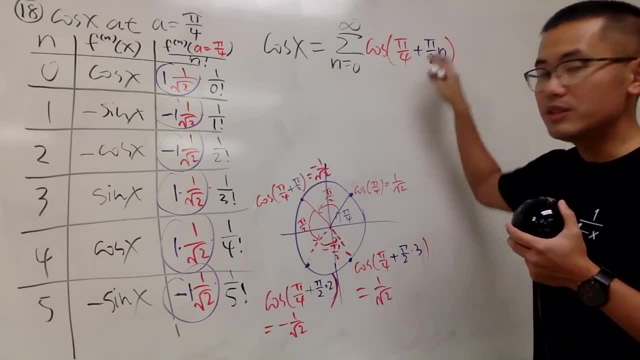 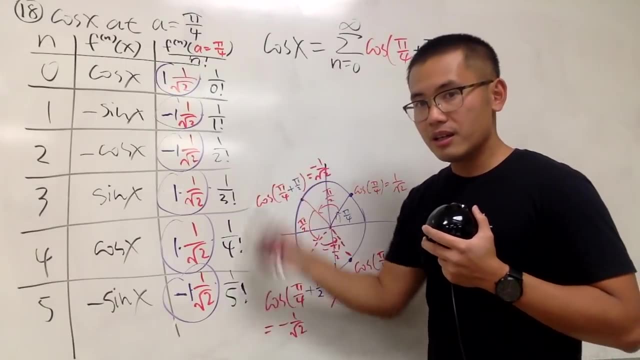 then you get this, And then when n is equal to 1, you just jump to here. So this right here covers the coefficients right here. But we also have to look at the factorials on the bottom. No big deal, We can just look at this. 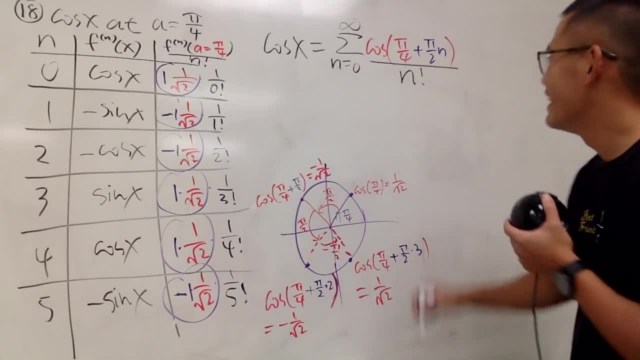 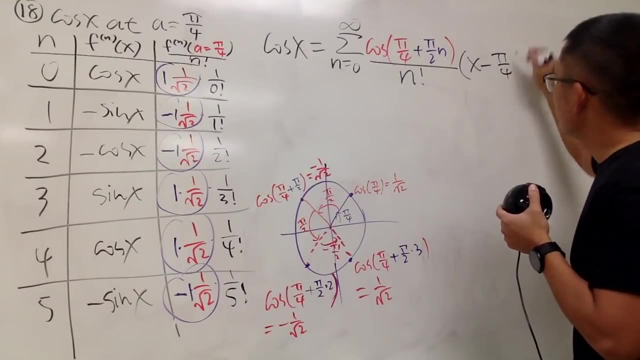 and divide it by n, factorial. That's it right. And because this right here, a is at pi over 4, so this is x minus pi over 4, raised to the nth power. like this, There's no 0 term. 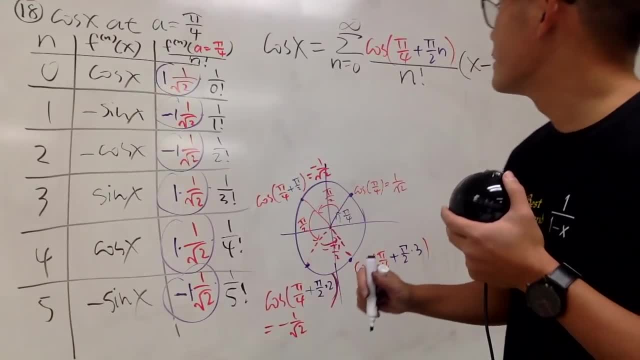 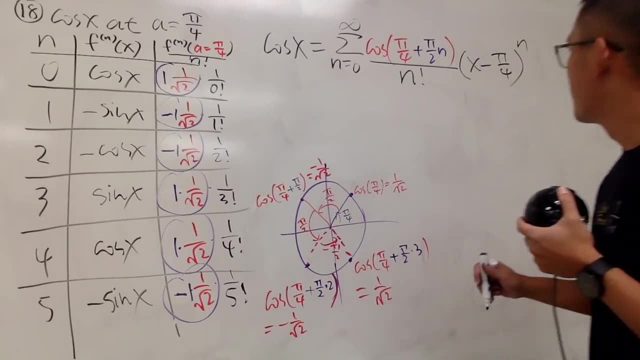 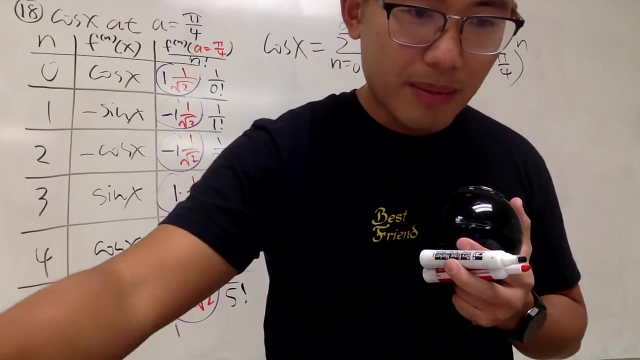 So this is very, very, very, very nice. Let's see. Huh, Okay, I am suspicious again. I don't know why on my answer key I put down 2 nth power. Let me just double check. Let me just double check for from alpha. 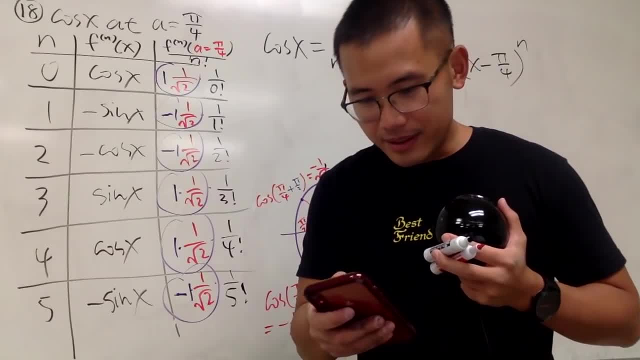 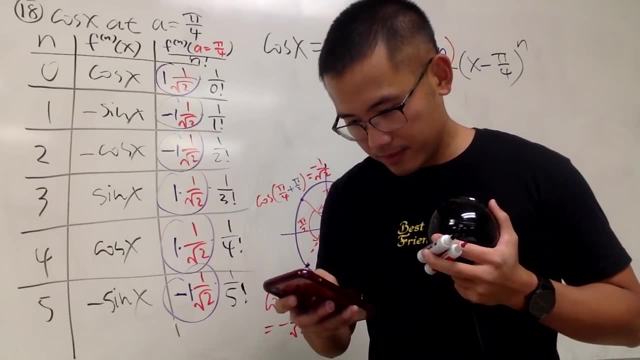 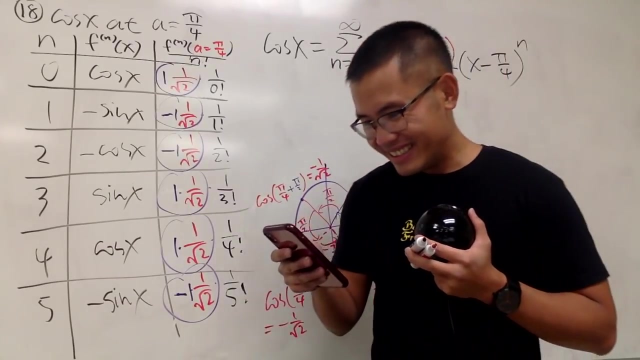 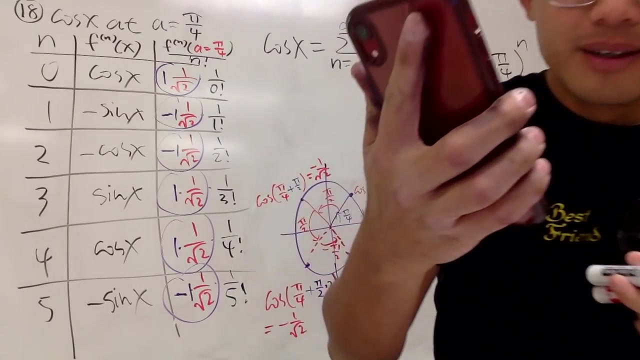 because I want to make sure that I give you guys the correct answer. Yeah, this way I can take a little break too, So it's a win-win situation. Yeah, I got this right here. I've opened alpha, Okay, And my answer key is wrong. 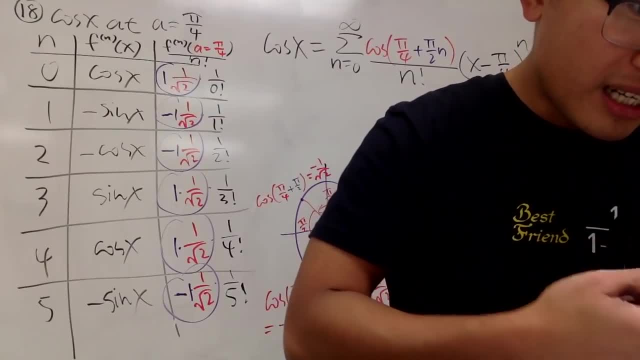 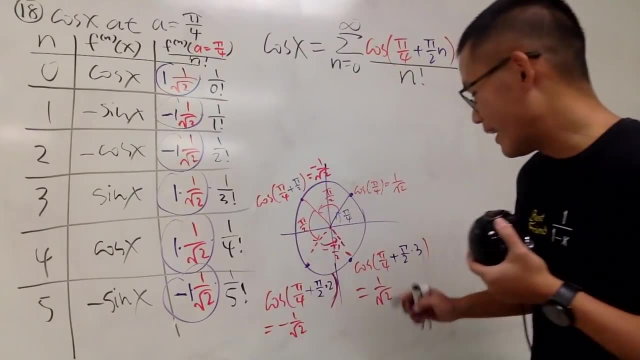 Haha, I had the 2 nth, so we'll just change that. So, as I said, I'm I don't know why whenever I come with answer keys, I just. That doesn't really work out. Anyway, this is it. 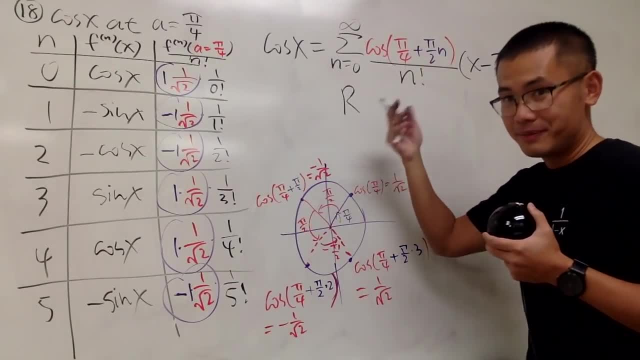 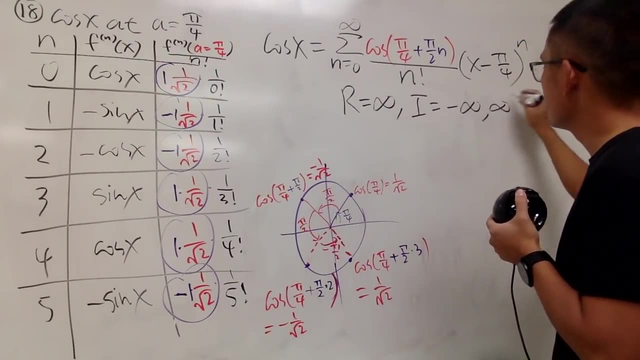 And, if you would like, you can just work this out with the formula I told you guys before. But r is infinity. Likewise, I will also be going from negative infinity to positive infinity And you're done. Huh, Yeah, So technically. 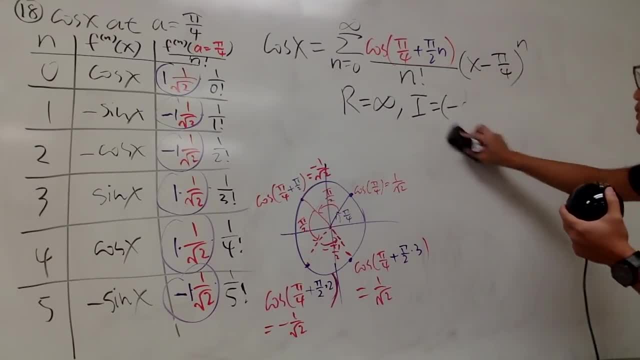 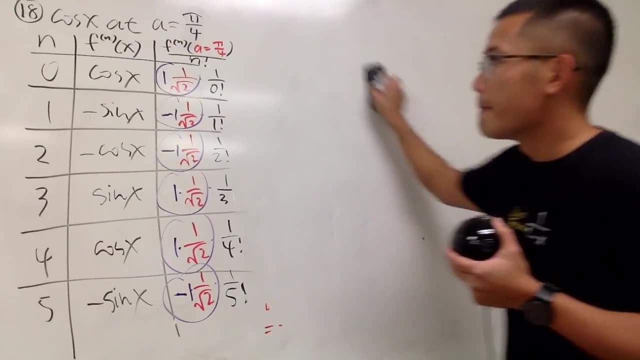 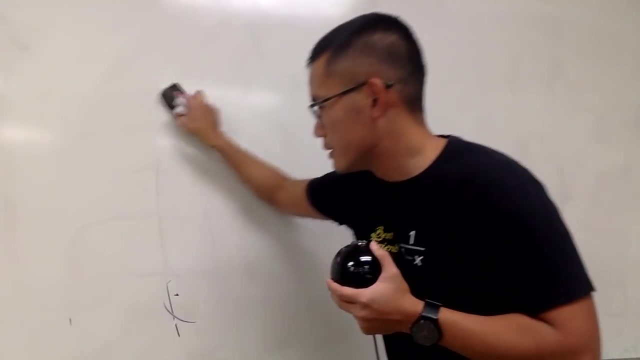 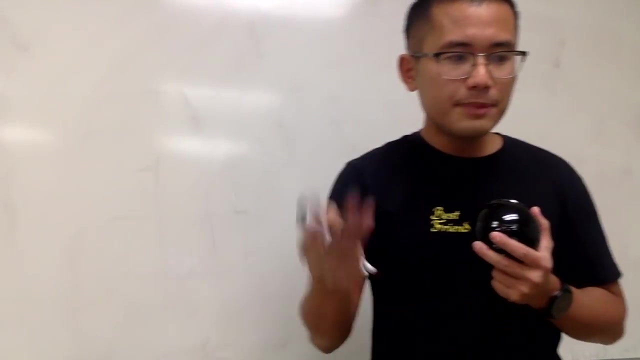 you should just work it out. But if you have a factorial on the bottom, it's actually just infinity. Just infinity, just worked out. Okay, Now I have 3 special functions to talk about Number 19.. Right, Number 19.. 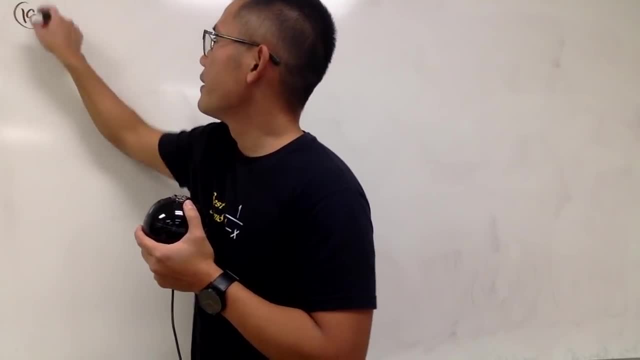 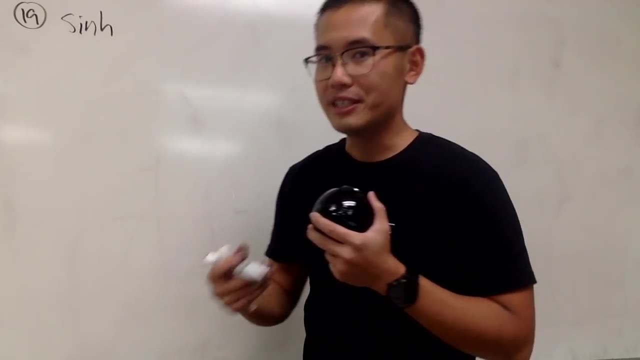 Oops, My bad. Number 19 here. This is the sign with an h next to it, And you can call this to be the cinch of x. Right, But don't worry if you haven't seen this before, because I told you guys the definition of this. 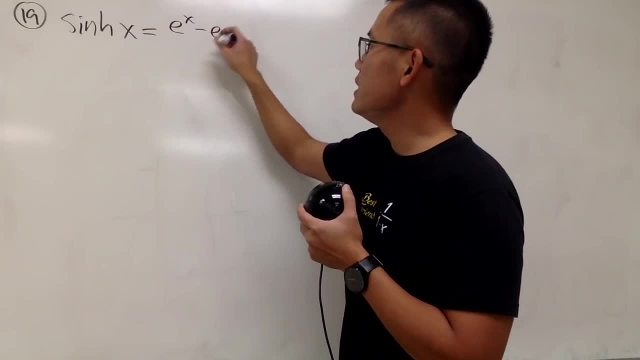 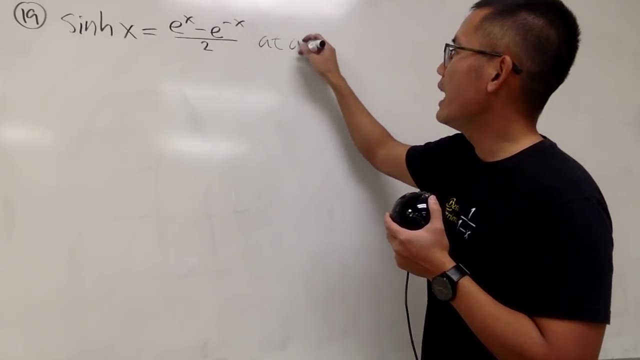 This right here is nicely equal to e to the x minus e to the negative x, all over 2.. Like this, We want to find a power series expansion for this at a equals 0.. Right, And maybe you haven't seen this before. 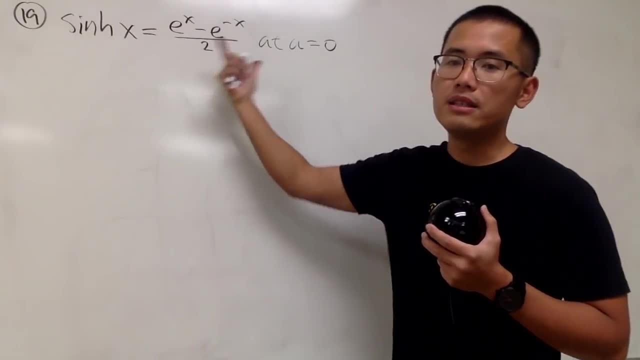 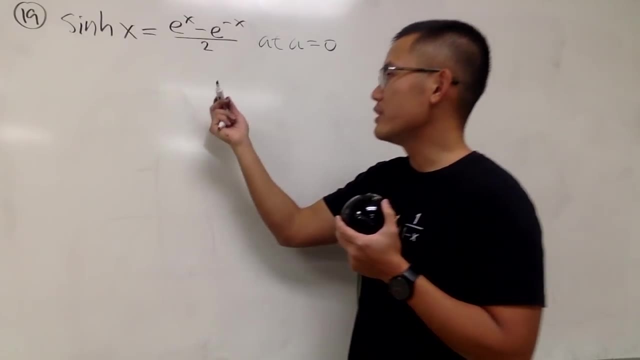 But it's okay, because you certainly have seen this Right. So all we have to do is use the e to the x to help us out for the power series. So we'll just look at this and just pretty much do the work. Well, I'll just write it down right here. 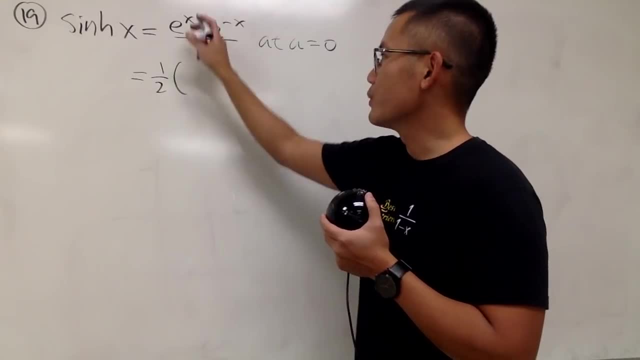 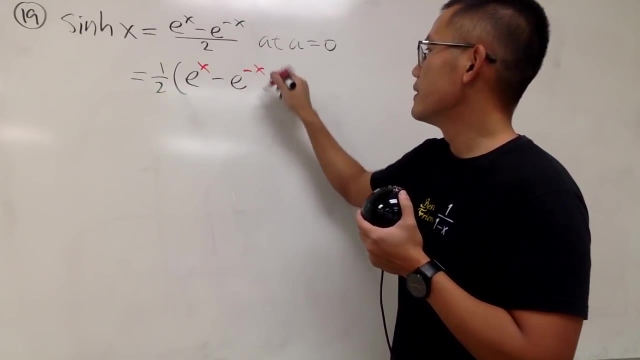 because we can write the 1 half in the front. So we can look at this as e to the x and then this is minus e and this is negative x, Right? So now we have the 1 half all the way in the front. 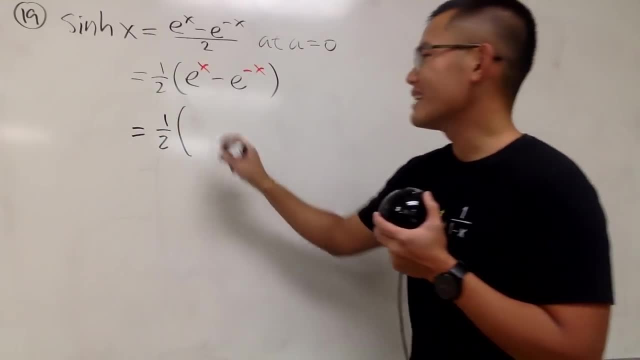 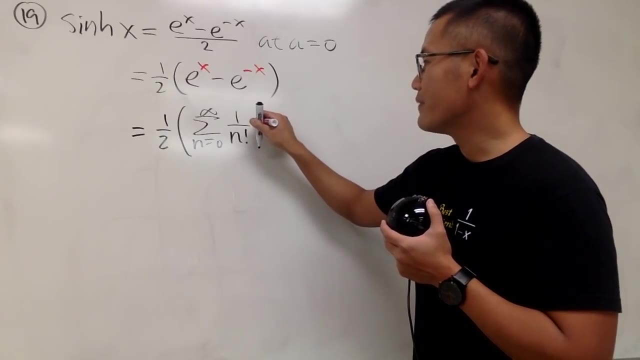 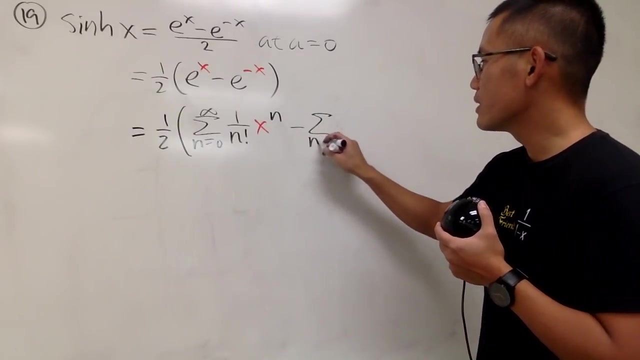 e to the x. you have to remember that this is the sum, as n goes from 0 to infinity. and you have 1 over n factorial and you have x to the nth power, Like this, And then minus the sum as n goes from 0 to infinity. 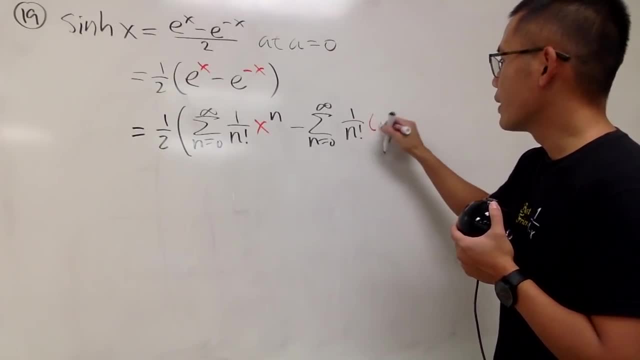 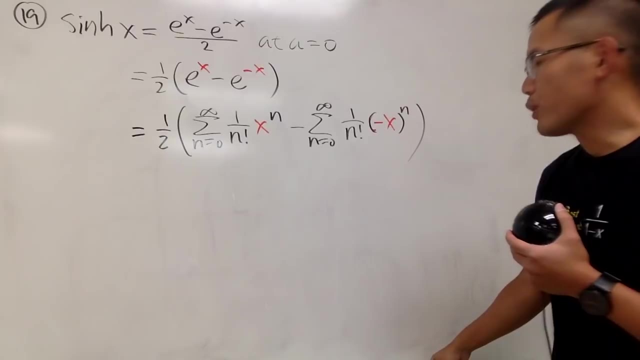 and you have 1 over n, factorial and I'll write it as negative x to the nth power, Like this, And it seems okay, But this is one thing I may, Let's see. Hold on, hold on, Let's see. 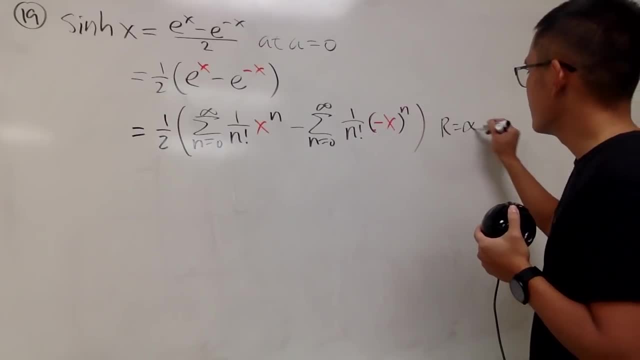 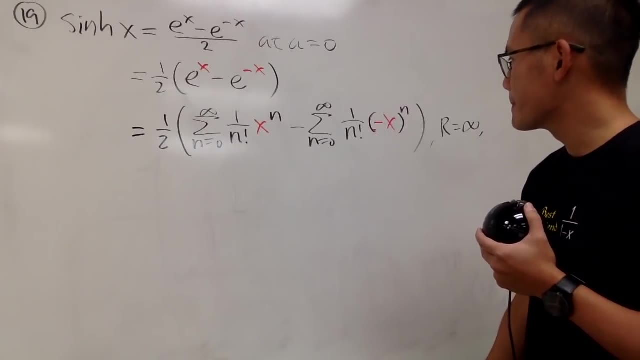 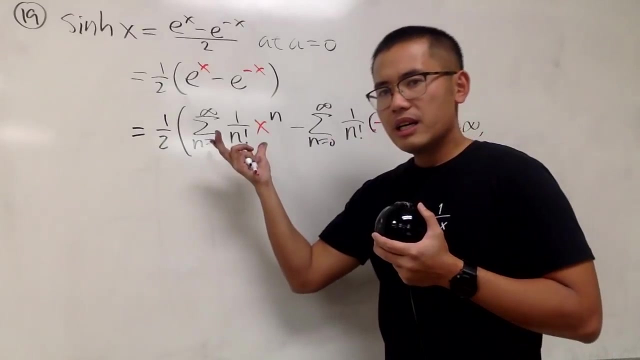 Hmm, Oh yeah. by the way, I should just write down: r is infinity, and of course we know that I'll put that down at the end. It seems okay. Hmm, Now, this is the bizarre part, okay, So just kind of bear with me. 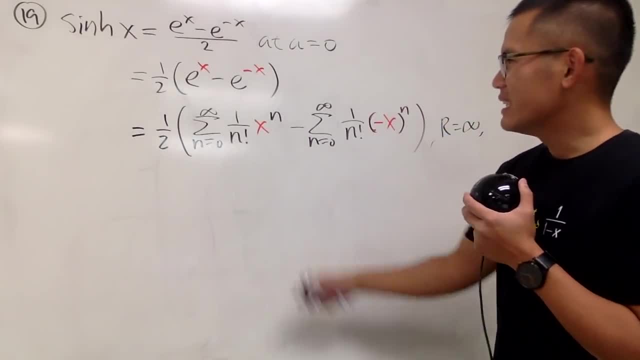 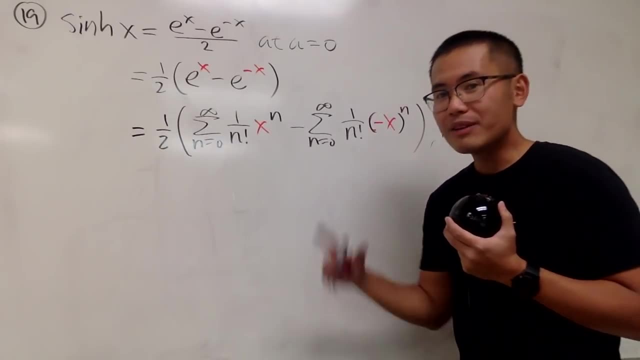 This right here is alternating. This right here is always positive And because they are of the same kind. so some terms are going to get cancelled and some terms are not going to get cancelled out. So we have to pursue this caution And depends if you want to stay with n or whatsoever. 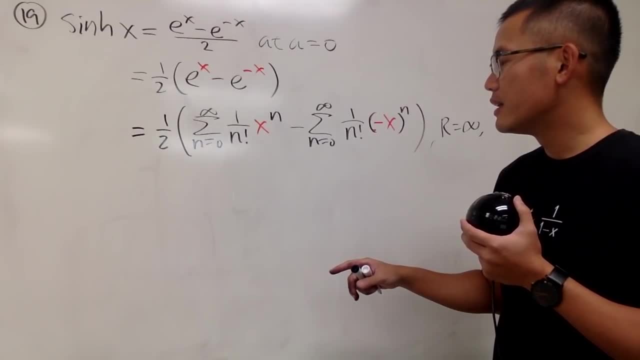 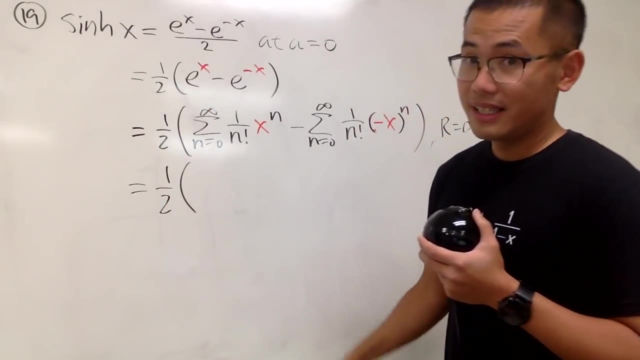 And let's do this, Let's do this, Let's do this One over two, That's one over two, Parenthesis that Let's just do the expansion. okay, So for this one, let's write it out: The first term, if you're putting zero in here and here. 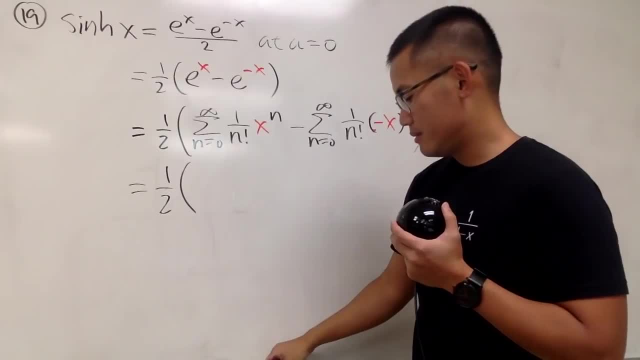 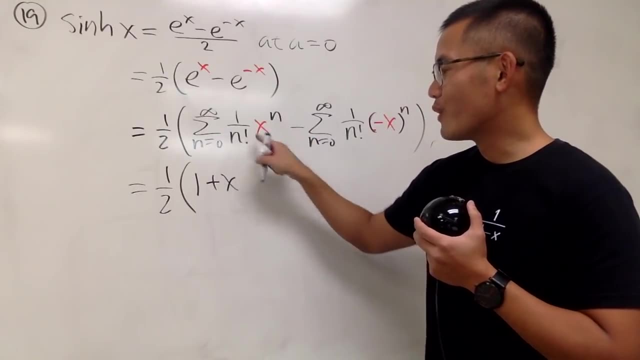 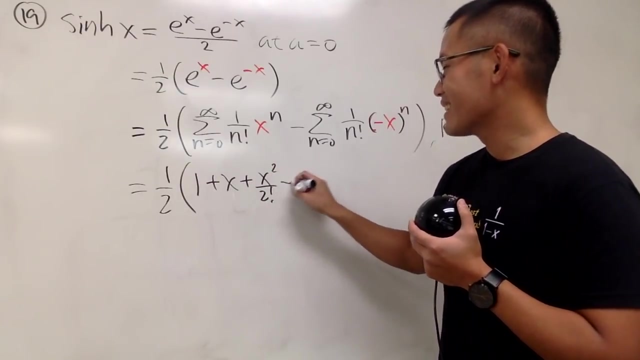 you get one. So I'll put this down in red In black: One. Next term you get plus x To the first over one factorial, so it's plus x. Next, you get x squared over two factorial. Next you get x cubed over. 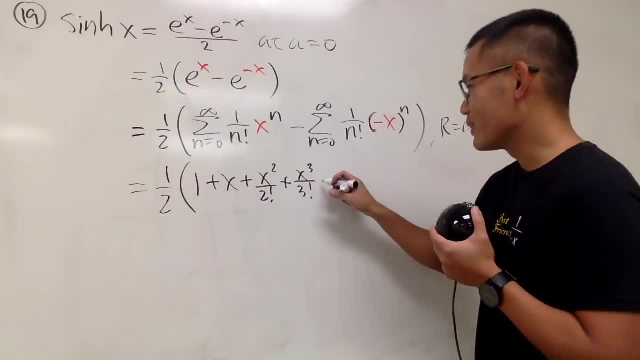 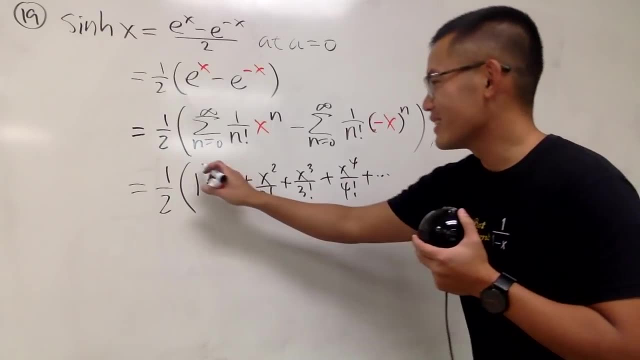 Over three factorial, And you guys can see the pattern. The next one is plus x to the fourth, over four factorial, And so on, so on, so on. So that's the first term, That's the first part, right here. Now we'll just put this down. 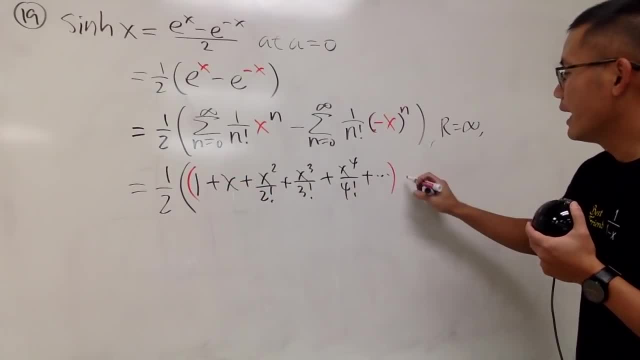 I'll put this down right here And then I will have to minus. Now, here is the small part. If you put zero in here again, you end up with one, So that's okay. Then if you put one in here, 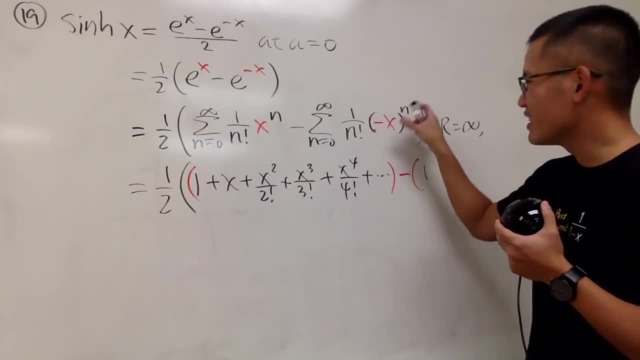 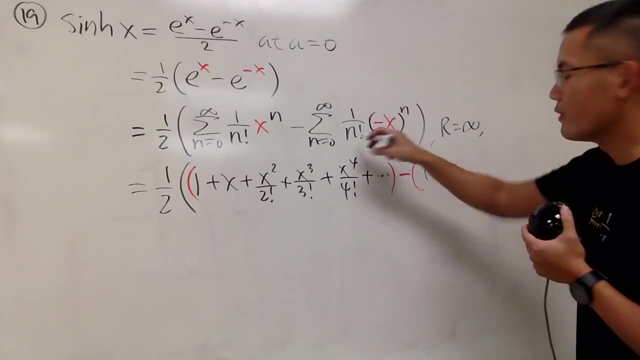 this is going to give you negative. It's going to give you negative one And negative one. Hmm, So it's a minus x to the first power over one factorial. So it's minus x, And then, when you put two, it's positive again. 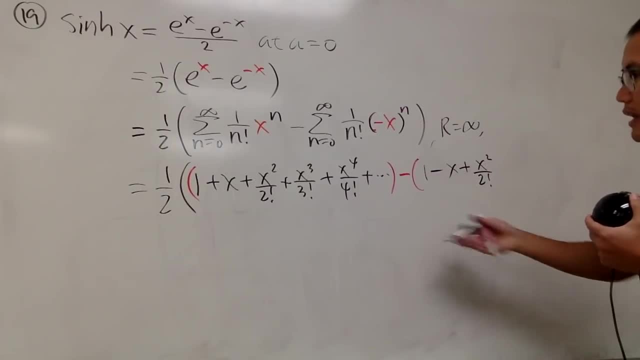 So it's plus x squared over two factorial, And you guys can see the pattern. It's an alternating version. So we have minus x cubed over three factorial, And then plus x, four over four factorial, And next one. Next one is going to be minus. 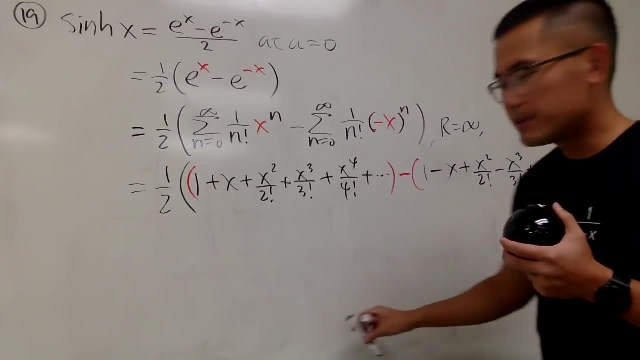 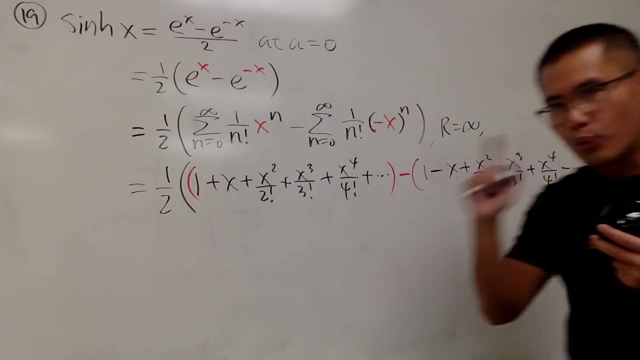 And so on, so on, so on. All right, So that's pretty much the expansion. if you write it out. And now check this out, We have one minus one. We know one minus one is equal to zero. So go ahead and cancel them out. 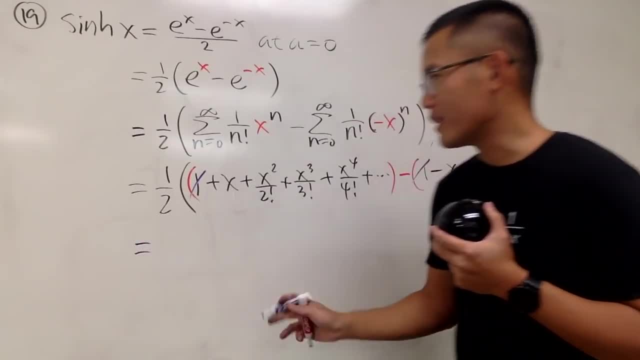 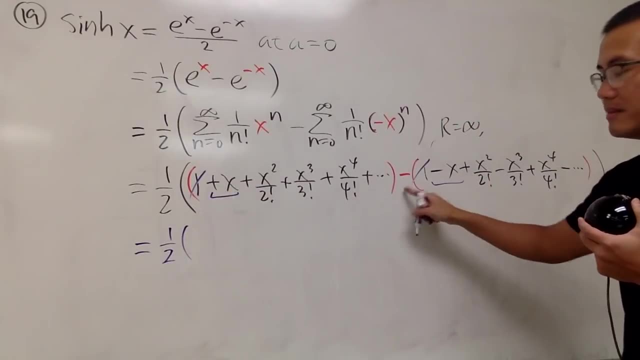 Then I will put on everything purple from now on. This is one half times, This is x, But minus negative. x minus minus becomes positive. So we end up with two x, All right, And then next you see, this and that minus. 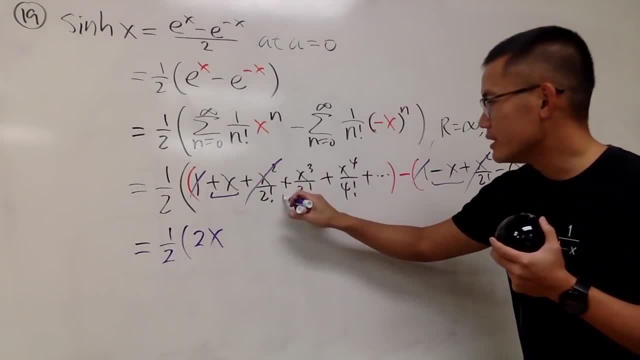 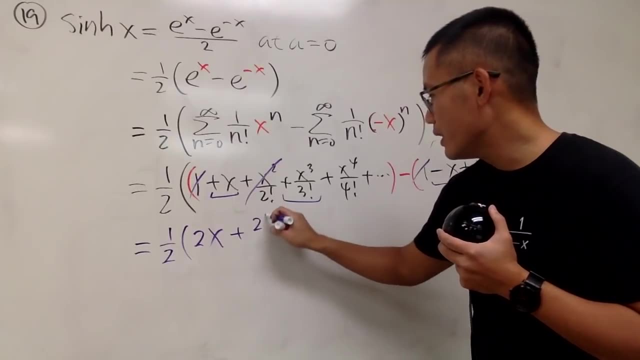 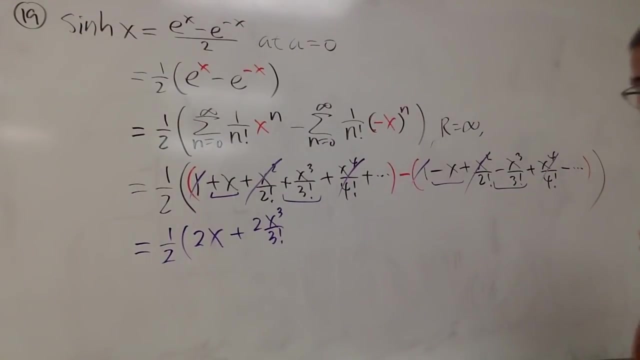 So they cancel out. And then next you see this and that, Well, we get two of them. So let me just write it as plus two x cubed over three factorial, And next this and that will cancel out And, if you would like, you see that this and this will maintain. 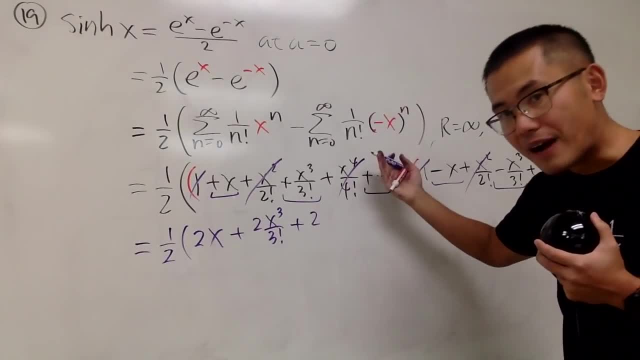 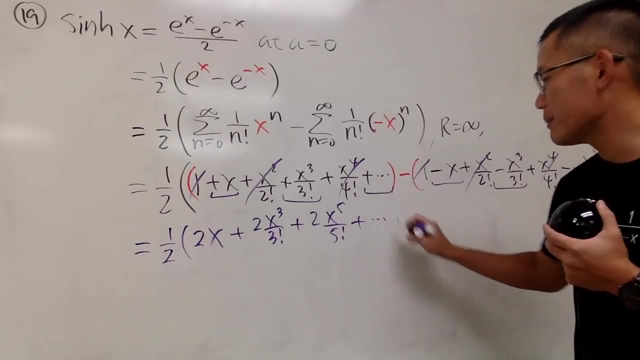 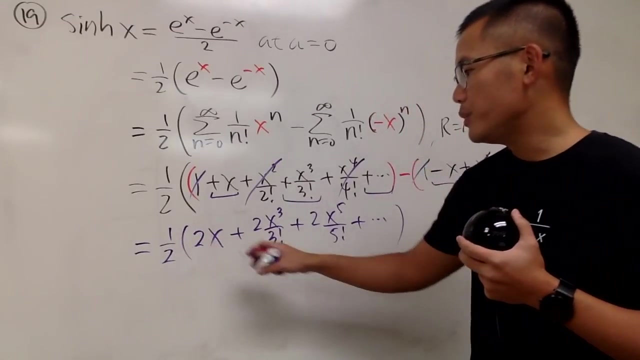 And that will have been two x to the five, x to the five over five, factorial. All right, So two x to the five over five, factorial, And so on, And just keep adding them up. All right. Now the good thing about the one half in front is that when you distribute, all the twos will be gone. 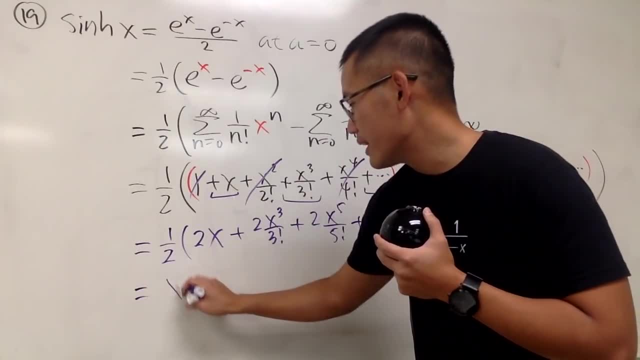 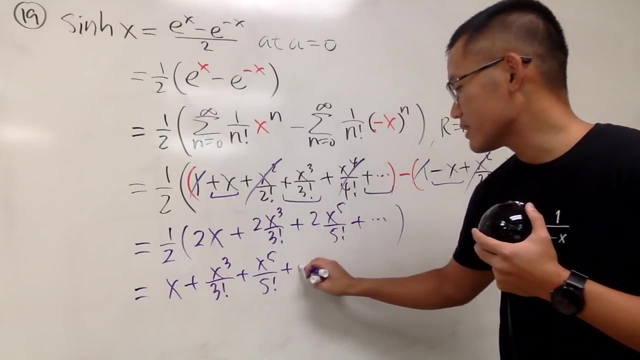 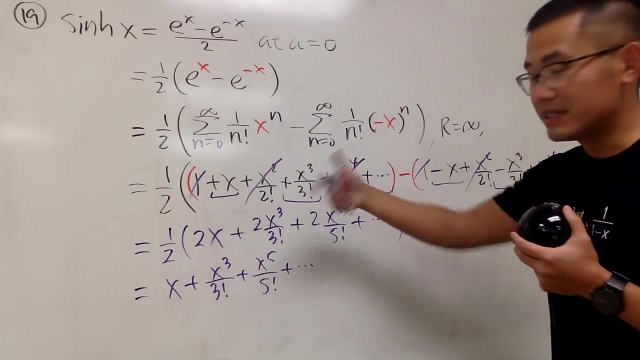 Isn't it? So if you look at all this, you get x plus x, cubed over three factorial plus x to the five over five factorial plus dah, dah, dah, Whatever. Here is the video. I'd like to just show you guys the expansion for this, because the terms will cancel out. 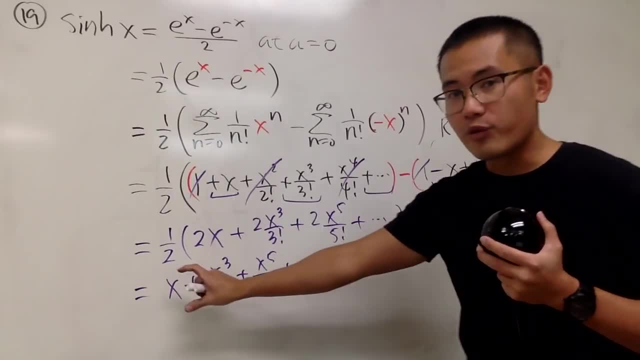 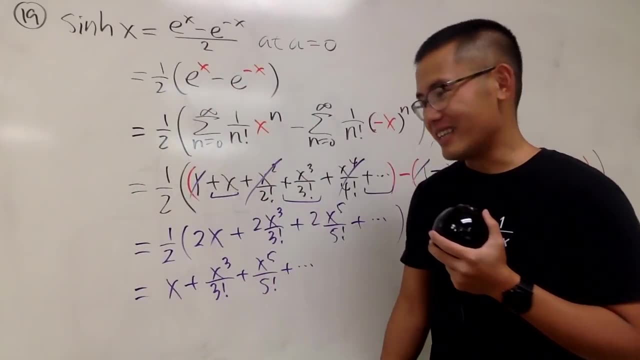 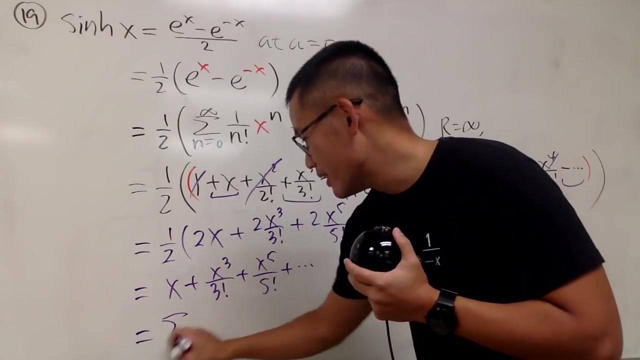 And of course, you don't want to write the zeros out, You want to just write down a formula for the remaining things That's very similar to the original sign. This is the hyperbolic sign called sinh. Truth is, if you work this out, if you put it in the sigma notation, it does not alternate. 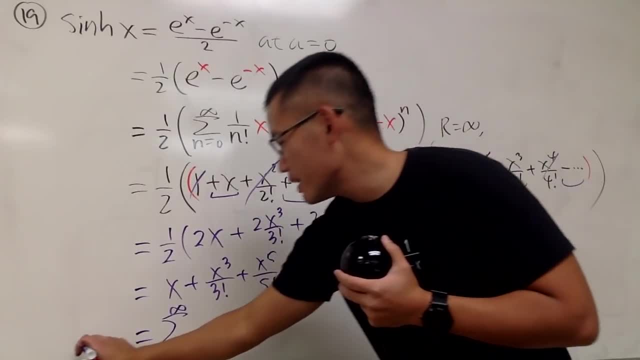 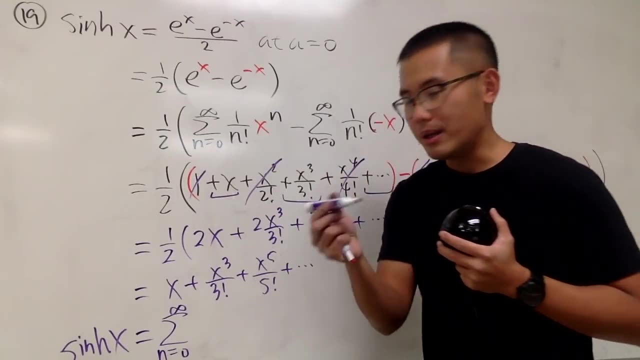 This is n going from zero to infinity. All right, This is the sinh x. Notice this n. it's very different. this n I put it in blue, I put it down purple. Okay, So I know, this is the index situation. 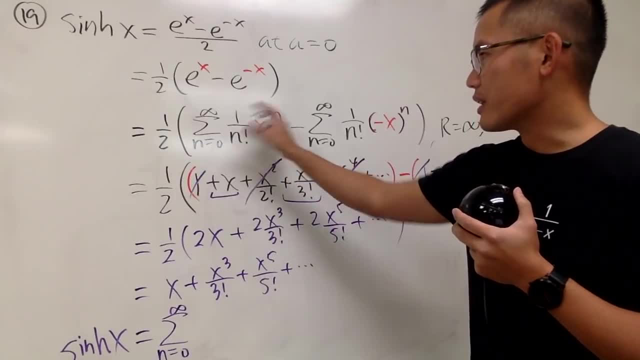 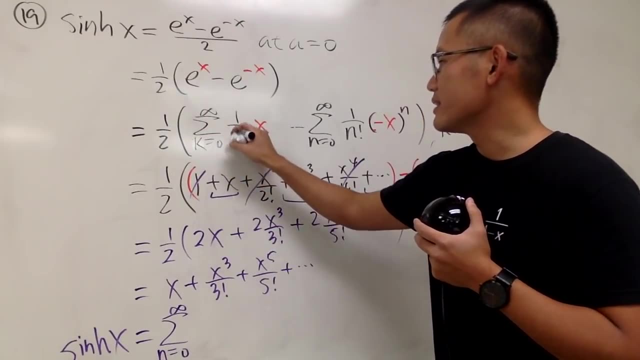 That's horrible sometimes, But if you didn't like the confusion, you can just change all this to k. If you didn't like the n that I used, like twice And it's like why it looks different, So just change this to k. 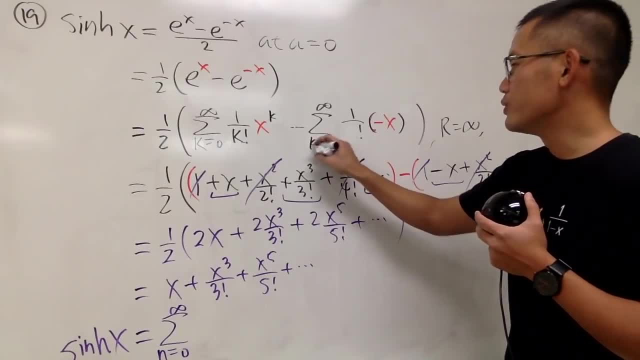 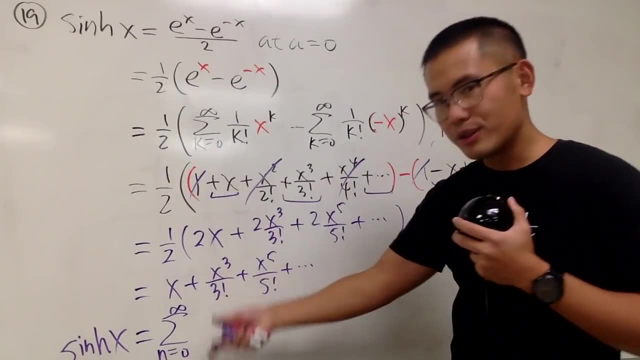 That's pretty much what I was doing with the original sign- The original sign question- earlier. It might be confusing, but once you get used to this you can do it too. So now there's no debate about the n or the k. 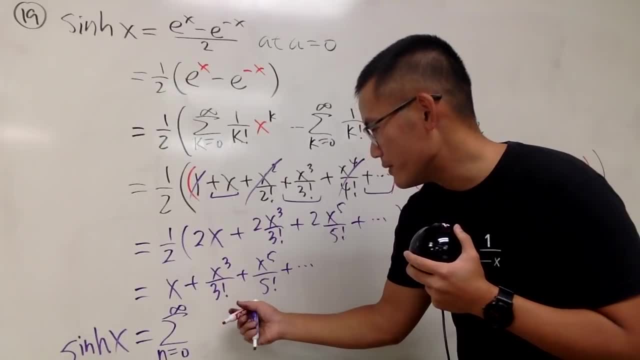 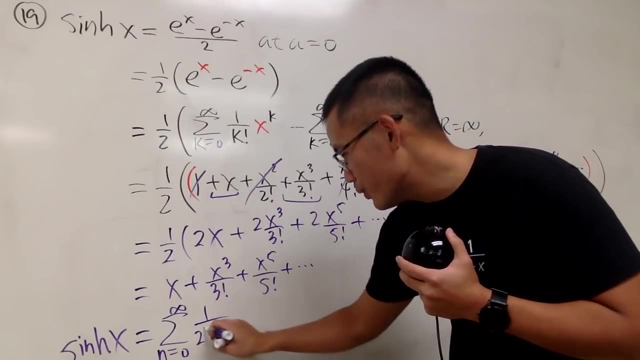 Anyway, nothing is alternating. This right here is just going to be the following: We only have the r numbers, the factorials and all that. So we have 1 over 2m plus 1 factorial and then times x to the 2m plus 1.. 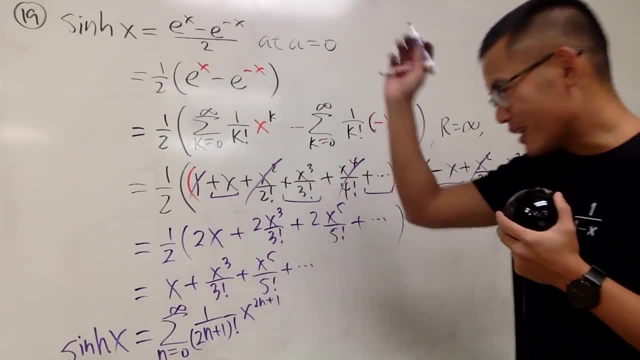 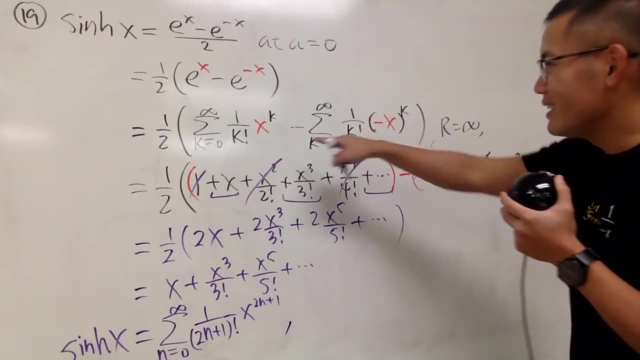 Just like this. There's no alternating. That's the sinh x, ladies and gentlemen, And you can guess it: if you run through the Oh, you actually don't need to run through because you know from e to the x, You know r is infinity. 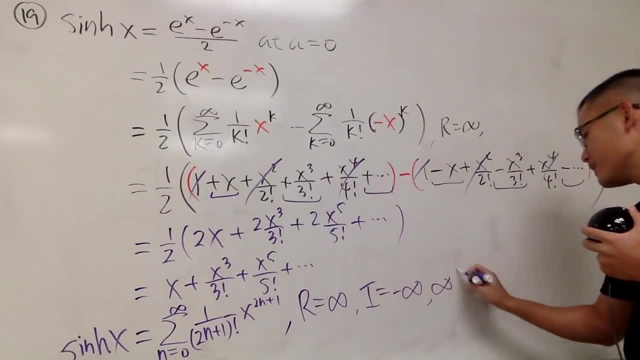 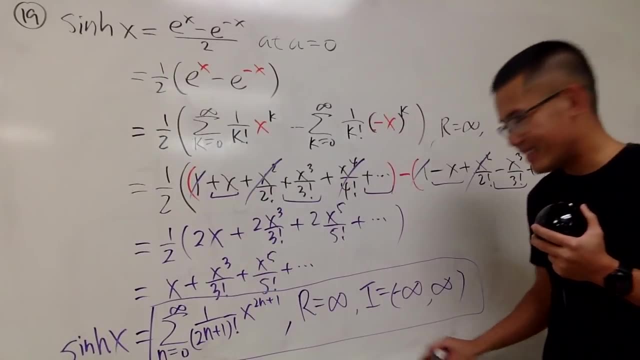 Likewise, i is negative infinity to positive infinity. Do not include infinities. Here you go. This is the answer for the sinh x. Okay, Very nice, isn't it? Now I will do number 20, because you might guessed it. 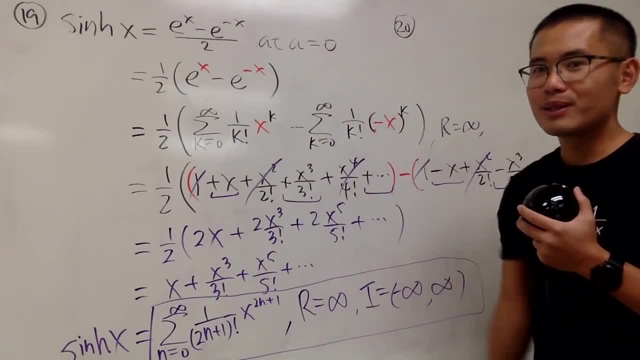 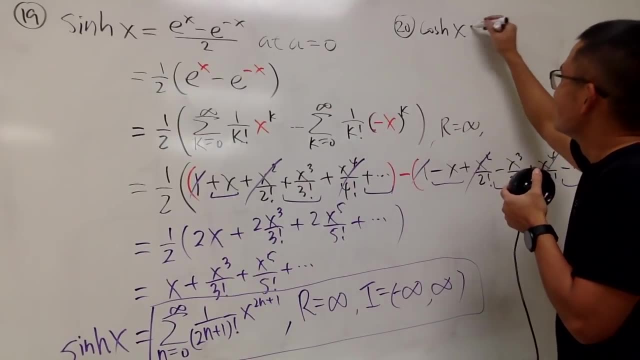 What number 20 is. Yes, it's the hyperbolic cosine for it. So let's look at cosh. If your name is Josh, shout out to you. But this is cosh. e to the x plus e to the negative, x all over 2.. 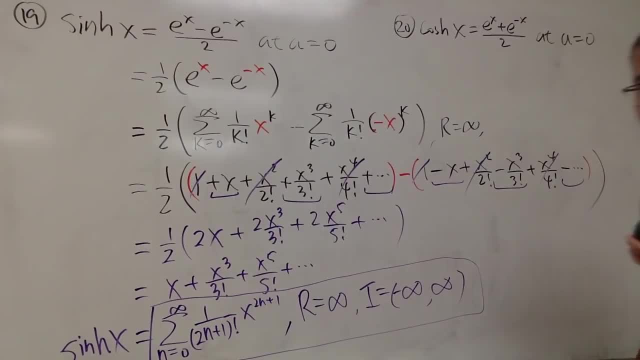 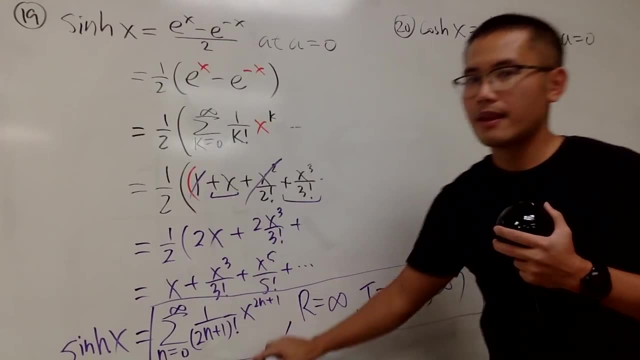 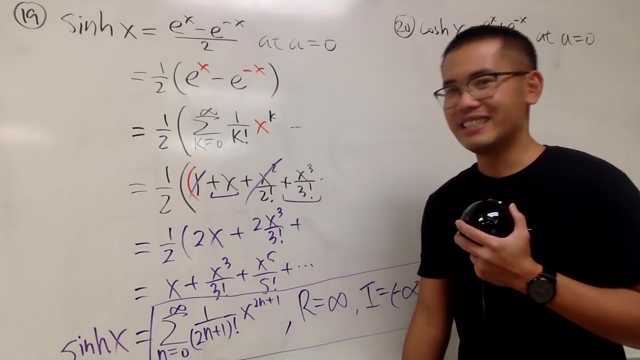 And a equals 0.. I will erase this a little bit, though Hopefully you guys don't mind. Well, is there any connection between sinh and cosh in terms of calculus? Of course there is Derivative, But what kind of derivative is this? 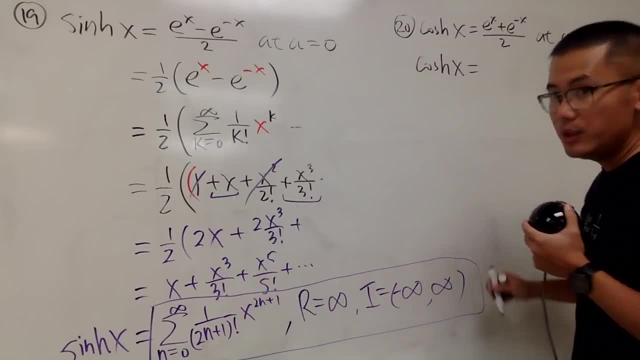 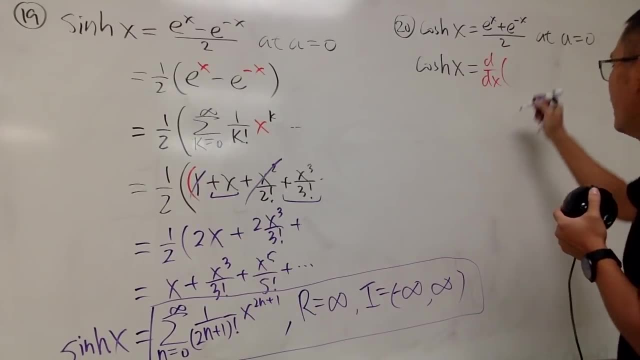 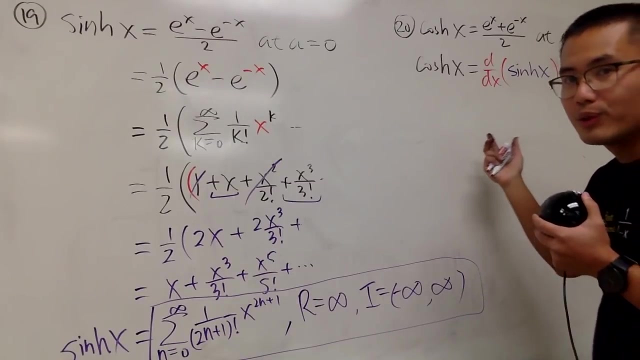 Well, the truth is, cosh of x is indeed equal to, if we differentiate sinh x. This is correct. Okay, So this is true. What we can do is: you can just go ahead and do the derivative right here. The one-half stays. 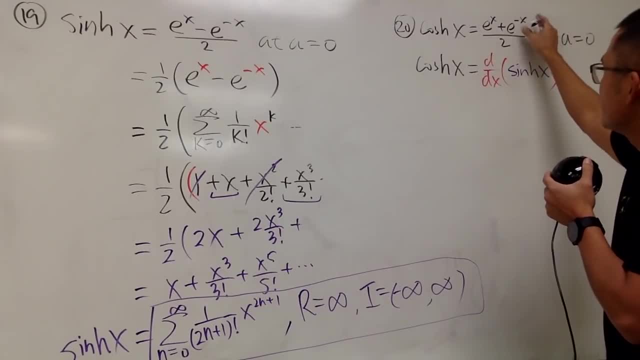 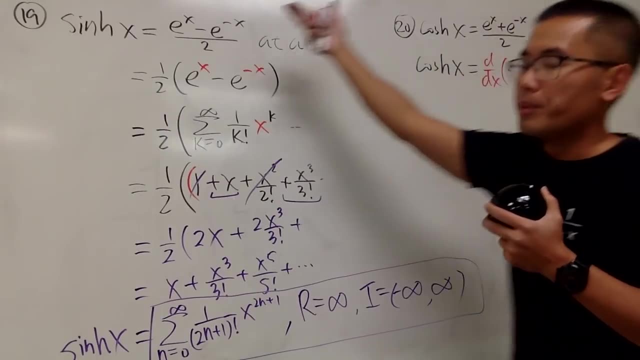 e to the x stays, The derivative e to the negative x stays, But don't forget to multiply by negative 1, because of the chain loop. So you have the negative right here, And that will be sinh. And here is the beauty, though. 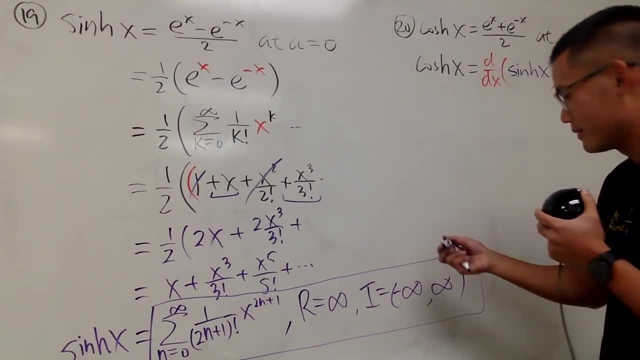 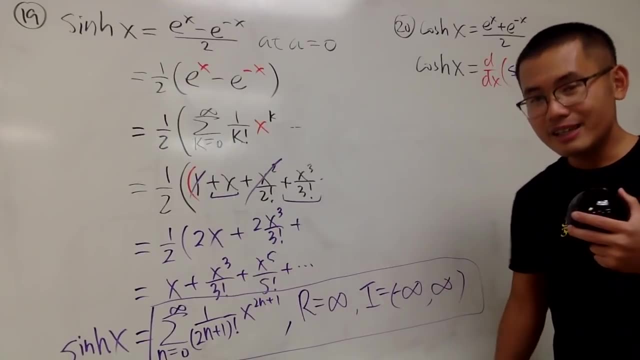 I will just actually tell you guys the following. I will just put it down right here somewhere: If you differentiate cosh, you get sinh as well. There's no negative. Derivative cosh is positive sinh And derivative sinh is negative. 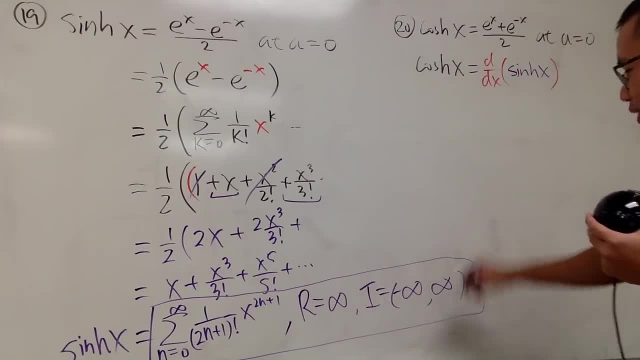 Derivative sinh is positive. cosh, Just go ahead and try that out if you would like. By the way, my job is to do the power series, So we will be differentiating sinh x, which is that over there. I will just write down the sum. 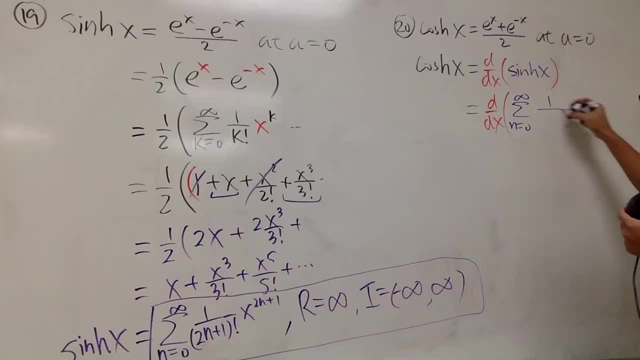 n goes from 0 to infinity And we have 1 over 2n plus 1 factorial this guy and x to the 2n plus 1. And we know r is infinity, So we will just put that down later. 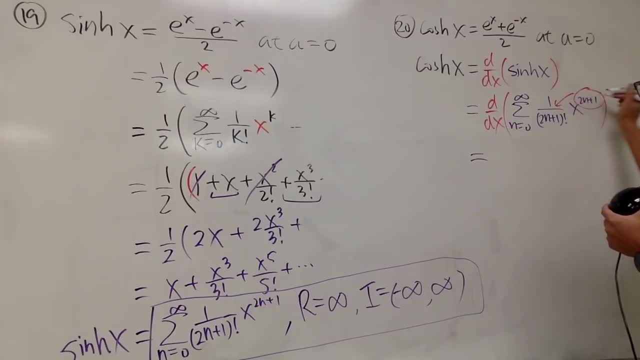 This right here is equal to well. do the derivative. Bring this to the front: Minus 1.. So you are looking at 2n plus 1. Break this down: This is 2n plus 1 times 2n, and then so on, so on, so on. 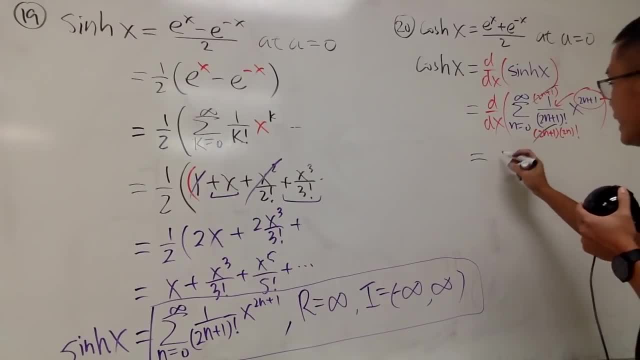 So you can factorial this, So this and that will cancel And in the end you end up with the sum n goes from 0 to infinity, positive 1 over 2n. factorial this guy, And then this is just x to the 2n. 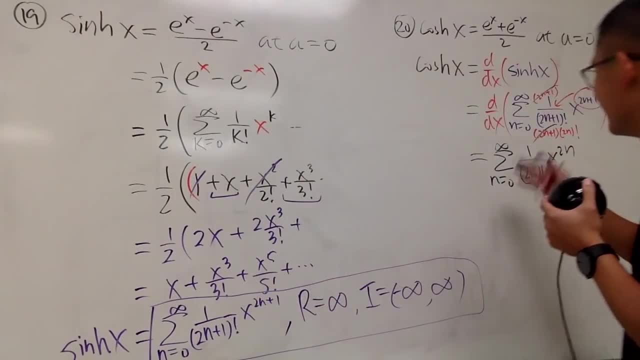 Yes, this is the cosh, And you don't have to alternate at all. And similarly, the r is infinity, i is negative infinity to positive infinity, And you can be happy, I can be happy too, because we are done Right. 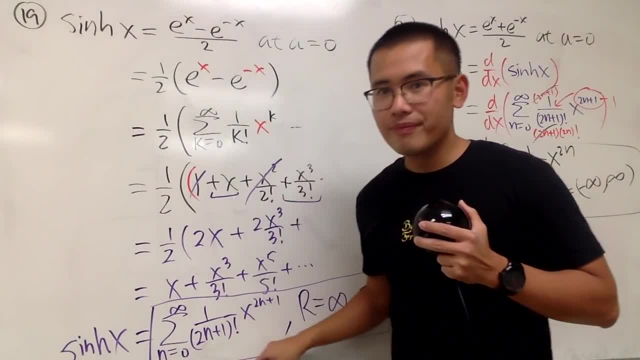 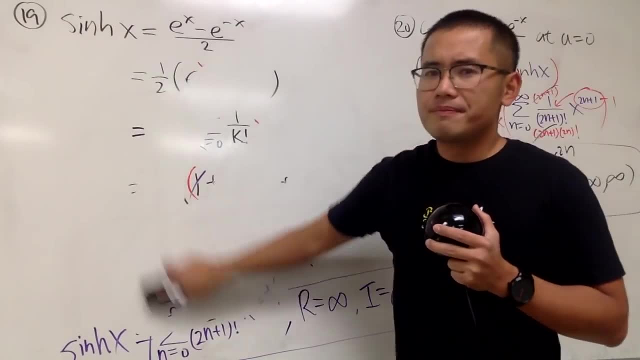 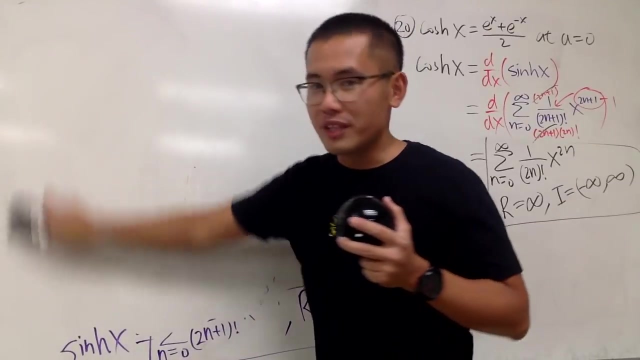 So, ladies and gentlemen, this is cosh, And you might be wondering how come we didn't do the original tangent? Because there's no easy formula. There is a formula, but there's no easy formula for the original tangent. That's why we only did the inverse tangent. 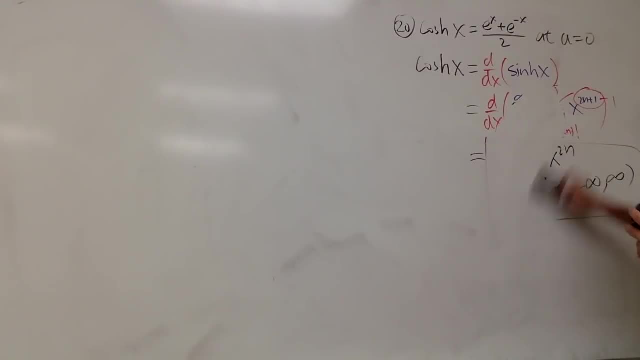 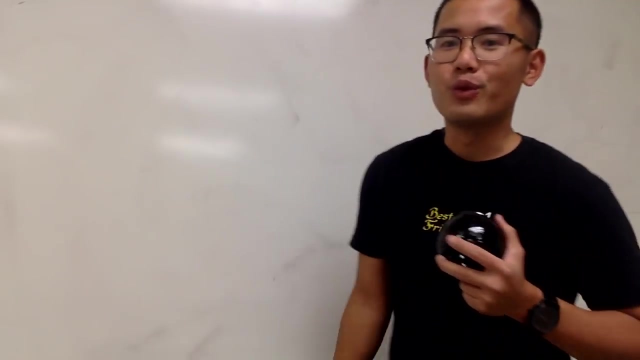 And for the tangent, if you really want to get a power series for that, you can do long division with sine over cosine, Or you can do the Taylor formula. So up to you. Now we have a couple more to go. 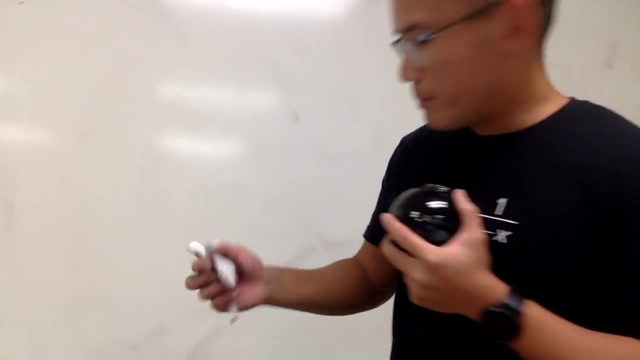 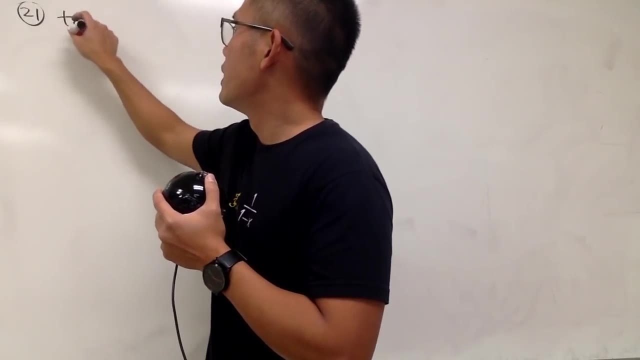 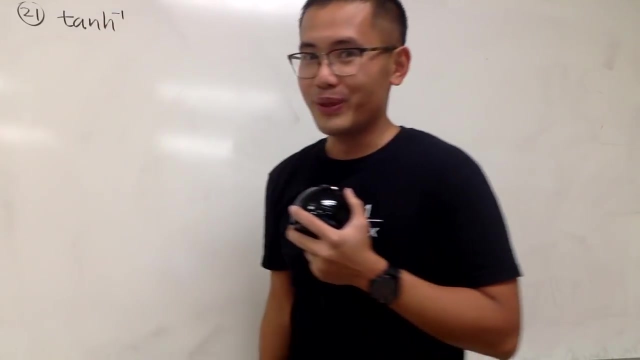 6.2. more to go, So number 21.. Inverse tangent, So number 21.. This right here is the hyperbolic tangent, But it's the inverse version of that, So I'll put a negative one right here of x. 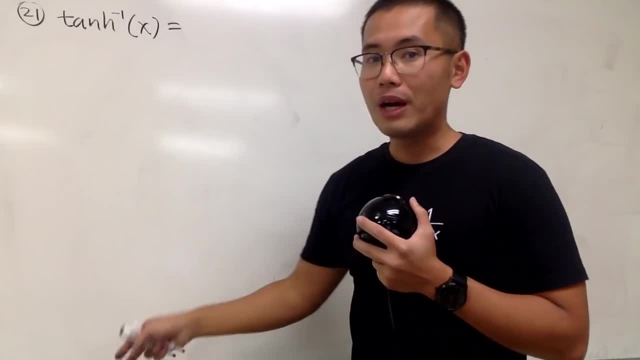 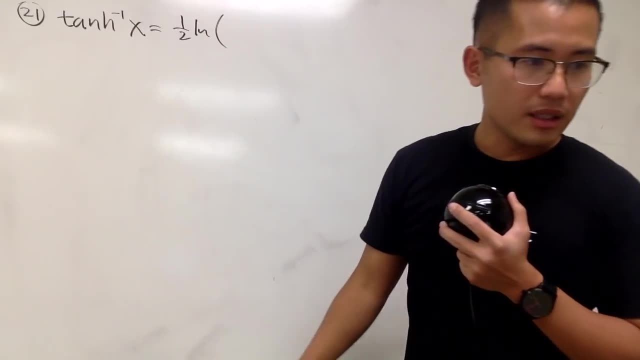 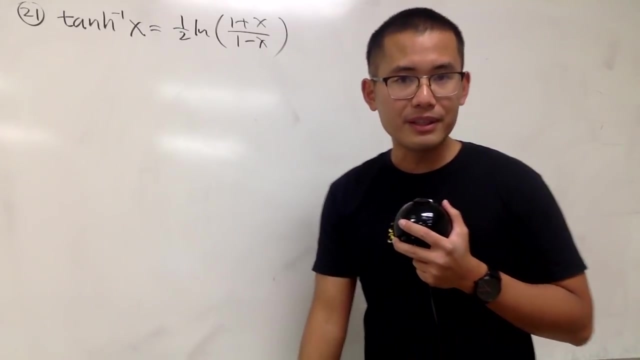 Don't worry, because right here I will have to tell you guys what the definition of this is. We don't need parentheses. This is 1 half natural log And we have 1 plus x over 1 minus x. So that's the inverse hyperbolic tangent. 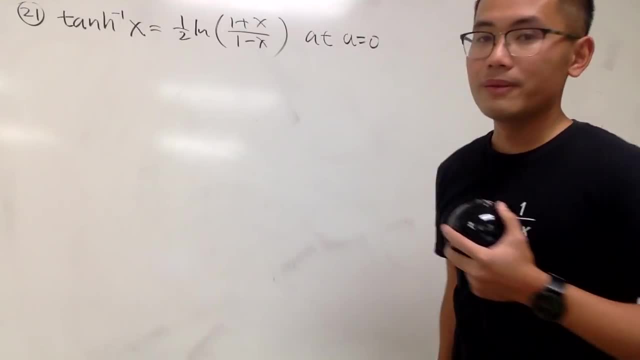 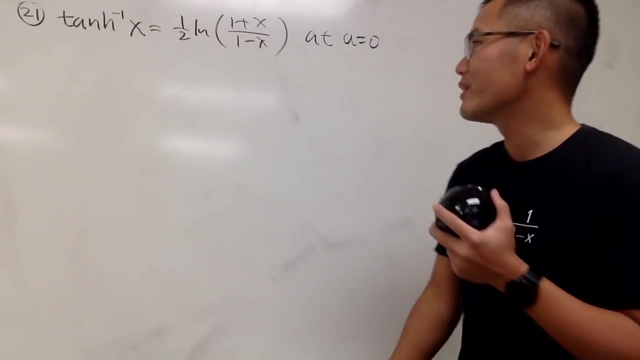 And we want this at a equals 0.. We may not know this too well, but we do know this very well. So attack this right here. right, So here we go. This right here. Division inside: we can just break down into two parts. 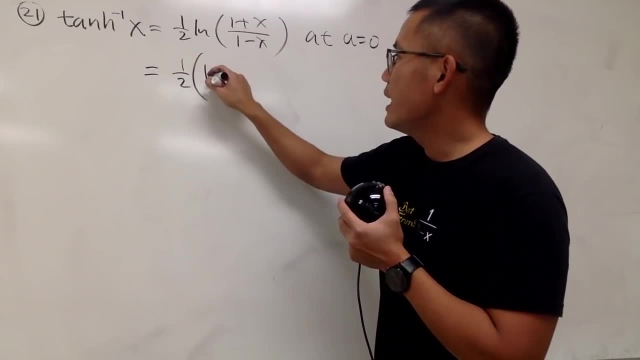 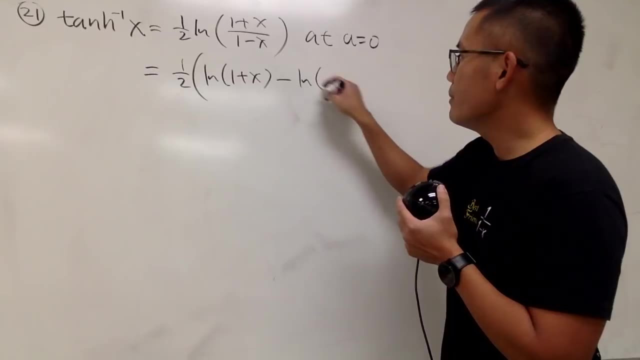 So here we have 1 over 2.. Parentheses that ln First thing is 1 plus x. Hey, don't we have this? Yes, we do right. And then minus ln: 1 minus x. 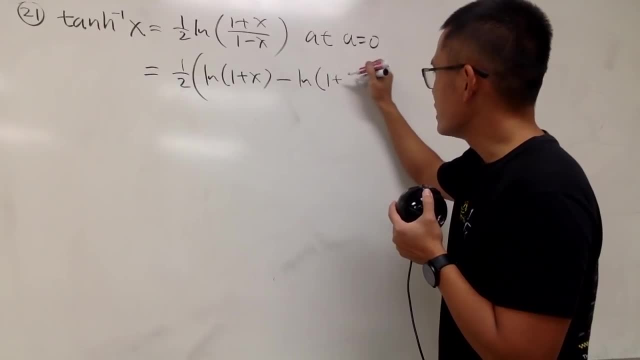 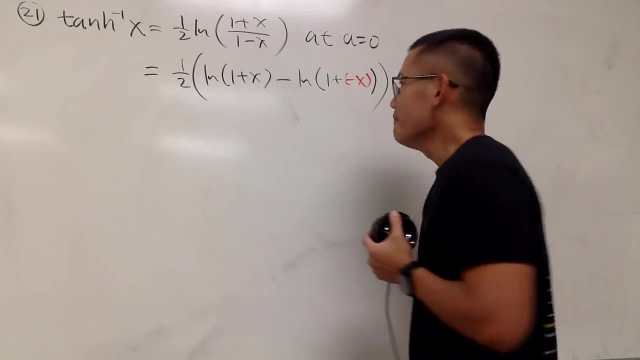 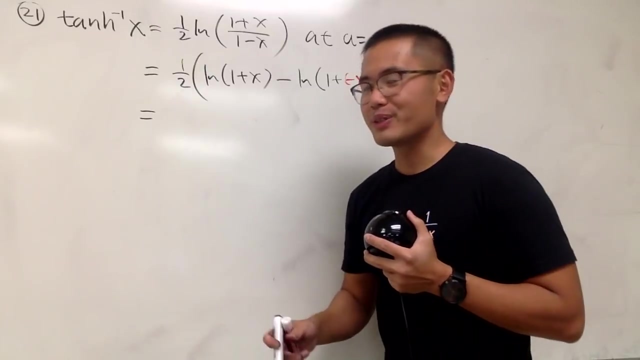 Like this, So I will put it as plus a negative x. Yeah, Okay, Ah, man, I know my power series. Okay, I will try, I will try, I will try, I promise I will try. Here we go. 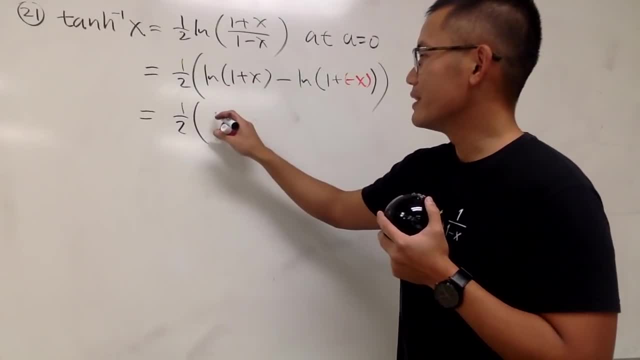 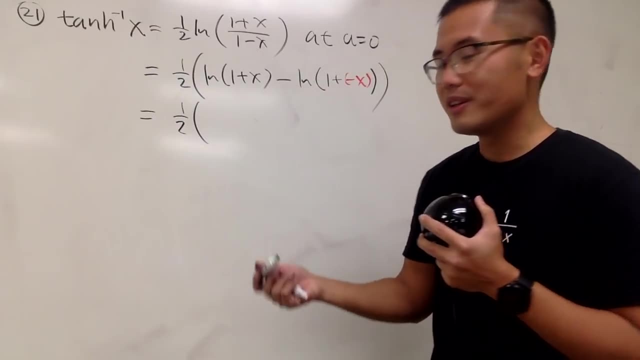 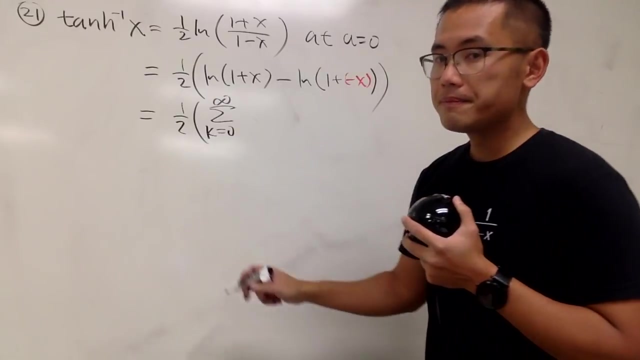 This is 1 half And this right here. the first thing is, let me just write it out And maybe it alternates again, so I will write it as k, just to avoid confusions earlier. So here I will just write: this is the sum as k goes from 0 to infinity. 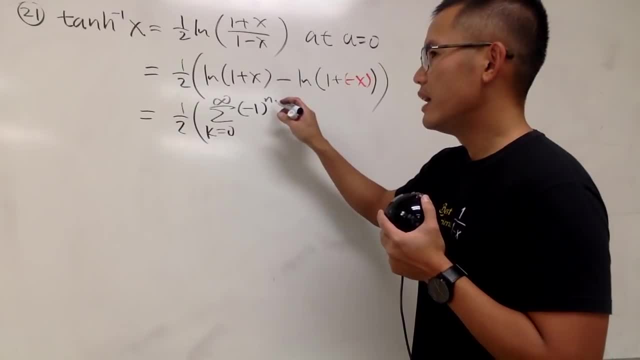 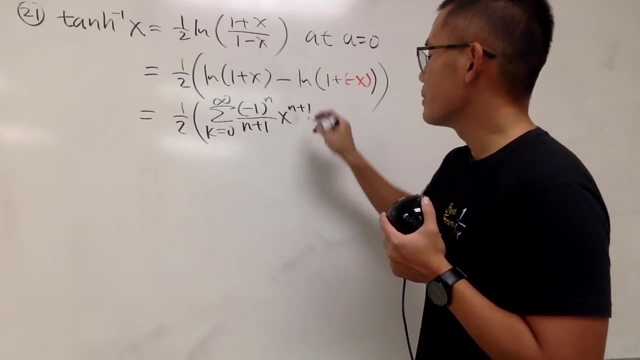 It does alternate And that's negative. 1 to the n And yeah, And then over n plus 1, x to the n plus 1 power, Because you have to integrate the best friend's cousin, right? So that's what we got. 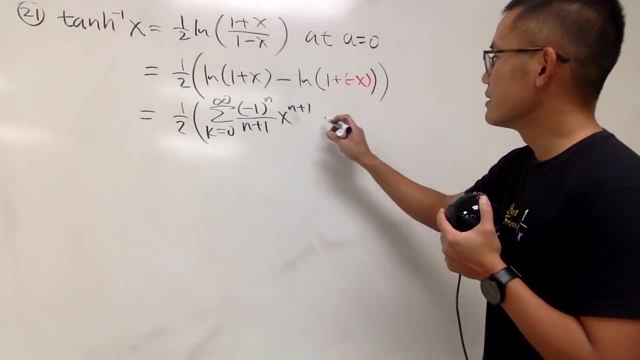 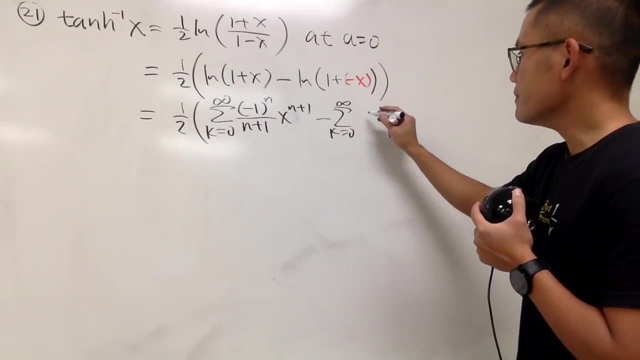 And yes, Yeah. Next, this is minus And we have the sum as k goes from 0 to infinity And we have negative 1 to the nth power Over n plus 1.. But we enter this right here, so we get negative x to the n plus 1's power like this: 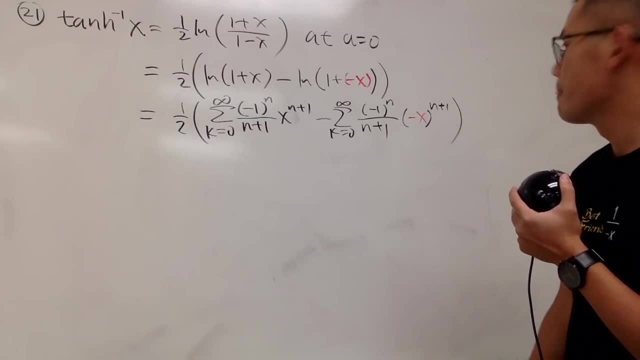 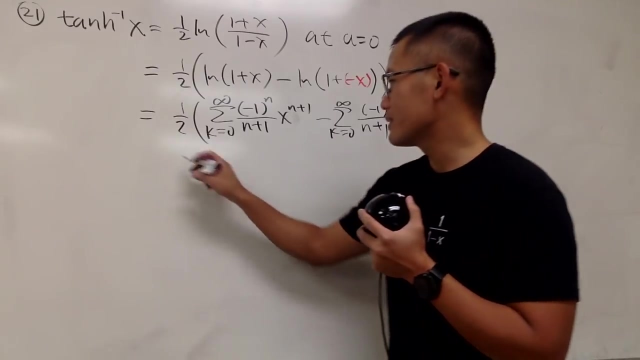 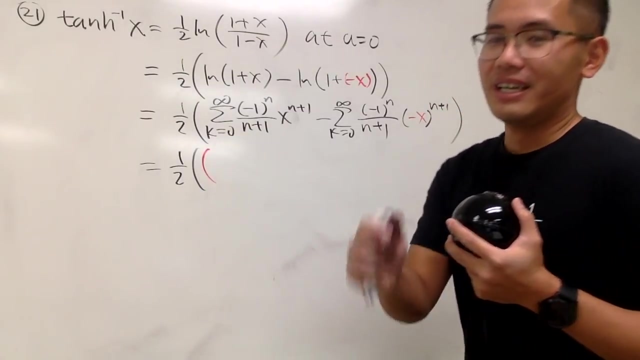 Okay, But again they just like to alternate. you know that, Yeah, So let's just go ahead and write down the terms, Right, Shall we? Okay, Here we go, And you guys can tell I'm kind of tired because, yeah, this is 9.21 pm, right? 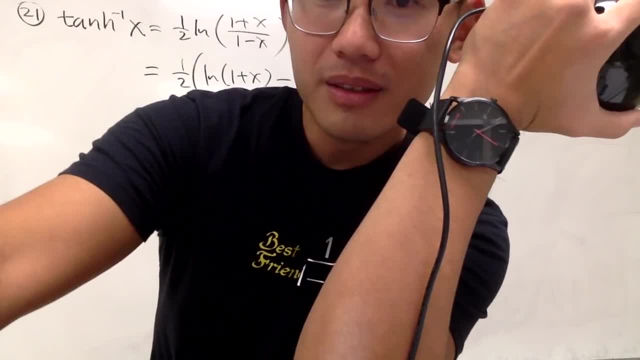 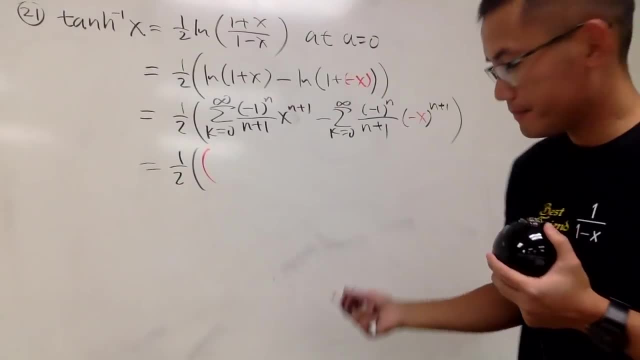 9.21 pm. You guys can see. So here we go. This is going to be kind of weird, But we will do it anyway. Yeah, We'll see. Okay, What k Whoops Man. 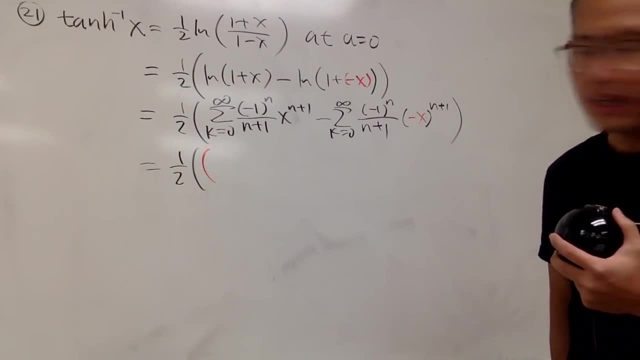 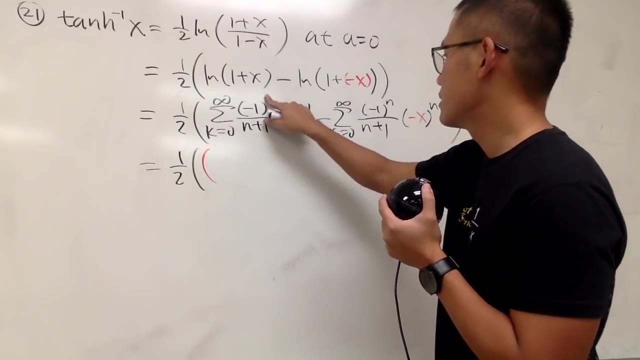 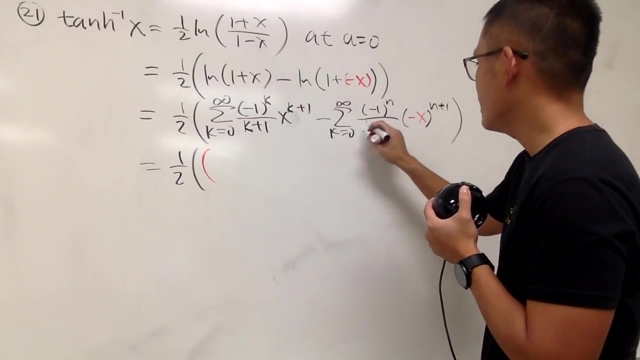 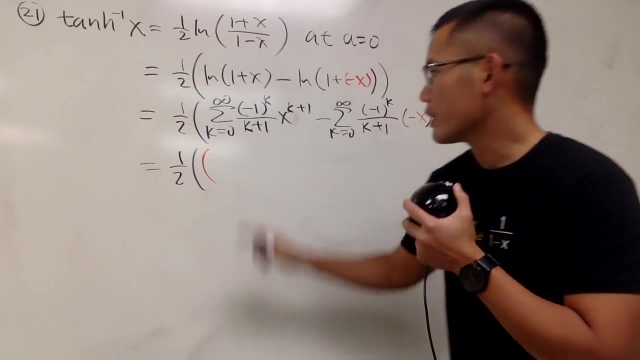 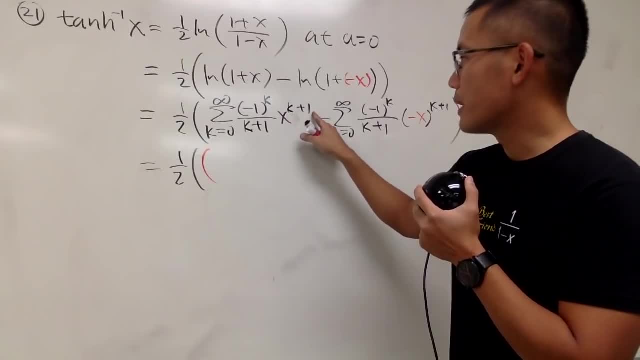 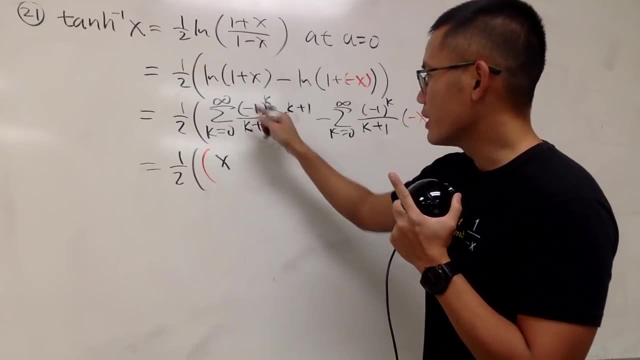 When k is 0, you put it here, put it here, you get x to the first power, yeah, and 0 to 1, so you have x. So that's the first term. That's good. Now, when k is 1, you put it here, you get negative and you get 1 plus 1, which is 5.. 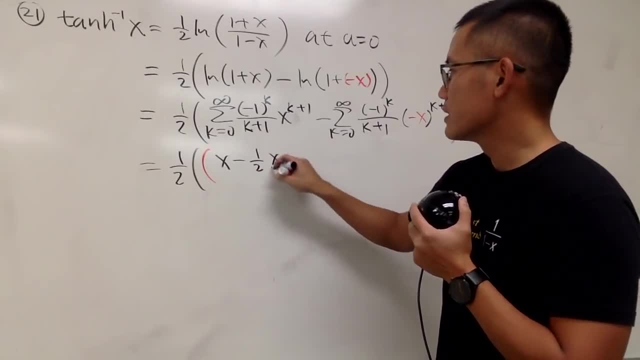 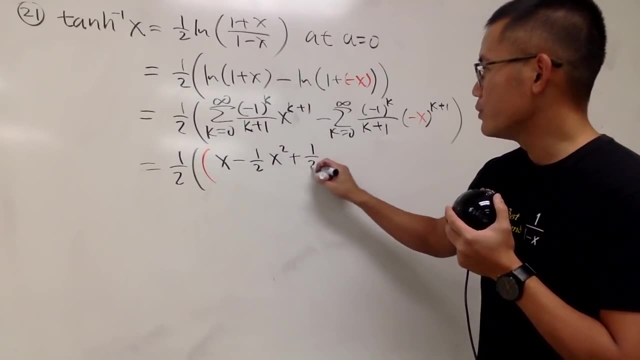 which is 1 half, and then you get x2, yeah. Next, when k is 2, this is going to be positive, and then that will be 1 over 3.. When k is 2, you get x to the third power. 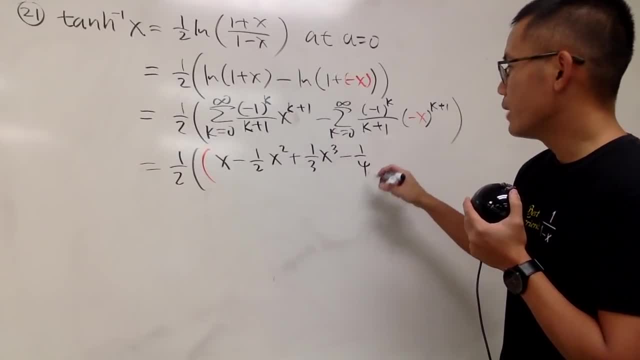 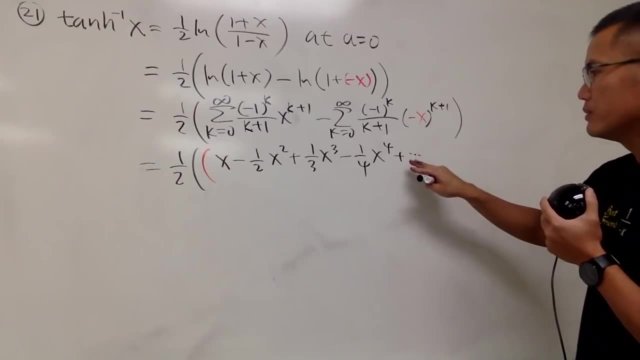 And if you do it again, you get minus 1 over 4, and you will have x to the fourth power and plus, so on, so on, so on, And perhaps let's do one more just to be safe. So plus 1 over 5x to the fifth power. 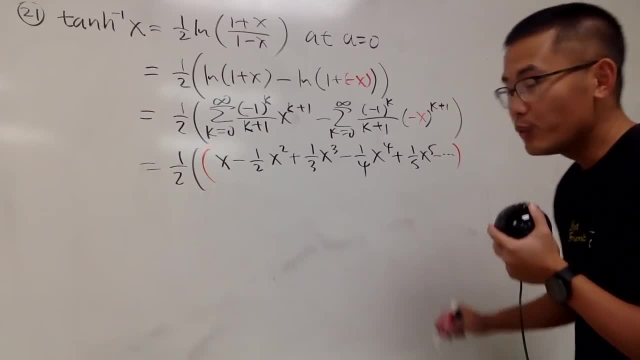 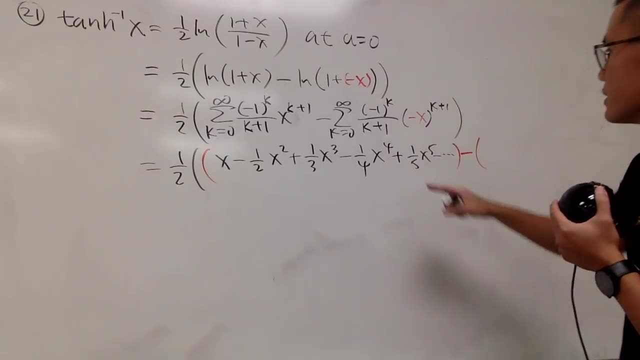 and then minus, so on, so on, so on. Okay, Then we are going to minus. Man, this is going to be the opposite of all that. so you actually start with negative first. If k is 0 in here you see negative x to the first power. so it's negative x. 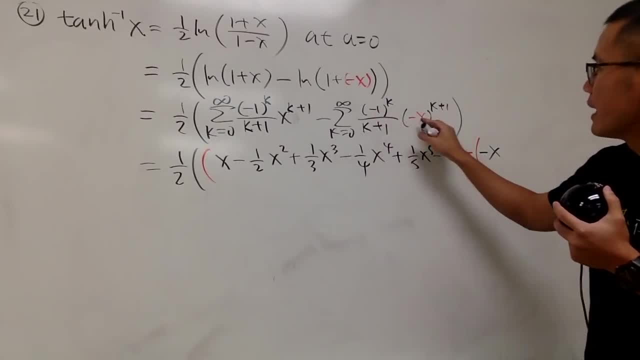 And if k is 1, well, this is negative. now it will be negative x. so that will give us, if k is 1, this will be this to the second power. so, Oh, let's break down Man. let me just break down the power here. 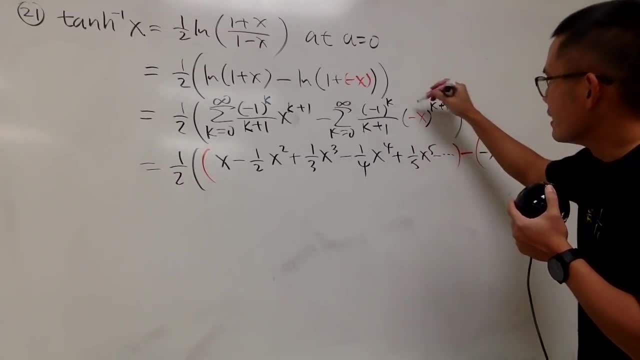 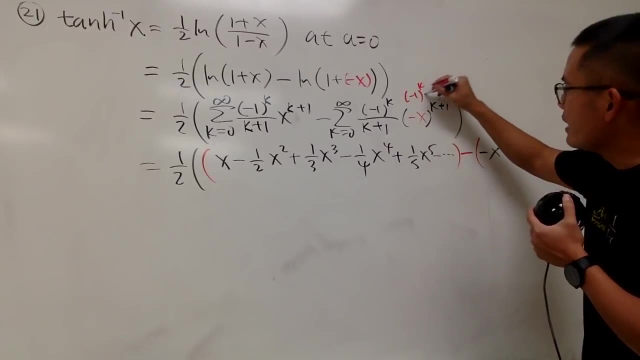 This is kind of confusing. So this right here, all right. This right here is the same as saying negative 1 to the k plus 1 power, right. So it's the same as negative 1 to the k times negative 1 to the first. 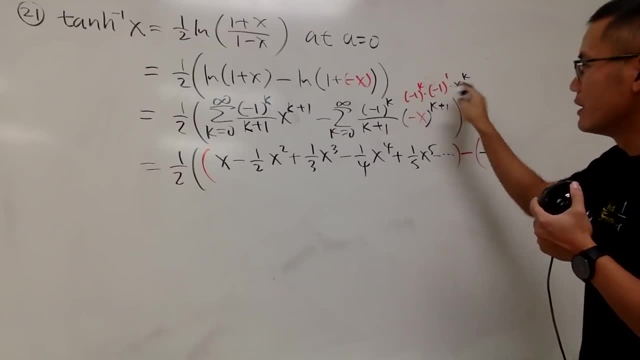 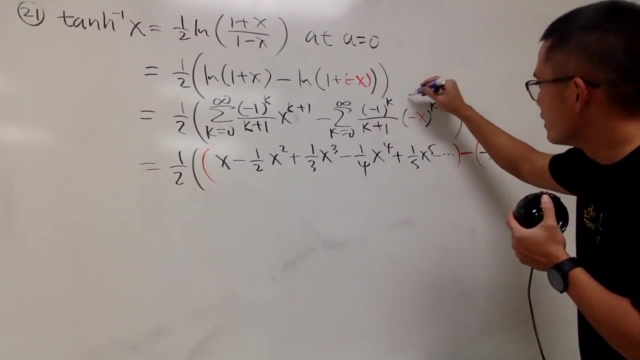 and then we have the x to the k's power, right? So let's look at this, And perhaps I'll put this down in blue for you, in purple, for you guys. So again, negative 1 to the k times negative 1 to the first. 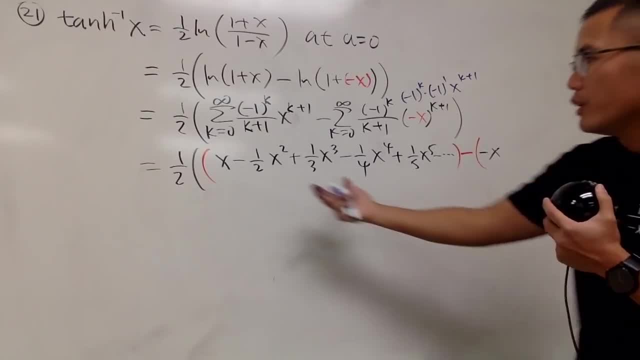 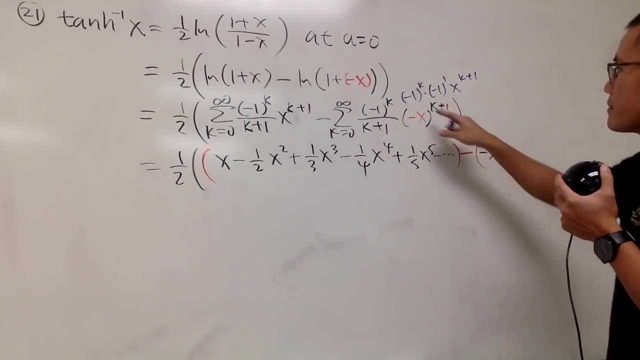 and then x to the k plus 1's power. So in terms of the power of the x will be the same, but the sine is the annoying part. Let's take a closer. let's take a closer. look. Good thing is that this and that. 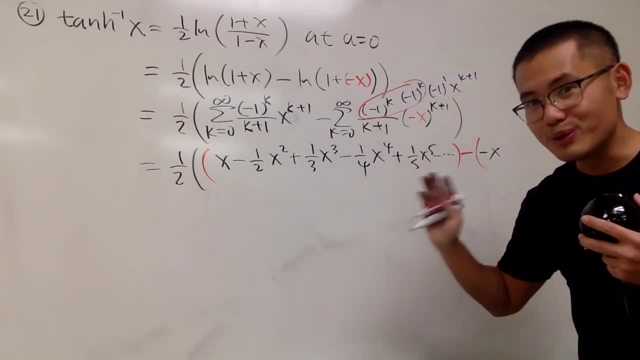 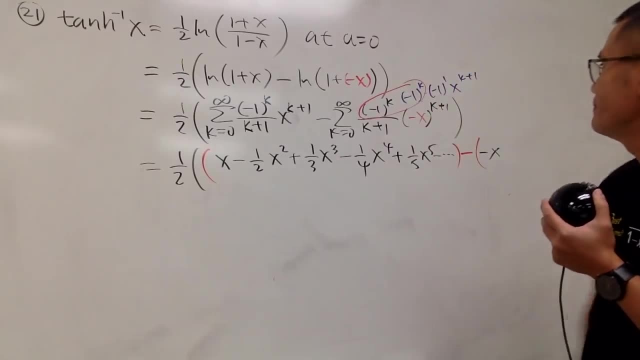 when you multiply, it becomes just negative 1 to the 2k power, which is positive 1.. And the truth is this: right here, it's not alternating anymore, It's just always man, it's just always negative. 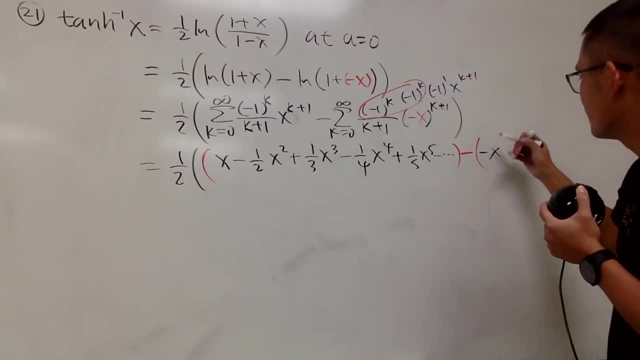 That's kind of bad, But however, this is always negative, okay. So, first of all, when k is 0, you get x to the 0 plus 1, which is just x to the first power over 1.. 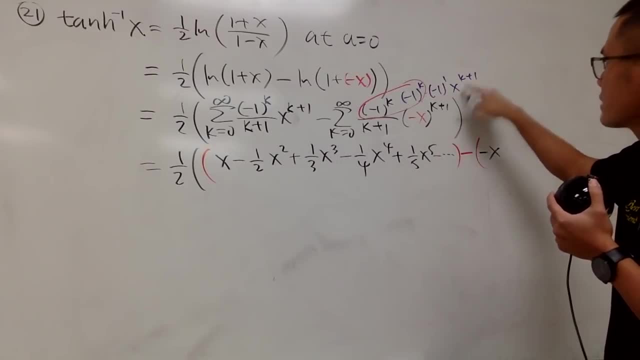 So that's what we have. And now, when x is 1, you put it here: so it's x squared, And this is still negative, so it's negative x squared over 2.. So I get it. So this is minus 1 half x squared. 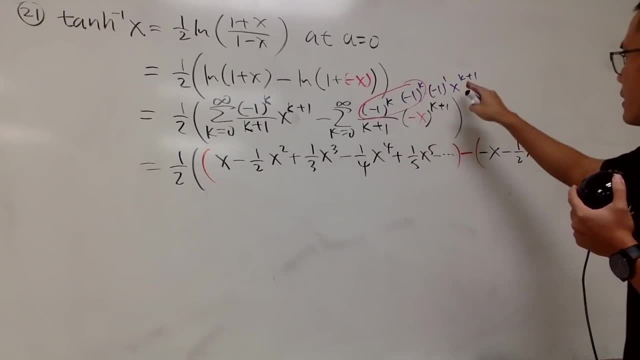 And then when x is 2,, you get over 3, but this is x to the and this is still negative. So it's negative. 1 over 3, x cubed, And it's always negative. Man, this is always negative. 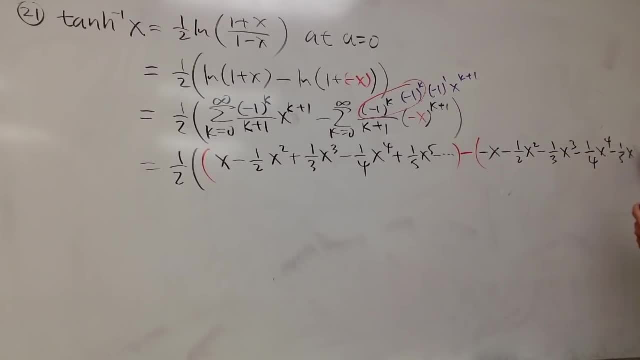 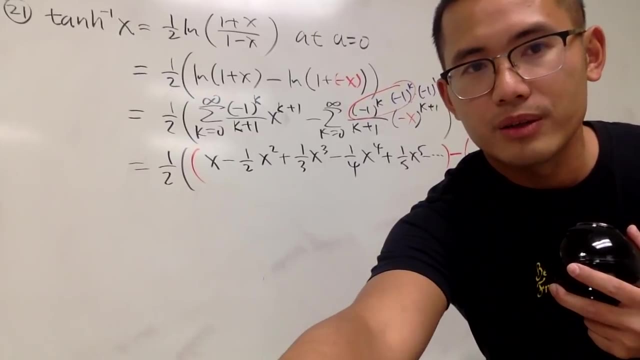 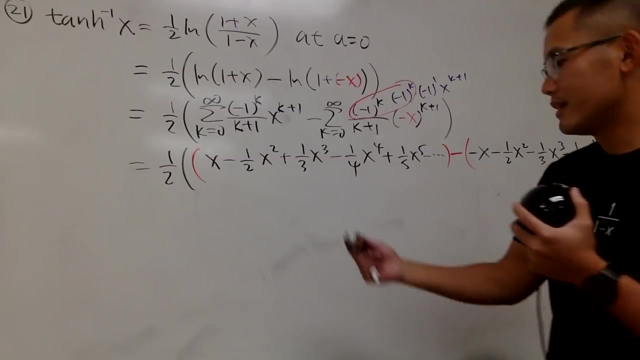 And minus 1 over 5, x to the 5, and so on, so on, so on, My bad for the camera angle, Yeah, okay, All right. So, man, this is 1 half all the way in the front. 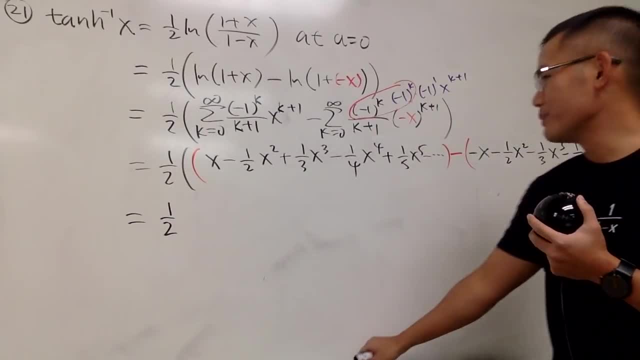 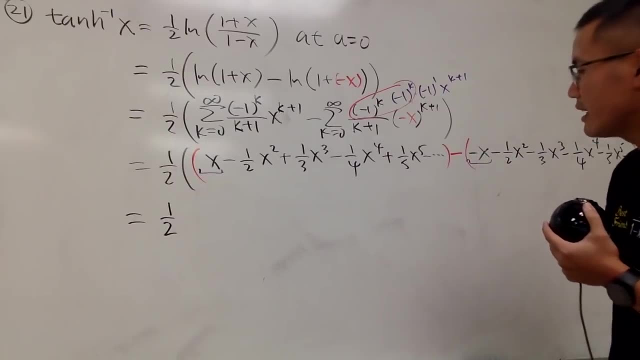 And now let's see which are the guys that are still maintaining: okay, First of all, this is x minus negative x, So that means I will have what? 2 x right here. Isn't it Next negative? that minus the same thing? 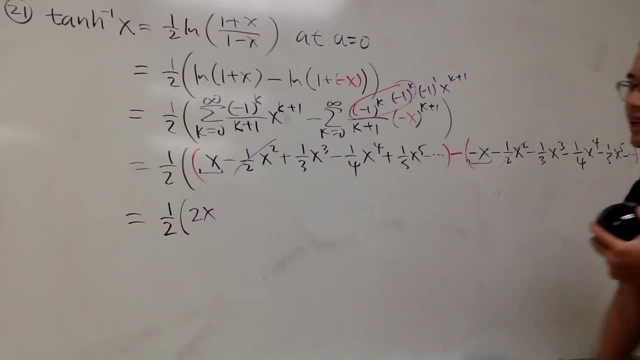 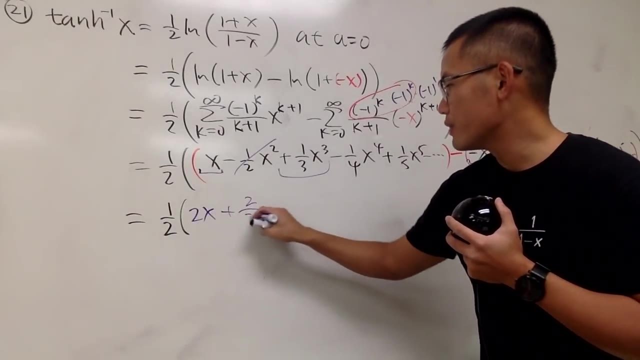 So this and that will cancel. That's good. Next, this minus minus becomes again 2 of them, So we have plus 2 over 3 x to the third power. Pretty good. This and that again they cancel. 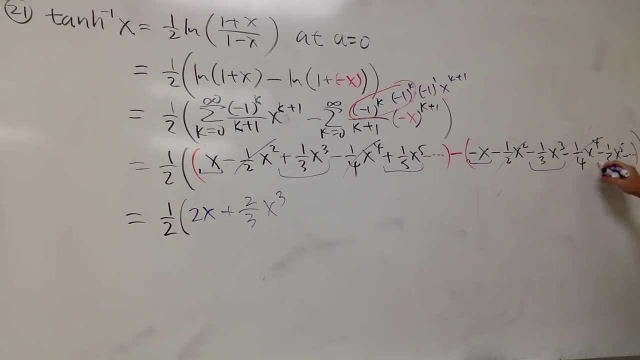 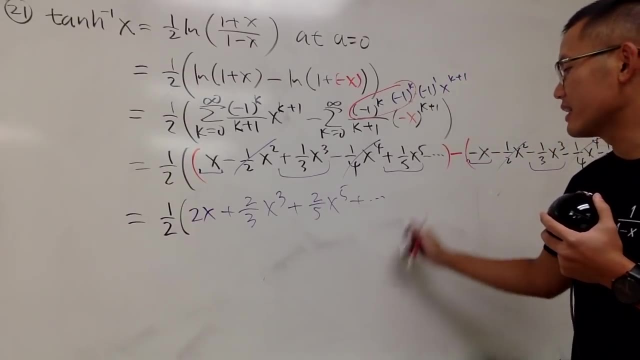 And lastly, the one that we have on the board, this and that together we get 2 of them again, So plus 2 over 3.. Again, so plus 2 over 5. x to the fifth power, and then plus the dot, like that. 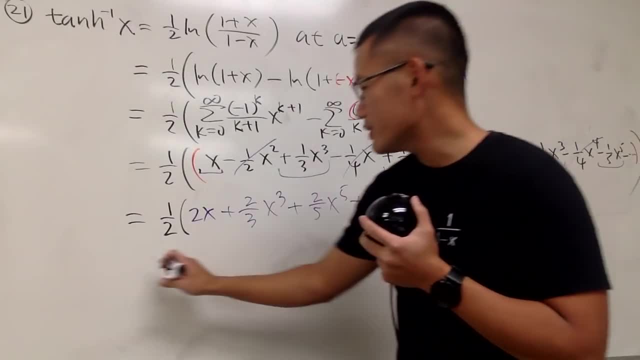 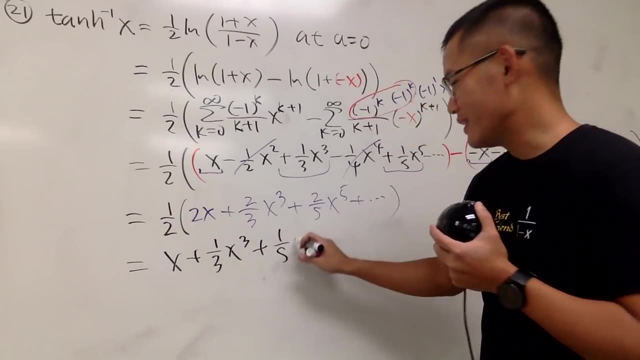 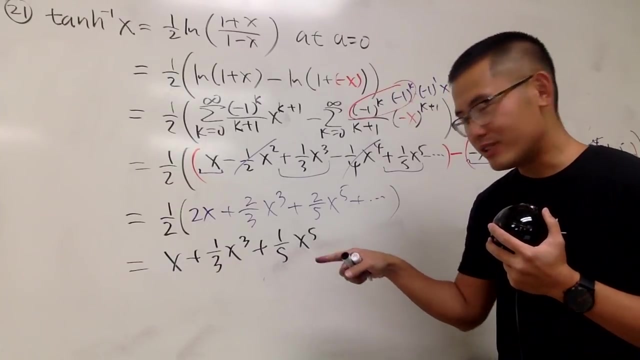 okay, And of course you can just reduce all the 2s, So we get x plus 1. third Man, this is not alternating, But does this remind you of anything? Yes, it should. That's the inverse original tangent. 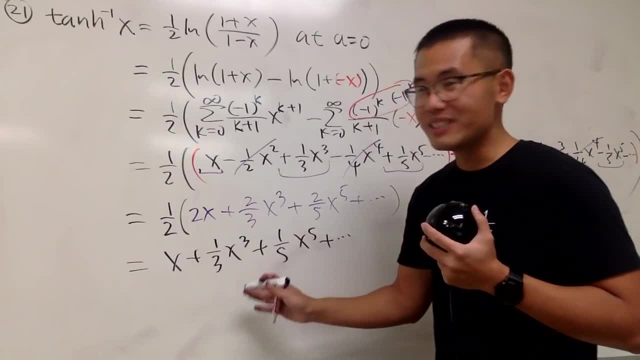 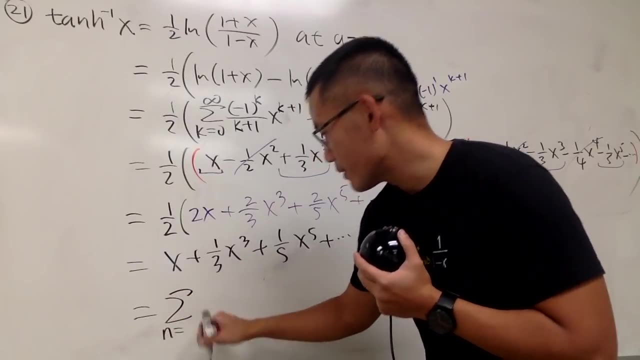 But this one right here is not alternating. That's why it's the inverse hyperbolic version, okay. So finally, we'll just say this is the sum as n goes from. I'm using n right here now. okay, 0 to infinity. 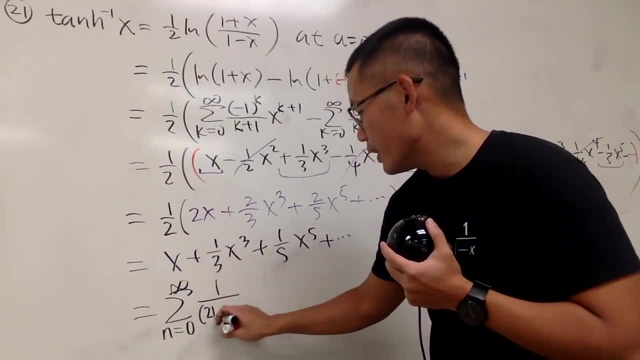 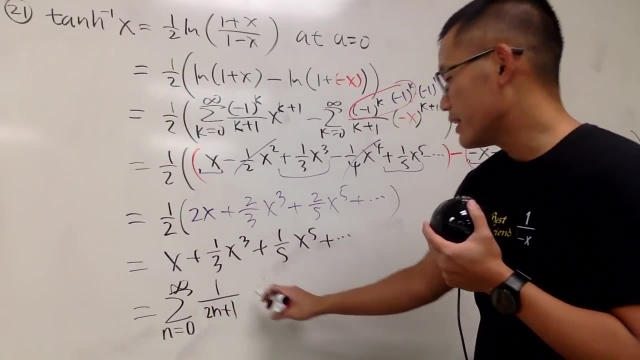 No alternating right, So just 1 over 2n plus 1.. And there's no factorial neither. It's just 2n plus 1.. And these are numbers, And then the power is the same as that. So we have x to the 2n plus 1.. 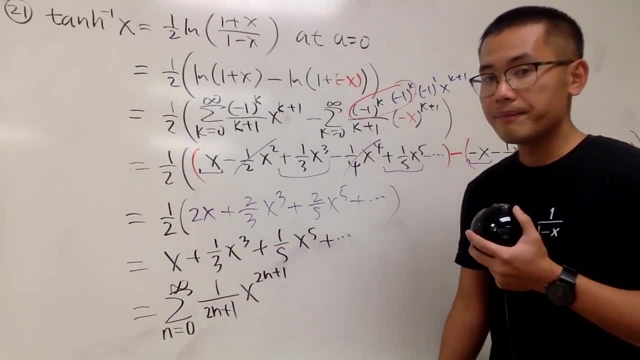 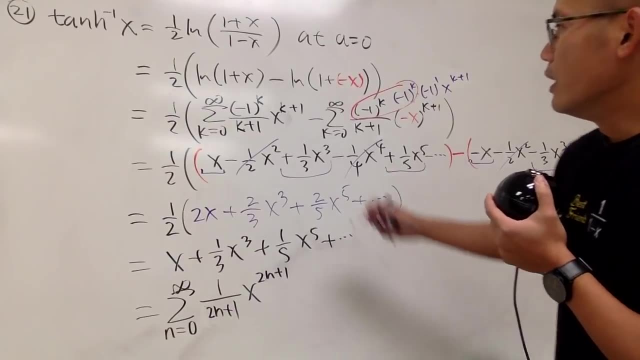 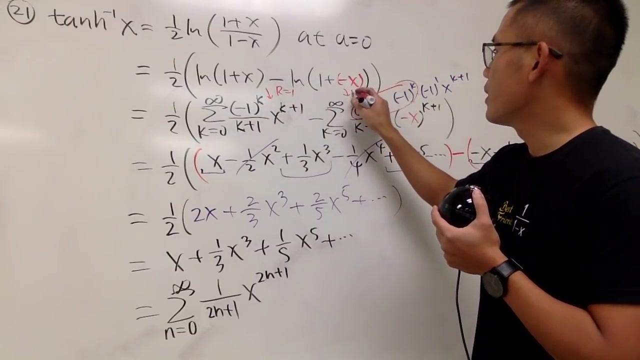 And notice that it says 0. So that's what we have, right. So that's pretty much it. Now check this out, though, From here to here. well, we use the r is equal to 1, right, And likewise. 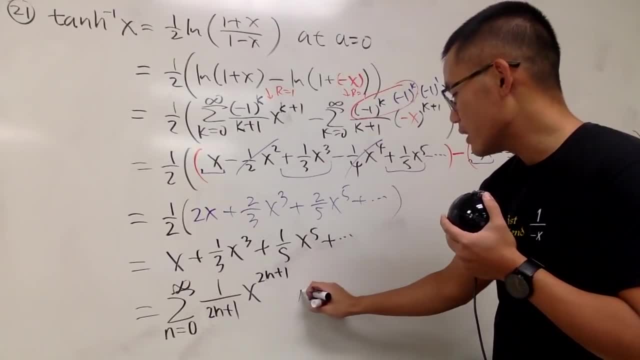 from here to here, r is equal to 1.. So of course now it's just algebra. So we still know that r is still equal to 1. And again, you can set up absolute value, but r is equal to 1.. 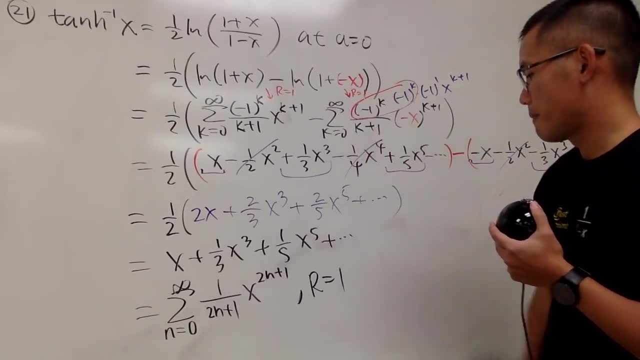 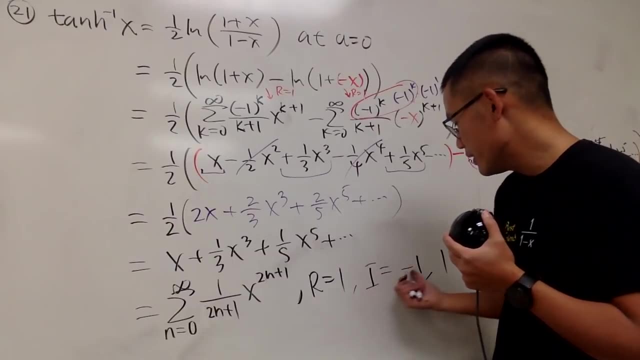 And then let's see What's i then. Well, it will be going from negative 1 to 1.. So check this out: If I put negative 1 in here, this is not alternating. And then negative 1 to the 2n is just gone. 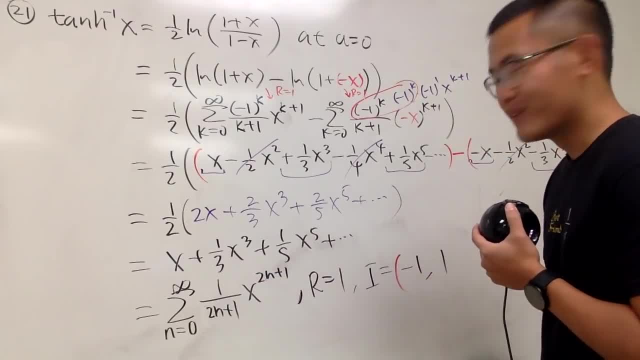 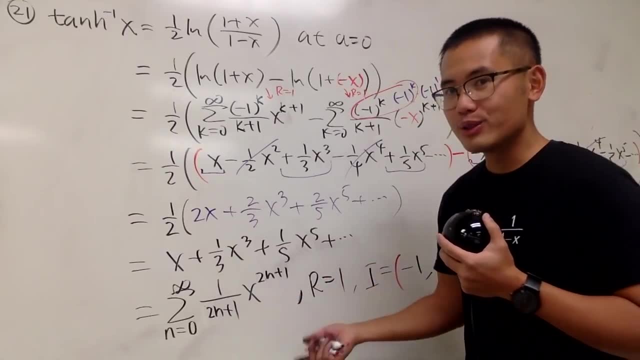 It's not alternating, So unfortunately it won't converge. And when we put in 1 right here again that will be 1 over 2n plus 1.. You can just do the comparison test with 1 over n. 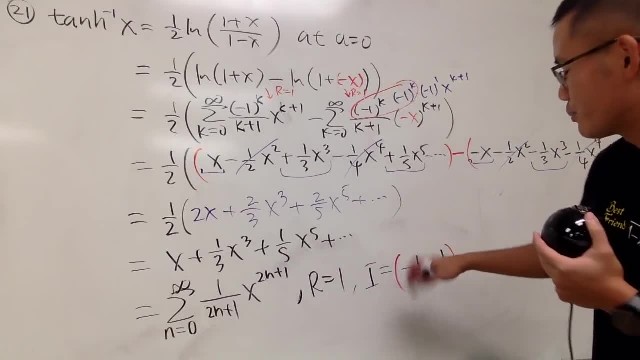 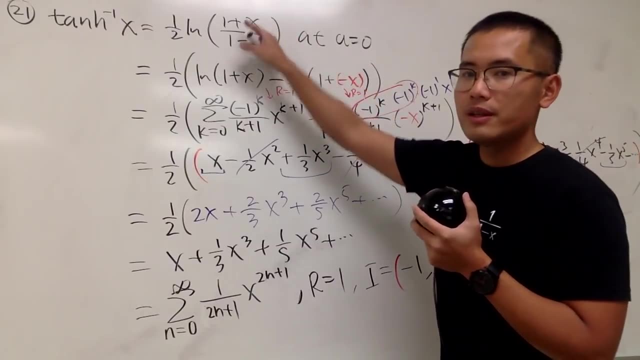 right, The series of 1 over n. It does not converge neither, So it's open parentheses, open parentheses. A fast way to do it is that if you put in negative 1 into the original function, that will mess up right here. 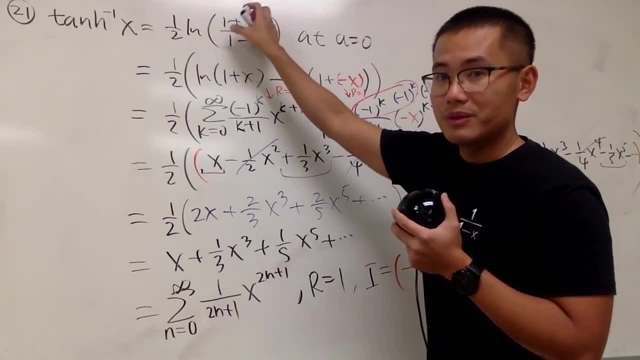 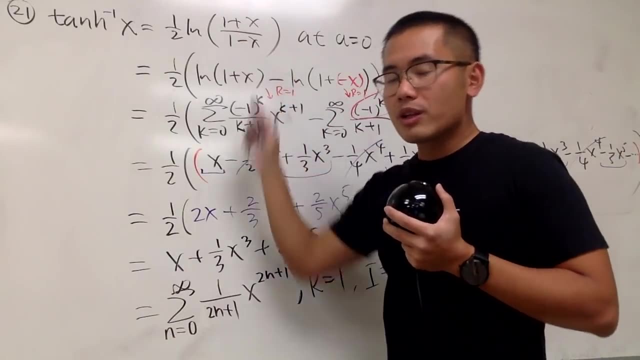 1 plus negative 1 is ln of 0 in here, right? It's 0 instead of the ln. So that messed up. So you cannot include that. If you put in 1, you have 1 minus 1 on the bottom. 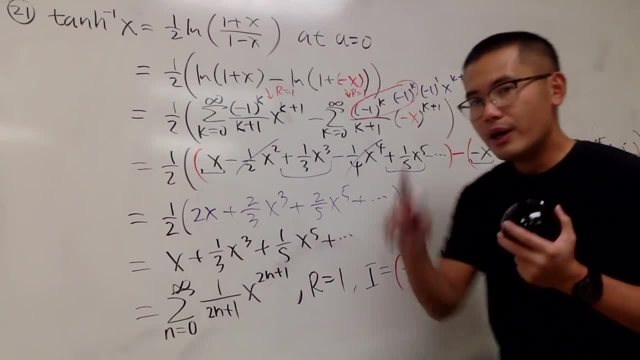 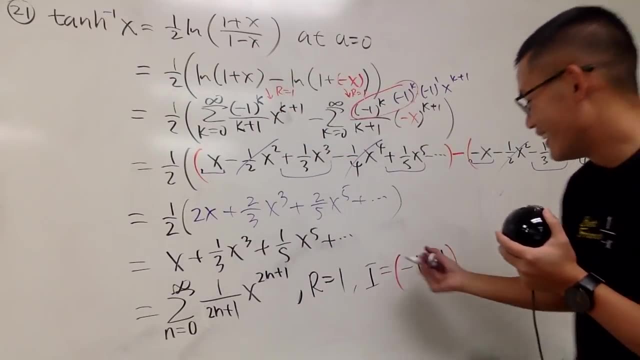 Again, that's messed up for the function. That means you cannot include that. Remember, remember, remember: If the function is messed up, then of course the power series will be messed up. Okay, So that's a quick way to do it. 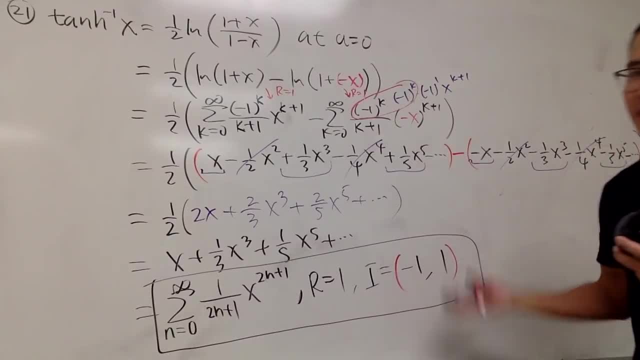 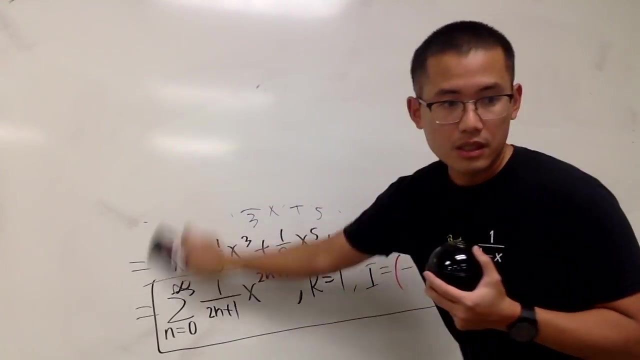 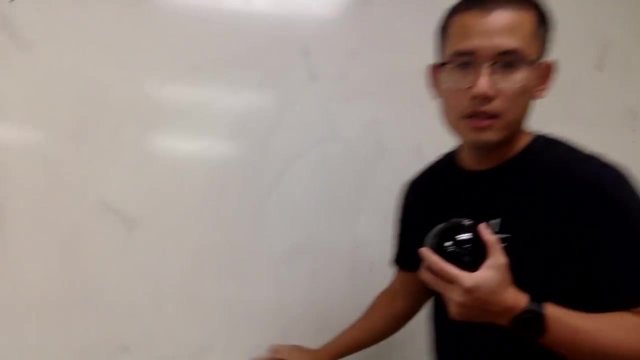 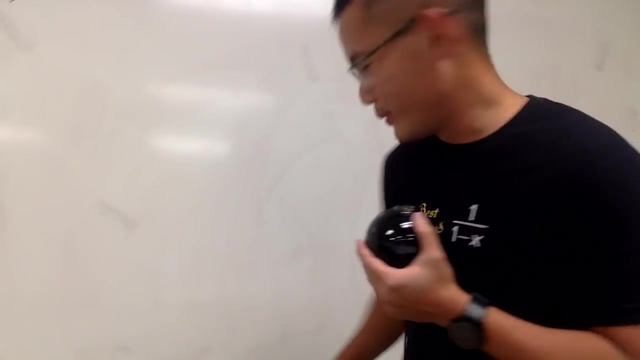 So you can just do it like this: Okay, So have a look, Ladies and gentlemen. inverse hyperbolic tangent. All right, Next one should be pretty fun to do. Okay, Next one: ln of x at 2. Okay. 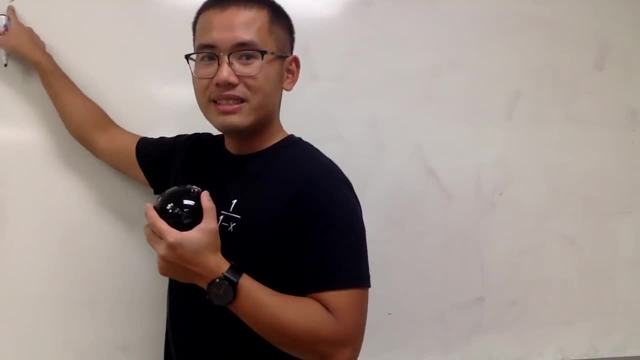 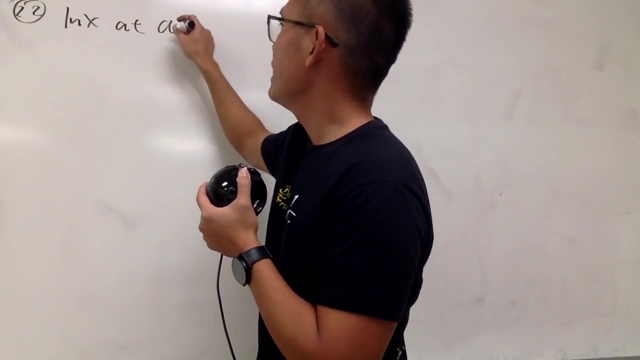 So I'm just kind of jumping back and forth with the natural log and all that. Let's see Number 22.. I want natural log of x at a equals 2. So it's a different center. now, right, Another different center. 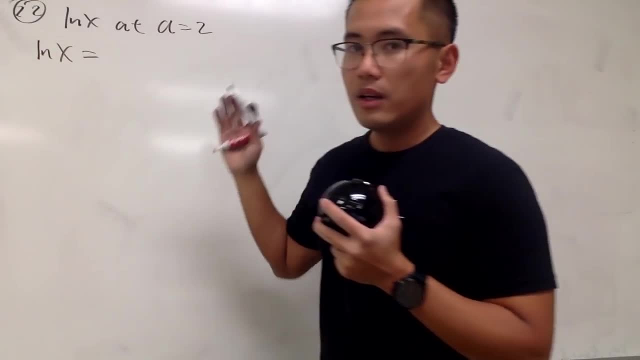 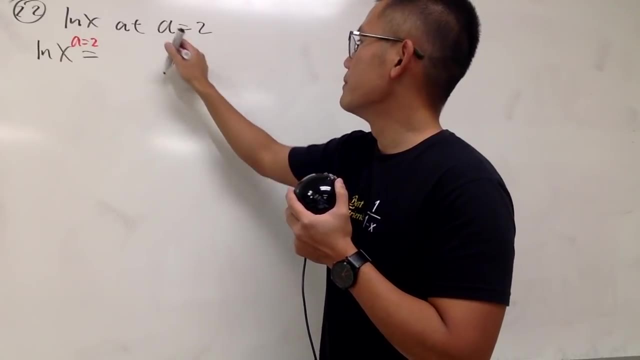 So here we go. This is ln of x When a is at 2, right. When a is 2, center is 2.. That means I want to have a factor x minus 2.. Well, inside, here I have x. 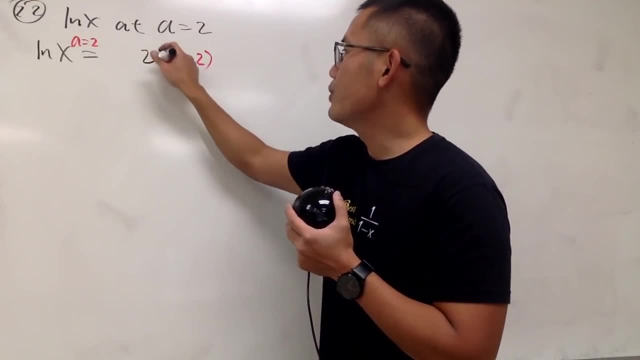 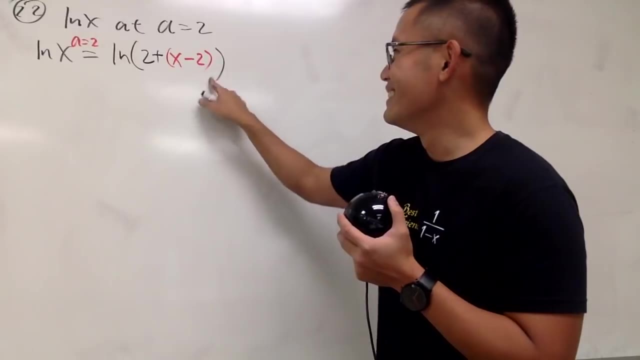 Now I have x minus 2.. It's okay Because I know 2 plus negative 2 is 0. So this right here will be the same And then just have the ln like this. That's pretty much it, right. 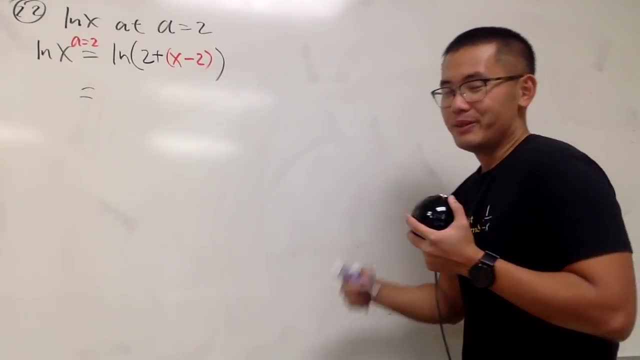 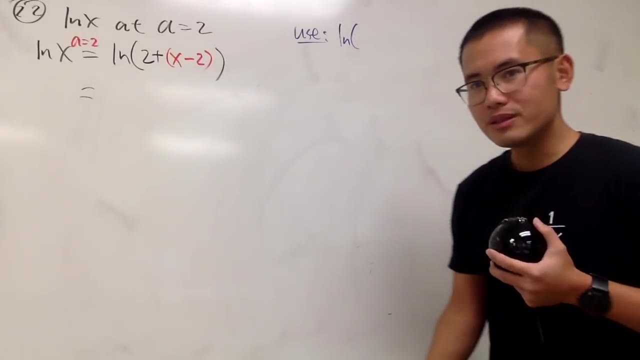 Well, in order for us to you know, do it a quick way, I'll just tell you we will be using ln of, and this plus sign is ready for us too. So that's very nice. 1 plus x. 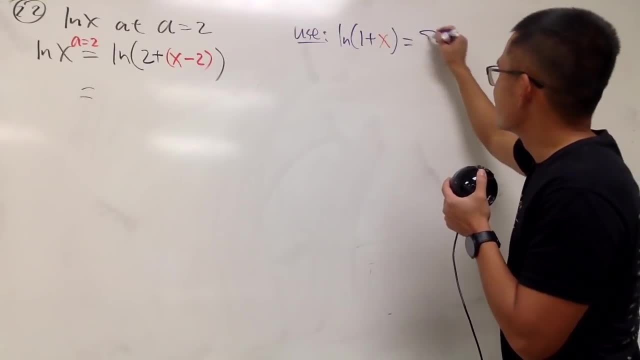 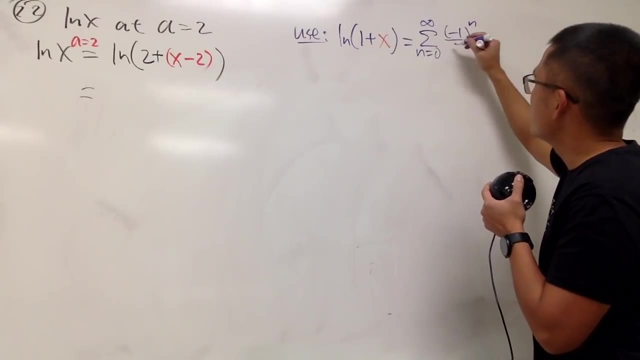 Didn't we just do this one earlier? Yes, we did. This is the sum as n goes from 0 to infinity And we have: this is negative: 1 to the nth power over n plus 1, x to the n plus 1th power. 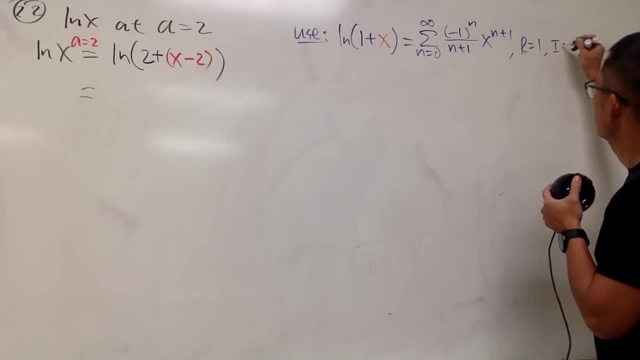 r is 1.. And in fact, the interval, notation interval of convergence is at negative 1, 1.. And I should also tell you, epsilon of x is less than 1.. Less than 1.. Sorry, Sorry, I can. 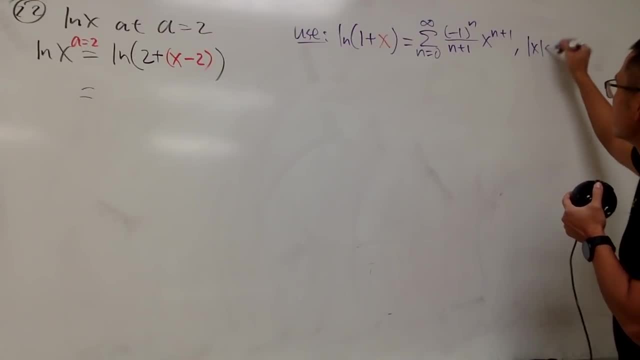 I will just write it down like this: Absolute value of x is less than 1.. r is 1.. And the interval of convergence: at negative 1, it doesn't work, But at positive 1, it does. There we go. 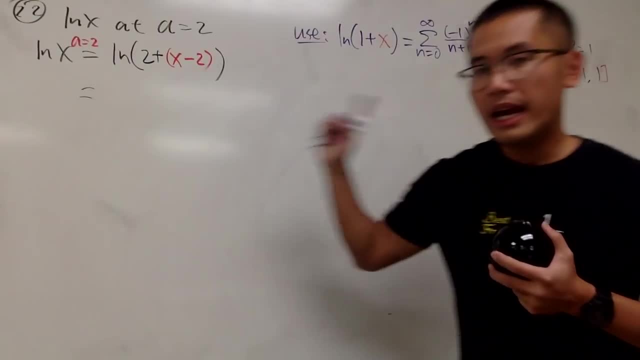 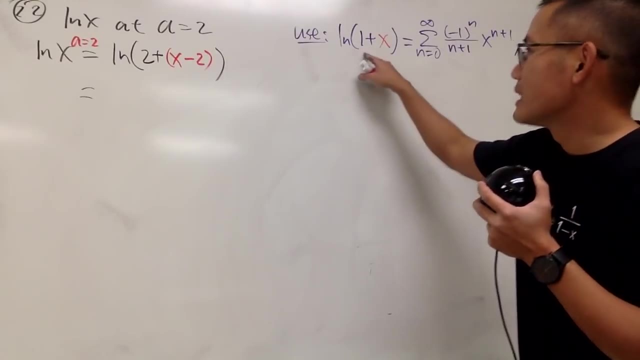 I wrote it down wrong earlier, So yeah, Anyway, this is what we are going to do. This is what we are going to do. In order for us to use this friend, notice that we must have a 1 right here. 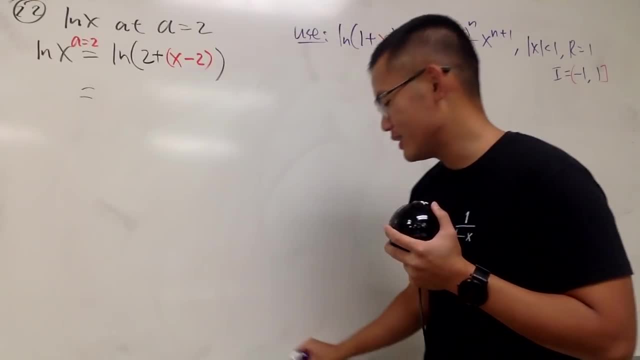 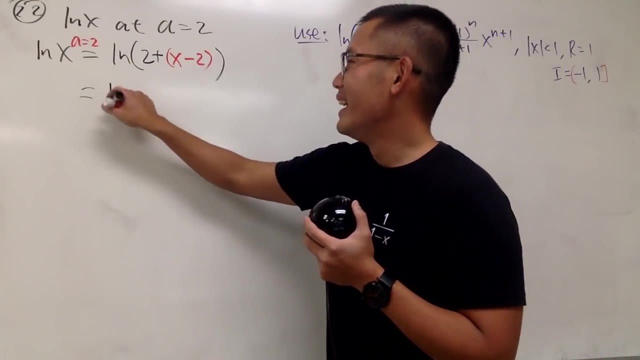 but that's a 2.. It's okay, Just factor things out. That's what we like to do, isn't it? I'm hungry, Anyway, ln I'll factor the 2 in the inside, so I will do this. 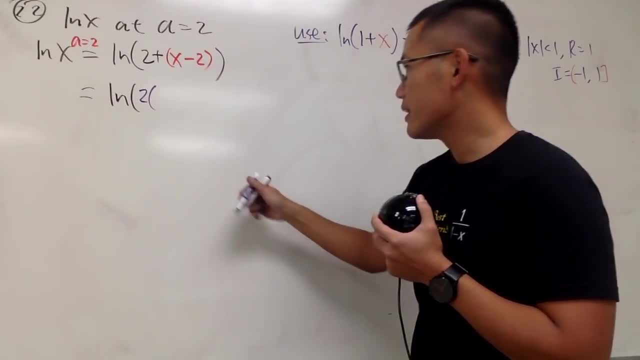 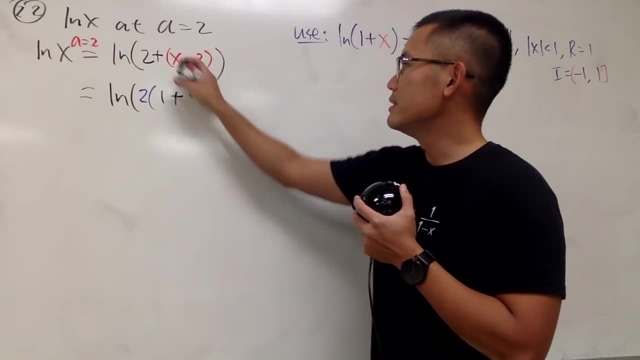 Let's say I have this, I have the 2,, like so, And we have 1, plus. if I factor out 2, that means what That means. this right here will be x minus 2 over 2. And that's pretty nice. 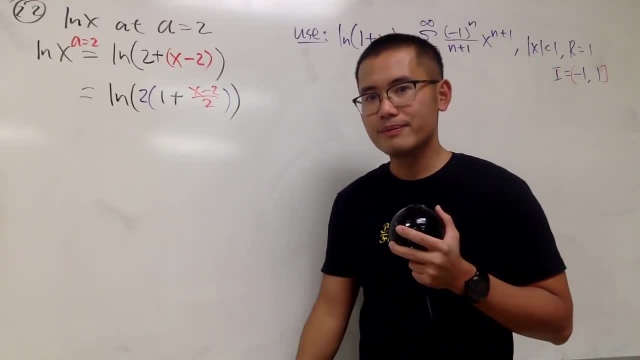 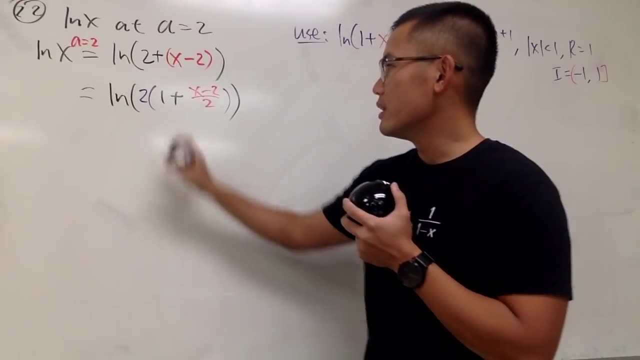 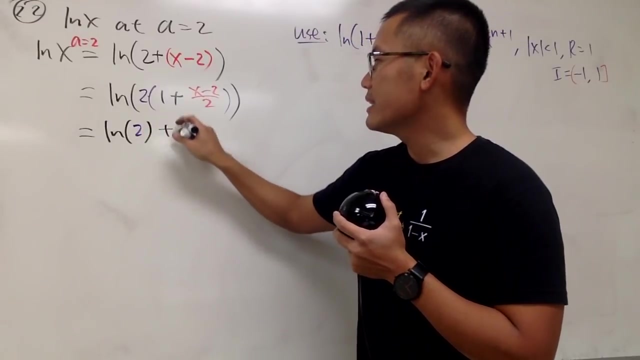 Close, close. What can we do next, though? Thanks to natural log ln of a product, it's the sum of 2lns, and this is 2 times all this, so first we will have ln of 2, and then we add ln of this. 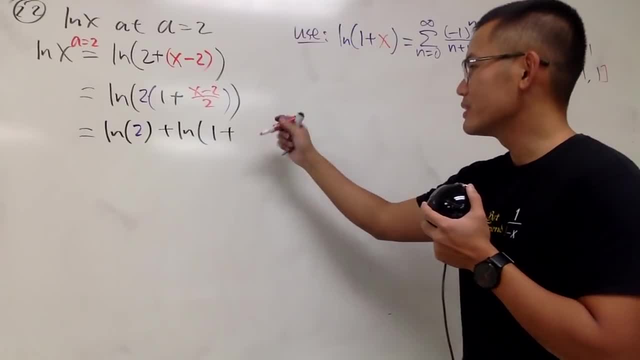 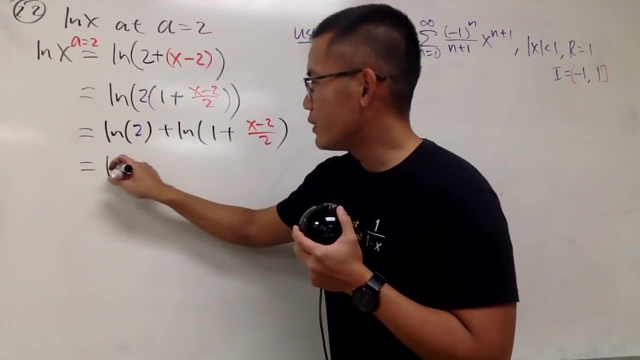 which is 1 plus, and then we have that which is x minus 2 over 2, like this: This right here, we're just going to leave it right now. plus well, this right here, we can use our friend right here. 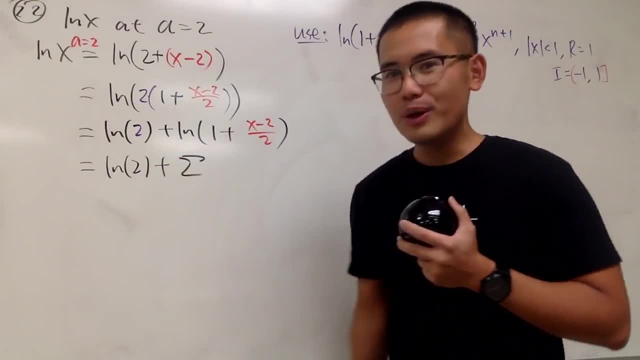 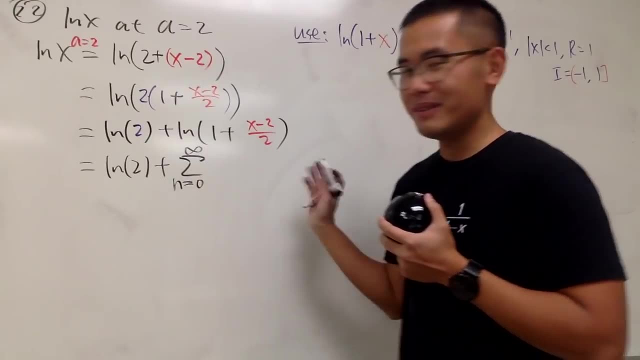 huh. So you need to know how to use your friends. Well, maybe not in real life, In math it's okay. In real life, man, that's kind of not good to say, but in math it's totally okay to know. 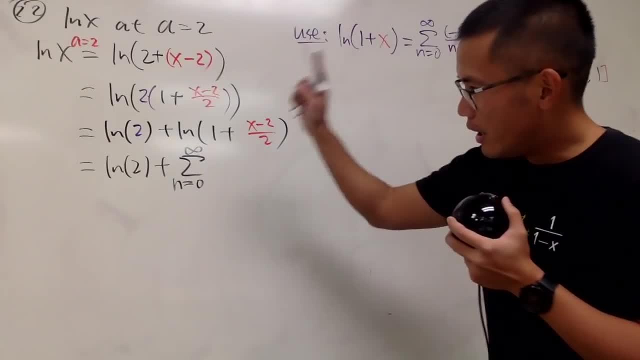 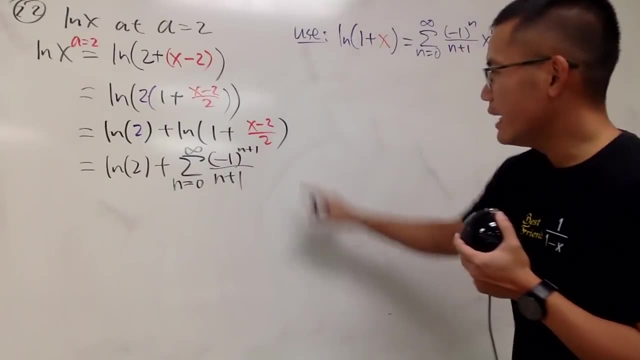 how to use your friends. It's important to Alright. so here we have negative 1 to the m plus 1's power over m plus 1, and you just enter this, guys in here. so we have x minus 2 over 2,. 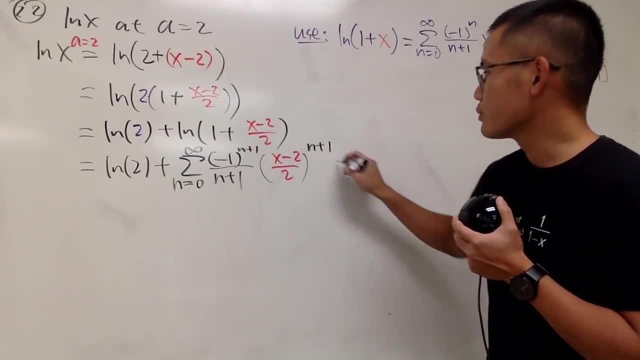 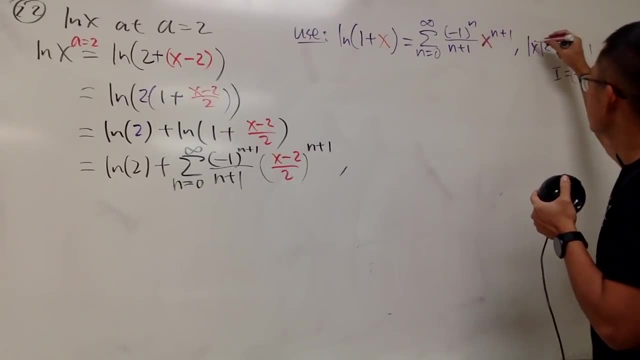 parentheses this and then raise to 1, and then raise to the m plus 1 power, and I will enter this right here in the absolute value as well. so this right here should be in red. likewise this absolute value of x minus 2 over 2. 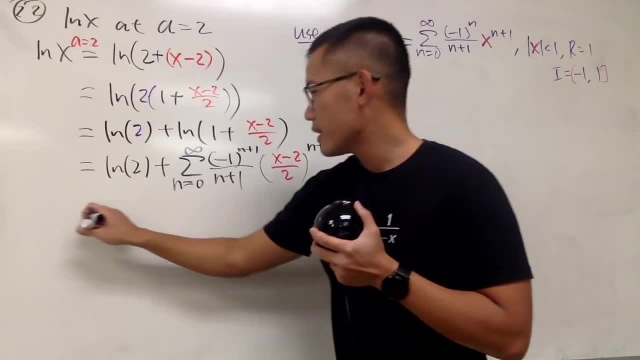 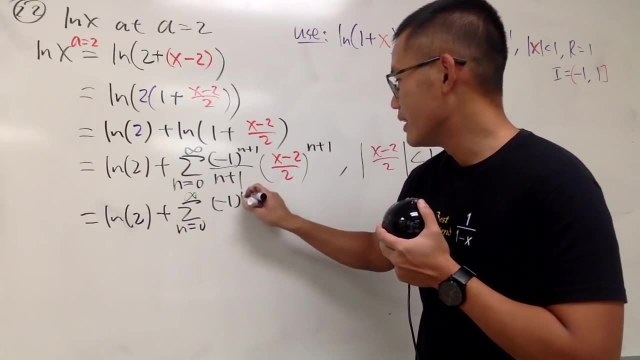 should be less than 1.. Okay, here we have ln of 2 plus the sum n goes from 0 to infinity. this is negative 1, m plus 1 over m plus 1, well, we have 2 to the m plus 1,. 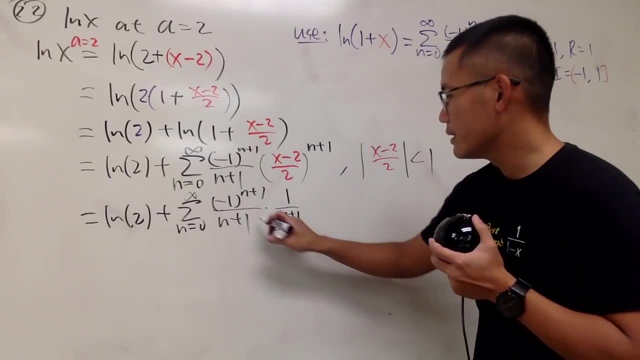 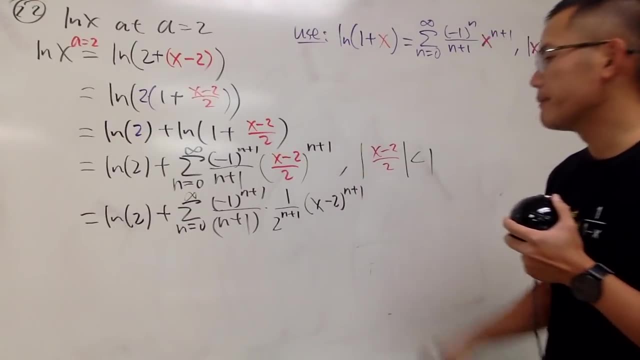 on the bottom, so I will write it as 1 over 2 to the m plus 1, and perhaps put parentheses to just make things more clear and have this on the side. Yeah, And now check this out. This is ln of 2,. 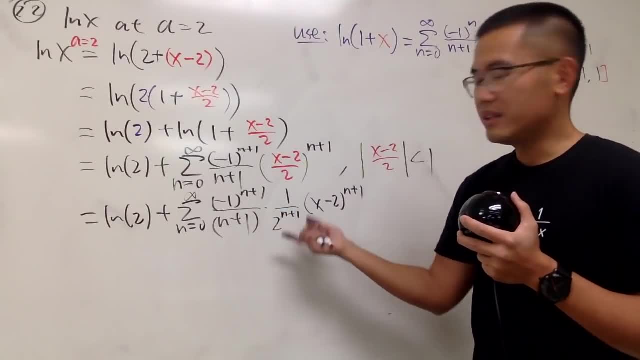 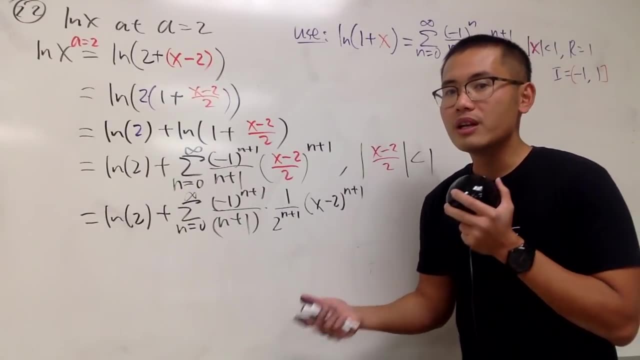 and there's nothing that we can combine with. In that case we just leave the ln of 2 all the way in the front. So this right here is pretty much it right. so we cannot do too much in this situation. 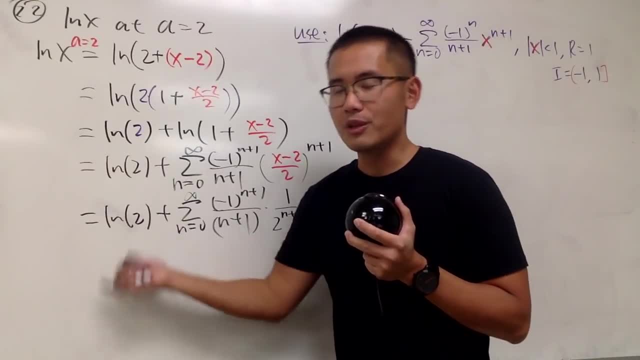 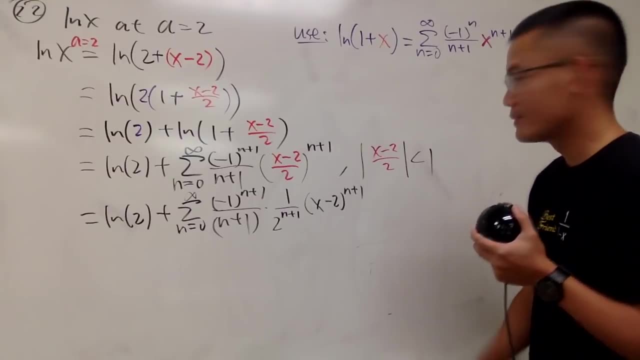 And for power series. sometimes it's okay to have like extra terms in the front so that the rest can be put in the similar notation. If this one cannot be done, then just leave it in the front, That's it. 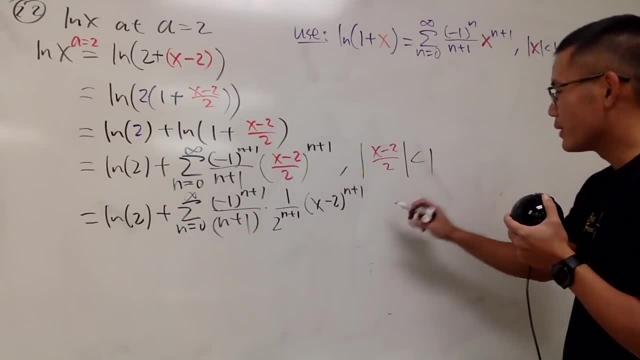 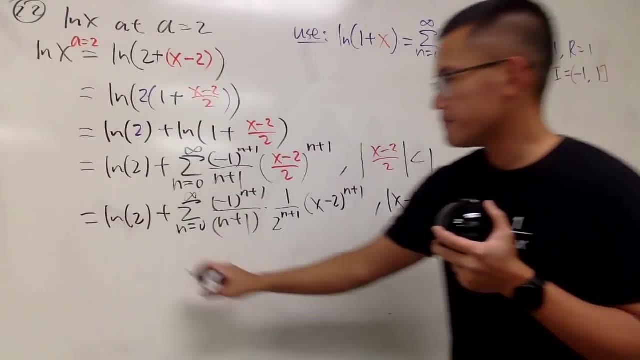 Yeah, I know, I know, Yeah. Anyway, right here, absolute value of x minus 2 multiplied by 2 on both sides, we have this less than 2.. So that means r is 2.. That means r is 2.. 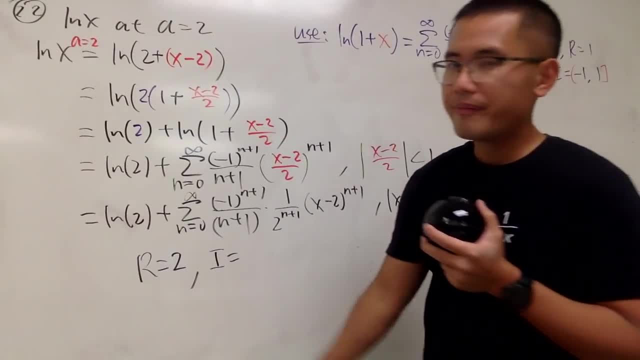 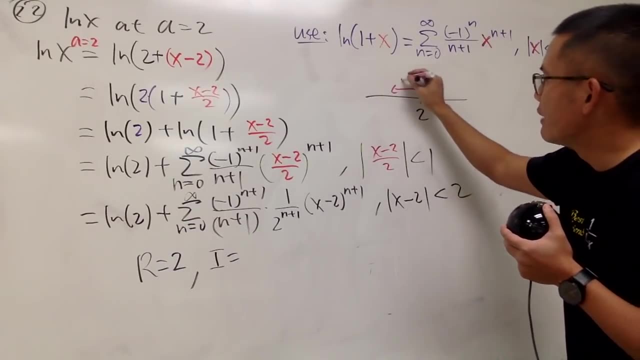 Then I notice a is 2, right a is 2. And r is 2.. That means you move to the left twice and you move to the right twice, So you'll be at 0 and you'll be at 4.. 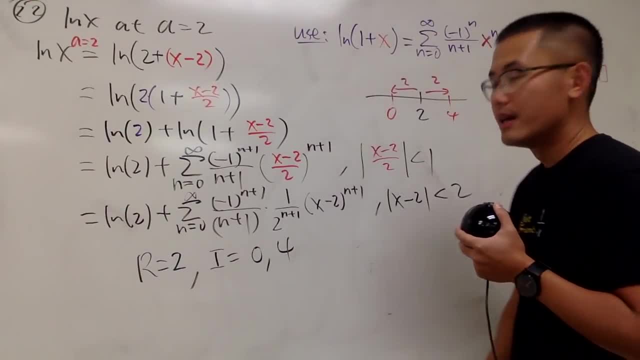 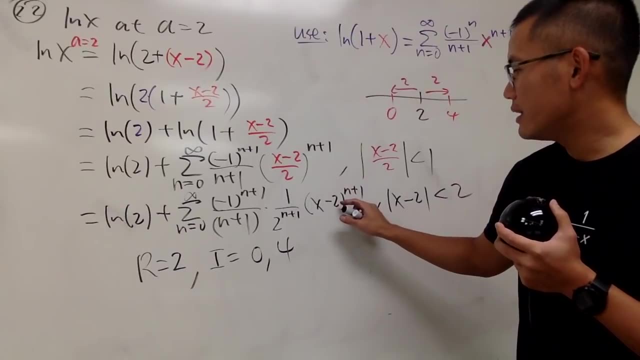 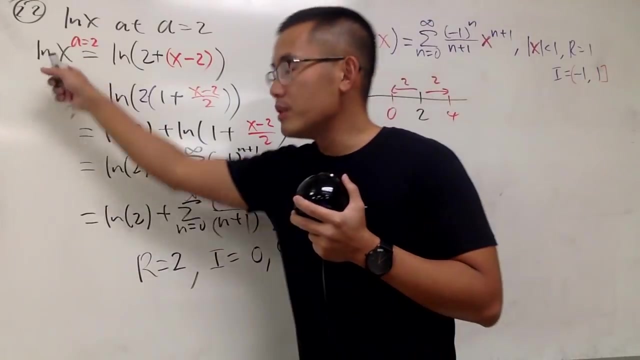 So I will be at 0 and 4. But what happens at 0?? If you put in 0 right here, you get negative 2. And you unfortunately cannot do 0. Why not? Because 0 cannot be put in here. 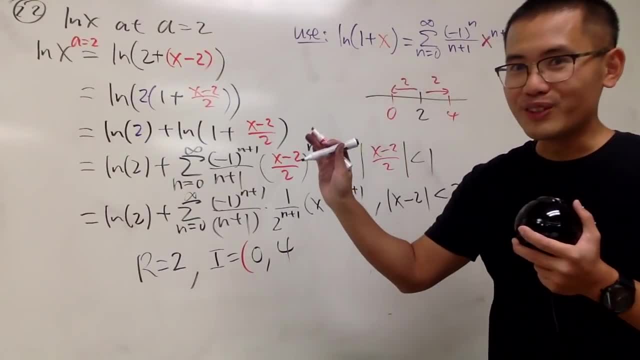 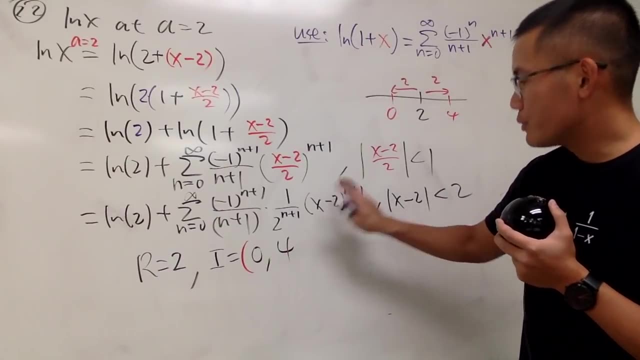 That's a quick way to do it. So if your function cannot work, positive 2 cannot work either. Okay, You should check 4.. If you put 4 in here, you get positive 2.. 2 to the n plus 1.. 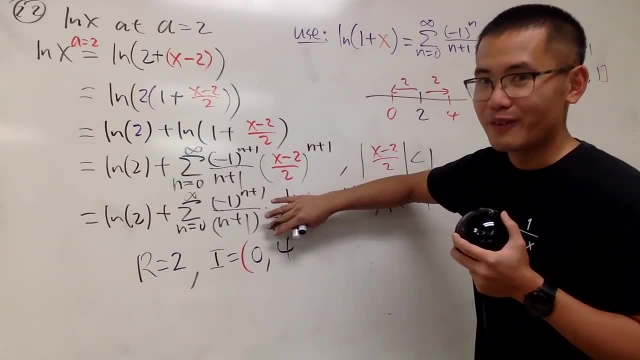 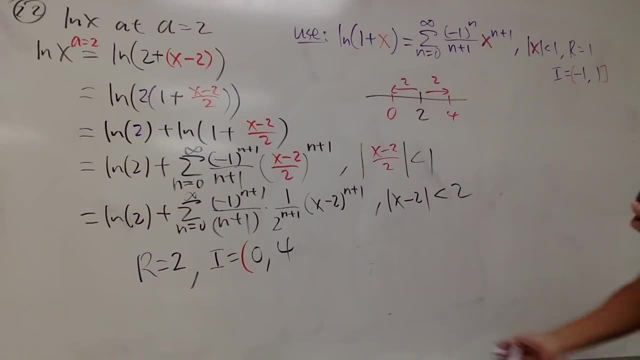 So this and that will cancel. In fact, this right here converges just like the one that we have right here. So in fact it's pretty much the same idea. Open parentheses, close bracket. it's the same thing. It's just referred back to what we did earlier. 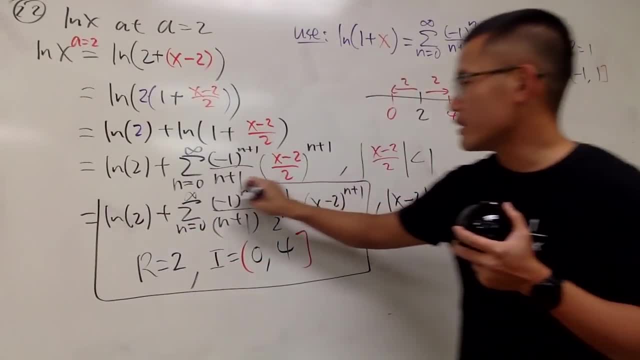 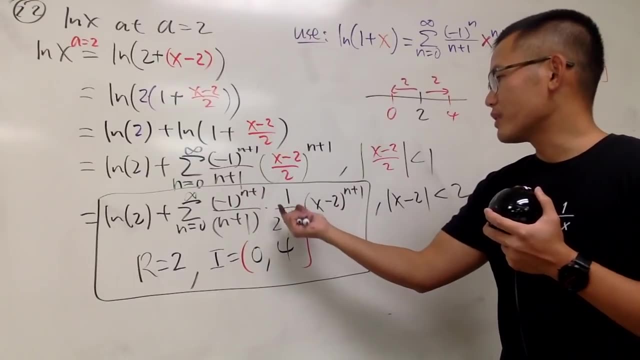 If you need to write down all the steps, just go ahead and do so And this is it right. So yeah, And of course you can just maybe write this down one time and maybe I'll just put this down, Doesn't really matter that much. 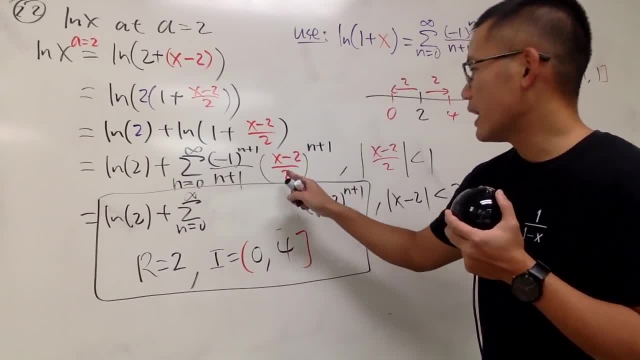 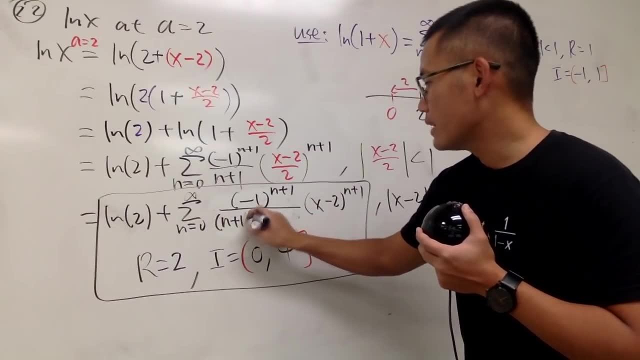 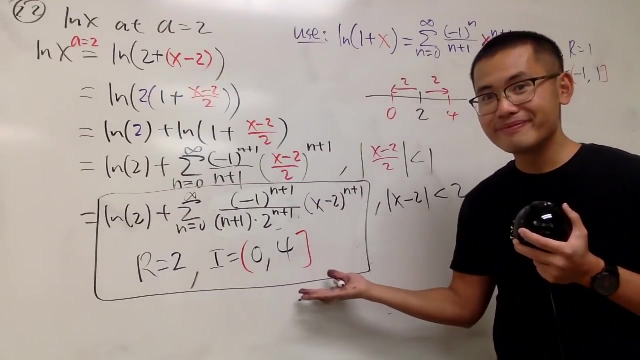 But I will put this down like this: Negative 1 to the n plus 1's power over. I'll put down n plus 1 times 2 to the n plus 1.. Looks better this way. right, Just like this. We're not done yet. 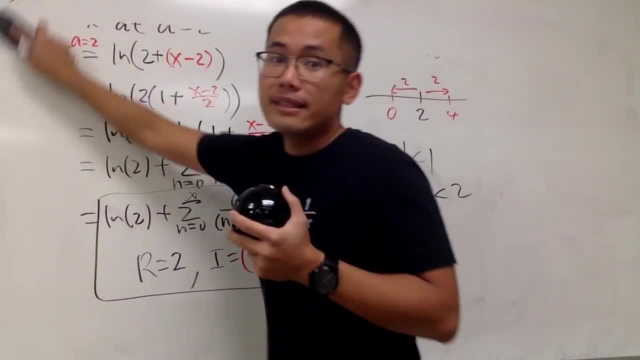 A couple more to go. Not so bad if you only have to do 26.2 questions, Otherwise I'll be like crying. Imagine 100 power series questions. Seriously, you guys, Seriously You guys are going to make me do that. 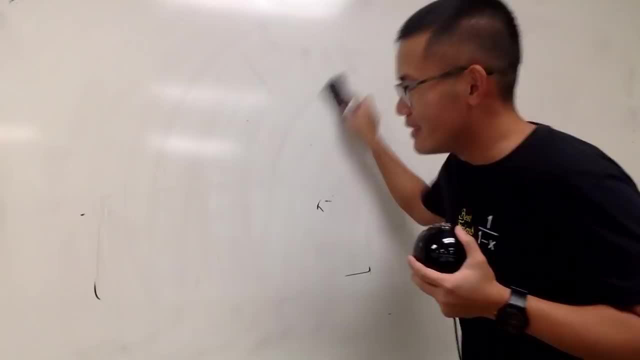 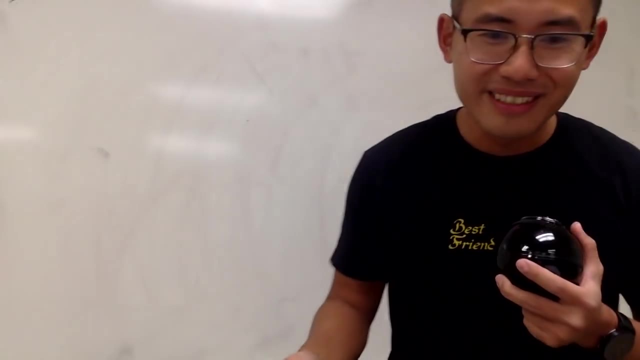 Seriously, You guys are making me do that. No, please don't. Next one, 23.. Next 23,, 23.. Here we go. We have 2x. Ah, this is the polynomial. This is the polynomial. 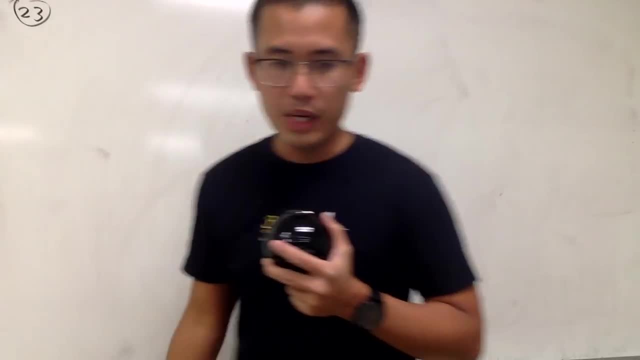 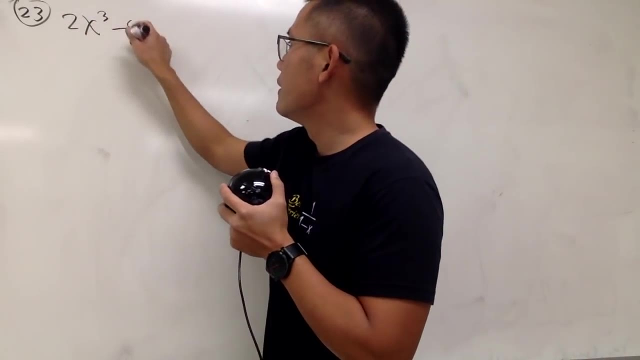 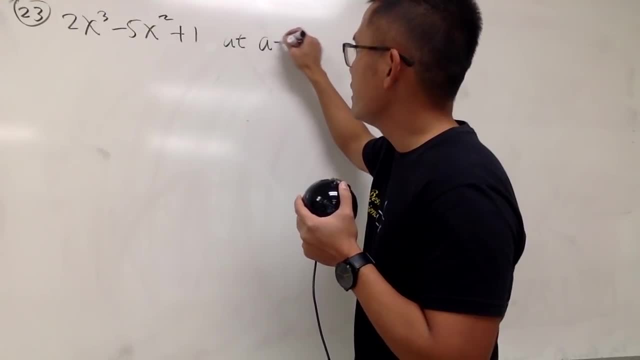 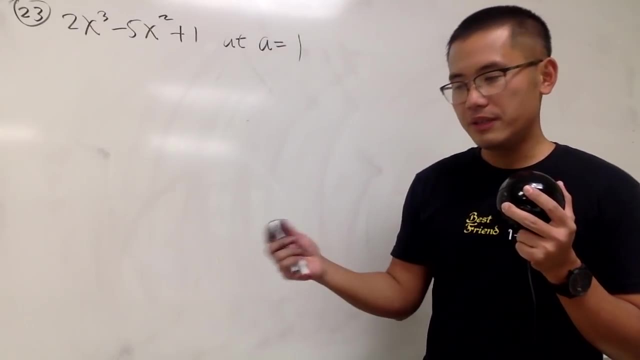 plus 1. And we want this to be at a equals 1.. In fact, you have a non-calculus way to do this. I believe you can just do some polynomial definitions whatsoever, But in this case I'll show you guys. 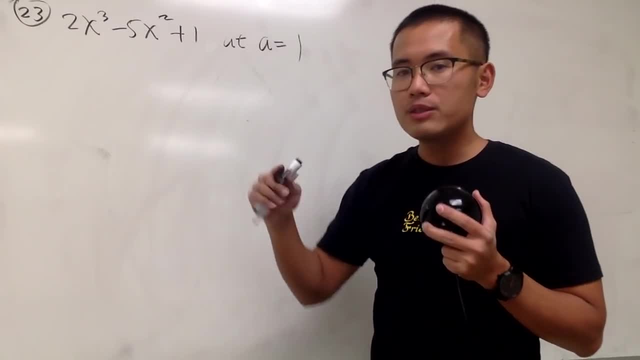 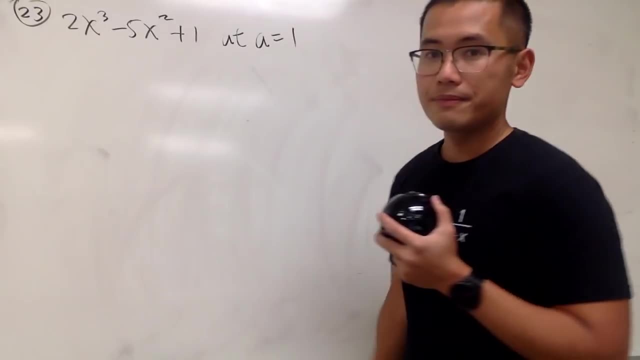 a calculus way to do this. Again, when a is at 1, that means you should have x minus 1 as your input. So just keep that in mind later on. This is at. a is equal to 1.. This is any better. 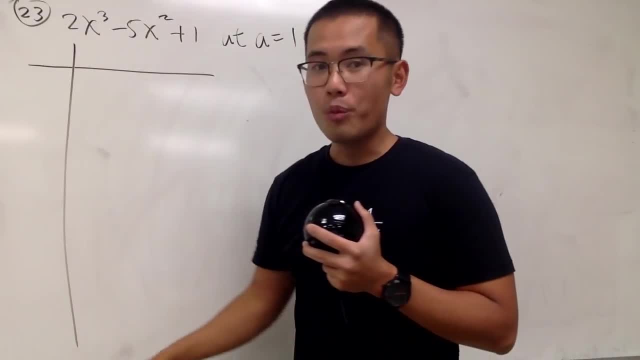 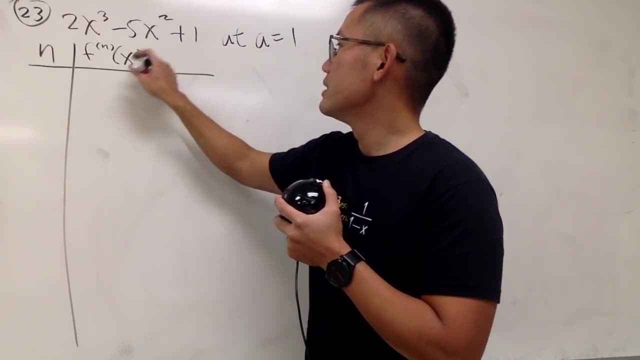 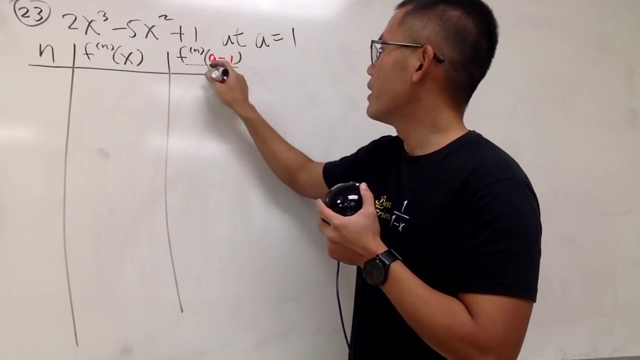 huh, All right, Anyway, I will use the Taylor formula to help us out. And and then this is the nth derivative. at here is the formula a at 1 over n, factorial. A very common mistake that students will make is that they forget about 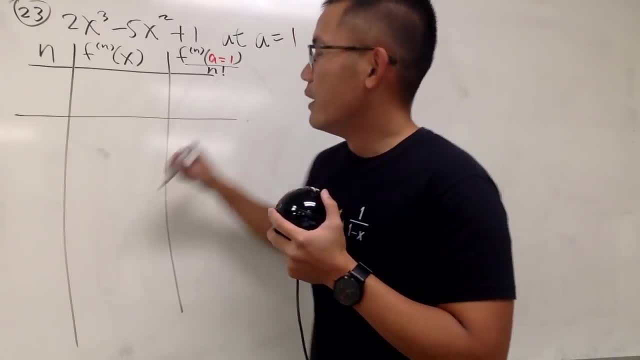 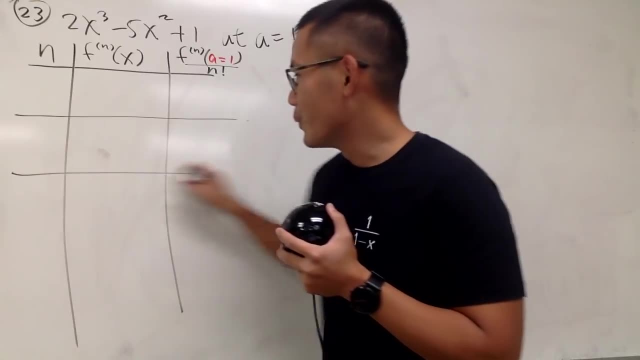 how to divide the n- factorial. This is not so bad because it's a polynomial. If we differentiate this four times, you know it's all over. So we don't need too much. So let me just put this down. 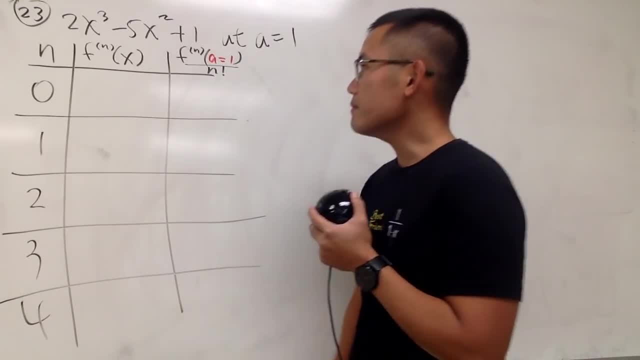 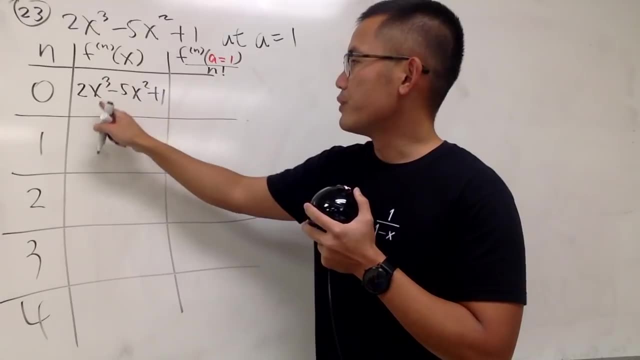 0,, 1,, 2, 3, 4.. I'll show you right here: if we're all done So, original, we have 2x third power minus 5x squared plus 1.. Go ahead minus 10x. 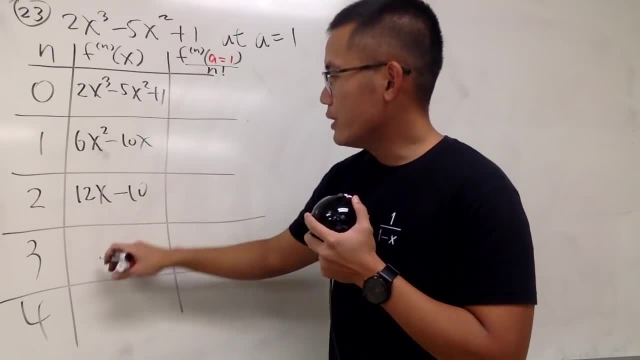 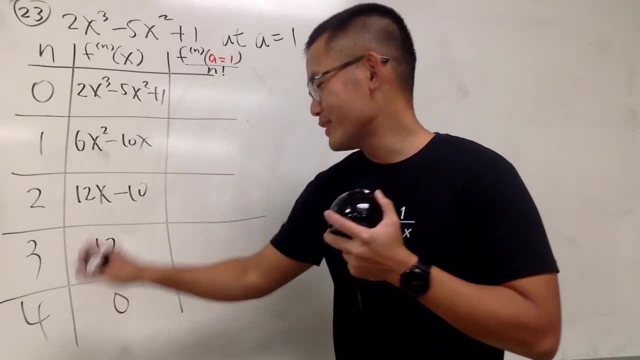 Differentiate this again, We get 12x minus 10.. Do it again: We get 12x, No, just 12.. Ha, ha, Ha ha. And then we get 0.. Anything after that is just 0.. 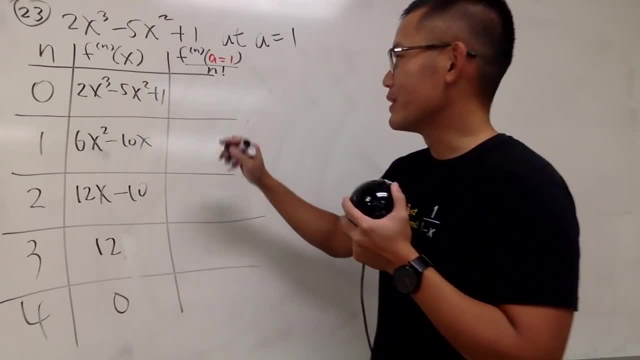 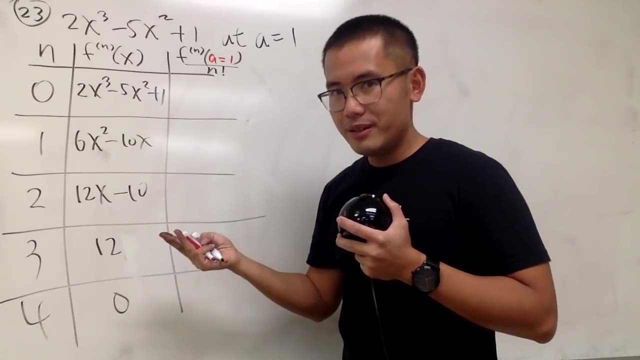 So bye, bye. Now. putting 1 in here. I want to make sure that I can do this in my head carefully. Putting 1 in here: This is 2 minus 5, which is negative. 3 plus 1 is negative 2.. 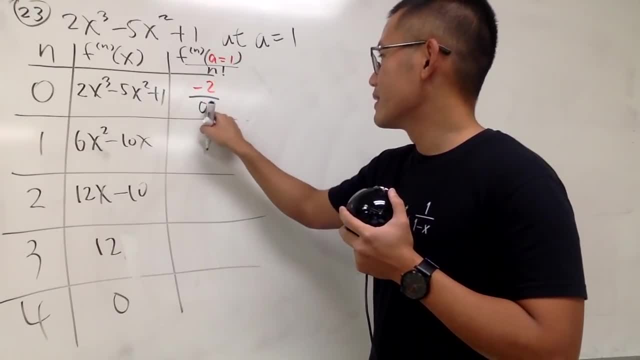 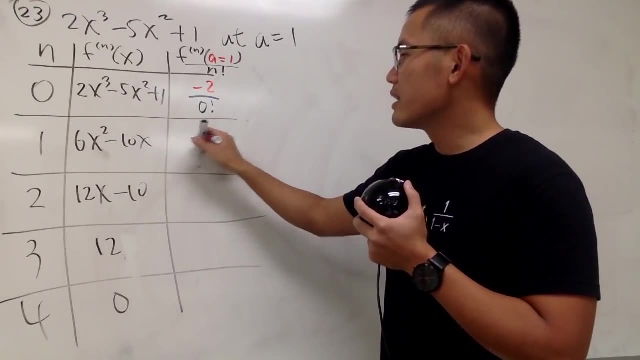 Yes, Divided by 0 factorial, Okay, 0 factorial. Next, putting 1 in here, we get 6 minus 10, which is negative 4, and then divided by 1 factorial: Good, And then next, this is factorial man. 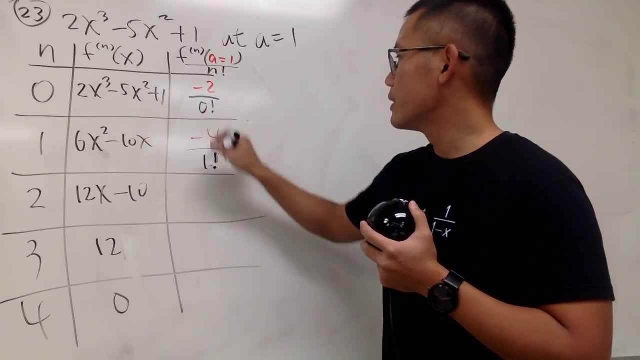 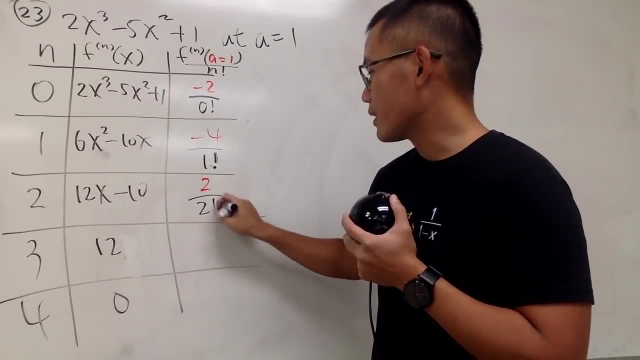 This is my factorial, And then, putting 1 in here, we get 12 minus 10, which is 2.. So we have 2, but divided by 2 factorial, And then, lastly, it's just 12.. Right. 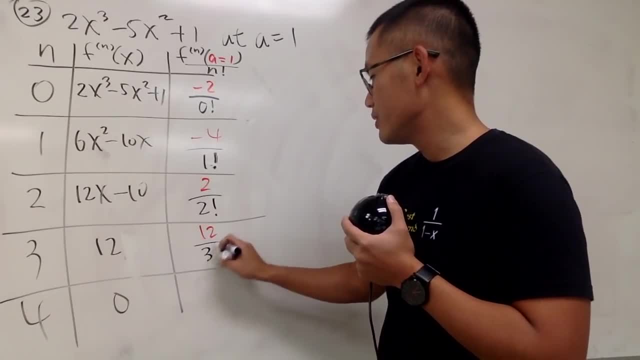 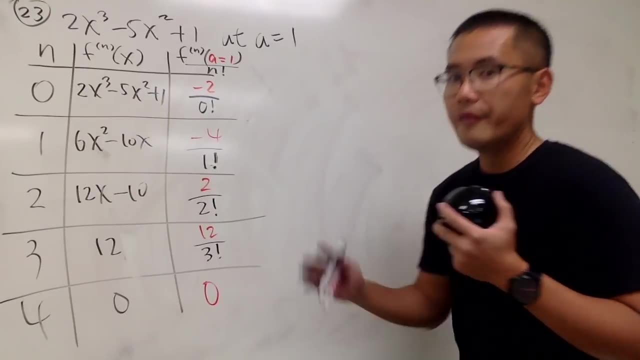 Because you didn't have x anymore Divided by 3 factorial. Well, in fact, anything after that will be just 0. So you don't have to worry about anything anymore. This is not like an infinite polynomial, because originally you start with a polynomial. 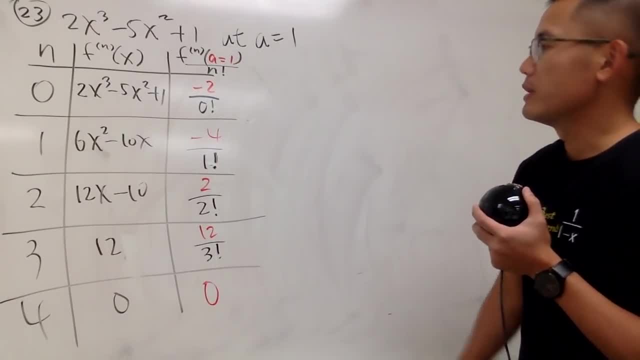 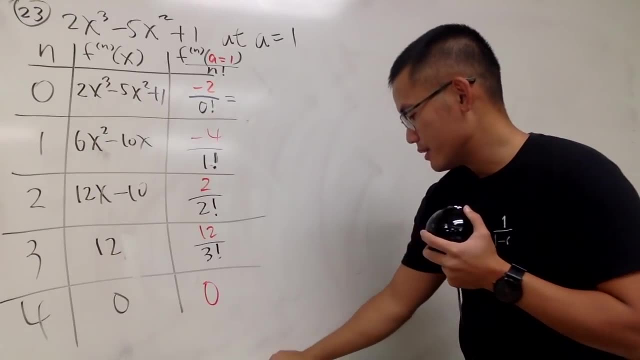 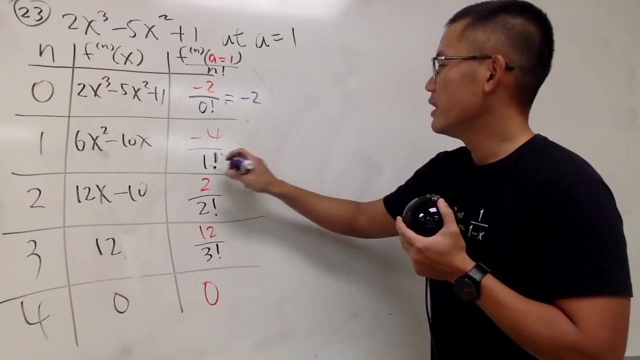 you will end Right, So let's see This right here. simplifies to negative 2. So I'll put this down in purple, just to make this cooler. This is equal to negative 2 for the coefficient, And this right here. 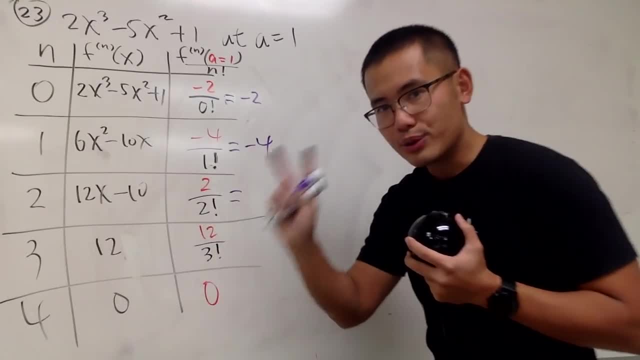 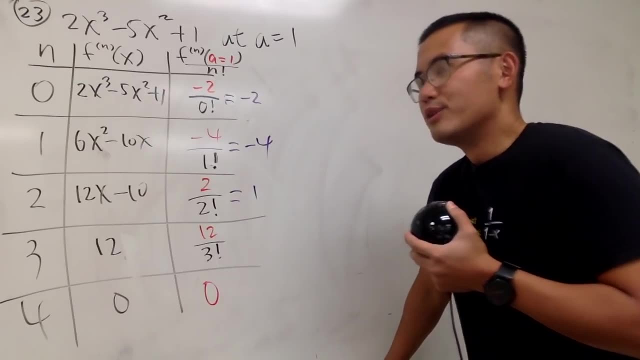 is equal to negative, 4.. 2 factorial is 2.. And you can see that my hands are really dirty. This right here is 1.. 3 factorial is 6.. Right, Because 3 times 2 is 6.. 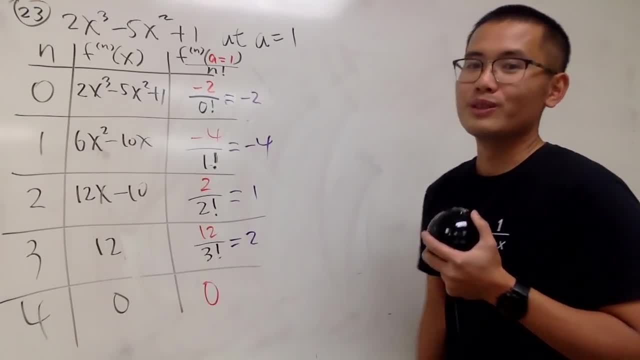 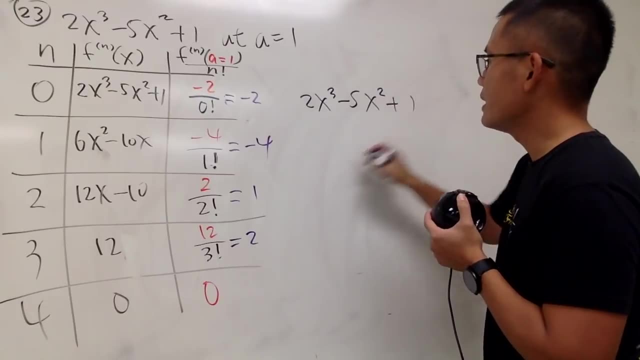 And times 1,, of course, And this right here is going to be 2., And this right here is, of course, 0.. So now here we go: 2x to the power minus 5x squared plus 1.. 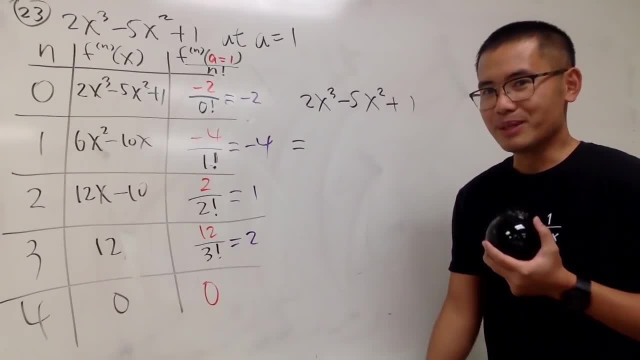 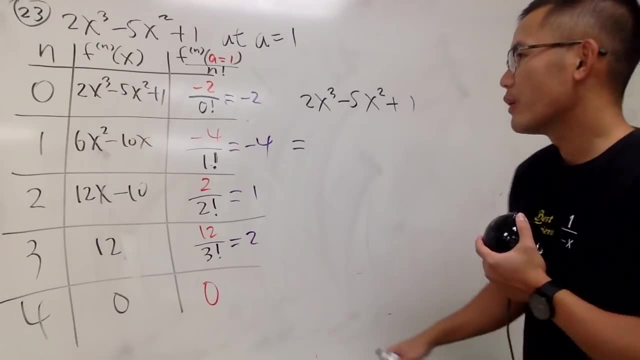 Let me tell you this one. we cannot really put it into the sigma notation because we just have four numbers And then, yeah, just write it out. That's all we do. So start with this, which is negative 2.. 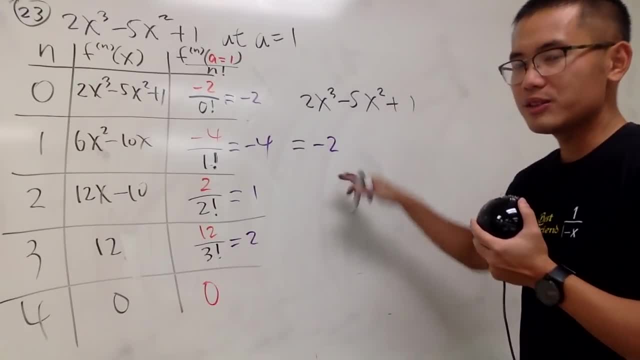 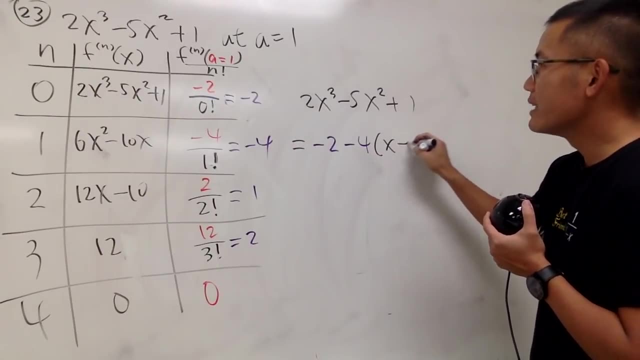 Right. And x to the 0th power. Nothing. x minus 1 to the 0th power. Next we do minus 4 times x minus 1 to the first power. Next we add 1. So we just 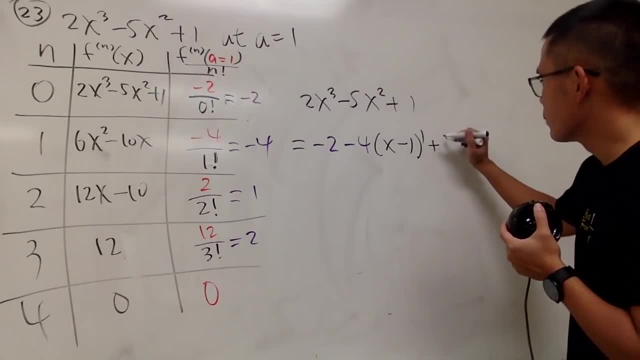 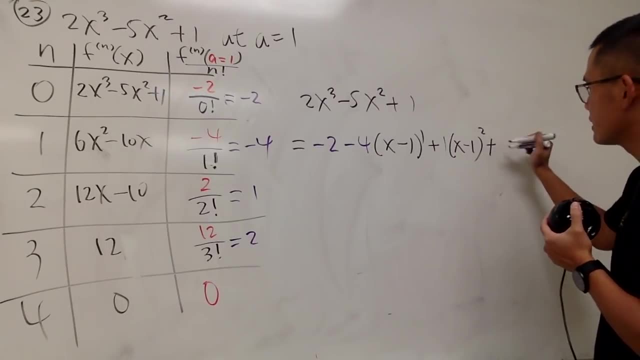 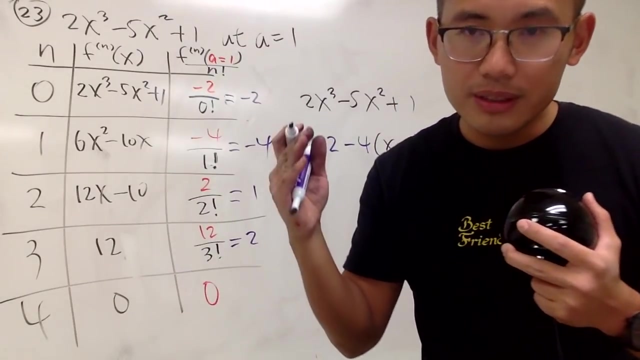 put this here: x minus 1 to the second power And the next one, we'll get plus 2, x minus 1 to the third power, Like this: And the good thing is that you stop, You stop, Okay, Let me just. 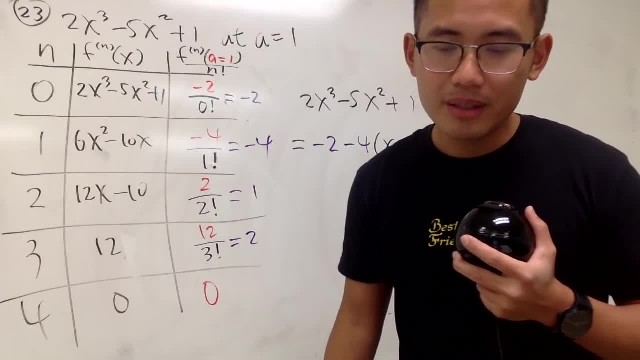 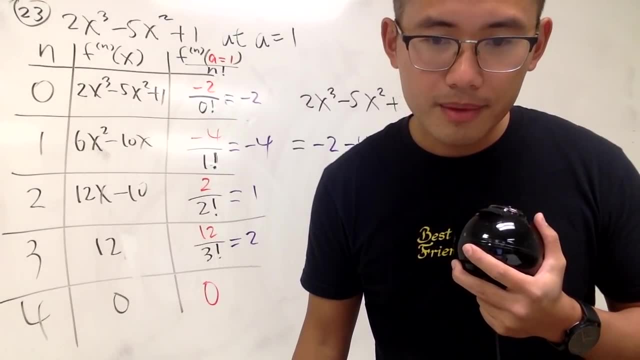 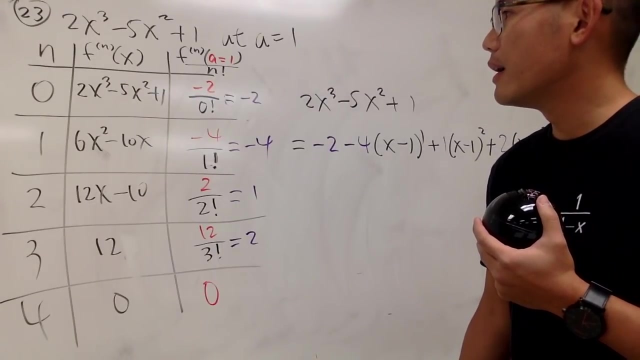 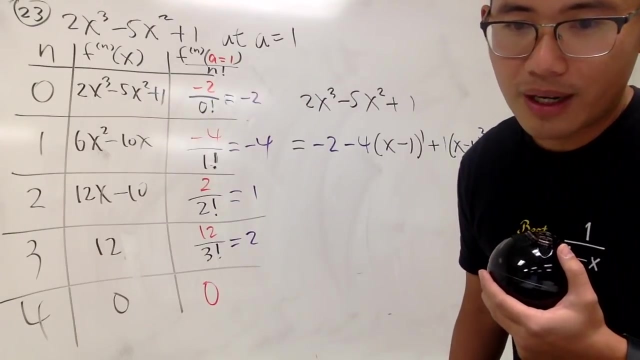 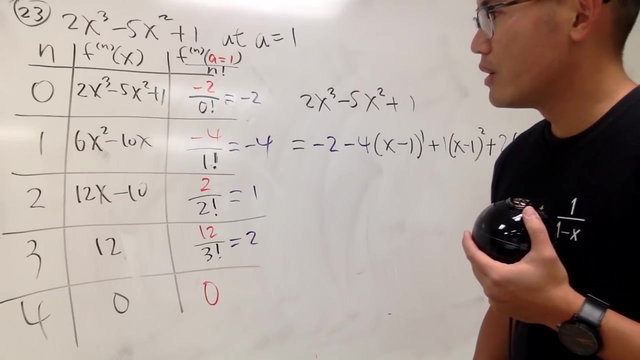 double check that I didn't make any mistake. Okay, Man, I don't know why it doesn't look right on my work. Okay, This is not funny. Why did I do that? I have a plus 8 on my answer key. 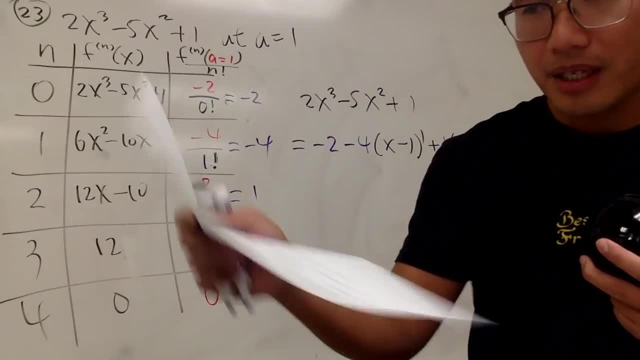 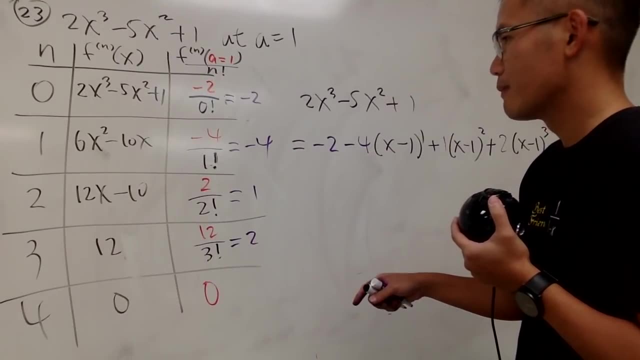 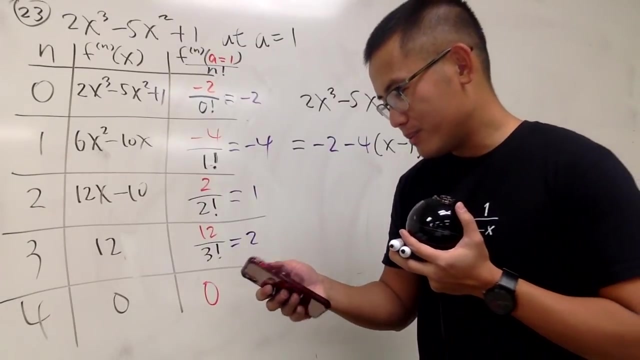 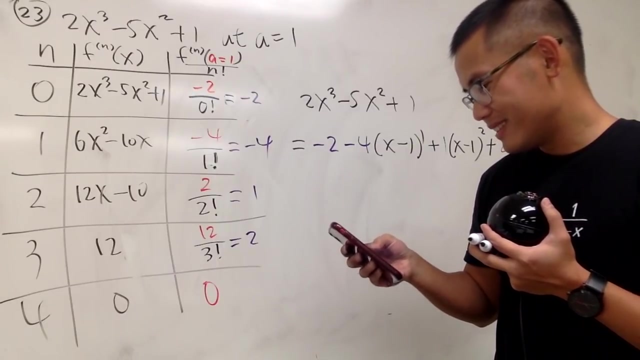 for the answer key for this term. So I will double check. As I said, most likely it's the one I'm doing right now is correct. Let me just check on Wolfram Alpha because again I want to give you guys the. 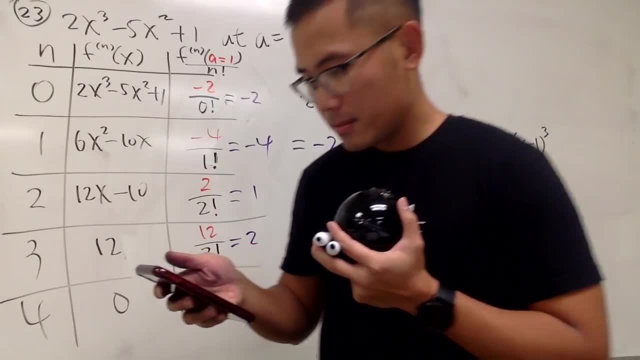 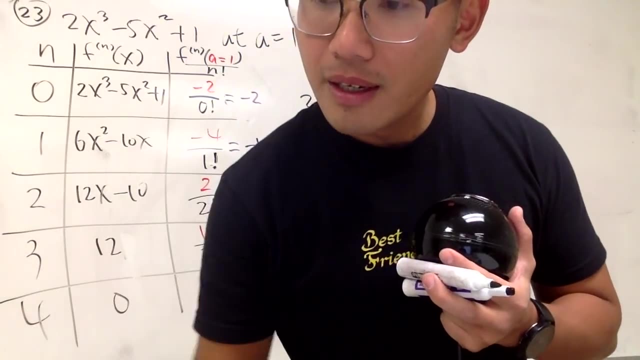 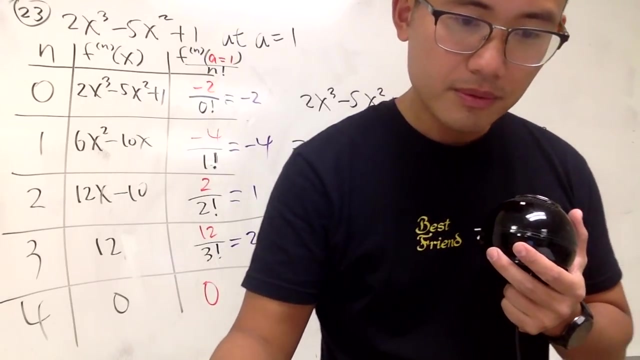 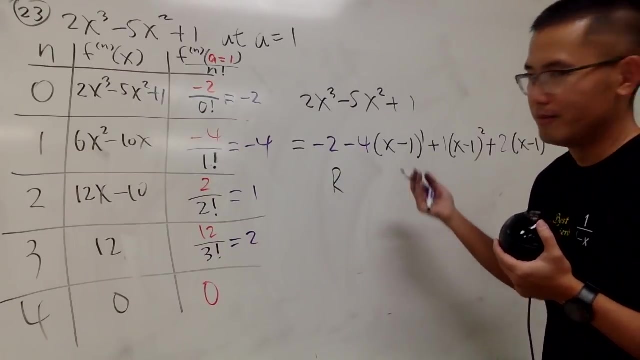 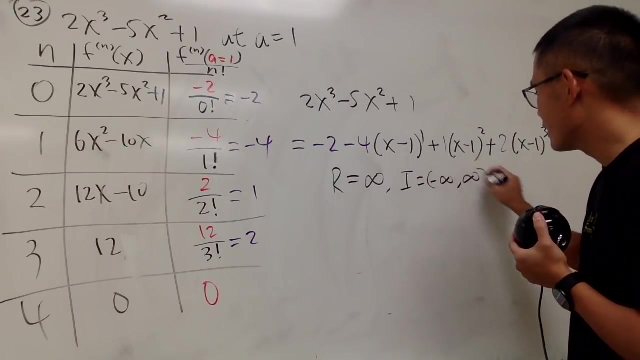 answer to this question. So I will have to fix that. Okay, Cool. So that's pretty much it. And let me tell you: they are identical polynomial. polynomial, So r is of course infinity. So yeah, So. 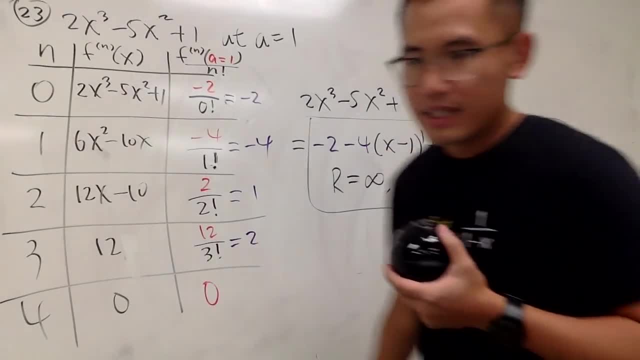 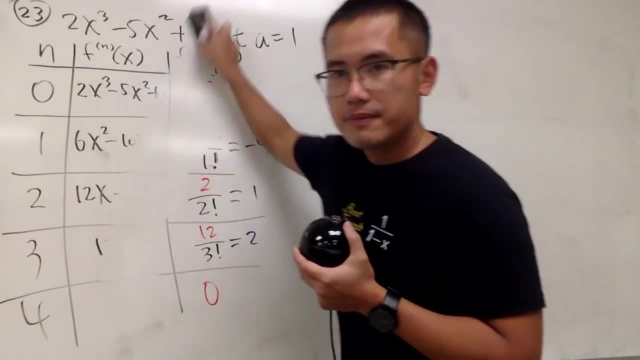 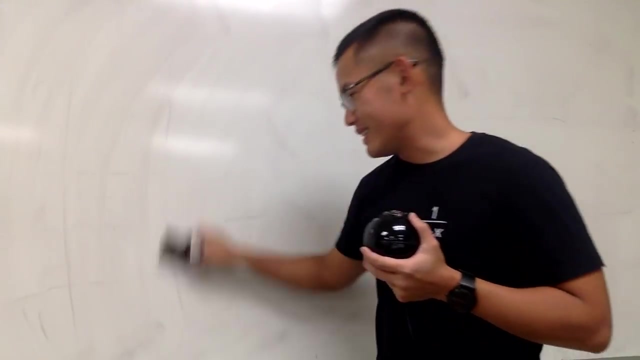 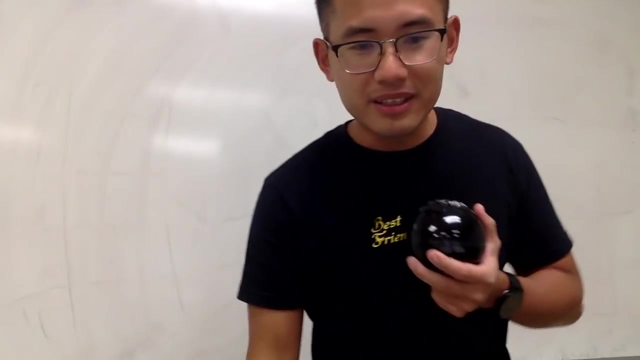 this is what you do with polynomials like this. All right, Okay, Just 3.2 more. to go Seriously, it's like running a mirror zone. That's why I picked the 26.2 out of all 30.. 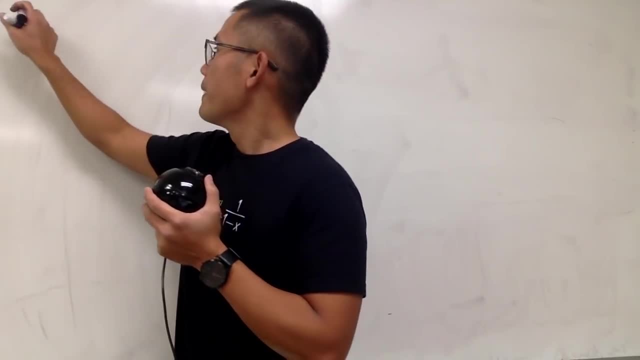 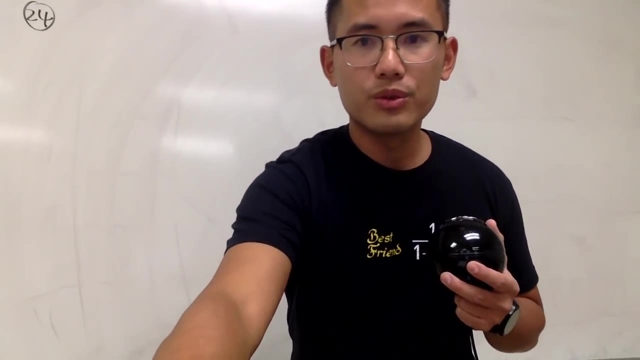 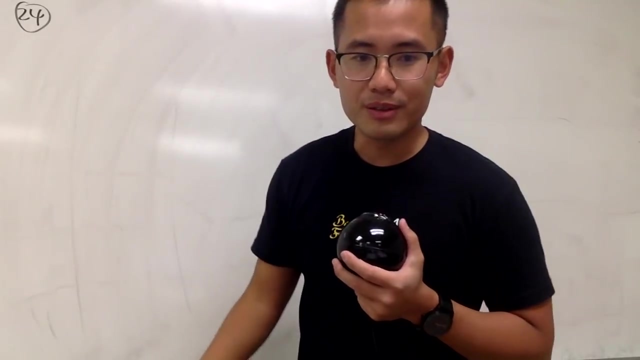 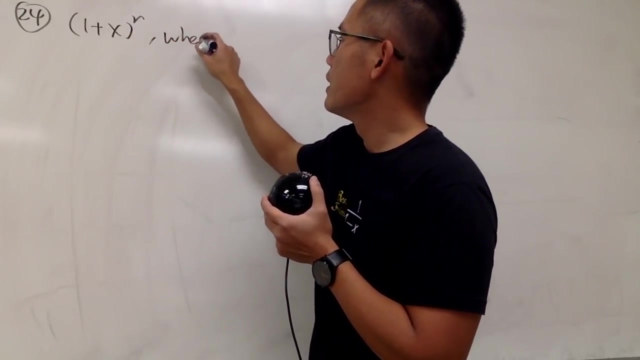 Anyway, next one. This is a famous one, This is number 24.. And for this one it depends if you are going over this or not in your class. Okay, So if you are not doing this in your class, then you. 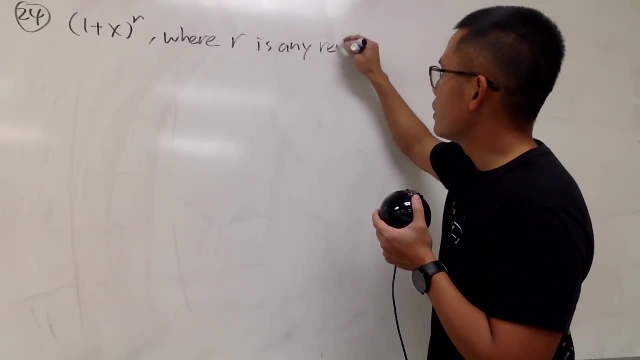 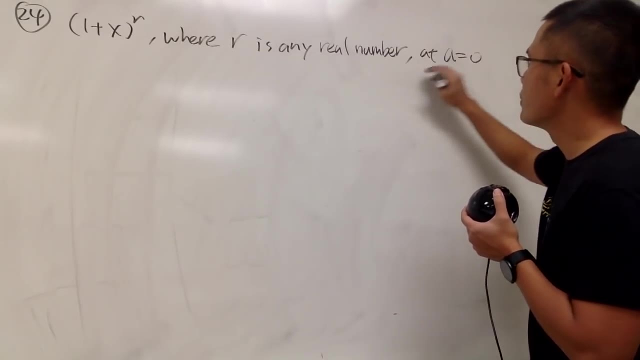 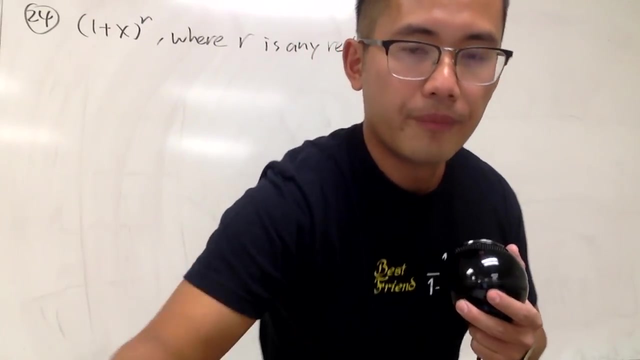 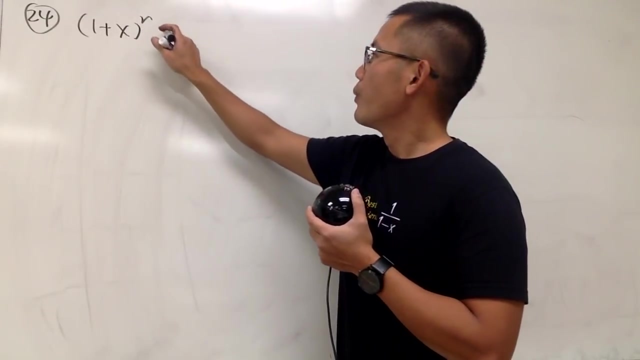 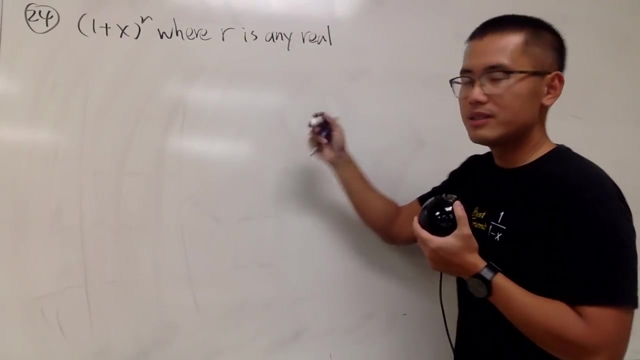 don't have any real number, All right, And we want to expand that at. a is equal to 0.. Now let me just tell you guys a few things. Okay, Why is my thing not so real? It's still the same. 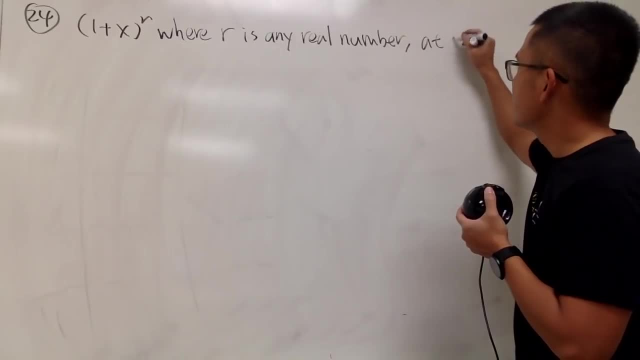 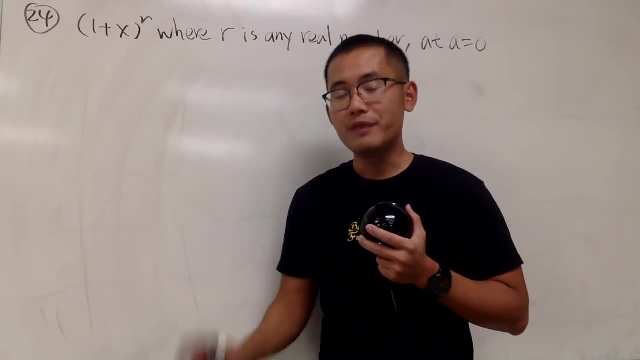 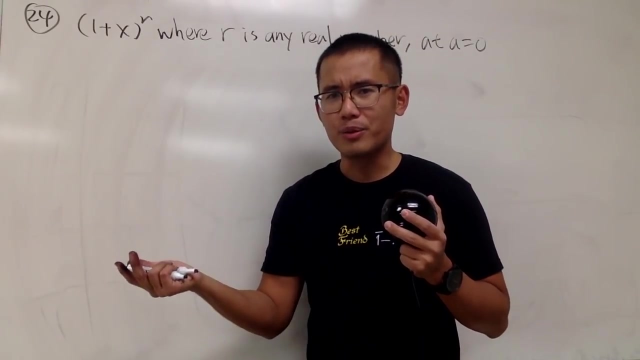 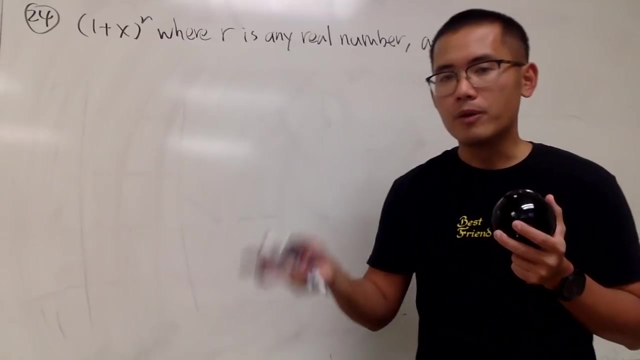 Any real number and at a equals 0.. Okay, So let me tell you guys a few things. If r is a positive whole number, or maybe if it's just 0, if r is 0, it's super easy. 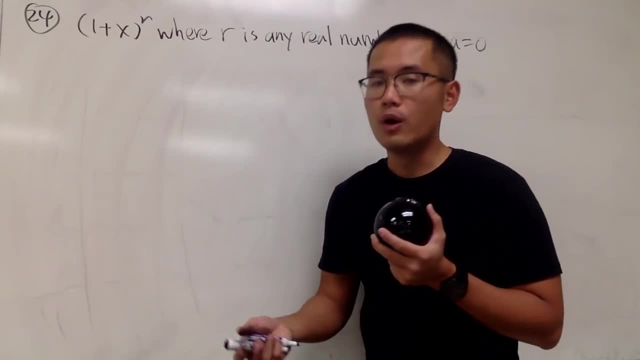 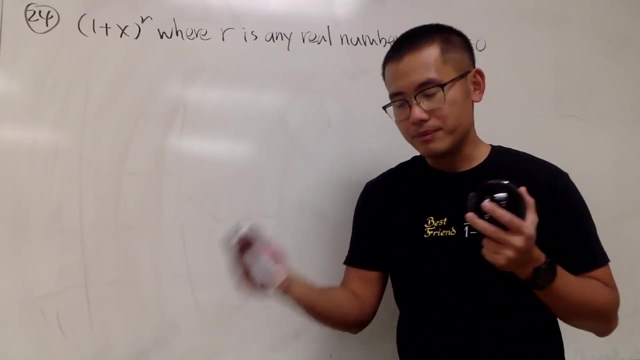 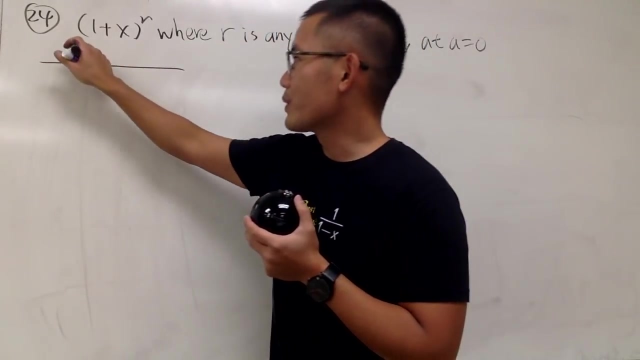 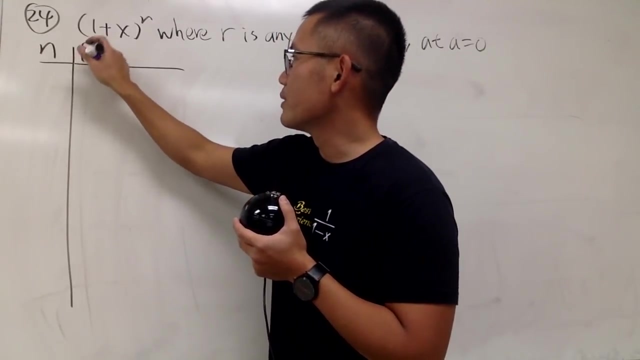 If r is a series, if r is, let's say, one-half or negative, one-third or negative five whatsoever, you can use the following one. So this right here covers the more cases, right? Hmm, Yes, you're going to. 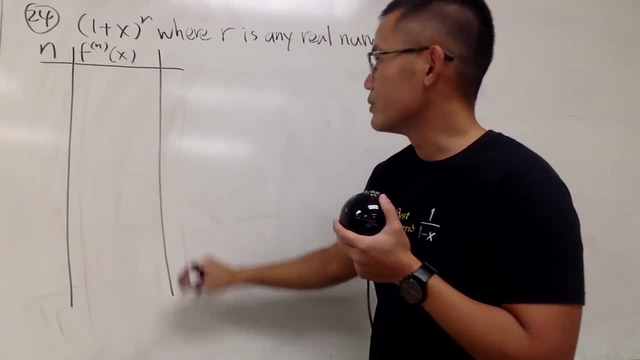 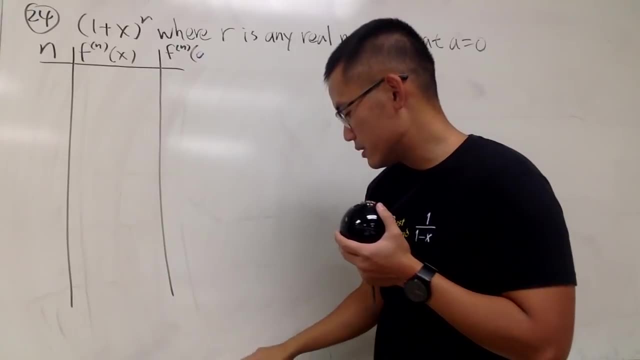 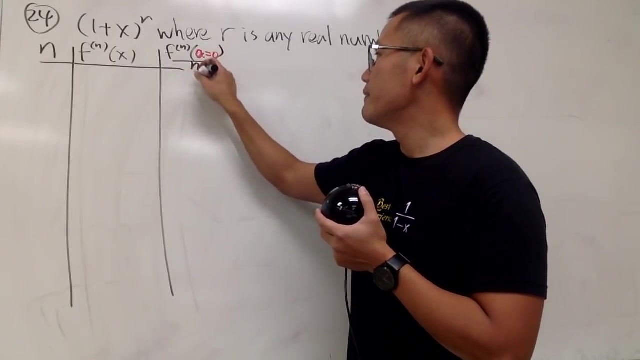 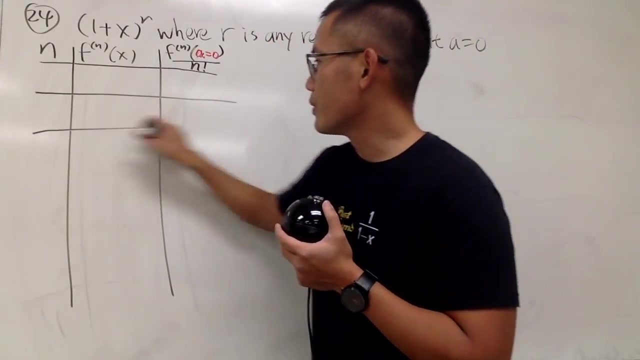 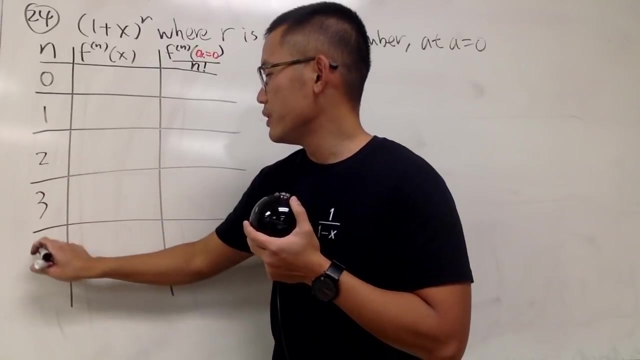 use the Taylor formula for it. And this is what. Yeah, the formula. And a is at 0 over m factorial. Okay, So just like this. Now check this out. This is kind of weird, so just kind of. 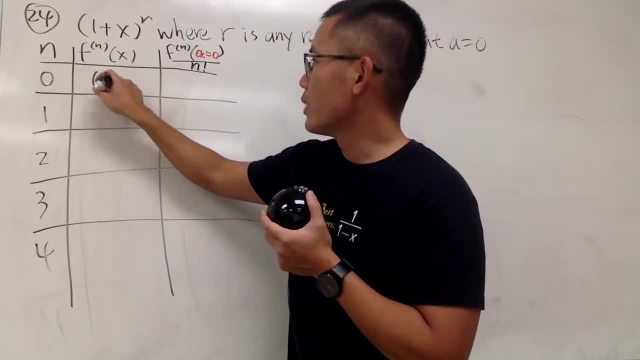 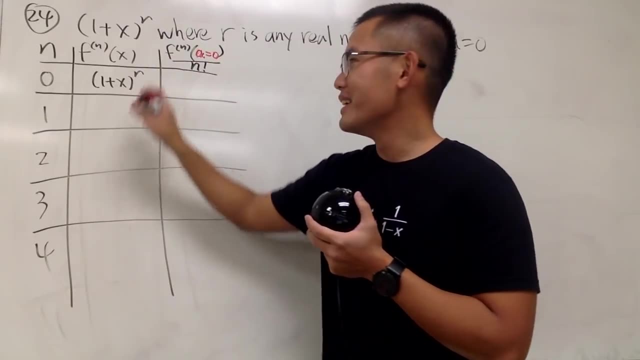 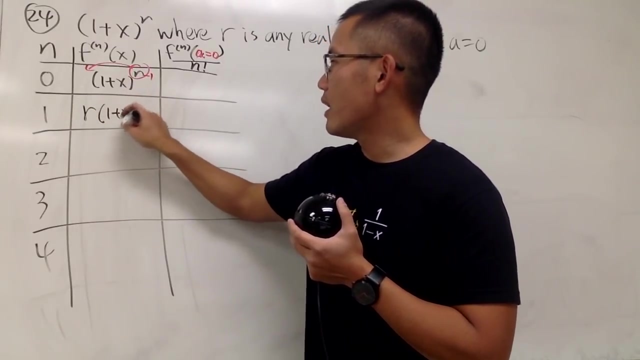 bear with the original one, which is 1 plus x to the r power Derivative. this, I mean, differentiate this: you bring the r to the front and then minus 1, yeah, So you get r and then 1 plus r. 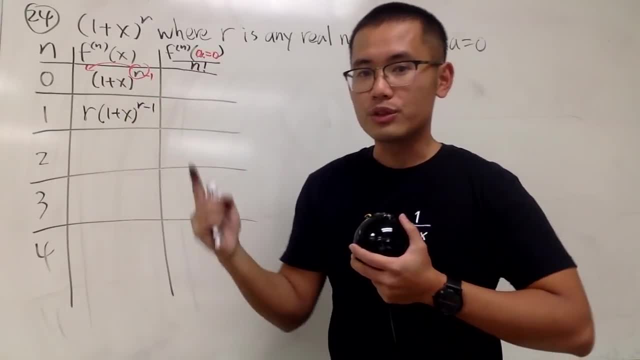 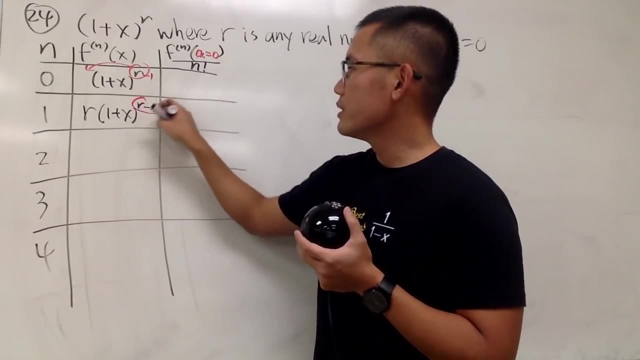 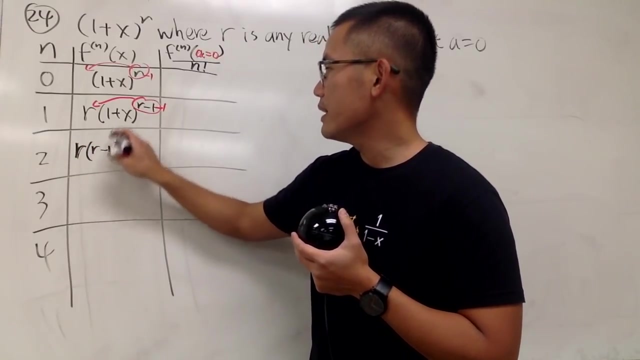 and then 1 plus x to the r minus 1 power, like this: Now, if you differentiate this again, though, if you bring this power to the front and then minus 1, you get r times r minus 1, and then this is: 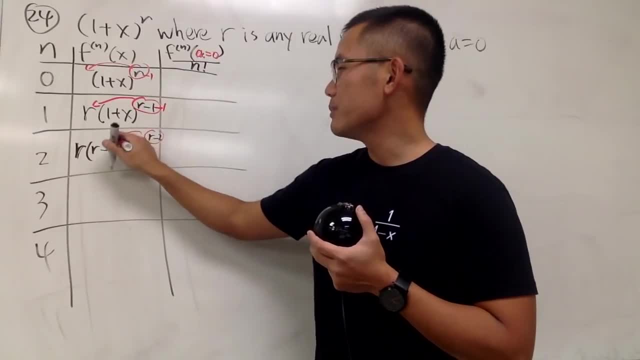 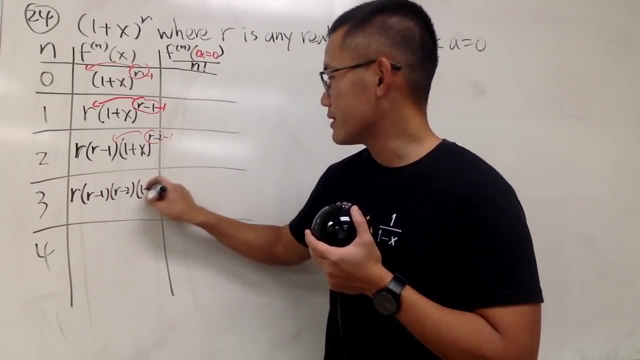 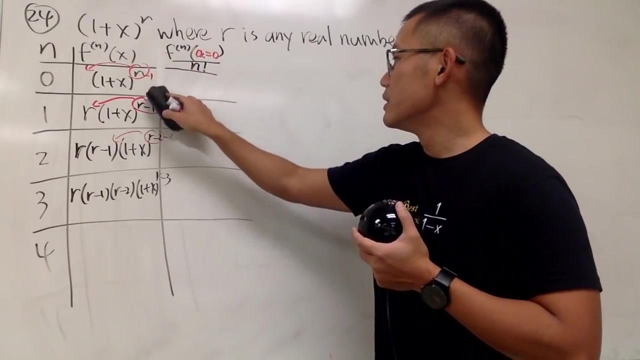 1 plus x to the r minus 2, right, And you can kind of see the pattern: if you just keep going, You get r r minus 1, r minus 2, r minus 3,. you get r times x. 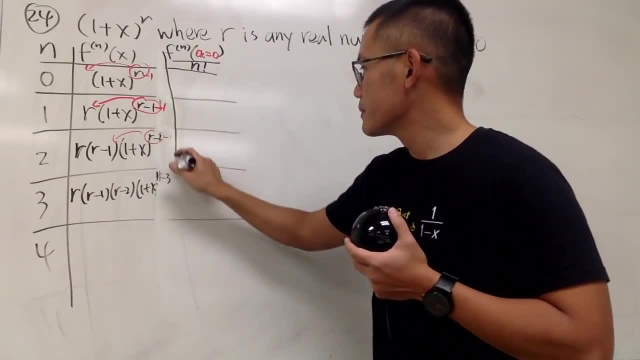 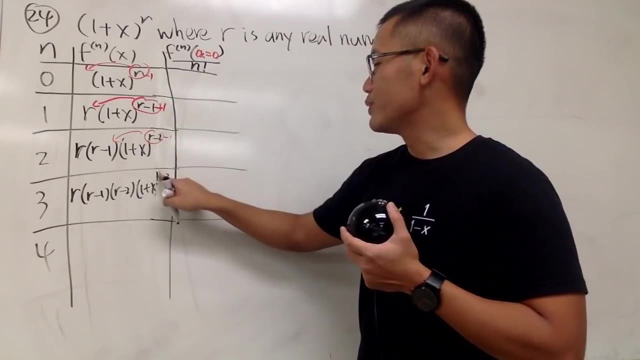 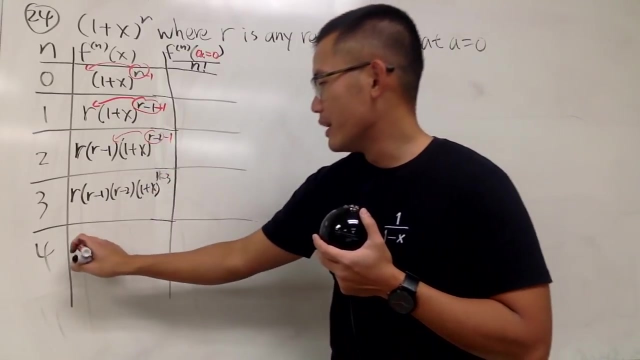 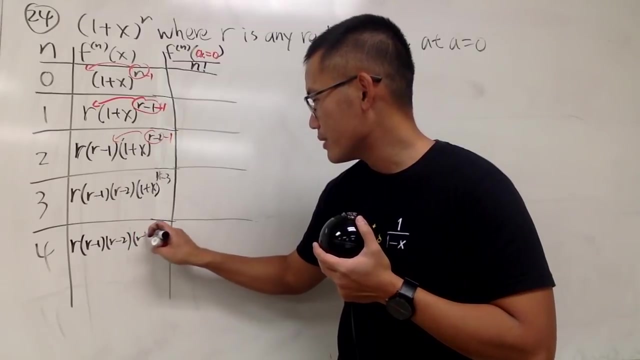 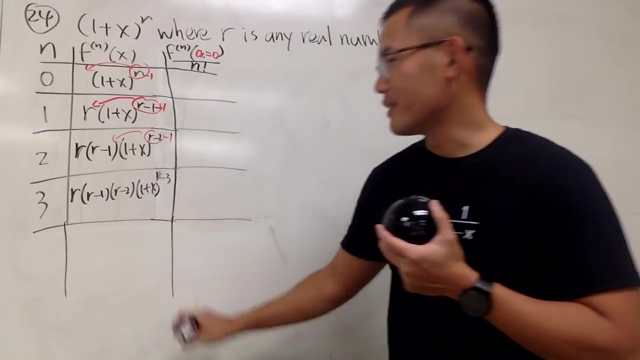 to the r minus 1, minus 2, r minus 3, and then you get r times x to the r minus 1, r minus 2, r minus 3, and y to the r minus 3,. let me just stop right here. so we have three terms, so that should be enough. 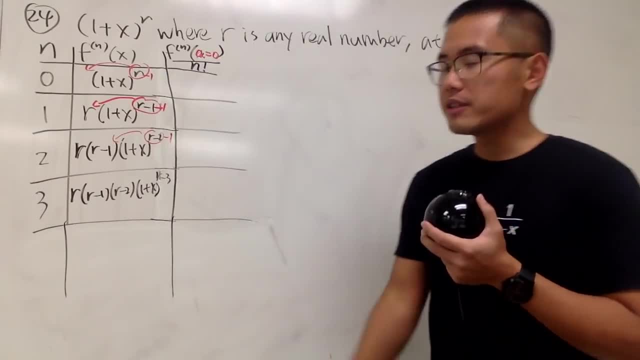 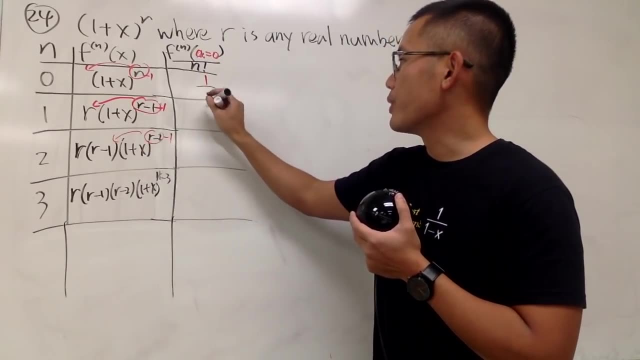 right. so that's what we have. now check this out: when I'm putting 0 into x, the first thing I get is just 1, and then over 0 factorial. so that's good, that's no big deal, okay. 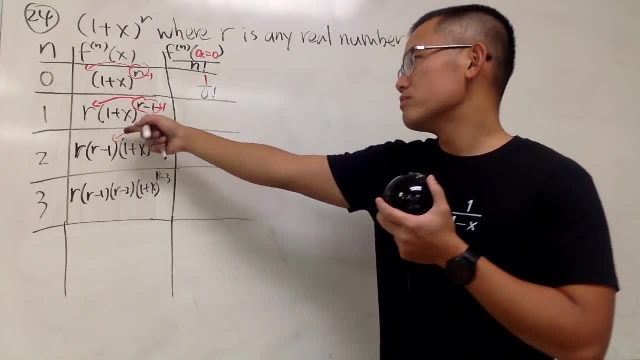 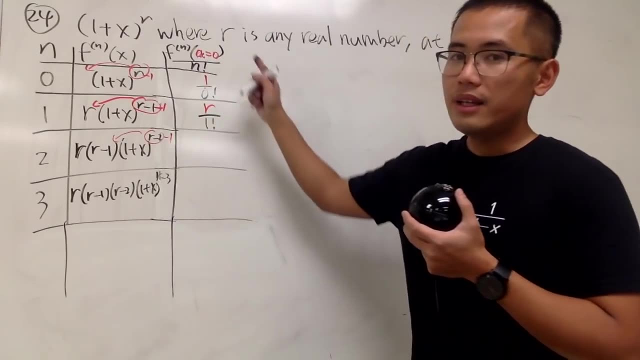 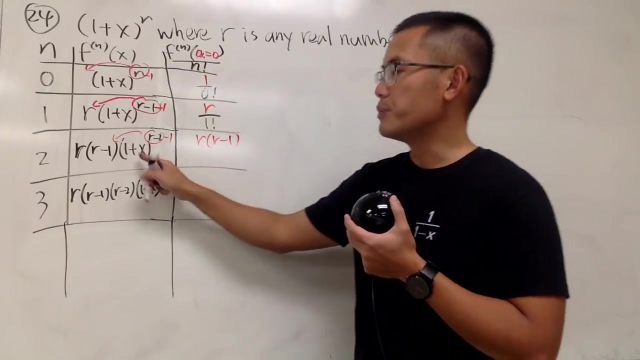 when we're putting 0 in here, I just get r times 1, which is just r. so that's good, that's just r, again, nothing crazy. and then over 1 factorial. next, if I put this right here, we get r times r minus 1, so we get r times r minus 1, because if you put 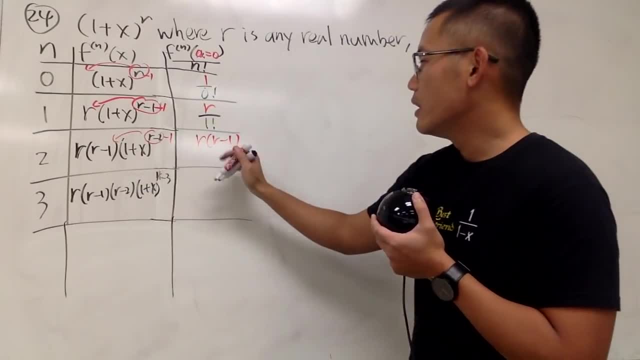 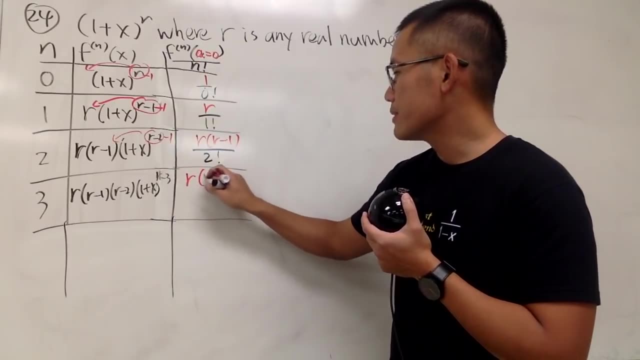 0 right here, this is just going to be 1 anyway. so we have that and over 2 factorial, and you can guess the next one. it's going to be r times, r minus 1,, r minus 2, and then 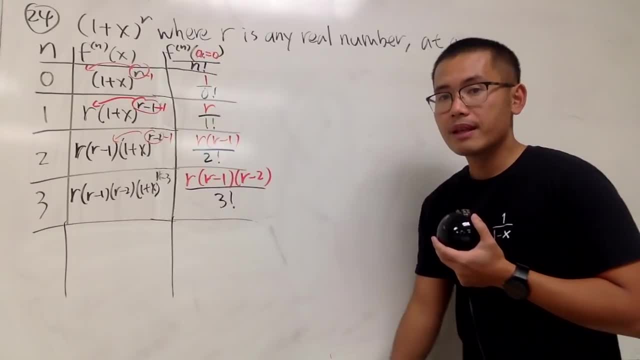 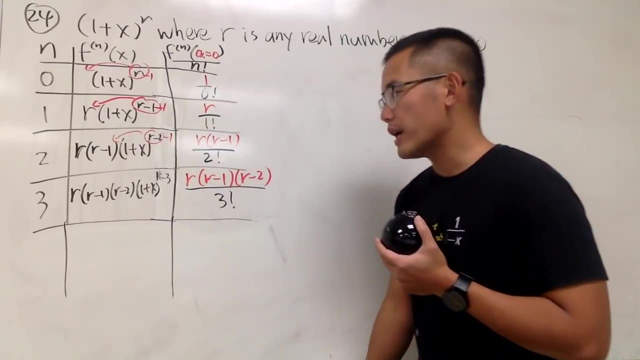 divided by 3, factorial, And so on. so you can guess. the next one is: r times r minus 1, r minus 2, r minus 3, over 4 factorial, and so on. right, therefore, let's go ahead and just come up with a pattern. 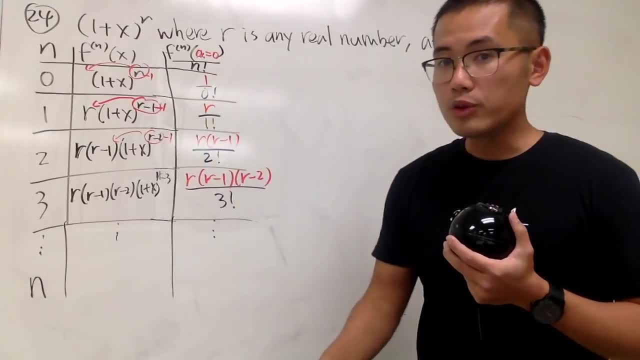 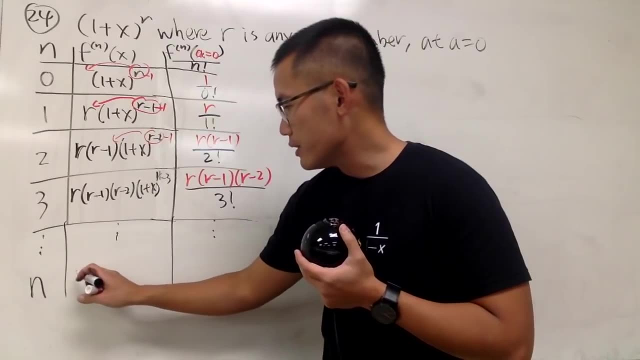 for this already when we have n. well, check this out earlier. when I have 3, I start with 1,, I stop it at 2, right? so here's the deal. if this is n, and let me make this in purple- 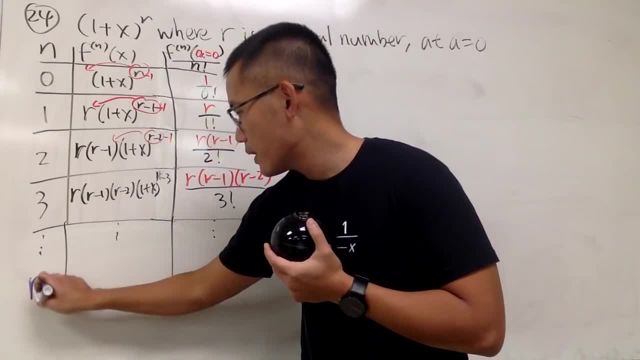 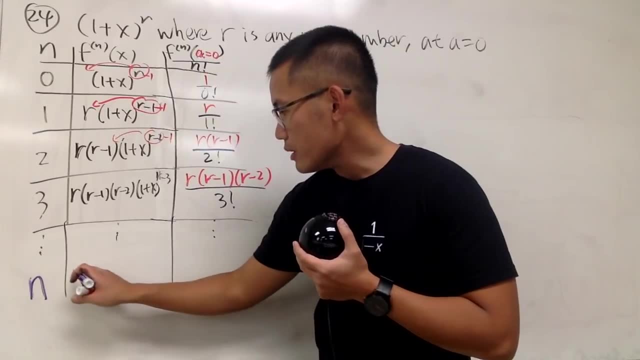 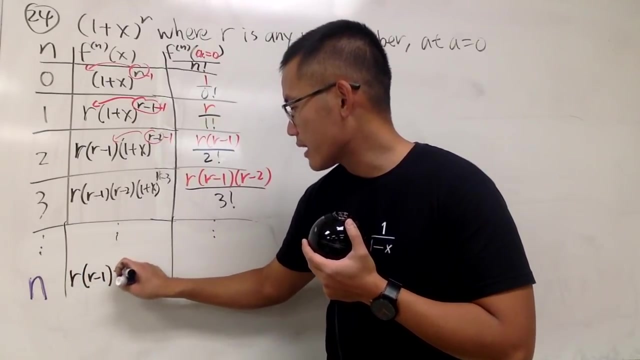 I will say: if this is n, Let's see how it should already. okay, if this is 3, I stop it at 2, so right here, I will get this. this will be r and then r minus 1,. dot, dot, dot, right, and then we. 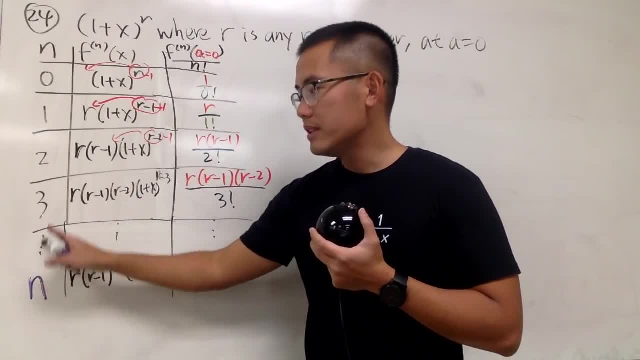 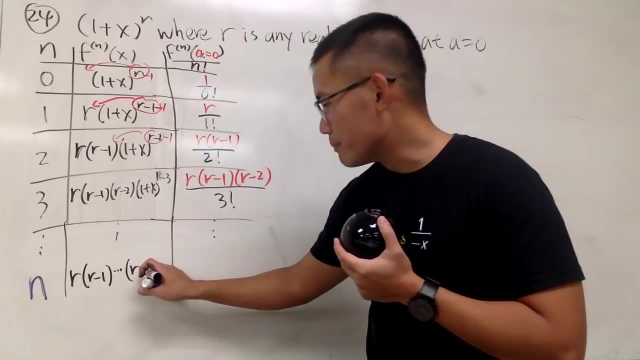 have to stop it at 1 less than whatever this is. This was 3, so you stop it at 1 less. right? so you stop it at 2,. so if this is n, we have to minus n, Okay. 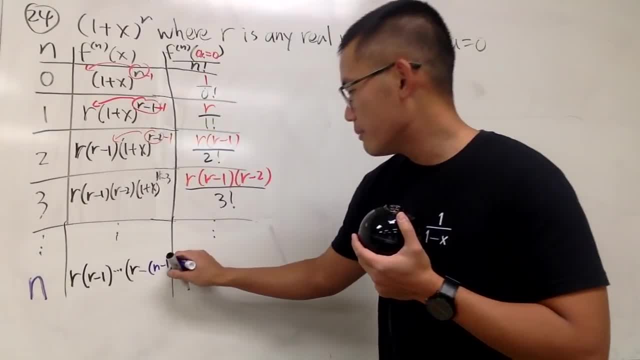 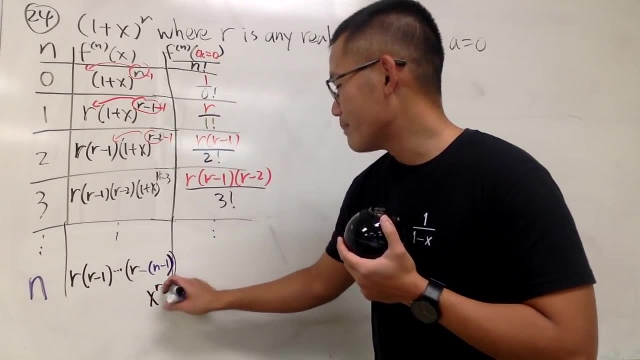 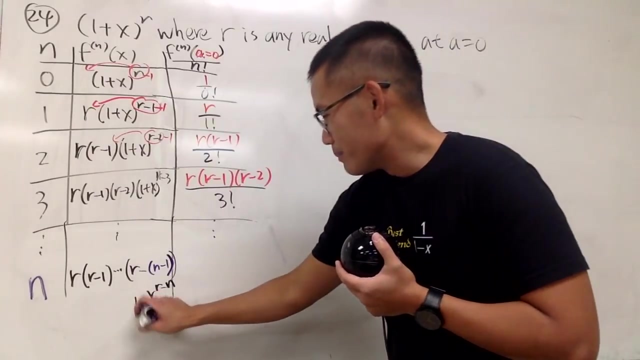 n minus 1, like this: n minus 1, in the purple parentheses like this: and then multiply by x to the r minus, this will be 3, so, yeah, so it will more be like this: oh, 1 plus. 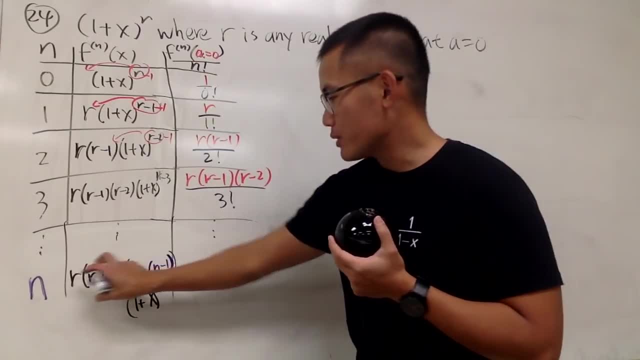 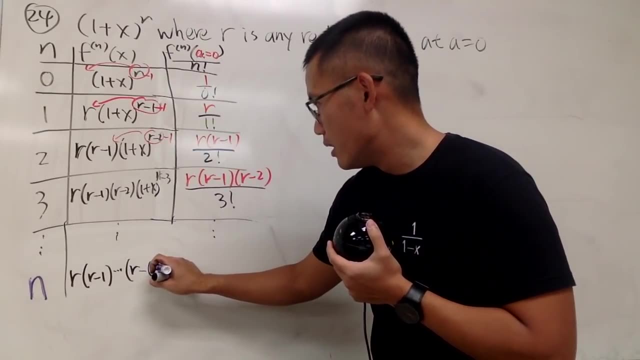 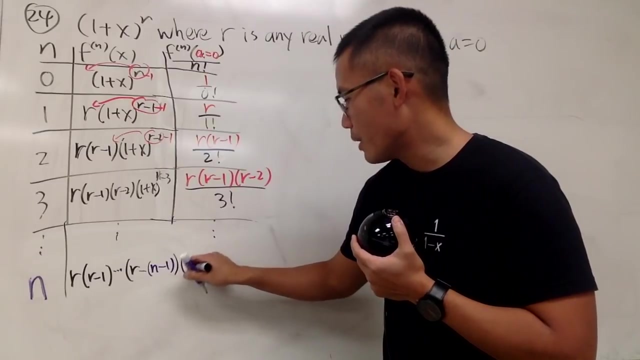 sorry, sorry, yeah, okay, so it's pretty much all this code. let me just write it down better. yeah, so it's all this: n minus 1, because it's 1 less right, and then you multiply by 1 plus x to the r minus. 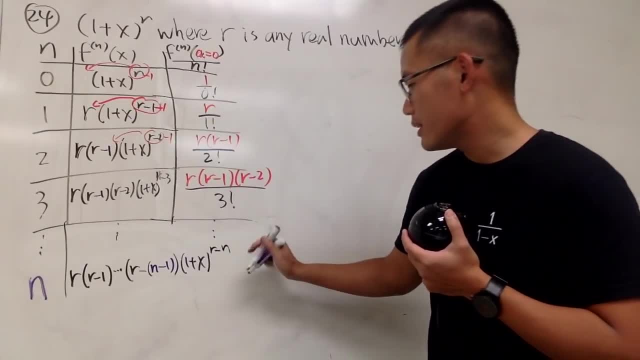 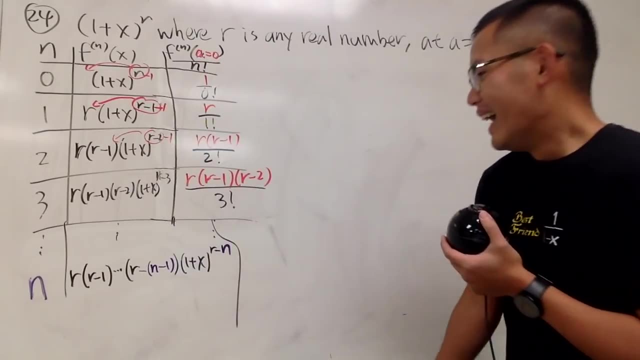 n's power like this: yeah, n's power, okay, And in the end, let me just write it down like that: When you're putting 0 in here, well, you just get all that, which is: I'll put this down. 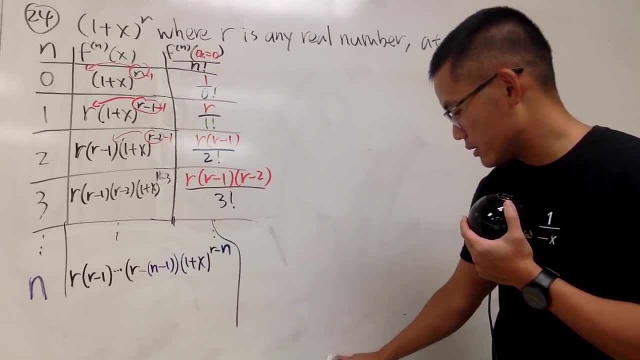 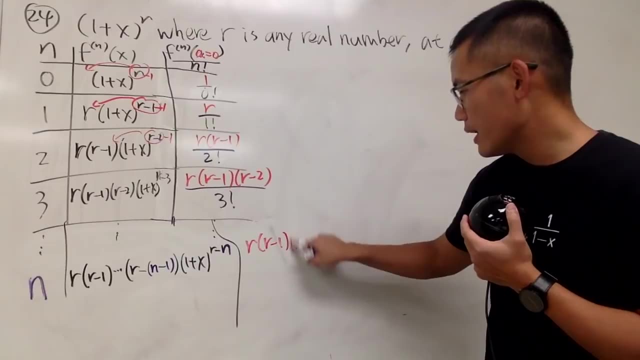 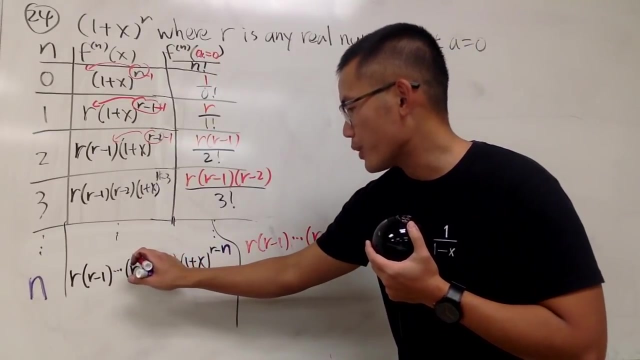 in red, Which is Okay, Okay, Okay, Okay, Starting with r, and then r minus 1,, r minus 2, and so on, so on, so on, and the last one we do is going to be r minus, and of course, you can distribute this real quick. this is: 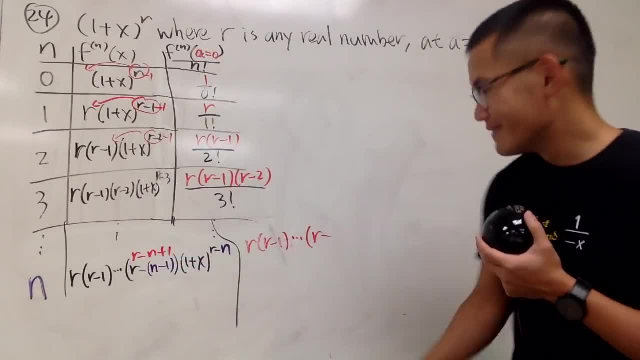 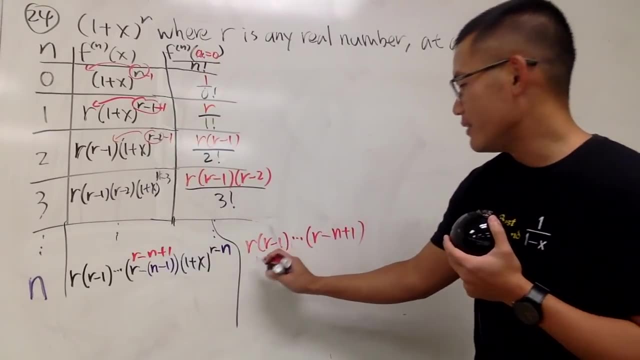 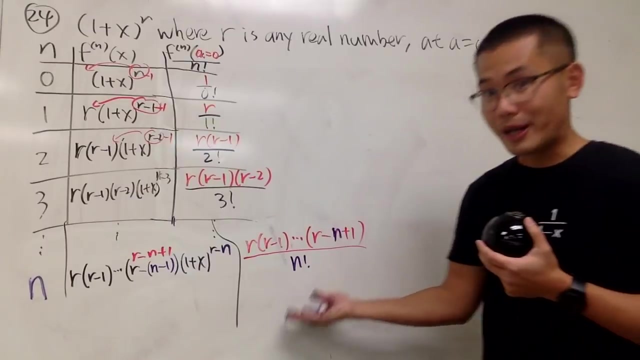 r minus n and then plus 1.. So we have r minus n plus 1.. That will be the derivative. And don't forget to divide it by the factorial. so divide this by n factorial, like this. But in fact, this right here, this right here, is the formula for the coefficient for that guy, right? 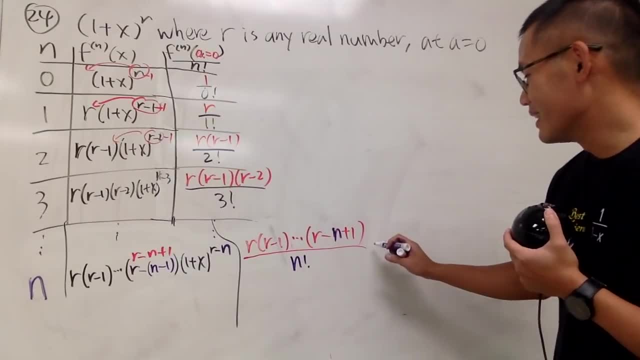 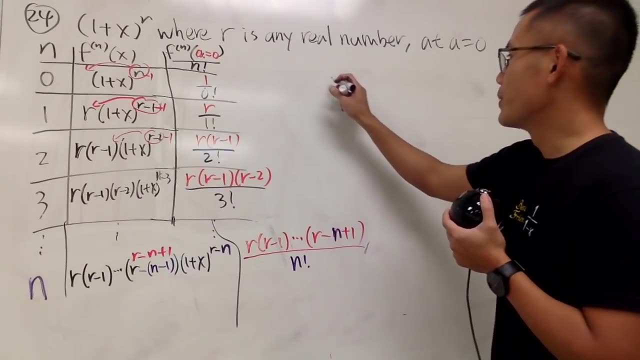 And the truth is we do have a nicer way to write this. This is how we define: I already done for you guys. already done for you guys. So let me just put this down right here for you guys already. This is the sum as n goes from 0 to infinity. 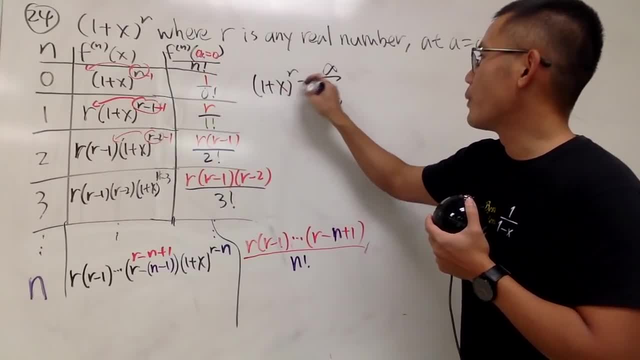 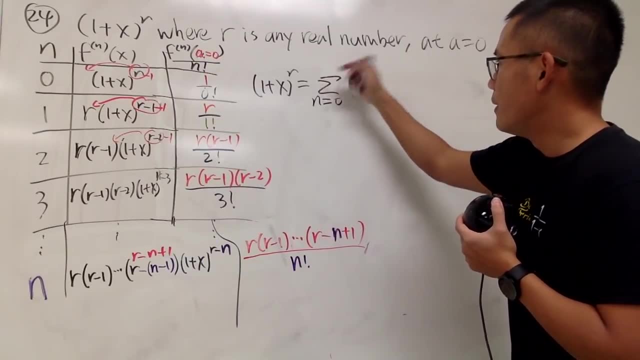 This is for the expansion 1 plus x to the rth power. What you have is that you write this down, which is all that, which is all that right, But a much better way to write this down is the following. 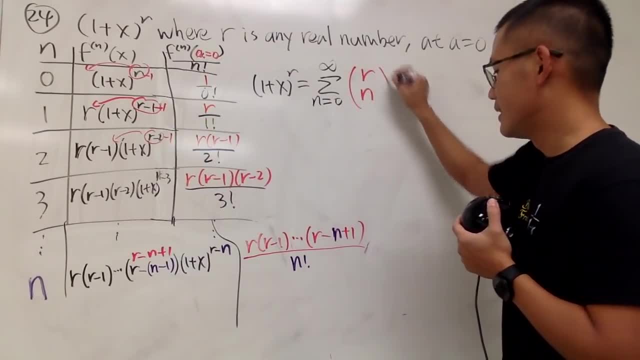 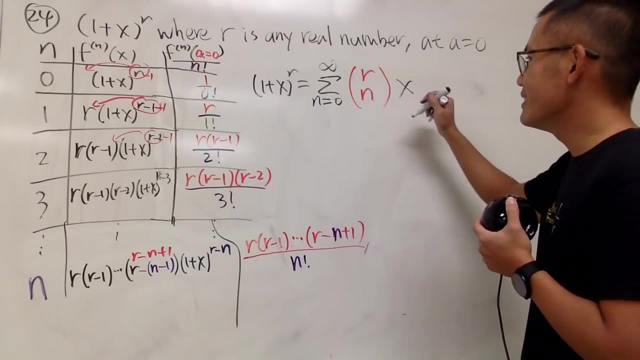 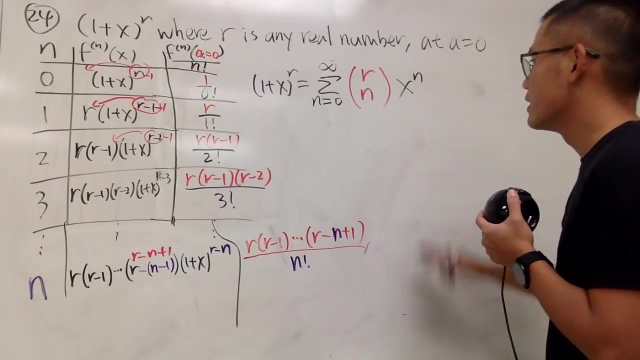 You can just go ahead and write down r, choose n like so, And then you multiply by x to the nth power. yeah, nth power, and like that, And again the center is at 0, so just x Minus 0 is just x, like this, right. 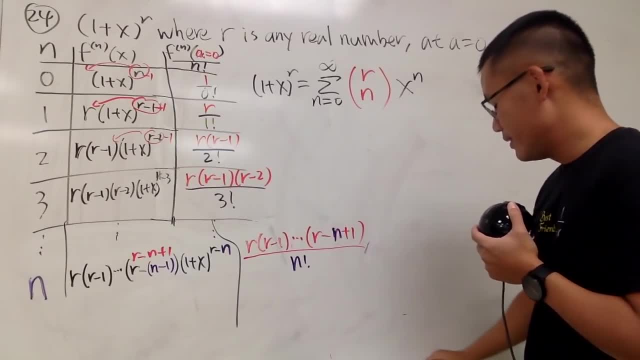 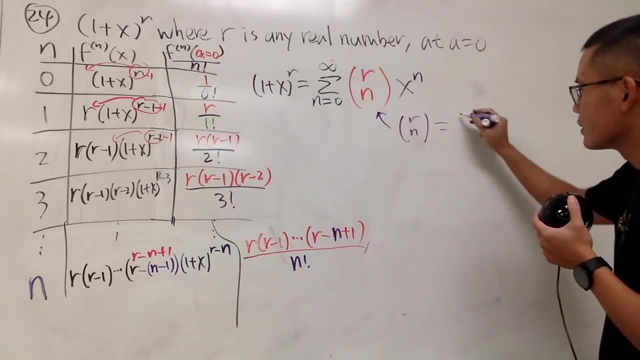 And now, what's this, though? This right here is precisely that, So I will just have to tell you: r choose n is precisely that, So it's r. r minus 1, r minus 2, dot, dot, dot. 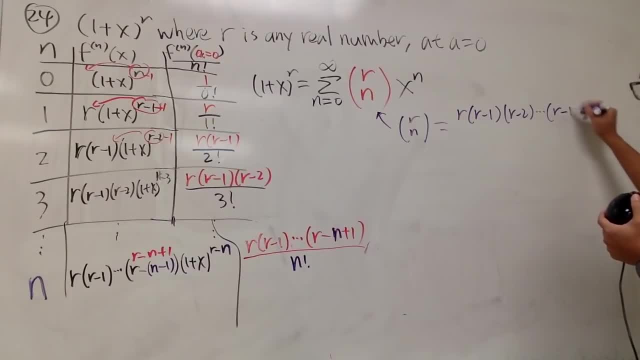 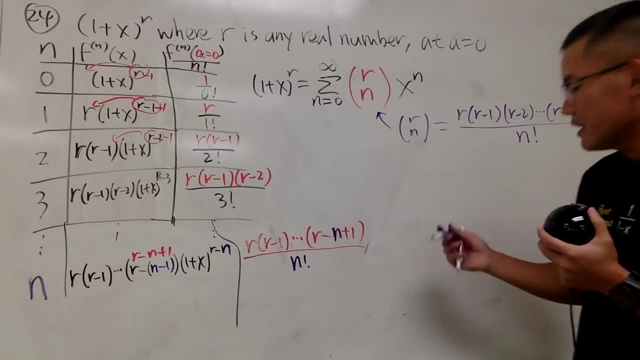 And we have r minus n, plus 1, or over n, factorial, like this. So let me give you guys some example, and it's rather bizarre. So here is an example. For example, if I have, let's say, 5, choose 3.. 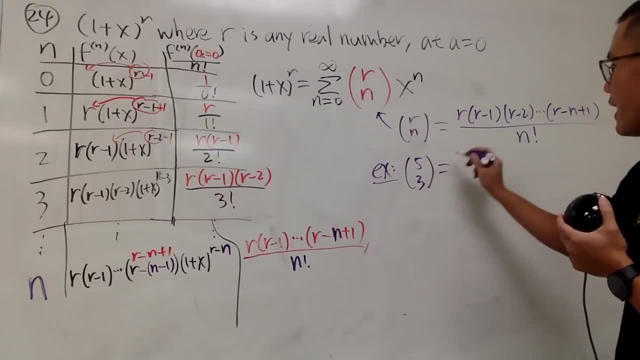 And the way you can say is: 5, choose 3.. What you can do is you start with 5, you go down next one, which is 4, and then you go down again, which is stop at 3.. Right, so this 3 tells you how many times you go down. 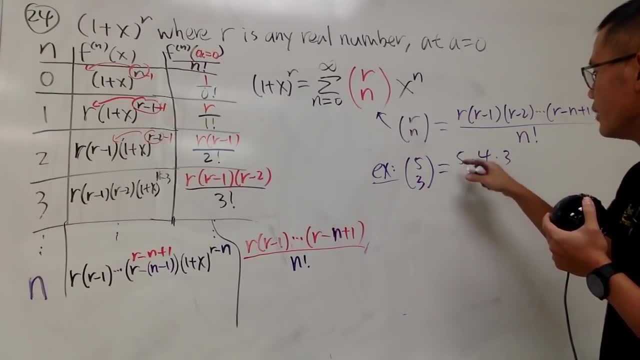 So you see, well, you have to have 3 numbers. sorry, Instead you go down once, you go down twice. But you should have 3 numbers right here. So again, if you follow 5, you go down twice, right? 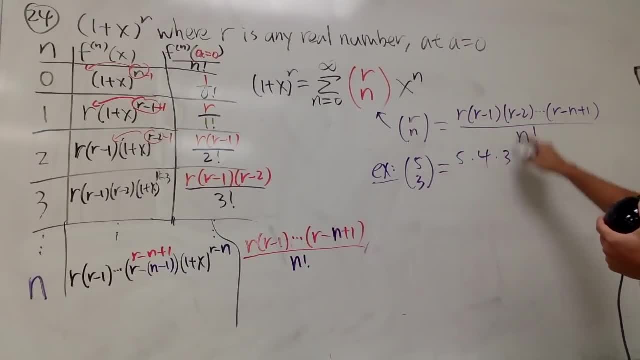 5,- right, That's 5, and then 5 minus 1 is 4.. And then 5 minus 2, and you stop it at. you do r minus 2 right here. so that's pretty much it. 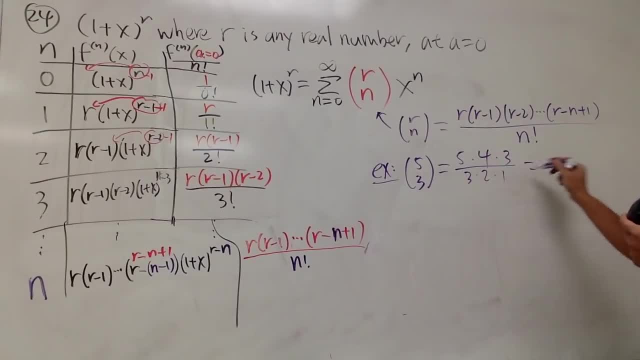 And divide it by 3,, 2,, 1.. On the top is 120, and on the bottom is 6.. So no, on the top is 60,, on the bottom is 6,, so it's 10.. 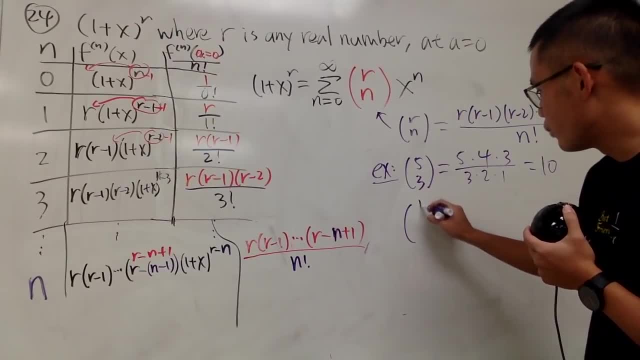 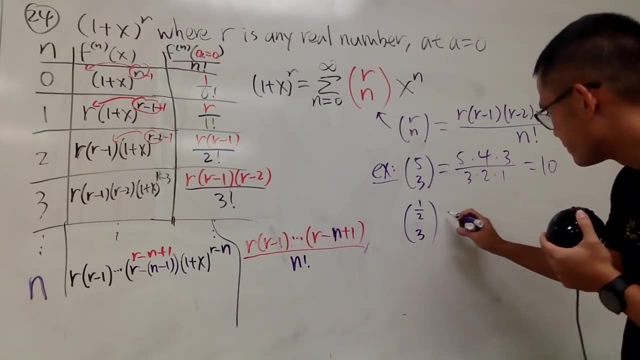 So that's an example. Let me give you guys another one. So suppose you have 1 half choose 3.. I didn't prepare this. I'm doing this in my head, so we'll see If we have 1 half choose 3, this is what we do. 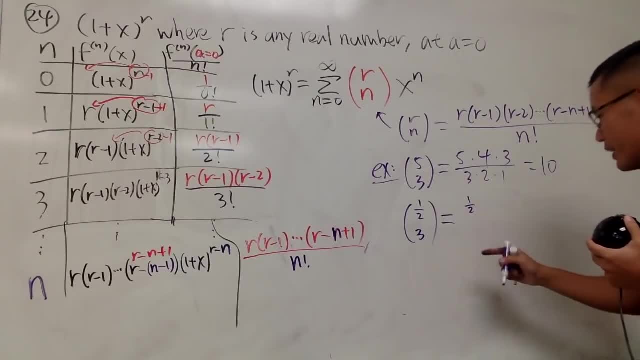 You start at 1 half. you start from 1 half, Next you do 1 half minus 1.. Next you do 1 half minus 2.. So again you have to have 3 numbers and then you divide it by 3,, 2, 1,, namely 3 factorial. 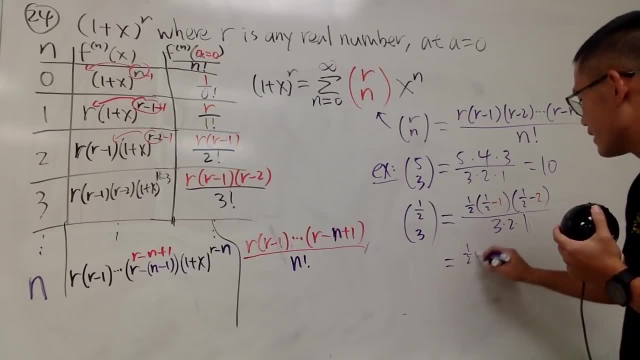 And then we can just do the math in your head. We'll just do the math: This is 1 half times 3.. This is man. this is negative 1 half, yeah. And this is negative 3 over 2, yeah. 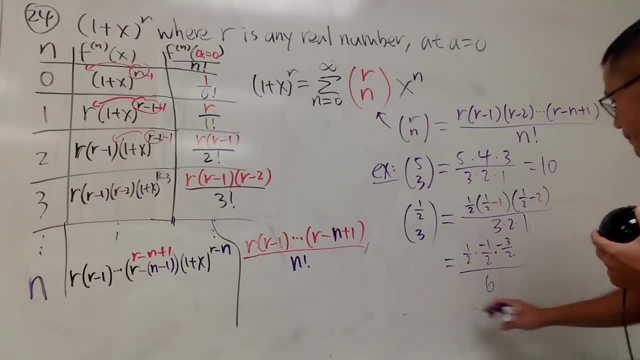 And over 6. Okay, this is 8. On the bottom is 48. And we have 3 on the top and this is positive. So altogether it's 1 over 16.. I believe this is the answer. 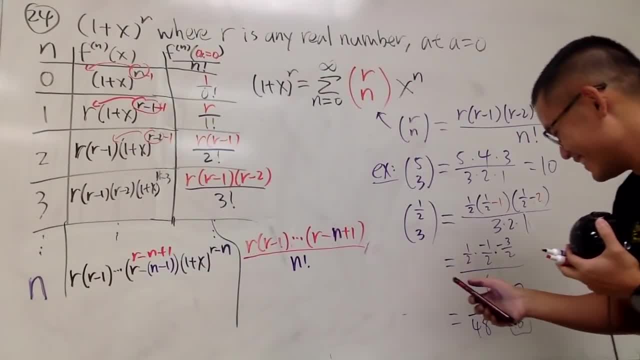 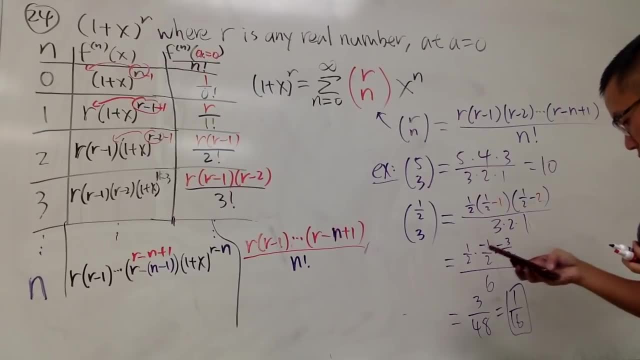 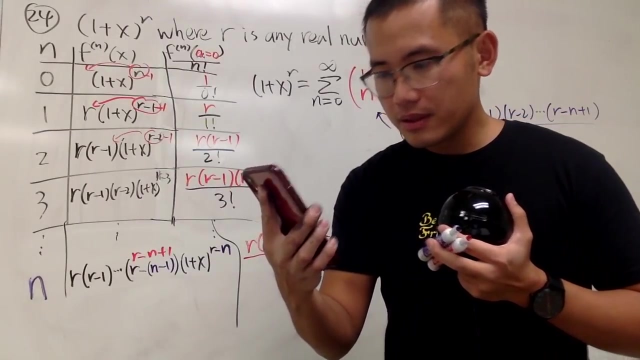 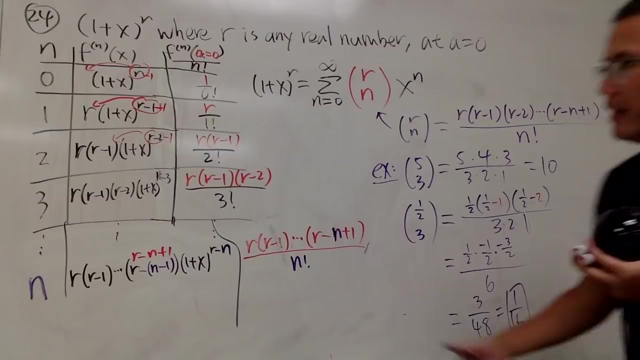 so let me just check WolframAlpha real quick on this. So the way you do it is just say 1 half, choose 3.. Hey, hey, I got it right. So that's pretty much the idea behind the coefficient. right here and again, this is the proper way. 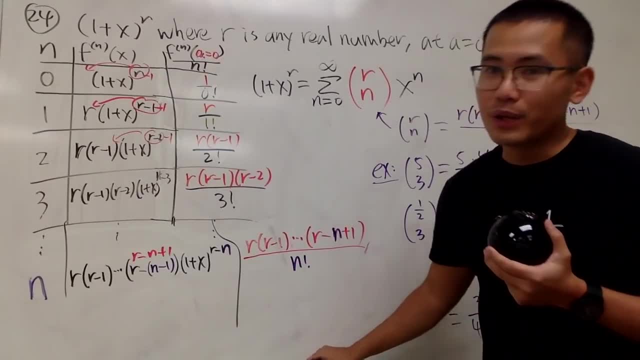 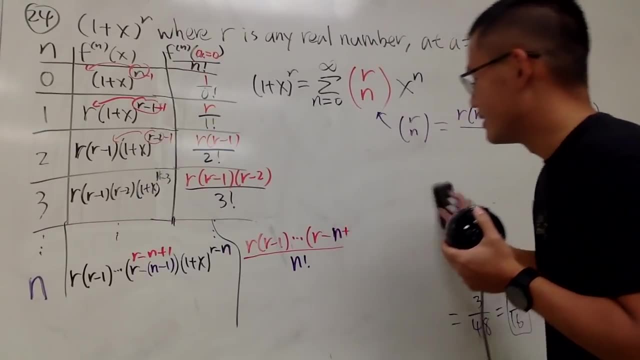 that you should expand it. What's the radius of convergence? I can tell you it's 1, but I don't know if I should prove it. I should, so I will do this real quick, So you can just write it down like this: okay. 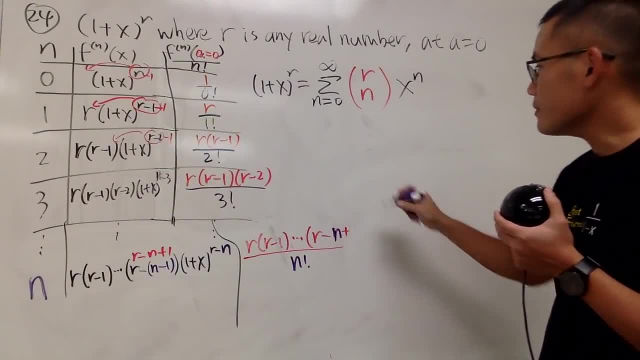 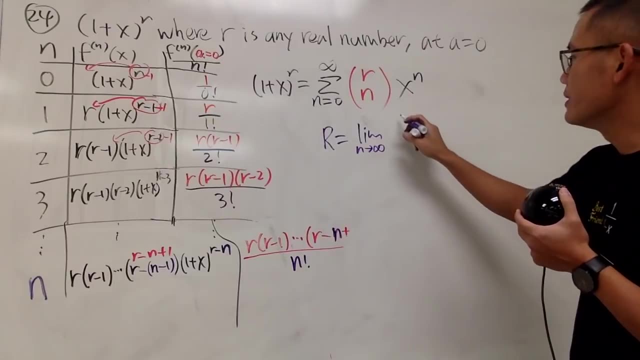 You can just write it down like this. I think it's totally legit. Well, what's the radius of convergence? You have to take the limit as n goes to infinity, And here we go. This is going to be the following: Take it up to value. 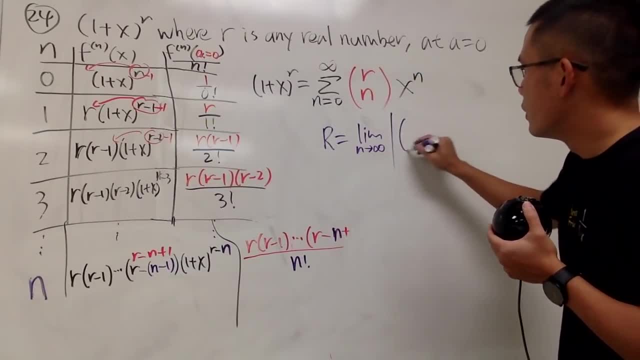 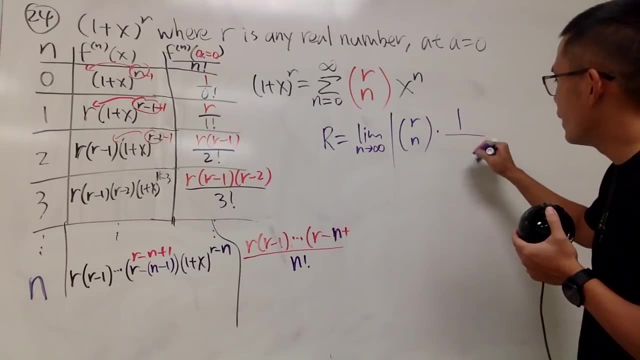 This is our cn, So we will just have okay, So we will just have r. choose n times the reciprocal of that. So you just have to put it as 1 over and we will have cn plus 1.. So the n becomes n plus 1.. 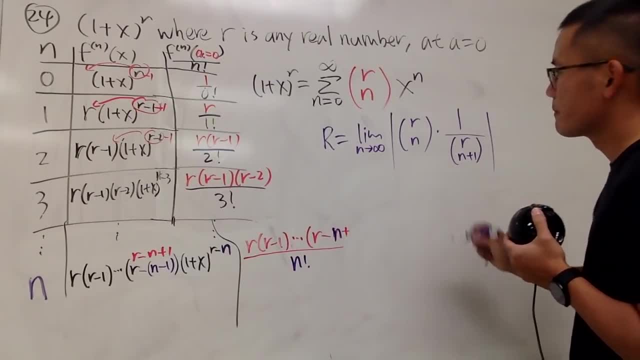 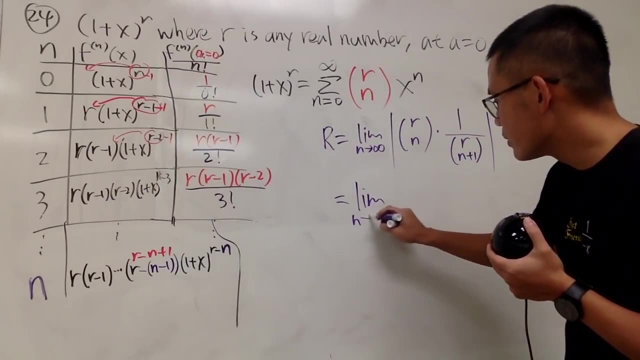 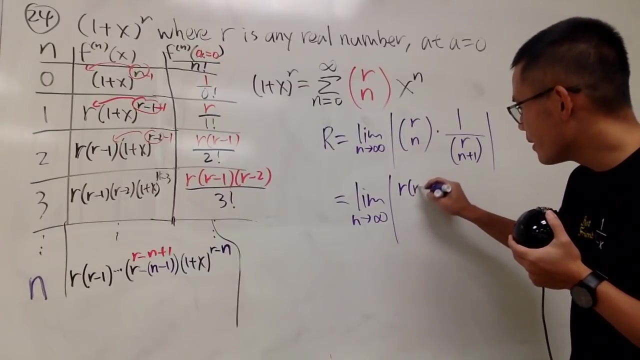 So we have rn plus 1, like this, right? So let's see if I have enough space to do all this or not. Here is the limit, as n goes to infinity. What's r choose n, Do we remember? Here is r times r minus 1. dot dot dot. times r minus n plus 1, okay. 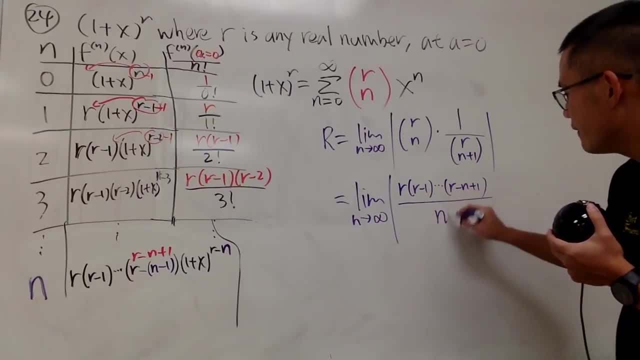 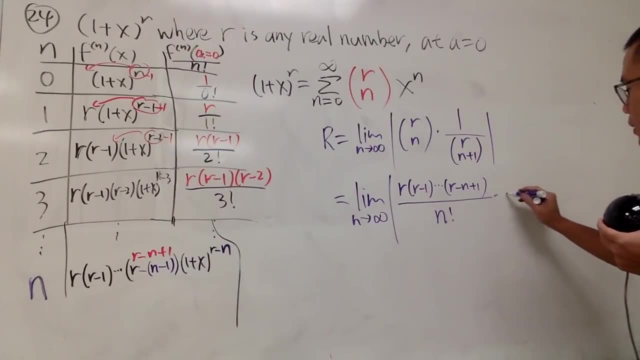 Like that, Divided by n factorial. okay, Now for the reciprocal version. you know you have to divide it by n factorial. So just put the sorry n plus 1 factorial. So just put the n plus 1 factorial on the top. 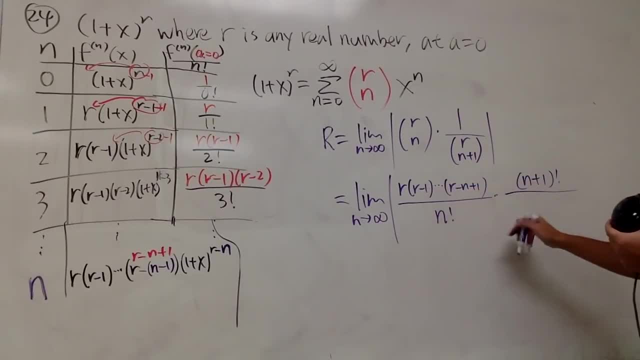 And then you do this pretty much. You have r times r minus 1 dot dot dot times r minus. what Well, this, right here again, is r minus n minus 1.. 1 less than whatever this is. Now we do 1 less than whatever this is. 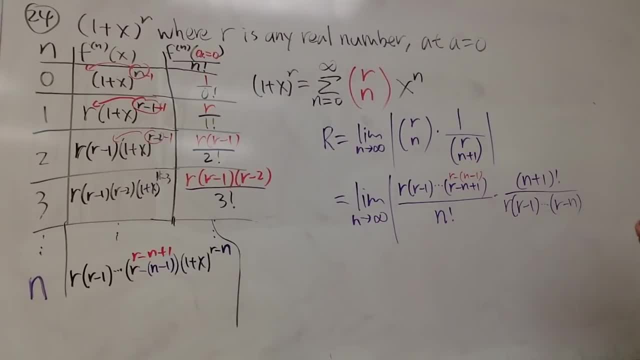 So it will be just r minus n, like that. Yeah, Okay, So let me see That is correct, of course. Okay, Now let's see what we can do for this. First of all, this right here is n plus 1 factorial. 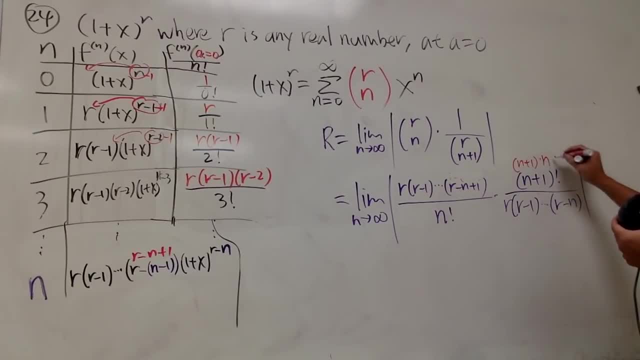 namely n plus 1 times n times n minus 1, and so on. So that's n factorial This and that can be canceled. That's very nice. Then let's see: This is r minus n. And again, this is r minus n minus 1 in the parentheses right. 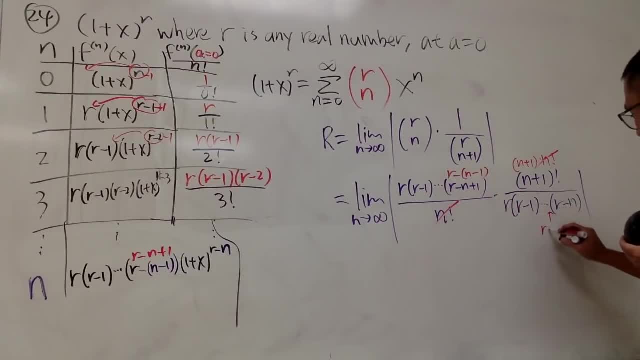 So the truth is there is a factor here: r minus n minus 1, namely a term before this right, Because this has more terms. So we do have this factor right here as well. We have a factor right in front. This is n's term. 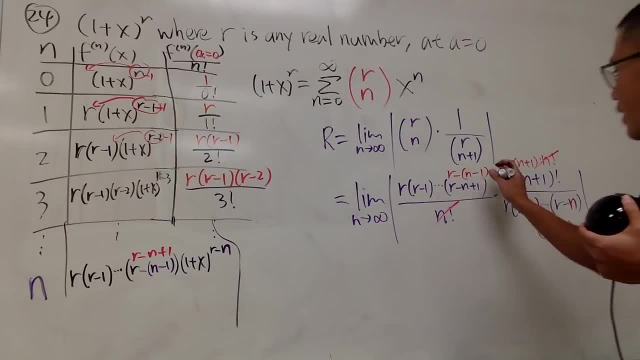 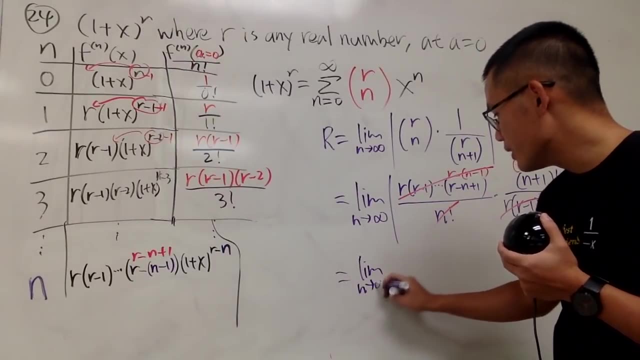 This is the n minus 1's term. The good thing is that all here will be canceled with everything here. So what do we have left? This is the limit, as n goes to infinity. On the top, it's just nicely equal to n plus 1, yeah. 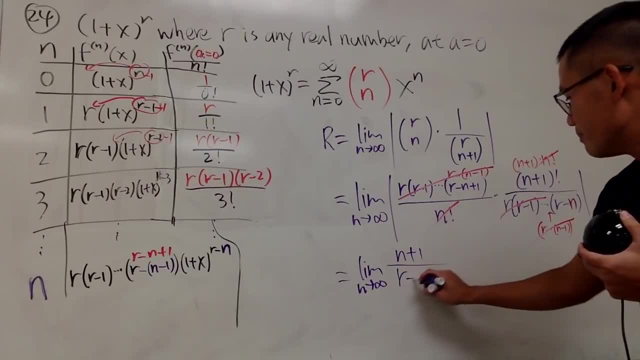 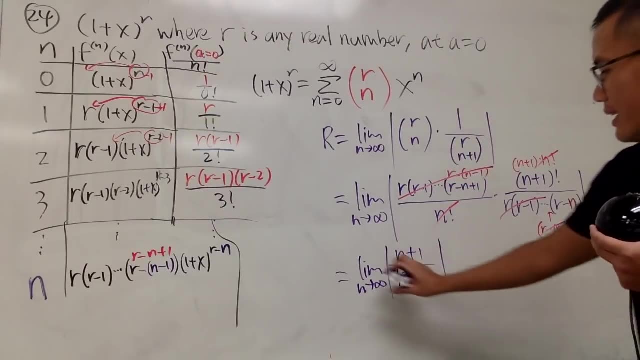 And on the bottom it's just this term, which is r minus n. Notice that we do have the absolute value because technically this is from the ratio test. Take the limit inside out. You get negative 1 in the absolute value, which is just positive 1.. 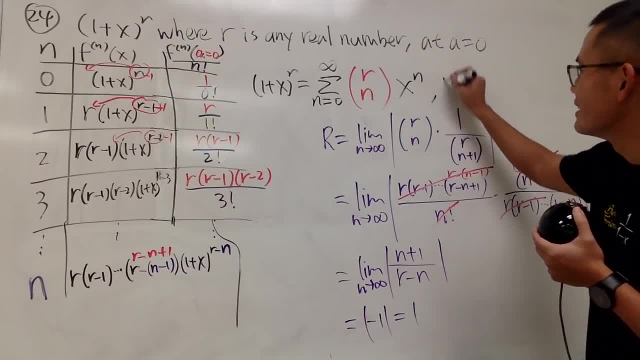 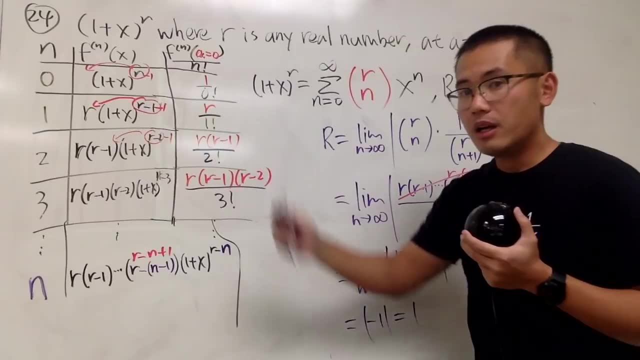 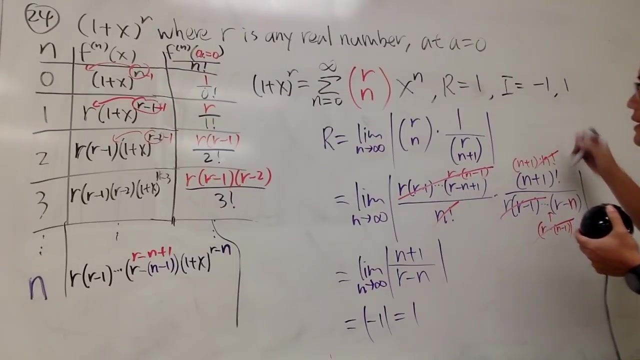 So let me tell you this: right here, r is equal to 1.. Very nice right, And usually for this, right here, to find out the convergence at the endpoint of the interval. right, Because we go from negative 1 to 1.. 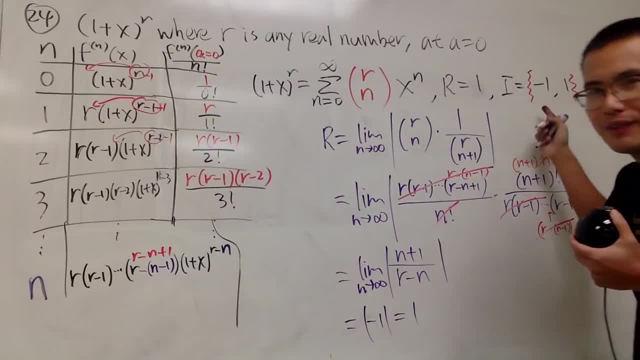 This right here. it depends, So I'll just do this right here. Have you guys seen this notation? Do you guys know what this notation is? You don't right, Because? yeah, I don't either, because I just make this up. 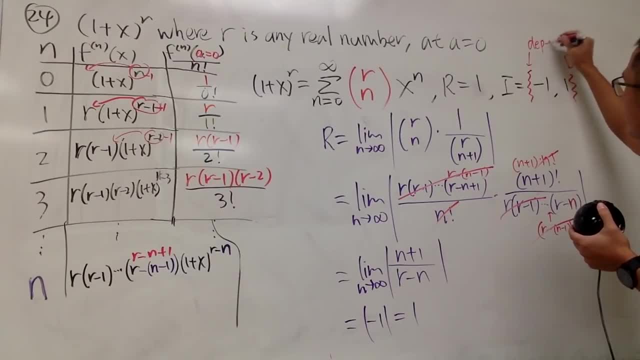 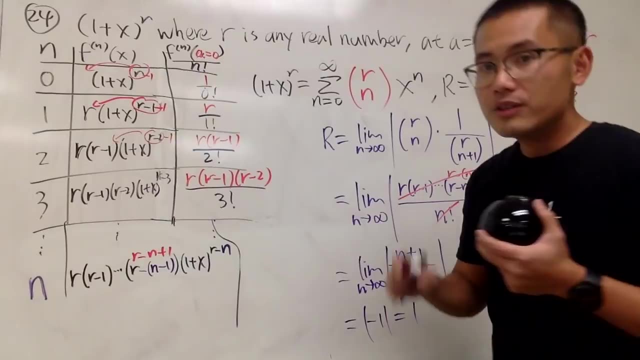 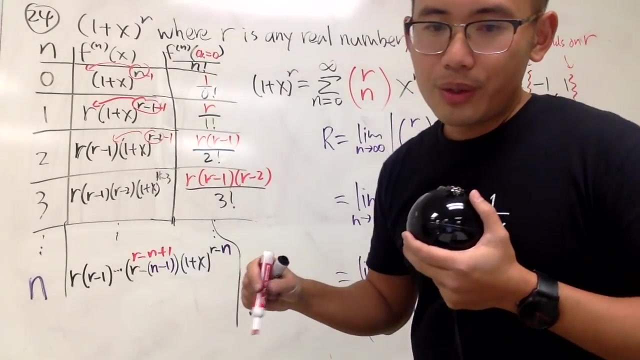 This right here. okay, This right here depends on r. It depends on r, Depends on r, So I will tell you. You, Let me just see You include the. This is right here, so you can just see it. 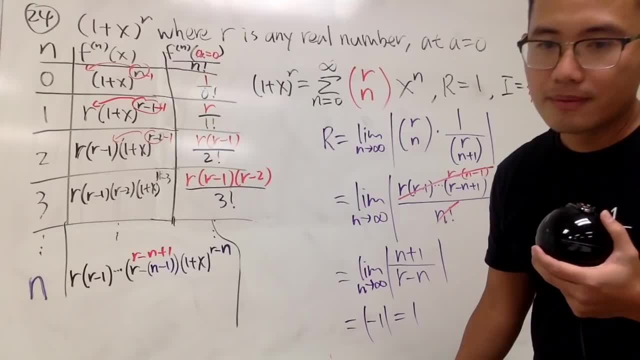 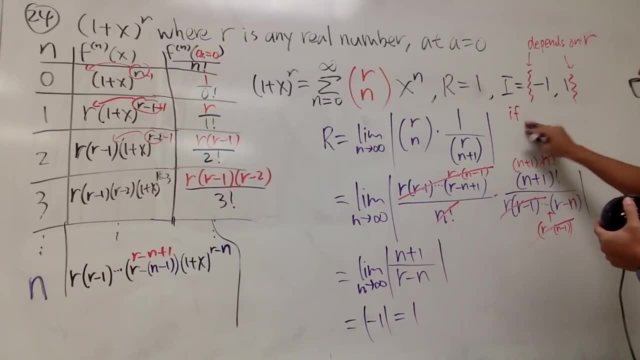 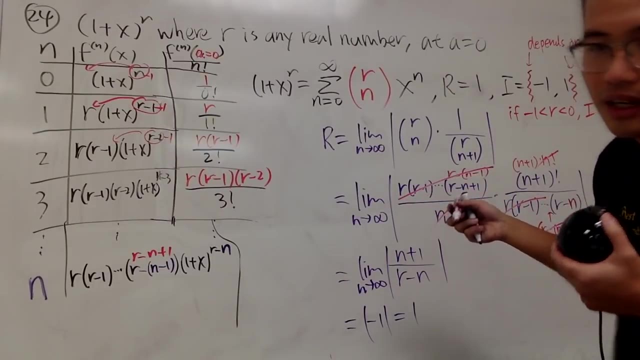 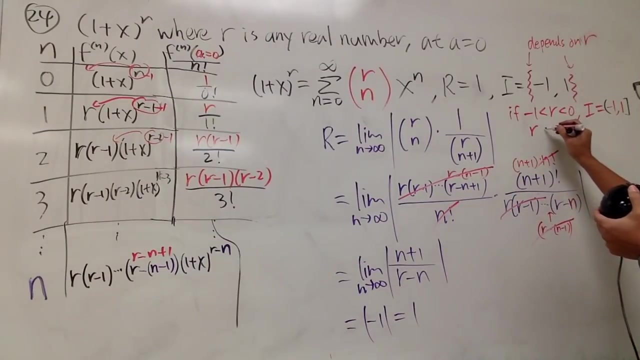 Yeah, Yeah. So I will tell you: if r is in between of negative 1 and 0, then the interval of convergence is negative 1 and 1, including this but not including that. Yeah, And then if the r is, 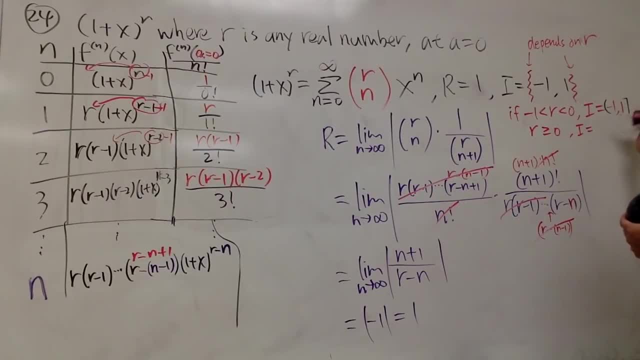 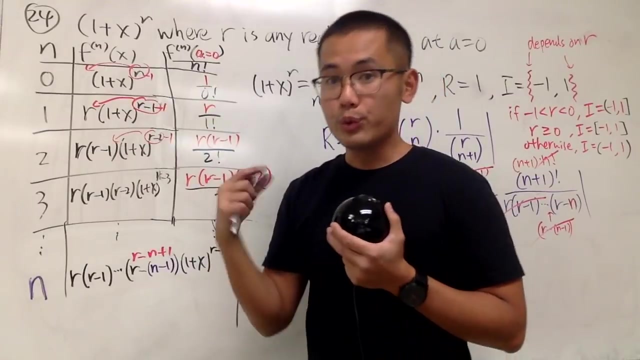 bigger than or equal to 0,, then the interval of convergence is both negative 1 and positive 1.. And otherwise I will just be negative 1, 1,, not including the endpoints. So for example, best friend right here is technically when r is equal to negative 1,. 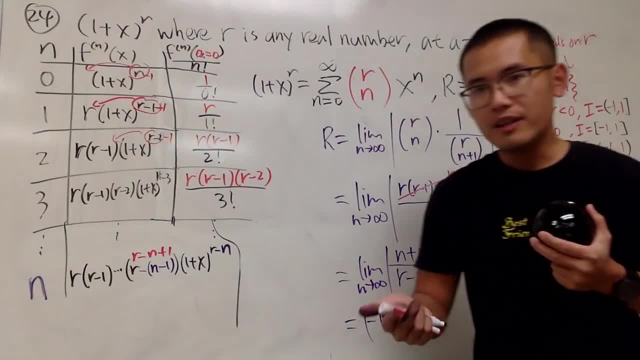 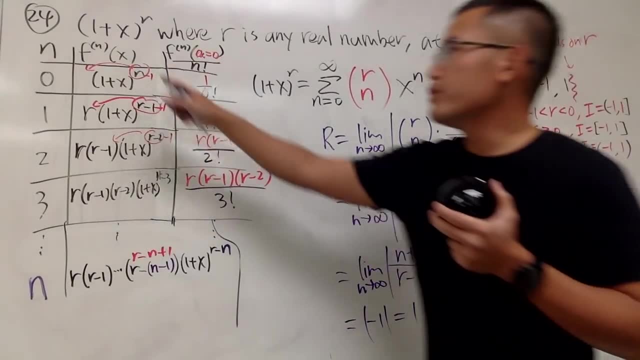 and that is actually right here. And if you have the best friend, if you differentiate, that again it will be right here as well. So that's the idea, And I do notice this is 1+, The best friend is 1-. 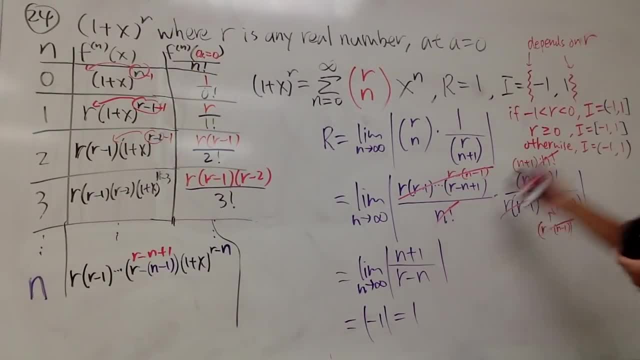 but it's a similar idea. You can just do the substitution. But, man, this is the binomial series man. Okay, so have a look. Oh yeah, of course, of course, of course, Box this, But I'm going to erase this right now. 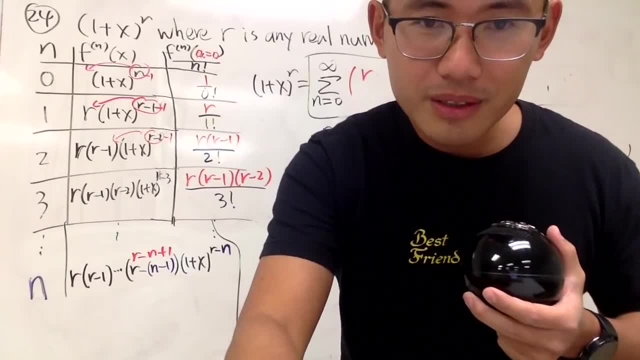 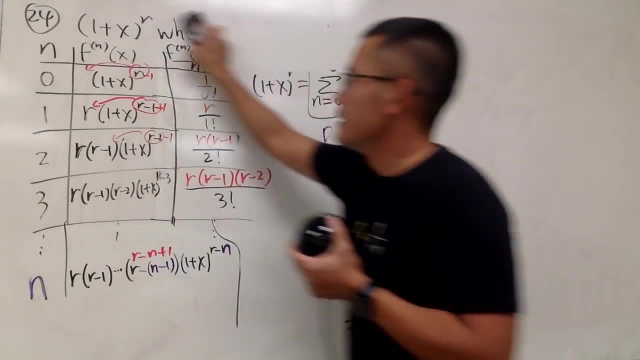 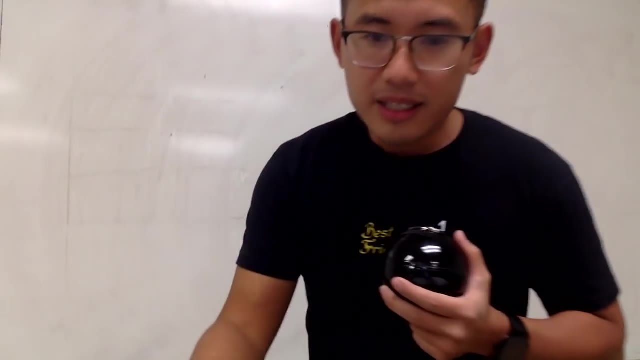 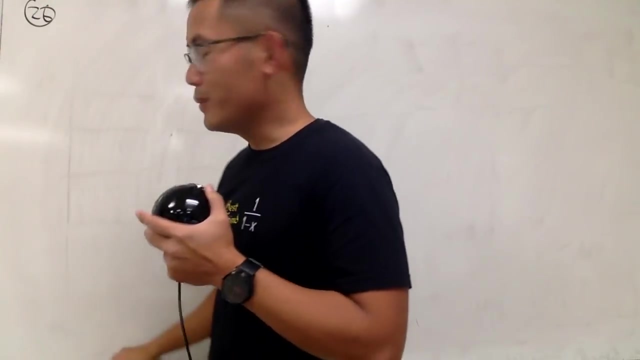 Man, this takes me. how many hours already. Let's see Three hours, Man, I can almost go to Vegas already. All right, So we have a couple more to go, All right, so just bear with me. Well, I'm doing this for you. 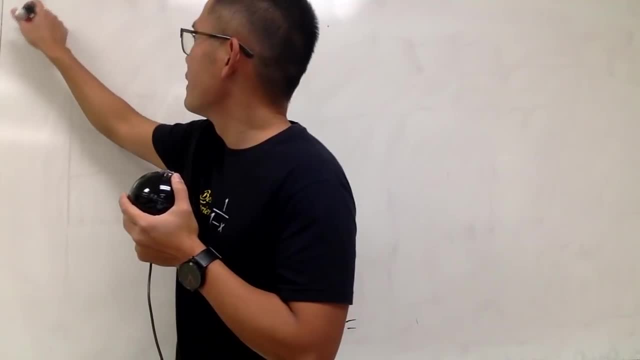 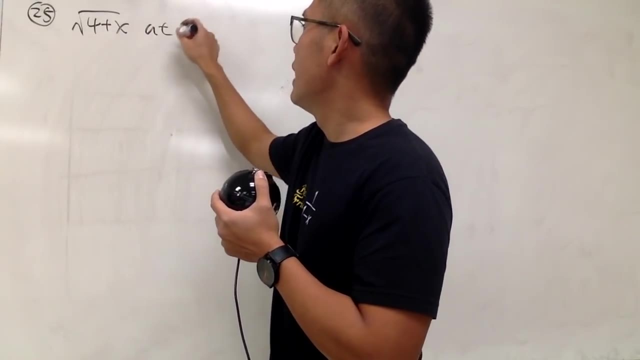 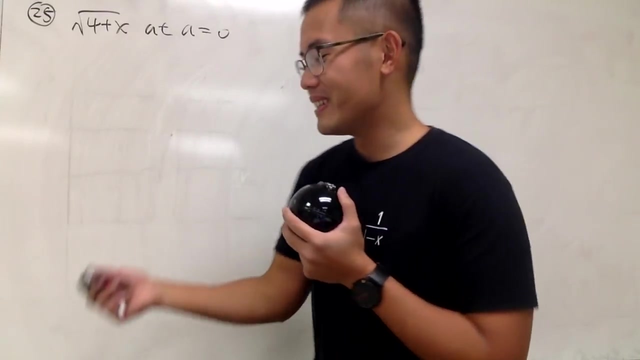 No, no, no, not 26, yet This is 25.. So here we go. Square root of 4 plus x at a is equal to 0.. Well, of course, we'll be using the formula we derived earlier. 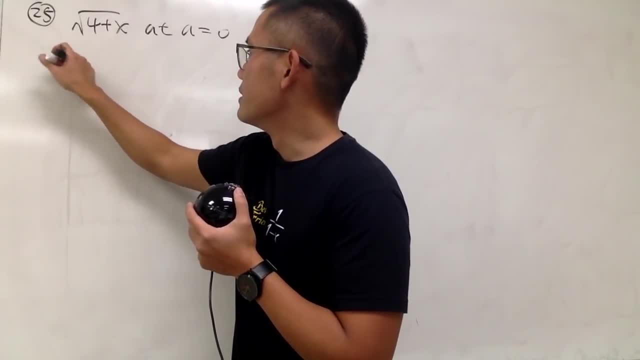 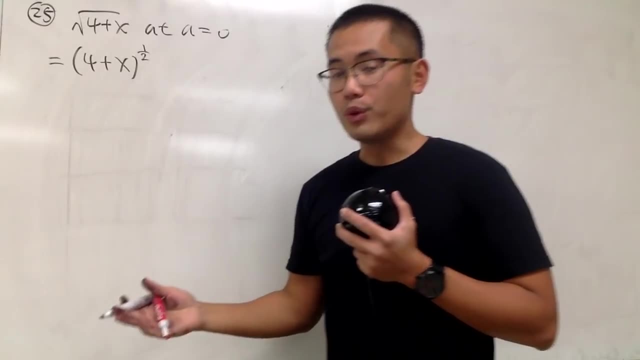 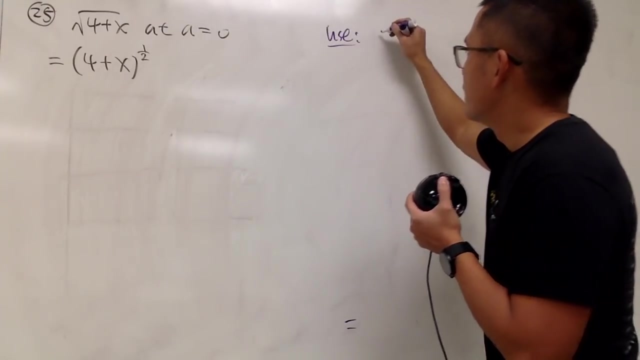 So you can see that this right here is the same as saying parentheses 4 plus x to the 1⁄2 power. But in order for us to use what we did earlier, and perhaps let me write it down to remind you guys, we will be using the binomial. 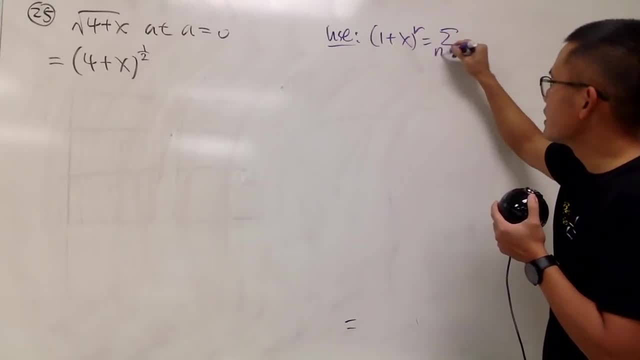 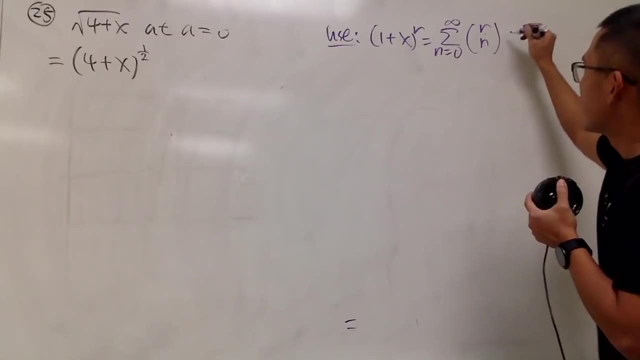 1 plus x to the rth power. That's the sum, as n goes from 0 to infinity, And I'm just going to write it as n, so r choose n times x to the nth power, like so, And then the radius of convergence is 1,. 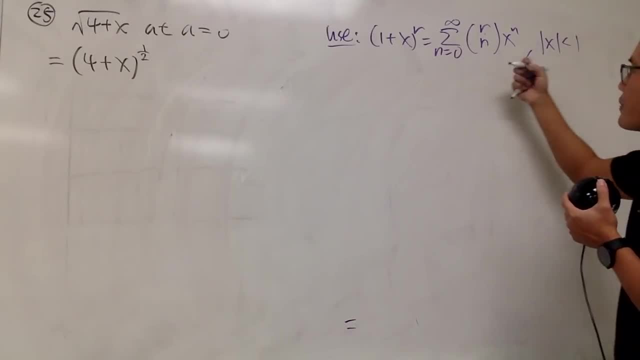 which is absolute value of x, is less than 1.. It's another way to say that, of course, And of course. here is the x in red, Here is the x in red, Here is the x in red, All right, 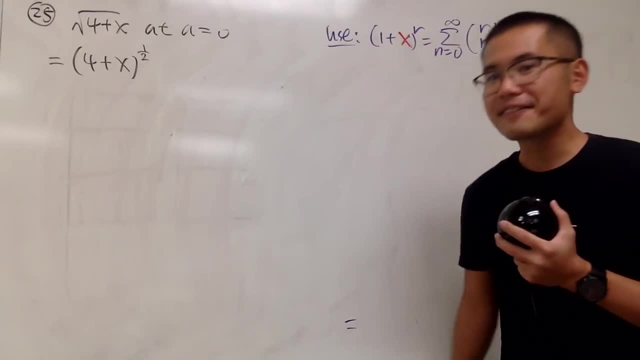 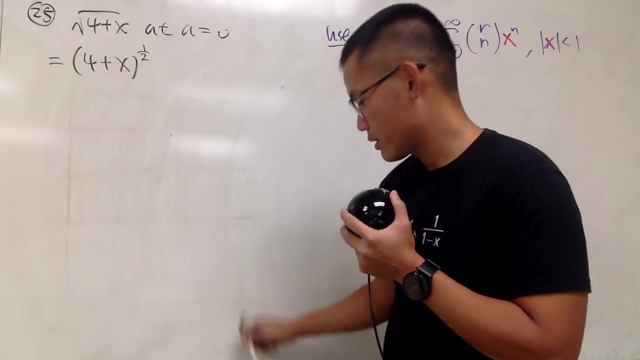 Now r is 1⁄2.. But we need the 1.. So you know the deal, We can factor things out. So here we go, Right here, Factor out the 4.. So we have the 4 right here. 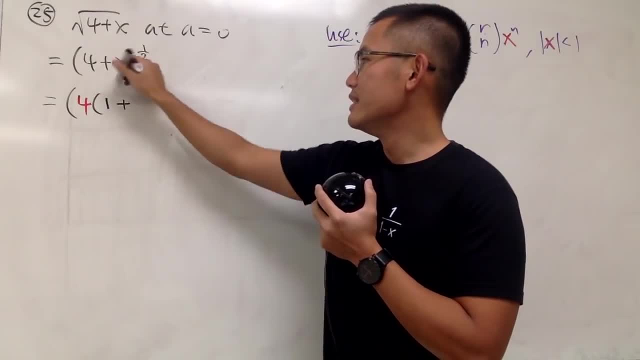 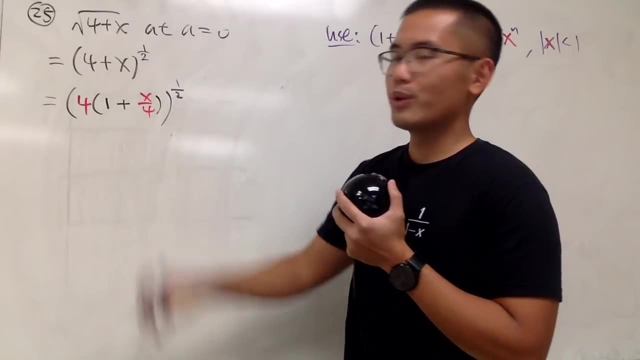 And this is going to be 1 plus. this is going to be what? x over 4, like this, And then we have the 1⁄2, which is the square root, of course, And of course, this right here: 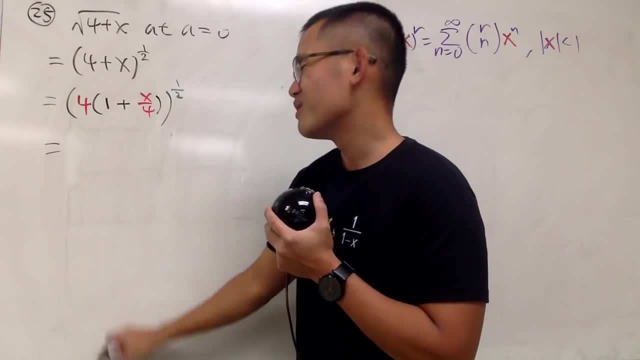 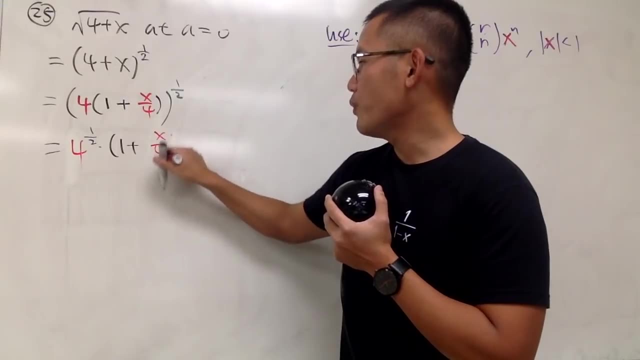 is the same as saying 4 to the 1⁄2 power. Let me just write this: 4 to the 1⁄2 power times 1 plus x over 4 to the 1⁄2 power, like that: 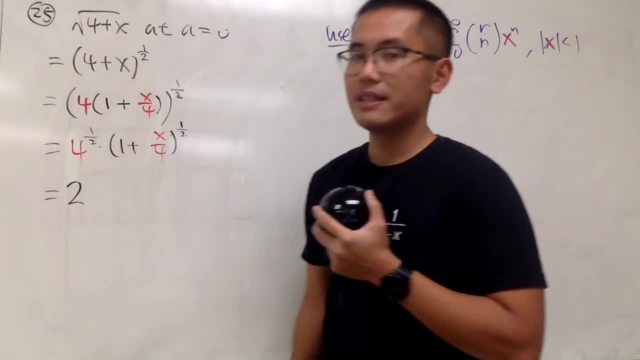 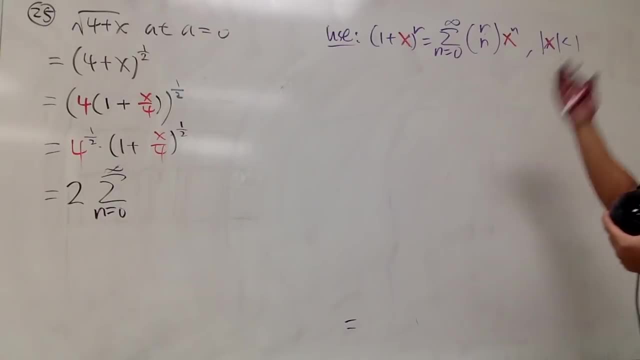 This right here is the same as 2.. Very nice, This right here is going to be the sum, as n goes from 0 to infinity And we'll just be using that right here. So we will have: r is 1⁄2. 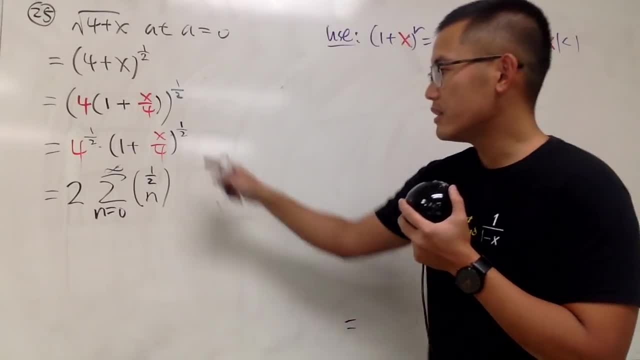 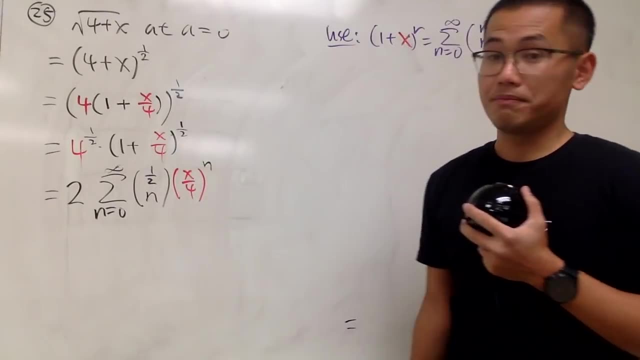 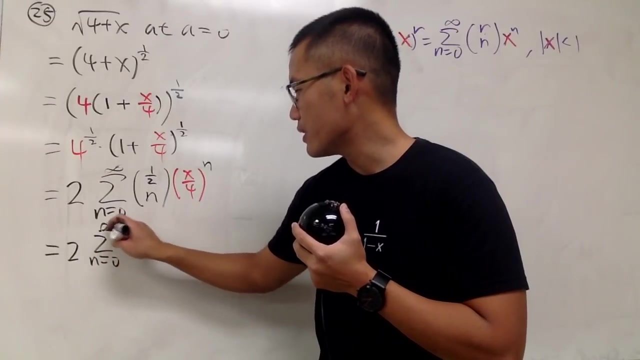 and n, n. We'll just enter this into the x, which is x over 4, raised to the nth power, like this. Pretty good, isn't it? Okay? so here we have 2.. Sum of the series, as n goes from 0 to infinity. 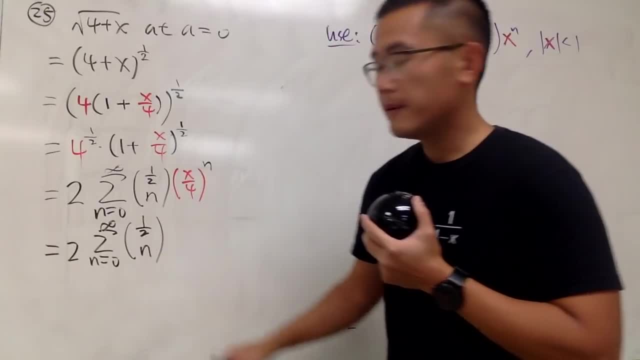 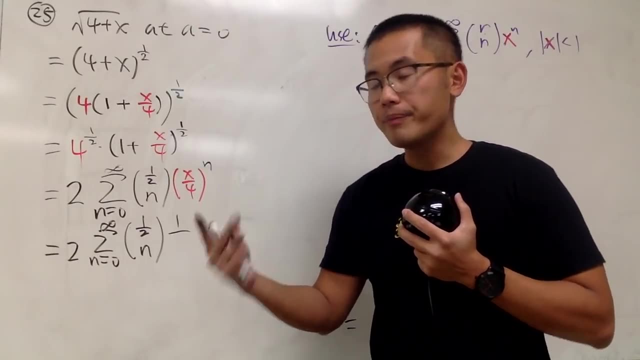 Just write it down like that: 1⁄2, n And let me write this down as 1 over 4.. It's the same as 2 to the 2nd power And then the nth power. I will write it as 2 to the 2 nth power. 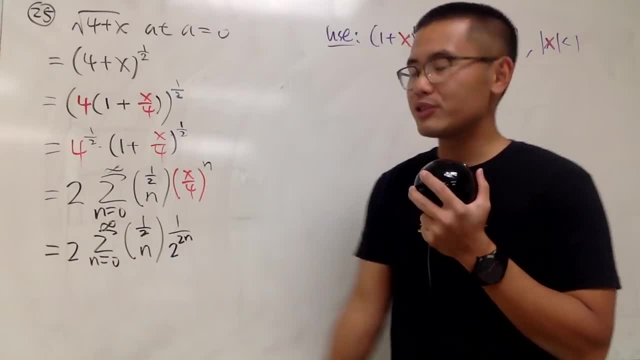 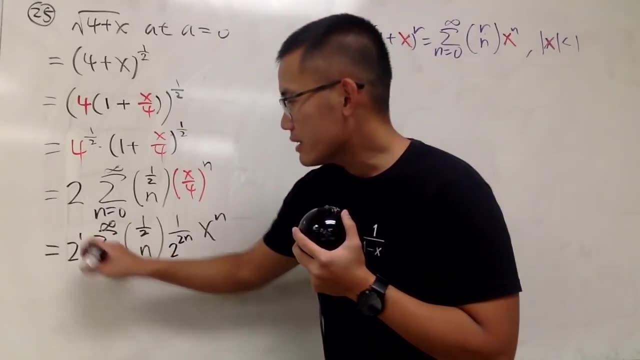 Because I have the 2 right here. I want to do this so we can match the powers, the base And this right here is x to the nth power, like this: Now, this is on the top, this 2 to the 1st power. 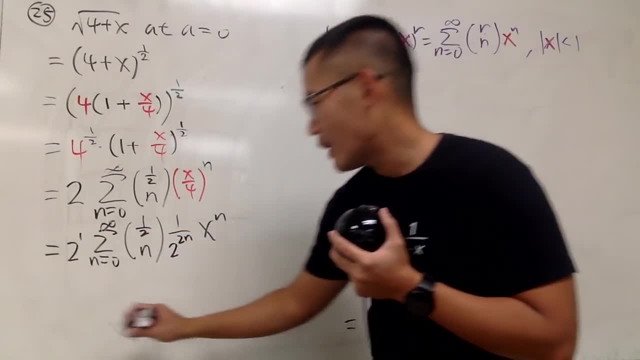 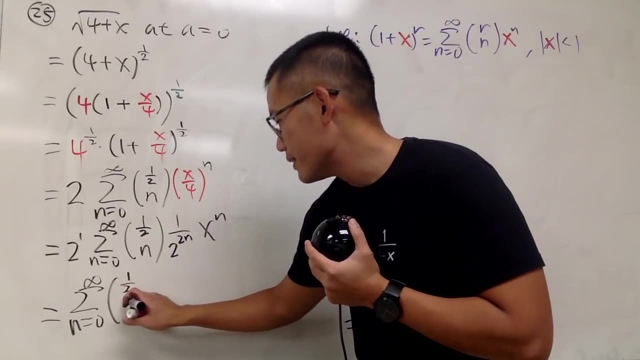 Technically I should do 1 minus that right, But I can do this. This is the sum, as n goes from 0 to infinity. 1⁄2, choose n. And how do I write it? I say: write 1⁄2, choose n. 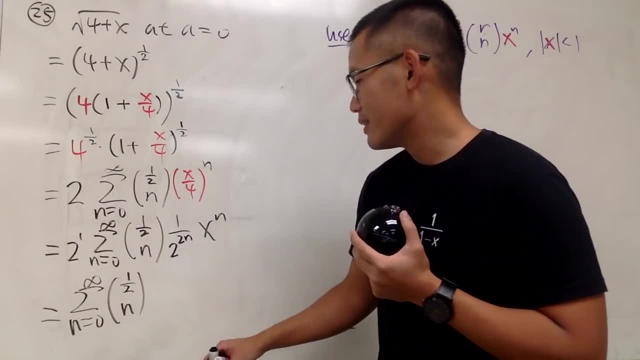 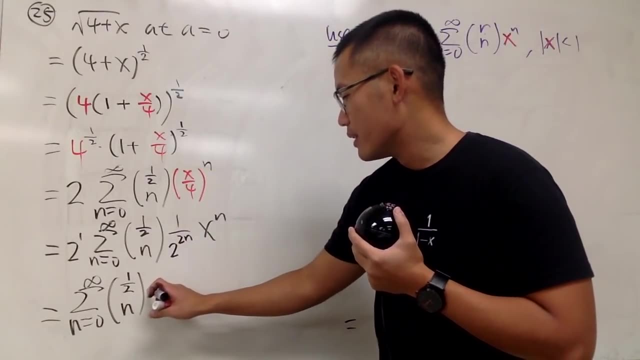 Oh yeah, put that down. Well, it doesn't really matter. Hmm, Yeah, let me just put down this first. My answer key had this part first. But anyway, Times 1 over. well, I can just do the bottom minus the top. 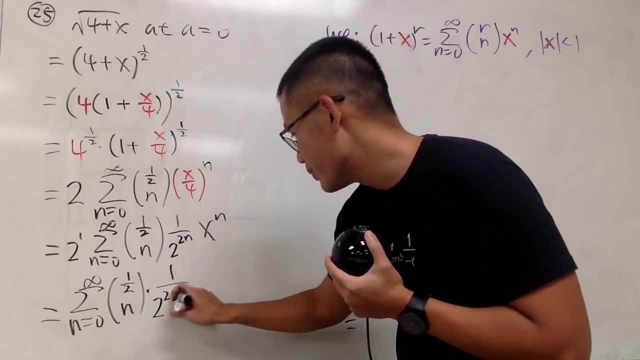 and then stay on the bottom. That's what you can do as well. So it's 2 to the 2 minus 1.. So if I stay on the bottom, this is what you do, And then in the end, you have x to the nth power. 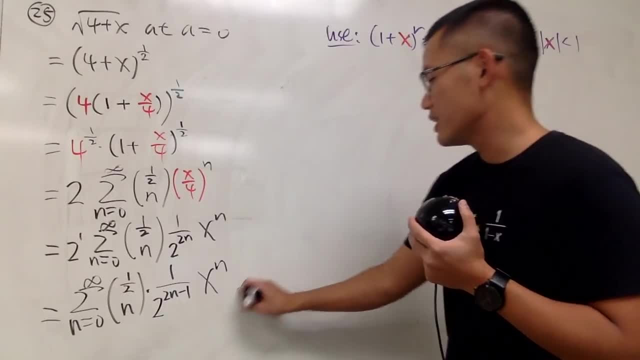 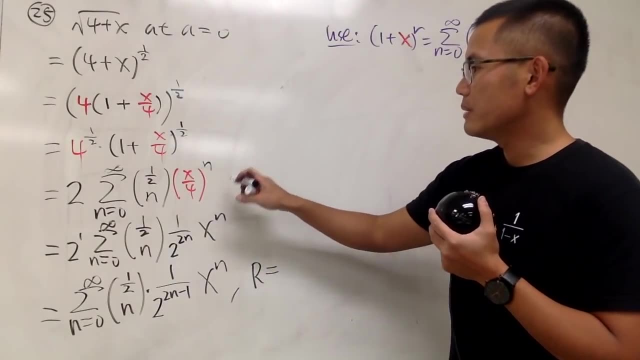 like that. Very, very, very nice. Now r is equal to. well, let's do that. I haven't done that yet, So pull the abstract right here. Absolute value of x minus 4. This has to be less than 1.. 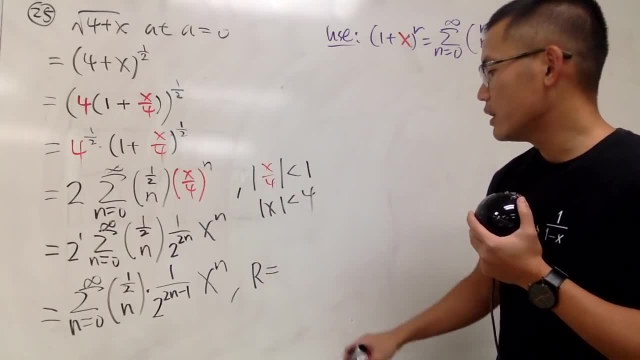 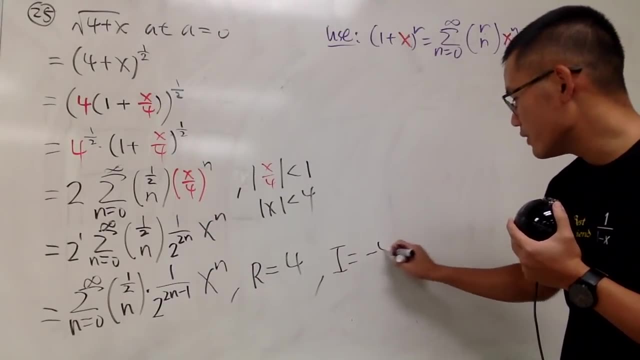 Multiply 4 on both sides, Absolute value of x is less than 4.. r is 4.. Radius of convergence, I mean the center, is a 0. So i is equal to negative 4 to 4.. Well, what did we say about intervals earlier? 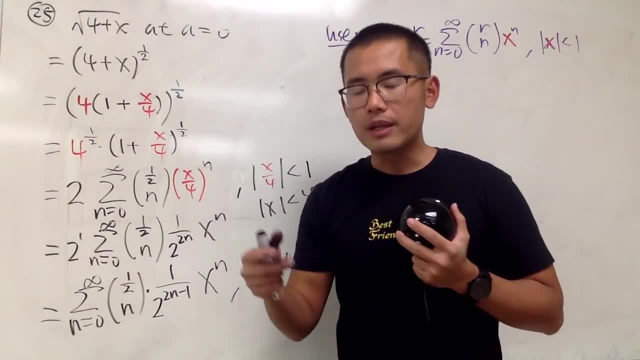 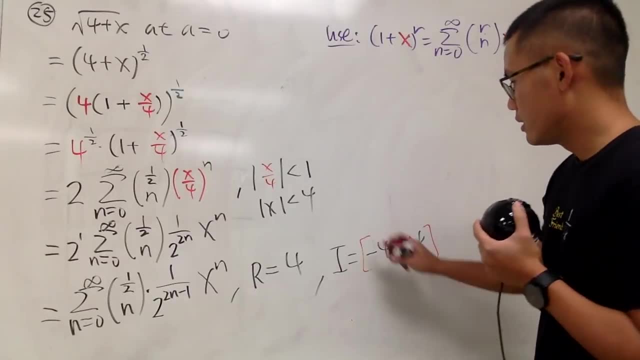 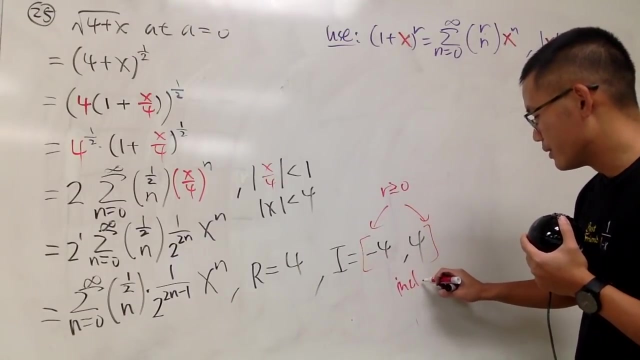 When r is positive, like 0,, as long as it's greater than or equal to 0, you include both endpoints. Right, This is, when r is greater than or equal to 0, include both. include both endpoints. And again, if r is, 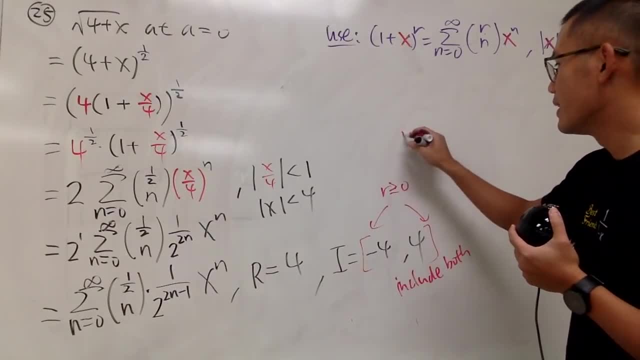 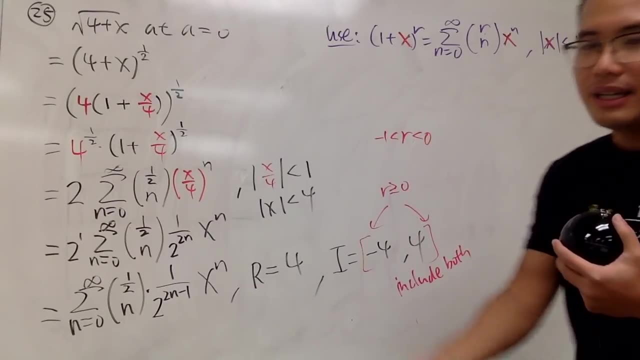 I forgot what I wrote. But like, if r is in between of negative 1 and 0, then just include one endpoint. Yeah, I'll type it out for you guys already. Just go to read. just go look at that. 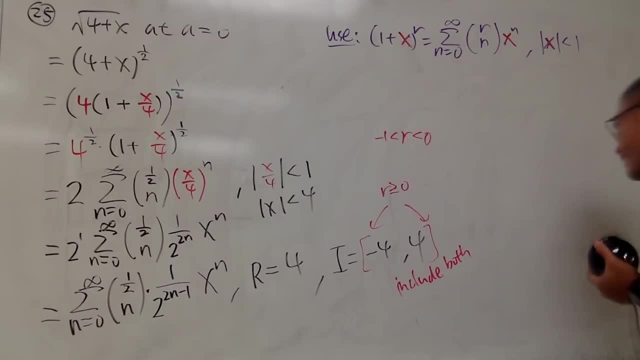 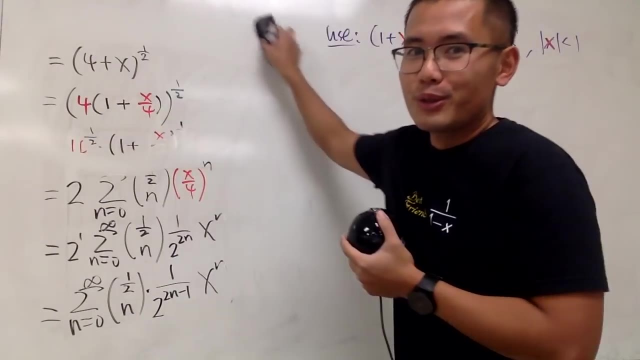 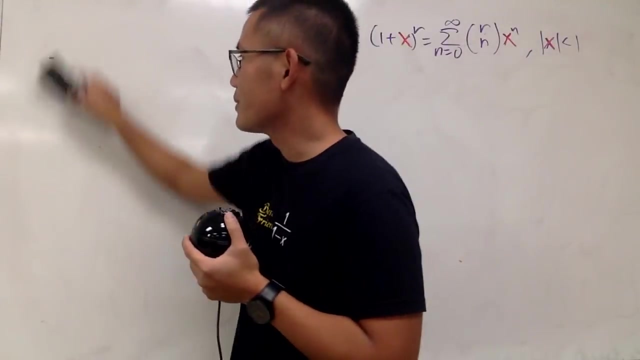 okay, So just yeah. Okay, So that's number 25.. Two more to go. I'm going to still use that. so yeah, This one is going to take me another, like 10 minutes or so. 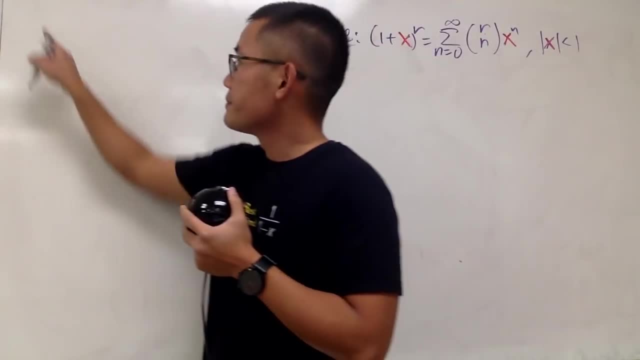 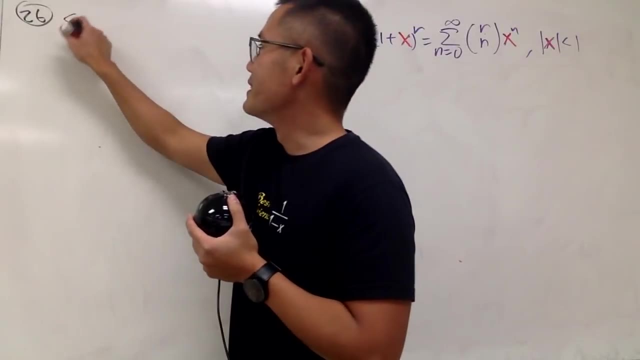 I don't know. I can do the easy way, I can do the hard way, I don't know. So number 26.. You know this is going to be the hardest one. Inverse sin x at x equal to, at a equal to 0.. 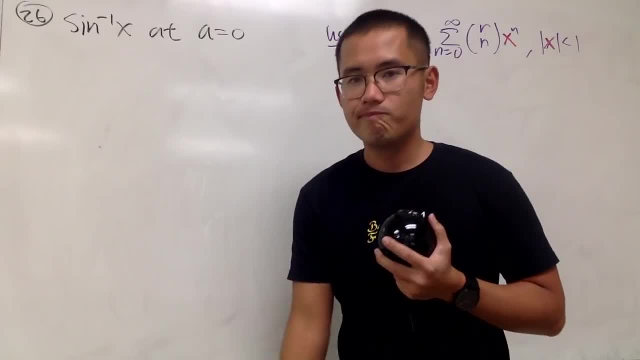 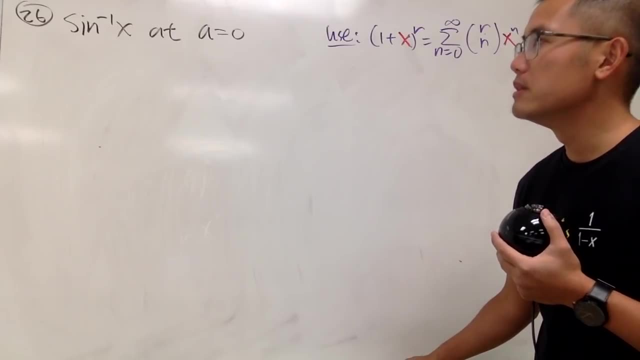 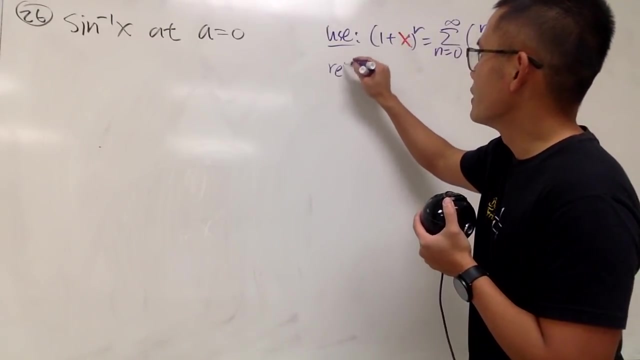 a is the center. so, yeah, Man, Hmm, Well, how can we get a inverse sin? Yes, we can use what Integration, So reminder. so this is just a little reminder, right? So if you integrate, 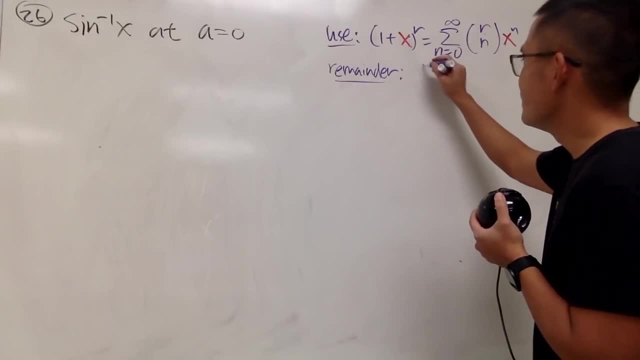 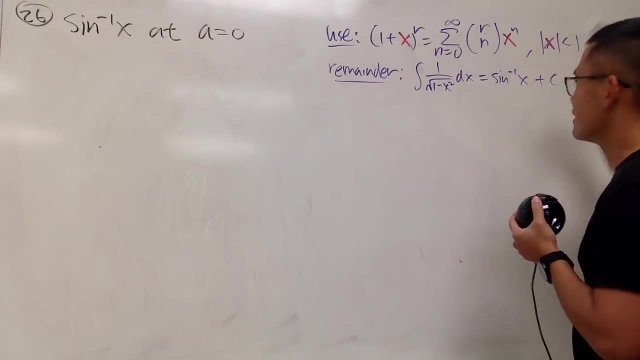 1 over square root of 1 minus x. squared this right here gives you inverse sin. yeah, So the strategy is: come up with a power series for this first and then integrate that. So here we go. So. 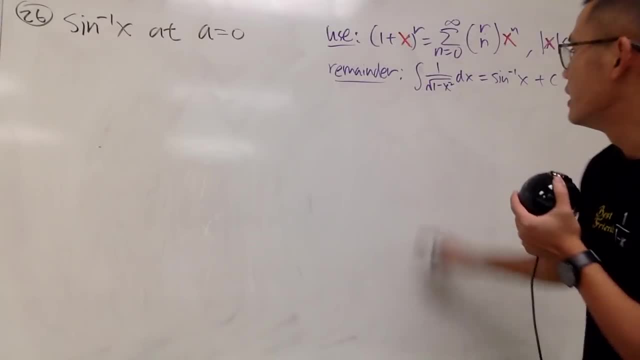 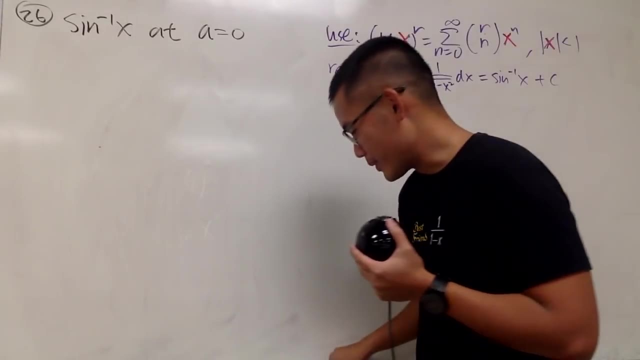 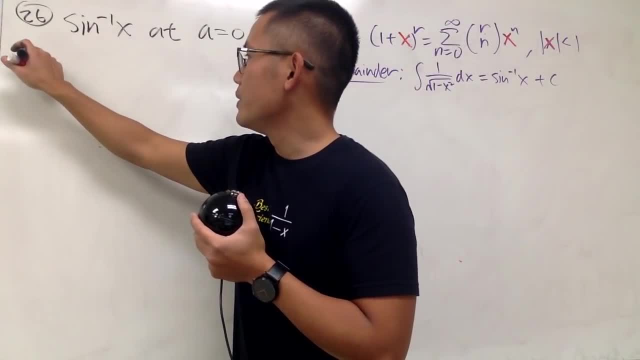 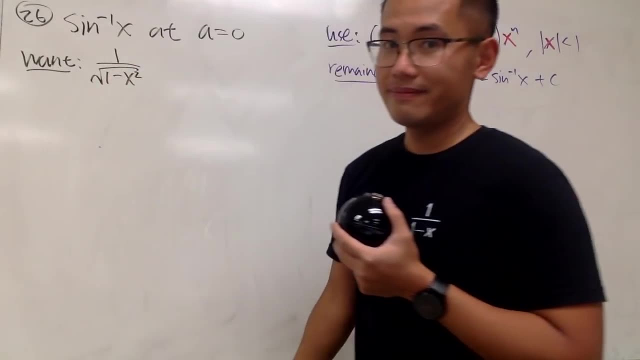 we need to find out. we need to find out, okay. So we, we want, okay, we want 1 over square root of 1 minus x, squared first. So that's what we want first, And here we go. 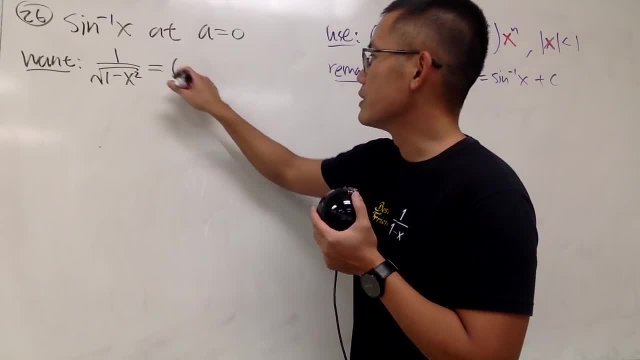 Square root on the bottom. we can bring that up and that's a negative 1 half power. So this is actually the same as 1.. I need to see a plus. I have to see a plus, It's okay. 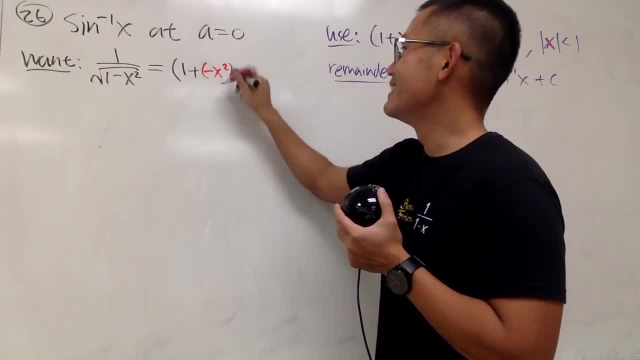 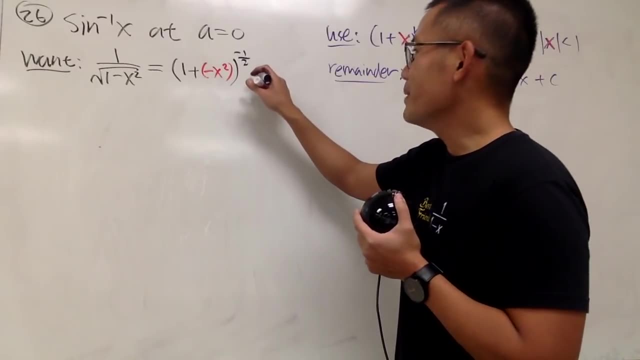 Just put a plus and that's a negative x squared, And then raise to the negative 1 half power, like this. Very, very easy, isn't it? It can be hard, it can be easy, depends on how you look at it. 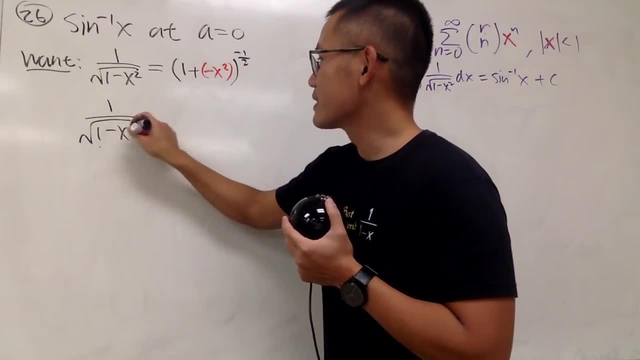 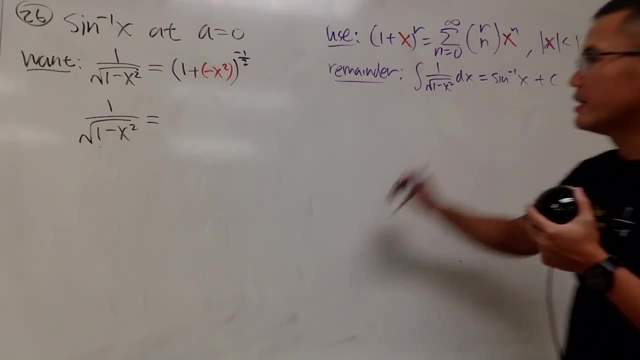 So we have 1 over square root of 1 minus x squared. This is going to be throwing negative x squared into here and there. So we have the series. N goes from 0 to infinity R in our case. 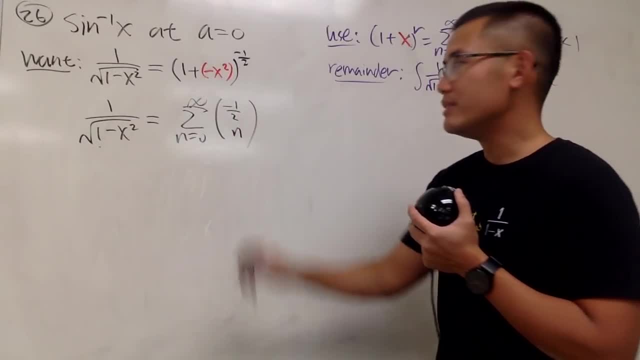 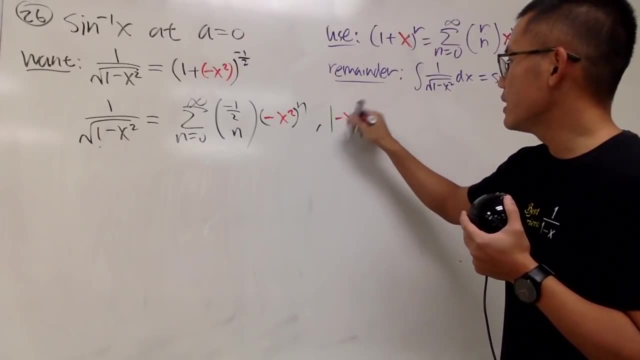 is negative 1 half, So negative 1 half. choose N And then just enter that Negative x squared raised to the nth power like this: Include the absolute value of negative x squared less than 1.. Then 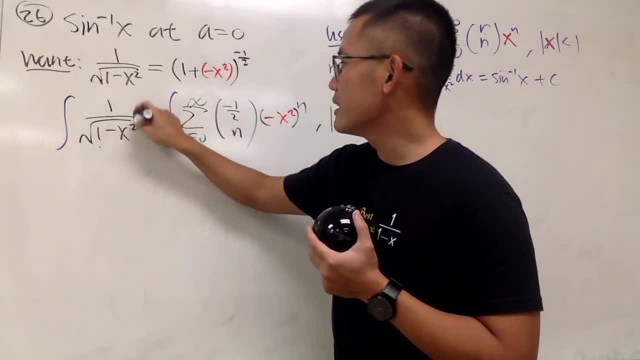 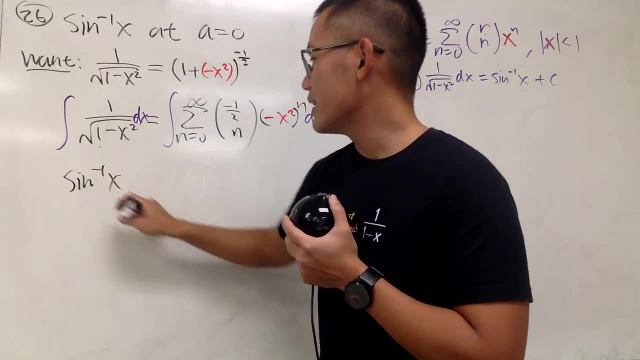 we integrate both sides, So integrate this, integrate that little dx, little dx. The left hand side, give us exactly what we want. That's the inverse. sin x is equal to c plus. Don't forget the c plus. 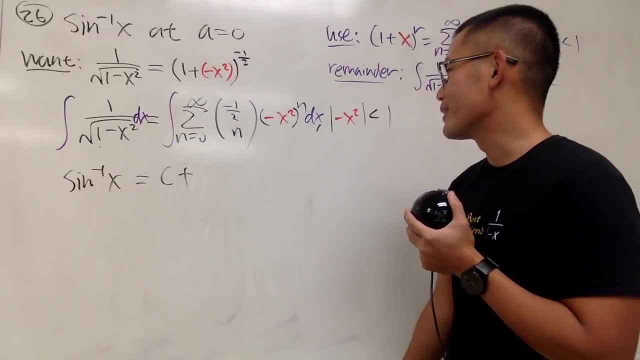 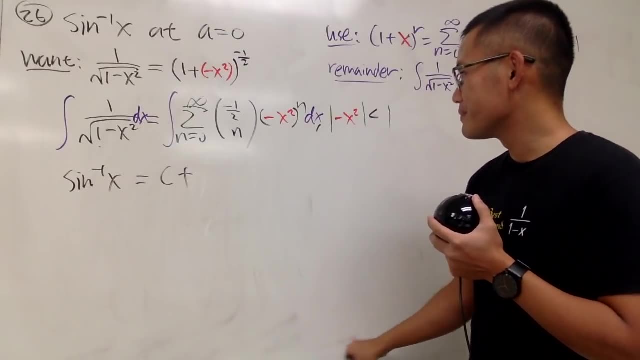 Here. integrate this. Oh man, I forgot to simplify this a little bit. Okay, Let me just do this right here real quick. okay, This right here is negative. 1 to the nth power, yeah, And then x to the 2nth power. 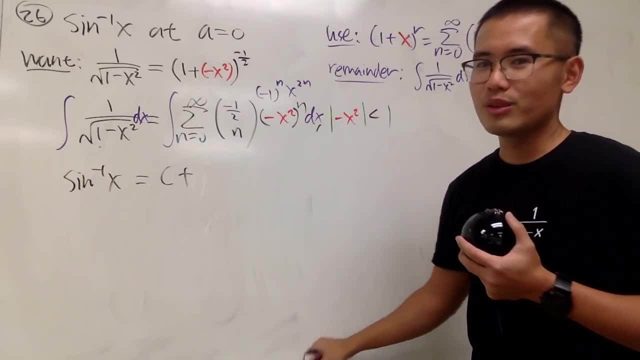 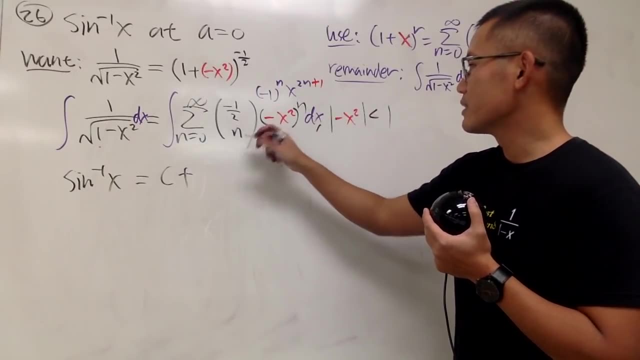 So, of course, simplify this. We have been simplifying this for like 26, 25 times already. Yeah, All right. So look at the new power, which is 2n plus 1, and divide it by that. 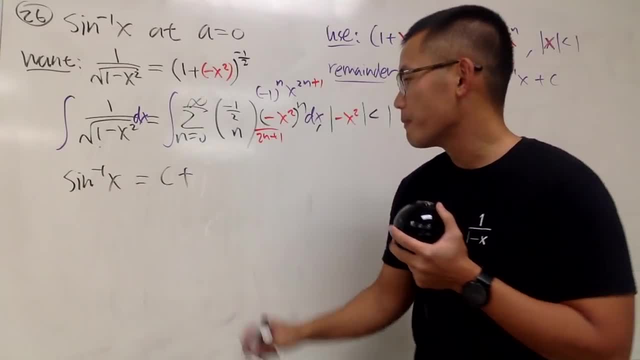 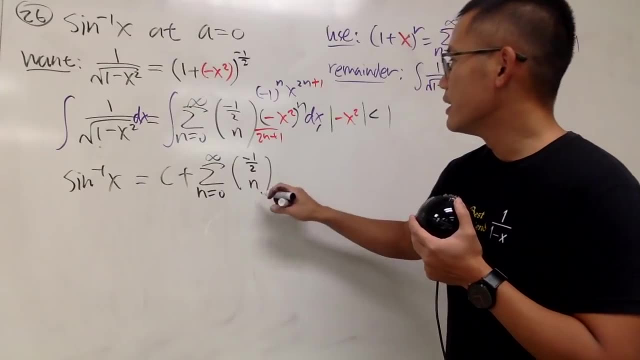 So that's pretty much it. Divide it by 2n plus 1.. So we get: the sum N goes from 0 to infinity. Let me write down negative 1 over 2, choose n times this. right here is what we need. 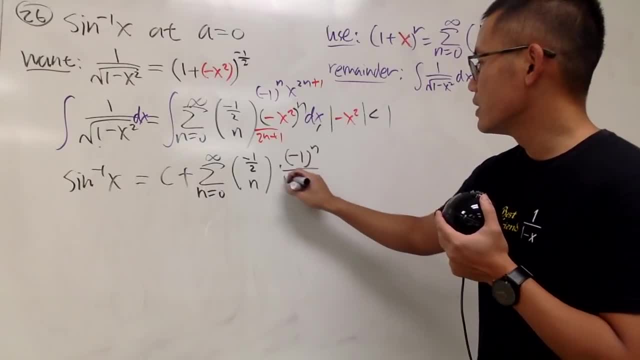 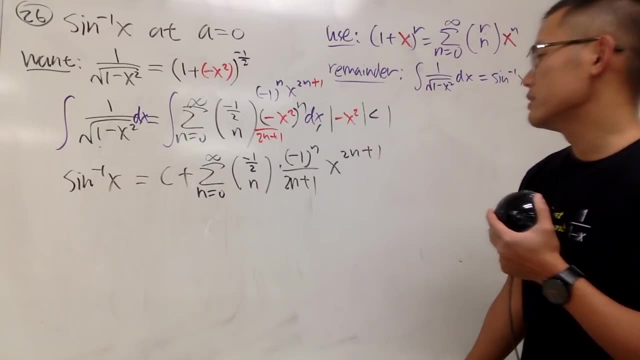 for the negative 1 to the n over this 2n plus 1.. And that's the new power: x to the 2n plus 1, power like this, And that's very good. Yeah, And to find out what c is. 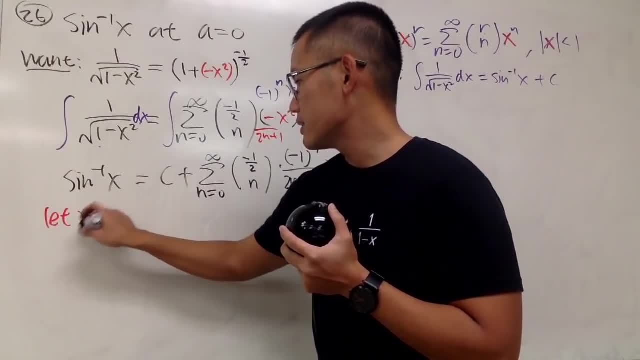 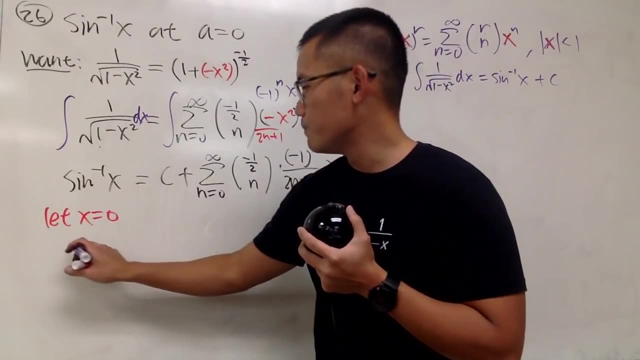 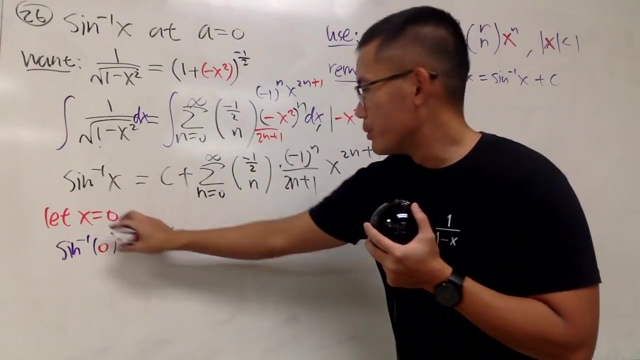 let's: x equals 0. When x is equal to 0, well, we get what We get, um inverse sine of 0. That's equal to c plus when we're putting 0 into here, everybody will be 0.. 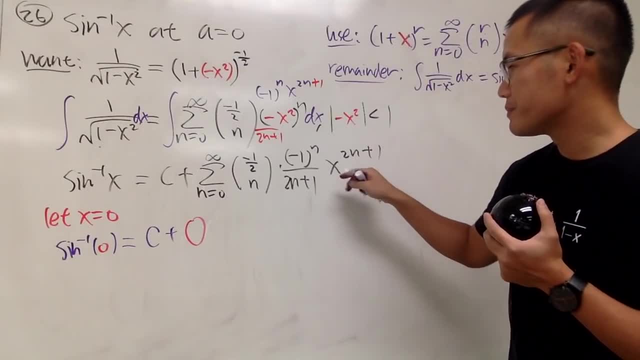 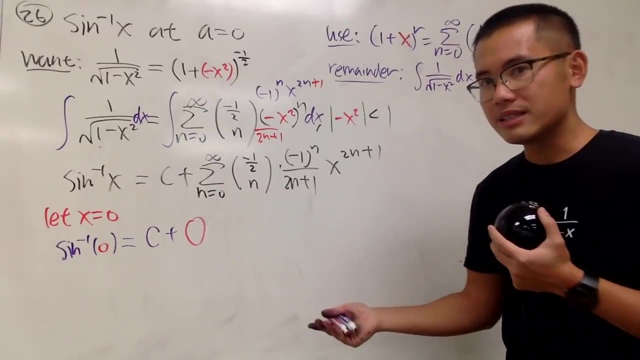 Okay, Because this is 0 to the first power. when n is 0,, right, When n is 0, you get 1, so it's 0 to the first power, and then everybody else has the x and everybody will be 0. 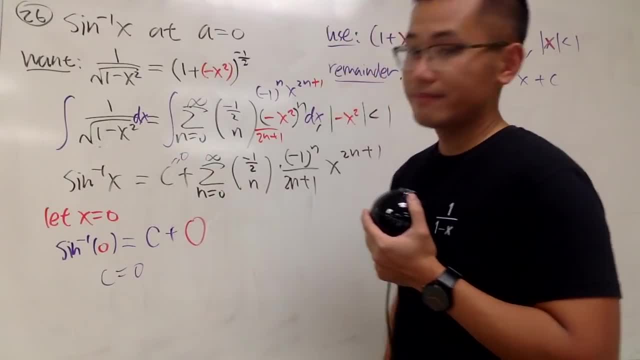 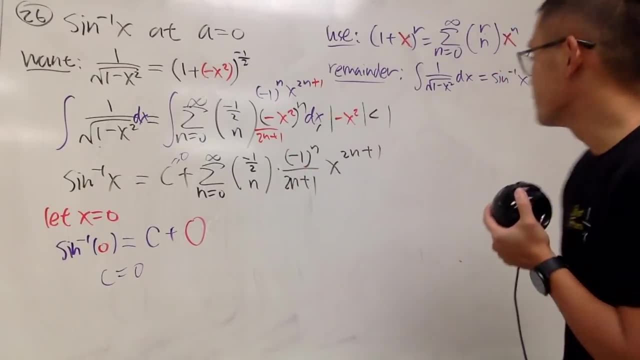 So, in other words, c is equal to 0.. So it's like that. Okay, so that's pretty much it. And yeah, this is the little multiplication, And you may be thinking this isn't so bad. 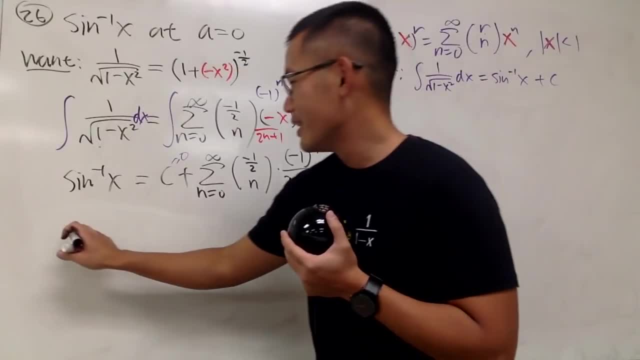 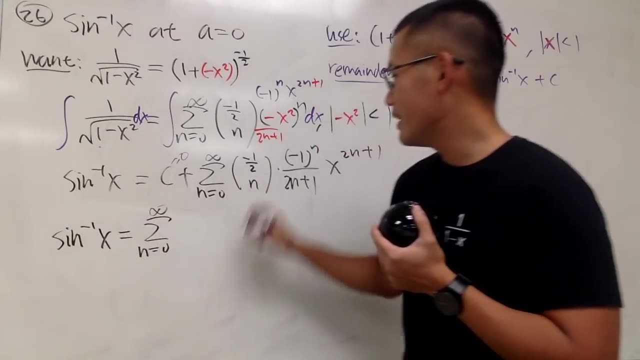 right, Why, And I say I mean, this is the long question. Let me just write this down nicely for you guys. The sum n goes from 0 to infinity. This is negative 1 over 2n, and this is negative 1,. 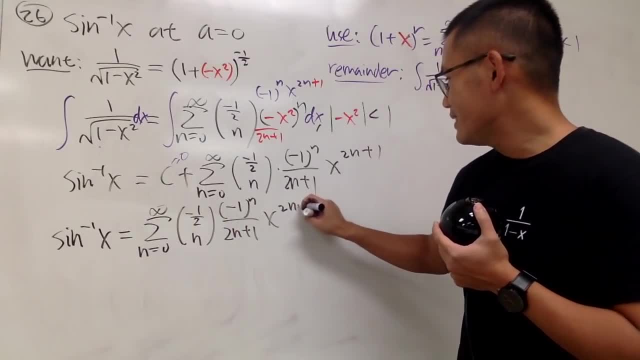 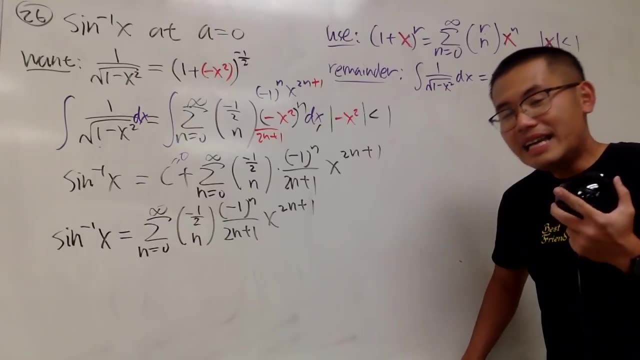 and it's power over 2n plus 1.. It's just a lot to write. It's not so hard, seriously, okay, Okay, why did I say this is like the hardest one? It's because some people may not take this as the correct answer. 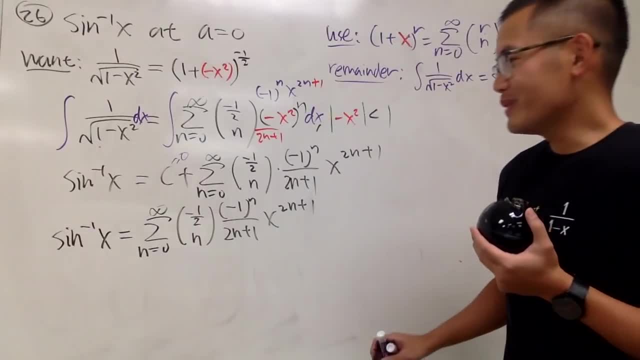 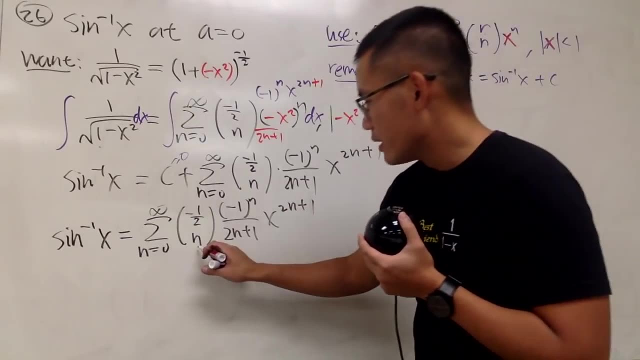 I don't know why They just want to break it down. I can break it down for you guys as well, So let's go ahead and do the breakdown Here. let's observe how this notation is going to look like. Check this out. 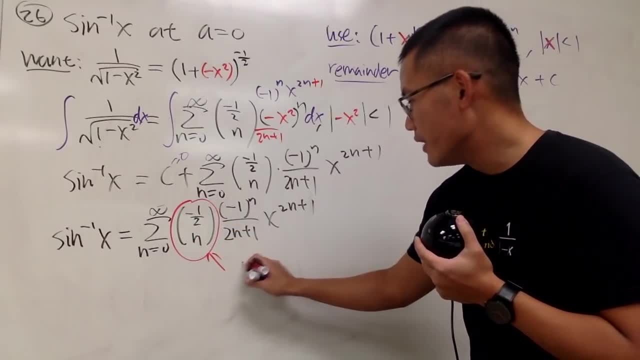 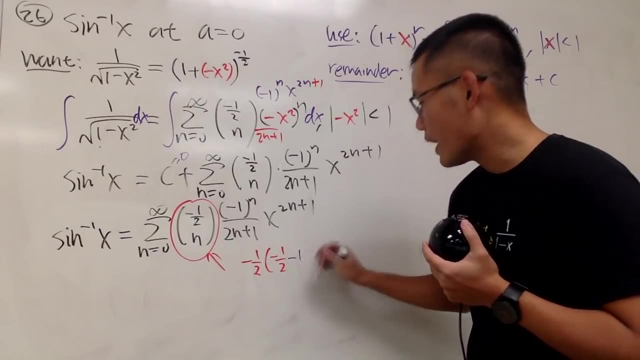 Negative 1 half. choose n. it's going to be negative 1 over 2.. That's your first thing, okay? And then times negative 1 over 2 minus 1, and then negative 1 over 2 minus 2,. 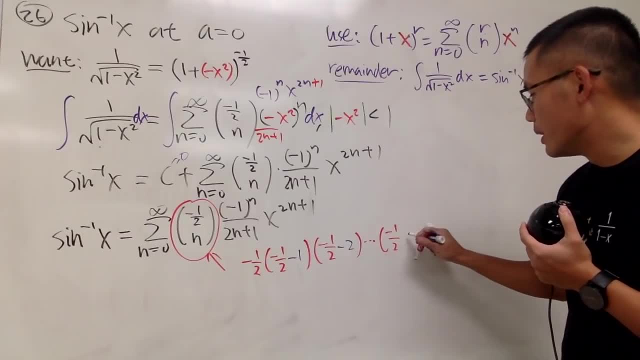 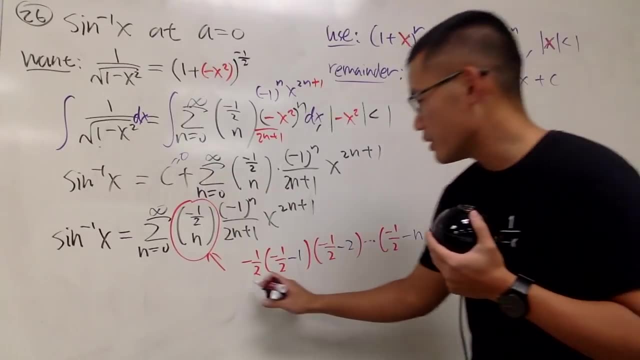 and then dot, dot, dot and then negative, 1 over 2 minus- let me just minus n- and then plus 1 after that. right, That's the definition I showed you earlier, Divided by n, factorial. okay. 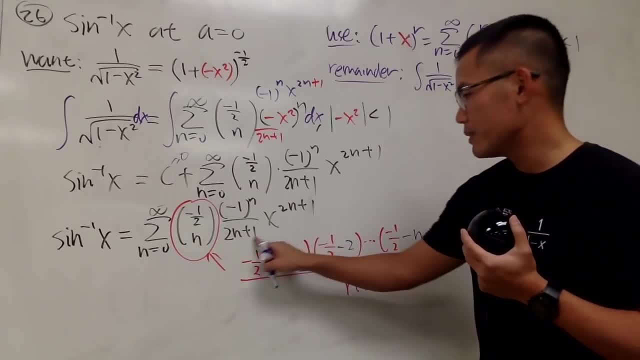 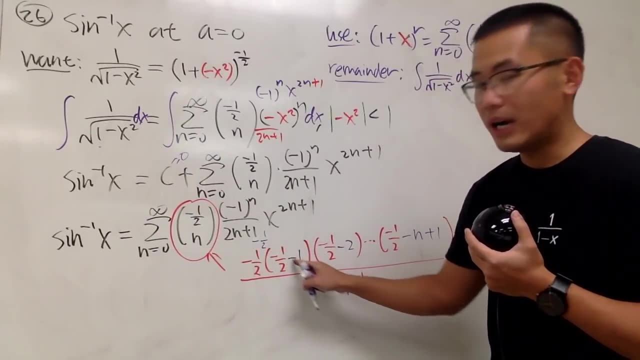 So let me see if I have enough space to work this out. I hope, I hope I do Now check this out. This is going to be negative 1 half for the first term, And this right here, if you add: 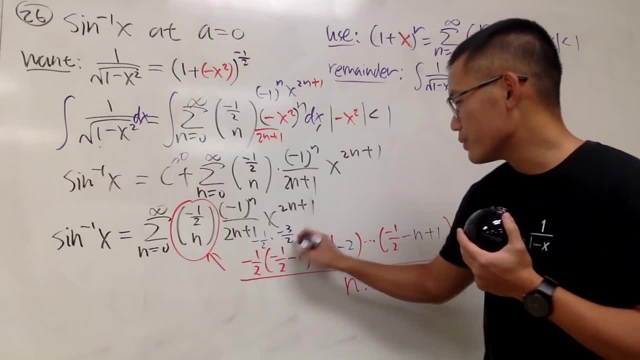 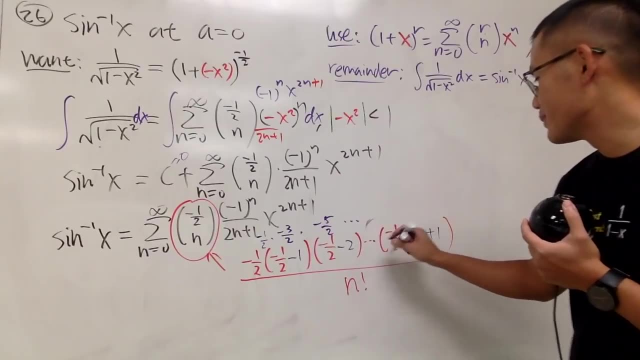 subtract the fractions, combine the fractions, you get negative 3 over 2,. okay, And for the next one, you get negative 5 over 2, and dot, dot, dot, dot. yeah, right here. Now, of course. 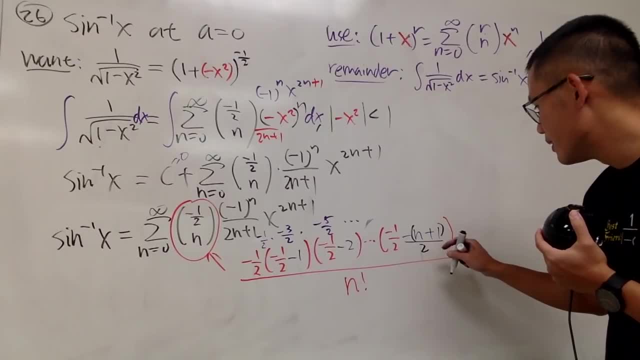 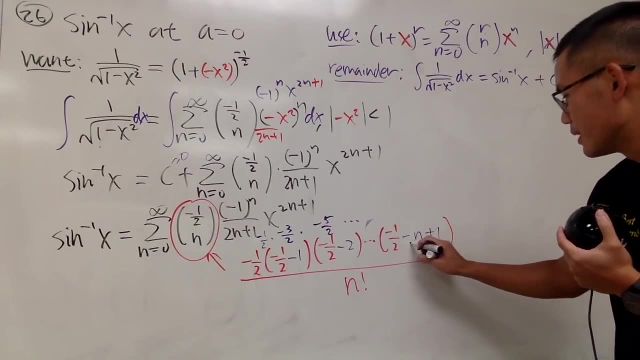 multiply this by 2, and no, it's, it's like by 2, and this. there was no parentheses, so I should, I should do this. I should do this: Multiply this by 2 and 2,. 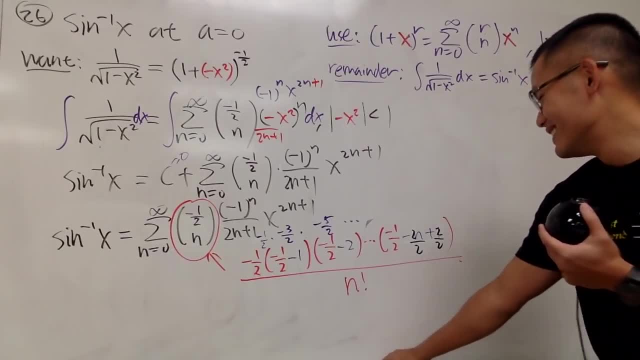 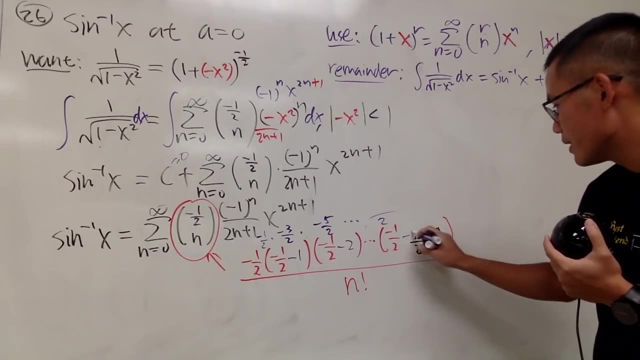 and then 2 and 2, so yeah, Power series, power series, man, Everybody has a 2.. On the top here. okay, let's see On the top here. okay, let's see On the top here. 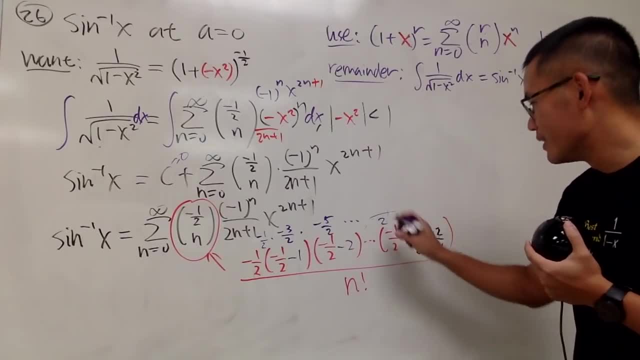 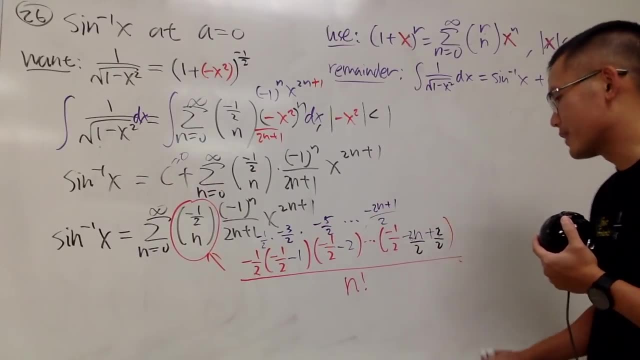 negative. 1 plus 2 is 1, so we have 1, but this is a minus 2, so it's minus 2n plus 1.. So here are your factors and all that stuff. okay, over n factorial. 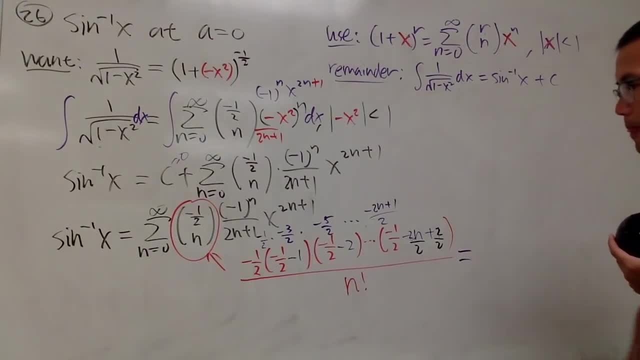 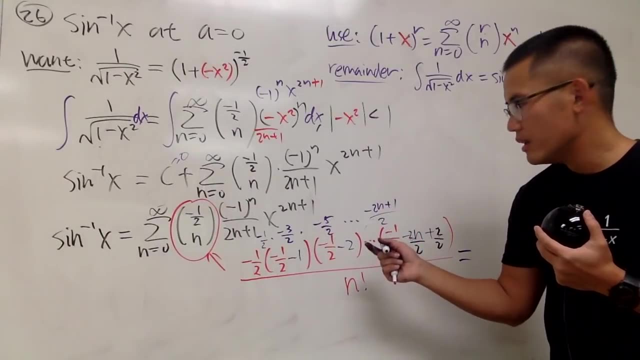 Now we're going to break this down more. Notice on the top is negative 1, negative 3,, negative 5, and so on, so on, so on. How many terms do we have, In fact, on the top? 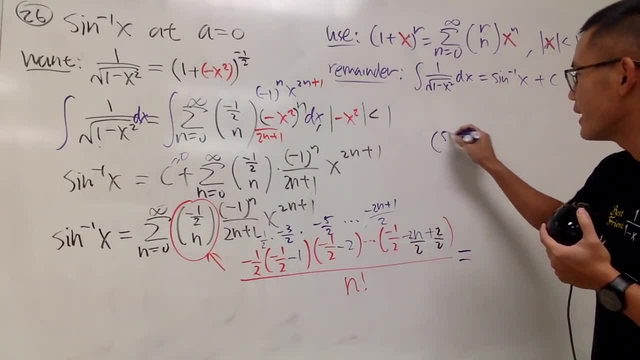 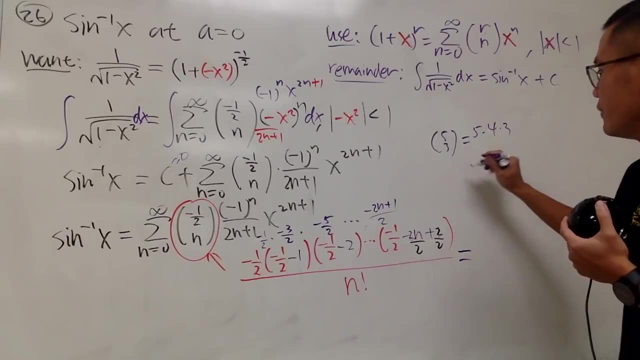 you also have n terms, just like the equation, the example of: let's say, 5, choose 3.. When you have this, you do 5, and then you write down a total of 3 terms right here. If you have 10, choose 6,. 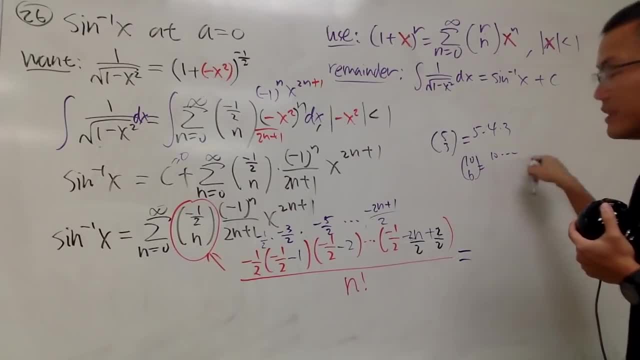 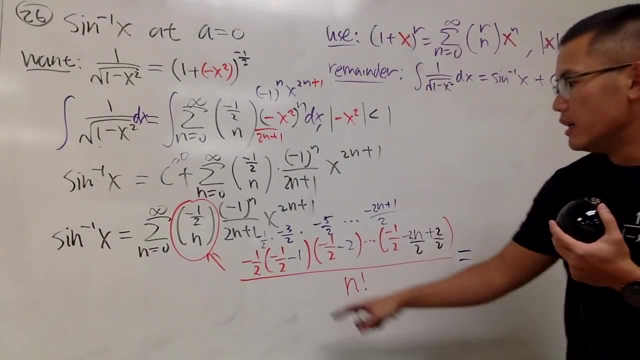 you will have 10, and then you have 6 numbers. So the truth is on the top. you also have n terms. So here's negative 1.. Everybody has a negative 1.. This right here. I can have a negative 1 as well. 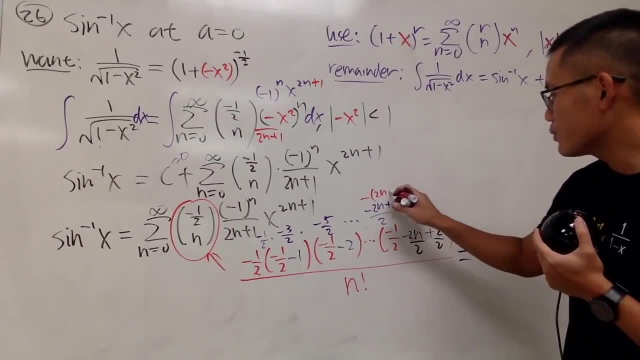 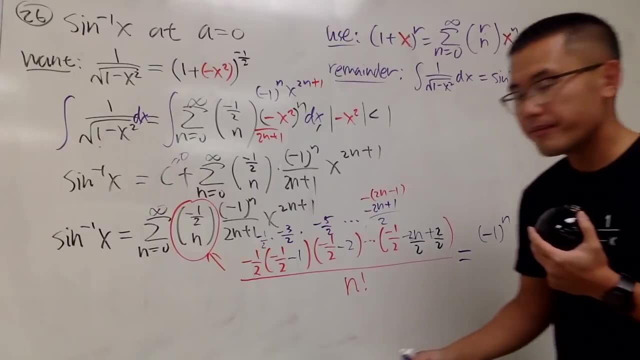 Look at this as a negative: parentheses 2n and minus 1.. So you have a negative 1 right here as well. Therefore, I will have a negative 1 to the nth power for that, And then we will have: 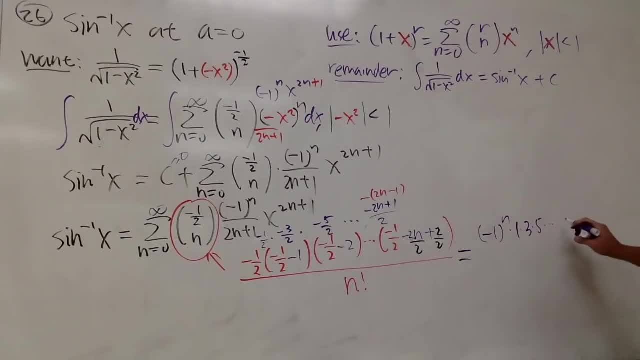 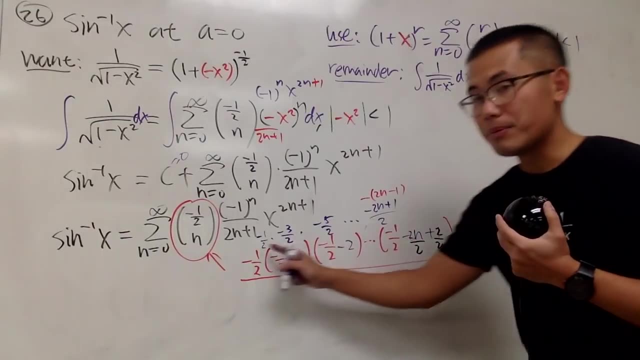 1,, 3,, 5,, dot, dot, dot up to 2n minus 1.. So that's like this: And then everybody has a 2 on the bottom, so we have the 2 to the nth power on the bottom. 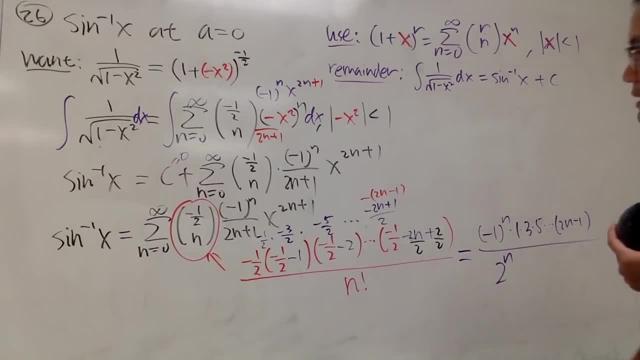 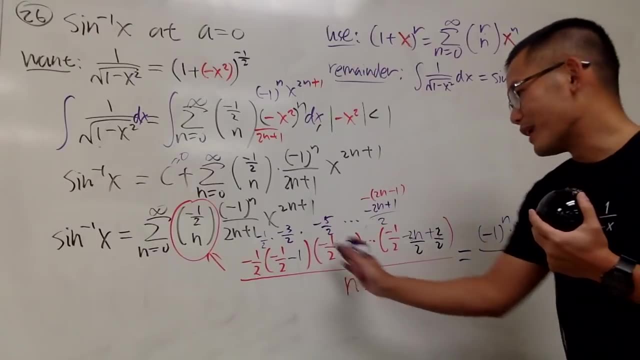 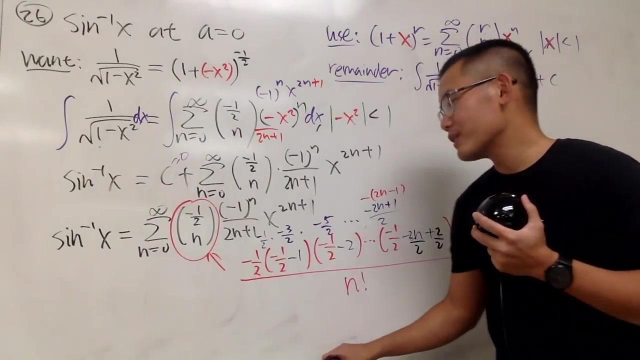 So this right here is 2 to the nth power, And then we have this which is n factorial Right. So all this right here is to show you. this right here is the same as that, Okay, So. 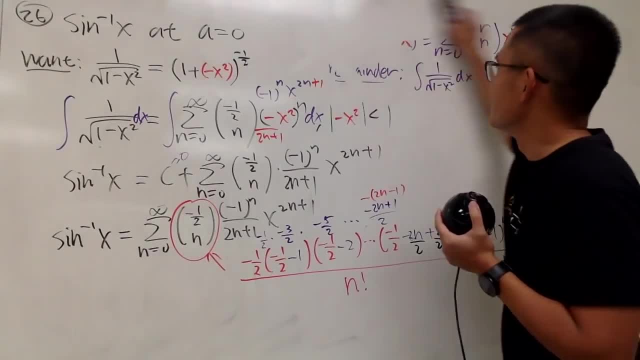 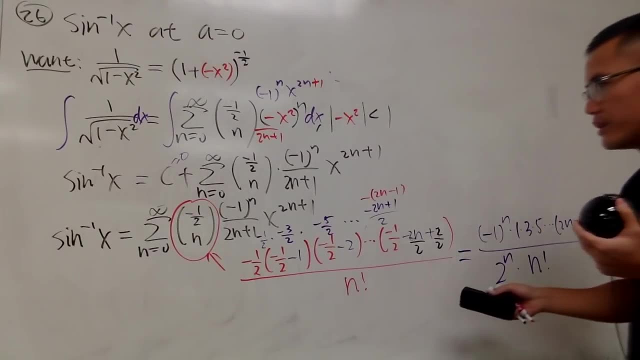 that's what we have And if you want, you can continue. I will continue, because it's making me mad for this question. I was trying to figure it out but like, yeah, I did and I will try to read this down for you guys, nicely. 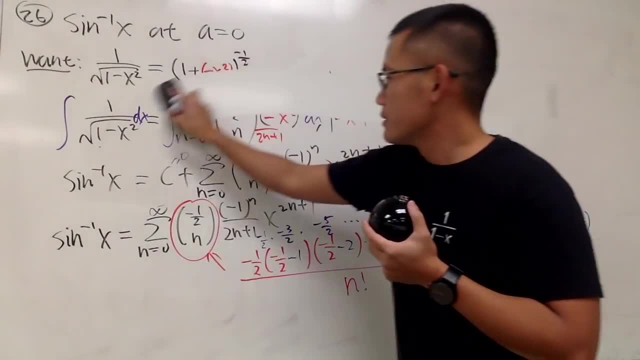 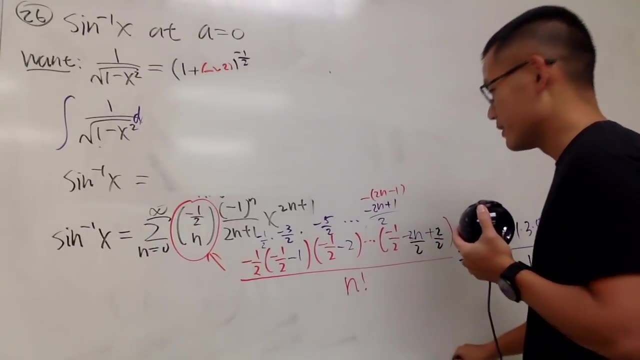 Let me see I need to have enough space. By the way, r is 1.. So just do that, okay, Just check the answer for that. I'm not going to do that. I'm going to conquer this guy. 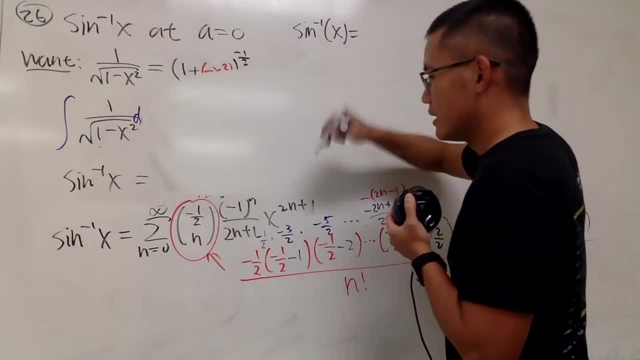 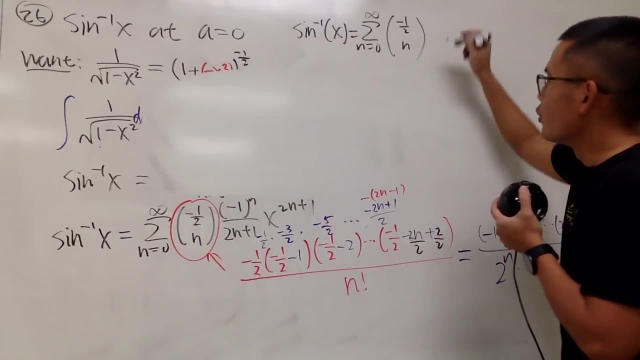 So here we go. This is sine inverse of x. This is the sum that goes from 0 to infinity. I believe if you write the answer down like this, nobody can be mad at you. Seriously, Seriously, okay, But 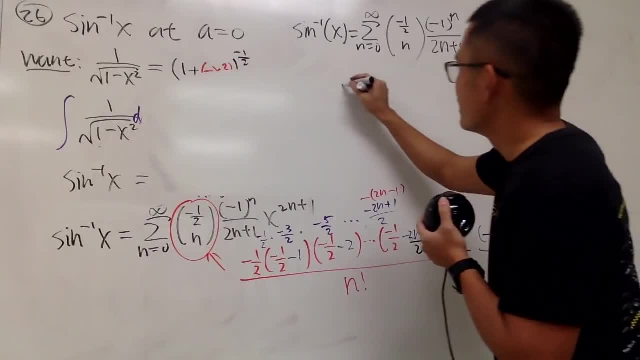 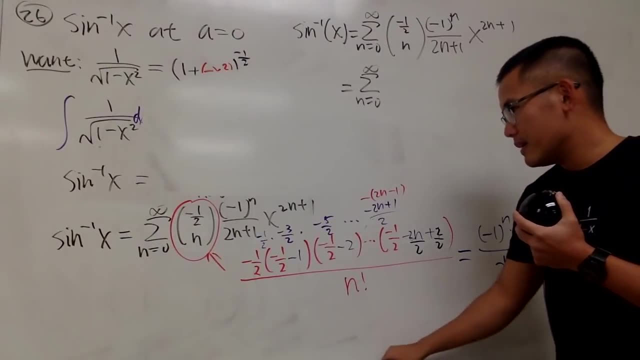 if you want to simplify it more, here is how you can do it. This is the sum that goes from 0 to infinity. Now, here we go. I will put all this down right here, and that's one of the answers that I have. 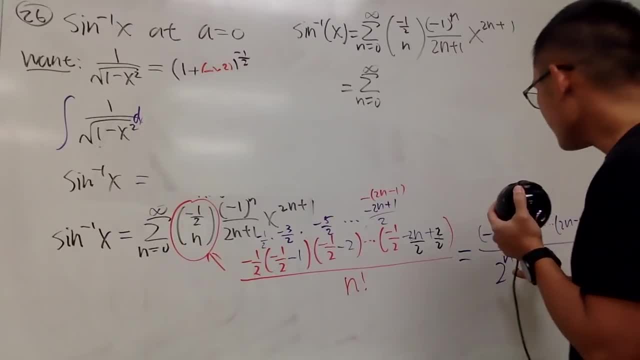 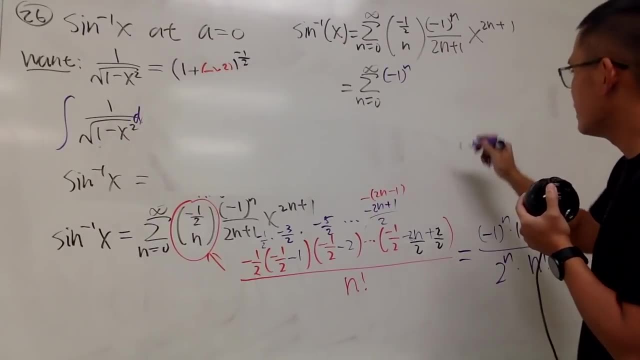 and this is actually the answer from the textbook, I believe. So I will just put this down right here. so we will have this, which is negative 1 to the nth power, and then all that, So it's 1,. 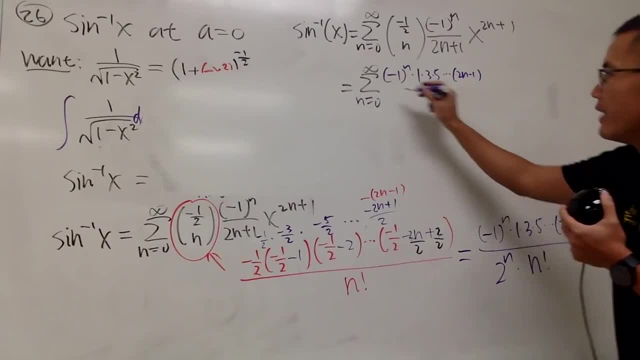 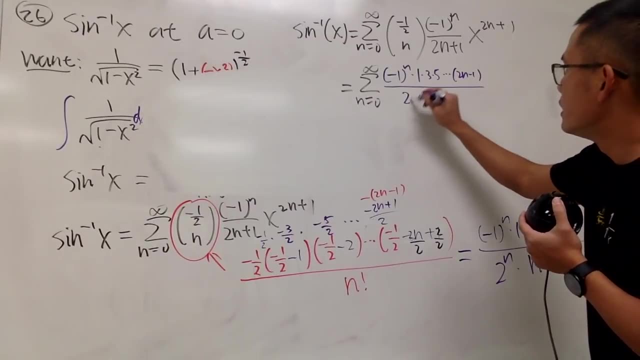 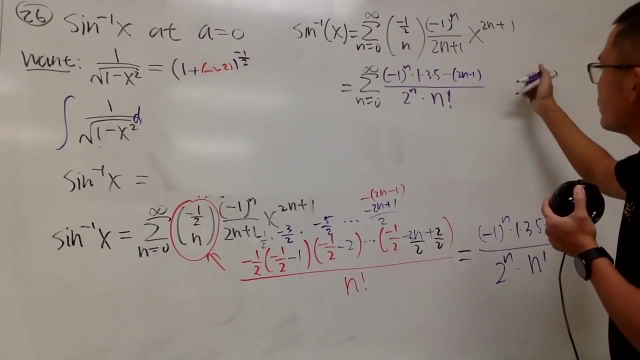 3, 2n minus 1, okay, And then on the bottom here we have 2 to the n times n factorial, okay. So that's for this one. Notice that we still have this part which is: 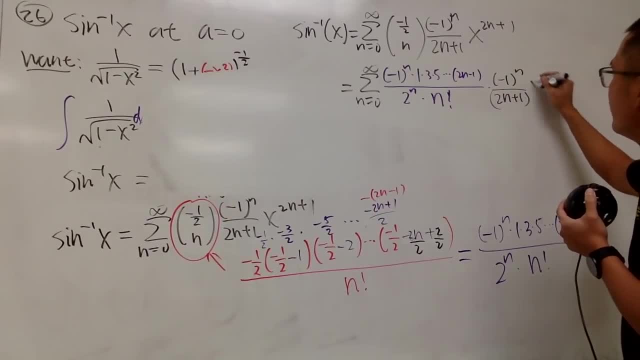 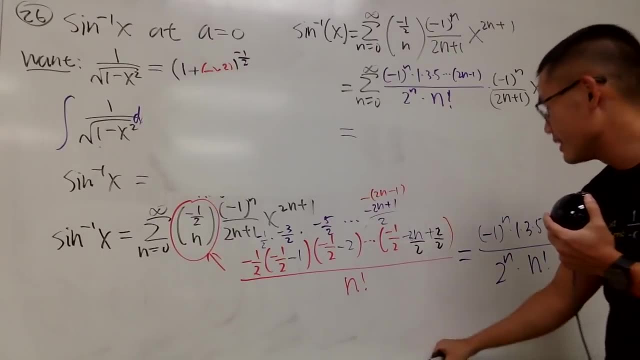 negative 1 to the nth power over 2n plus 1, and then x to the 2n plus 1th power. okay, So that's what we have: Negative 1 to the n times. negative 1 to the n. 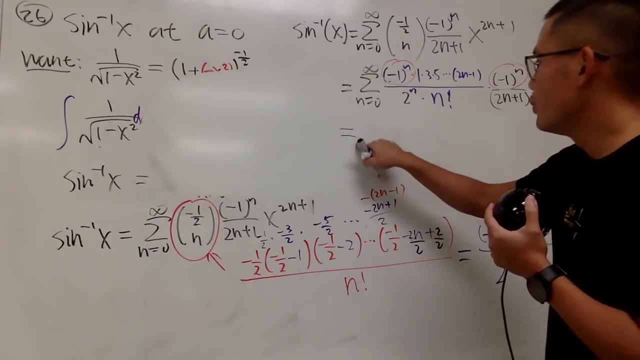 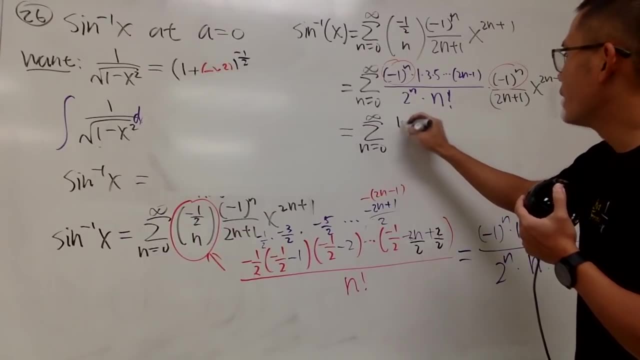 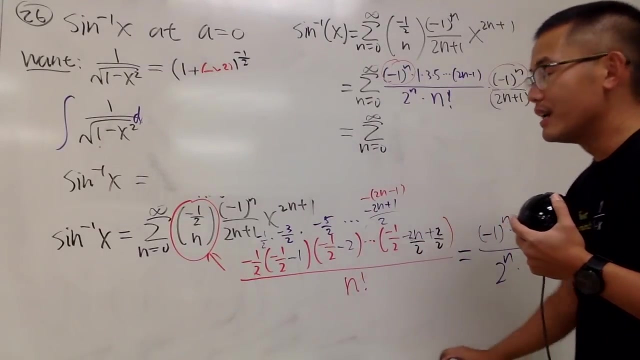 is just negative. 1 to the 2n. That means everybody will be positive. So you end up with this. This is the sum, as n goes from 0 to infinity, and you just get 1 times 3 times 5. 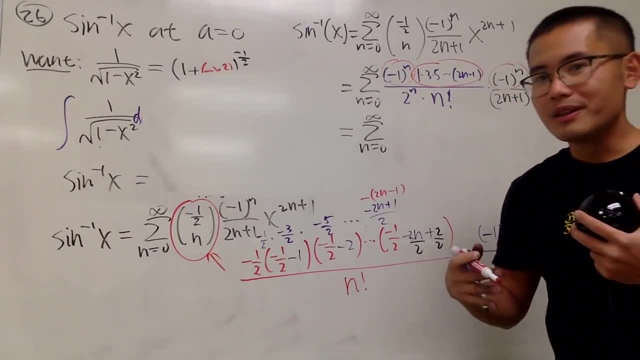 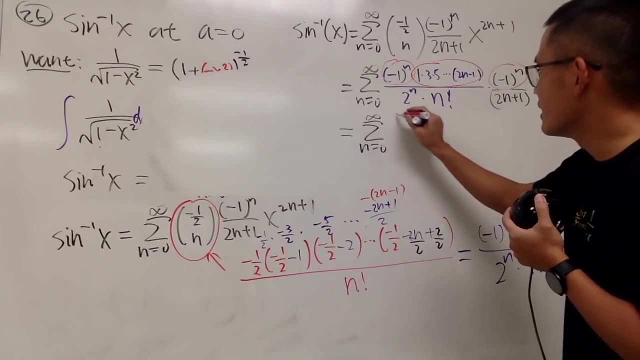 times all that stuff, But I'm going to tell you guys what all that stuff is. What this is right here is this: This is an odd number, so what you can do is you can write this down as 2n minus 1. 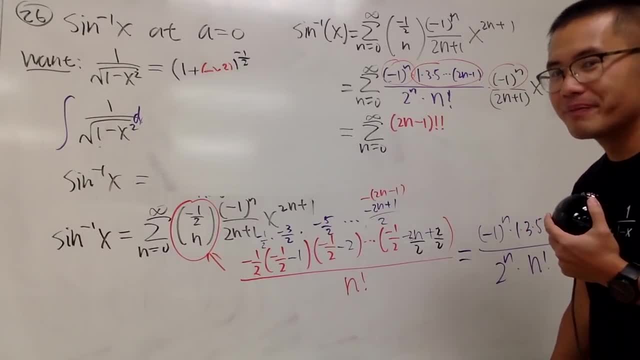 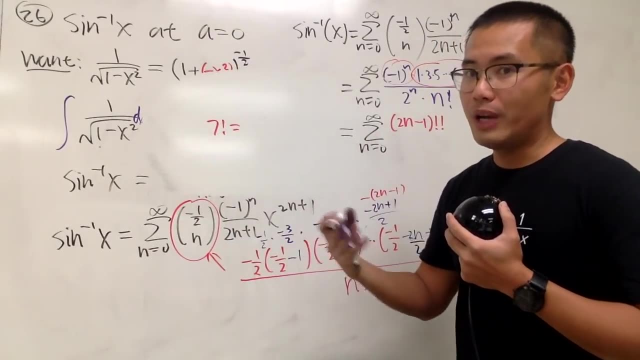 factorial, factorial, that This is called the double factorial. Quick example: It has to be an odd number inside. In that case you get, let's say, 7 factorial. You just go down by 2. every single time All these numbers are odd. 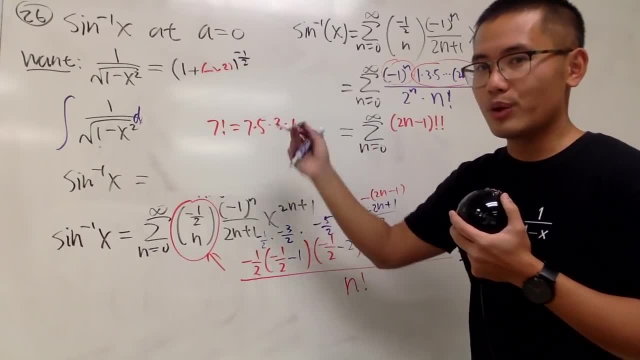 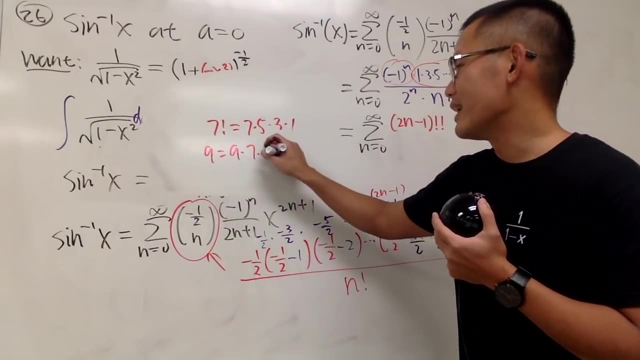 So you, for example, 7 factorial, 7,, 5,, 3, 9 factorial is of course 9, 7,. yeah, I lost creativity right now. Oh sorry, double factorial, double. 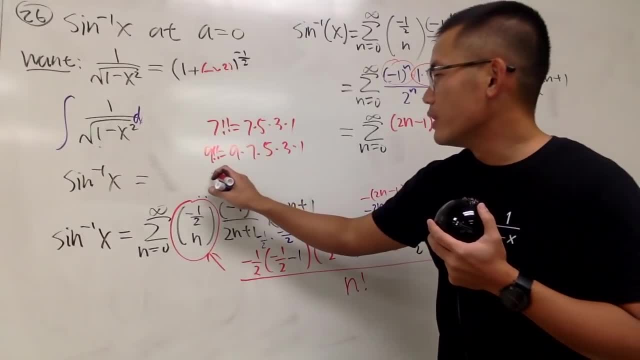 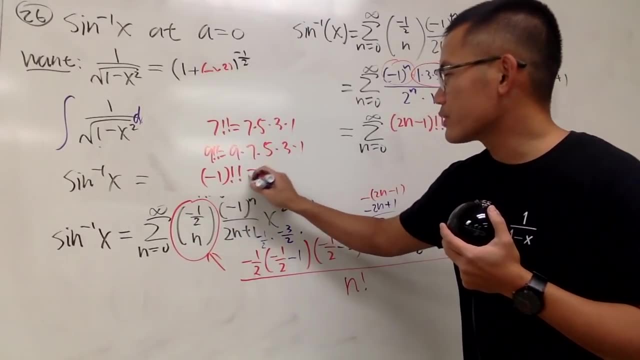 double factorial. okay, And with this notation, you have to be careful. though You can prove so, you cannot. you can use the definition negative: 1 double factorial is actually 1,. okay, I will do a video for you guys. 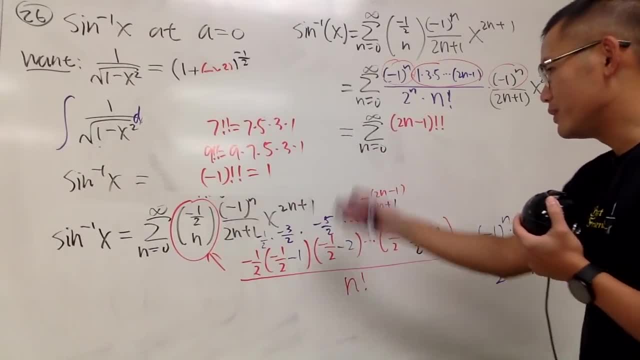 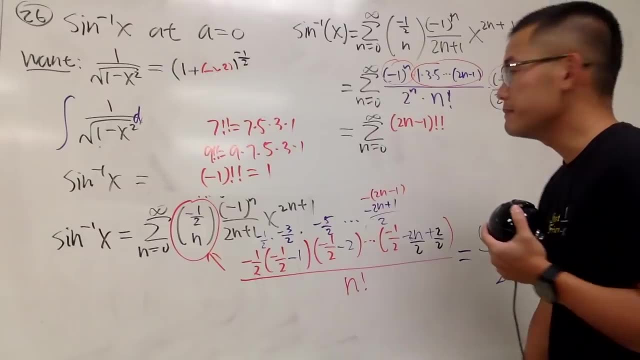 if you like, Negative 1 double factorial by definition is equal to 1, so when you're putting 0 here, you end up with negative 1 double factorial: it's 1, right. So again this right here. 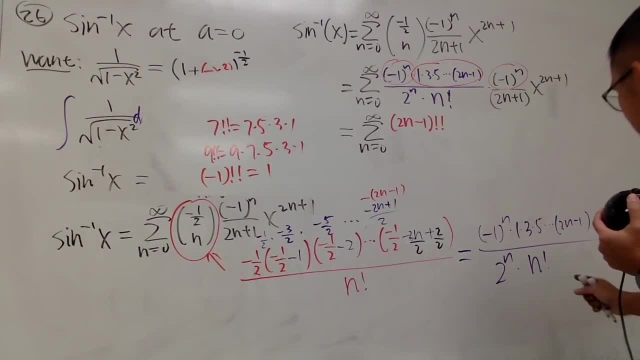 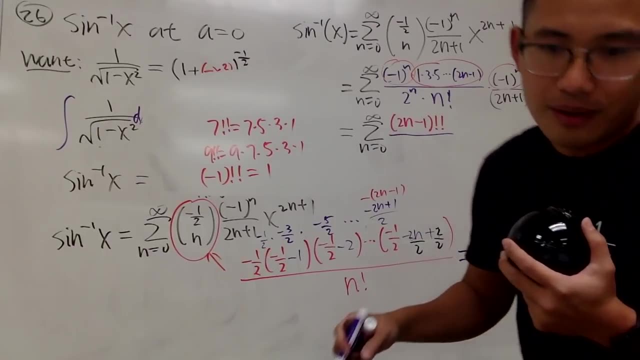 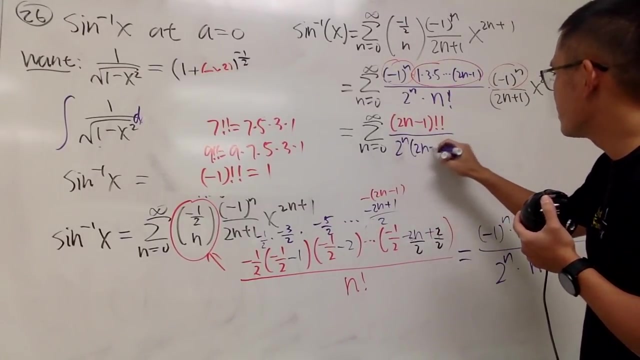 just merge it into 2m minus 1 double factorial and then this guy on the bottom we have over, and I believe the textbook answer is yeah, it's just this. So we have 2 to the n and 2m plus 1. 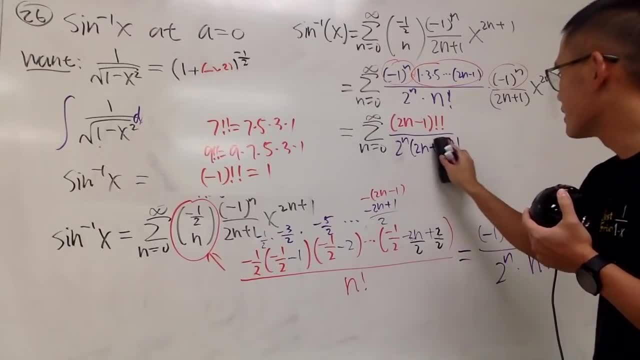 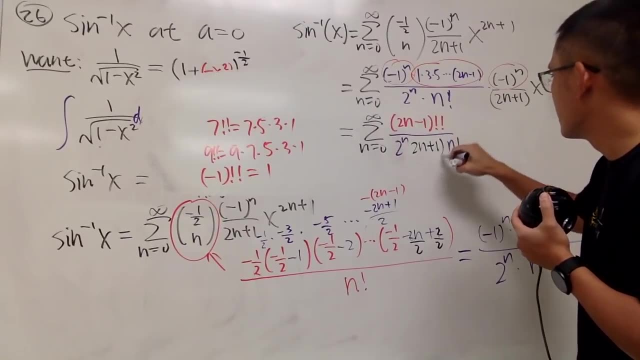 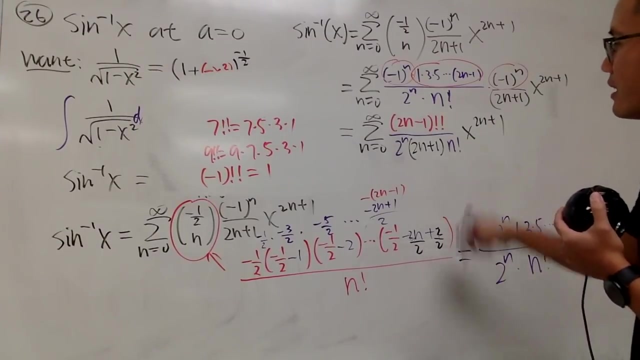 and then n factorial. So it's like this: and now we'll have the this in black- 2m plus 1, and we still have that x to the 2m plus 1.. So this is totally okay again. 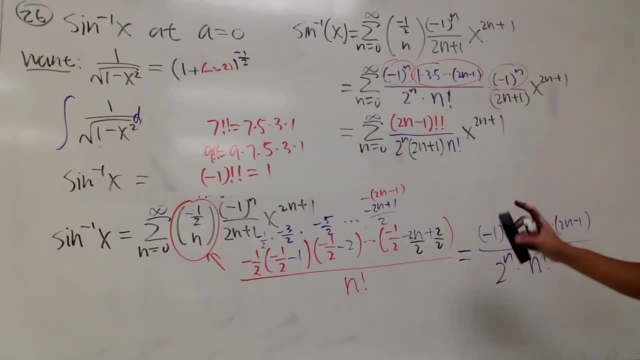 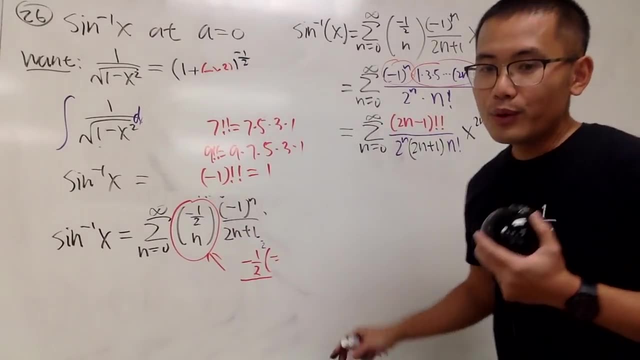 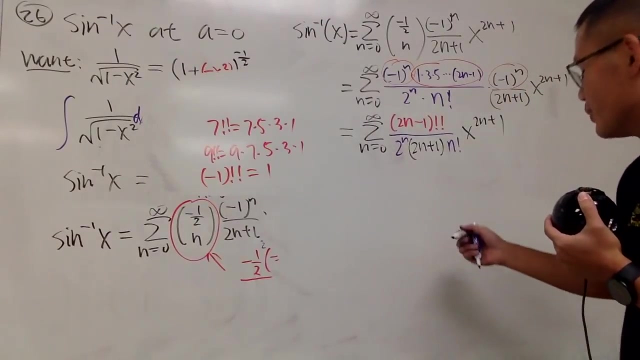 right. So again, look at this, look at that and look at all this. Now, if you want to simplify more- which I have another one for you guys- if you want to simplify more, the truth is this is 2n. 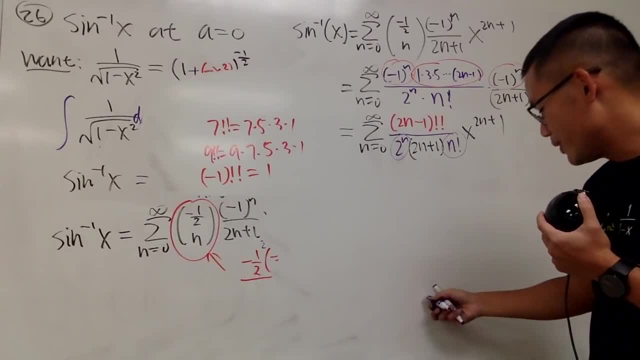 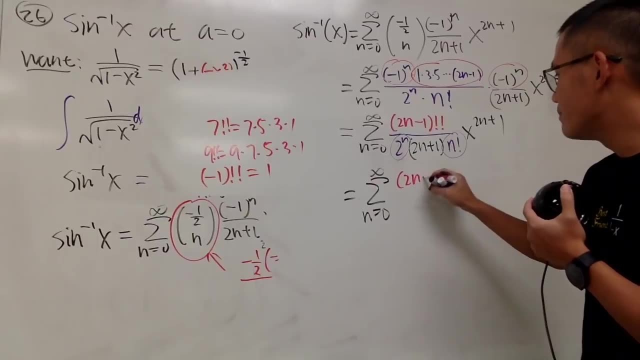 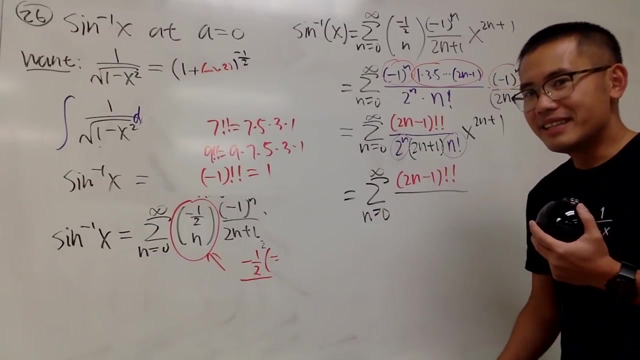 2 to the n times n factorial. You can write it down like: the sum n goes from 0 to infinity. On the top is 2m minus 1 double factorial and then on the bottom this and that is the even double factorial. 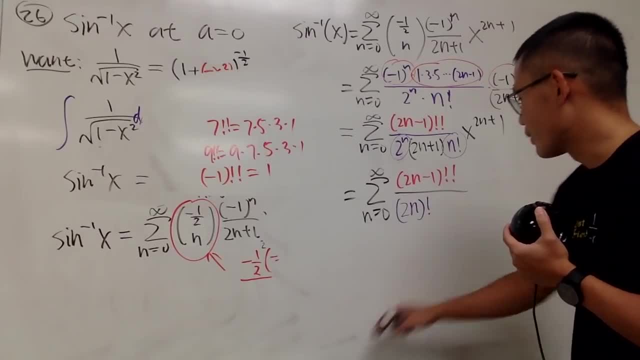 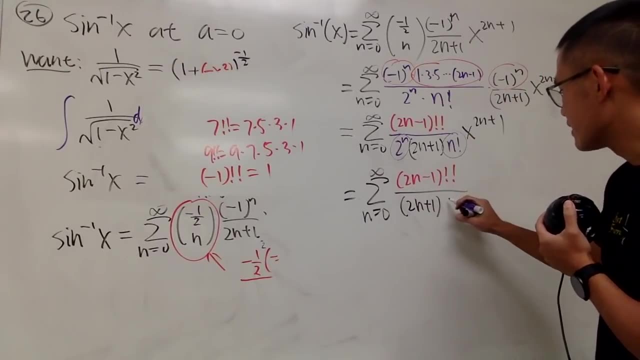 So it's 2n double factorial and because I have the factorials, I will actually write down this: first, 2m plus 1, and then this, and that together becomes the 2n double factorial and then you have the x to the. 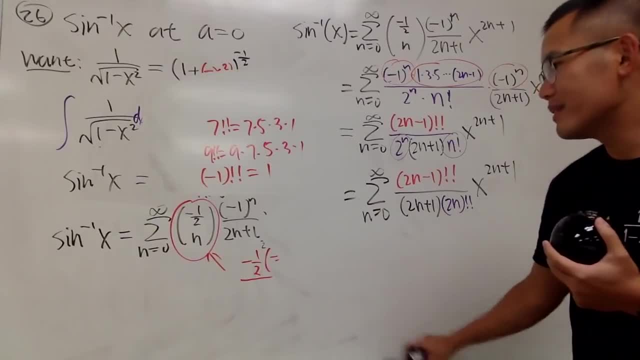 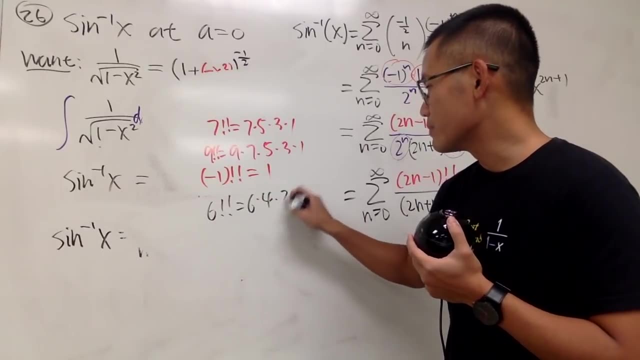 2m plus 1's power Man, and then for the 2n factorial, what you do is well, it's just, let's say, 6 double factorial, it's just 6 times 4 times 2. 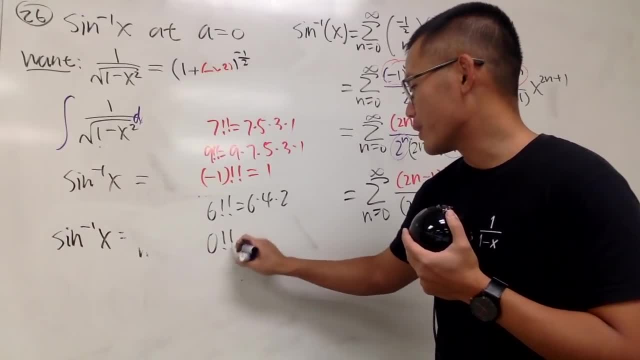 and you stop. You don't go to 0 and work that out. 0 double factorial equals 1.. I have another video. you guys want to check that. I have that for you. So this is by definition. and then 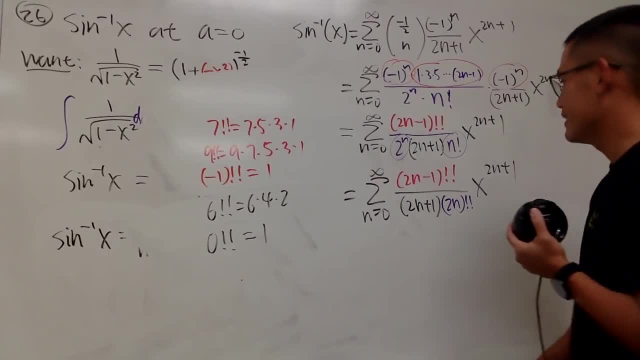 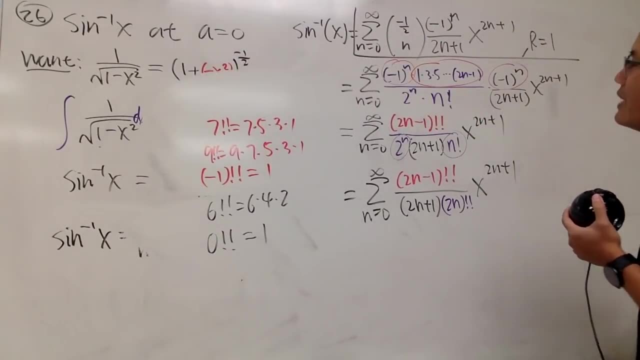 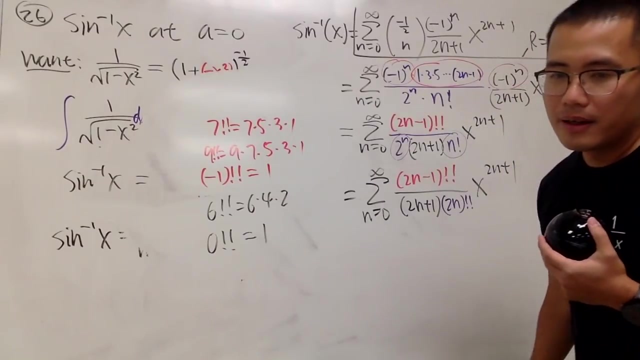 the other one, just how you do it. So why don't we just stop right here? I really don't know. r is equal to 1, and let's see what's my radius of convergence. Oh yeah, the. 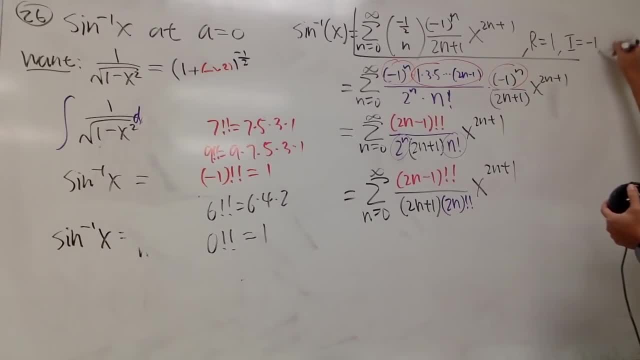 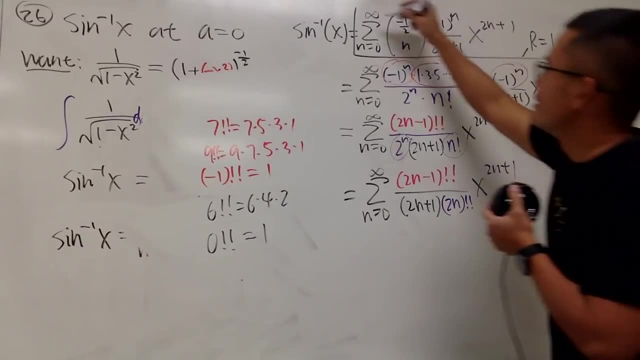 well, I will let you guys tell me what's the, what's the interval of convergence, right here, right? So I did enough of this. You guys leave a comment down below, okay? So this is number 26.. 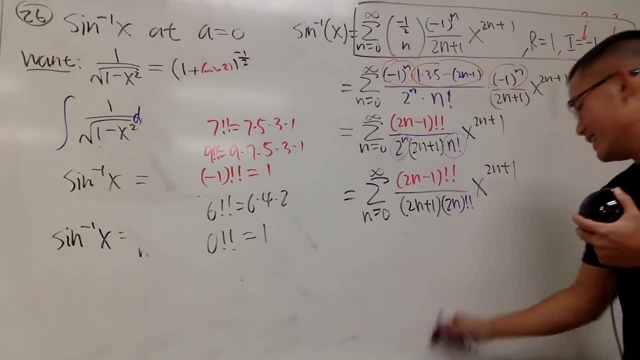 So have a look. So that's it. Wait, that's it Or that's it. So depends on how you want to present your answer Up to you right Now. I will just write down the last one. 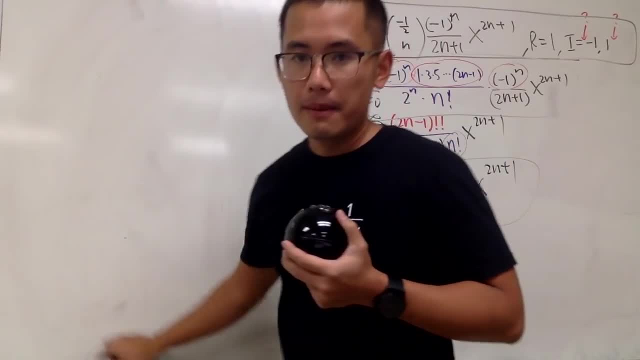 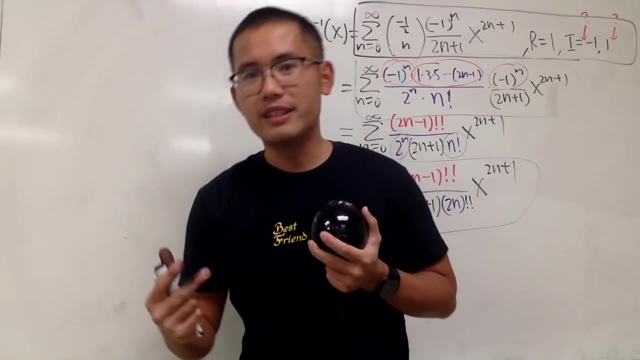 for you guys here. Now you guys know, after you finish the marathon, the worst part is not the 26 mile, it's the last 0.2 mile. okay, So here is the last 0.2, 26.2.. 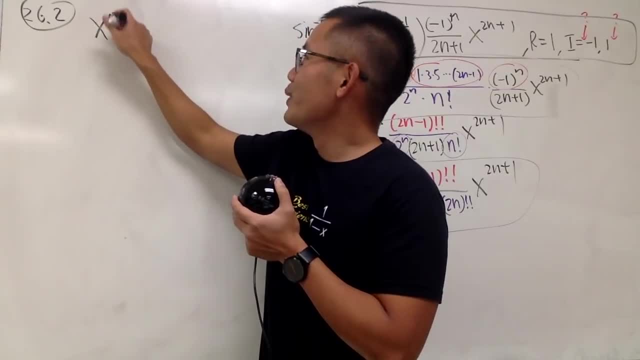 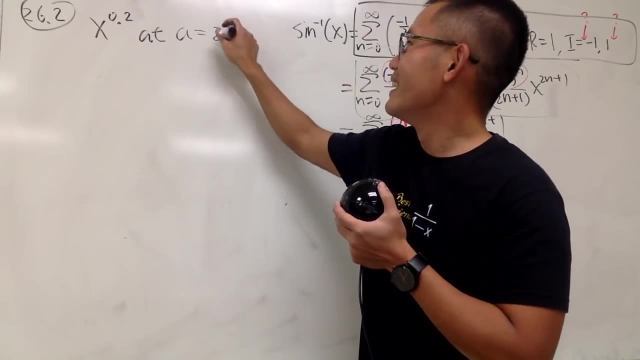 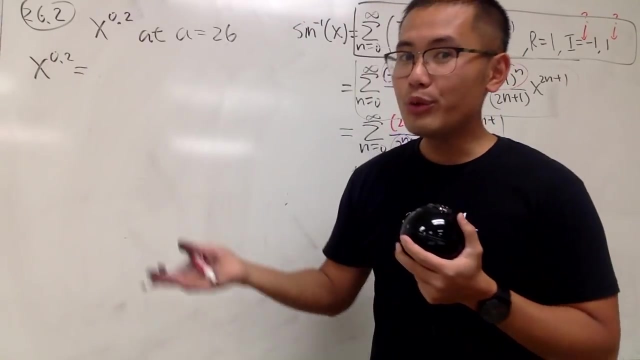 And here I have x to the 0.2 power at a equals 26.. Okay, This one is actually go pretty quick. Here we go: x to the 0.2.. Well, I need to have a what factor x minus 26.. 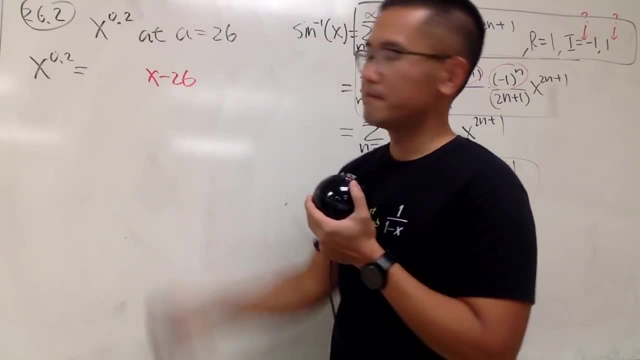 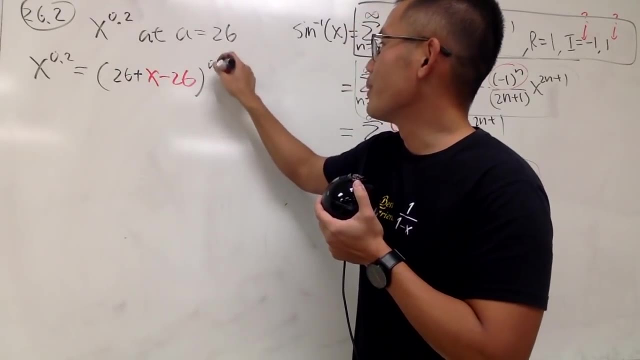 So let's look at this inside: x minus 26.. Well, this is x, So what we have to do is just add the 26 back and then raise to a 0.2, like. so Now we have the 26,. 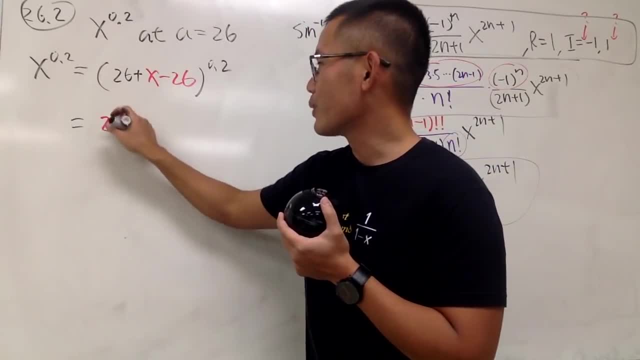 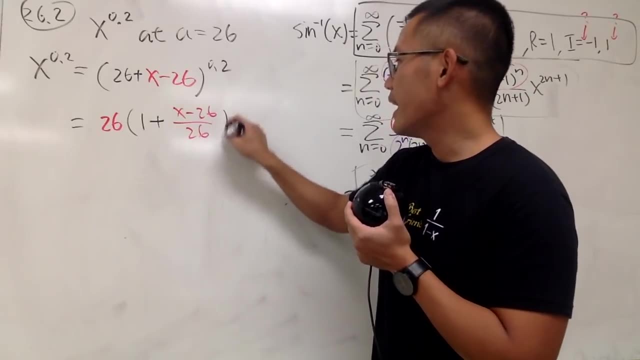 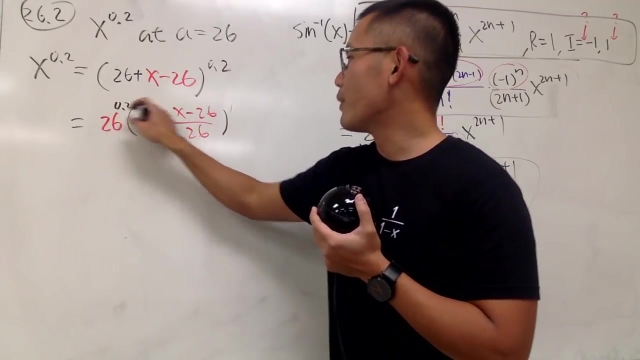 right, Just factor it out. So factor out the 26 and we have 1 plus this is x minus 26 over 26.. And then, well, you guys know, just do this in your head. okay, This is going to be raised to the 0.2 power. 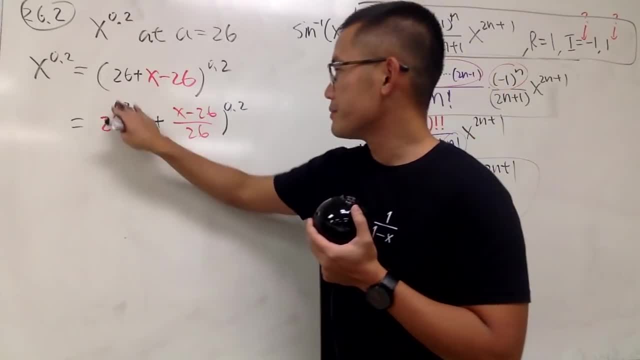 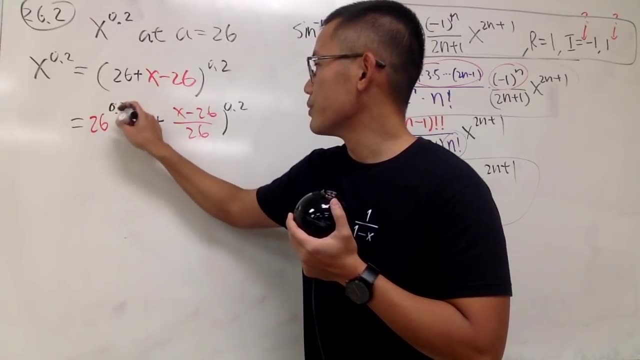 and this right here is going to be raised to a 0.2 power as well. Alright, So this is going to be. let's see, this is 26 and this is the 0.2.. I will leave it right here. 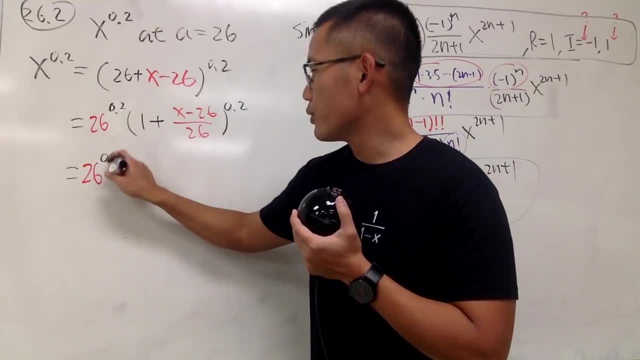 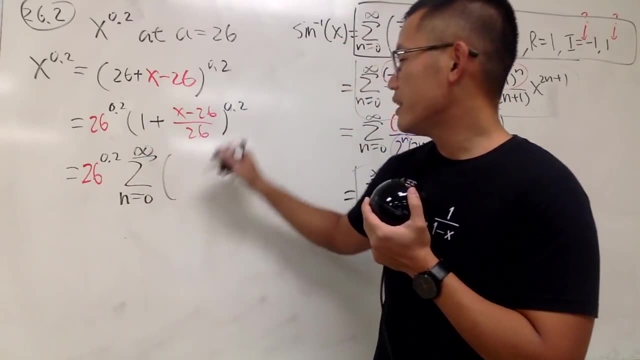 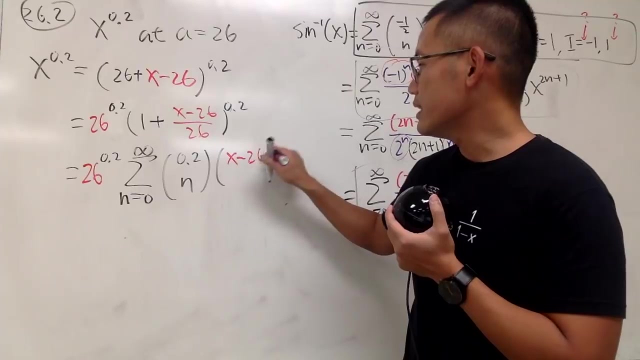 26 to the 0.2 power. This right here, use the power series Sum, as n goes from 0 to infinity. Here is 0.2.. Choose n and then the input is x minus 26 over 26 raised to the nth power. 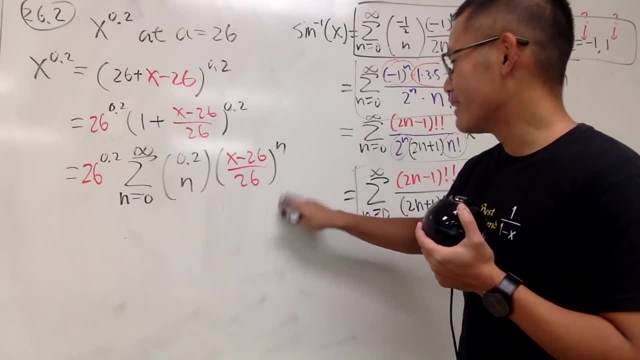 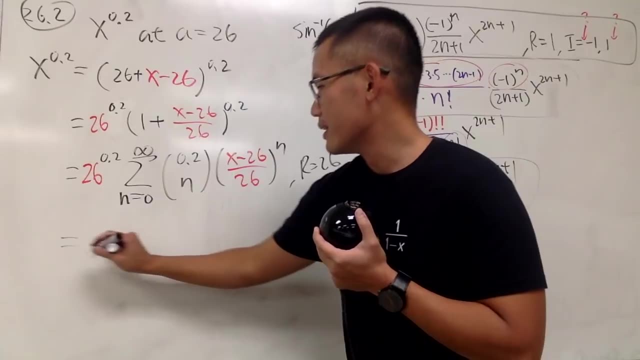 Right, And, of course, do the absolute for your order. but let me tell you, r is equal to 26.. Right Now, we just have to simplify this a little bit. We will do something in our head, okay. That's why I've done enough of. 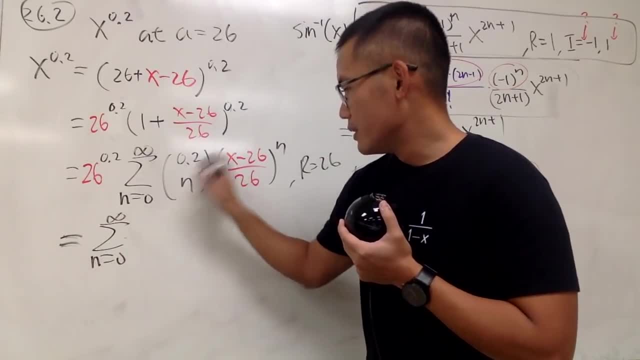 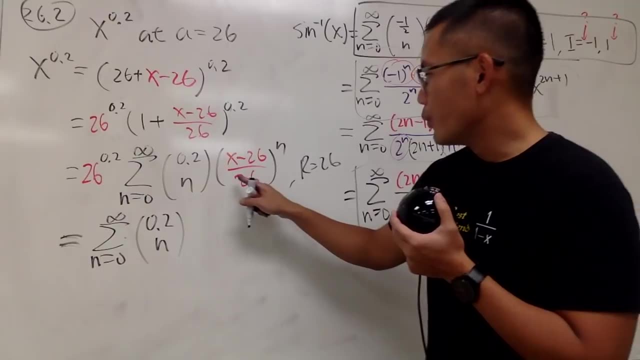 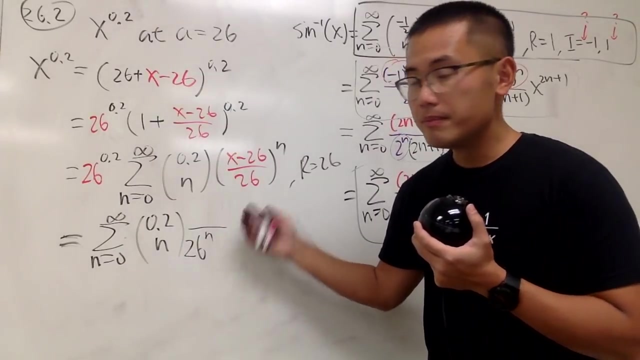 all the details for you guys already. Leave it Seriously, don't do things like that. Seriously, Leave it 0.2.. Choose n: We will have 26 to the nth power on the bottom, but then here we have the 0.2 power on the top. 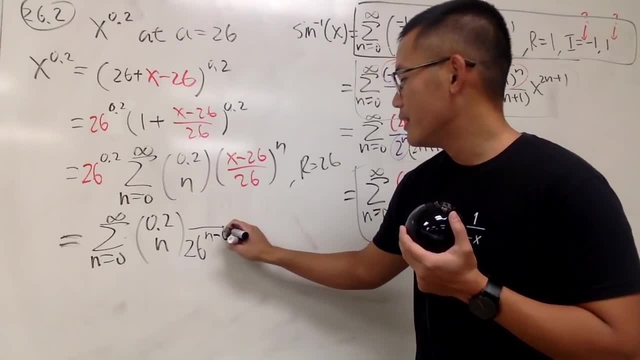 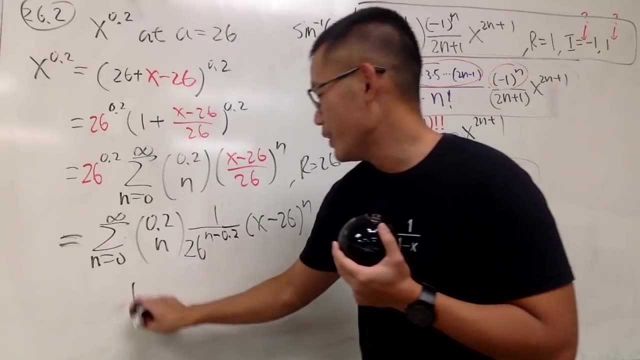 So we just have minus 0.2, and this is 1, and then we have x minus 26.. Choose nth power. Man. let me tell you we are done. r is 26 and the interval of convergence started at 26. 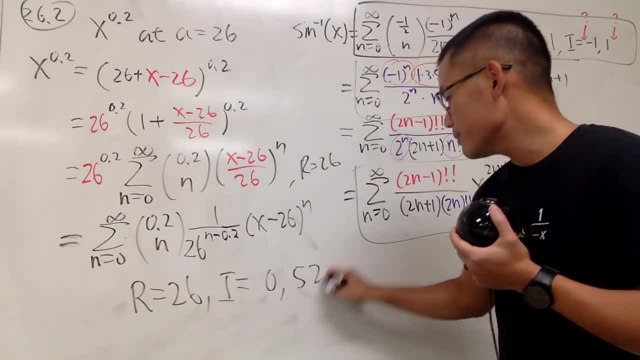 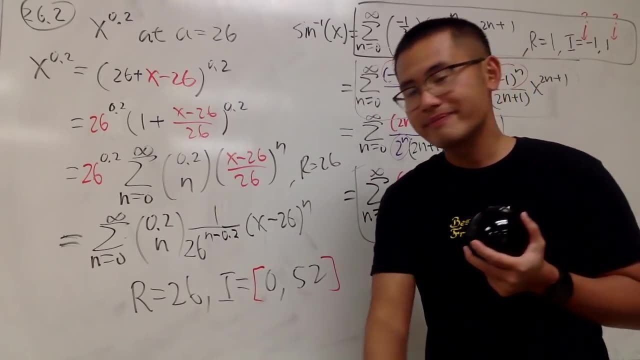 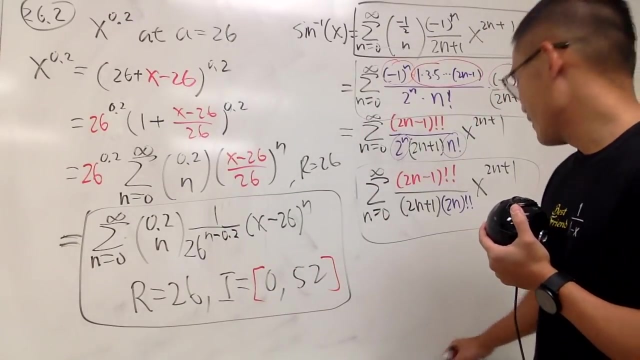 left right. So you have 0 and 52.. This is positive r right, 0.2.. So you include both and points. Oh man, This is how you finish a marathon. Seriously, You finish everything. 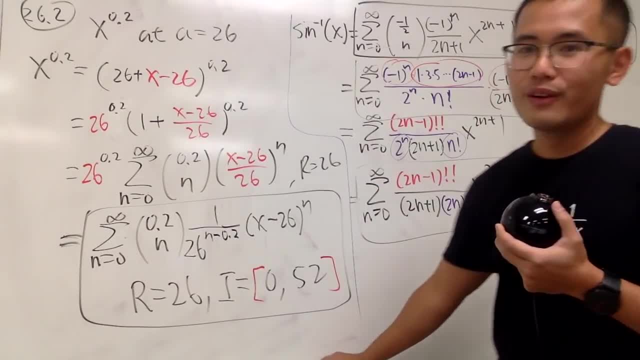 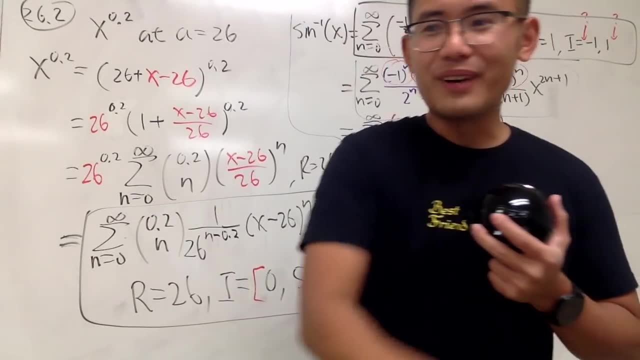 non-stop In one go. That's how you do a marathon, All right. So how long did this take me? Three and a half hour, Man. my hands are all dark because of the marker and also the dirt and all that stuff. 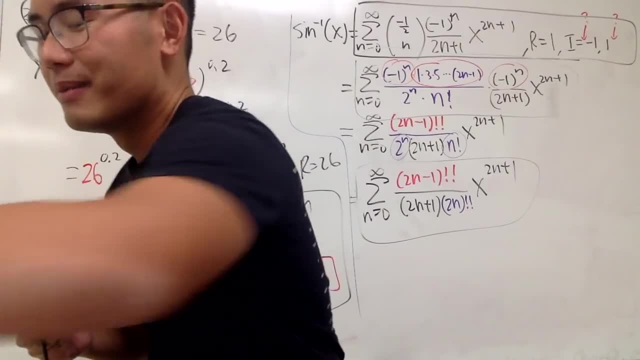 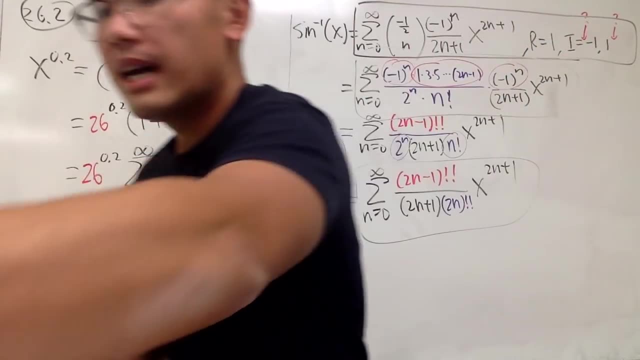 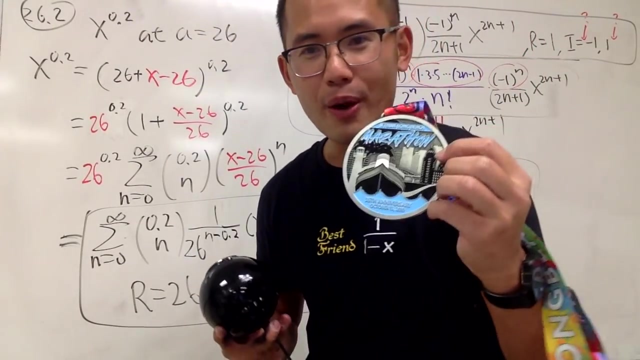 but I still would like to put on my Man. my arms are so tired. Let me drink something first. I have my marathon medal. This is the Long Beach Marathon that I just ran about like three weeks ago. Yeah, Long Beach Marathon, right. 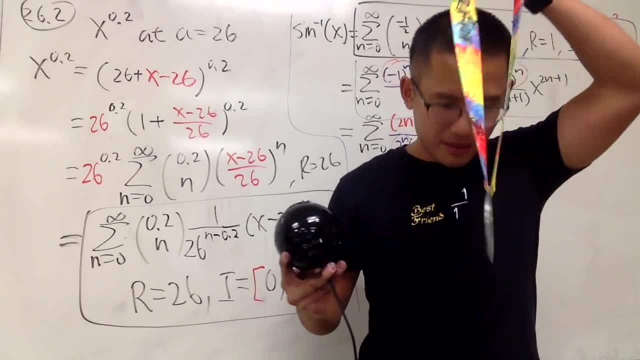 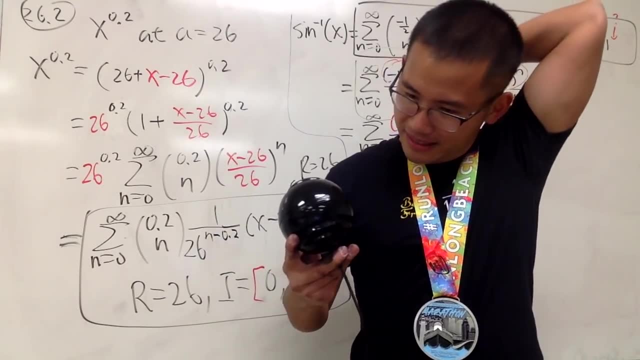 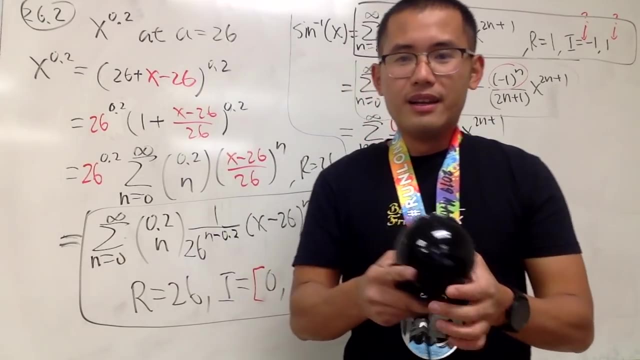 So I'm going to put this down. This is actually pretty. I don't want to. I didn't want to touch my medal with my left, my right hand because it's dirty. as you can see, I messed up, but oh well, Let me show you.